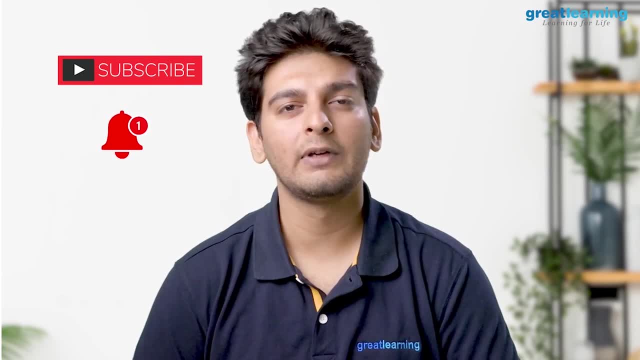 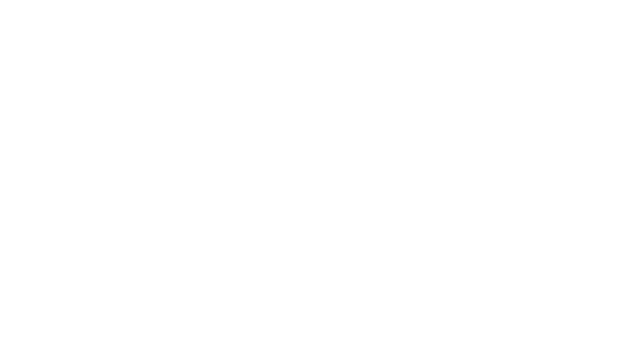 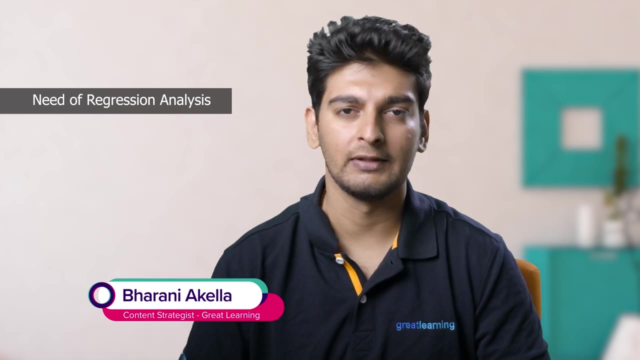 Great Learning's YouTube channel and click on the bell icon so that you have a notification of our upcoming videos. Now let's have a quick glance at the agenda. We'll start off with the case study, where we'll understand the need of regression analysis. Then we'll have a brief 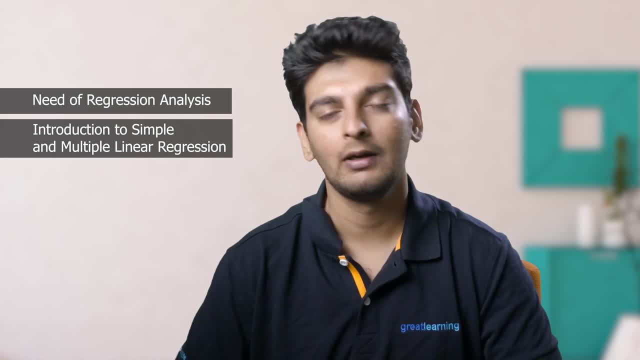 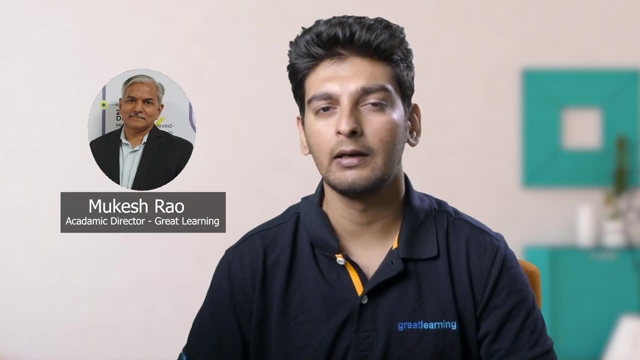 introduction to simple linear regression and multiple linear regression. After that, we'll have a demo in both Python and Python, Our languages. going ahead, we'll have Professor Mukesh Rao, who is the academic director at Great Learning, explaining all the concepts of linear regression comprehensively. Professor Mukesh Rao. 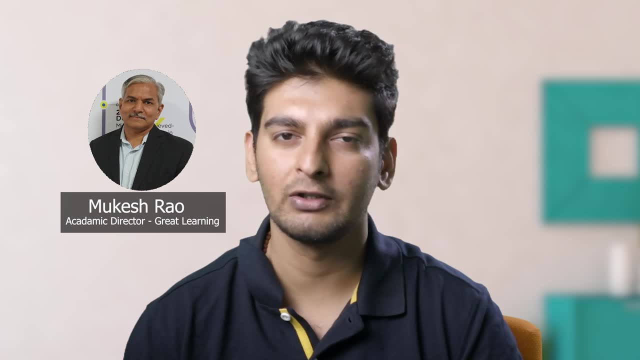 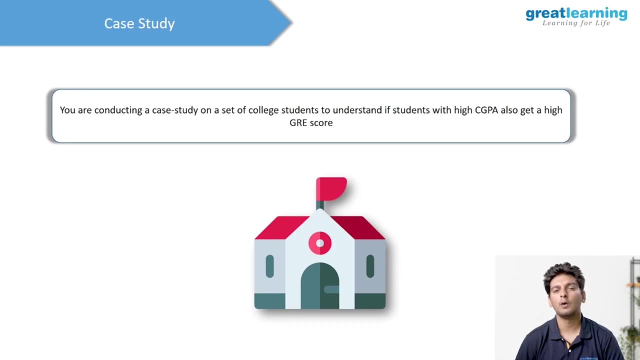 has over 20 years of industry experience in market research, project management and data science. So let's start off with this case study. Now. let's say you are connecting a survey on a bunch of college students and you'd want to understand if there's a relationship between 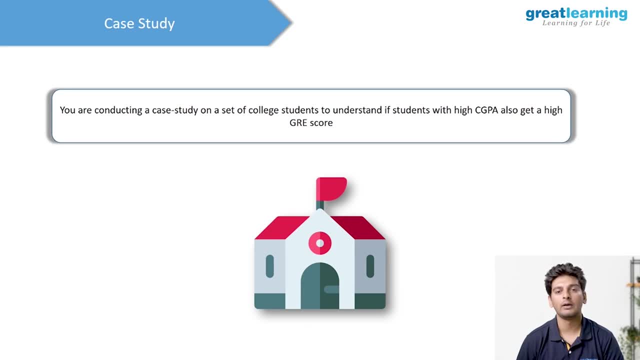 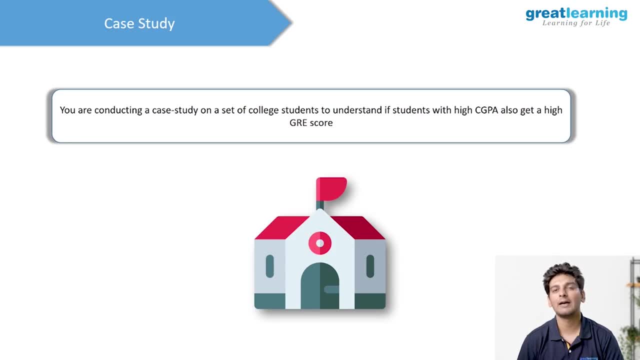 also tend to have a higher GRE score and, similarly, if students have a lower CGPA, then would they have a lower GRE score. So this is the problem statement. Now, to find out the solution for any problem, you need to gather data. So that is what you go ahead and do. So let's say, you go to around 500 odd. 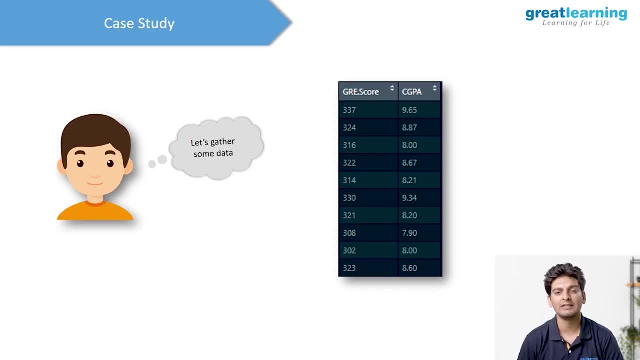 students and ask them their GRE score and also ask them their CGPA, and then you create a table out of this. But if you just look at this table, would you be able to draw any sort of inferences from this? Obviously no. So this is where you do. 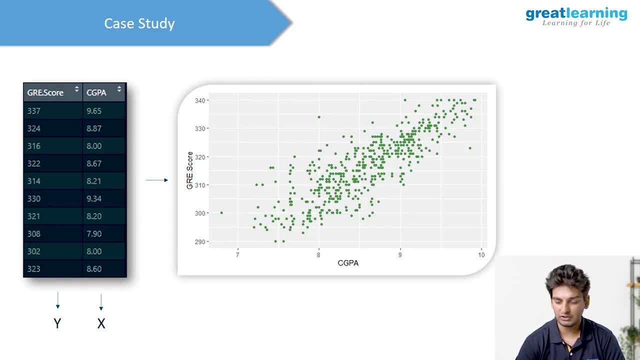 some sort of data visualization. So over here, you've got this GRE score and you've got the CGPA. Now what you'll do is you will map the GRE score onto the y-axis and you'll map the CGPA onto the x-axis and you'll build a scatter plot for these two. And as soon as you build this graph, you can 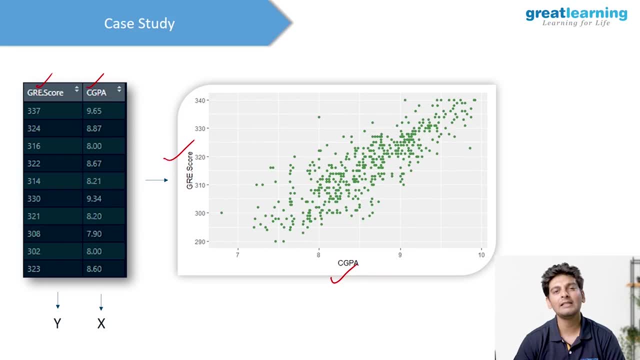 clearly draw inferences. So what you understand is, as the CGPA of the student increases, the GRE score increases. So there's sort of a positive linear relationship between the CGPA of the student and the GRE score of the student. So with this you can clearly state that if a student has high CGPA then he'll have a 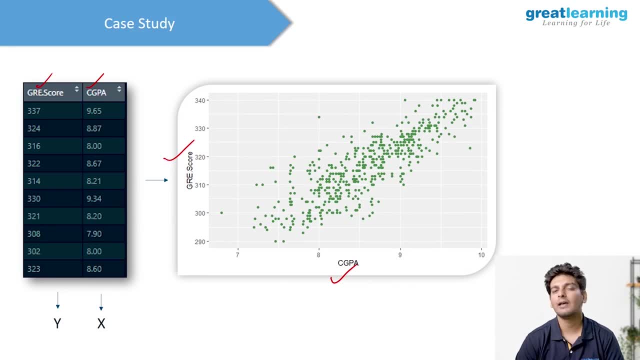 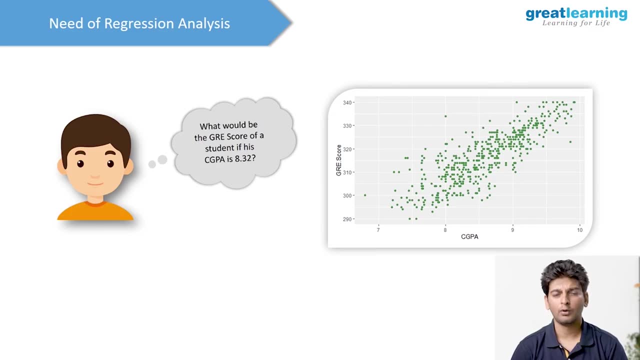 high GRE score. Similarly, if the student has a low CGPA, then he'll sort of have a low GRE score. Now, this inference was quite easy to draw from this visualization. Now what if I actually change the question? So let's say, if I ask what would be the GRE score of the student and what would be the 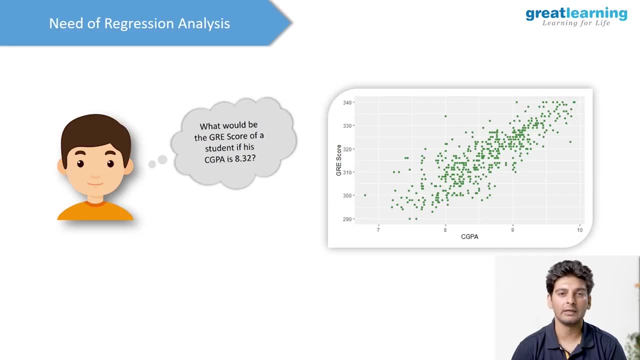 score of a student if his CGPA is 8.32.. Now, if you just look at this graph over here and if I say that the CGPA is 8.32, would you be actually able to tell what would be his GRE score? Now that would. 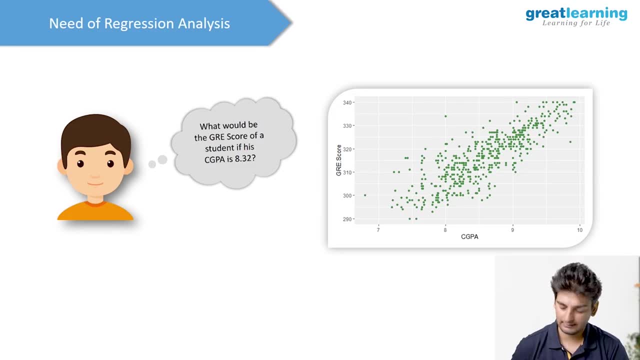 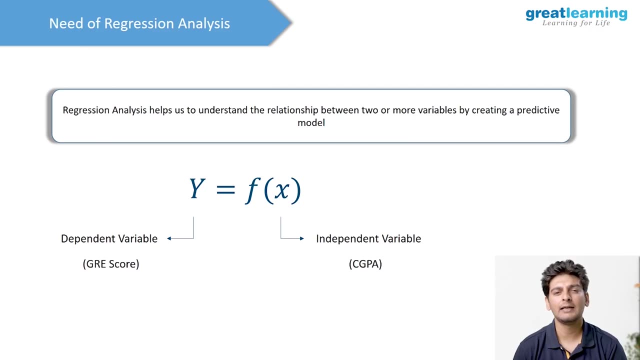 be difficult, and this is exactly where regression analysis comes in. So let's understand what exactly is regression analysis. So, as it is stated over here, regression analysis basically helps us to understand the relationship between two or more variables by creating a predictive model. Now, this simply means that you have a dependent variable and you have the independent variable. 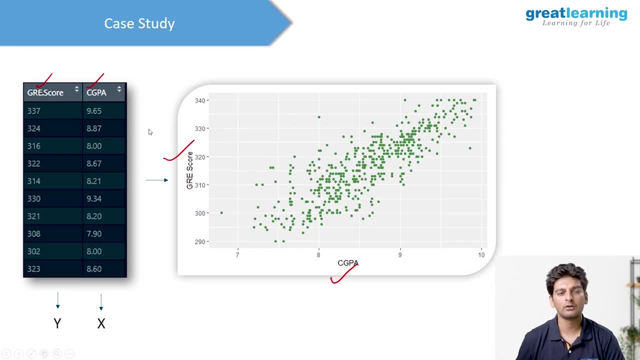 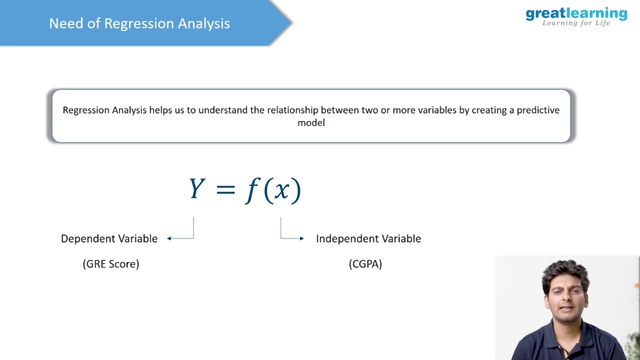 So, as we saw in the previous graph, we had mapped the GRE score onto the y-axis and the CGPA onto the x-axis, But when it comes to regression analysis, we'll do something different. So in regression analysis, you basically have a dependent variable and one or more. 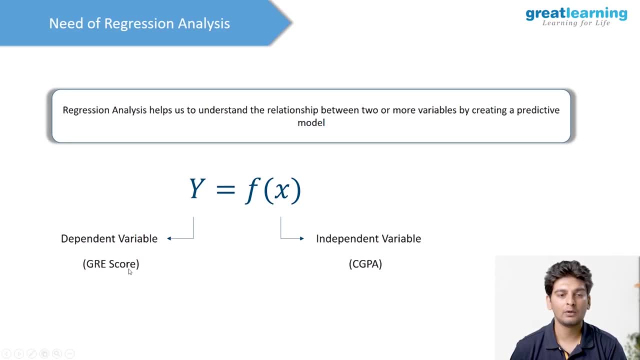 independent variables. Now we will map this GRE score as our dependent variable and we'll map the CGPA as our independent variable and we will try to understand how would the GRE score of the CGPA score vary with respect to the CGPA? Or, in other words, we are basically trying to understand. 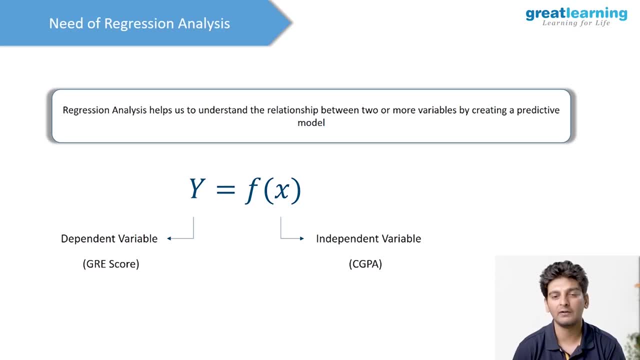 how would the dependent variable change with respect to the independent variable Now, since we already know the value of CGPA, which was equal to 8.32,. so I would have to take this value of CGPA, plug it into the x variable and then I'll get the value of y. So this is how. 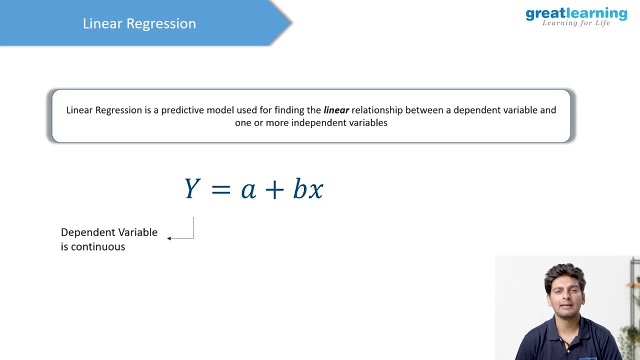 regression analysis works. Now, the simplest category of regression analysis is linear regression, where we basically try to understand the linear relationship between the dependent variable and one or more independent variables. And the important thing to note in linear regression is: your dependent variable needs to be a continuous numerical value. 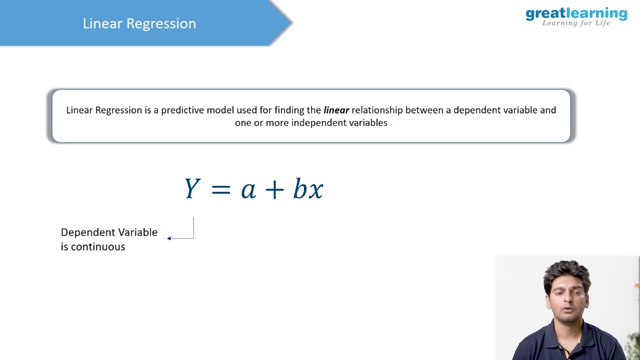 So, and this is what we have with respect to our problem statement. So over here, GRE score is our dependent variable, which is a continuous numerical value, and we are trying to understand how does it change with respect to the CGPA of the student, which would be our independent variable? 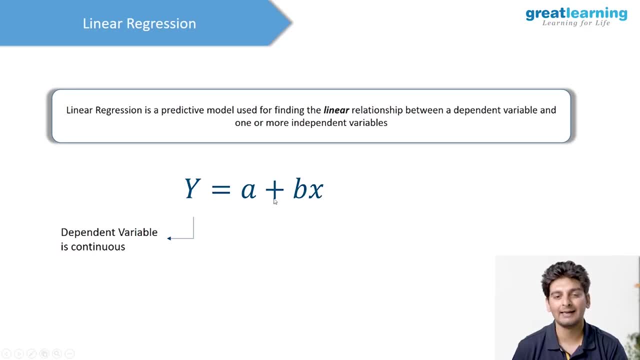 And when it comes to linear regression, we basically have a straight line. So a straight line is a linear equation and that is why this algorithm is known as linear regression. So we have y and we are trying to understand. how does y vary with x? 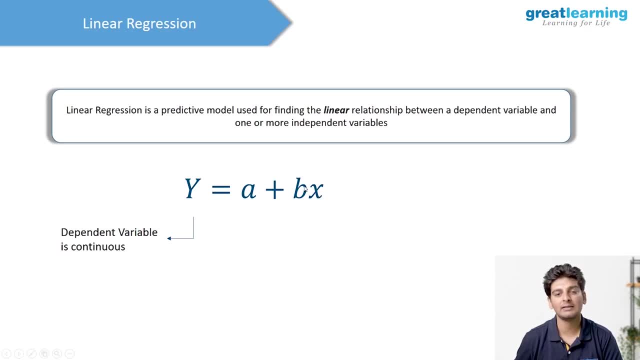 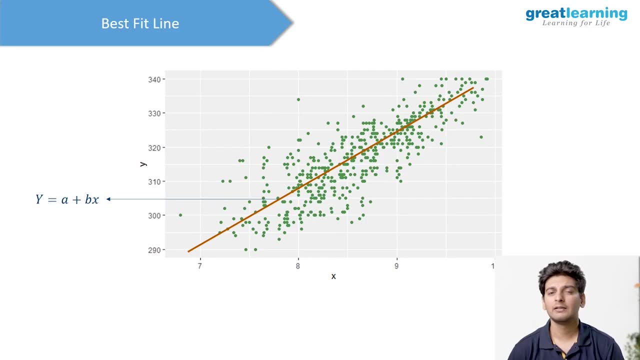 So this b, what you see. so this is the coefficient of x and this is basically the slope of the line, and this a what you see. this is the intercept of the line on the y-axis. Now let's extend this concept of linear regression to the previous problem statement. 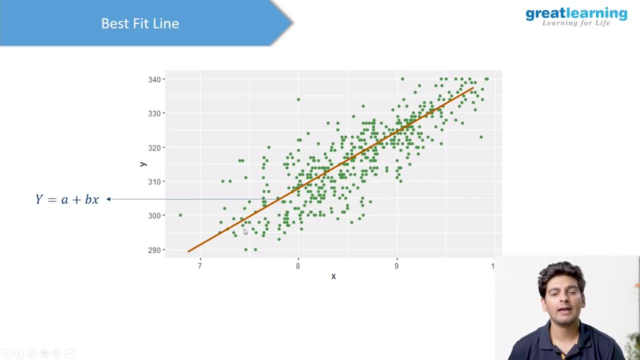 So we had the GRE score of the student mapped to the y-axis and the CGPA of the student mapped to the x-axis. Now we know the CGPA of the student was 8.32.. So let's see: if this value over here is 8.32, then the corresponding value of the GRE score. 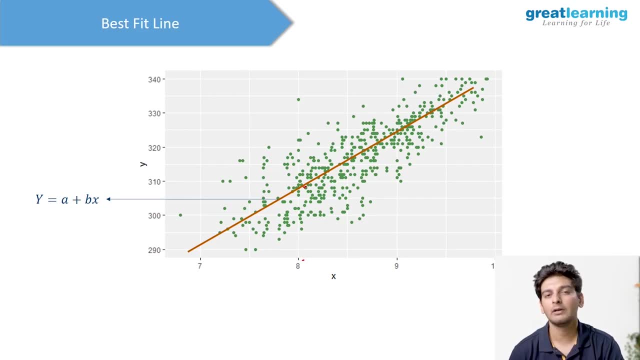 of the student would be around 308 or 309.. But the question over here which arises is: how do you know that this is the best fit line? Now let's see if I draw another line like this and the CGPA of the student is again 8.32.. So for this value of 8.32,, 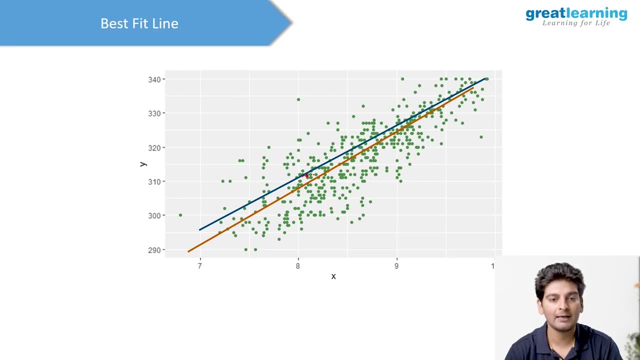 the GRE score of the student could be something else. So this time the GRE score could be around 312 or 313.. So, as you see, when we change the equation of the line over here, the value of y also changes. Now let's say I draw another line like this. So again the value of x is same, but 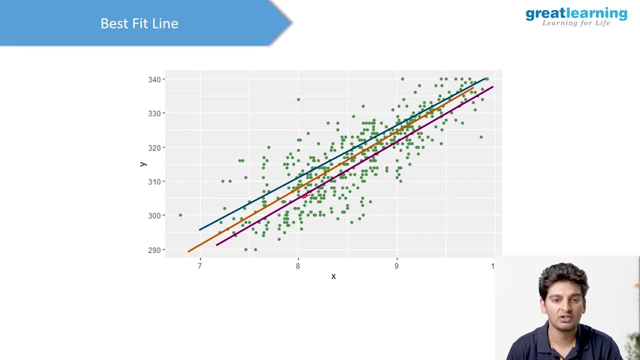 the value of y will change, So this time the GRE score would be around 305.. Now, similarly, we could have a million other lines passing through these set of points. How do you know which is the best fit line? So to understand that, we'll take this example over. 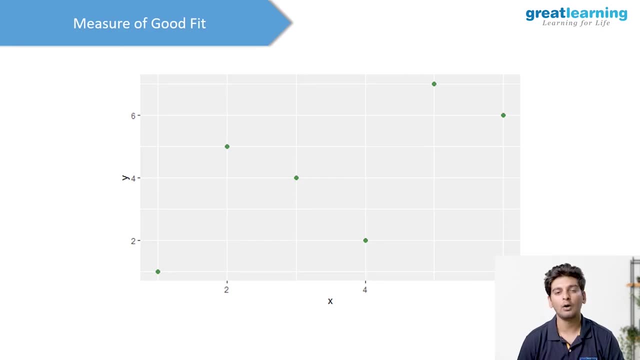 here. So there is something known as measure of good fit. Now, instead of taking all of those points, we'll just take these set of six points over here and I'll start off by drawing an arbitrary line over here. Now, these green points which you see. so these are the actual observed. 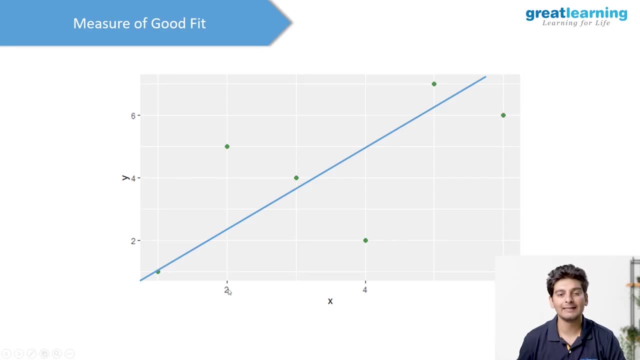 values for the value of x. So when the value of x is equal to 2, the observed value of y is 5.. But then again the value which is being predicted by this line would be around 2.2.. So the difference. 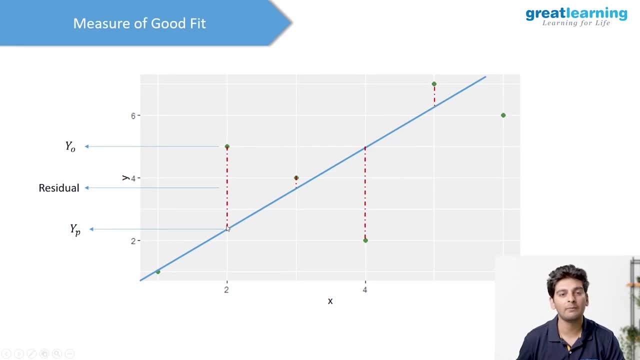 between this observed value of y and the predicted value of y by this line is what is known as the residual or the error in prediction. And similarly, you'll have a residual for all of these points over here. So let's take this point now. Here the x value is equal to 2 and the observed value of y 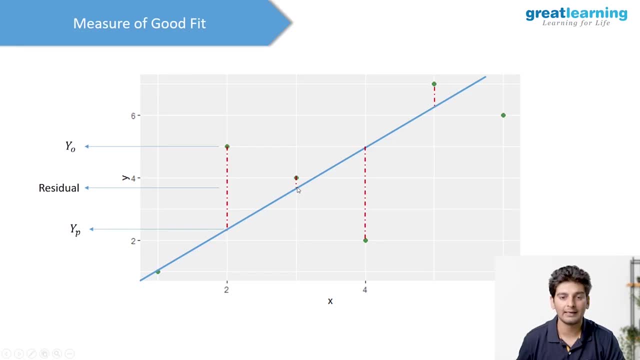 is 4, but the predicted value of y would be around 3.8.. Similarly, if you take this point, x value is 4 and the observed value of y is 2, but the predicted value of y over here is 5.. 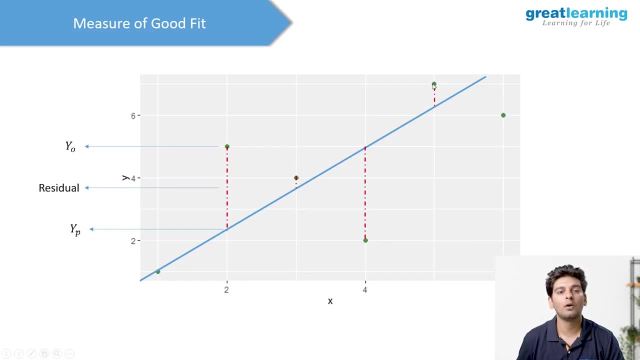 And if we take this point, x value is 5, observed value of y is 7 and the predicted value of y is around 6.5.. Right, so, these dotted red lines which you see, these basically indicate the residuals or the error in prediction. And to get that best fit line, don't you agree that we would basically have? 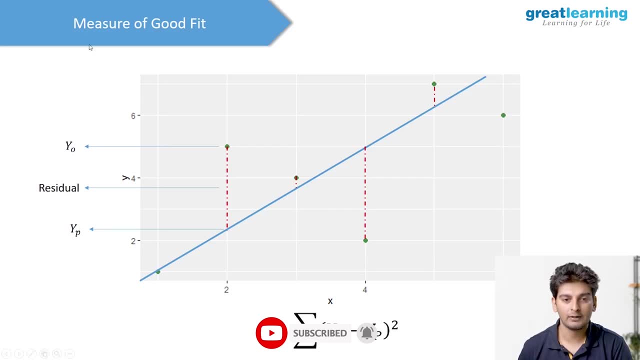 to take the sum of all the residuals, or the error in prediction as the sum of all the residuals. So that's where we have something known as the residual sum of square. So what we do is we'll go to this first residual and we'll square this up. Then we'll go to the second residual, we'll square. 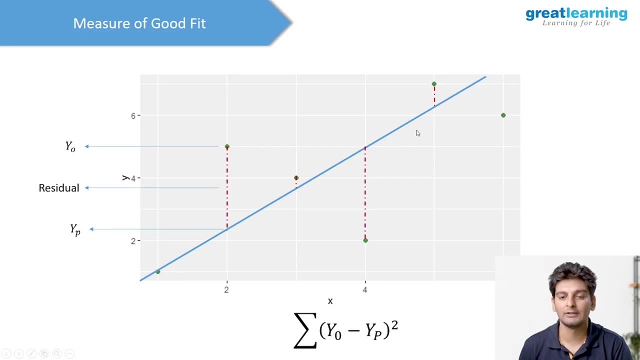 this up, Go to the third residual and then we'll square this up And we'll do this for all of the residuals and then we'll take the sum of all of the residuals. Now, when we take the sum, this has to be as low as possible and whichever line would have the lowest value of residual sum of squares. 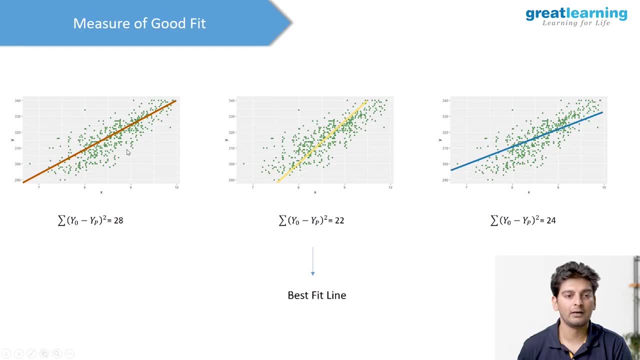 this concept to the previous problem statement. So this was our problem statement, where the GRE score was on the y-axis and the CGP of the student was on the x-axis, and we've got these three lines over here. So for the first line, the residual sum of squares comes to be around 28.. For the 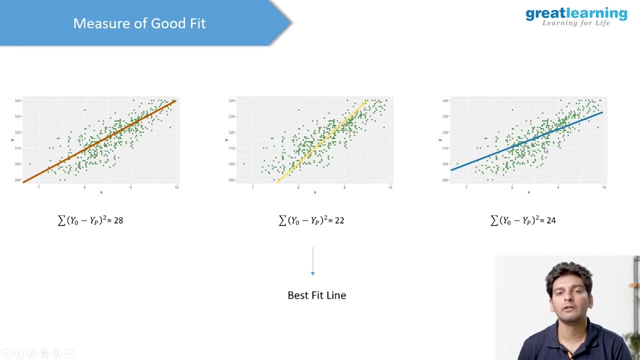 second line, the residual sum of squares comes to be around 22. and for the third line, the residual sum of squares comes to be 24.. Now, when we compare all of these three residual sum of squares, the second line would be the best fit line for our problem statement. So now we've got the best. 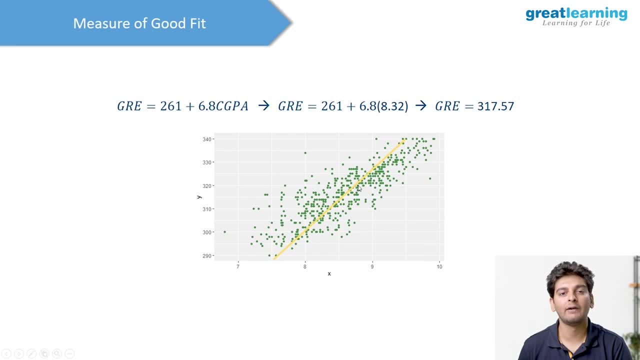 fit line and we already know that a linear line would have an equation associated with it, which is basically: y equals mx plus c and that is the equation over here. So, over here, y is basically the GRE score of the student and x is the CGPA of the student, and these two, which you see, the m. 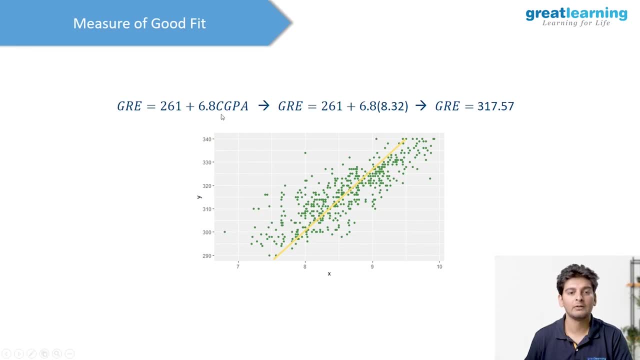 value and the c value. this we've got from the best fit line, So the m value, which is the slope of the line, comes to be around 28.. So we've got the best fit line and we already know that the 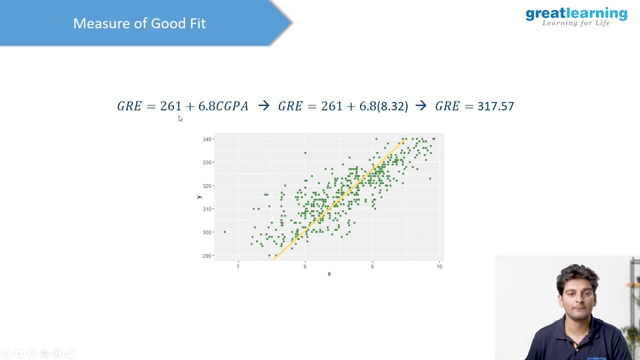 linear line comes to be around 6.8 and the y intercept comes to be 261.. Now to get the GRE score of the student, all we have to do is plug in the CGPA of the student, which we already know. 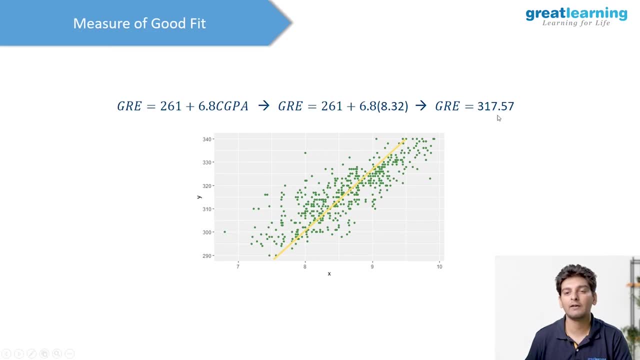 So we'll plug in 8.32 into this equation and we'll get a final value of 317.. So this is how you are able to get the GRE score of the student: by just knowing the CGPA of the student and this. 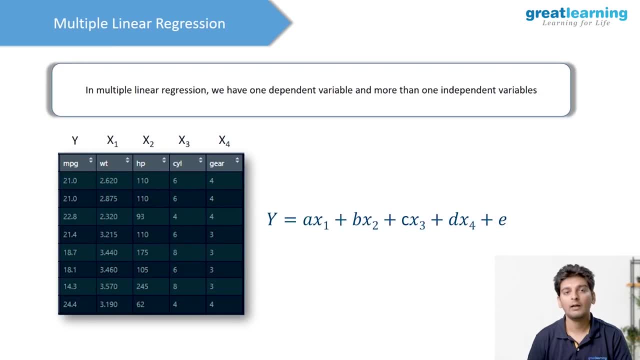 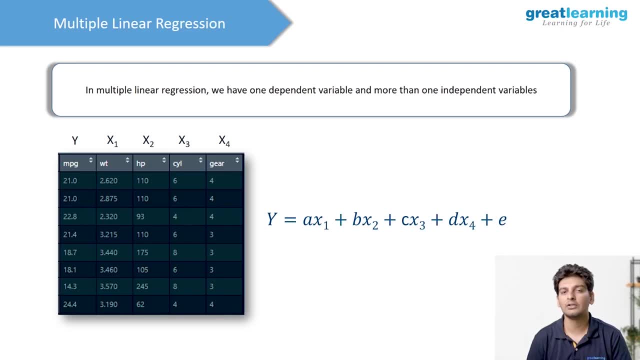 something known as multiple linear regression. So in multiple linear regression we'll have multiple independent variables instead of just one independent variable. So to understand that, we'll take this data set over here. So this is the famous empty cars data set, where we have 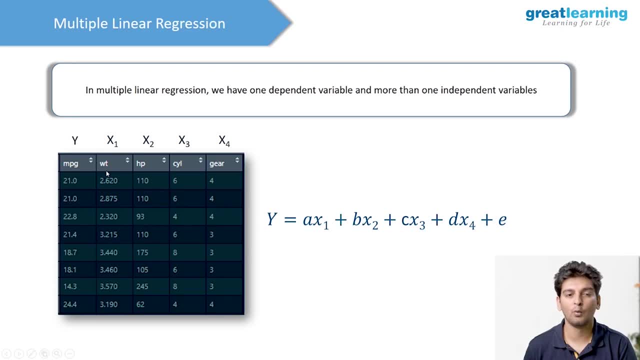 these columns. So this is the miles per gallon column. Then we've got the weight of the car, the horsepower of the car, the number of cylinders in the car and the number of gears in the car. And we want to understand: how does the mileage of the car vary with respect to all of these other? 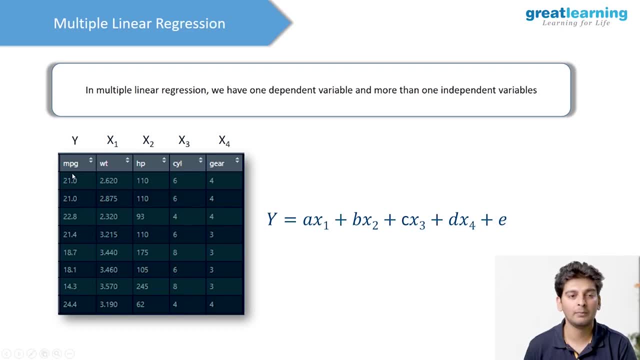 independent variables. And since mileage is our dependent variable, we'll denote it with y, and all of the other independent variables would be denoted like this. So weight, I'm denoting it with x1, horsepower with x2, number of cylinders with x3 and number of gears with x4. And this is 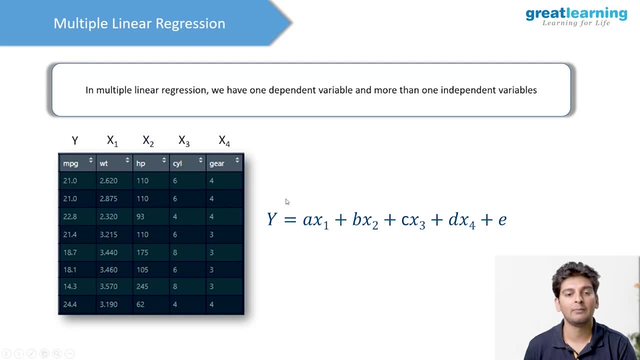 the final equation of this hyperplane over here. So we'll type in: y equals a x4 over here. So x1 plus px2 plus cx3 plus dx4 plus e, And this would be the equation of the hyperplane. So to: 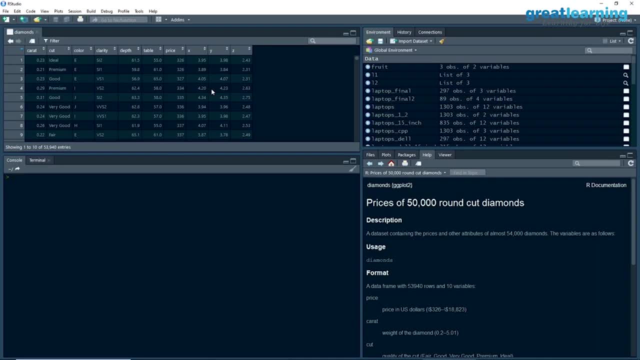 implement the linear regression algorithm. we'll be working with this diamonds data set And let's have a glance at the description of this data set. So this data set comprises of 10 columns and there are 53,940 rows, Or in other words, there are 53,940 diamonds. So we've got the price. 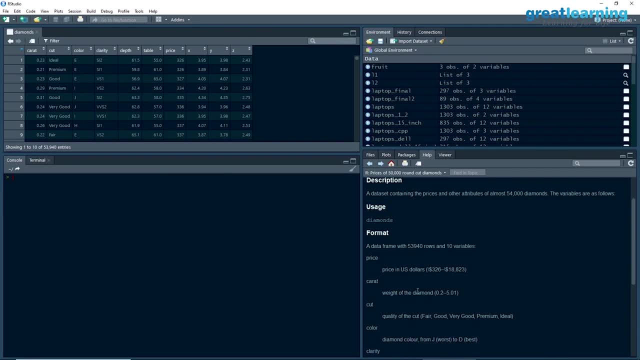 column, which basically denotes the price of the diamond, then US dollars, Then we've got carat, which denotes the weight of the diamond. Then we've got cut, which is for the quality of the cut. So we've got all of these different columns over here. Then we've got x, y and 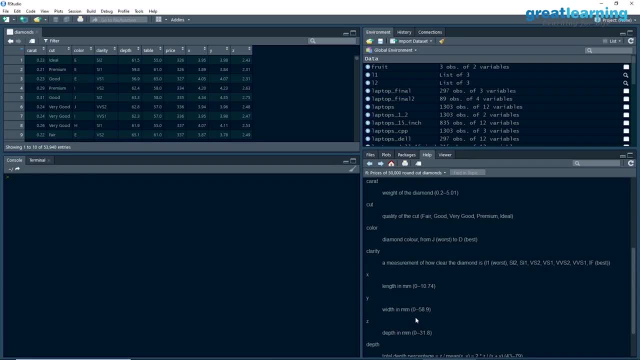 z, which basically denote the length of the diamond, the width of the diamond and the depth of the diamond in millimetres. All right, Now, before we go ahead and start off by implementing the linear regression algorithm, let's do some data manipulation and data visualization and let's 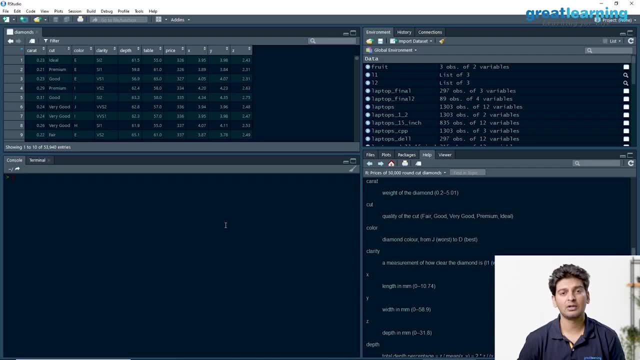 understand this data set properly. So I'll start off by looking at the structure of this data set. and to look at the structure of this data set, we'll use this data set. For instance, if I had to use of the data set, i'll use this str command and inside this i'll pass in this data set, which is: 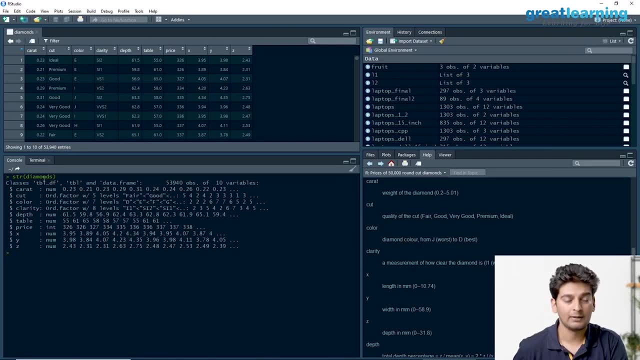 diamonds. so i'll type in diamonds over here, right? so these are all of the columns over here. so you see that carrot is a numerical column and then we've got cut, color and quality, which are factors. then again we've got numerical columns over here, right? so this is the structure of this. so we saw. 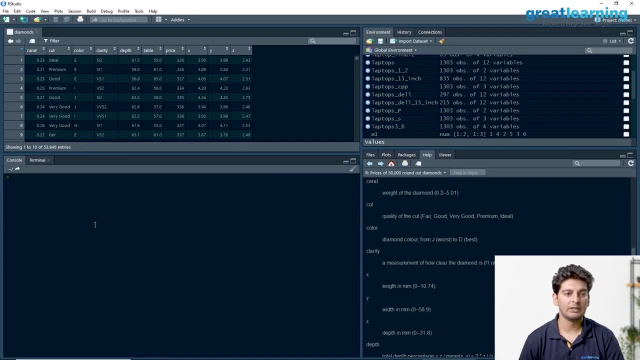 the structure of the data set. now we'll go ahead and perform some data manipulation operations. so let's say i wanted only a subset of this entire data set where the cut of the diamond is equal to premium and the price is greater than five thousand dollars. so for that i'll be using 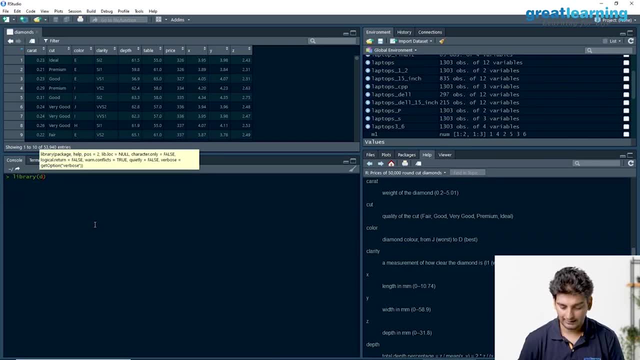 the deploy package. so let me load up the deploy package. so i'll type in library of deployer and we've got the filter function from the deploy package. so i'll start off by giving the name of the data set, which is diamonds, and then i'll use this pipe operator. now, this pipe operator. 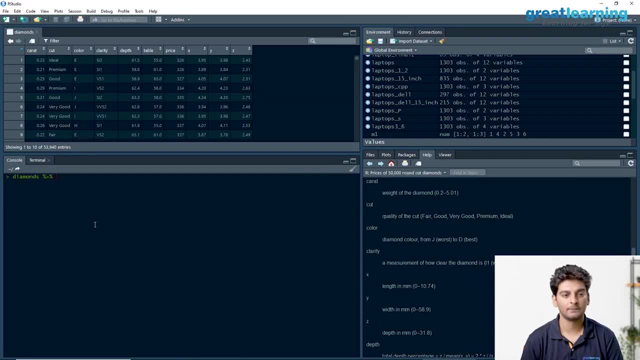 is the name of the data set, which is diamonds, and then i'll use this pipe operator. now, this is used to connect different objects and functions together. so, with the help of this pipe operator, i am connecting this diamonds data set with the filter function and inside the filter function. 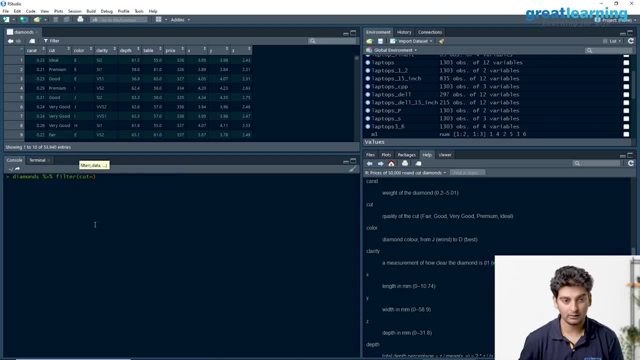 i'll give in my conditions. so the first condition would be: the cut of the diamond needs to be equal to premium. so i'll type in premium over here and then i'll give in the second condition, which is the price of the diamond needs to be greater than 5000. so i'll set the condition, which is price is. 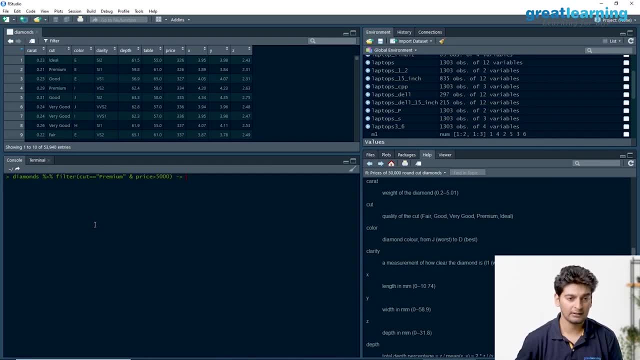 greater than 5000, and i'll show this in a new data set and name it as, let's say, premium price. let me have a glance at this. so have a glance at the data set. i'll be using the view function and inside this i will. 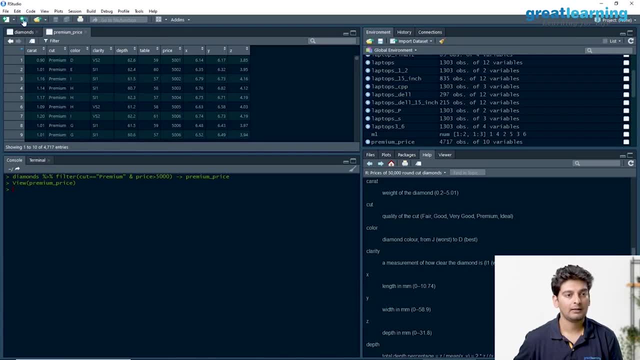 give in the name of the data set, which is premium price, right? so out of the 53 000 diamonds we have extracted only 4717 entries where the cut of the diamond is equal to premium and the price of the diamond is greater than 5000, right? if you look at these two columns closely then you see that in the 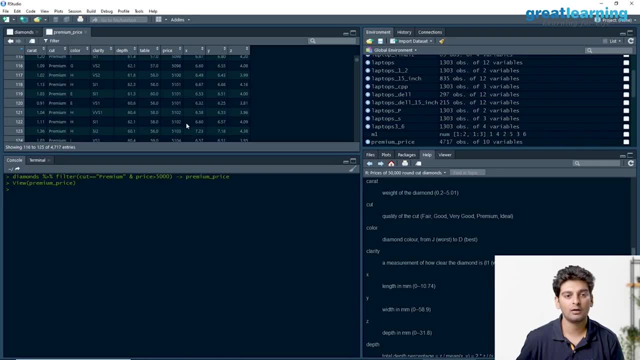 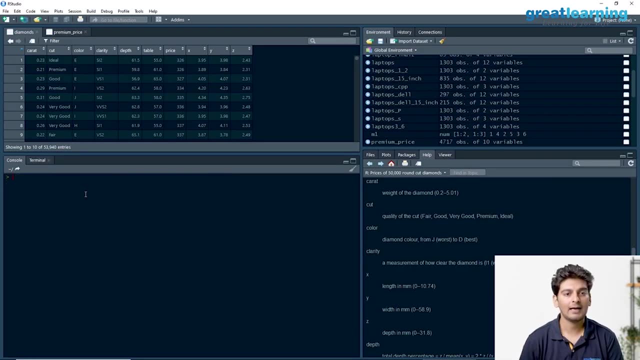 cut column the value is only premium and in the price column it is greater than five thousand dollars. now, similarly, let's do some other operations. now let's say i want the length of the diamond to be greater than four millimeters, so let's go ahead and give in that command again. 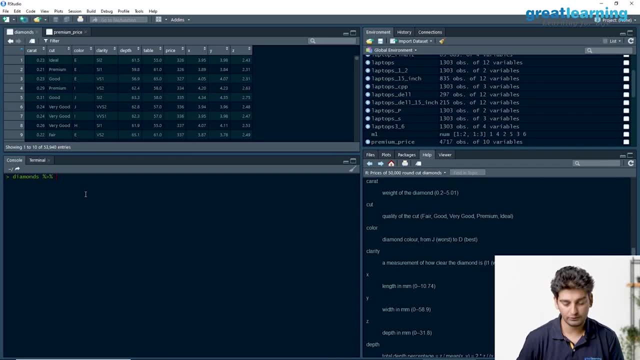 i will start up by giving the name of the data set. after that i will use the pipe operator and then use the filter function and inside this i'll give the condition. so x needs to be greater than 4. i'll store this in diamonds underscore length. now i'll have a glance at this view of diamonds length. 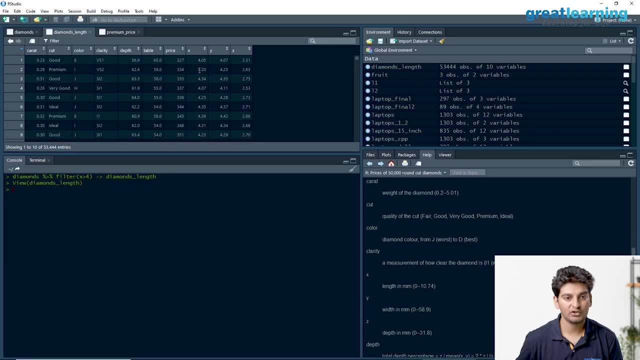 so, as you see over here, if you check this length column, which is x, you see that the length is greater than 4 millimeters. so these were some basic data manipulation operations. now we'll go ahead and perform some data visualization operations using the ggplot2 package. so i 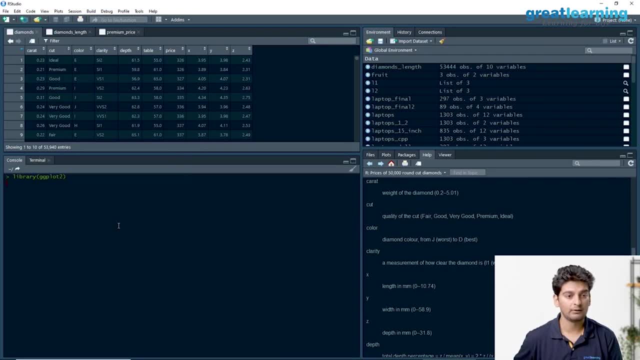 loaded the ggplot2 package, i'll type in library of ggplot2 over here now. this data set basically, which i'm working with, the diamonds data set, is also part of the ggplot2 package. so if you want to implement all the same code in your system, then you'd have to load the ggplot2 package first. 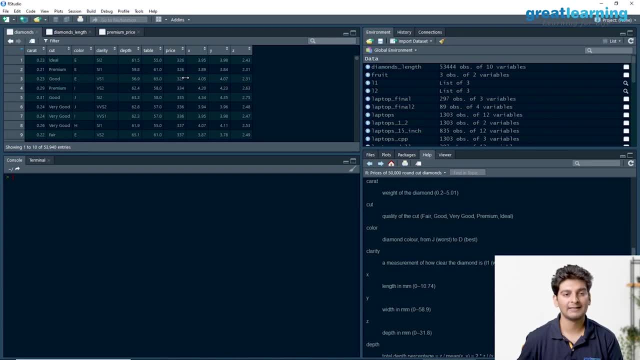 now i want to understand the distribution of this price column. so to understand the distribution of this price column, i'll just go ahead and build a histogram. so this is how we can build a histogram: i'll type in ggplot and i will assign the diamonds data set onto the data layer. so 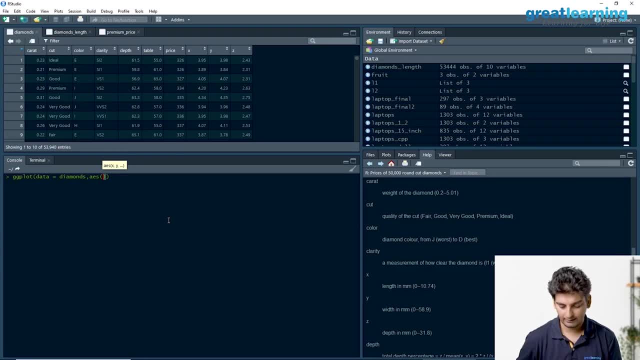 once the data layer is done, i'll go to the aesthetics layer and i will map the price column onto the x aesthetic. now i am done with the data layer. so i've mapped the diamonds data data layer and i've also mapped the price column onto the x aesthetic. now it's time to determine. 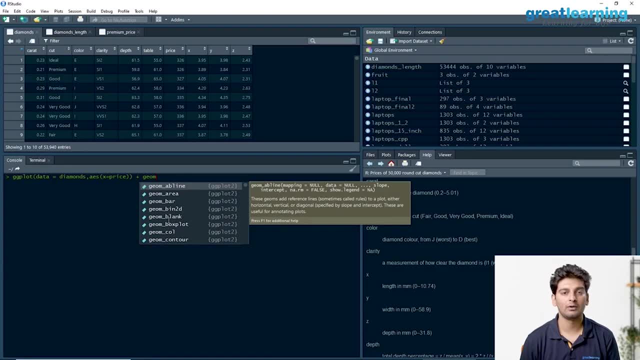 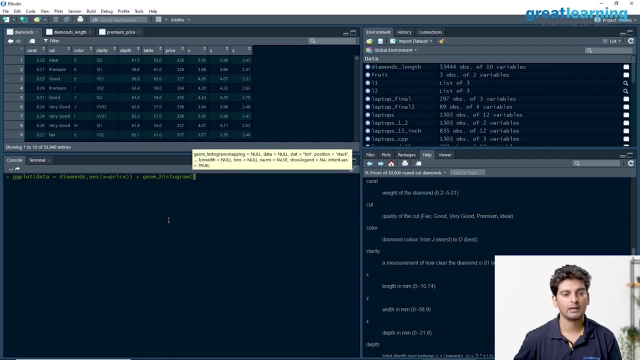 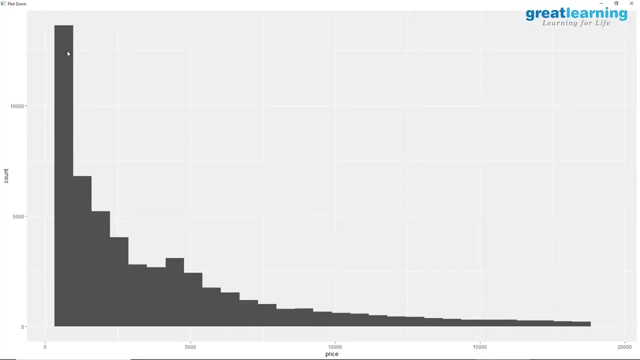 the geometry. so geometry is basically the type of plot which i want to create and i want to create a histogram. so, to create a histogram, we've got the germ histogram function. now i'll just hit enter and we've got this really beautiful plot over here. so let me zoom this right. so, as you see, 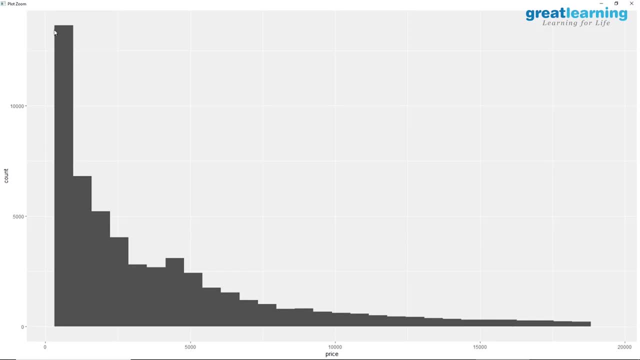 there are a large set of diamonds, so there are around more than 15 000 diamonds whose price would be less than around thousand dollars. right, and there are very, very few diamonds, so there would be not even around 20 or 30 odd diamonds whose price is greater than 15 000. 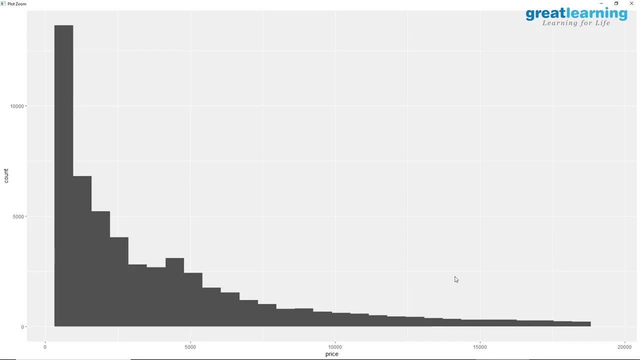 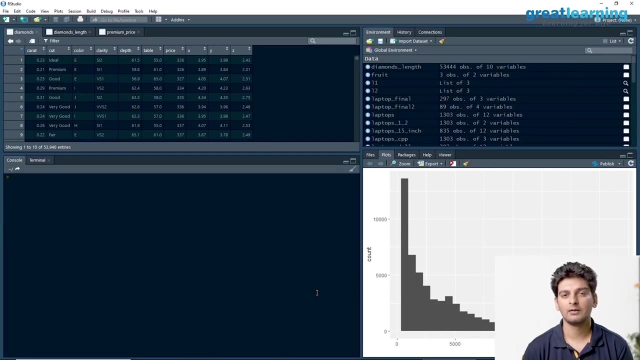 dollars. so these were some of the simple inferences which we were able to draw by building this histogram. so now that we are done with the basic data manipulation and data visualization, we'll head on to the main part where we'll be building the linear regression algorithm. now we want to 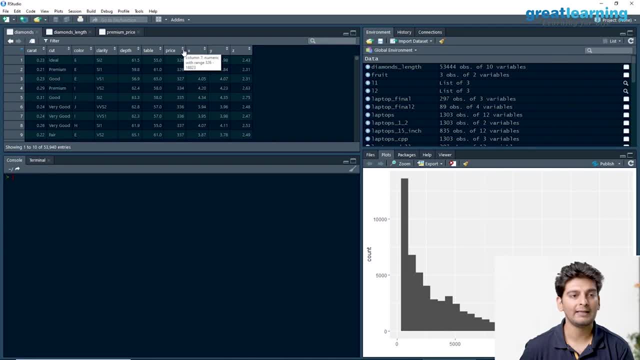 understand. how does the price of the diamond vary with respect to the carat of the diamond? so let's say, if i given a carat value of around 1.3, so if the carat value is 1.3, then i'd want to know the exact price of the diamond. so this is. 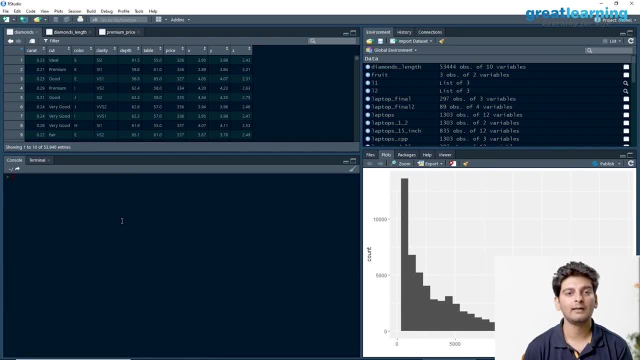 where linear regression comes in. now, before we build the linear regression algorithm, we actually have to divide our data set into training and the testing set. so we'll be building our model on top of the train set and we'll be evaluating the results on top of the test set. 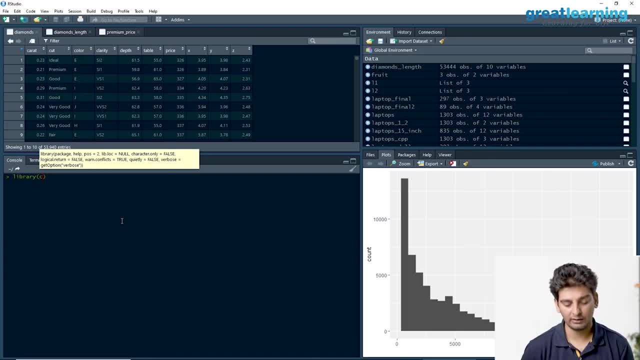 so to split the data set into training and testing sets i would need the ca tools package. so the ca tools package gives me the sample dot split function. so let me just type in sample dot split over here, and this takes in two parameters. so the first parameter is basically the column. 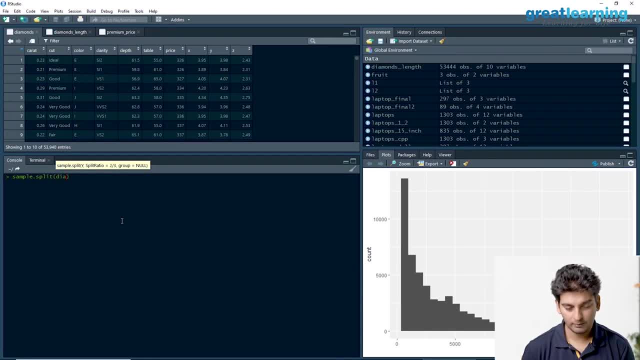 with respect to which i want to split my data set and i want to split this data set with respect to the price column. so i'll select this price column over here and i will give in the split ratio. so i'll give it a split ratio to be equal to 0.75 and i will store this in a new object and i will name. 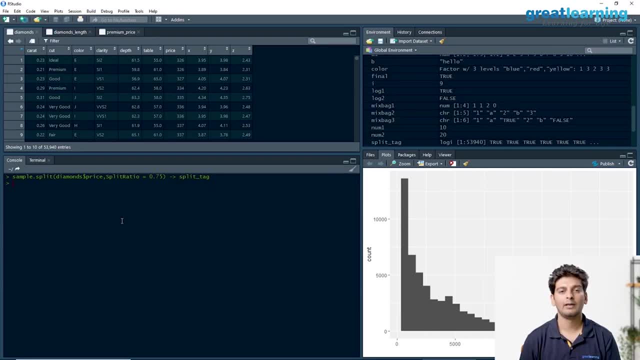 that object to be split tag now. i'll just wait till this command is executed. now you guys must be wondering: why do you have to divide our data set into train and test set? so let's take this example to understand it better. so let's say you have a math test tomorrow and you haven't learned. 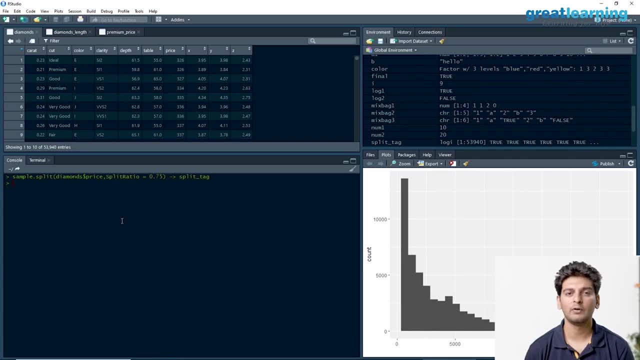 anything at all. but your friend luckily steals the question paper from the principal's room and when you see the question paper you see that there are five questions and you perfectly learn all of those five questions. now there are two situations. if all of those five questions would, 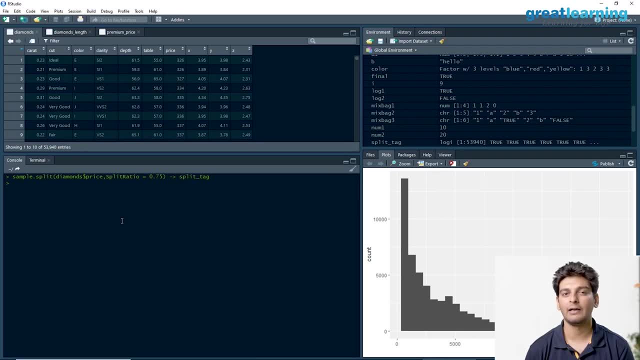 appear in the exam, then you'd ease the exam, so you'll get five out of five. but what if none of the questions appear in the exam? then you'll get zero out of five, right? so this is what i'm trying to tell you. so we'd have to divide the data set into training and testing set, so you'd have to. 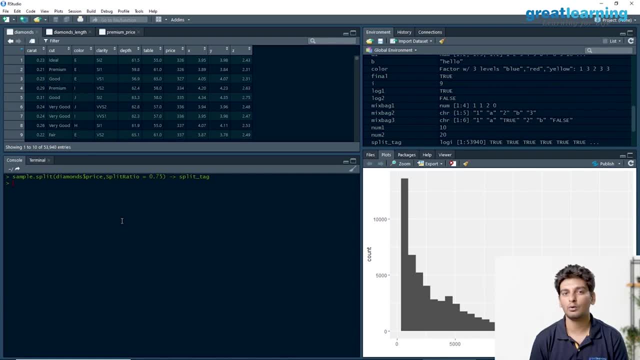 test it on another set. and if you don't do that and directly go ahead and build your model on just one particular data set, then there are very good chances that it might fail on a new data set. so this is the reason why we divide into two particular data sets. so over here we've got the 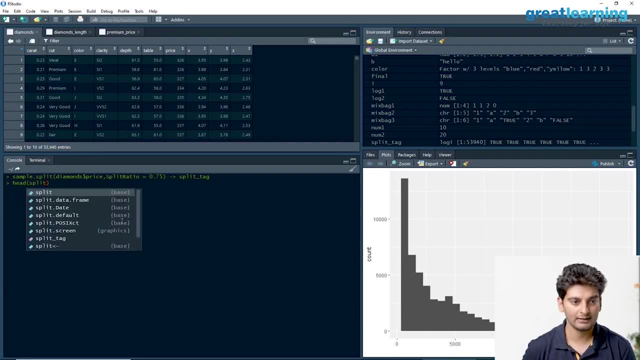 split tag. now let me use the head function and see what is there in the split tag. so split underscore tag. now, as you see, you just got a bunch of true values over here. so what this function basically does is it assigns 75 of the records with the true values and 25 of the records with the false. 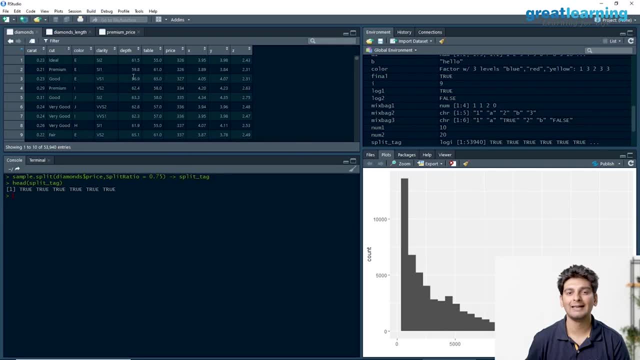 values. now, using these true and false values will divide this entire data set into two parts. so for this i'd have to use the subset function. so i'll type in subset over here and the first parameter would be the name of the data set, and then i'll use the split tag. i'll just type in split tag over. 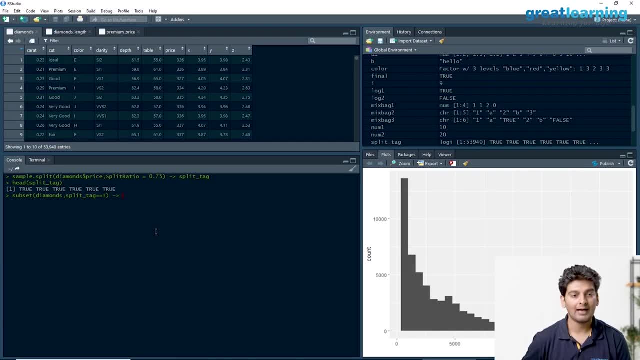 here and wherever the value of split tag is equal to true, i'll store this in a new data set and name that data set to be equal to train. similarly, i'll use the subset function again and i'll pass in the first parameter, which is the name of the data. 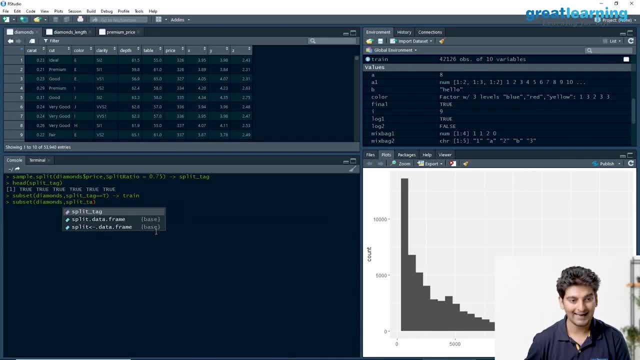 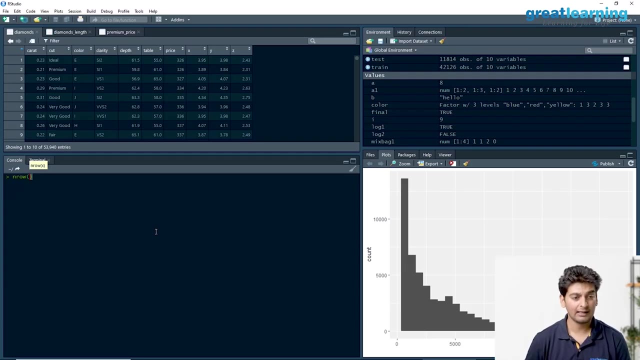 frame, and this time i will set the split tag to be equal to false. so wherever the split tag is equal to false, i'll take all of those records and i'll store them in the test set. so now we've got the train set and the test set ready. now let me have a glance at the number of rows in the 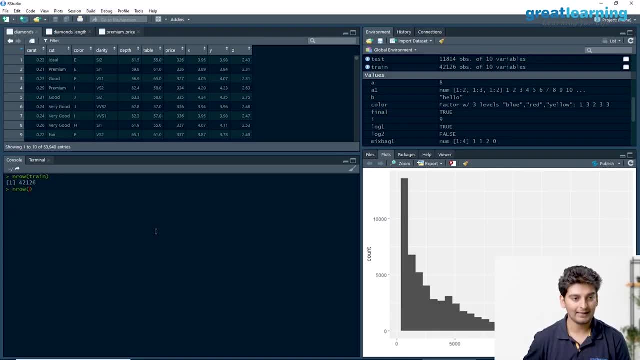 train set and the test set. so i'll type in n row of train and n row of test. so we see that there are 42 126 entries in the train set and there are 11 814 entries in the test set. so now it's time to go. 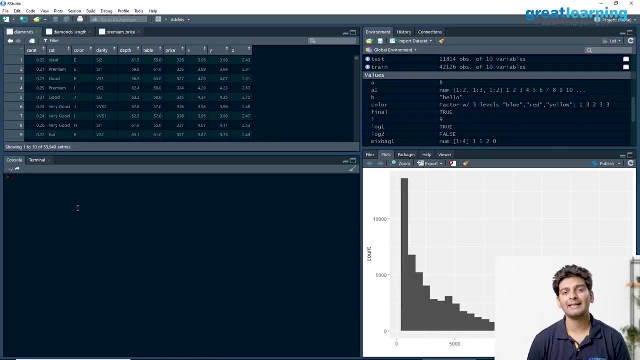 ahead and build the model on top of the train set and to build the linear regression model. we've got this lm function, so i'll just type in lm and the first parameter is the formula where we're given the dependent variable and the independent variable. so my dependent variable is price. after that i'll give in the tilde symbol and then i'll give in the 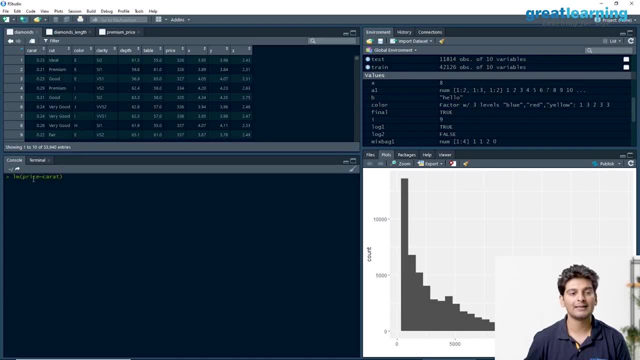 dependent variable, which is carat. so i want to understand: how does price vary with respect to the carat? so whatever value is given on the left side of the tilde symbol, that will be taken as a dependent variable, and whatever values are given on the right side of the tilde symbol, all of them. 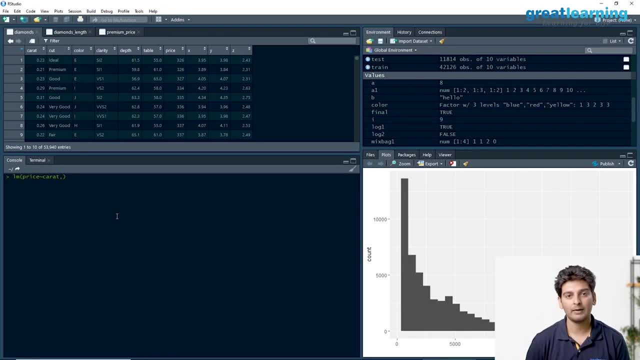 would be taken as the independent variables. so this is my first parameter, which is the formula, and then i'd have to give in the data set on which i'd have to build the model. so i've already told you, we are supposed to build this model on top of the train set, and i will store this in a new object and i'll name it as, let's say: 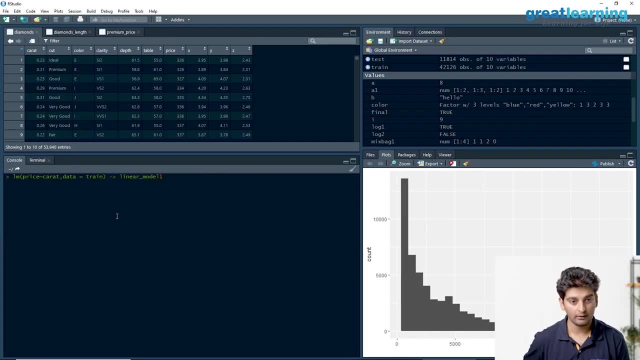 linear model one. let me just print it out over here: linear model one, right? so this is what we have over here. so call. you see that we have the formula price with respect to carat and it is built on top of the train set and beneath that. 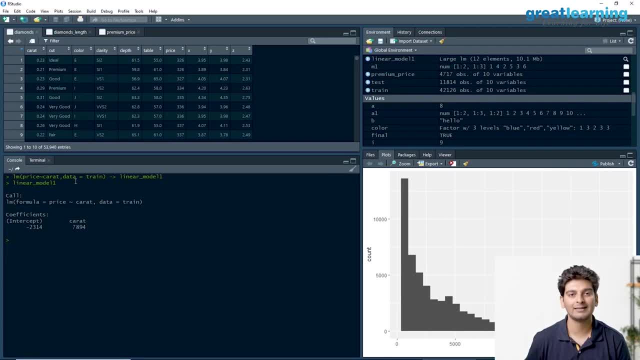 we've got the y intercept and the m value for this independent variable. so x is carat and the m value, or the coefficient of this carat is 7894, and the y intercept. so y intercept for the equation a is equal to bx would be the a value over here. so we've got the y intercept and we've also got the. 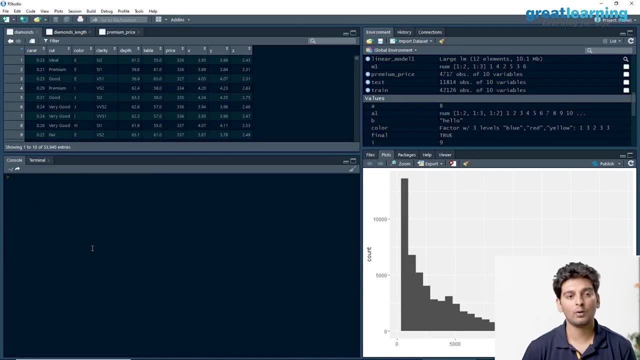 m value over here. now that we've built the model, let's go ahead and predict the values on top of the test set. so i'll type in predict now. this takes in two parameters, so the first parameter would be the model which you've built and the 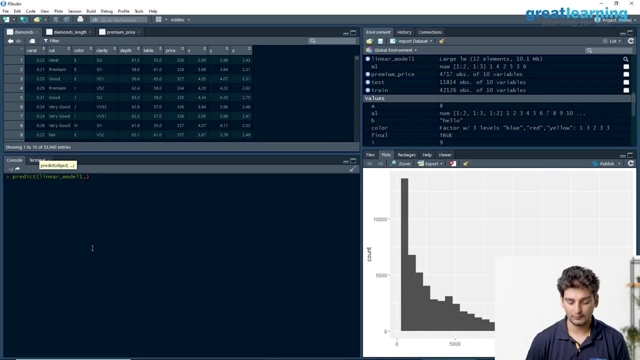 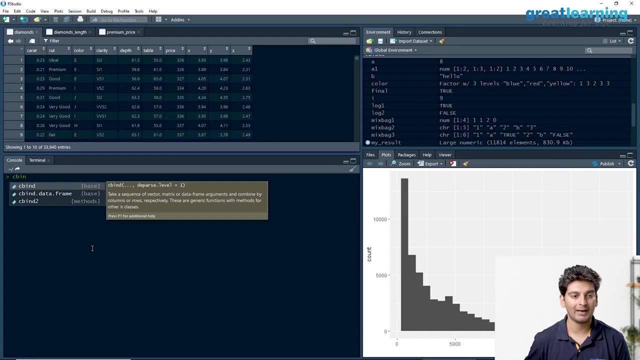 second parameter would be the data set on which we're supposed to break the values, and i want to predict the values on top of the test set, and i will store this in, let's say, my result. so we've got the actual values and we've also got the predicted values. now i'll go ahead and combine. 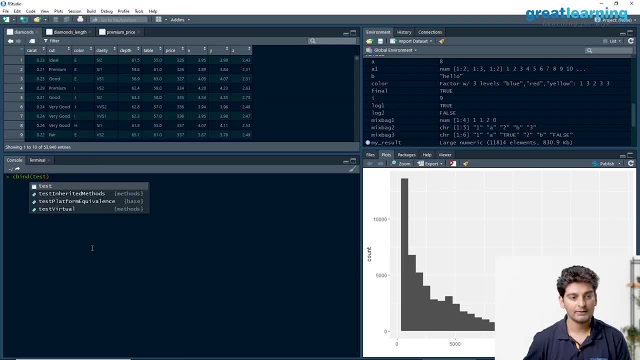 these two. so to combine these two i'll use the c bind function. so the actual values are present in the price column of this test data set. so i'll just name this column as actual and then i will create another column which is predicted, and these predicted values are coming from my result and i will store. 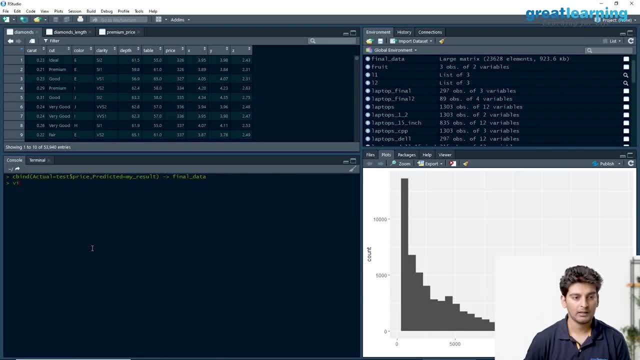 this in final data. now i'll have a glance at this. so view of final data. so we've got the actual values of the diamond and we've got the predicted values of the diamond right. so let's see. if this is the actual value- 351- the predicted is 54.. so there's a huge error in this prediction over here. 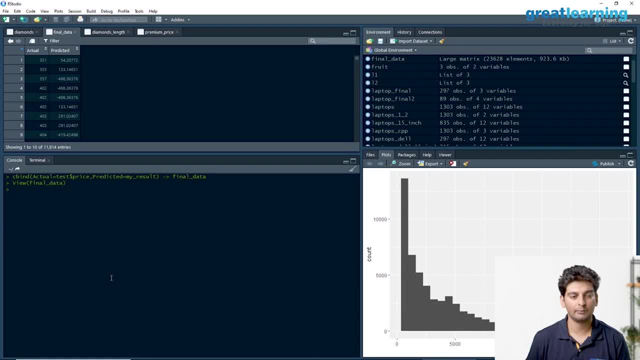 now we'll go ahead and find out the residual or the error in prediction, so that would be basically actual minus predicted. that's how we find the error in prediction. now i'd have to convert this into a data frame first, so this is actually a matrix. so i'll use as dot data frame and i'll 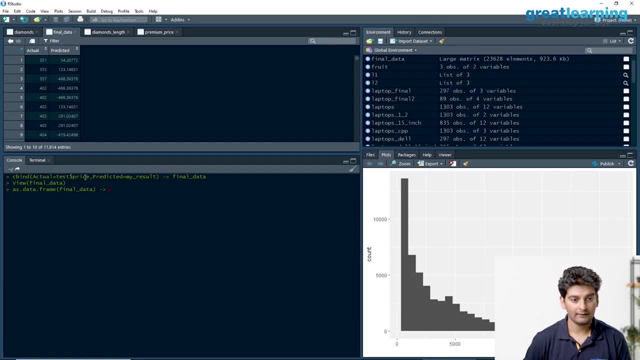 pass final data into this and i will store this back to final data and once we are done with this, i will go ahead and subtract the predicted values from the actual values. so final data dollar actual minus final data dollar predicted. so i'll cut this out. i'll 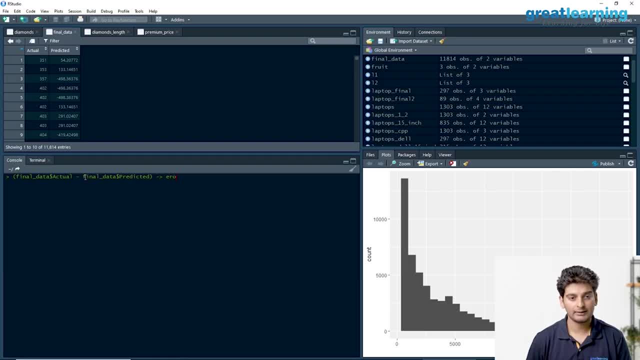 paste this inside these round braces and i'll store this in a new object and i'll name that object to be equal to error and i'll bind this error back to the same data set. so c bind of data and i am binding it with error and i am storing it back to the same data set, which is: 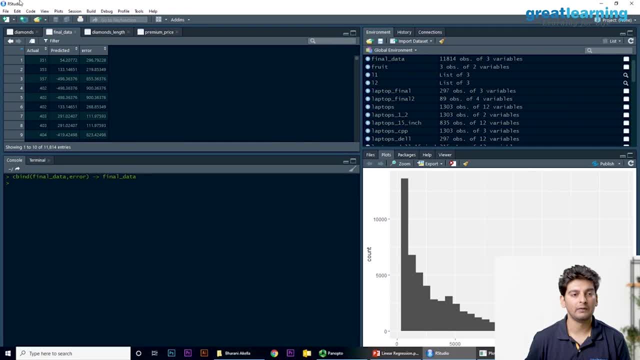 final data right. so we've got the actual values, we've got the predicted values of the price of the diamond, and then we've got the error in prediction. so these are the individual residuals with respect to each point. now we'd want to find out the residual sum of squares. 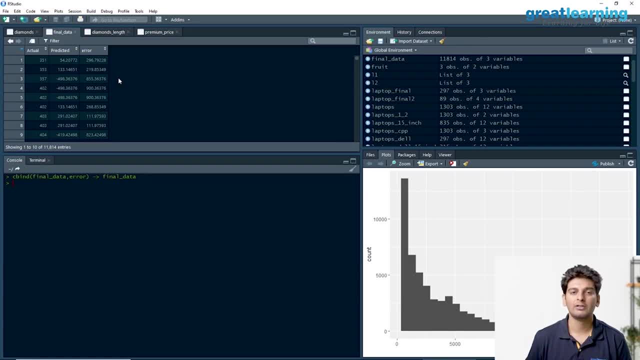 so we have something known as the root mean square error, which basically gives us the average error for the entire model. so, as it is stated in the name, root mean square error. so first we'd have to find out the square of all of these errors. so i'll type in final data: dollar. 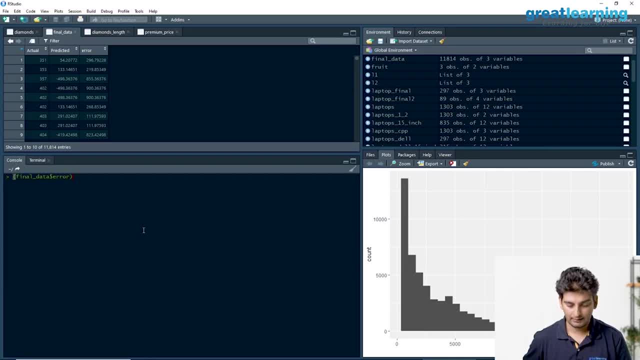 error. let me cut this out and i will go ahead and find out the square of this now, once this is done- so i have got the square of all of these errors. then i'd have to find out the mean of it, right, and finally, i will go ahead and also calculate the square root of it. i'll paste it. 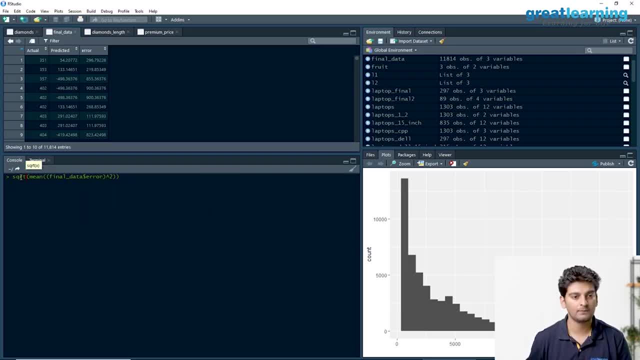 inside this and i'll use the sqrt function right. so root mean square of error, this is what i'm finding out, and i get a root mean square value of 1221, which is actually quite huge. so this tells us that the model which we built is not actually accurate for us to give us the right results. 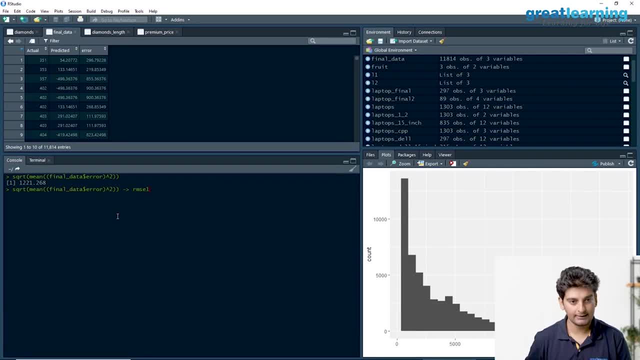 and i'll store this in, let's say, rmse1. so this was a simple linear model where price was our dependent variable and carat was our independent variable. now we'll go ahead and build a multiple linear regression model, so this time we'll use multiple columns as our independent variables. 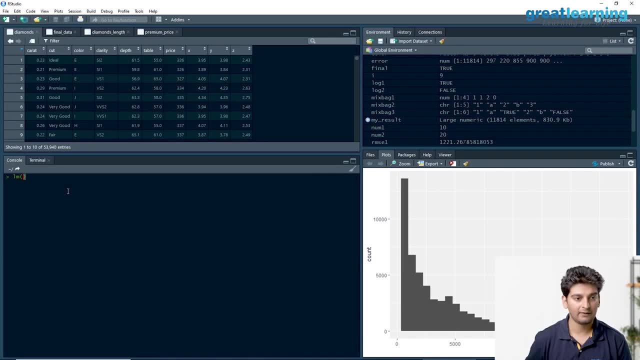 so let me go to this data set and let me use the lm function again. so price again would be my dependent variable and my independent variables would be, let's say, x, y and z, which are basically the length, width and the depth of the diamond. so i'll type in x plus. 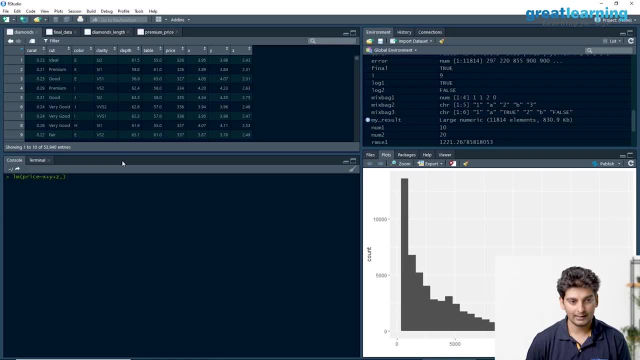 y plus z, and i am building this model again on top of the train set, so data would be train and i will store this in linear model 2. i have built my model and i'll go ahead and break the values, so i'll use the predict function and the first parameter would be the model which i've 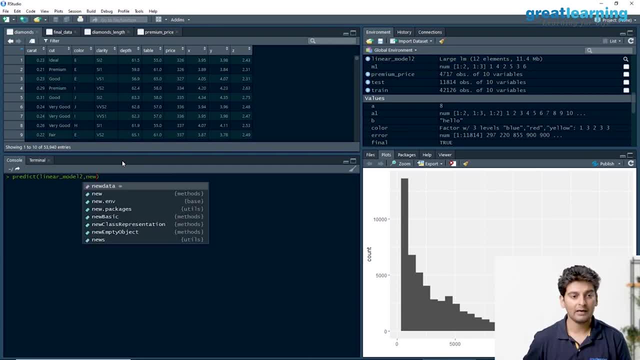 built, which is basically linear. 2. and then i will give in the data on which i'd have to break the values, which is new data. so i want to predict the values on top of the test set and i will store this in my result. 2. 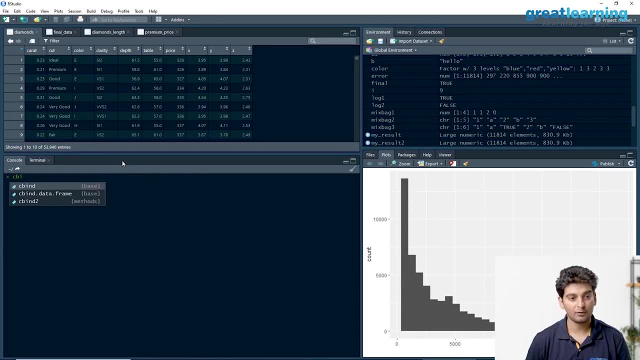 i have also predicted the values. now it's time to bind again the actual values and the predicted values. so the actual values are present in test dollar price and the predicted values are present in the my result 2. right now let me give them their proper names. so i'll give an actual over here and i'll also give 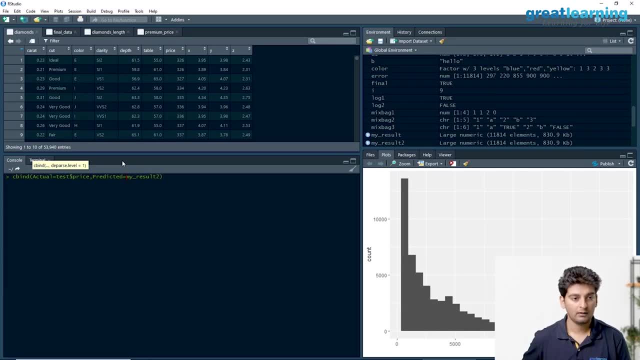 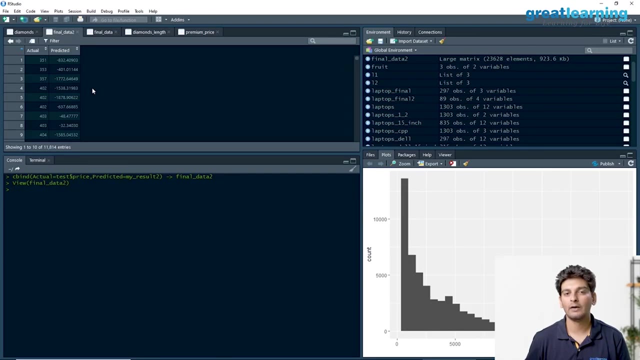 in predicted over here and i will store this in final data 2, so we have our new final data ready. so view of final data 2. right, so for the second model which we've built, where we had three independent variables, these are the actual values of the diamonds and these are the 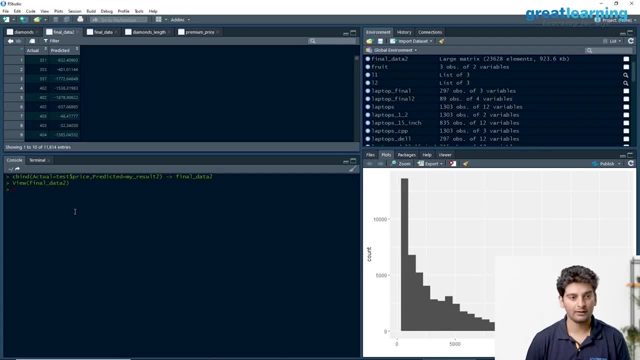 predicted values of the diamonds. now let's go ahead and find out the error in prediction. so before that, we'd have to again convert this into a data frame, so as dot data frame of final data 2 dollar. this has to be final data 2 and i will store it back to final data 2. 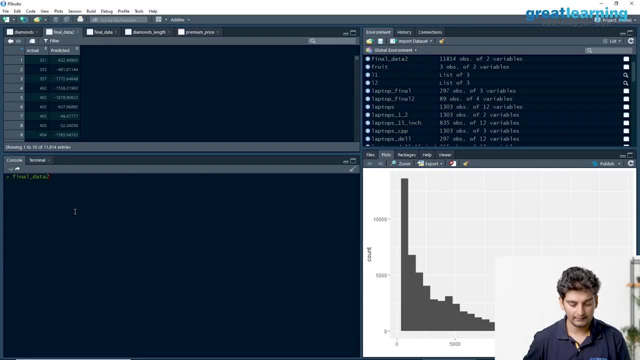 all right. now it's time to find the error. so final data 2 dollar actual minus final data 2 dollar predictor. i'll cut this out and i will store this in error 2. now it's time to bind the error back to the original data set. so c bind of final data 2 and i am binding it with error 2, which is stored again. 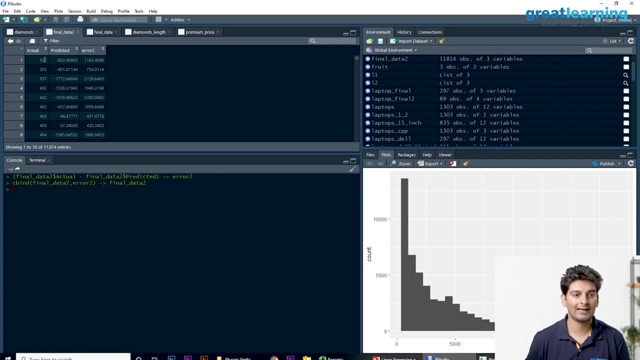 in final data 2. so we've got the actual values, the predicted values and the error in prediction. now it's time to find out the root mean square error for the second model. so final data 2: dollar error 2. i'll cut this out, paste it inside this, let me. 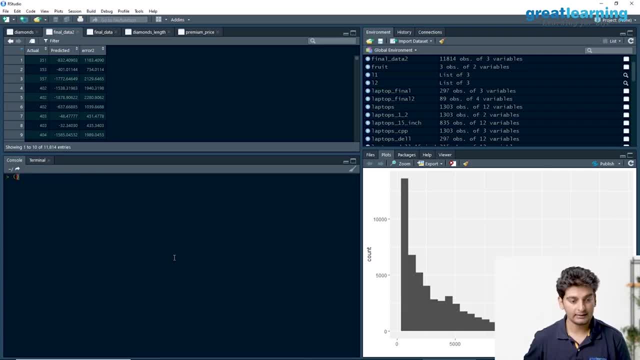 take the square of the error. once i take the square of the error, i'd have to take the mean of it, and once the mean is also done, i'd have to take the square root of it. so i'll type in sqrt over here, right? so this time the root mean square error comes to be around one, five, seven, four. 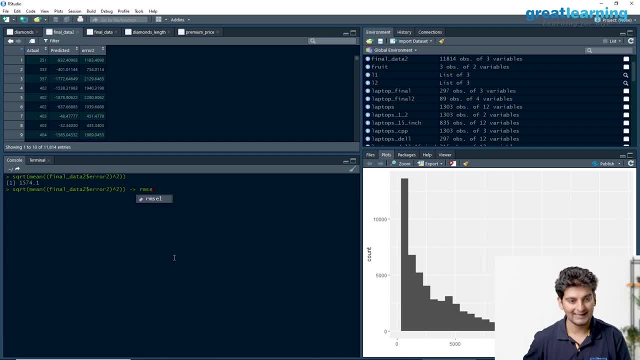 and i will store this in. let's say, r m s e 2. now let me print out both rmsc one and rmsc 2 over here, right? so for the first model the root mean square error is one, two, two, one, and for the second model the root mean square error is one, five, seven, four. 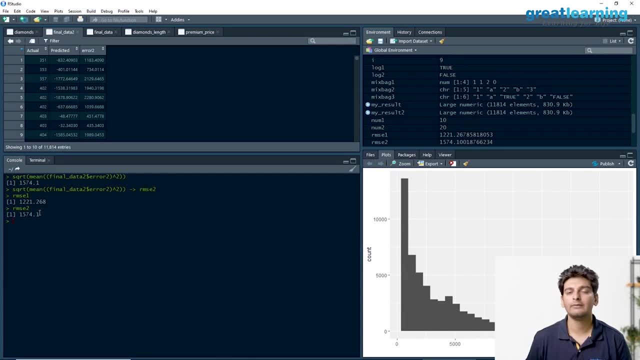 so for the second. so for the second model, the root mean square error is higher. this means that the first model is considerably better than the second model. so this is how we can put it: build multiple models and compare their accuracy with each other. So we have successfully implemented. 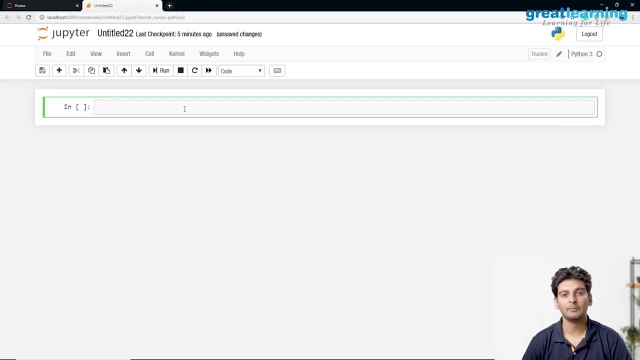 the linear regression algorithm in our language. Now it's time to implement the same in Python, and for this purpose we'll be working with the iris dataset. So my first task would be to load the pandas library. So I'll type in import pandas as pd. Now I'll be using the read underscore csv. 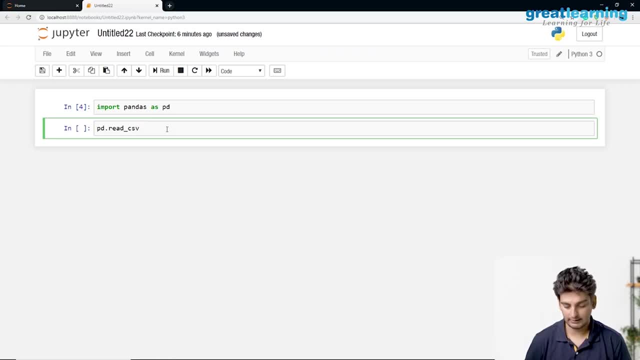 function. So I'll type in pdread underscore csv, and inside this I'll give in the name of the file, which is basically iriscsv, and I will store this in a new object. Now I'll name that object as iris. Now I'll have a glance at the head, So irishead, and this will give me the first. 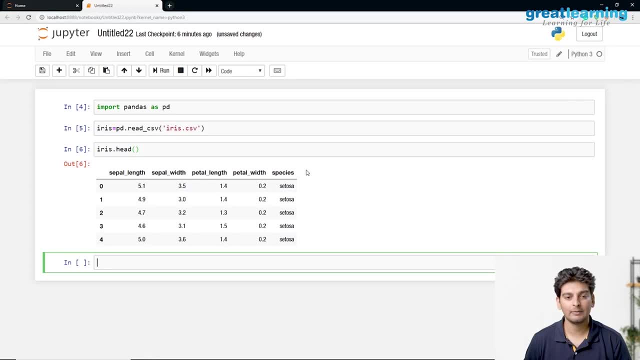 five rows which are present in this dataset. Now, this dataset is about the different species of the iris flower, which are cetosa versicolor and virginica, and these are the different features of these species. So we've got the sepal length, sepal width, petal length and petal width. 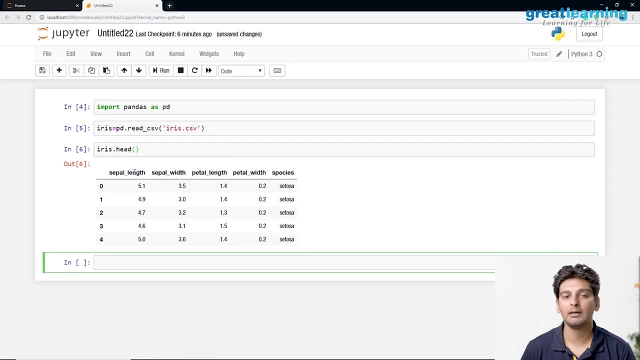 Now for this model. I'd want to understand how does sepal length of the iris flower vary with respect to the petal length of the iris flower? So sepal length would be my dependent variable and petal length would be my independent variable. So I'll go ahead and divide this entire dataset. 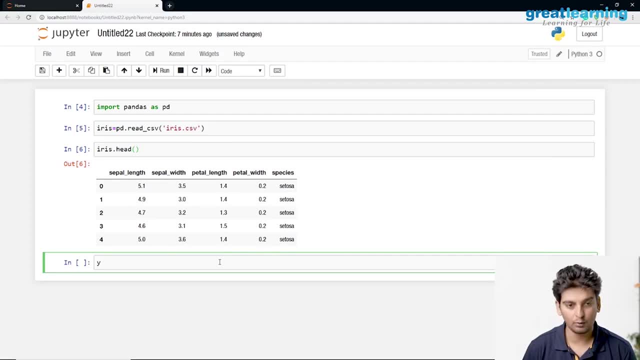 into the dependent variable and independent variable. So I will store the sepal length and petal length of the iris flower. Now I've written in the iris flower length into y. so to do that i will just given the name of the data frame, which is iris, and i'll give. 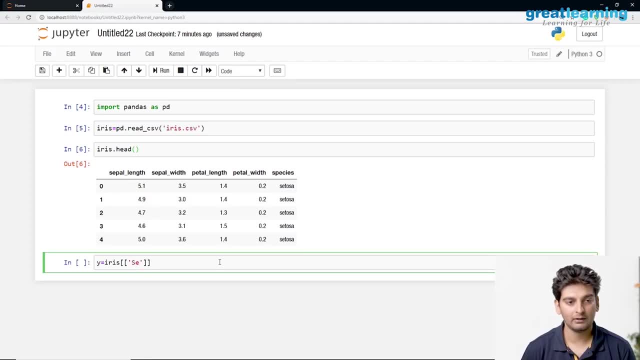 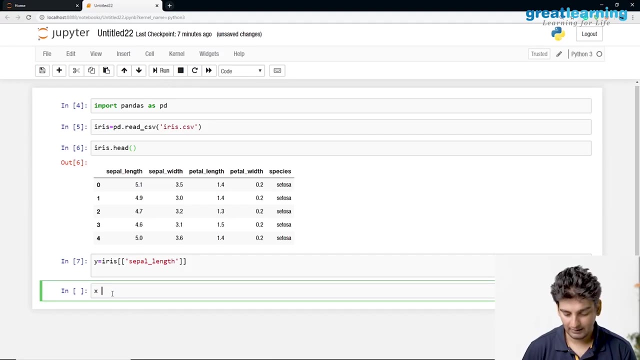 in double braces over here and i'll put in codes and i'll give in the name of the column, which is sepal length. so let me just type in sepal underscore length over here. so i am extracting this sepal length column and i am storing it into the variable y. similarly, i will extract: 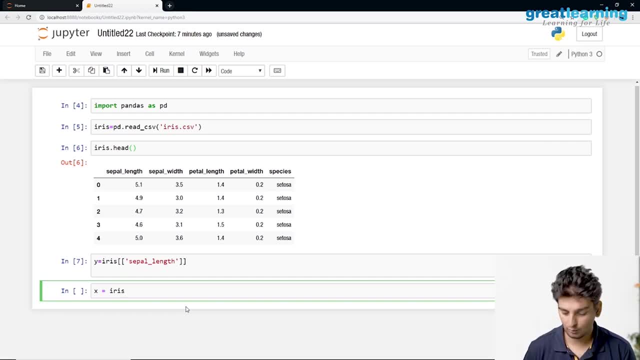 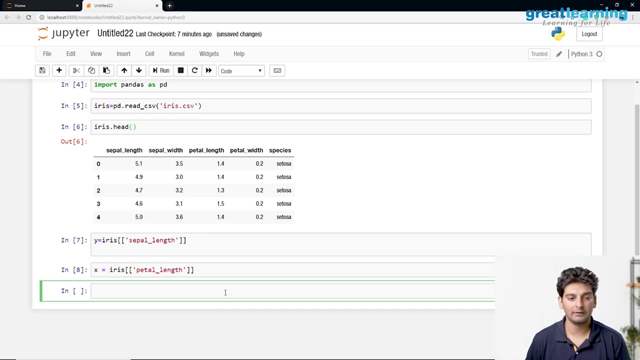 this petal length column from the iris data set and i'll store it into x. so i'll give in two braces over here and i will give in the name of the column which is petal underscore length and i am storing this into x. so i have my dependent variable and independent variable ready. 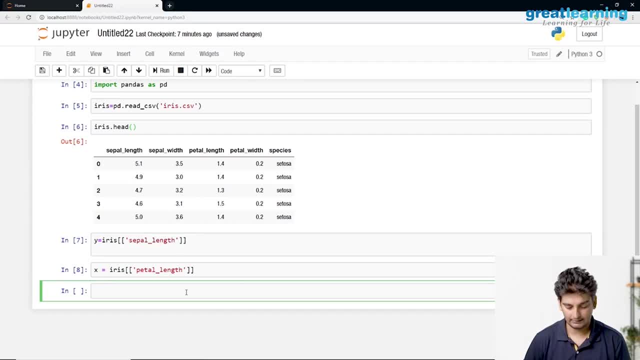 now it's time to divide these two into the training set and the testing set. so for that purpose i'd have to import the train test split method from the sklearn package, so from sklearn dot. it would be model selection. so i'll type in model underscore selection. 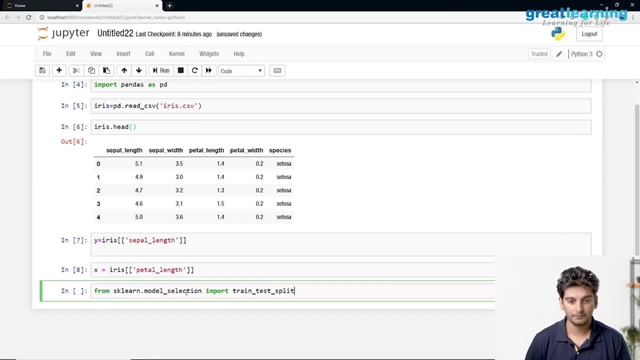 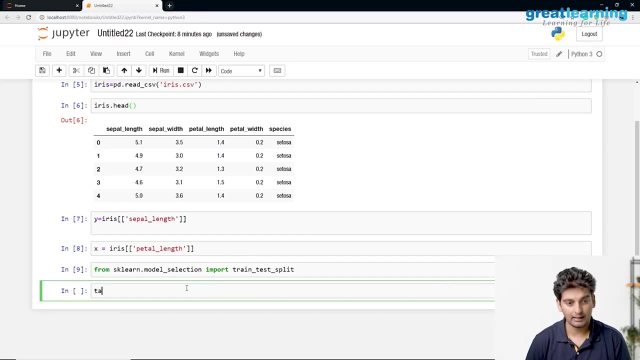 import of train test split. so i'll go ahead and import this method from the sklearn package. now what is done? i will use this function. so train test split. i will pass in the x value and the y value and then i'll give in the test size. so the test size would be equal to 0.3. 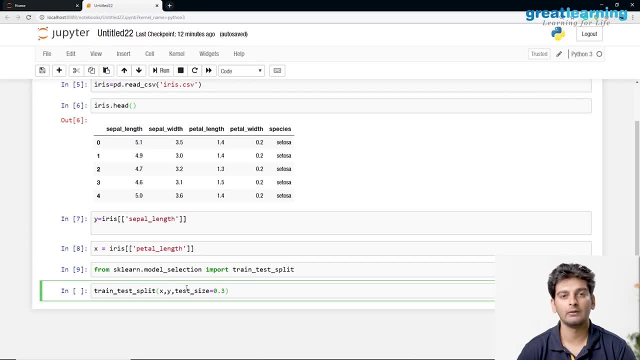 so this means that 70 of the records go into the train set and the 30 of the records go into the test set, and this would basically give us four results. so let me just type out those results. so the first result would be x train, and then we've got the. 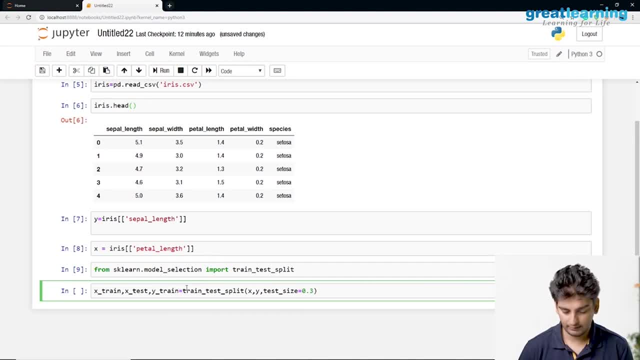 x test, after that we've got y train and then finally we've got y test. so what are these four variables? so x train is basically the training set of the independent variable, then x test is the test set of the independent variable. then we've got y train, which is the train set of the 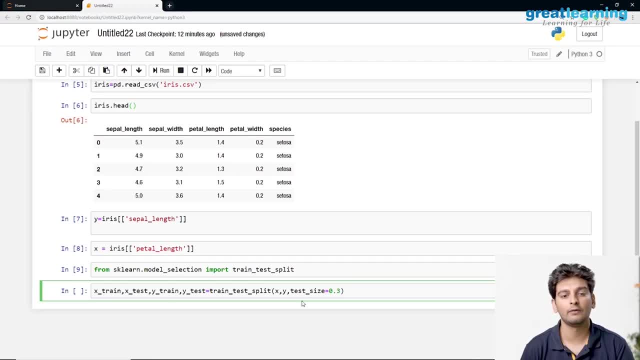 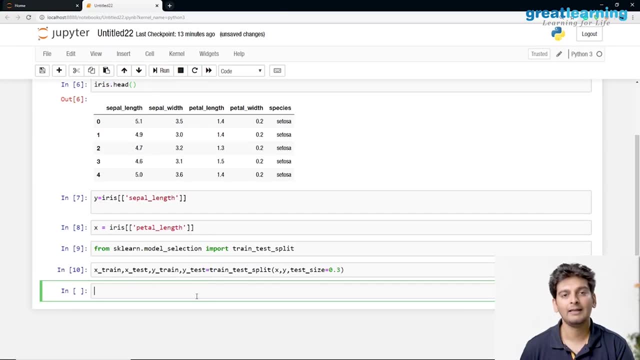 dependent variable. and then we have the y test, which is the test set of the dependent variable. so these are the four results which are given by train test split. so now that we have all of these, it's time to build the linear regression model on top of the train set. so i will import the 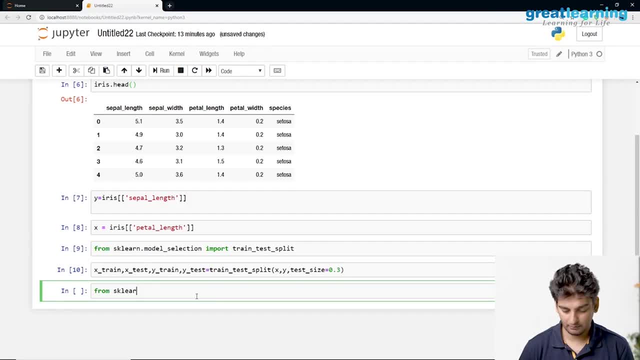 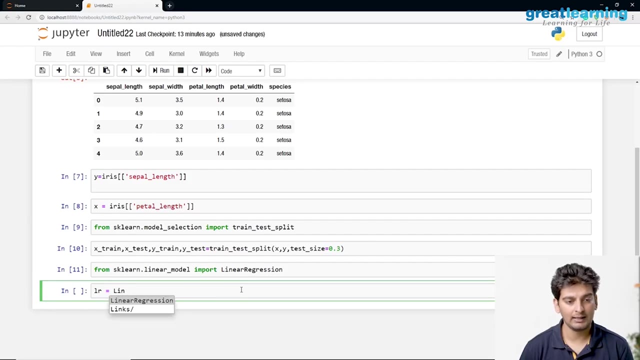 linear regression model from sklearn. so i'll type in from sklearn dot linear model. i'd have to import linear regression. so now that i import linear regression, i have to create an instance of it and i'll name that instance to be l r right. so i have successfully created an instance of this. 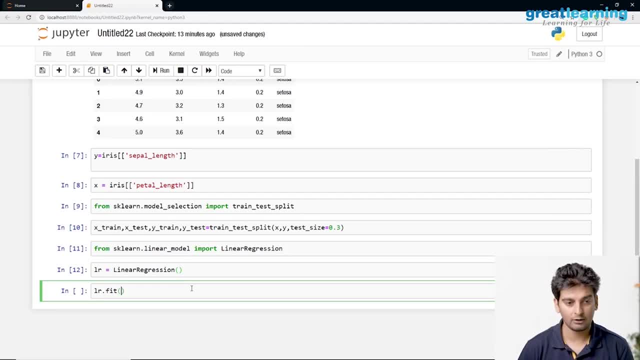 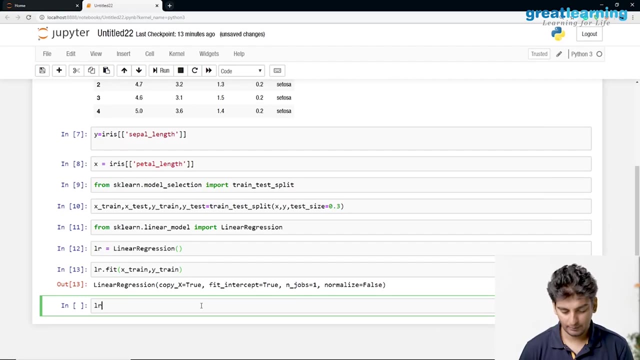 linear regression model and i'll go ahead and fit this on top of the train set. so l r dot fit. and i am fitting this on top of x train and y train. right, so we have fit this model. now it's time to break the values on top of the test set. 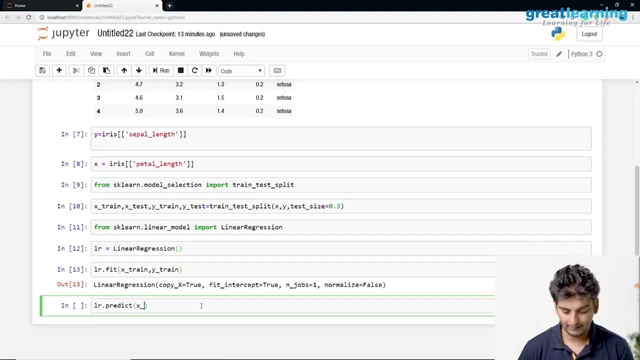 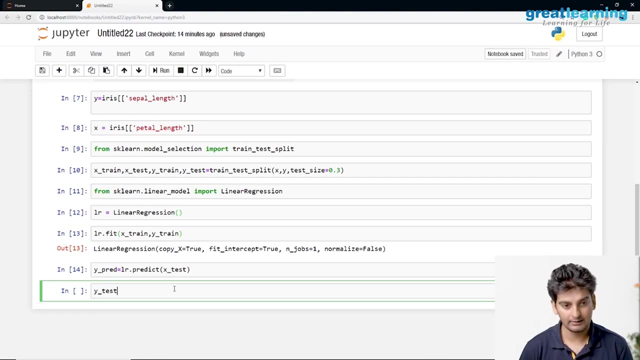 so we've got the predict function, so lr dot predict and we'll be predicting on top of the test set and i will store this in, let's say, y underscore pred. now we've got the actual values in the predicted values, so the actual values are present in y test. 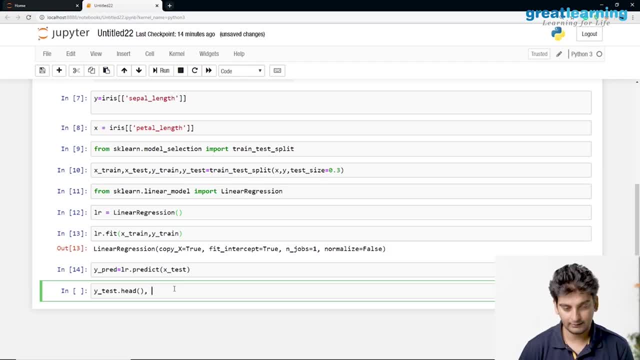 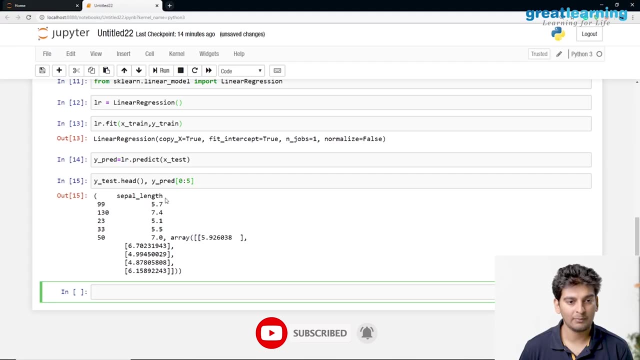 i'll type in y, test dot head, and then i've got the predicted values which are present in y. so this is a numpy array. so i want to have a glance at the first five records. so this will go from 0 to 5, actually, right? so these are the actual values of the sepal length and these are. 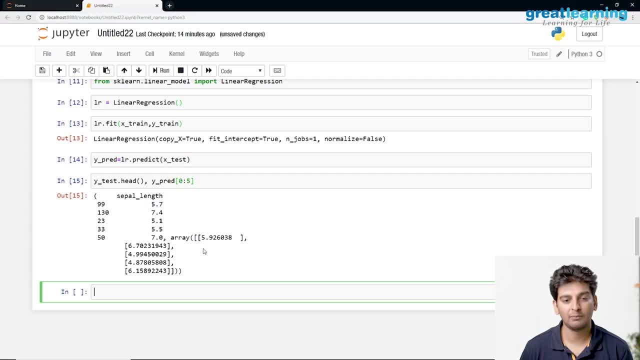 the predicted values of the sepal length. so the actual value was 5.7. the value predicted by this model was 5.9. the actual value was 7.4. predicted was 6.1. then we've got 5.1, which was predicted as. 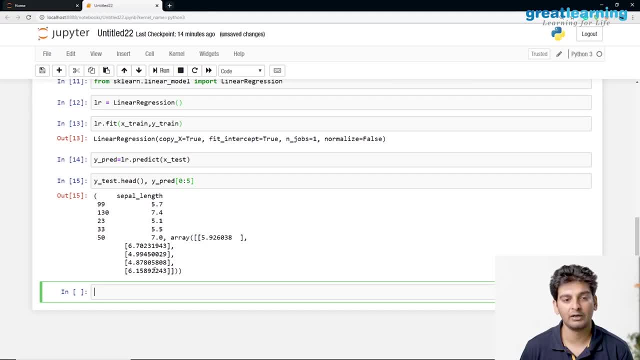 4.9. right, and if we take this value, 7, it was predicted as 6.1. so we've got the actual values and the predicted values. now it's time to find out the error in prediction. so i load the mean squared error from the matrix of sklearn. 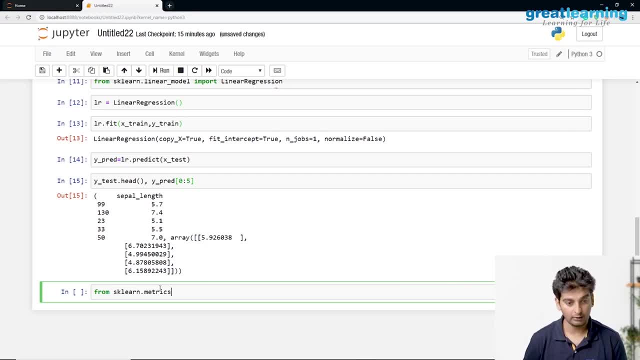 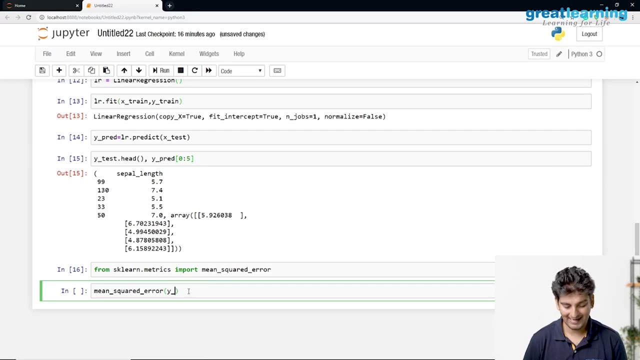 so i'll type in from sklearn dot matrix. i would basically be importing the mean squared error. so now that i import it i will go ahead and find out the mean squared error of this model and inside this i'll pass in the actual values which are present in 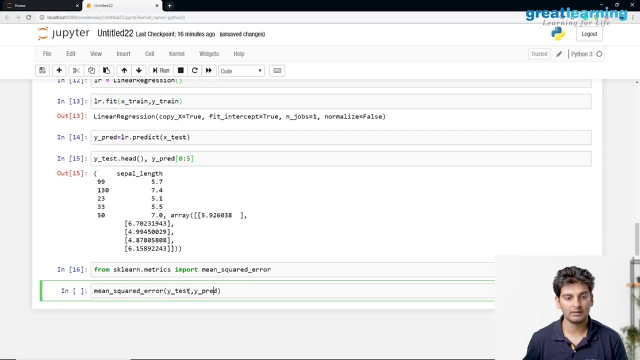 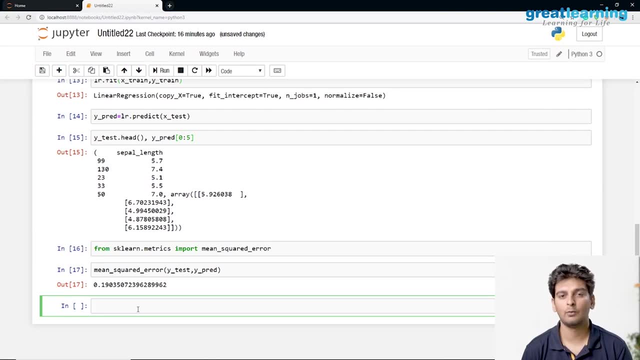 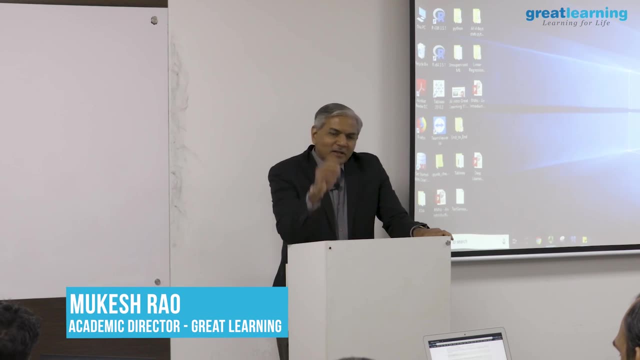 y test, and then the second parameter would be the predicted values which are present in y pred. so the mean squared error comes out to be 0.19, which is actually quite less. So seems that this model which you built is quite good. So in linear regression it is one of the most popular algorithms in production because it 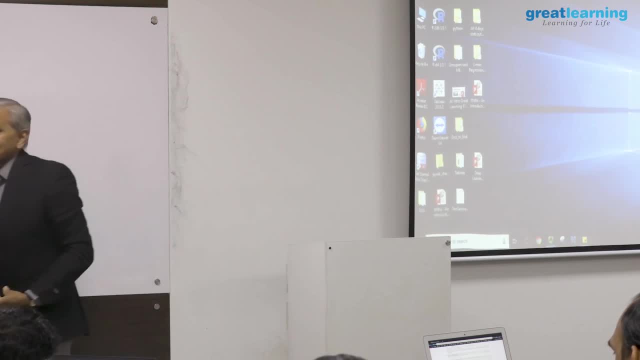 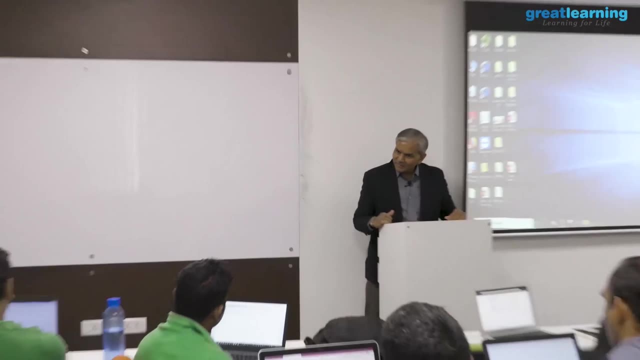 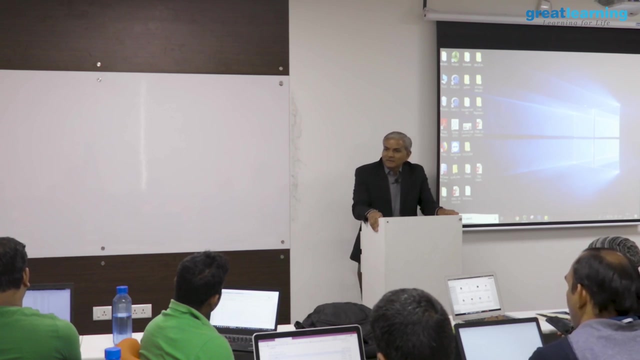 can be used for classification. it can be used for regression. It also happens to be one of the core algorithms that is used by many other algorithms. Logistic regression is a linear regression based model, right, If you take support vector machine- another very famous algorithm in data science, it is: 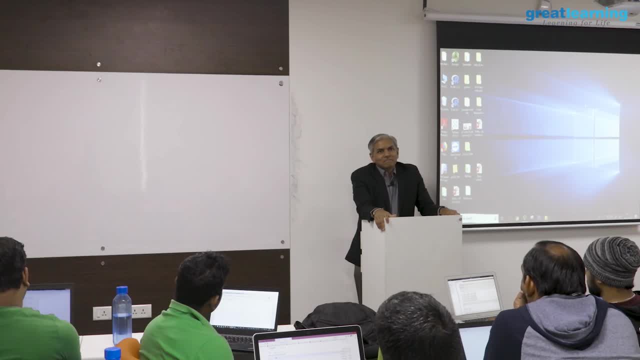 a linear model. or if you take, if you build, do linear models using binned data, what you call binned b-i-n. binned data sets- Then the model that you get It behaves like a decision tree right. 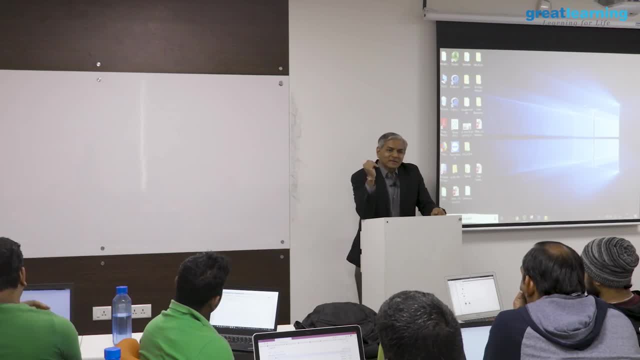 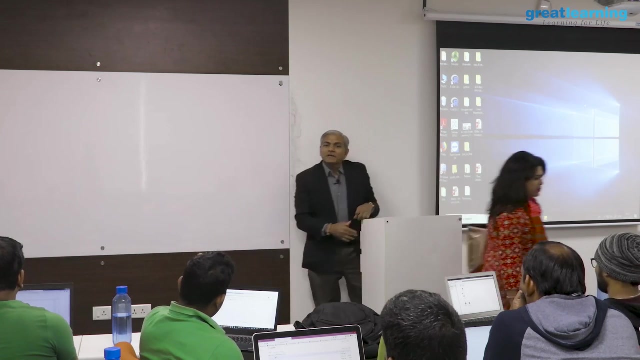 So many of the other algorithms which are very popular in the industry. internally, they are linked to linear models. You can spend your entire life time studying linear models. It has so much of depth and breadth that it takes lot of time to actually get used to. 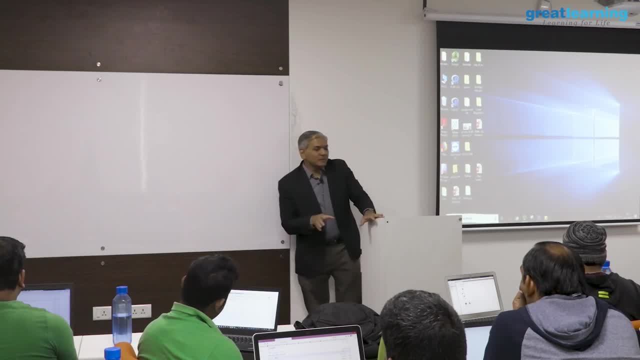 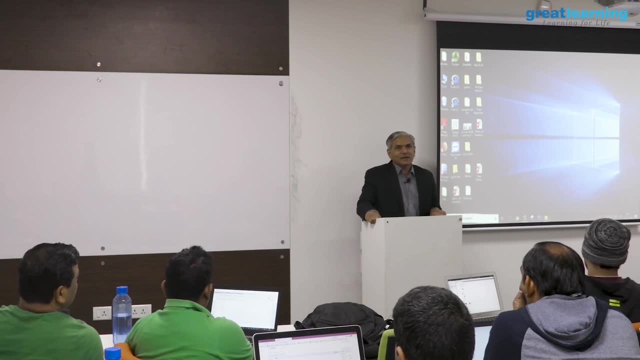 all these things. So today I am going to start by introducing you to simple linear models, The core concepts, and then subsequently I will leave some advanced discussions for the next visit where we will be covering FMT feature engineering model tuning. There we will discuss some further advanced concepts on linear models. alright, 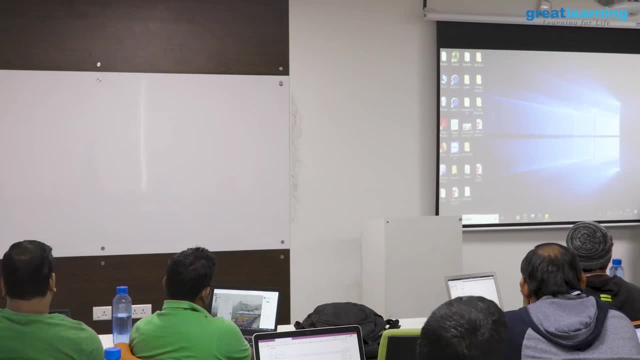 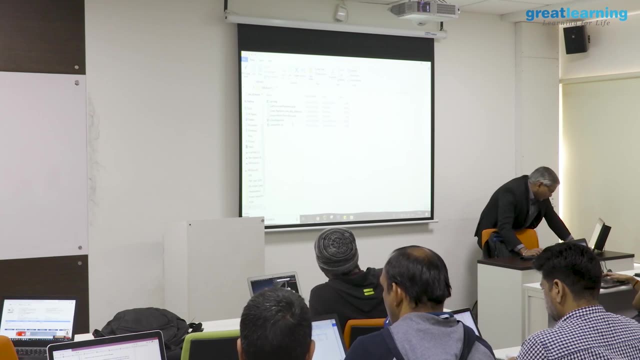 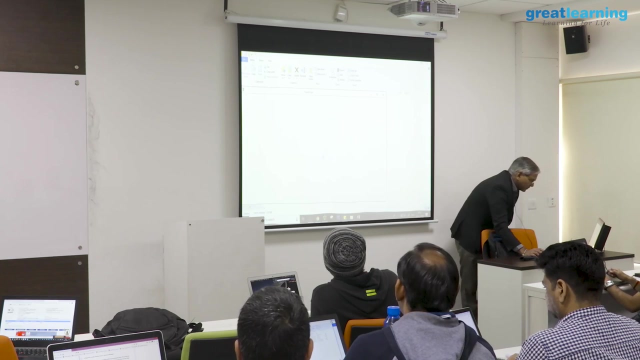 So I hope these people have loaded my. my team has loaded the data set, everything. I am going to give you three codes today, Of which I will cover one in the class. The other two is for you to go and explore further. ok, 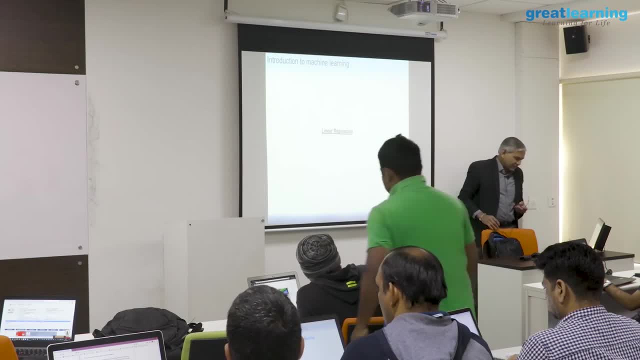 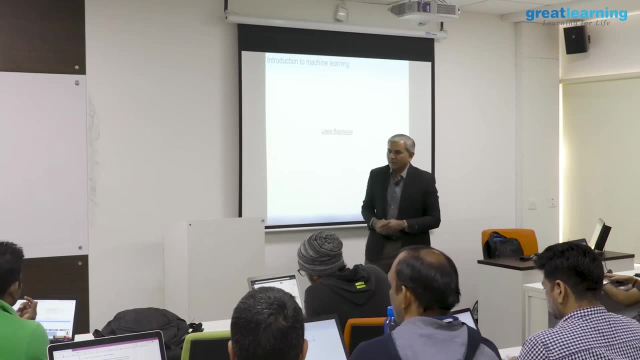 Based on what we discussed in the class, This PPT is accessible to all of you. Can you access this PPT? I think she has gone to you, can you can? ok, The code is also available: The PPT, the code, the data set. 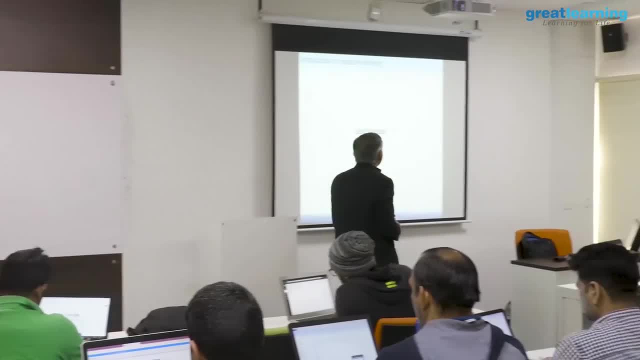 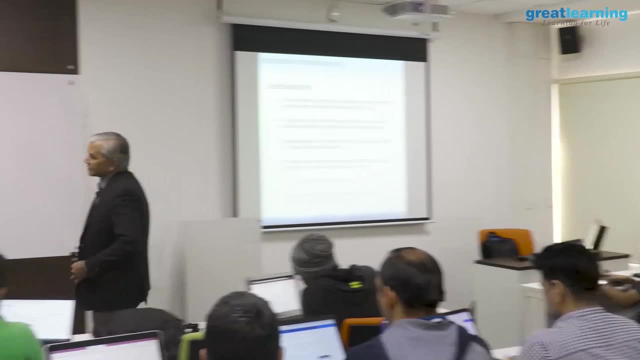 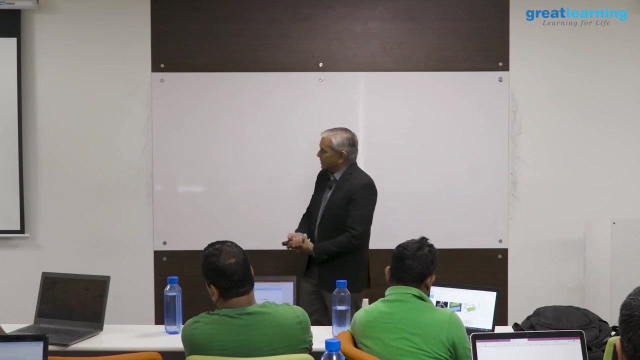 You should have received three codes, Alright, Ok, Ok, Let us start. As the name suggests, this algorithm is called linear regression, And the reason why it is called linear regression, as the name suggests, is it is based on the concept of a line. 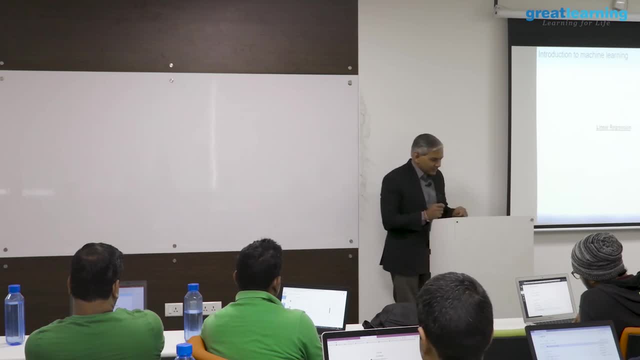 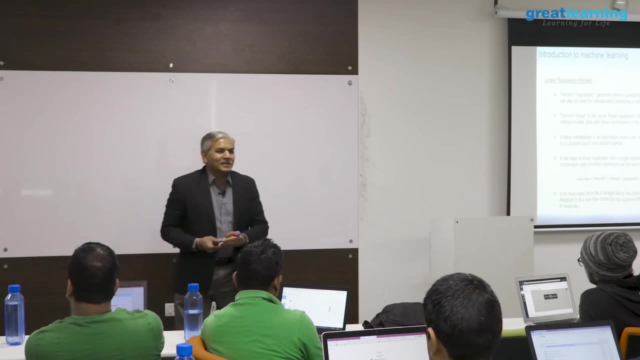 A line, a plane, a hyperplane- we call it by these names. ok, So to begin with, I need to ask you whether you know how a line is represented- Line line- in mathematics. Are you all comfortable with this? 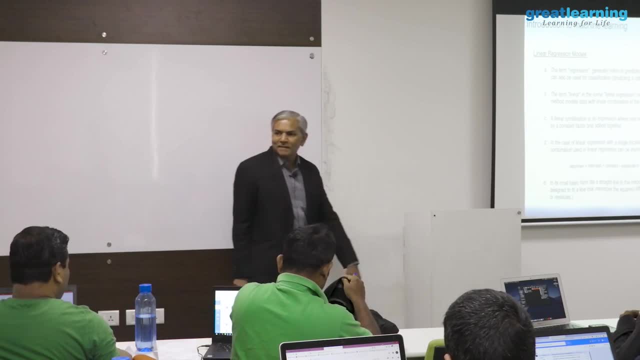 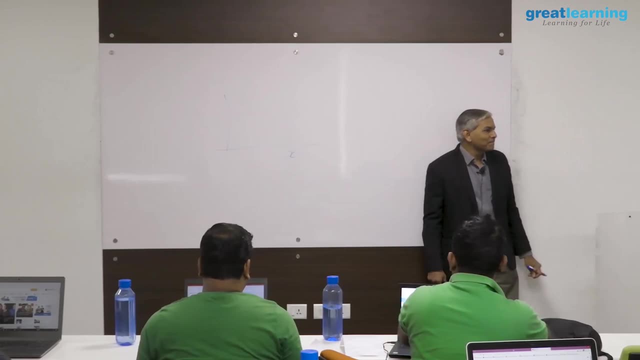 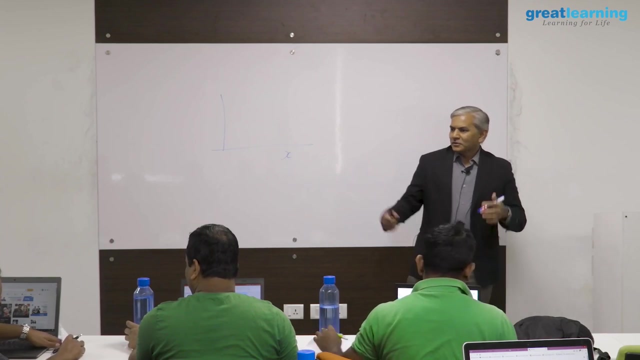 Alright, So let us start. Imagine I give you two dimensions. This is x. X is your, one of your independent attributes. We call it columns in our data frame, right? So I have loaded a data from a table into my data frame. 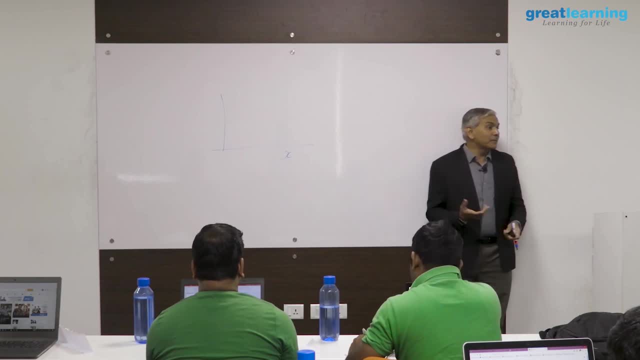 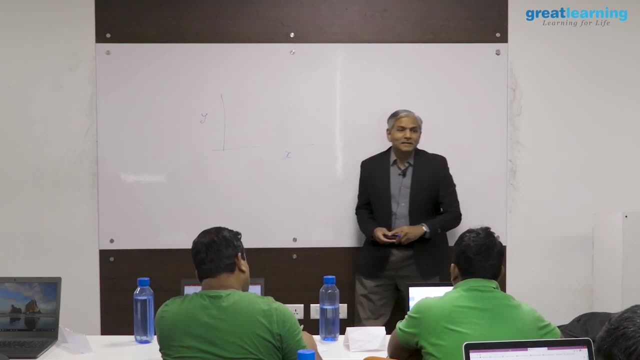 And one of the columns in the data frame. I call it x. This is my independent variable. The other column which I want to predict, the target column, I call it y, Could be anything. Y could be the miles per gallon. 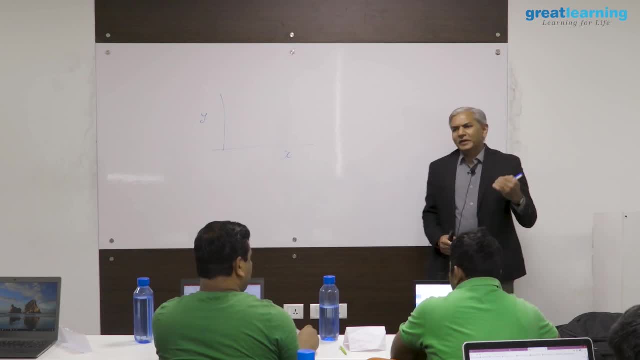 And x could be the weight of the car. The more the weight of the car, the less the miles per gallon. right, So y is my dependent variable, x is my independent variable. Imagine this: x has 4,, 5,, 6,, 7,, 8,, 9,, 10,, 11,, 12,, 13,, 14,, 15,, 16,, 17,, 18,, 19,, 20,, 21,, 22,, 22,. 23,, 24,, 25,, 26,, 27,, 28,, 29,, 30,, 31,, 32,, 33,, 34,, 35,, 36,, 37,, 38,, 39,, 40,, 41,, 42,, 43,, 44,, 45,. 45,, 46,, 47,, 48,, 49,, 50,, 51,, 52,, 52,, 53,, 54,, 55,, 56,. these are the units 1,, 2,, 3,, 4,, 5, 6.. 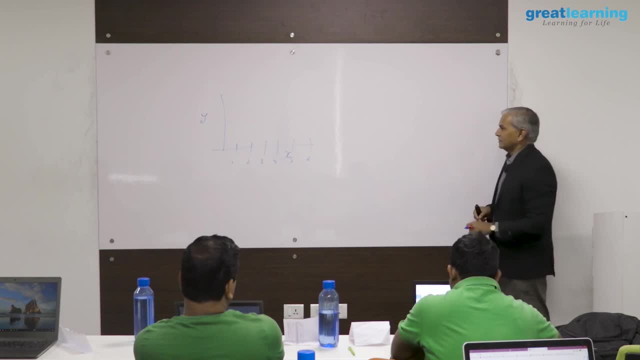 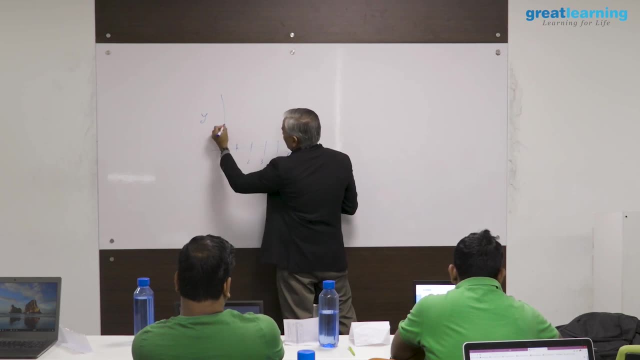 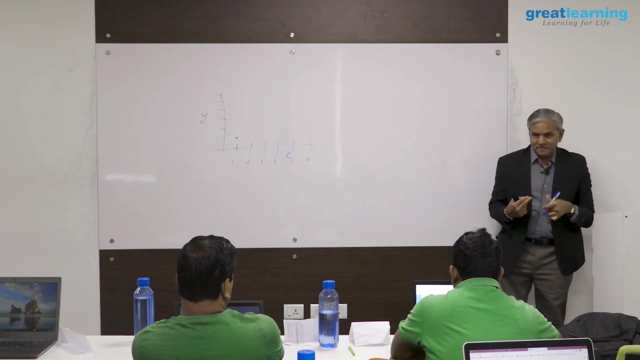 These are the measurements of x, And let us assume, for sake of discussion, let us assume- that whenever x is 1, y is also 1.. So, whenever x is 1, y is also 1.. That is what you are seeing in the data. 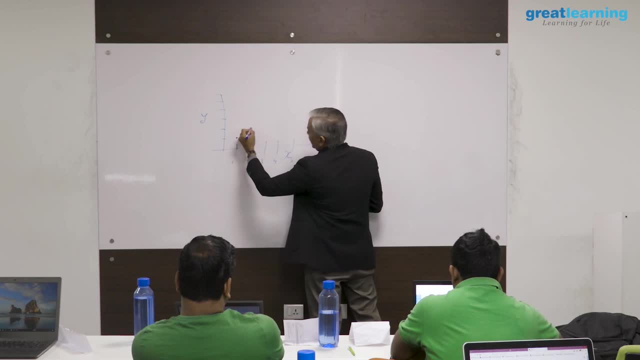 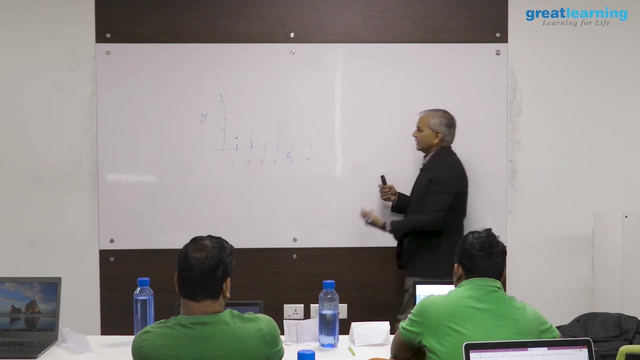 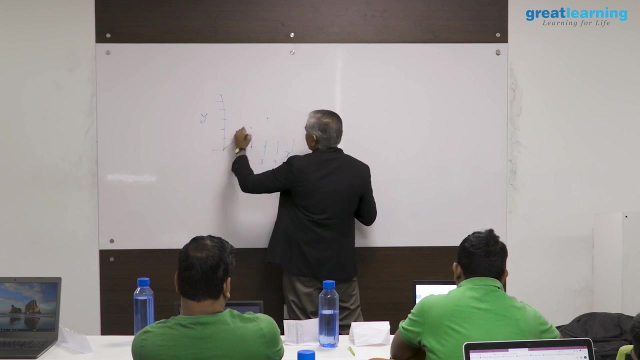 You take another record. There you see x is equal to 2.. Then y is also 1.. y is also equal to 2.. Take the third one: x is 3.. y is also 3.. So when you try to draw a line, a relationship between them, you see it is a straight line. 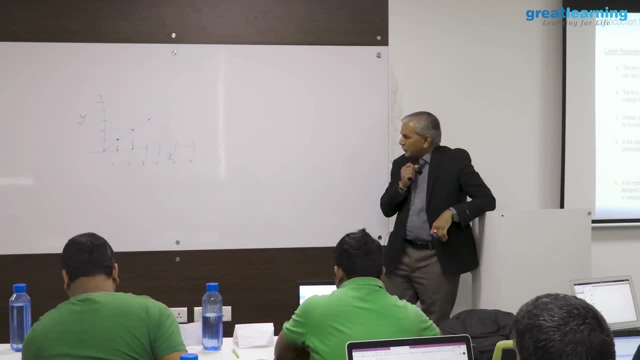 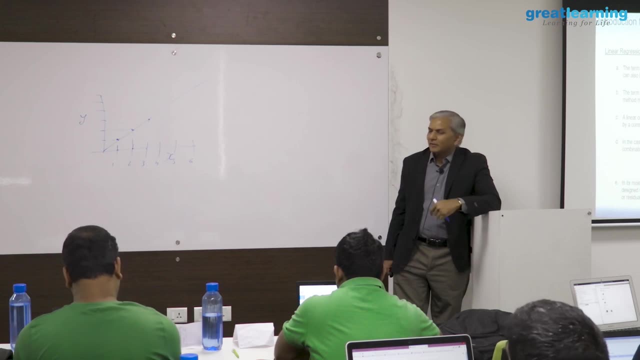 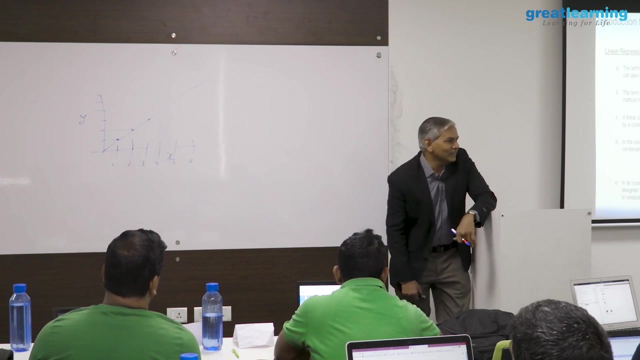 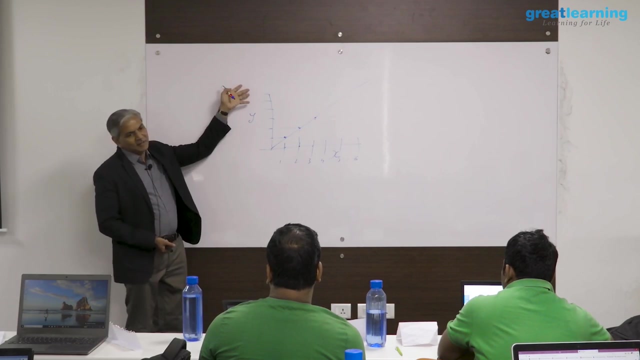 The straight line tells you the relationship between x and y. How are these two related to each other? We in data science call these things as models. Models are nothing but surfaces in your feature space. What is a feature space? Feature space is collection of your independent attributes and the dependent attributes. 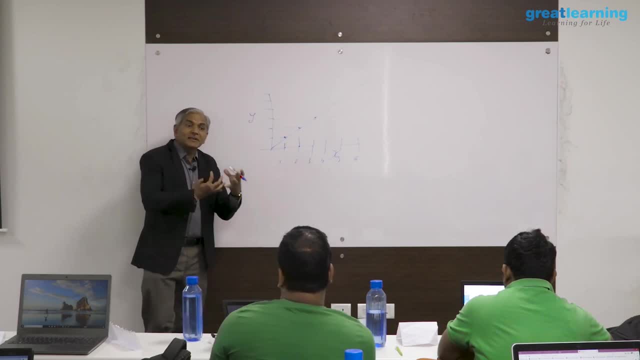 You are trying to explore how this y and this x interact with each other. That interaction is what we represented as models. So models are nothing but lines, surfaces, heights, And we call them as models. So models are nothing but lines, surfaces, heights. 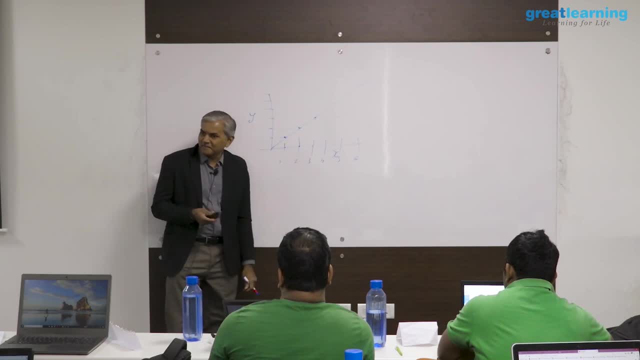 And we call them as models Because models and structures and models and structures are the member and they separate more like a breadthень ofetic layers from the other other layer and they are medium ofetic layers than the others. So a political example of this theory is we are teaching a fish as dimes. 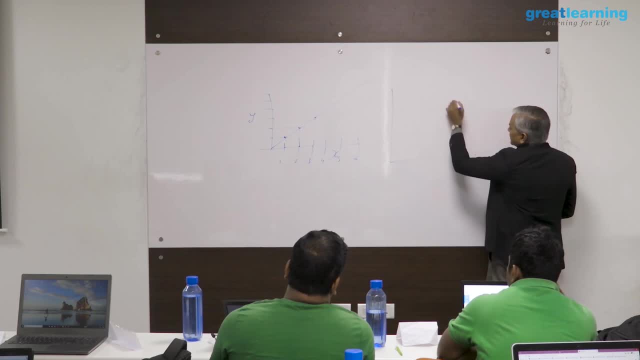 And a fish consist of a group that is longer than 3 meters, allows aSND of animal face, analyze it on the dimes And we keep it in good order for the individual to withel Ε to a PD L1. Sir Donald 표현. 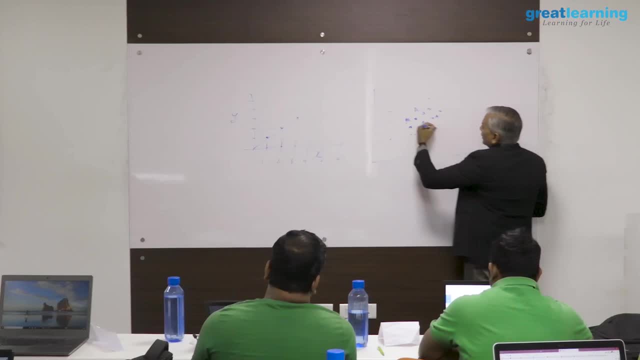 Okay, When you build k-nearest neighbors in k-nearest neighbors, you have different classes of data points. Suppose these are different classes And let me make it slightly more complex. standard systems, arems related to the radius of the dimensionallyGirl Zero and organizer region variables pies. that is the data. 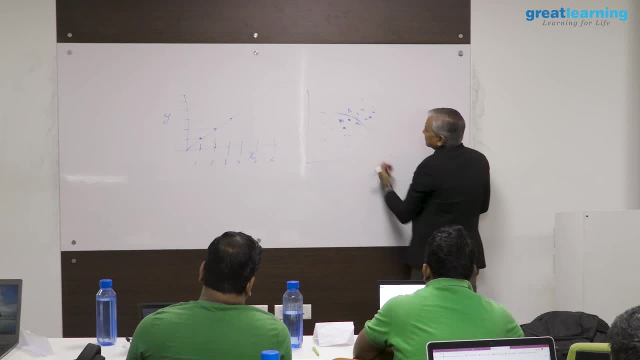 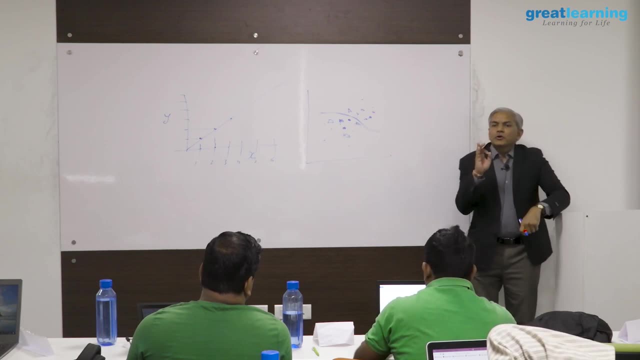 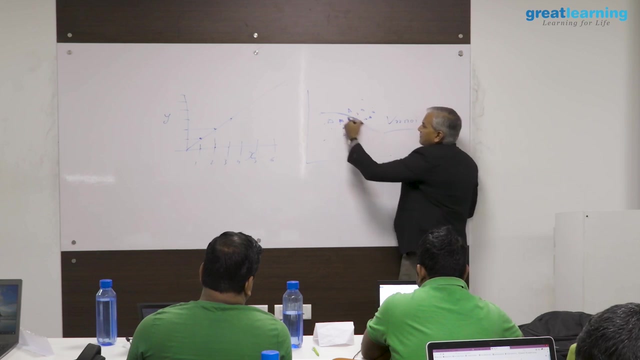 regions. so it says this region belongs to the circular point, this region belongs to the triangular point and you have things on the wrong side. K nearest neighbors splits your mathematical space into regions. Those regions are called Voronoi regions. So this imaginary surface is the model in K nearest neighbor. 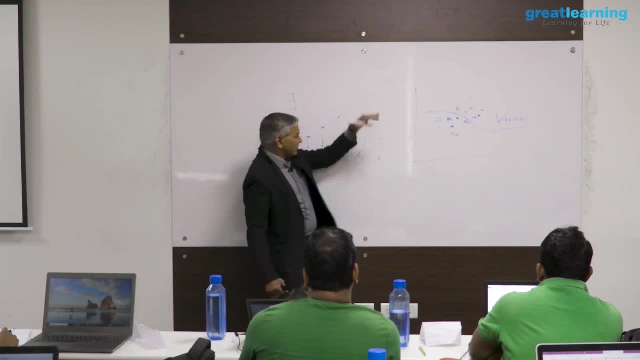 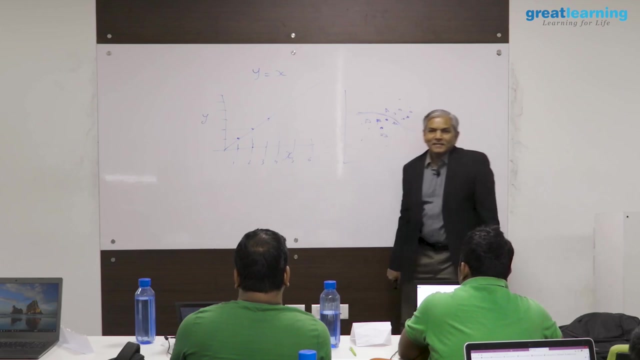 So in linear regression, this line which represents the relationship in x and y, this line is my model. So I want to predict the value of y given the value of x. What the line is saying is: y is equal to x. So the prediction is: whenever x is some value, y will also be the same value. 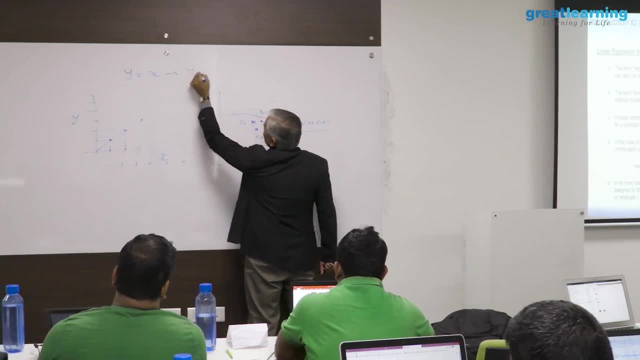 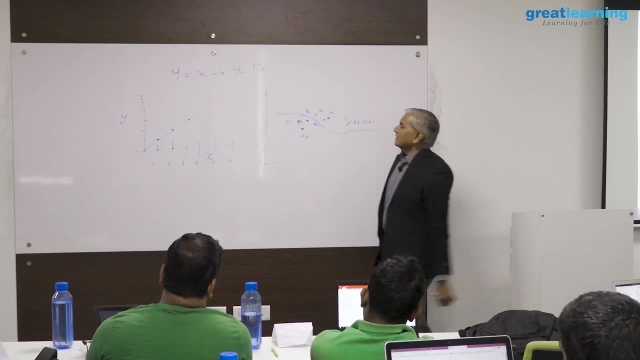 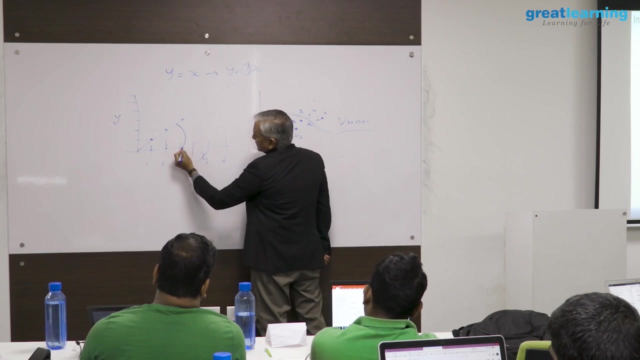 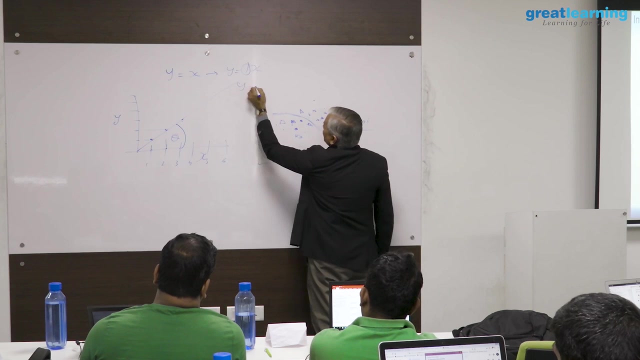 Can I write this expression as y equal to 1x? Does it make any difference? 1 into x, This 1, in mathematics it has a meaning. this 1 is nothing but this angle. that line makes, with the x axis, the tan of that angle, of that angle into x. 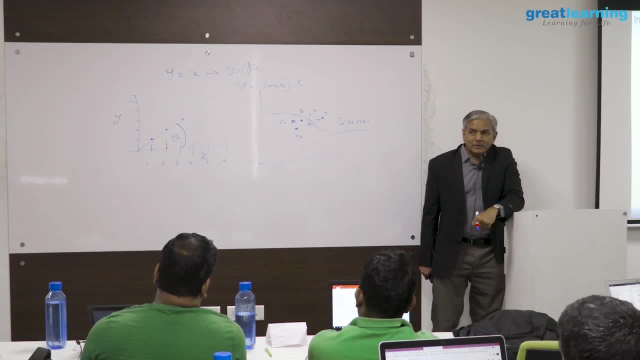 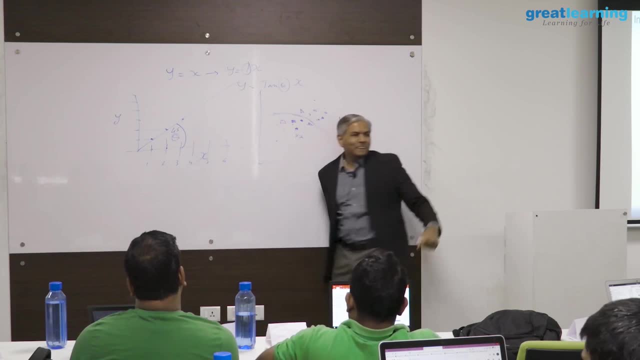 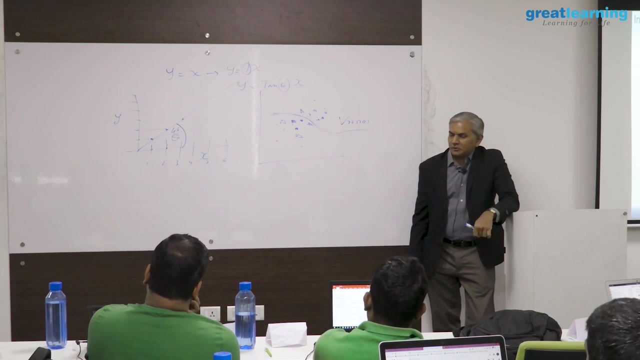 Ok, Ok, Whenever y is equal to x, this angle will always be 45 degrees. ok, And in trigonometry, tan of 45 is always 1.. Now you might be wondering: what is this trigonometry, tan, t, tan, all these are all jargons. 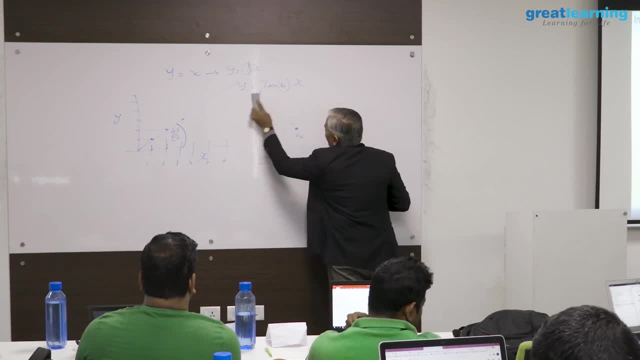 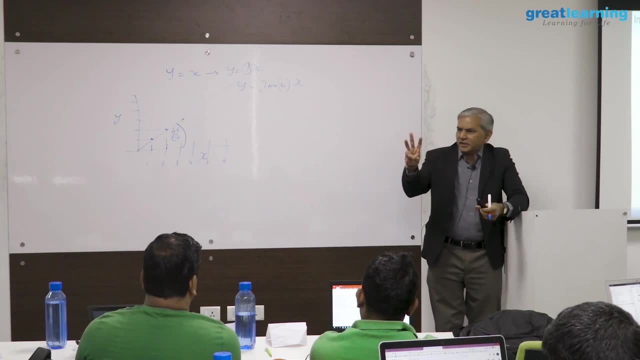 Actually, it is all common sense. Look at this. Ok, Ok, Ok. When we studied in school, we came across trigonometry. in trigonometry, we came across: sine theta cos theta tan theta, What are these? sine theta cos theta tan theta, what are these things? 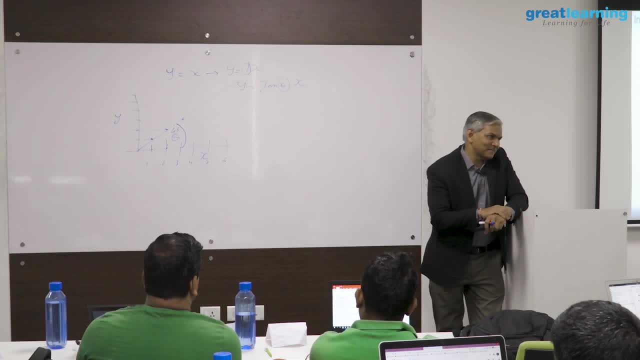 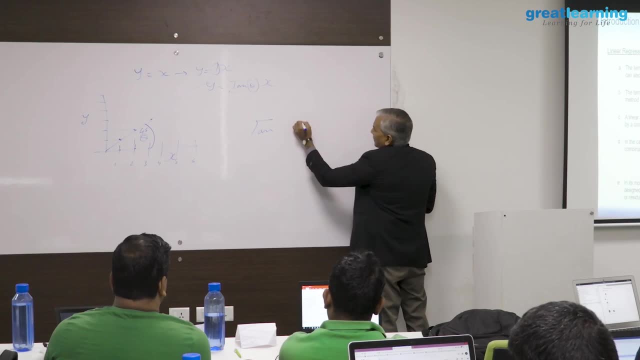 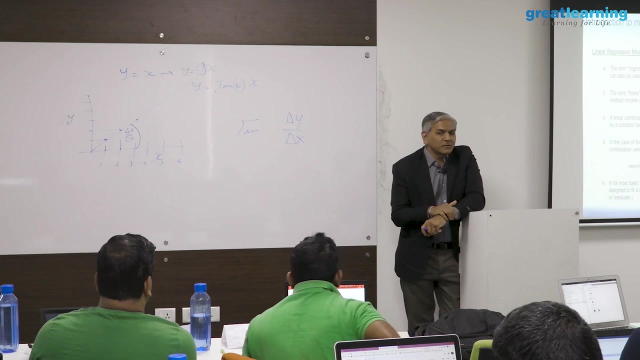 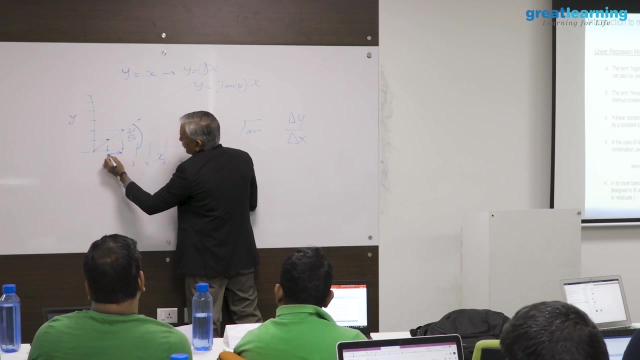 These are names given to certain ratios, So tan theta is. tan means the ratio between: we show it as dy by dx. how much y changes whenever x changes by 1 unit. That ratio is called tan. How much y changes when x changes by 1 unit. 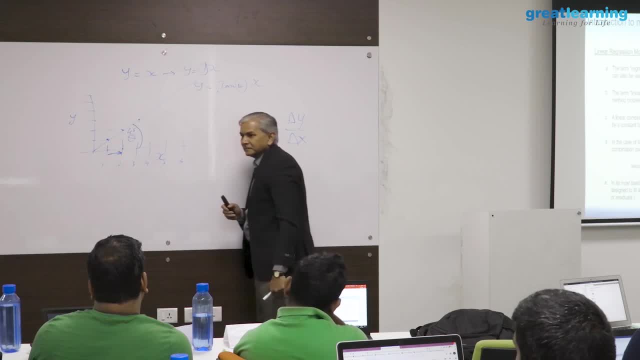 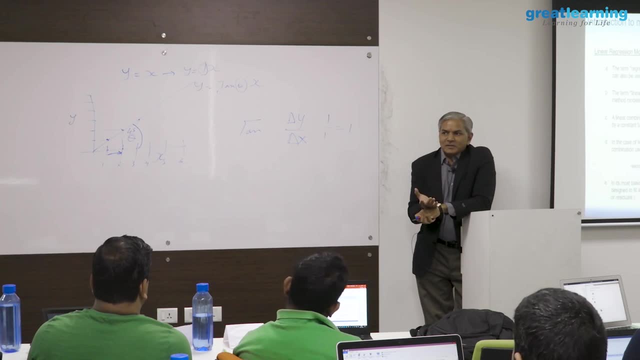 How much y changes in this graph when x changes by 1 unit. So 1 by 1 is equal to 1.. dy by dx. how much y changes by small change in x: 1 unit change in x. That ratio is called tan theta. 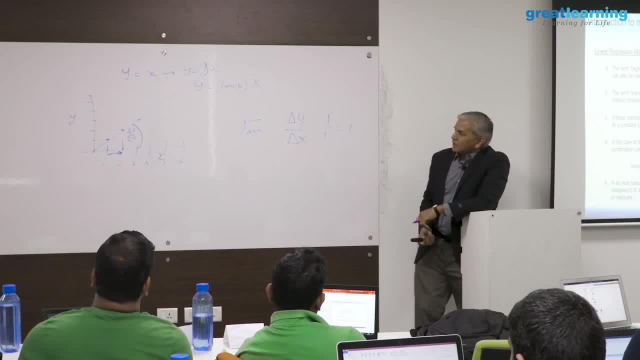 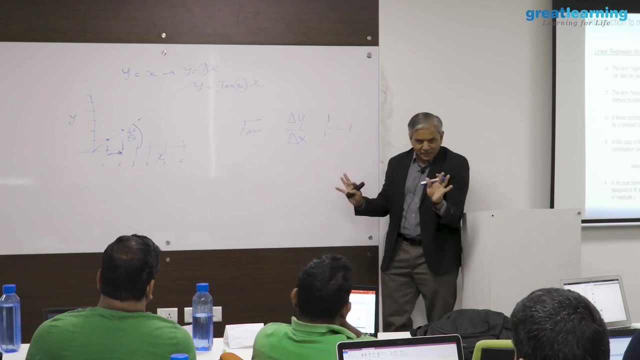 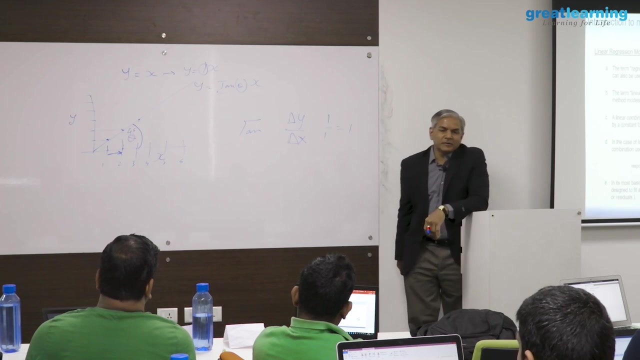 Sounds very high five, but that is what it is, Ok. Ok, So both of them synchronize. whenever x changes by 1, y changes by 1, it will always happen when this angle is 45. So we say that tan of 45 is 1.. 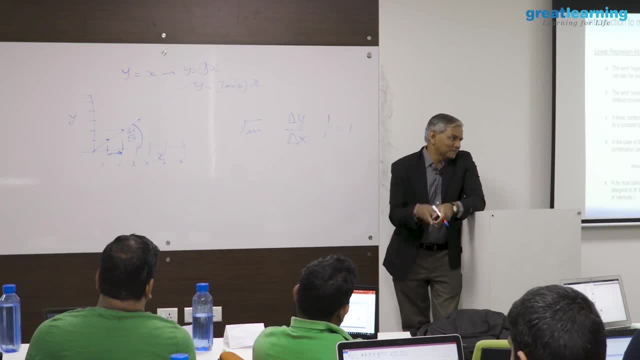 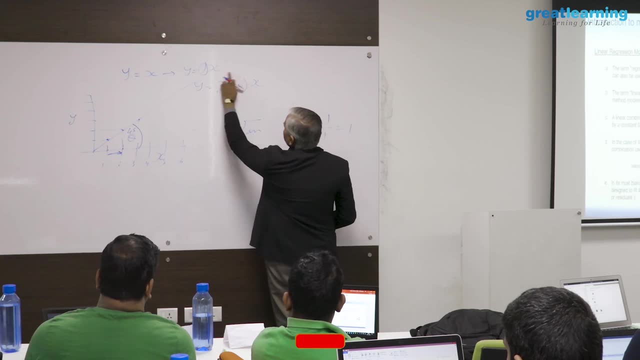 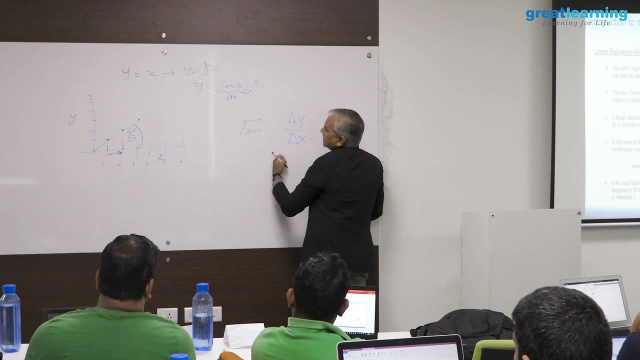 So when you say tan of 45, dy by dx will be 1 by 1, it will always be 1.. Alright, Let me modify this a bit. So right now this expression is represented as m. Ok, This is the standard practice, where we represent it as m. 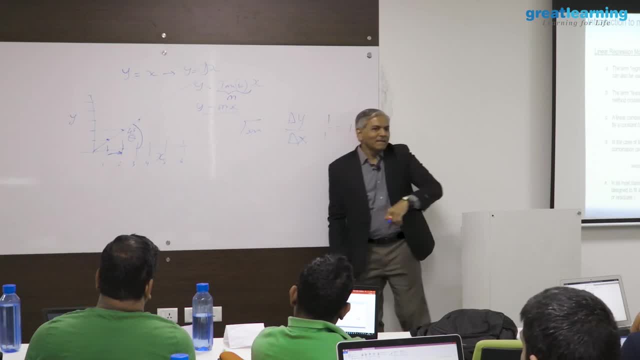 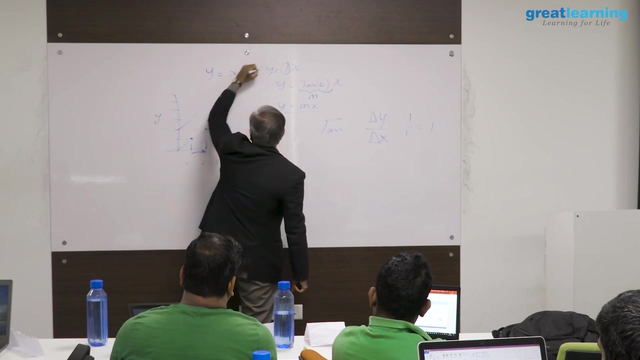 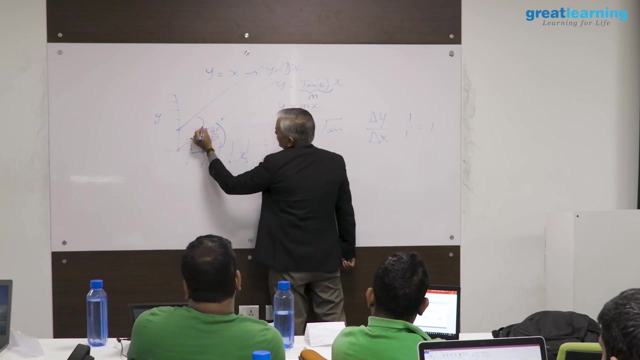 So y equal to mx is the expression mathematical expression of this line. Suppose I put a line here, ok, and it is parallel to this line. It is parallel to this line, ok, which means this line is also making 45 degrees to the. 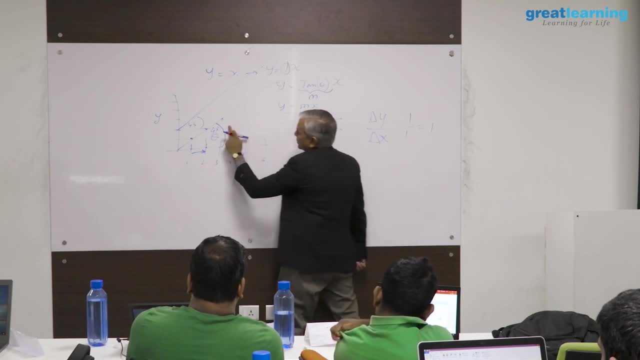 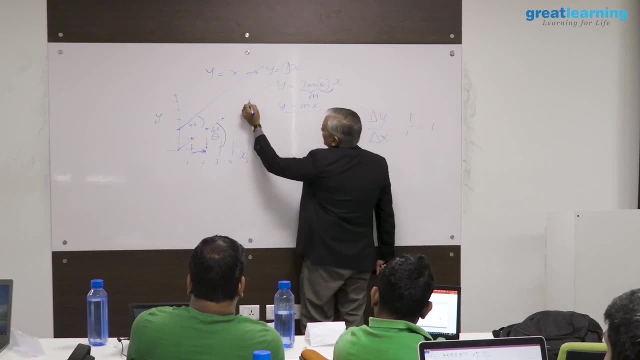 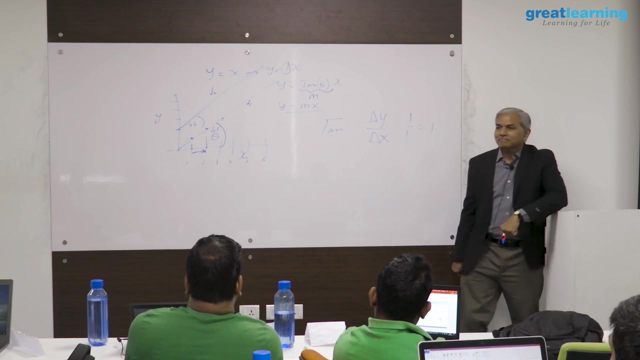 line parallel to x axis. I am not going to show this line here, ok, just to make it less cumbersome. So I have another line here. this is l1,, this is l2.. Now can I say: y equal to x. 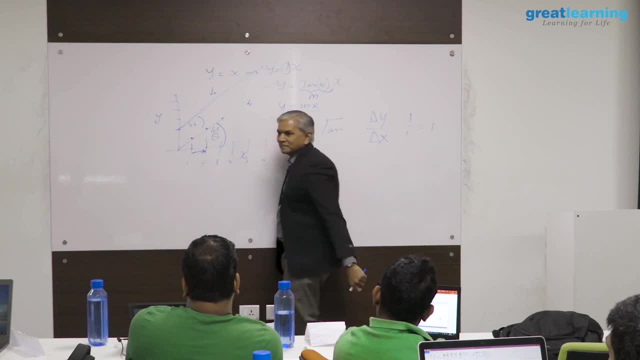 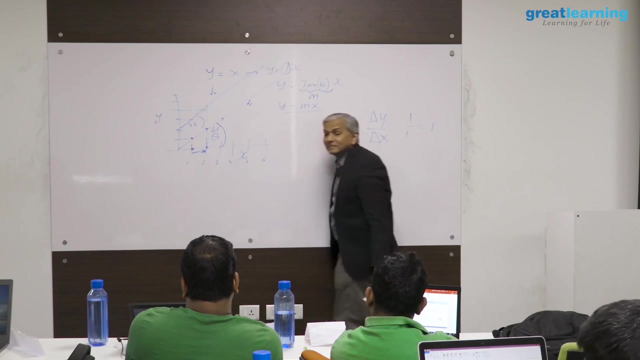 When x is 0, y is not 0,, y is 2, when correct: when x is 1, y is not 1, y is 3.. When x is 2, y is not 2, y is 4.. 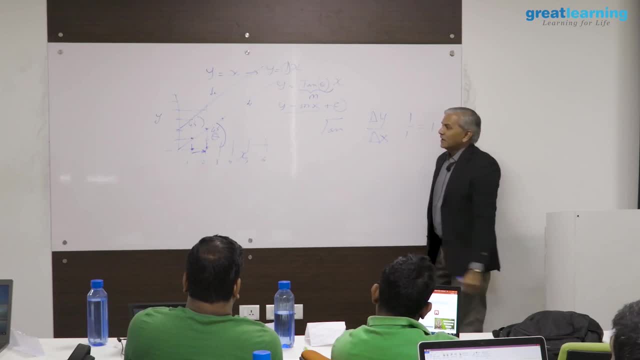 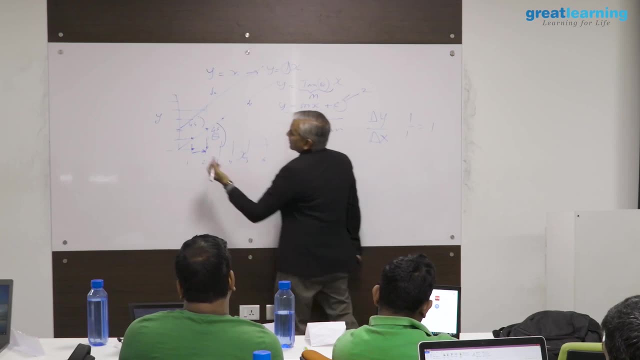 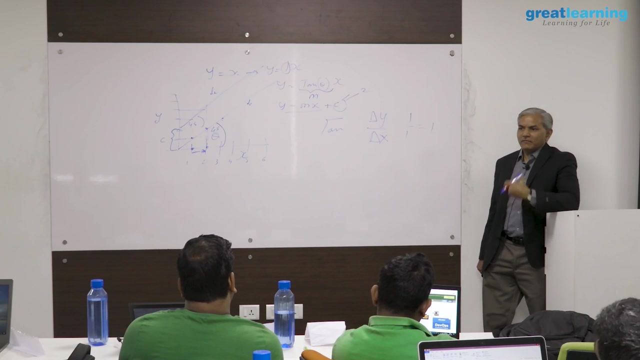 So we add a constant to this. This constant is equal to 2 right now. for this line, This constant is nothing. but what is the value of y when x is 0?? What is the value of y when x is 0?? 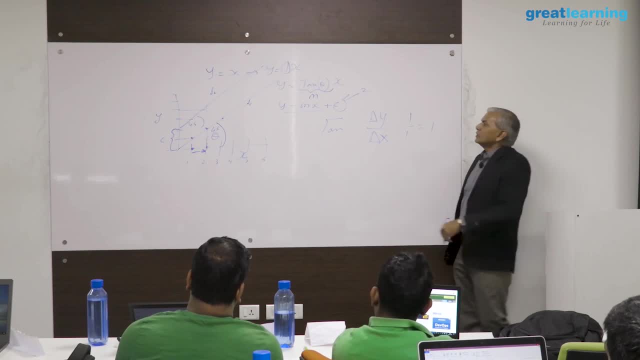 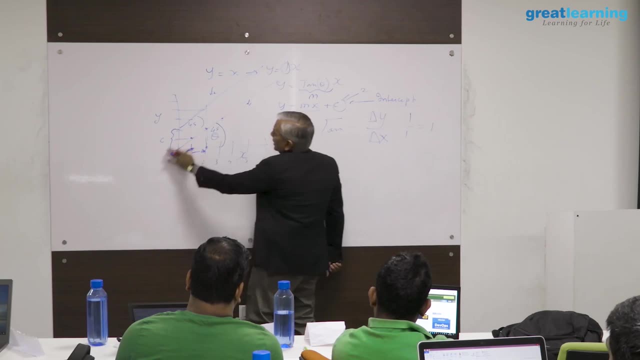 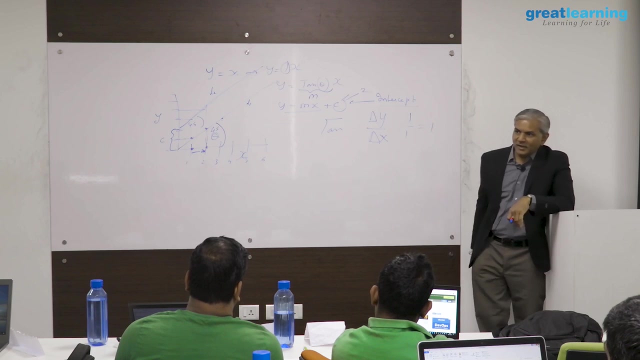 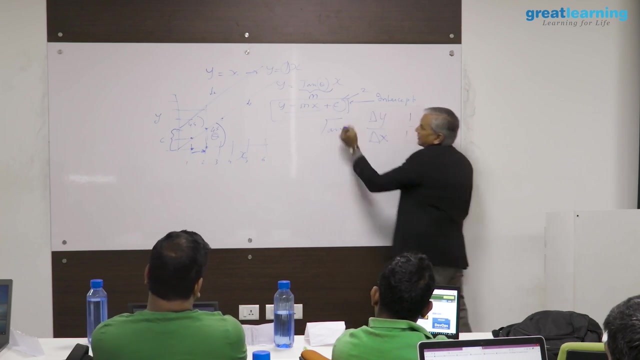 That is called c. It also goes by the name of intercept. Where in your mathematical space, on the y dimension, where on the y dimension, does the line intercept or cut the y axis? So this is the generic equation of a line y equal to mx plus c. 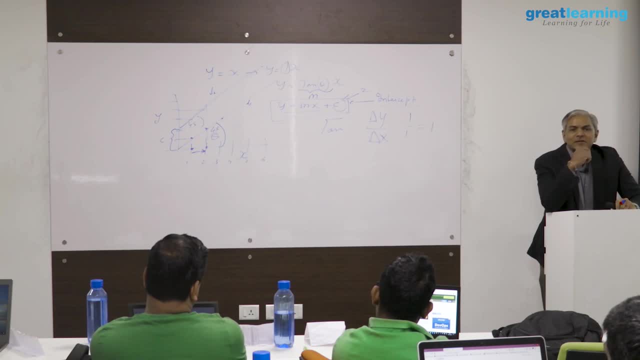 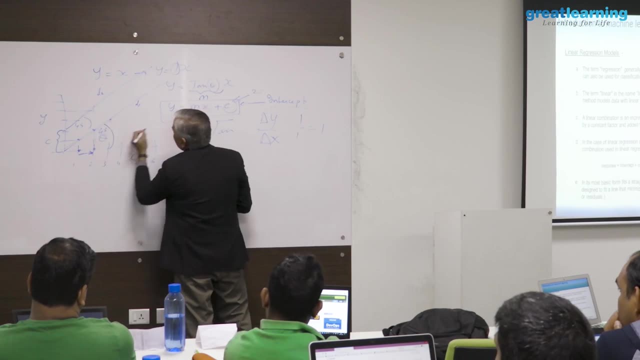 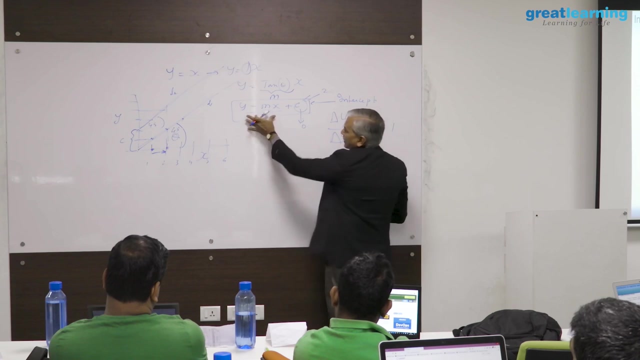 It tells you how to do it, How y and x are related to each other. If you look at this line, l1,, if you look at l1, then this becomes 0. So y equal to mx. If you look at l2, l2, this becomes not 0 but 2.. 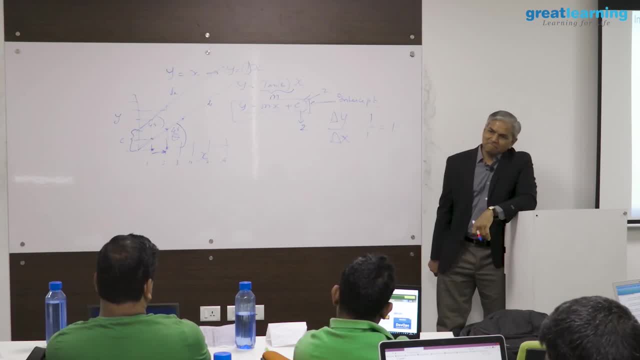 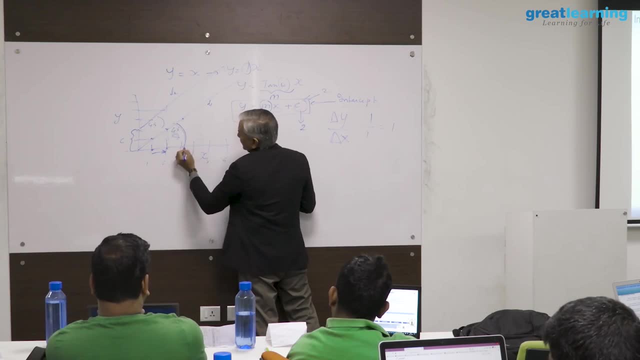 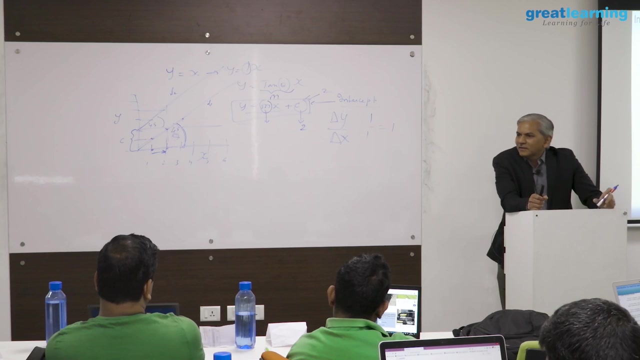 So this relation continues to remain same. In both the cases the m is 0.. The m is 0. This is the same. m is nothing but tan of the 45 degrees We call it slope. So this is the generic equation, one way of representing a line y equal to mx plus c. 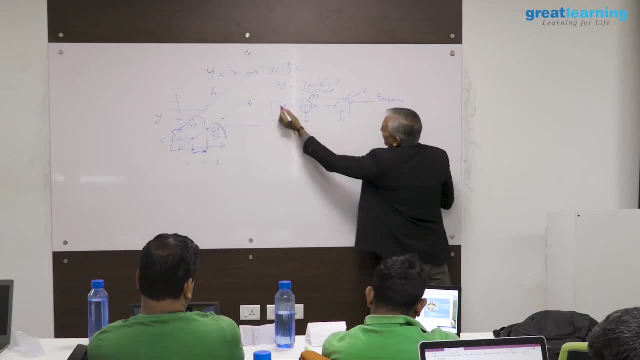 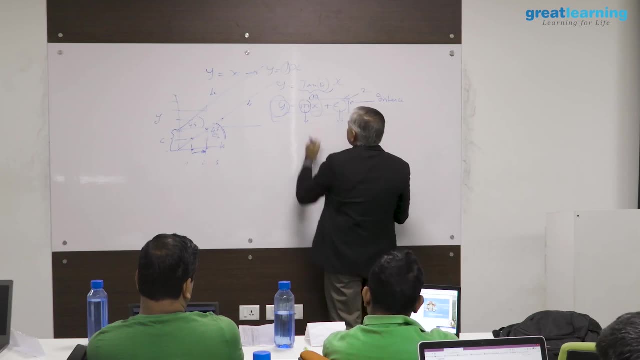 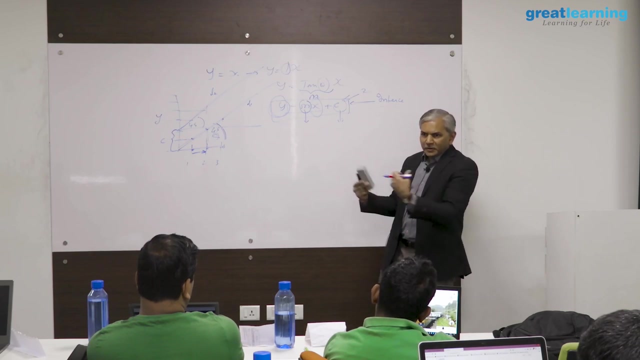 So in this expression, y is given in your dataset, It is a target column. X is given in your data set, It is the independent columns, the independent attributes From this data that you have given to the algorithm. the algorithm has found out for: 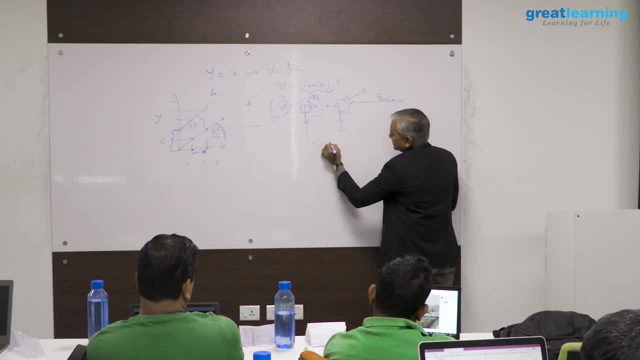 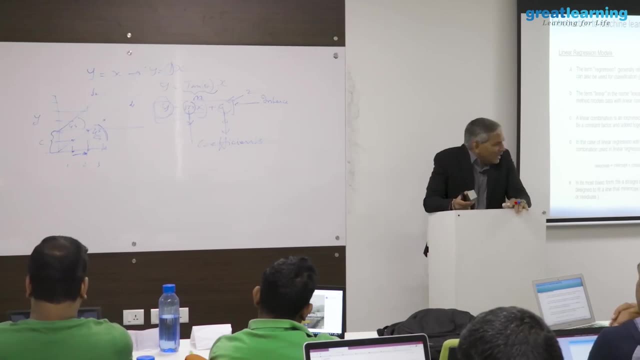 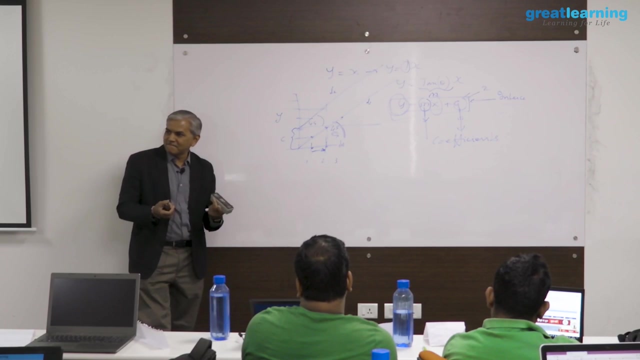 you the M and the C. We call these coefficients coefficients of the model, This M and the C. they reflect the relationship between Y and X in your data set. So the M and the C is what forms the model for you. Shall I complicate a bit more? 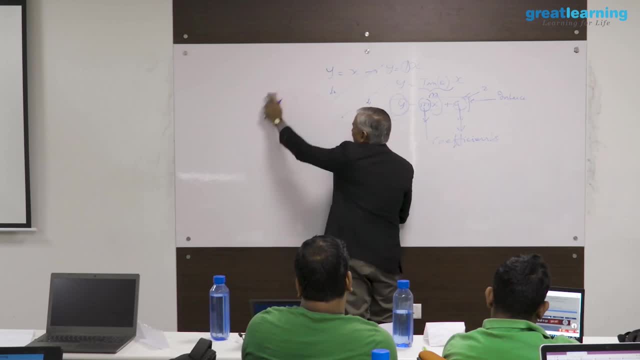 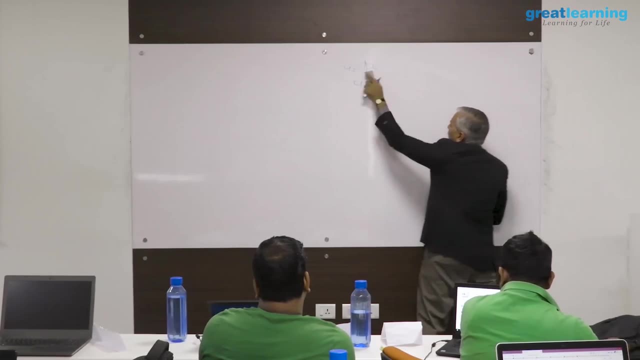 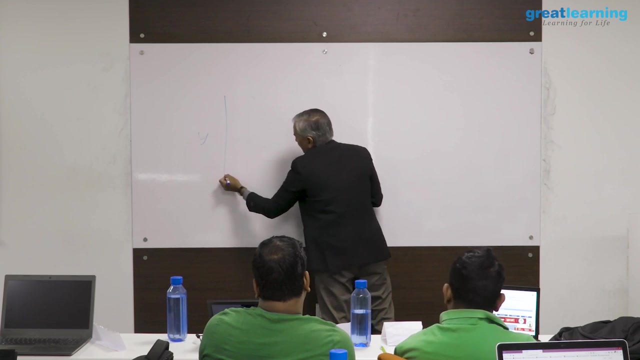 We will complicate a bit more. Suppose, instead of having 1, or let me just continue with this- only So you have one target variable Y, one X. In this case, tan of 45 happened to be 1.. But suppose your line is like this: 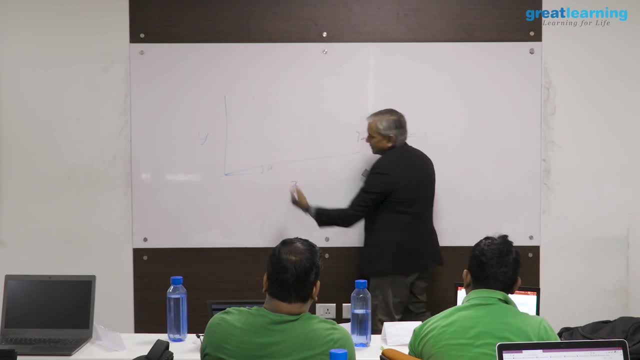 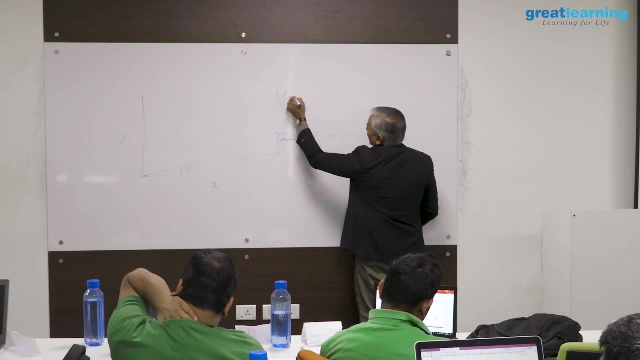 It is a straight line, but it is not at 45 degrees, it is at 15 degrees. Then in that case also the equation of the line, The line will be Y equal to M- X. the reason why I am not putting C is C is 0 here. 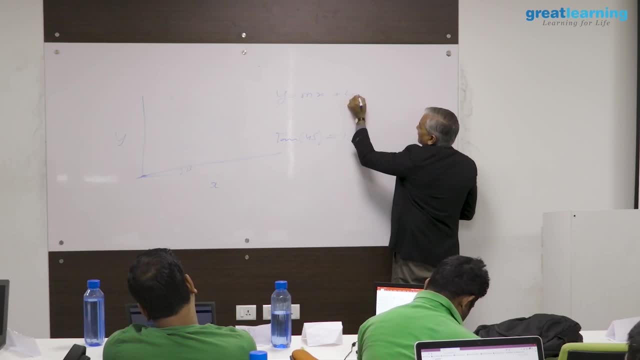 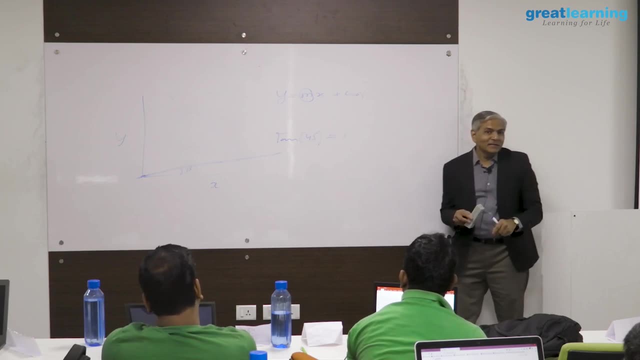 C is 0. You can put C, but C is 0. And this angle M, this value of M, will not be 1.. It will be 1 only when it is 45 degrees. it is less than 45 degrees. 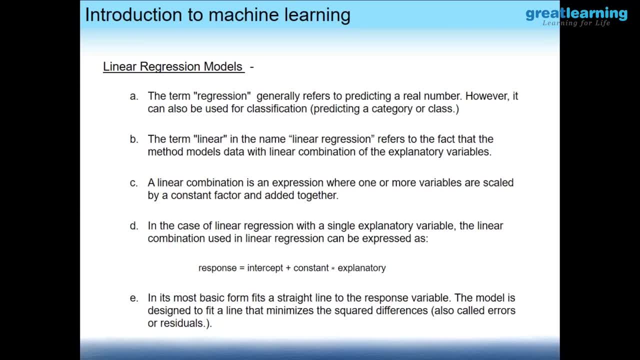 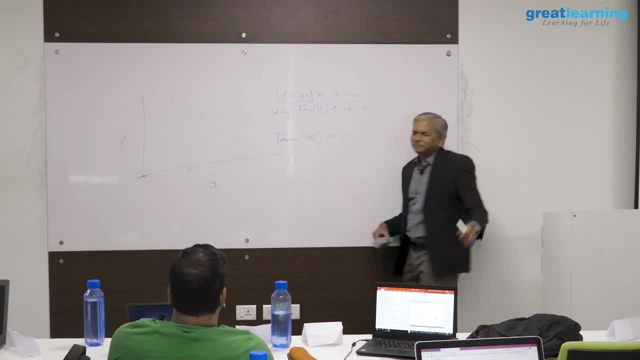 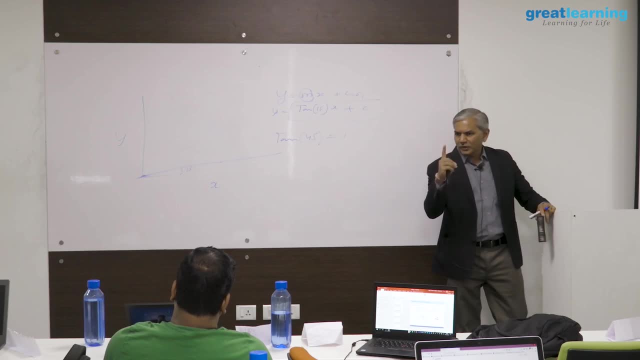 So tan of 15 degrees into 1, into X plus C. This will be equation of this line. What is tan theta? Tan theta is nothing but how much Y changes for 1 unit change in X. We call it tan. Alright, let us complicate this a bit more. 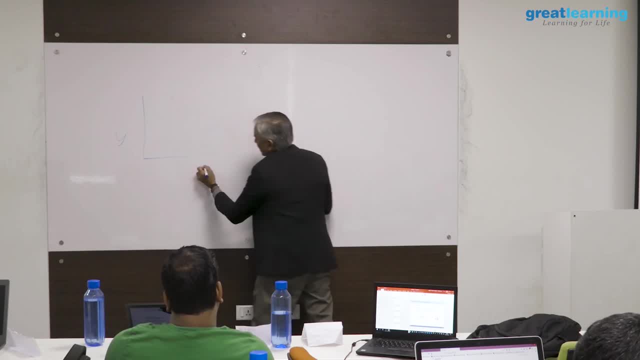 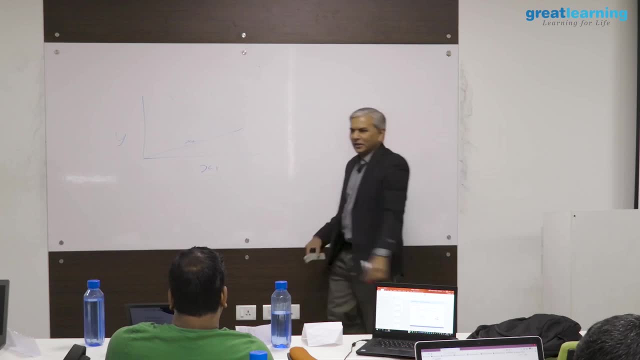 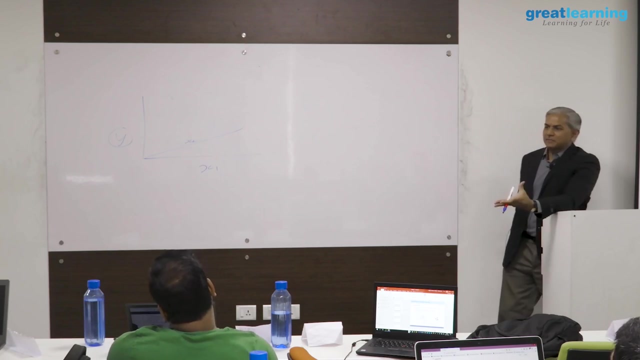 Suppose: instead of only one variable X, Now you have X1.. And you have another variable, X2.. And you have only one dependent variable, Y. In such case, the algorithm will find out the relationship between X1 and Y, X2 and Y. 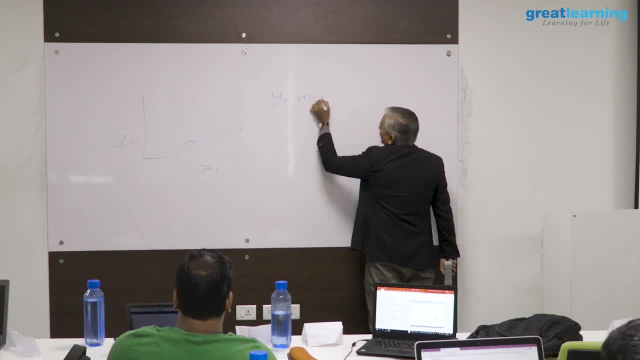 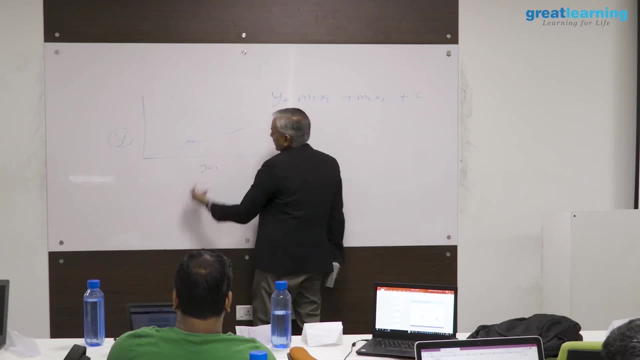 So it will express that relationship as Y equal to M1 X1 plus M2 X2.. And there will be only one constant term, Because now, Instead of having a line, you will have a plane, where the plane goes through the Y axis. 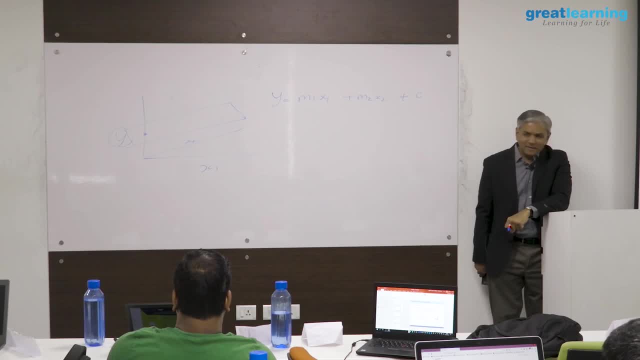 at some point. It cuts the Y axis at some point. So now you have two edges. One edge is on X2, the other edge is on X1. The two edges may have different slopes, different angles with X axis. Those are reflected over here as M1- M2.. 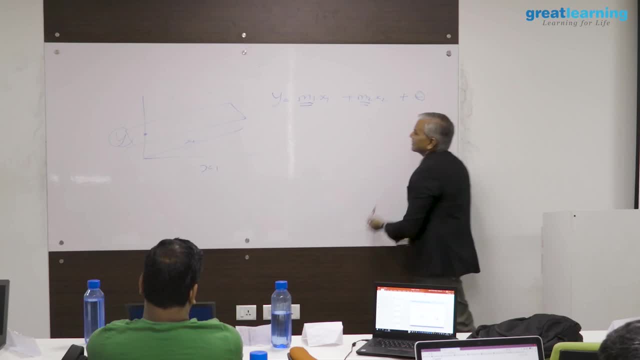 So the two edges of X and Y should be in the same plane. There is no point in having an X2 or Y axis, but we are actually going above it. So this is the C. The C continues to be the same, C. 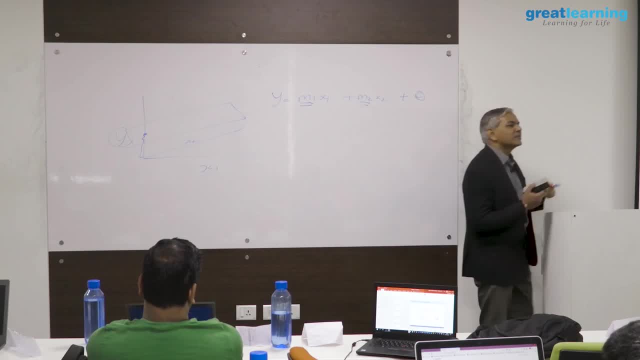 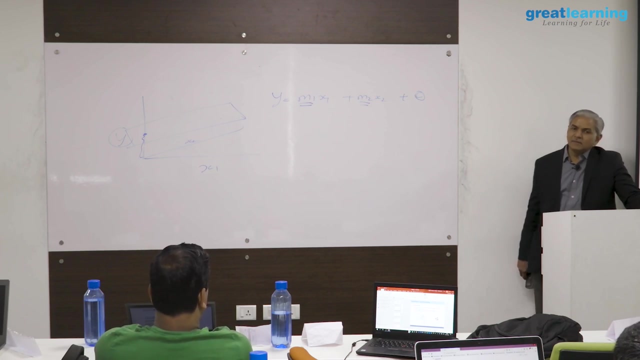 Where is the plane cutting the Y axis, Which means what is the value of Y when X1 and X2 are 0?? That is called the intercept, So we will have only one plane, Like if we have a multiple plane In case of. 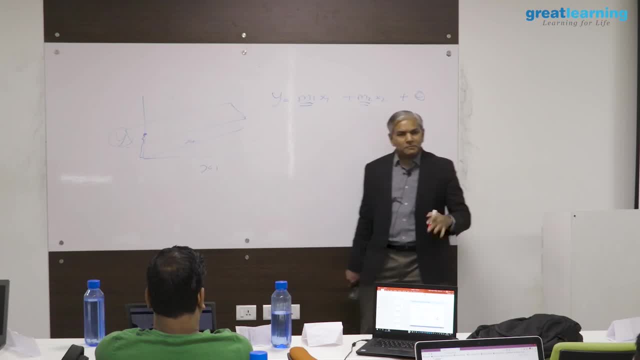 Like if we have a Z, also Can we can, we can have. We will be having a. It will be called a hyperplane plane. we do not know how it looks, but it will be only one. yeah, So human minds can imagine only three dimensions. 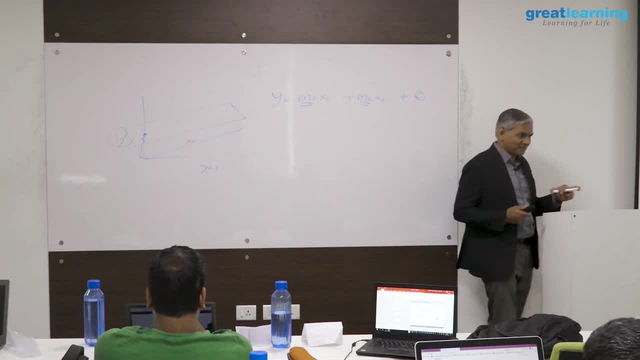 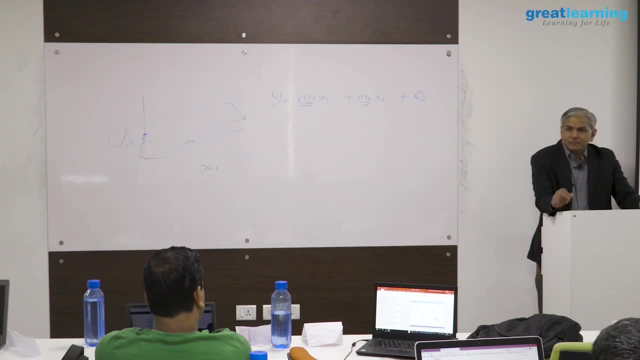 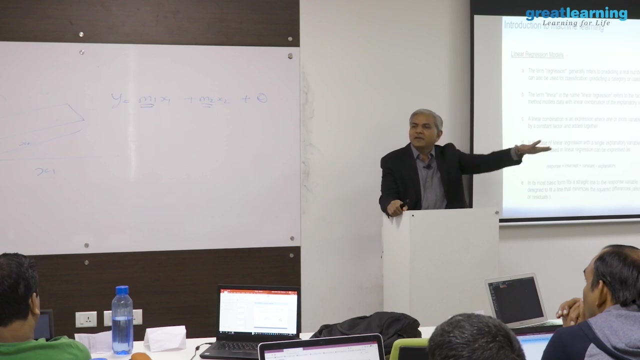 But suppose they go beyond three dimensions? there also the linear models work. Those planes are called hyper planes. Hyper planes- how do they look? we cannot imagine so, we do not know that. but they will also be one single plane And there will be no ups and downs, no curves, nothing. it will be straight plane. 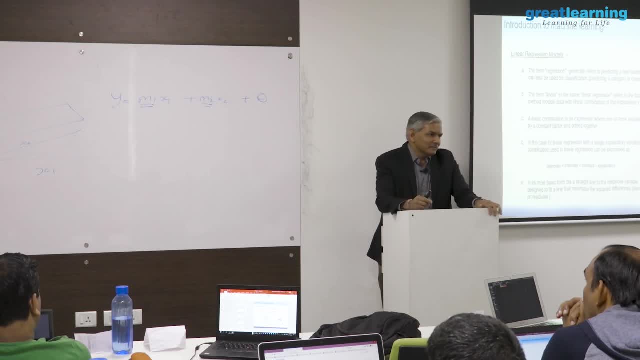 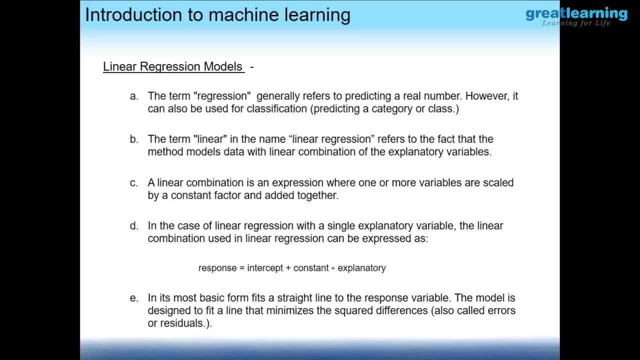 What do you mean by straight plane in four dimensions? no idea. It will have the same properties as the properties of a plane in three dimensions. So these x1 and x2 need to be in the same plane or it can be in a different plane, like. 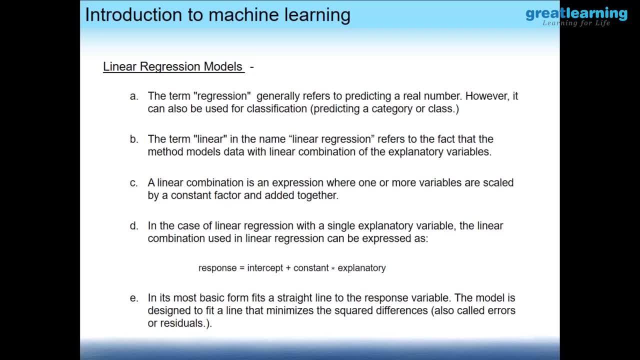 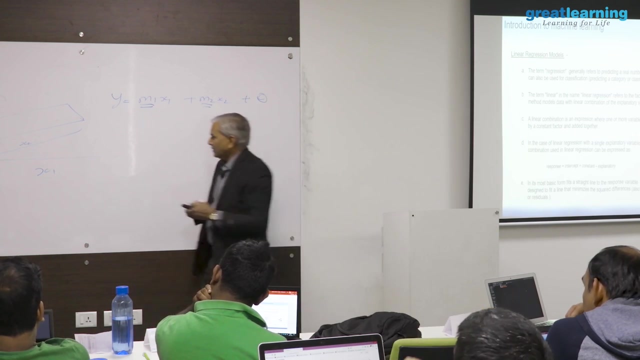 the x1 is in one plane and x2 in different plane. is it possible? They will be in the same plane. they cannot be in it. right And Actually 90 degrees. This angle in linear models this is a three-dimensional isometric view. this angle is always 90 degrees. 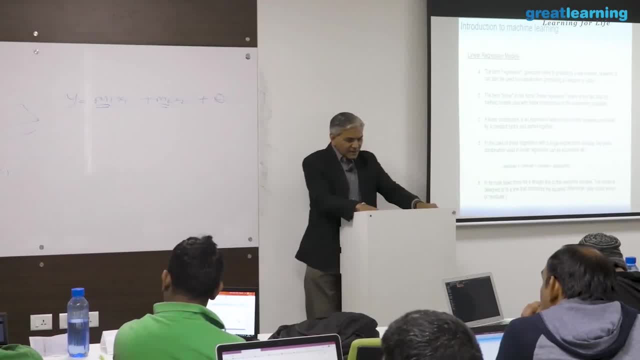 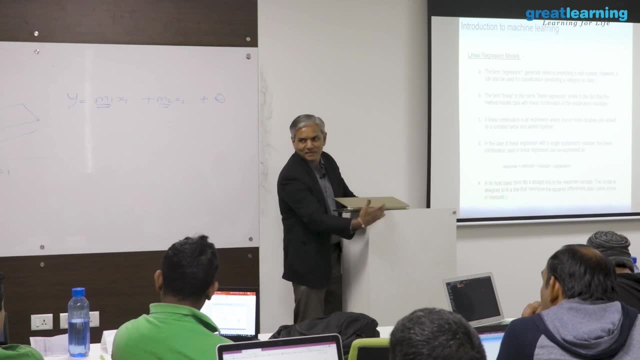 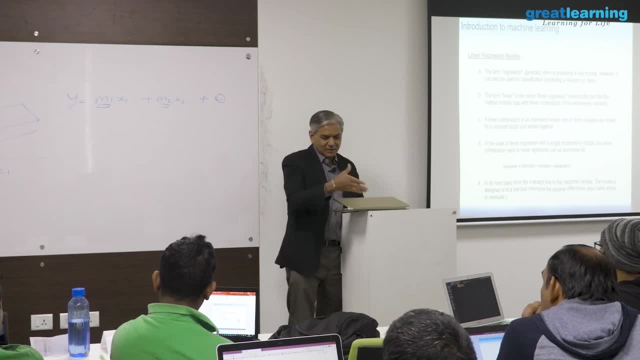 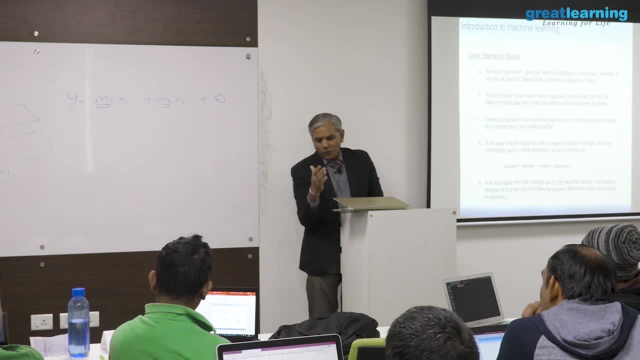 This is my m2,, this is my m1.. So at what angle the plane is to? x2 and x1 will decide the value of y. ok, In this case, the value of c will be 0 because the plane is touching the y axis. y axis is: 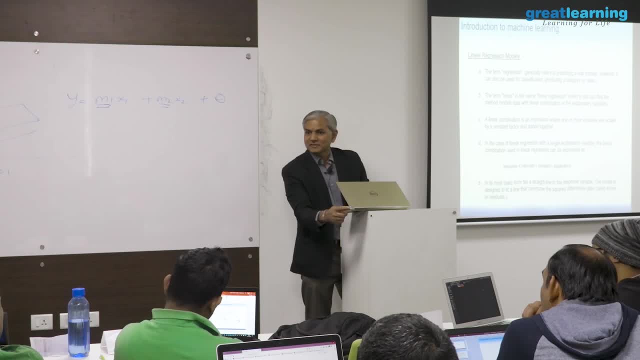 perpendicular like this. it is touching the y axis at the origin, The zero point. So imagine I can remove this. if this was a yoga tablet, I could remove this. ok, And imagine I am putting it in some angle, cutting the y axis at some point. 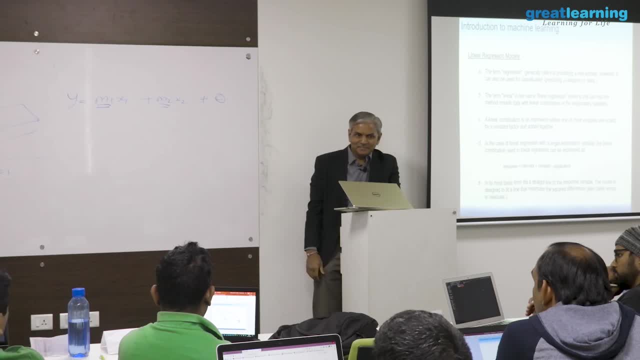 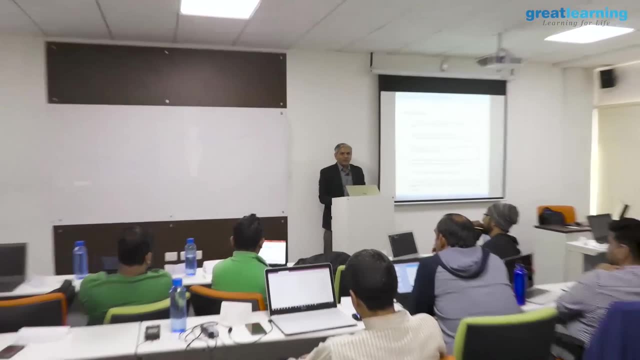 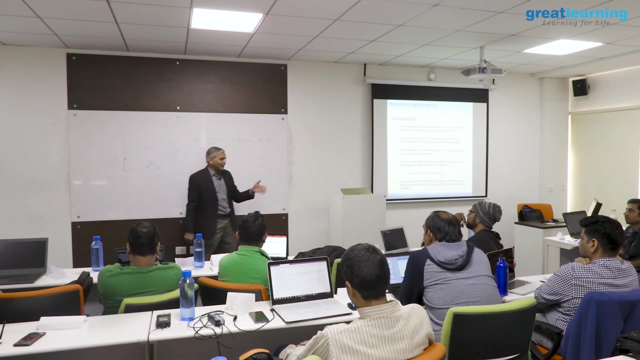 Then this angle. this angle is my m1, m2.. The point at which the plane cuts the y axis is my c. We cannot imagine beyond three dimensions how the planes will look, But they will have the same mathematical properties as a plane in three dimensions. 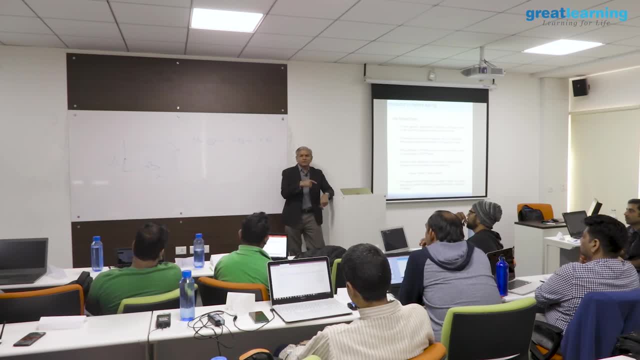 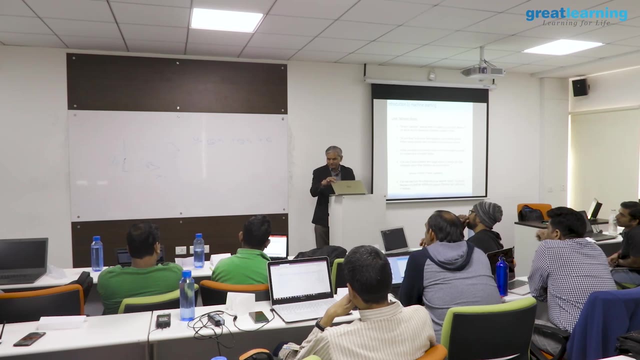 A point that you should probably keep in mind. it will become useful to you down the line when you do deep learning and so on and so forth. The number of dimensions of a model. This is the model right now. the surface, The number of dimensions: how many dimensions is this model? 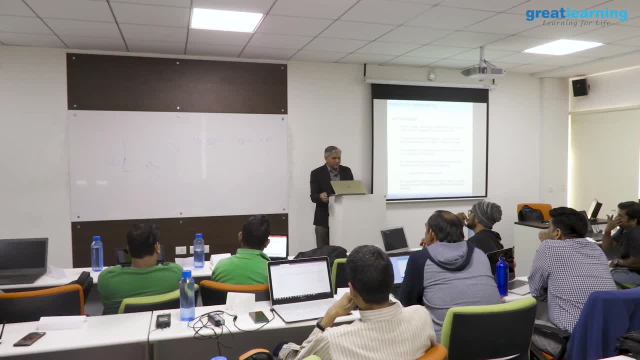 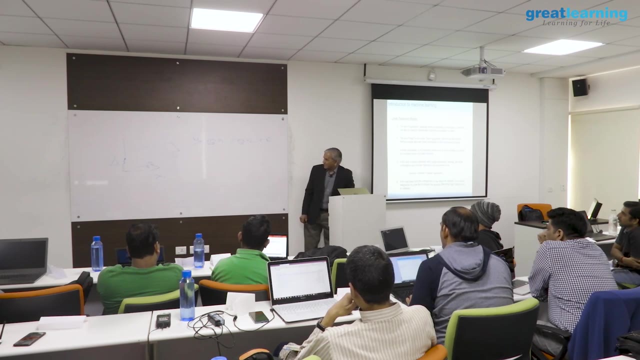 Two dimensions. length into breadth, The model is only two dimensions. The feature space is three dimensions. So the number of dimensions in a model will always be one less than the number of dimensions in the feature space. Right, Alright, You can call it anything you like, that is not a problem. 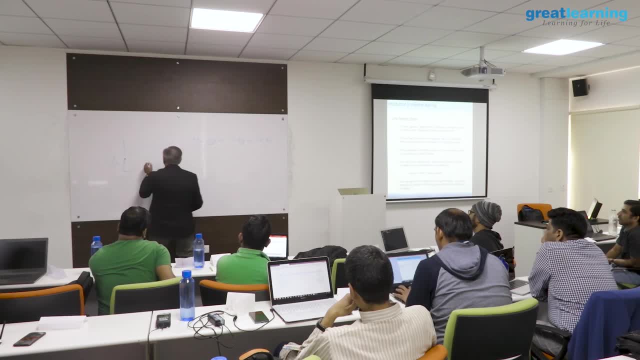 x, y, z. ok, that is what I am saying. You want to call it z, you call it z, it does not matter, It just replaces with z. Basically, these are indicators. Ok, These are independent variables. This is the target variable. 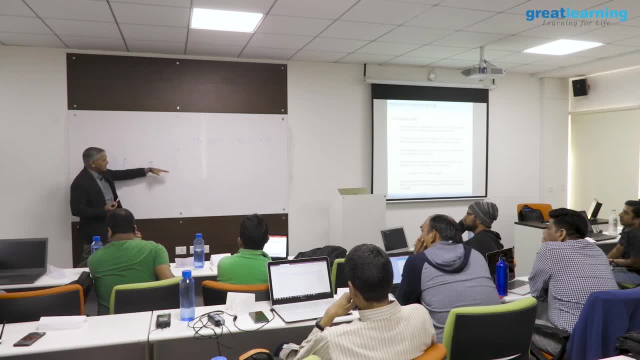 So we are trying to understand how the target variable is influenced by these. Say, you have three- x1,, x2, x3, right? So how, in that case, the model dimension will be so still, the model dimension is two only. 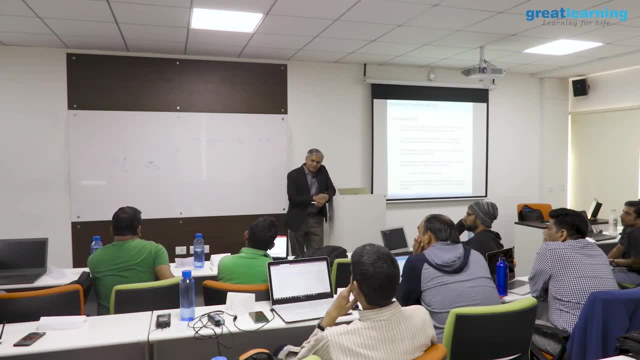 right. No x1, x2, x3 are three independent variables, So they have one target variable also. So that makes it four. Four dimensions, Four dimensions, Three dimensions, Three dimensions Model will be three dimension in that case. 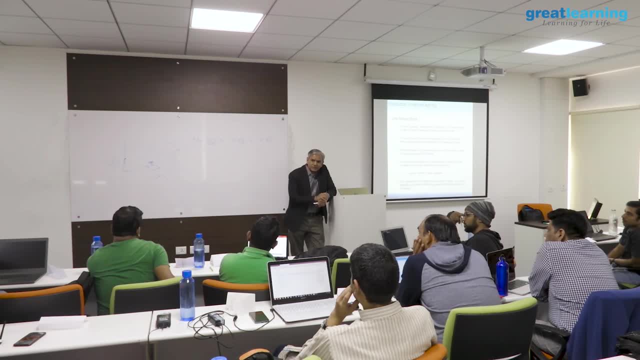 What will be the three dimension? I mean, however it looks, I do not know how it will be. how will it look? It will have three, three edges. We do not know how it will look, so that is why we do not talk about it. 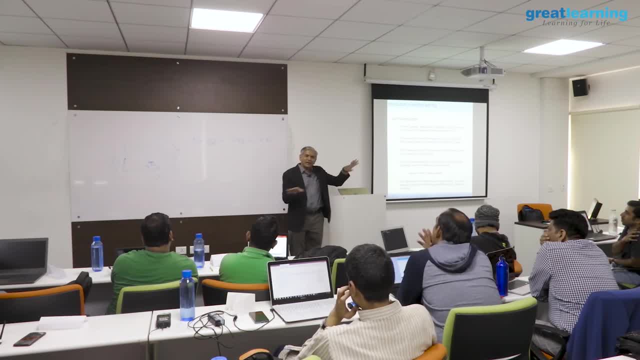 But the properties of that model will be similar to properties of a plane, a line, so on, so forth. So, independent variable, we have to always consider as the orthogonal in the check. That is what the algorithm is. Yes, Yes, That is what the algorithms assume. 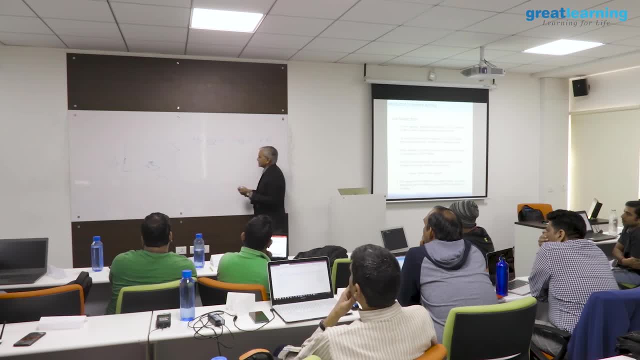 All the algorithms assume that your independent variables- ok, suppose you have a data frame. In the data frame you have multiple columns. These are independent variables: IV1, IV2, IV3, and this is my target. All algorithms assume that independent variables are independent of each other. 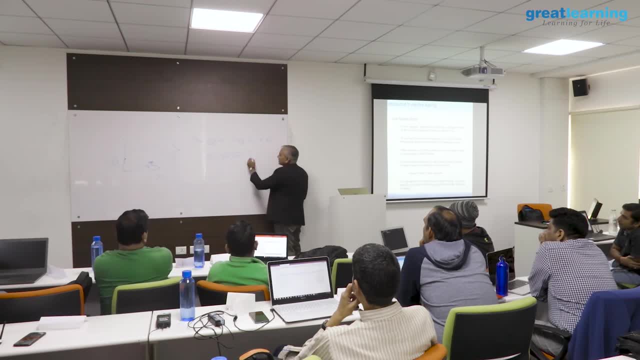 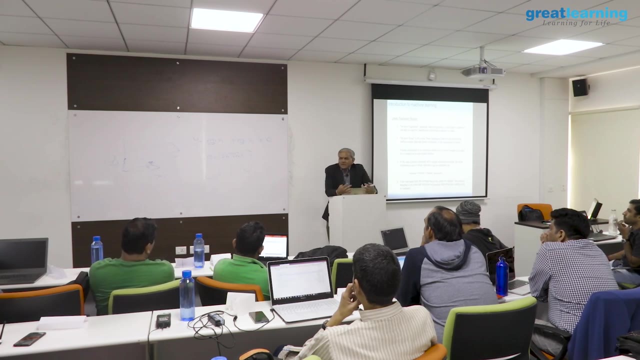 They do not influence each other. They only influence the target. That is what they assume, But in real world that is not true. Ok, Suppose I want to predict miles per gallon of a car, Given the weight of the car, given the horse power of the car. we know that they are related. 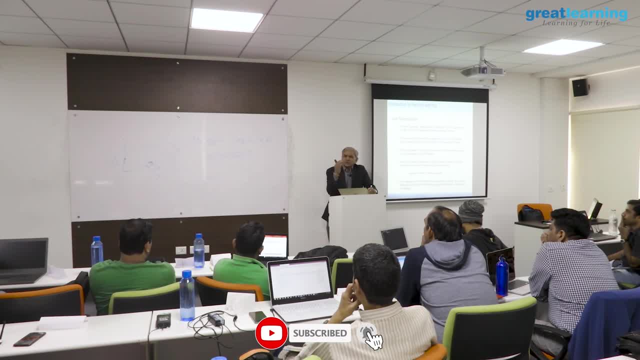 So we can build a model. But we also know that horse power and weight are also related to each other. More the weight of the car, more the horse power. They are positively related, But the algorithm assumes that they are not related. This problem in linear models it is called the problem of collinearity. 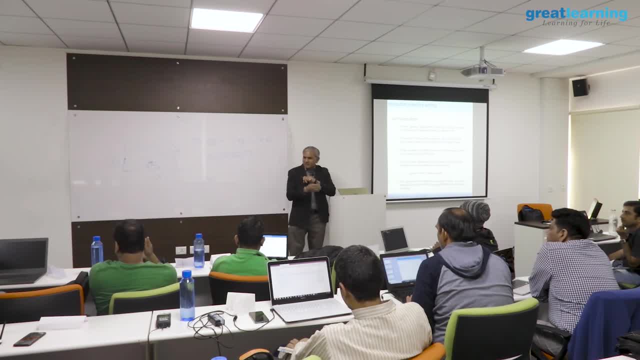 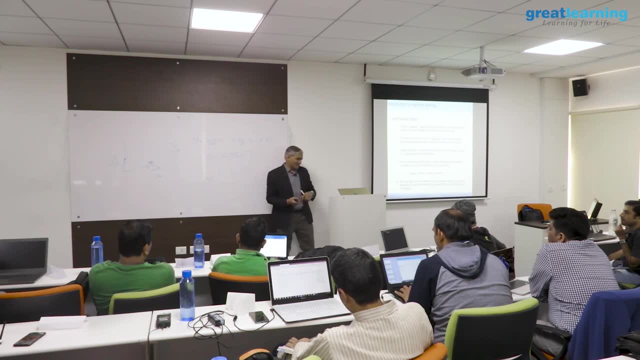 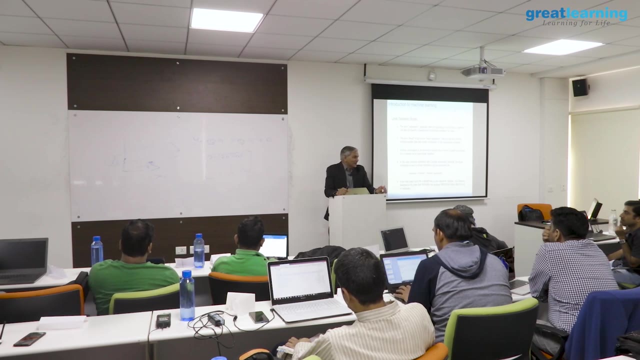 Where assumption is each dimension is independent of the other but in reality they influence each other. that problem is called collinearity. ok, This collinearity where independent dimensions interact with each other, they are not independent. This collinearity can lead you to a problem when you productionize your models. 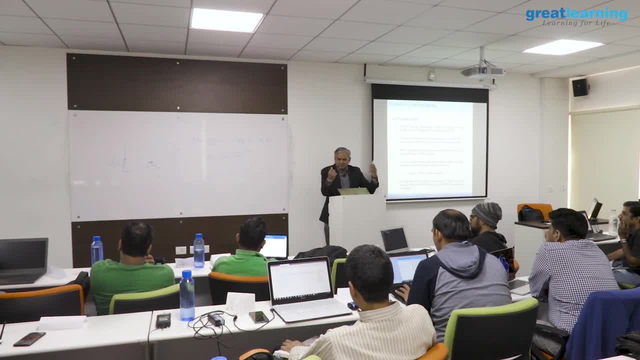 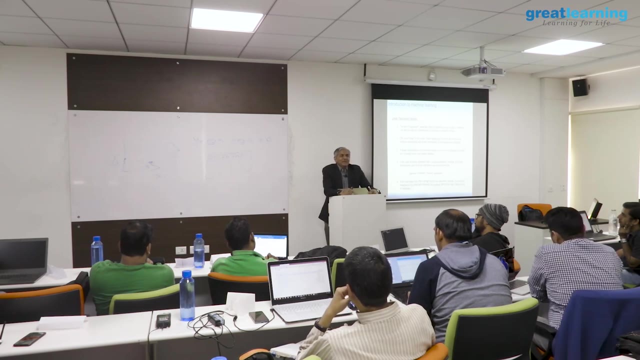 The models may be less effective- less what do you call predictive power- Than required to be because of the collinearity. So one of the things that we do when building models is we see what the collinearity is between the dimensions. 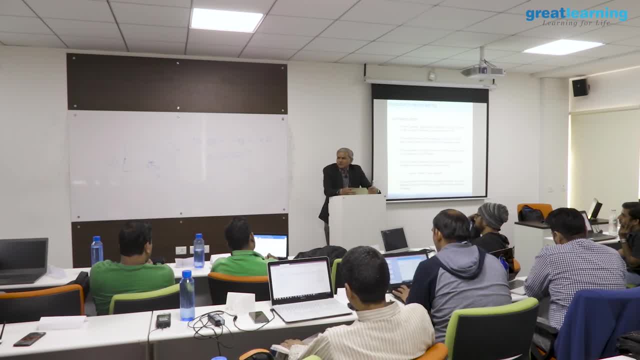 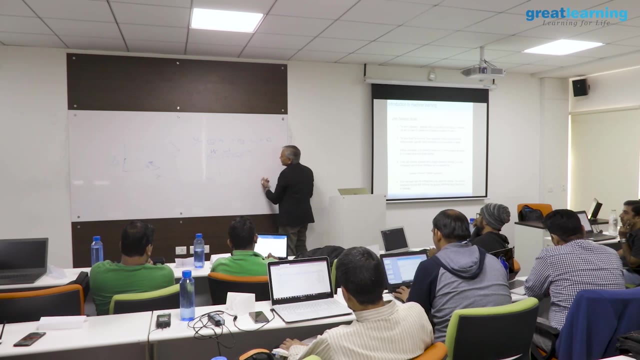 If the collinearity is very strong, they are very strongly related to each other- the independent variables- then we may have to resort to some techniques. Suppose this is my horse power and this is the weight of the car, And if I plot a graph between these two, can you tell me how that will look? 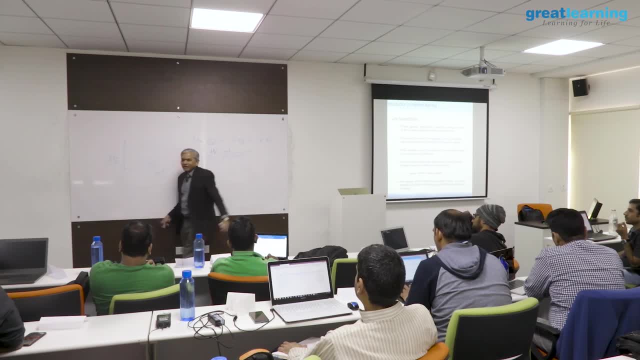 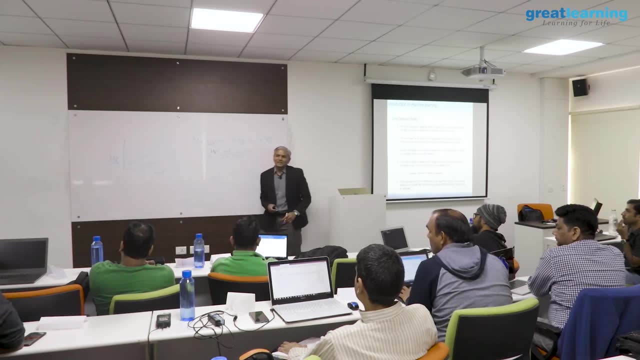 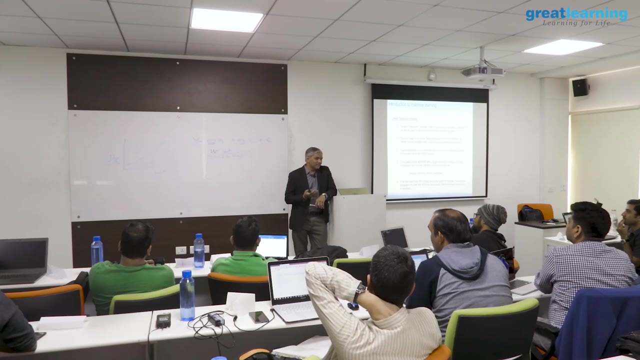 This is weight of the car. this is horse power of the car. If I plot a graph between these two, take all the data points. You will see some linear trend. ok, All of you know what is R value, coefficient of correlation, R value statistics you have. 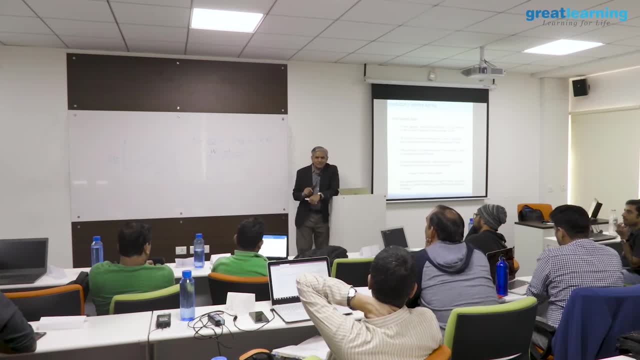 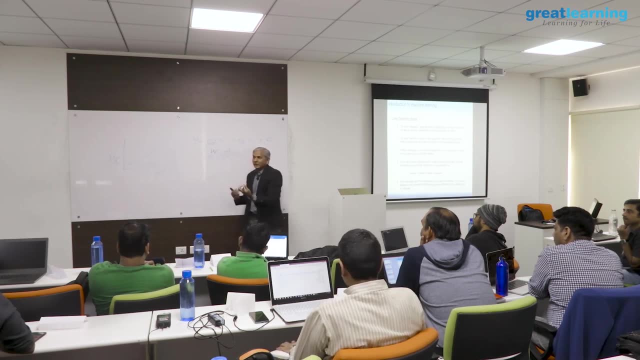 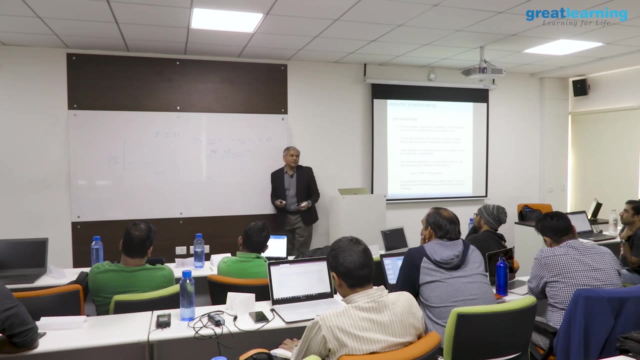 done statistics right, Ok. R value is measurement of how these two variables relate to each other. how strongly You will see that R value comes very close to positive 1, in this case, The maximum it can be is 1, so it will be very close to positive 1, ok, which means 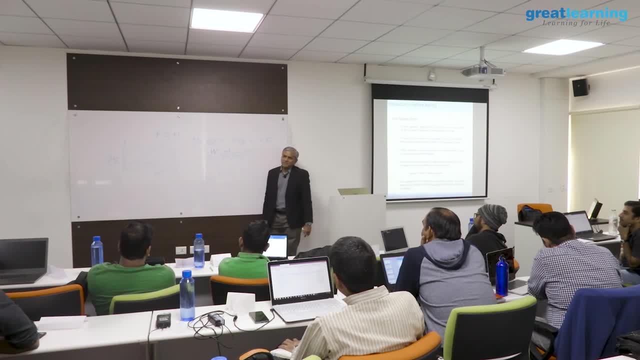 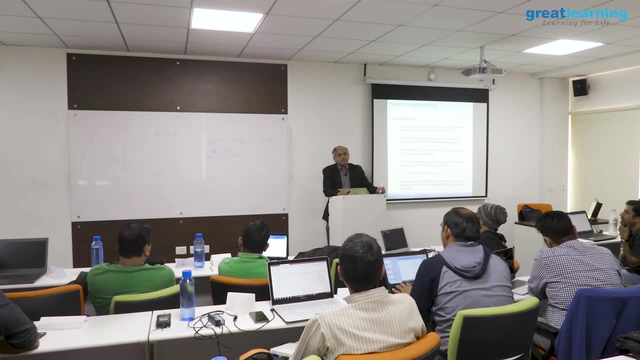 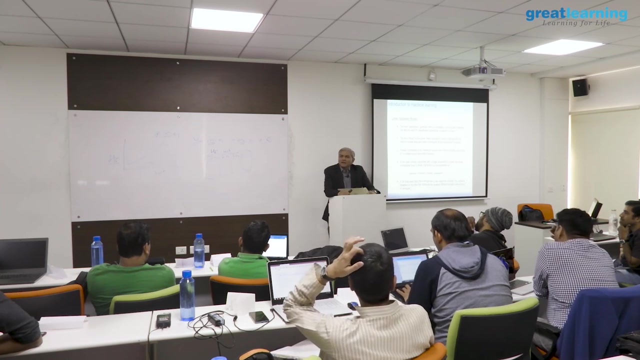 these two variables are not truly independent of each other, but the algorithm wants all the dimensions to be independent of each other, So in such cases we resort to a technique called dimensionality reduction, which is not simply dropping the dimension. I may convert them into a composite dimension, both the dimensions put together I create. 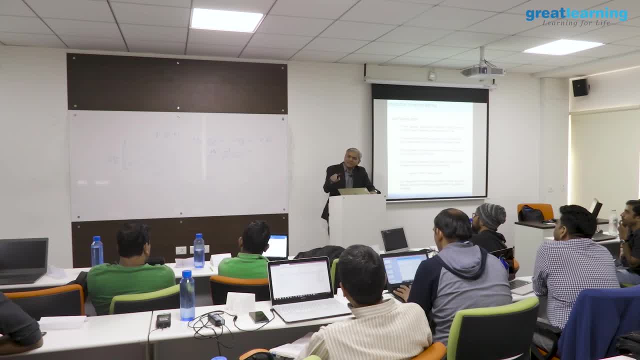 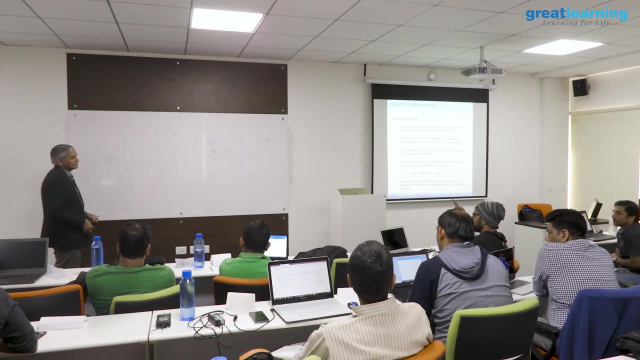 a synthetic dimension and I use that synthetic dimension in my model building rather than these two. Just a question. Ok, In this case the horse power and the weight of the engine is same, almost same, like it is increasing in the same non-linear line. if I put both of them, it will have the same. 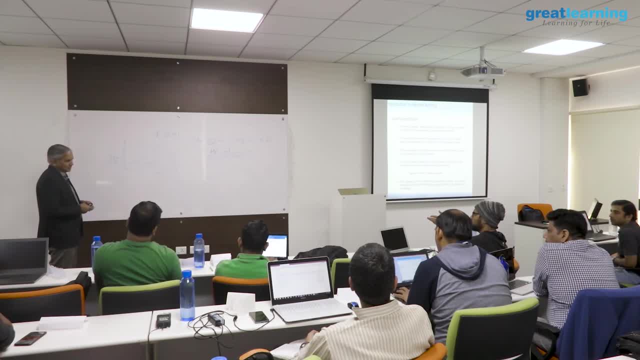 effect in the model. right, If I remove one of them also, then it will have the same effect in the model. the model will not change anything, right, If that removal is an option to you when the relationship is absolutely aligned. but you? 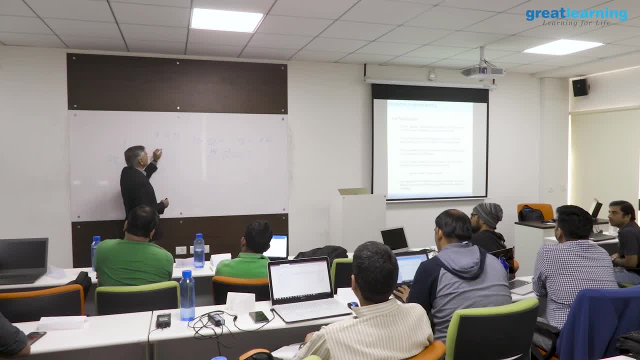 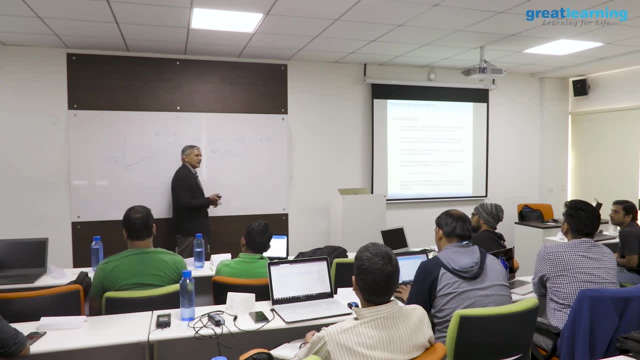 will see that it is generally not aligned. it is a spread And the spread is also curved. So which one should I drop? Should I drop this or this? That depends on which dimension is more prone to errors when you calculate, when you capture. 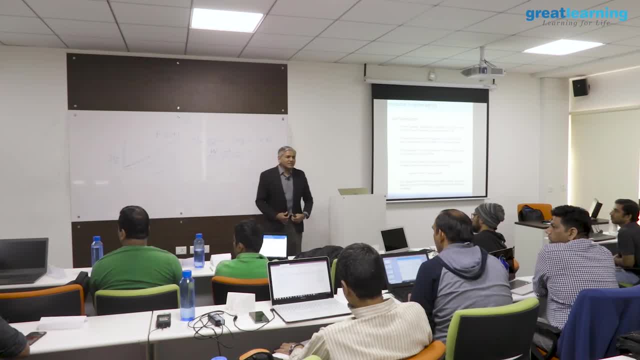 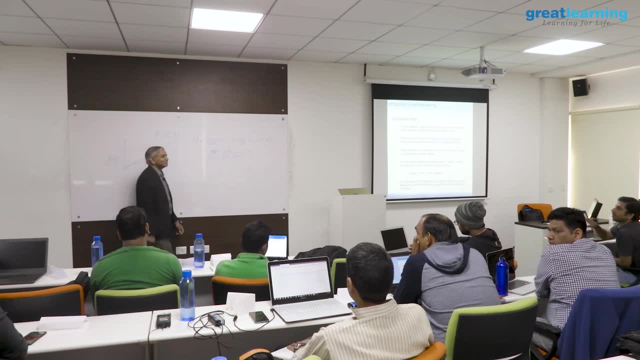 the data. So instead of doing all that analysis, I might convert into a synthetic dimension using a technique called PCA- principal component analysis. Sir, in the previous example we looked at the x 1 and x 2 and they are separated by: 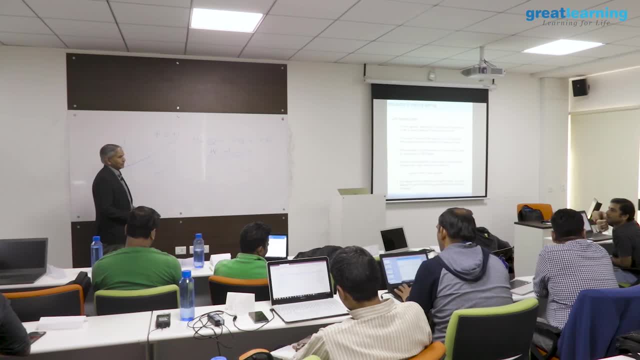 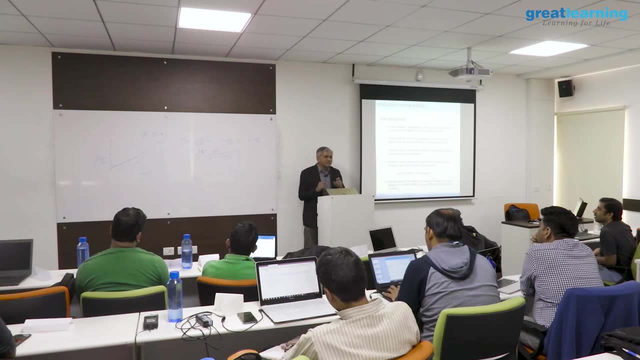 an entity, right, Yeah, So in that case we can have only four dimensions. No, no, that is what I am saying. That is our brain. Our brain can see only three dimensions, But the algorithm can work in 300 dimensions. 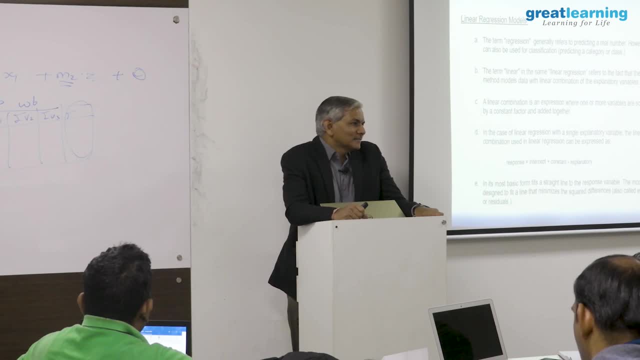 All the 300 dimensions, mathematically will be orthogonal to each other. Why is it a problem if these elements are actually very collinear? and they are collinear. Why is that? Why is that a problem? Okay, Let us move on for a minute. 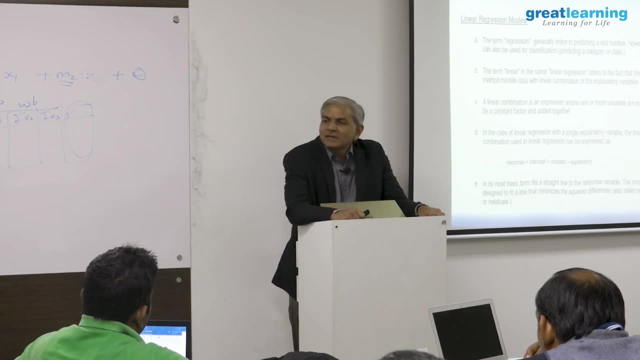 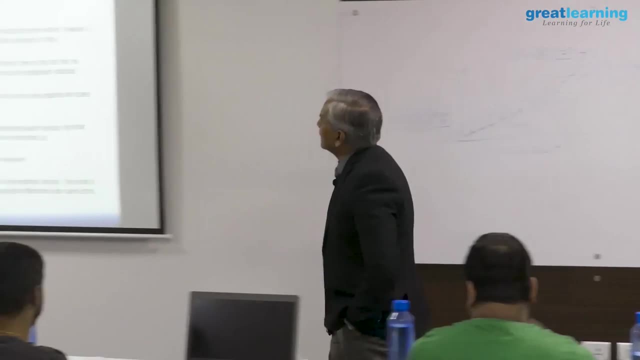 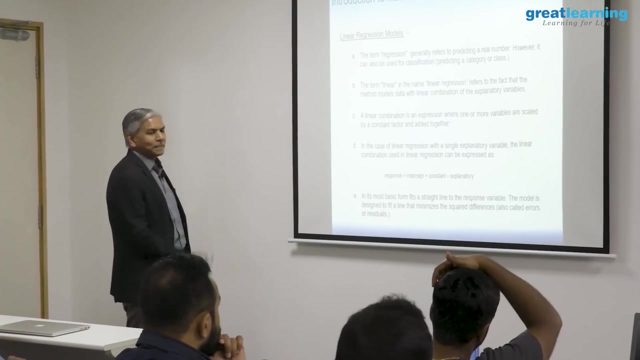 I want to cover some ground before I answer that question, because that is a very important question you have asked. All right, Let us move on. The term regression indicates that we are going to predict some values. Whenever you build models to predict values, we use the word regression. 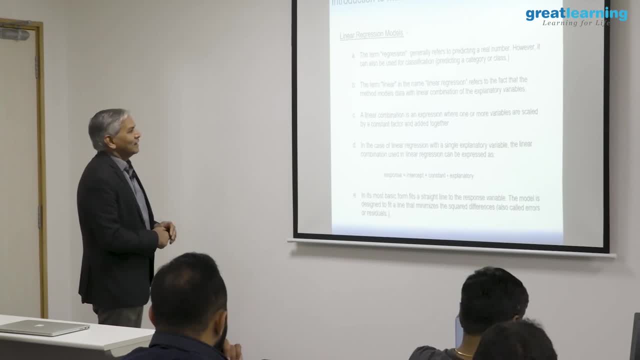 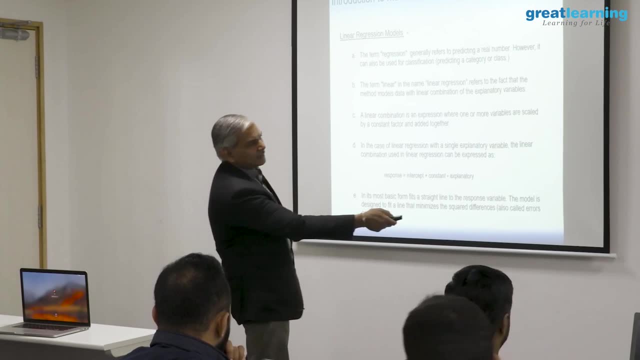 The term linear. now you understand where it comes from. So your linear model is nothing but a combination, addition of weighted variables. Okay, This weighted variable, this is another weighted variable. you are adding the two to predict the value of y. 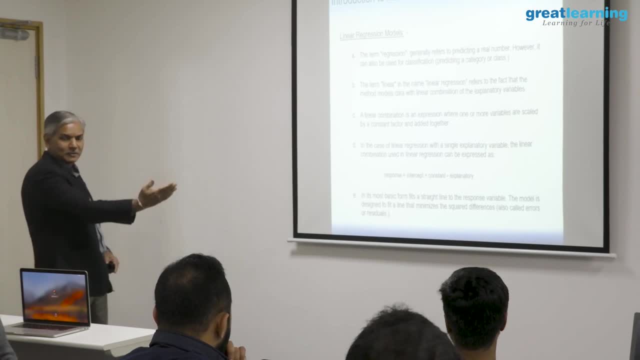 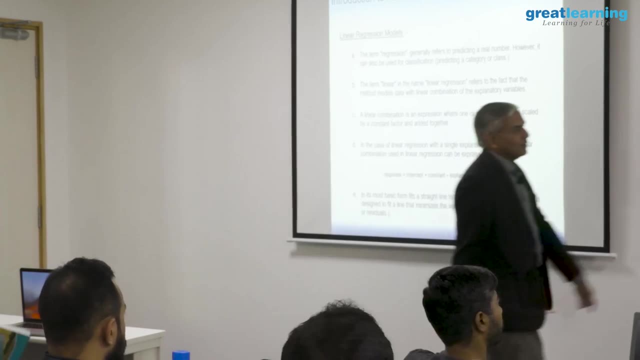 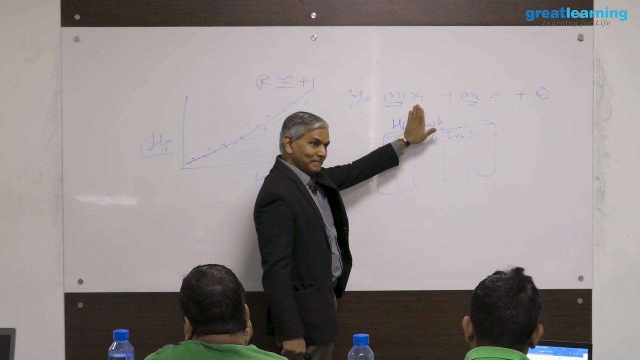 It is a linear combination of one or more variables with weights. The weights are called coefficients. Okay, So once again I repeat: What is this M1?? M1 is how much y changes whenever x1 changes by one unit, keeping x2 constant. 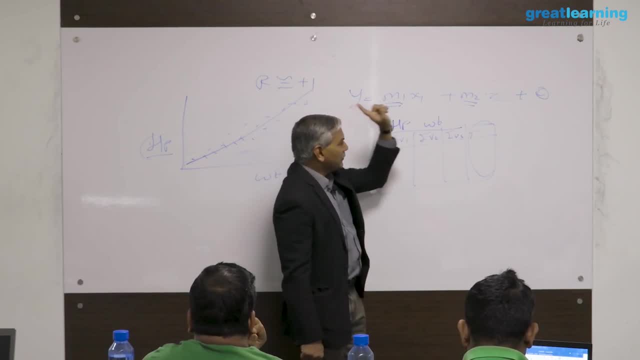 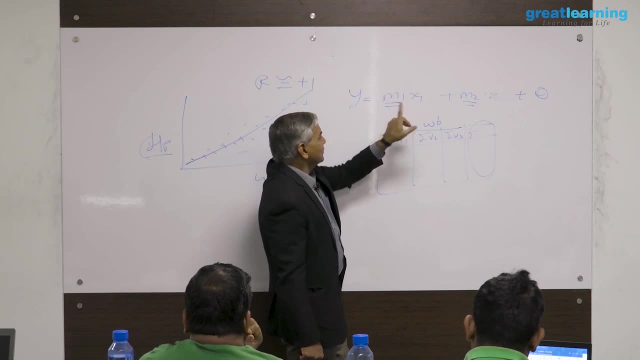 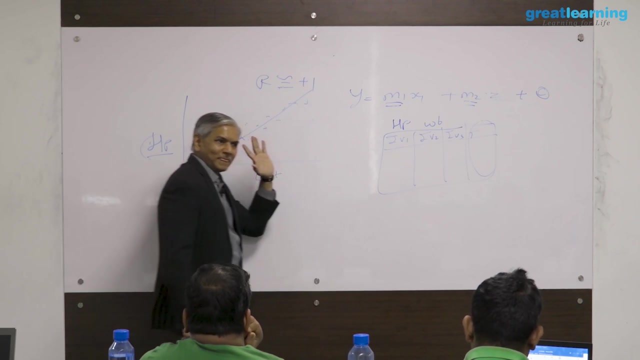 What is this M2?? M2 is how much y changes. M2 is how much y changes whenever x2 changes by one unit, keeping x1 constant. Okay, So this is the relationship between x1 and y. This is the relationship between x2 and y. 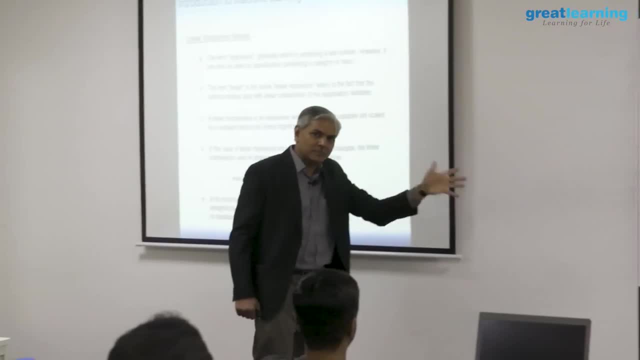 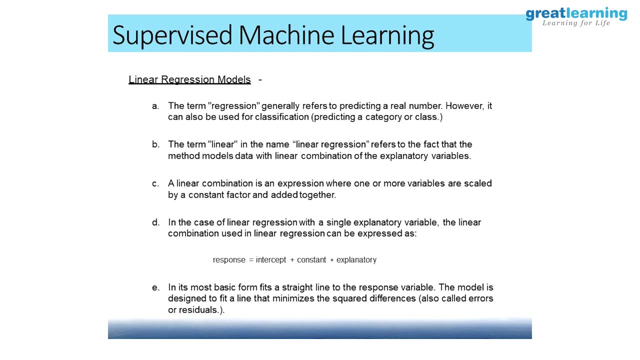 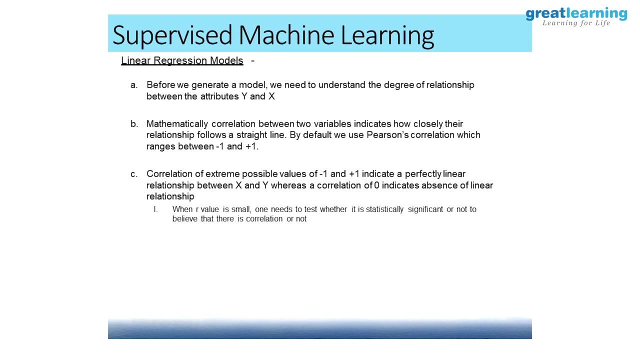 The relationship is how much y changes whenever input changes by one unit. That is a relationship, And that relationship is what we call linear models. Okay, We have already seen this. We are going to move on. So, before we start building our models, before we start building our models, we actually 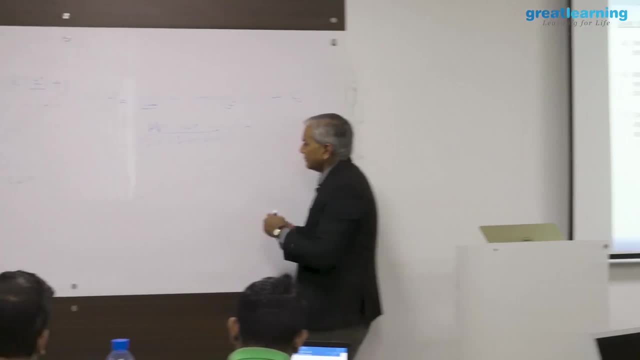 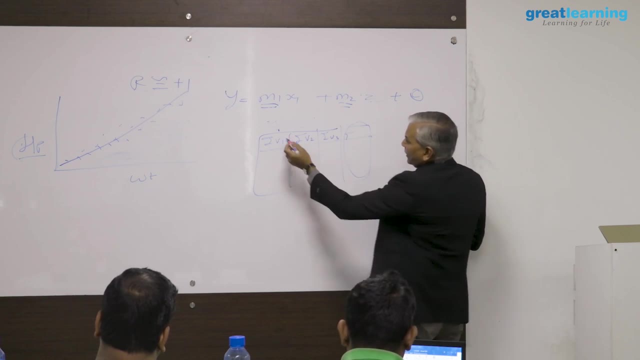 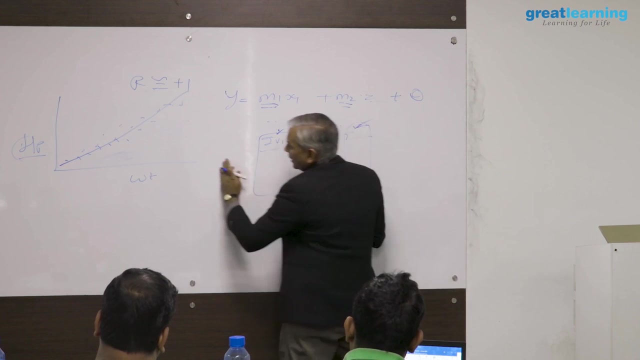 need to analyze our data set, And what I mean by this is suppose this is my data set. I will go and analyze between this IV1 and target IV2 and target IV3 and target, which one of these is strongly related. 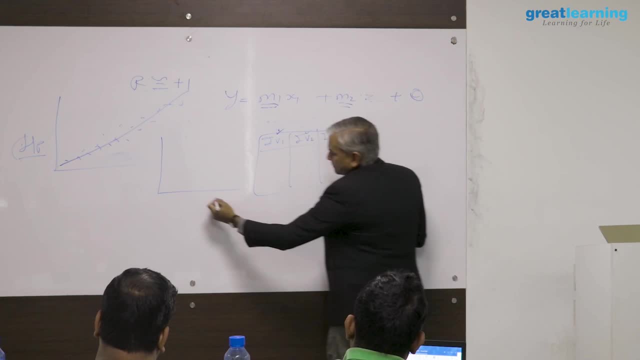 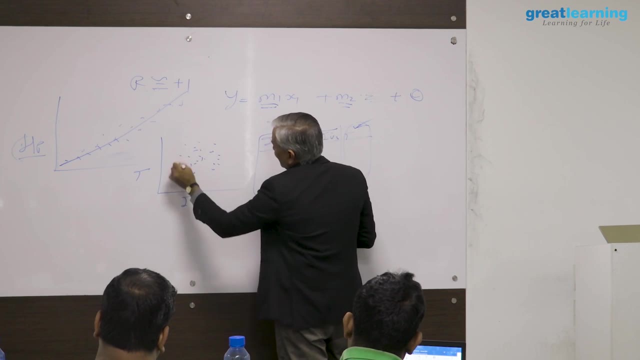 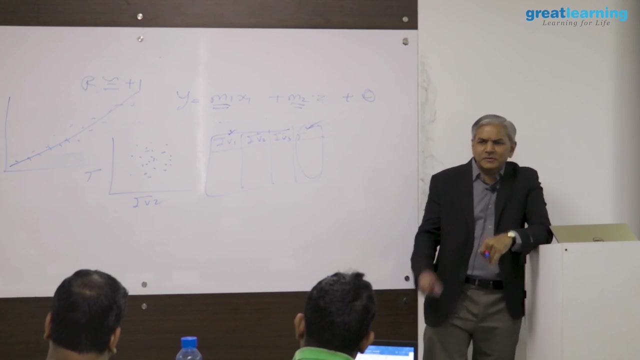 with the target. If suppose IV2 and the target, the distribution is scattered all over the place, It's like a cloud. The data points are spread like a cloud. There's no trend you are seeing in the spread. Then in that case IV2 is not a good predictor of the target. 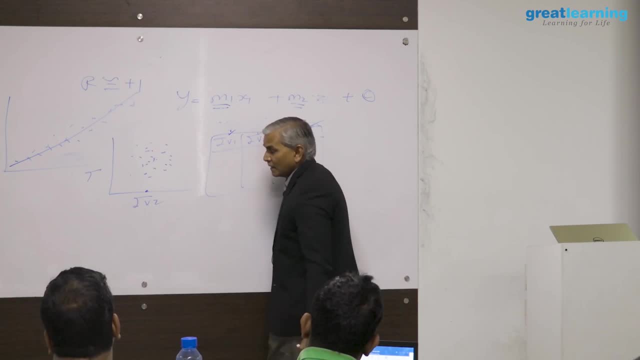 How can you say that? Take any value of IV2.. Draw a straight line. Draw a straight line. Draw a straight line For that value of IV2, you have multiple values of target. Which one should I take? I don't know which one to take. 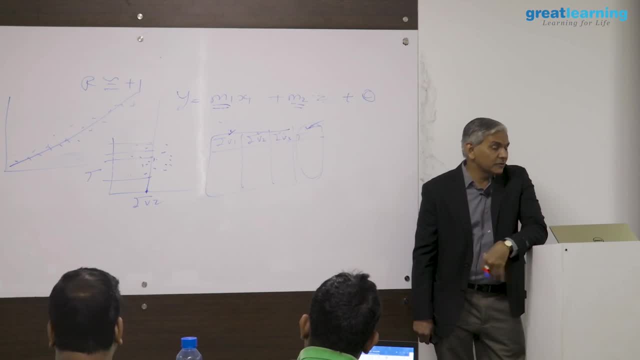 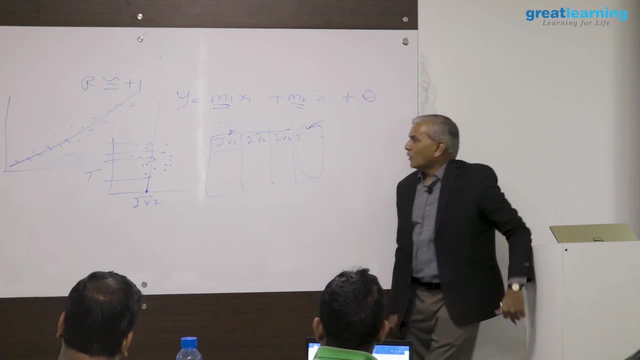 So we say that IV1, IV2, sorry, we say that IV2, independent variable 2, is not a good predictor of the target. On the other hand, if suppose between, say, IV1 and IV3, which one should I take? 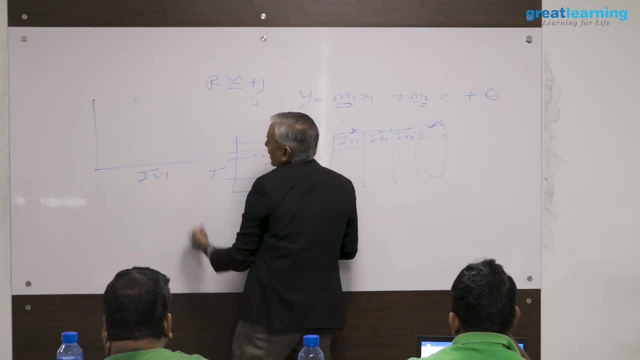 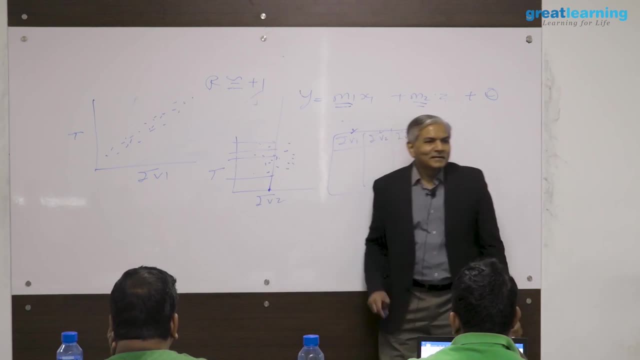 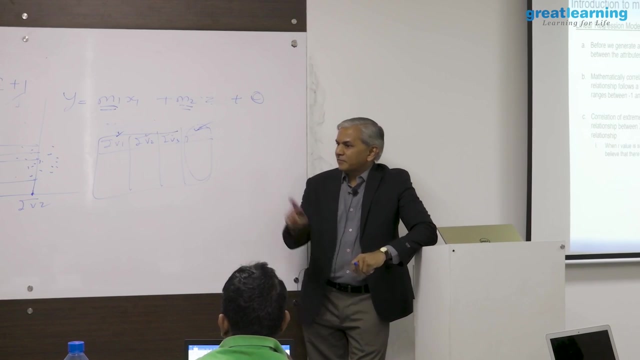 Which one should I take. Which one should I take? And the target? we see the data points are scattered in some form of a trend. Then we say that IV1 is a good predictor of the target. So the first filter that you will apply in your data set is of all the columns given. 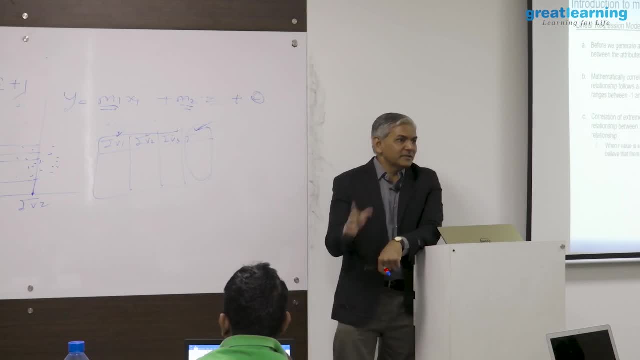 to you which columns strongly relate to the target. Those columns which don't relate strongly with the target. you are going to determine Which columns strongly relate to the target. Those columns which don't relate strongly with the target you are going to determine. 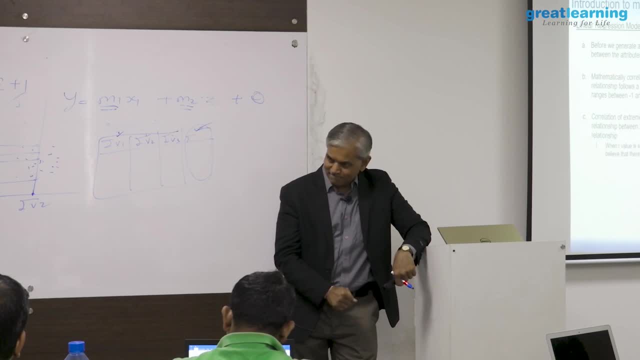 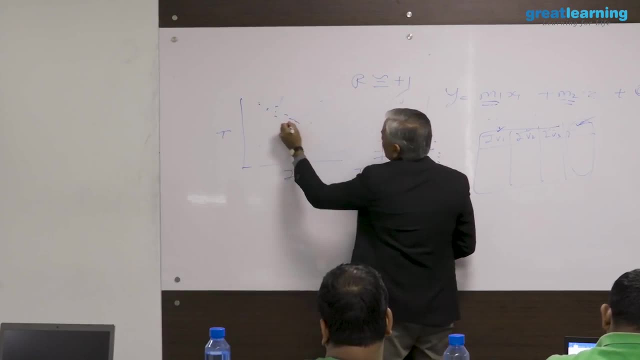 You will drop them from your analysis. You are not going to build your linear model on them. So the relationship could be positive or the relationship could be negative. it could be downwards also. I want a strong relationship. doesn't matter whether it is this way or that way. I don't. 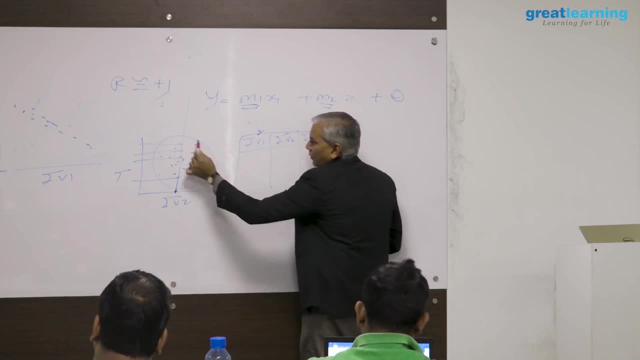 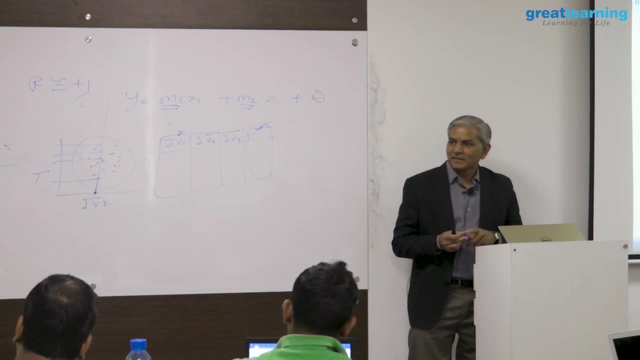 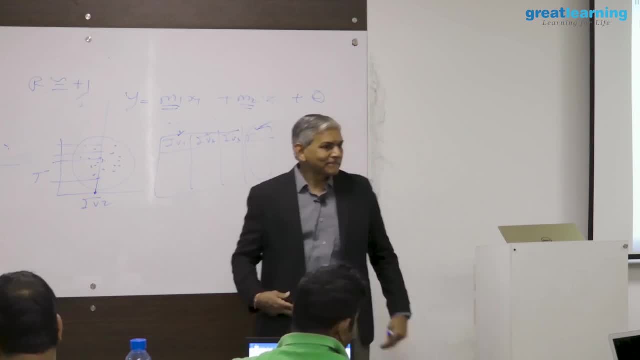 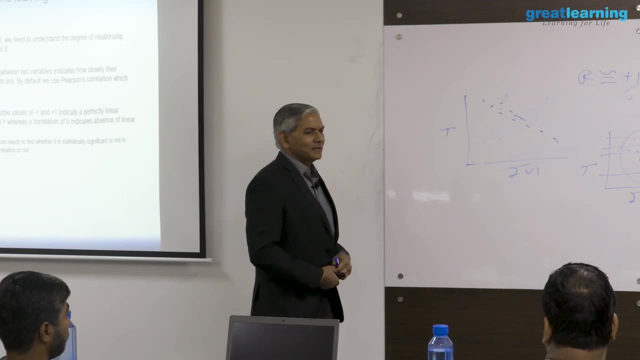 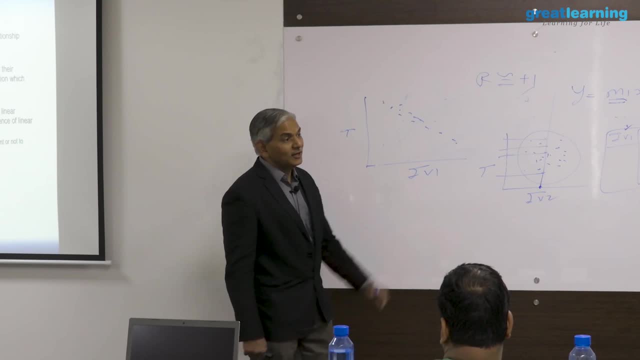 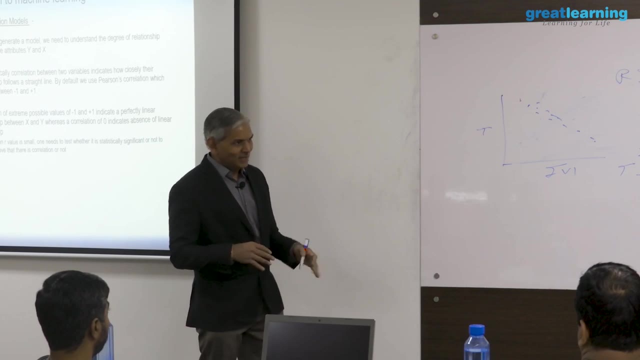 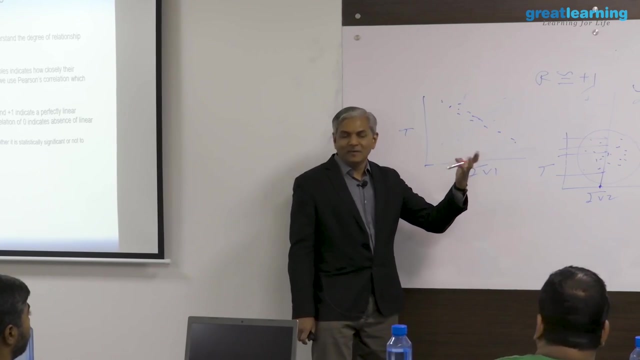 If you see non-linear relationships, then you might want to resort to non-linear models. Linear models they expect linear relationship between y and the independent variables. Then your models predictive power will be very high. However, as you will see now, those are all very perfect conditions. 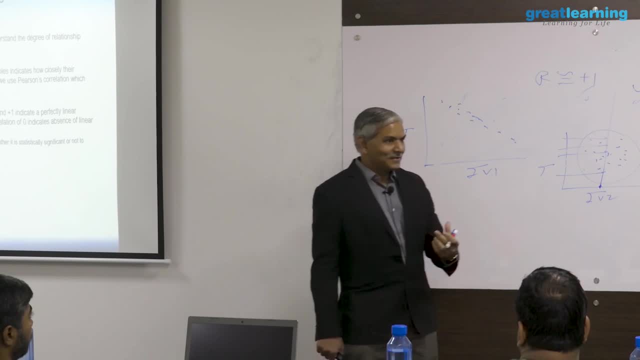 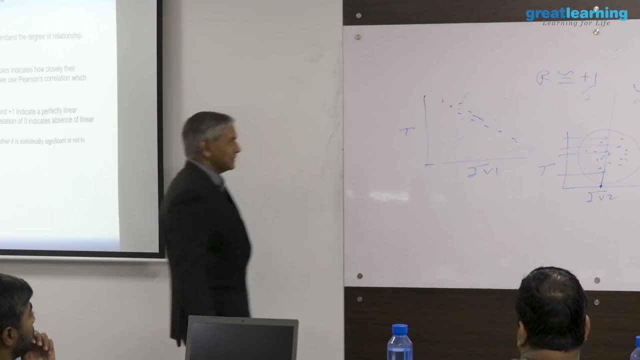 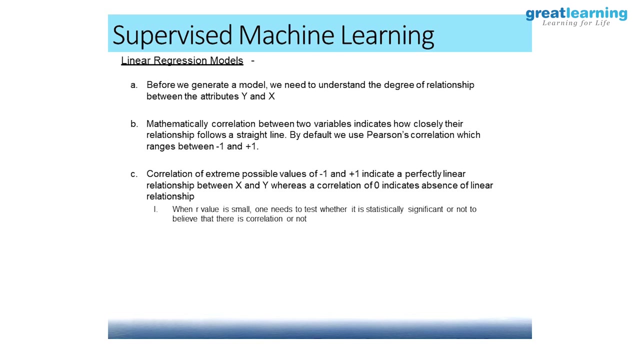 In the real world we hardly have such perfect conditions, right? So sometimes, even when the relationship is not linear, we go up, build a linear model. We will see that down the line. Ok, How do you measure the strength of the relationship between independent variable and the target? 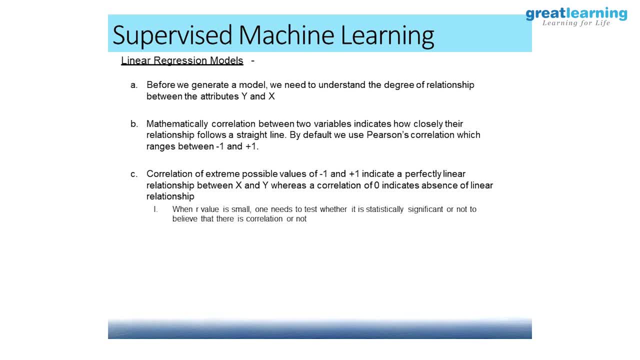 For that we use a metric called coefficient of correlation, How these two variables, the target and the independent variable, how they co-relate, how they relate to each other, which we express using a character called r. I will tell you what this r is. 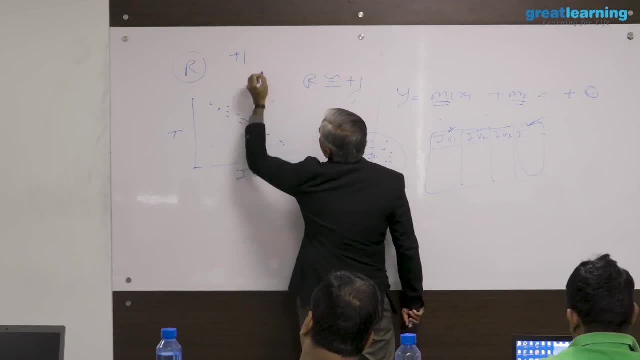 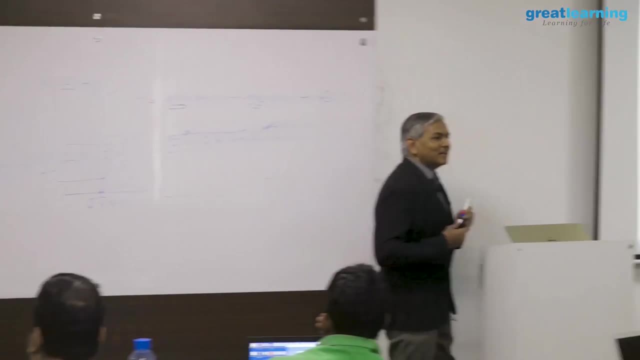 This r metric can have a value of plus 1, minus 1 to plus 1. in this range, The least it can have is minus 1.. The max it can have a value of minus 1.. Ok, So the value is plus 1.. 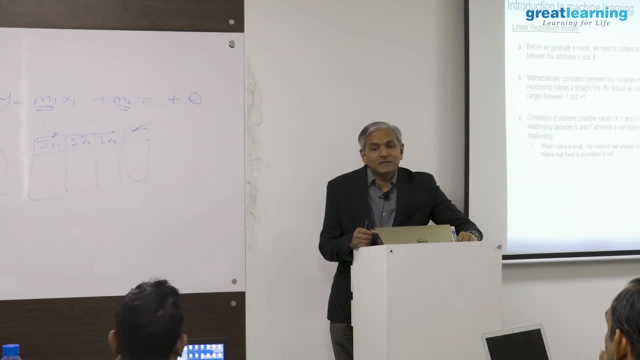 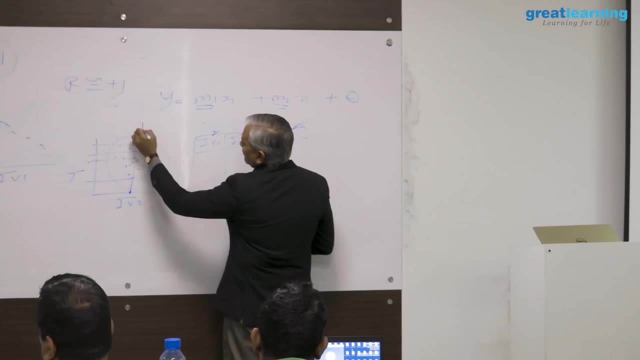 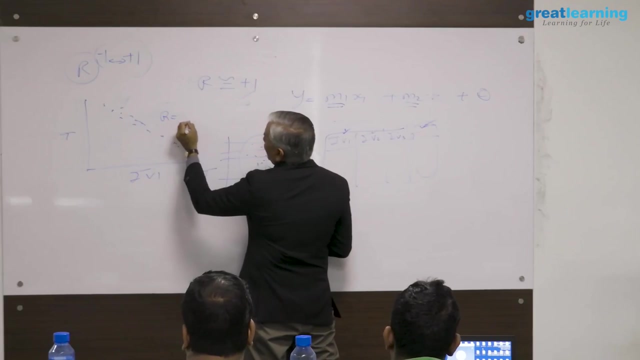 It cannot be beyond this range. R value can be 0,. can be 0.. When you have spread like this, your r value will be very close to 0.. When you have a spread like this, your r value will be very close to minus 1.. 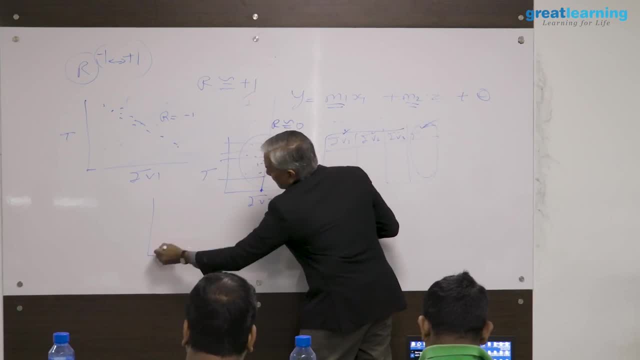 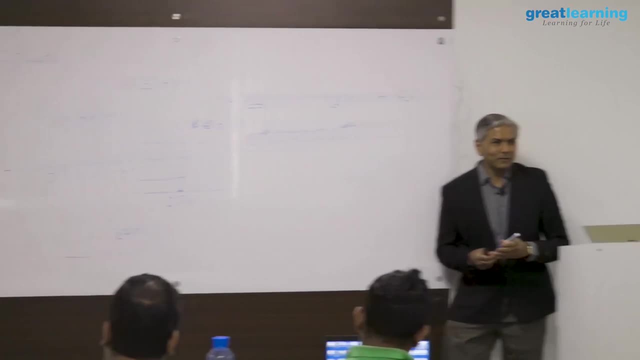 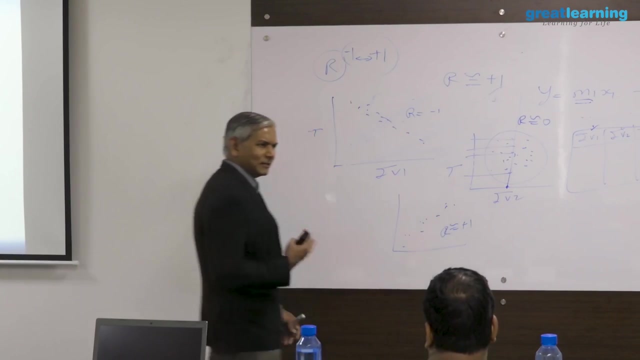 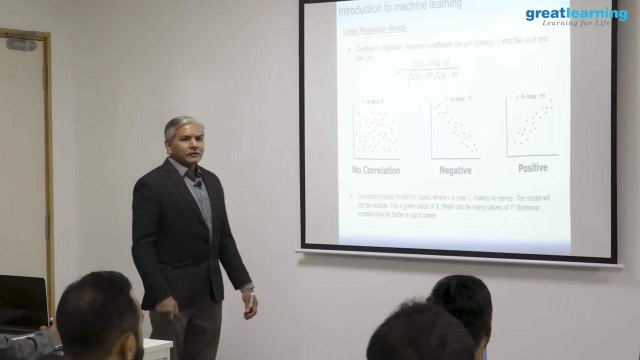 When you have a spread in the other way, your r value will be very close to plus 1.. Ok, So r value is an indicator of how strong the relationships are. So let us understand this r value in slightly more detail. The formula for r value is this: 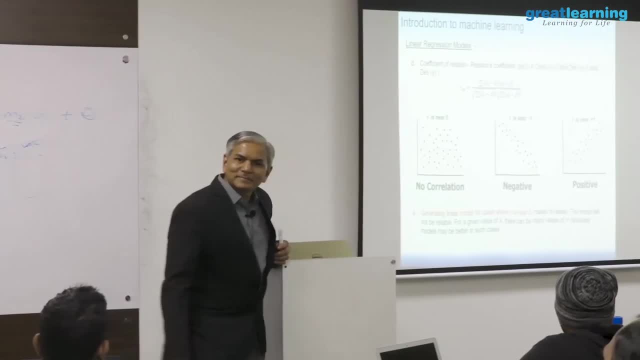 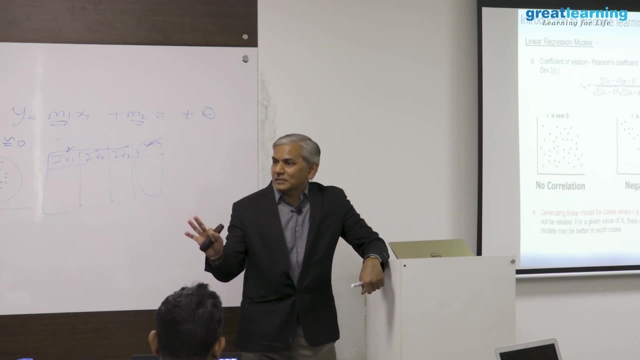 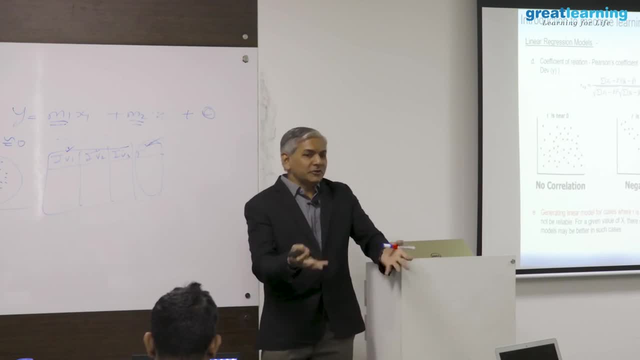 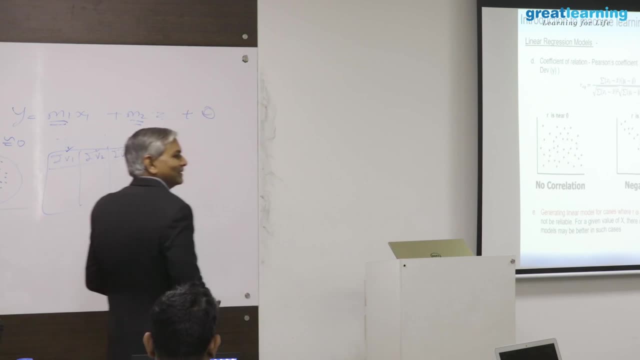 Understand the concept. All the formulas are there in the library. We just need to call those functions and get our things done, But get the concept in place. Yeah, Sir, if I have different units of my circuit, independent of different values, how does? 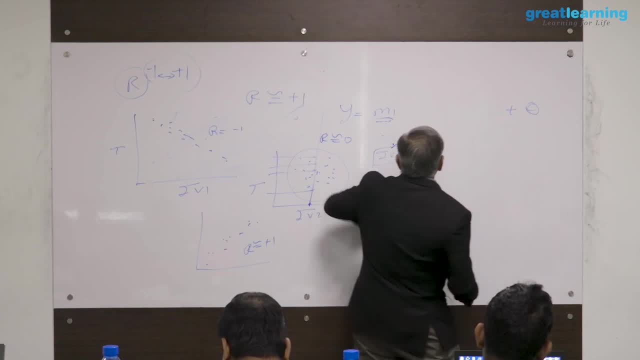 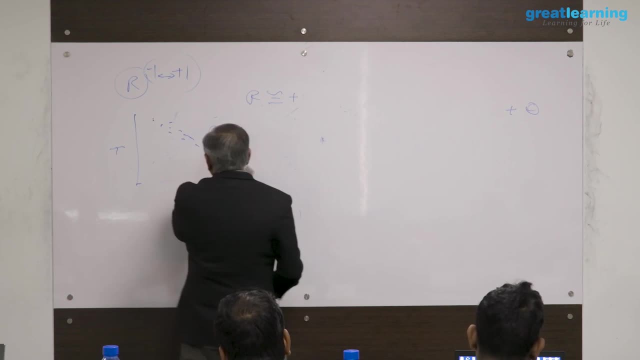 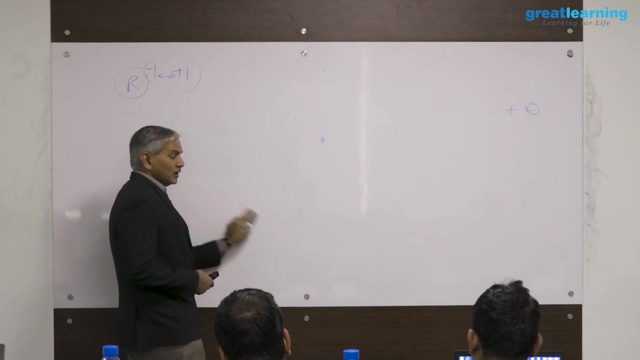 the r value. in that case, work Does not matter. R value is a measurement based on the spread of the data. Now have you heard of scaling? Scaling, Yes. Linear model is one model: linear regression, where scaling has no impact. 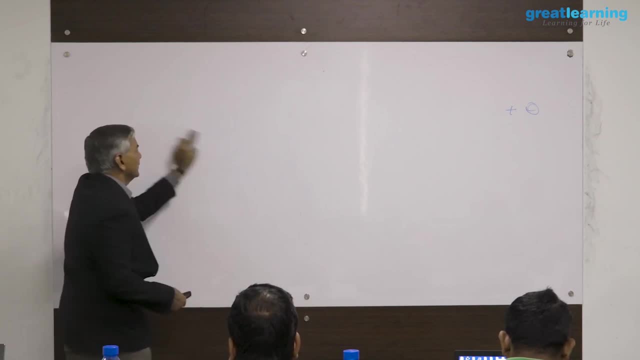 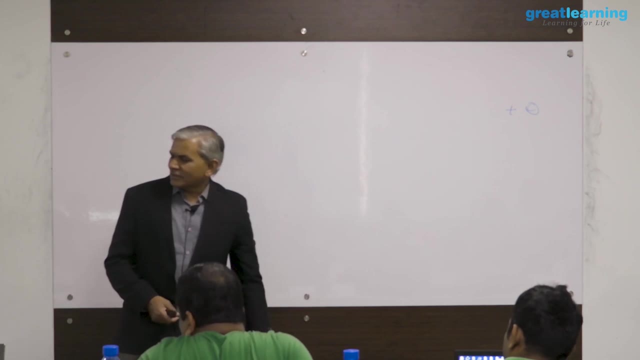 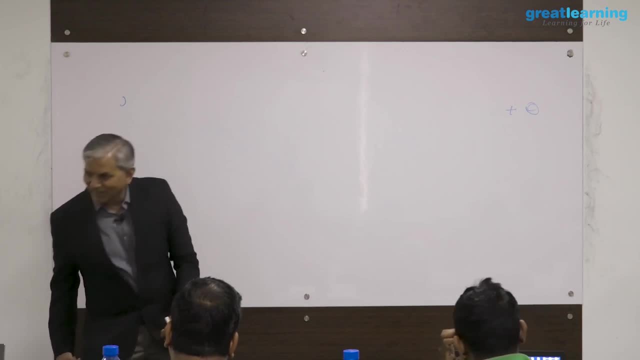 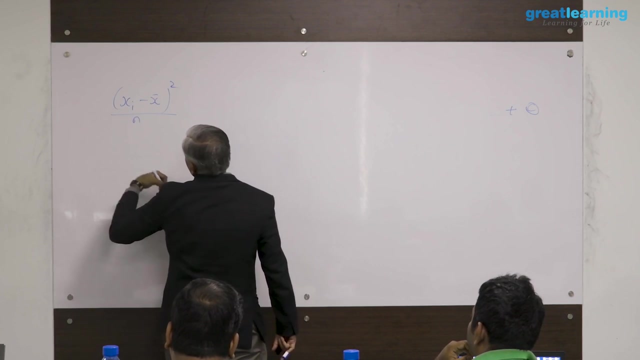 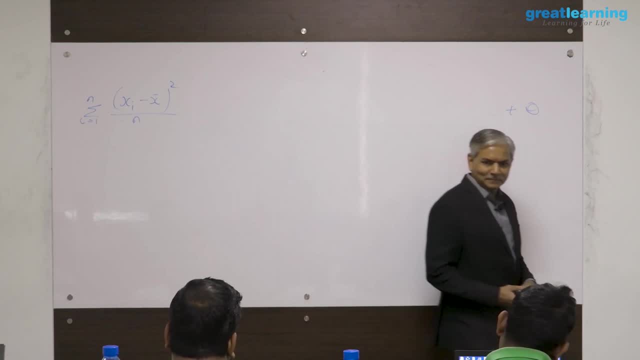 mu various x minus mu. square x minus i. I minus x бар, you can call it mu. the whole square n I is equal to 1 to n. Let us keep it n, but otherwise we use n minus 1.. 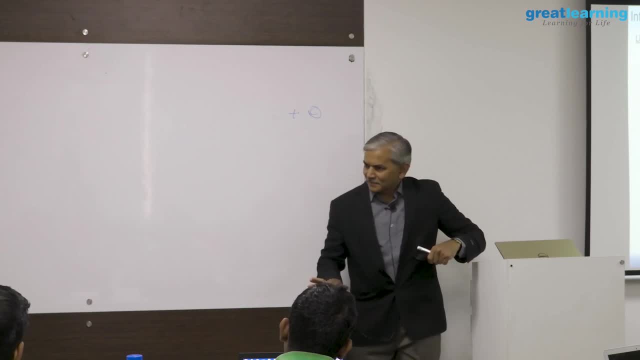 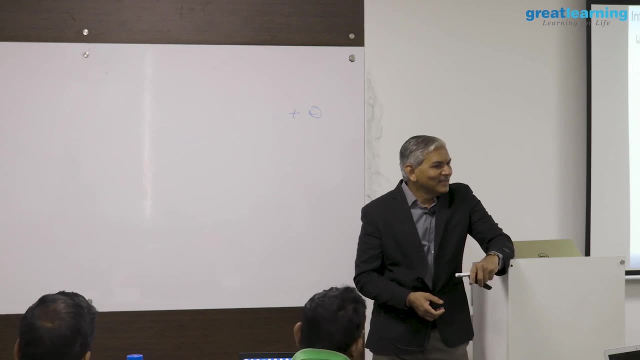 If sample size is less, we use n minus 1.. All of you OK with this? Do not worry about these things. What is this variance? Thank you, I know it is spread. what is it telling you? What is central value? what is x, bar or what is mu? what is the central value? Do not give. 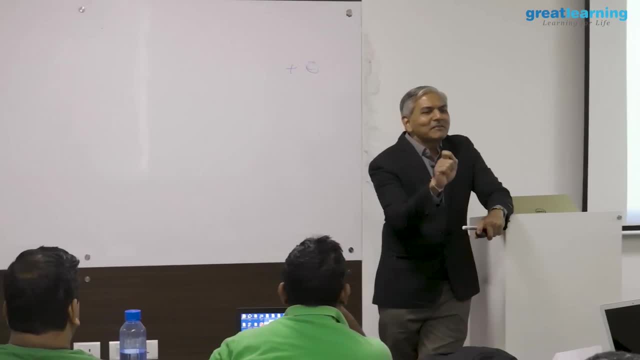 me the formula. do not give me the formula. I know the formula. Central value is a value which represents all the data points that you have. ok, So if I take all your heights, add it up, divide by a number of students in the class, that will be average height. 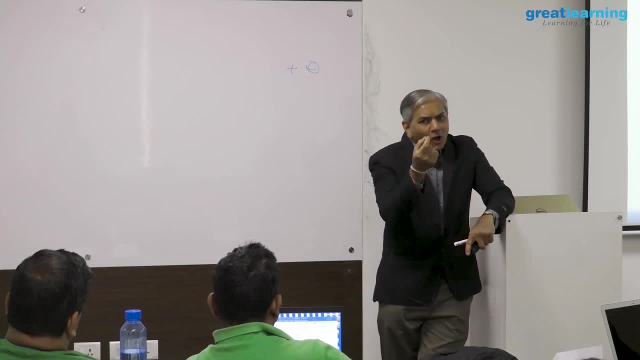 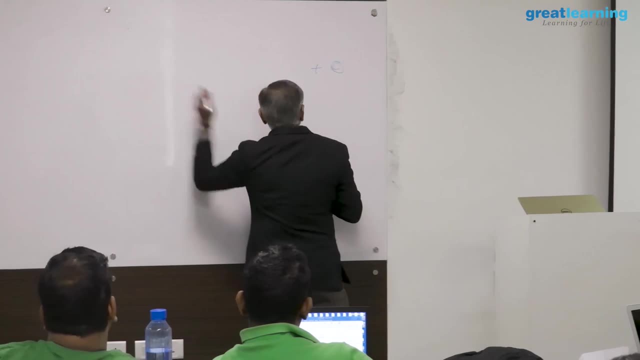 of a student in this class. Now how good this average is. First of all, why do we take averages? why do we need mean and median? why do we do all these things? There are many. that is statistical answer. yes, you are right. 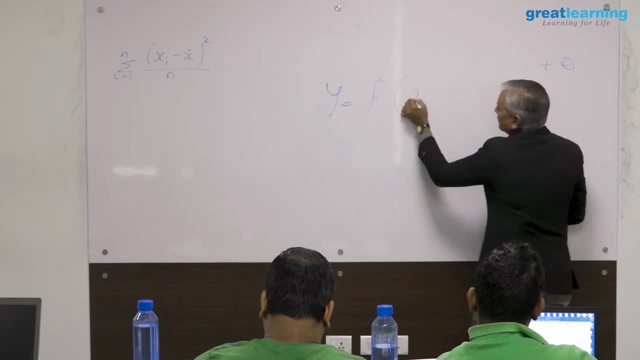 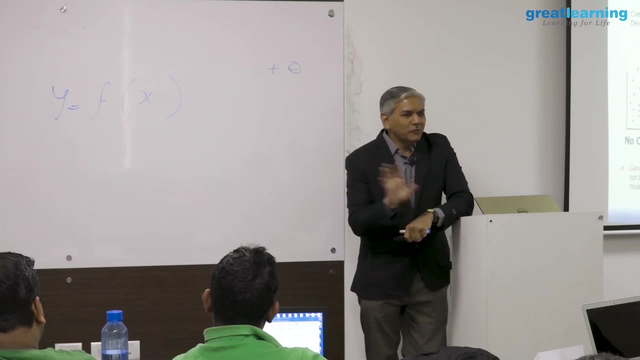 But many times in data science you will come across a situation where you have a function and the function takes as input only one value to predict something. Now, which one of the values should I put? There are 30 students in the class. each one has a different height. 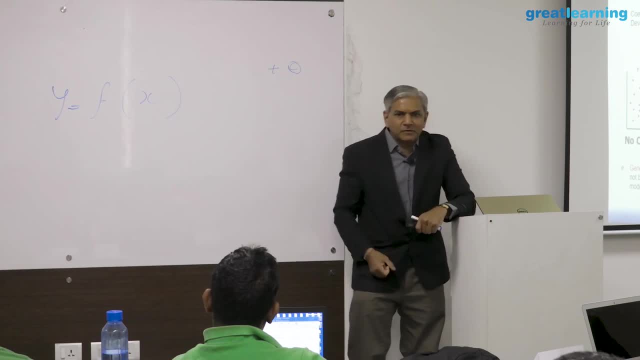 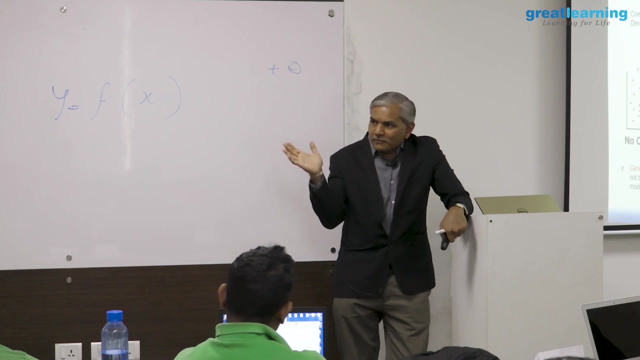 right, I want to say: order some kind of a code for all the students in the class, a great learning stamped code. Now, what size should I tell the manufacturer? I cannot give different sizes and one unit of every size, So I have to give some size which will represent all of you, so that all of you can fit in comfortably. 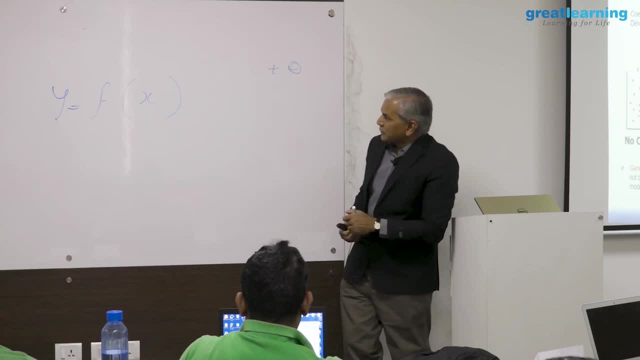 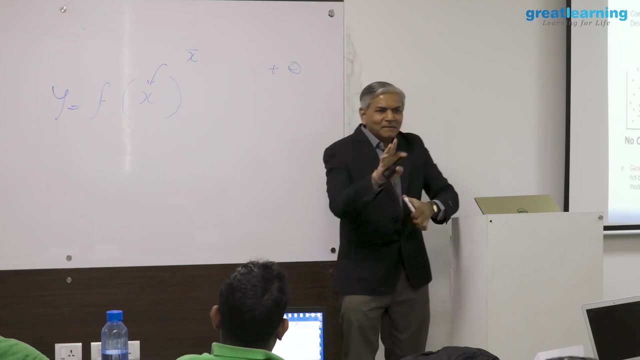 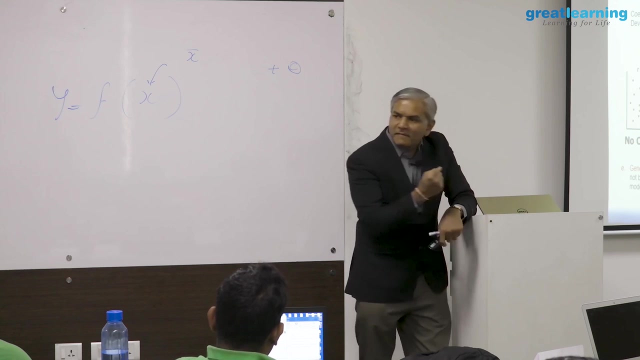 right, That is the idea. ok, In such situations we need to input only one value. So we what we do is we find the x bar or the mu, But the question is: how reliable is this x bar? Suppose average height of the student in this class comes to 5.5.. Some of you might be six. 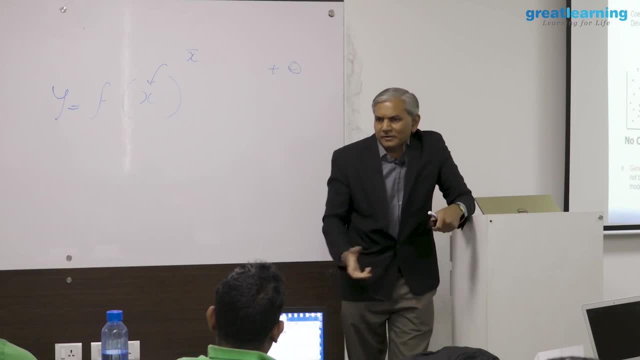 footers. you might get often the dual say: boss, I am six footer, how can you say I am 5 footer, 5.5.. So how reliable your central values is, based on which you are going to do further actions. how reliable your central values is that reliability is given by the measure. 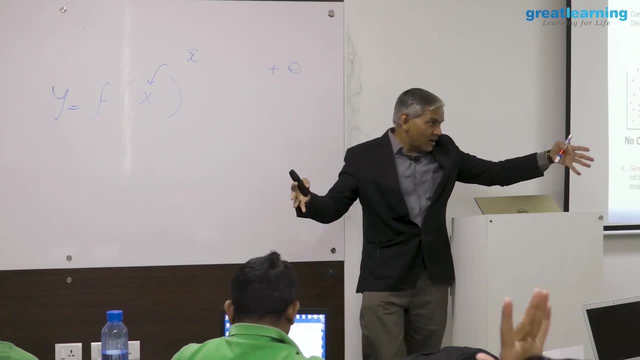 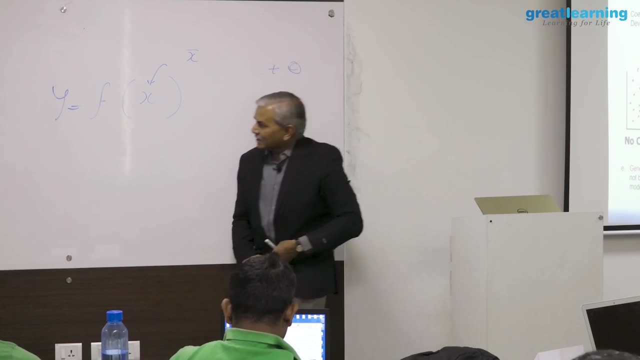 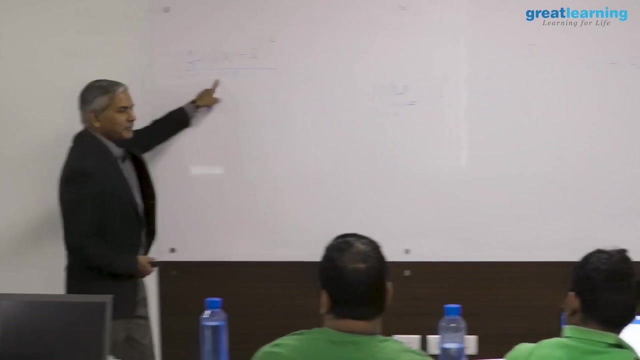 of variance. If the variance is too large, the central value is not reliable, right? So the variance gives you the reliability of the central values, How reliable the central values are. So the formula for variance is this right? Just look at the numerator, just look at the. 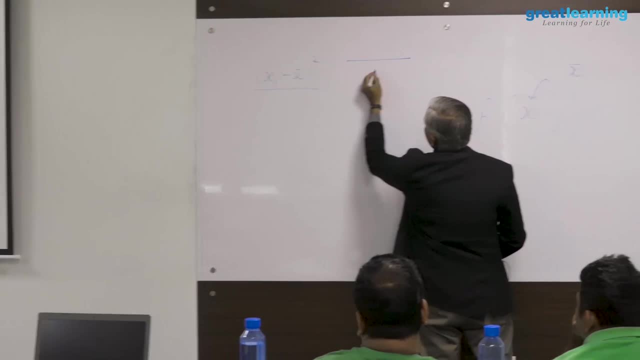 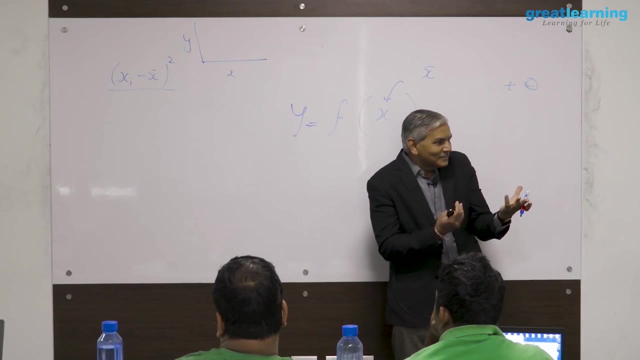 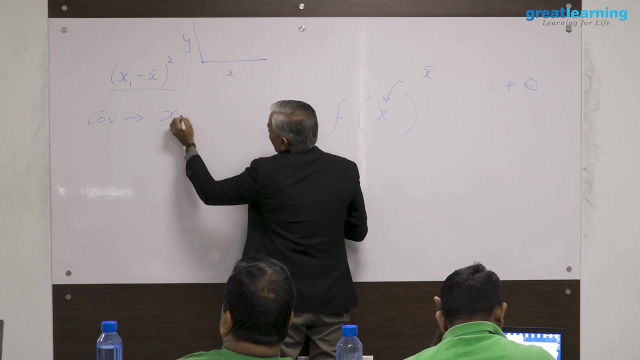 numerator. This is the case when you have only one variable, x. Now I have two variables, x and y. I want to see how they vary together, how they influence each other, vary together. That is called covariance, which is given by xi minus x bar, which is equal to x bar. 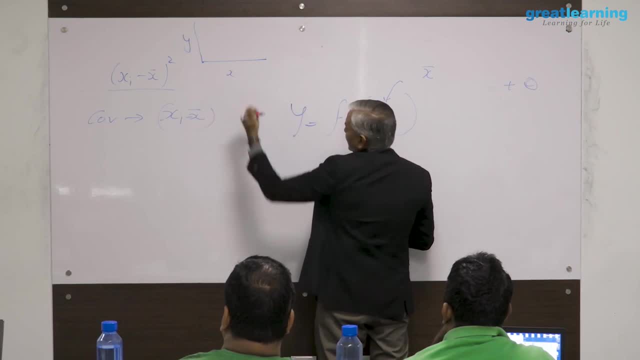 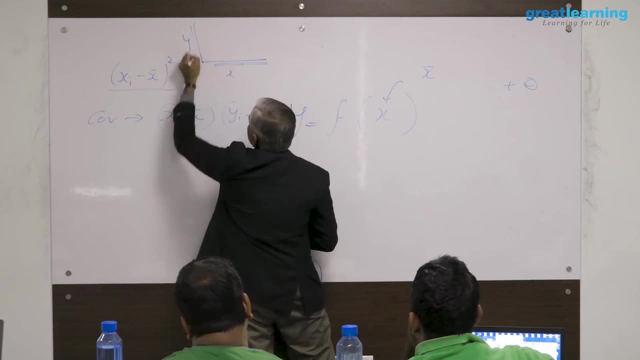 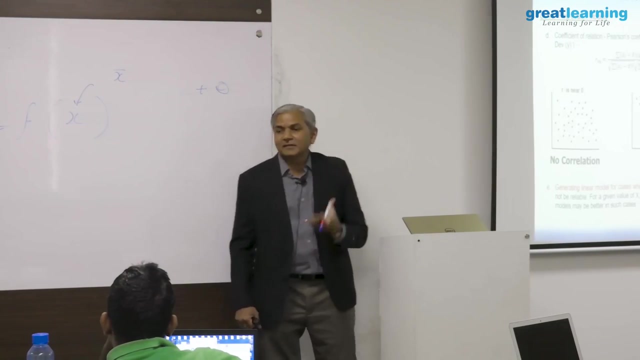 We do not square it into yi minus y bar, So we find out xi minus x bar multiplied with yi minus y bar. That tells me how the data points in the feature space. they vary together. That is called covariance. 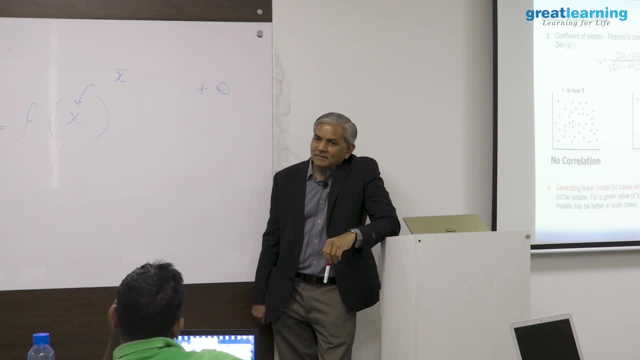 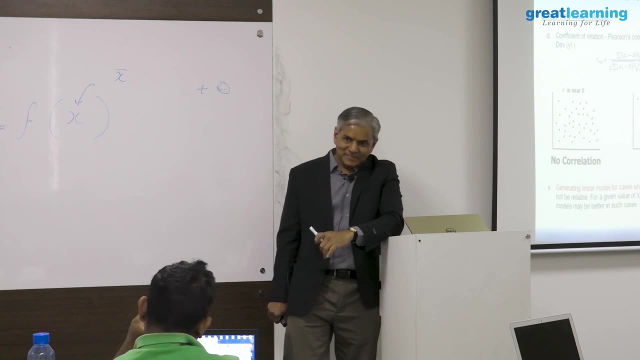 So they should not vary together to have a right covariance. Independent variables- independent variables. Independent variables should not have covariance. Target variable and independent variables should not have covariance. Target variable and independent variables should have strong covariance, Otherwise you do not use those independent variables When you are building linear models. the target: 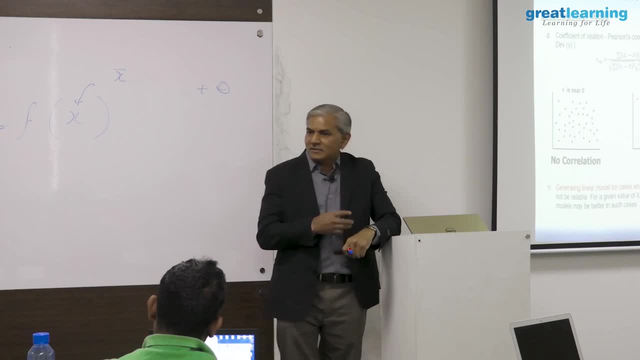 variable, the y, and the independent variables. ivs should have very strong covariance, But within the independent variables the covariance should be 0. That is an ideal situation. Practically it never happens Now, given this covariance. now we will look. 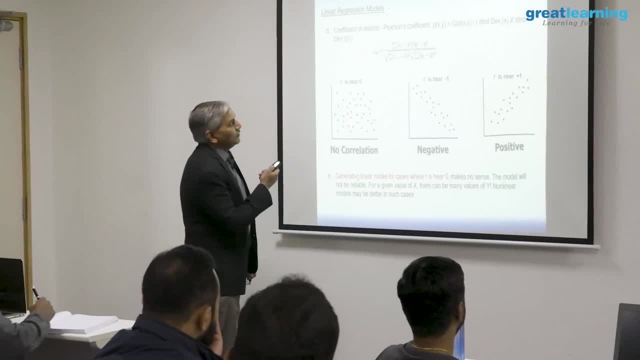 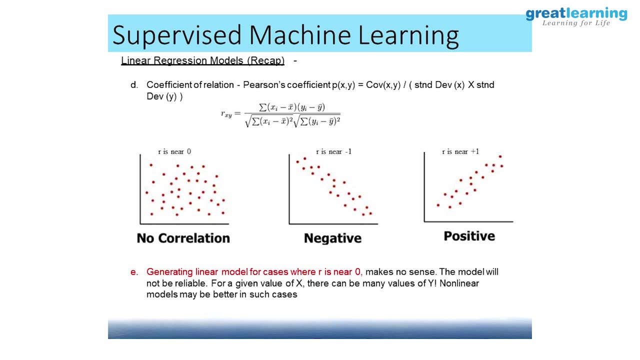 at the formula for r On the top in the numerator, you are seeing covariance and if you look at it carefully, the units on the top and the units on the denominator are same. This is also xi minus x bar. this is also xi minus x. this is yi minus yi bar. this is also yi. 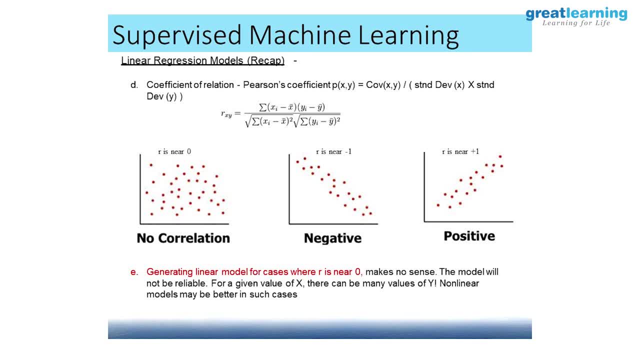 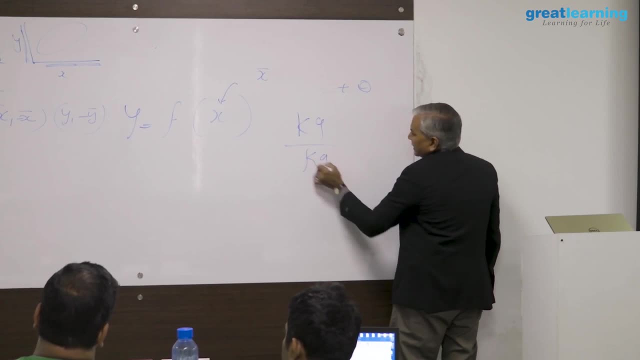 minus yi bar. It is a square term, but there is an under root. This is also square term. it is an under root. So both numerator and denominator are going to have same units of measurement agreed. So if I have a kilogram by kilogram case, then the units cancel each. 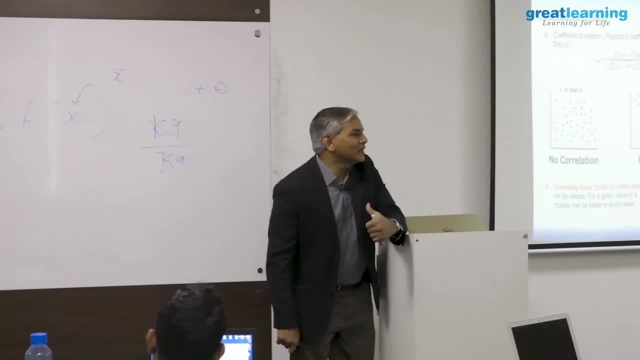 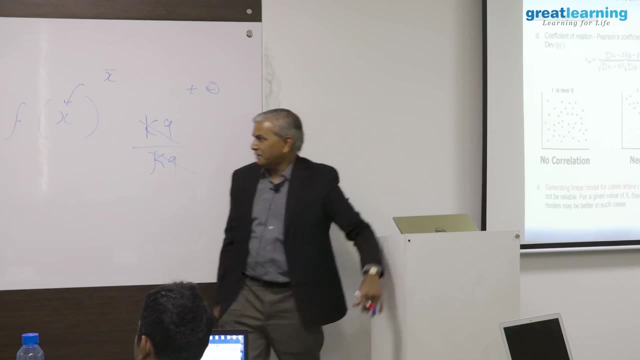 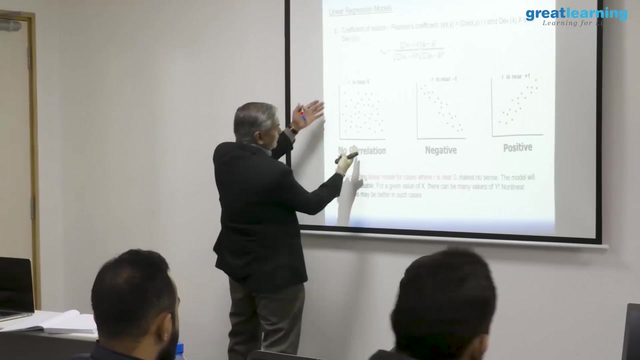 other out, It becomes a unit less quantity, it is a ratio. R value is a ratio. ok, Now, when you have a diagram, when you have a plot like this, between two variables could be independent variables, target and independent could be anything. When you have this kind, 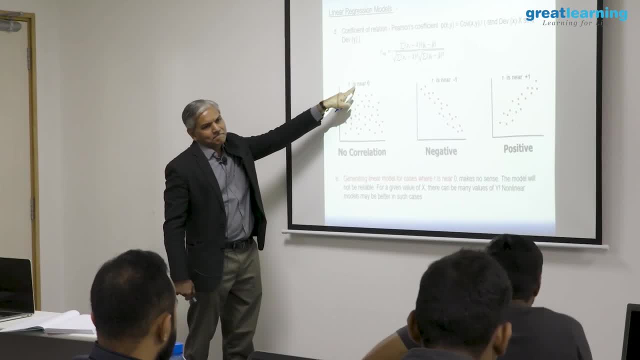 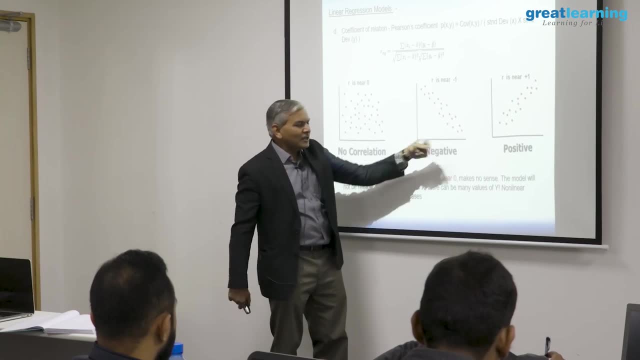 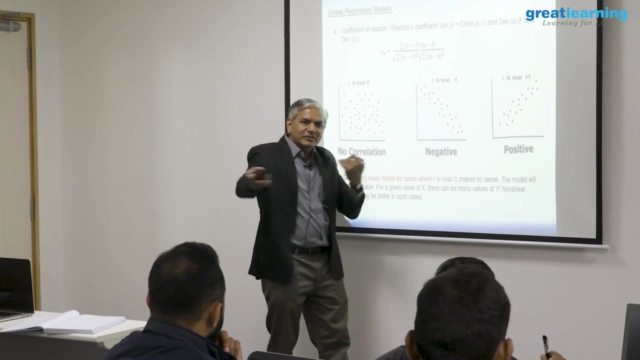 of plot, you will see that R value is close to 0.. We will see why this happens When you have this kind of a plot where you see a trend but as X increases, Y decreases, they are going in different directions. X increases, Y decreases. they are opposing each other. 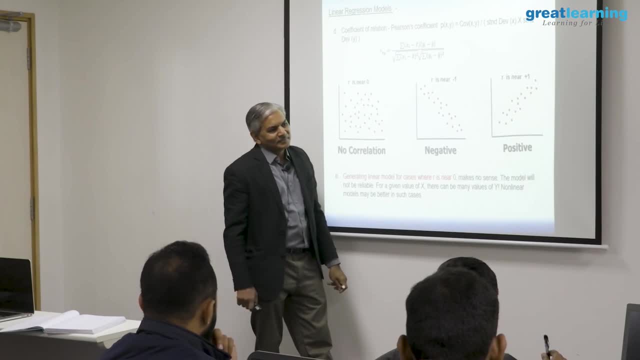 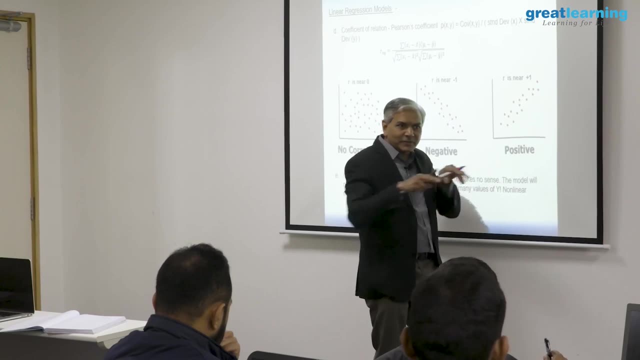 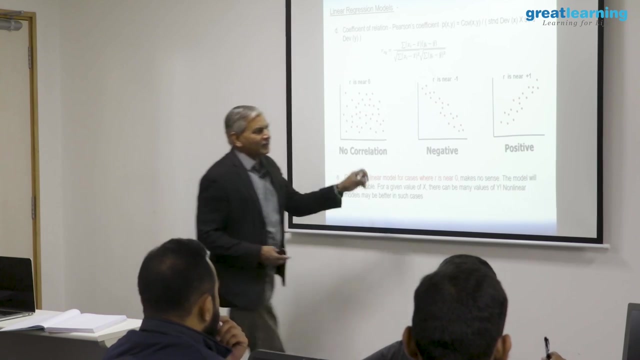 Then we will have R value close to minus 1.. Whenever they go hand in hand- when X increases, Y also increases- they go in the same direction together. Then R will be close to plus 1.. And it is not very difficult to understand why. Let us look at this particular case closely. 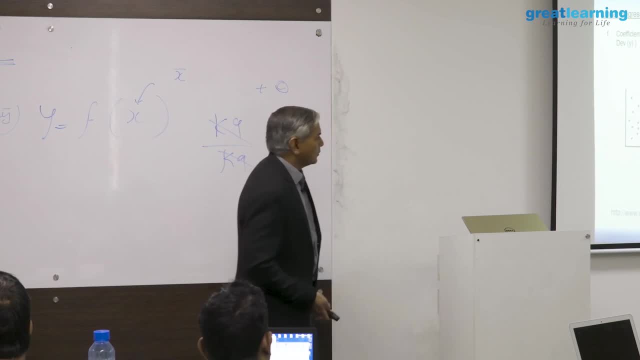 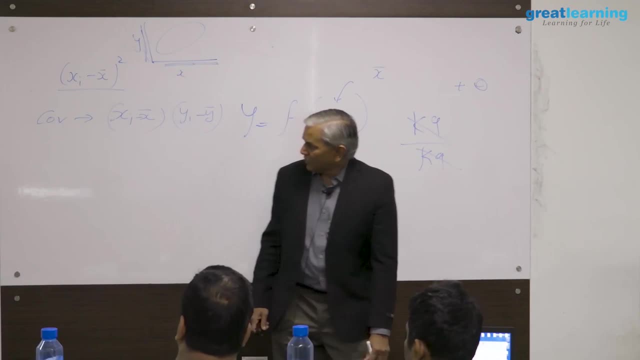 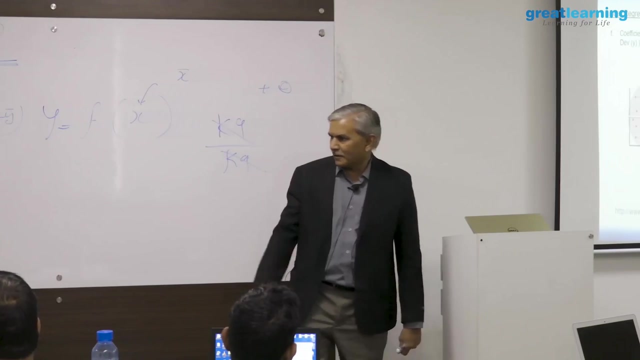 I am going to look at this particular case closely. yeah, This is my mathematical space, or feature space. Both X and Y have some X bar and Y bar, the average right X bar- Y bar. Keep in mind all linear models that we build, linear regression models. they will. 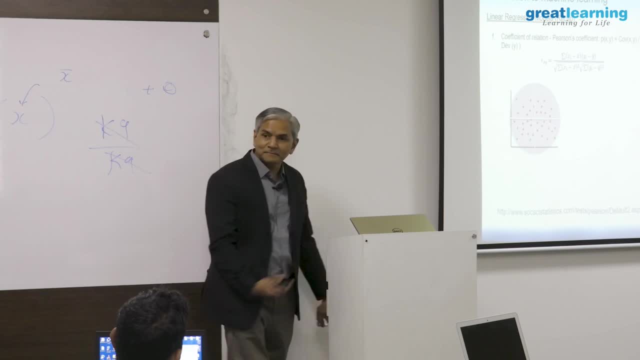 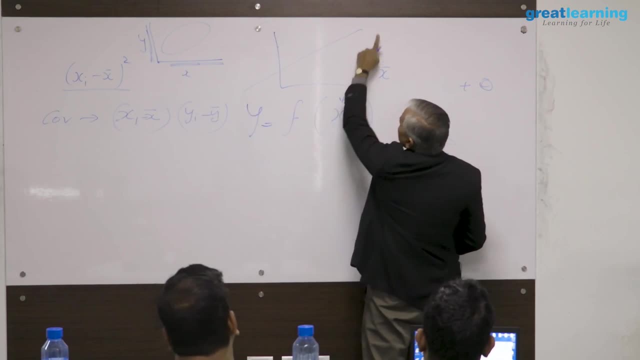 always go through the point where X bar and the Y bar meet. So the linear model that we saw a few minutes ago, this model, will always go through wherever the X bar and the Y bar meet. It will be hinged. hinged on to that point, That point will act. 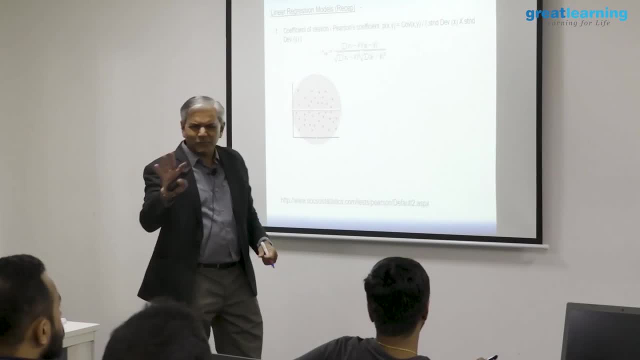 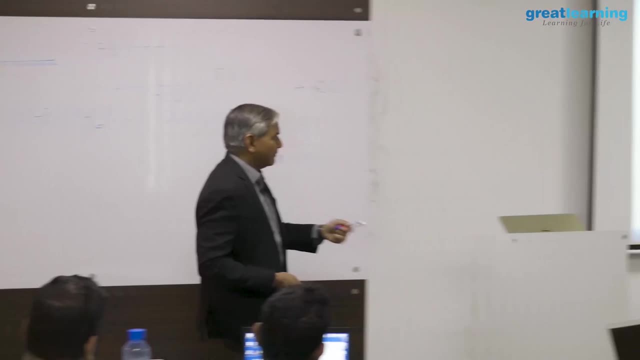 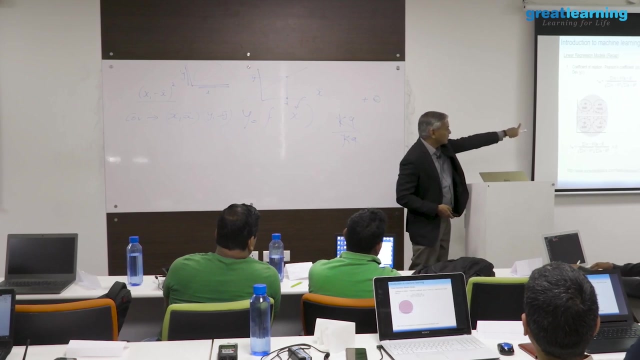 as a fulcrum, alright. There is one particular point: that linear regression models will always go through X bar, Y bar. I am really surprised and I find it very difficult to understand why this is not told. Now. look at the look at the points over here. ok, Let us look at. 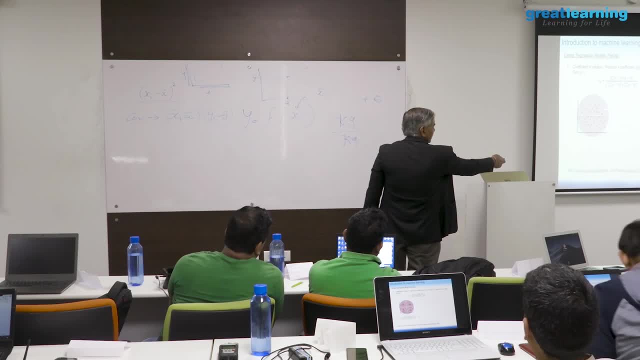 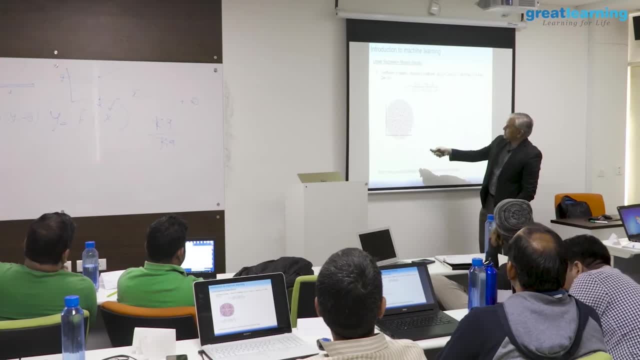 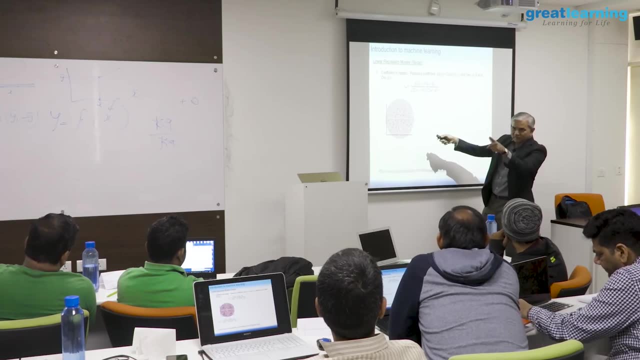 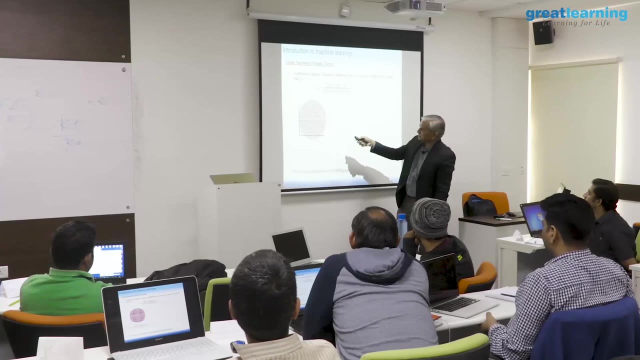 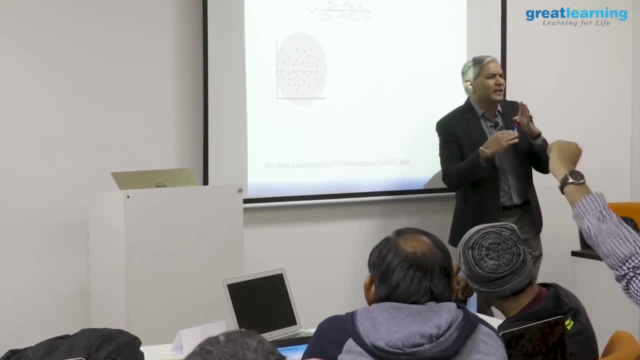 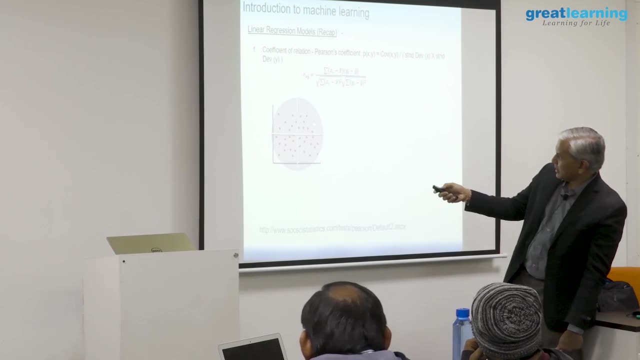 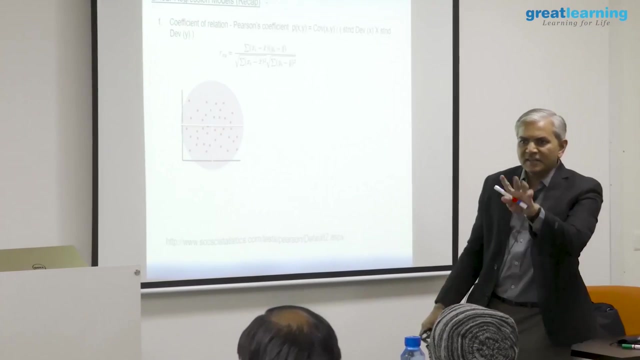 yi minus y bar is positive. so when you multiply these two, it is like finding the area of a rectangle length into breadth, So xi minus x bar into yi minus y bar, for this point is nothing but the area it covers over here. this is the area. This area is a positive. 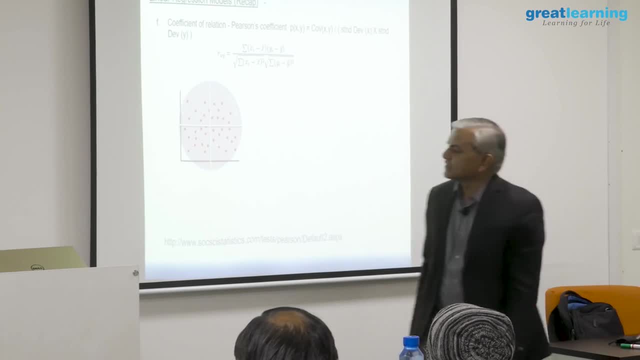 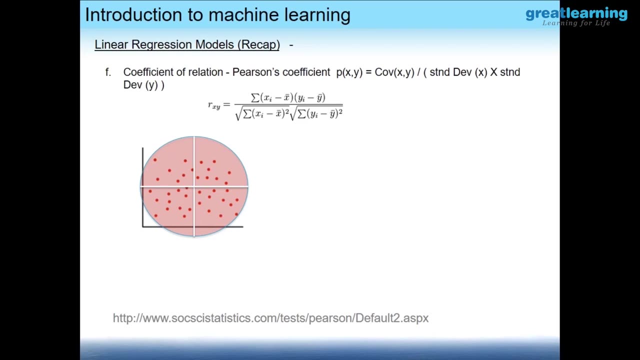 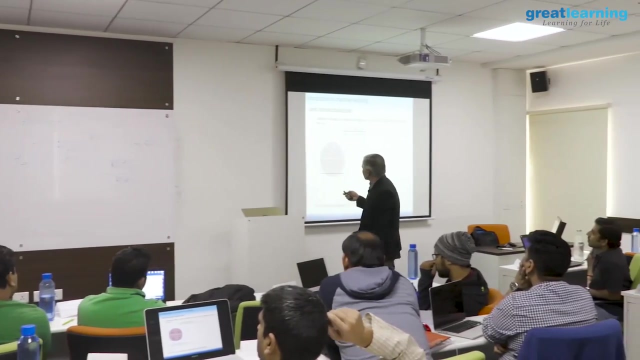 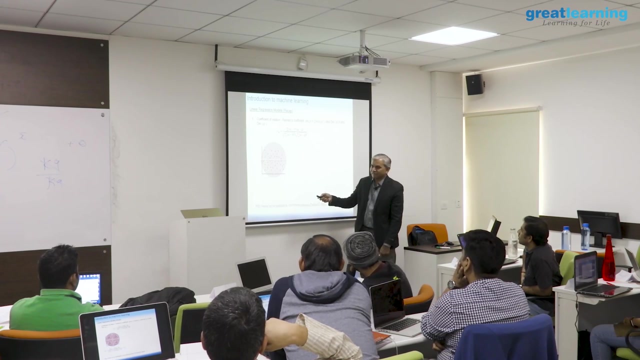 area, All of you. okay, Let us take another point at the bottom of the screen. say this one: For this point, xi minus x bar, x bar is greater than xi, so xi minus x bar is negative. So for this point, xi minus x bar is negative. yi minus y bar is also negative, Negative. 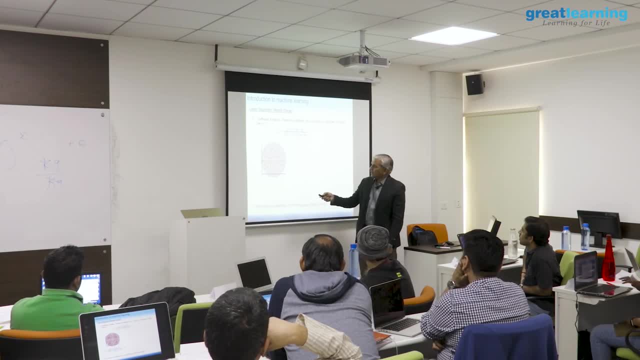 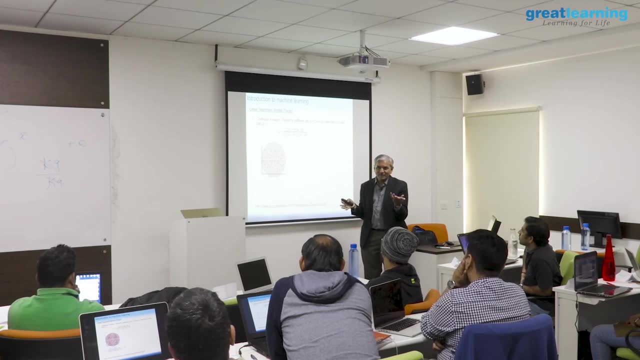 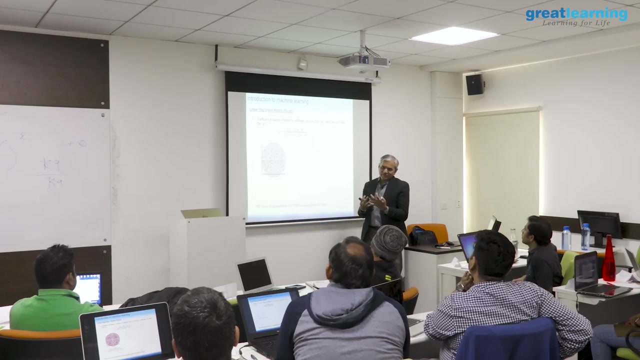 into negative becomes positive. So all the areas over here will be positive. all the areas over here also will be positive. Agree, Take this point: xi minus x bar is negative because xi is less than x bar. negative yi minus y bar is positive. So positive into negative will give you negative All these. 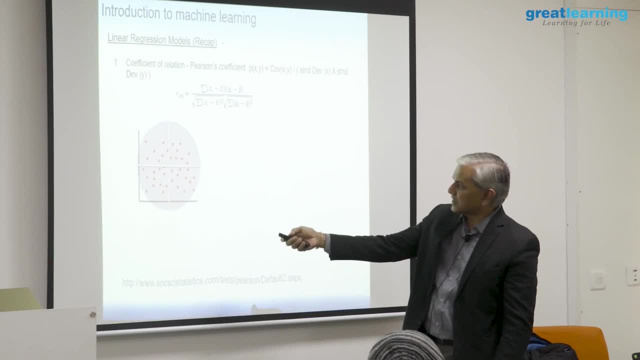 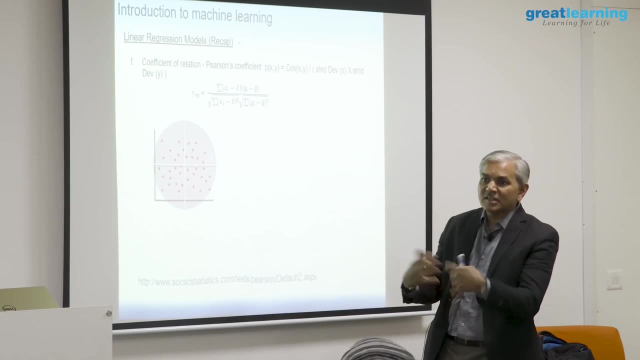 data points will have negative areas. All these data points will have negative areas. When you total this up, sigma- you see sigma over here. Sigma means sum up all the areas. When you sum up all the areas, you will get negative. When you sum up all the areas, you 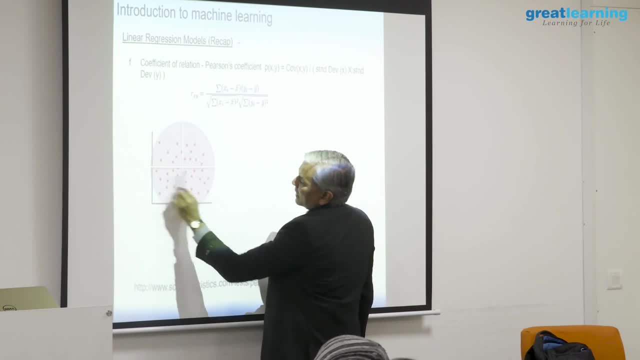 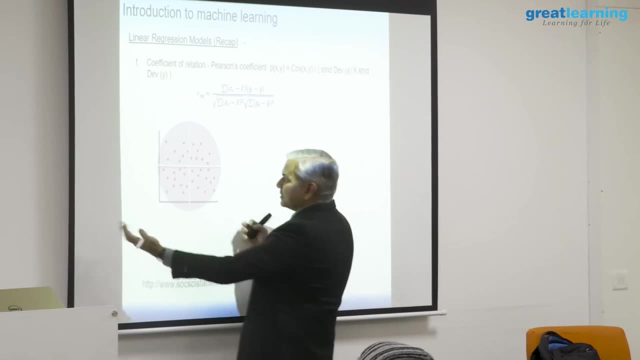 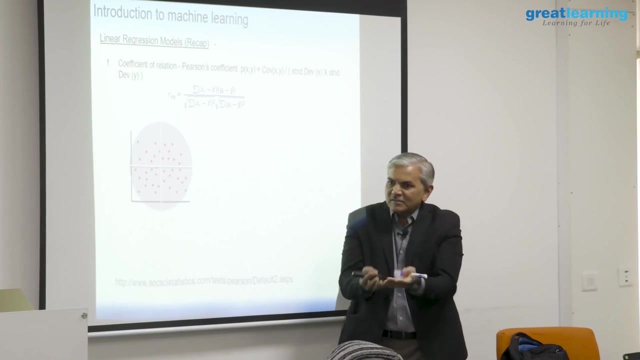 will get positive When you sum up all the areas here. all the positives and the negatives will cancel each other out. The reason why they will cancel each other out is each quadrant has same density of these points. The points are distributed like a symmetrical circle. 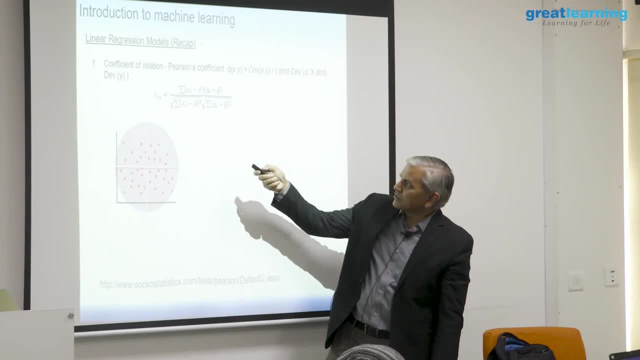 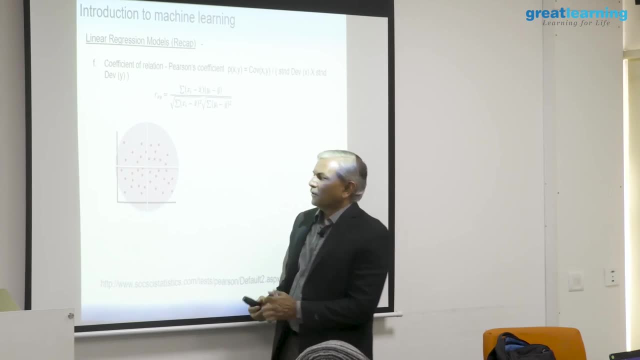 So whenever r value is close to 0, that is because your numerator is becoming 0. Numerator becoming 0 means your distribution is like this: For a given value of x bar, x bar is equal to 0.. So the value of x. I have multiple values of y. Which y should I take? I do not. 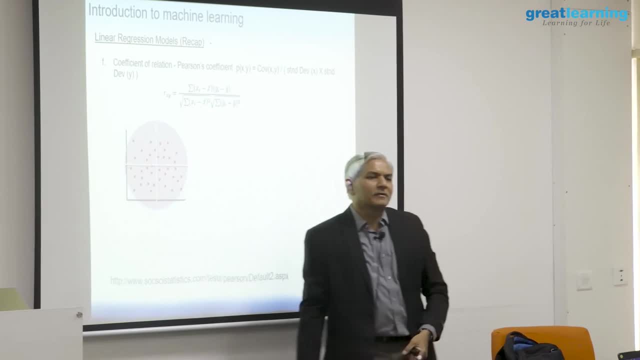 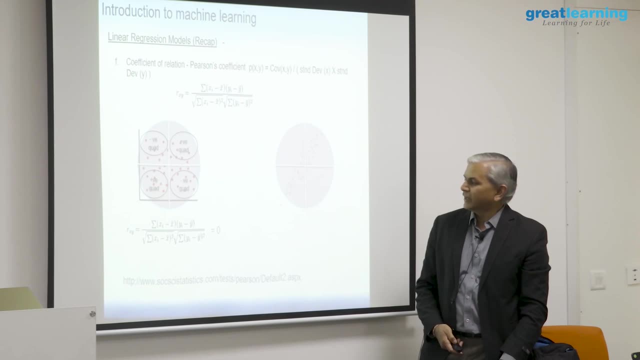 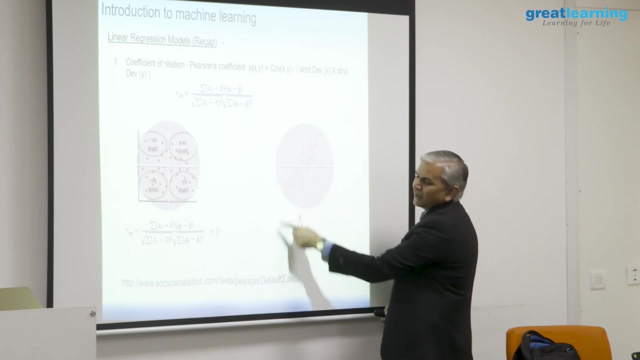 know. So we say that x is not a good predictor of y. On the other hand, if you take another, this plot, if it becomes tighter, then positive areas is greater than the negative areas. So r value will be close to plus 1.. It will become 1 only when all the data points lie. 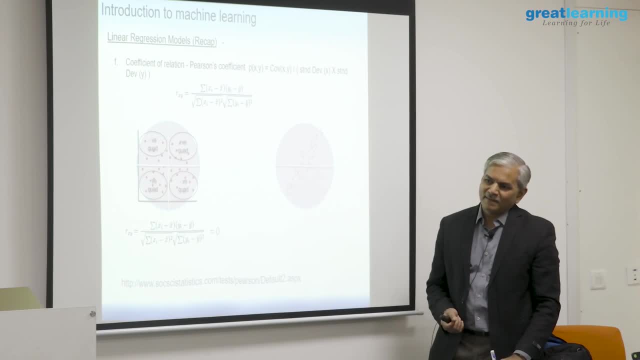 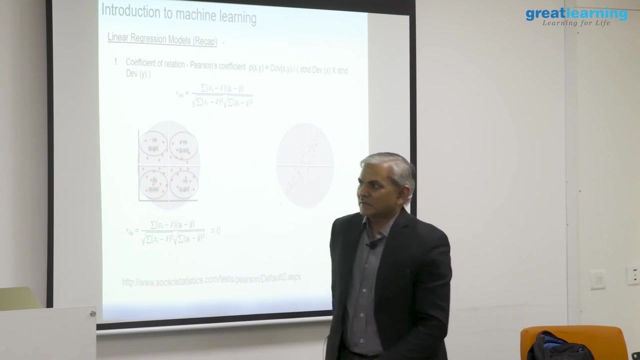 on a straight line, which will never happen. If this plot was this way, all the negative areas will overwhelm the positive areas. then r value will be close to minus 1.. Right, All of you? okay, So this is a concept of r value. So what we do in linear models is we test. 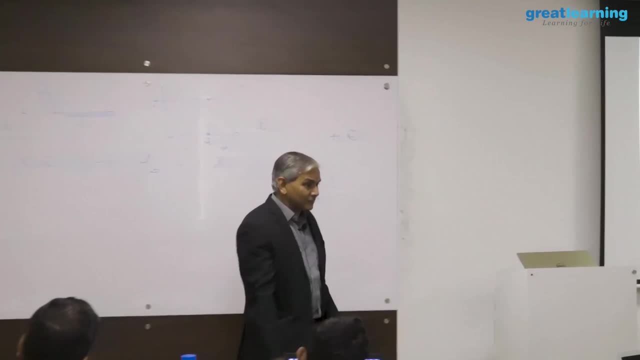 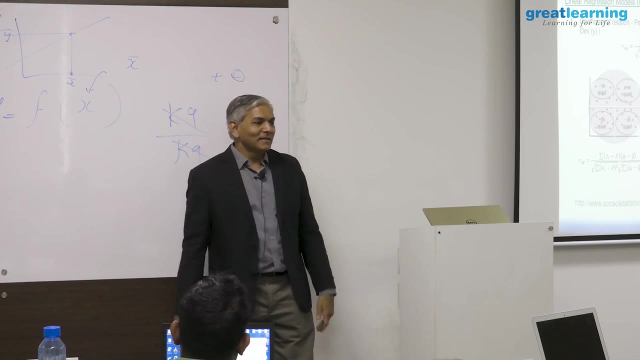 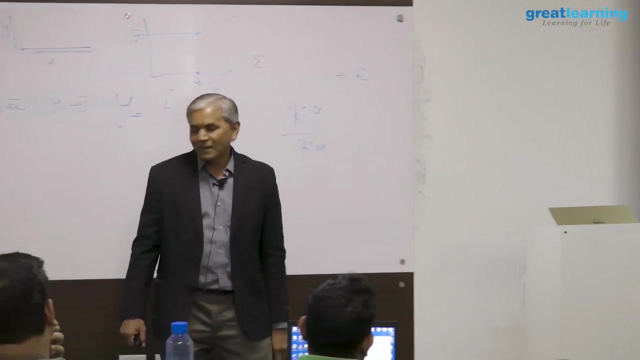 the r values of every independent dimension with the target variable. We select only those whose r value is either close to minus 1 or plus 1.. Any dimension with r value close to 0, that dimension is a useless dimension. How close to 0 is useless, That depends on. 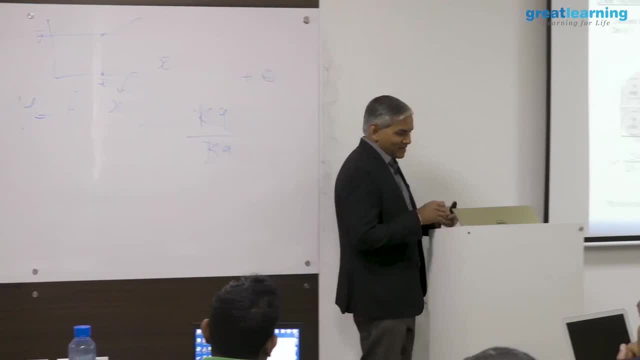 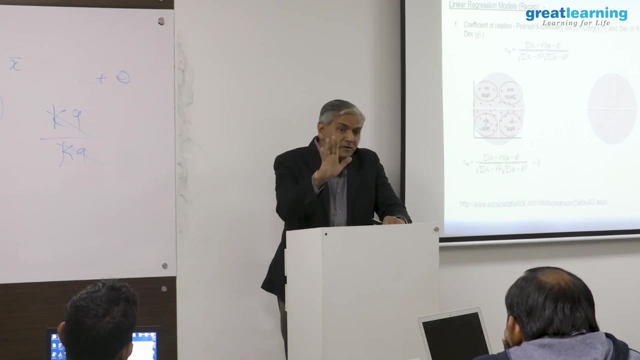 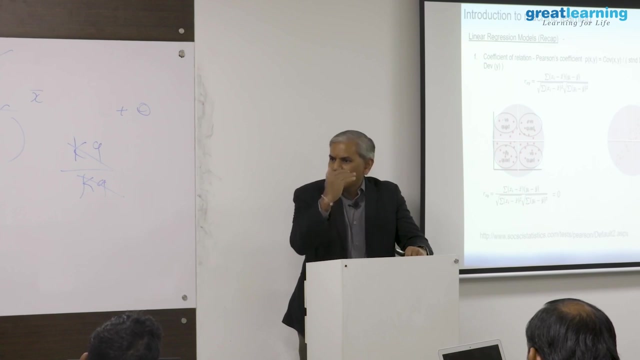 your particular problem statement. So generally, any r value greater than 7,, 0.7,, minus or plus, it is considered as a good variable. Any variable with r value between 0 and plus means 0.5 and 0.7,. it requires further research whether this relationship is real or is it. 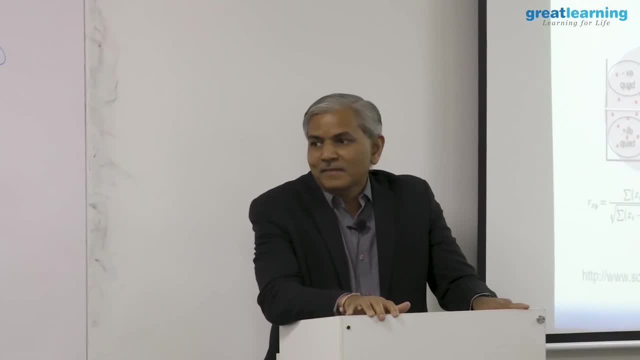 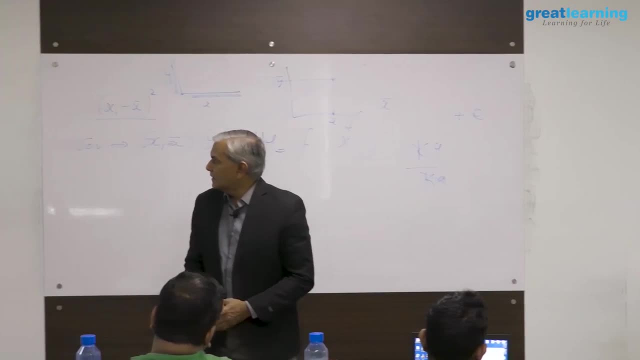 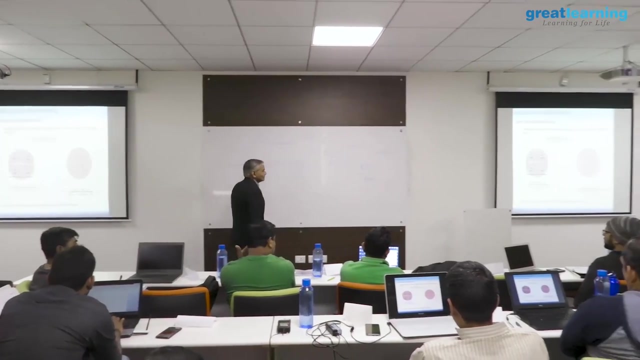 a fluke by chance that you are seeing in your data set Any r value close to 0, not worth considering. What about the second case? you told fluke. what does it exactly mean? I do not understand. Why is it fluke? 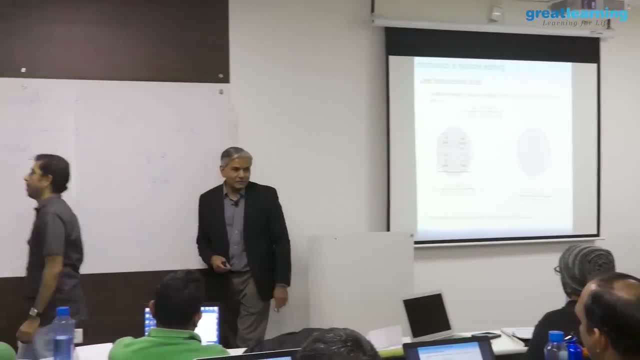 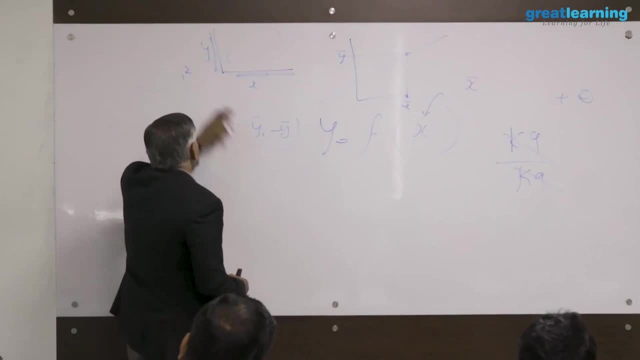 It could be a sampling error The way you selected your samples. something like this: in the population that leads to the r value. Now observe this. Since you asked this question, let us discuss this out. For r value to be 0, if this is my x and this is my y, this: 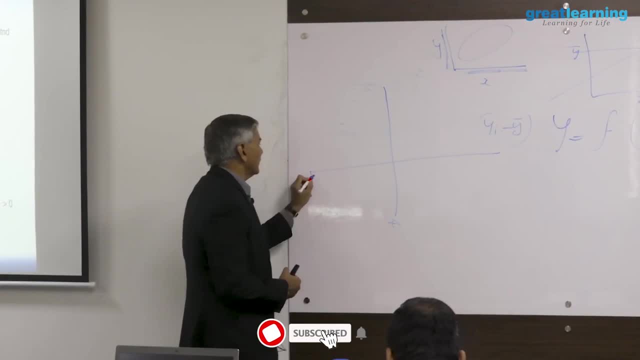 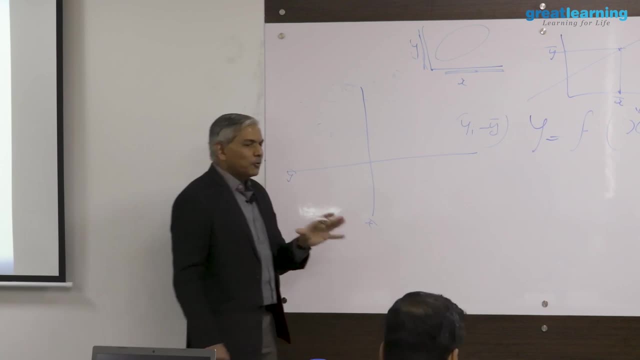 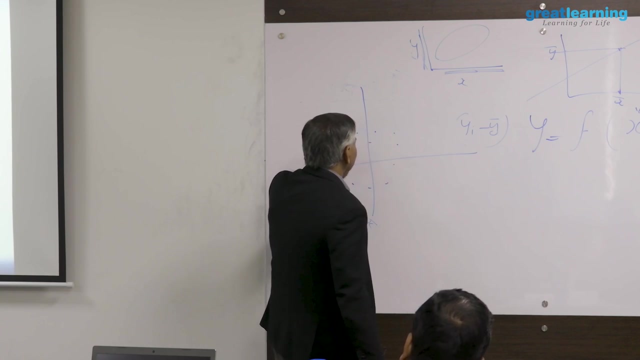 is x bar. this is y bar. I am not showing you the coordinates. For r value to be 0, the data points. suppose I give you 10 data points. the data points have to be absolutely symmetric, symmetrically distributed. 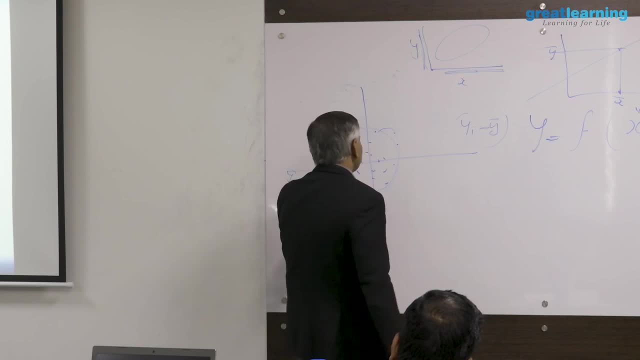 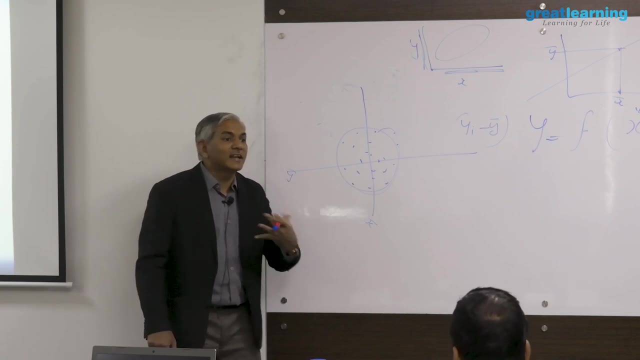 Symmetrically distributed. for r value to be 0, absolute symmetrical distribution in all the quadrants. What is the probability that when you are doing random sampling, you will get data points in such a way that they get symmetrically distributed around this? 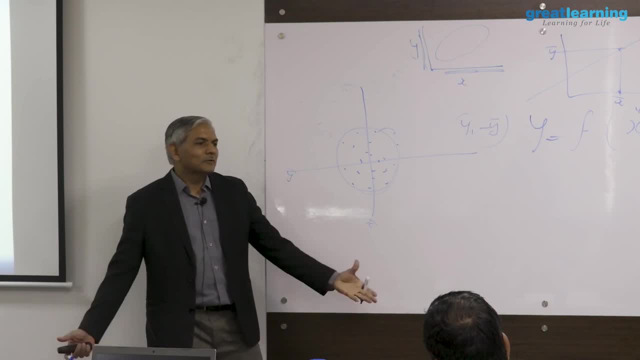 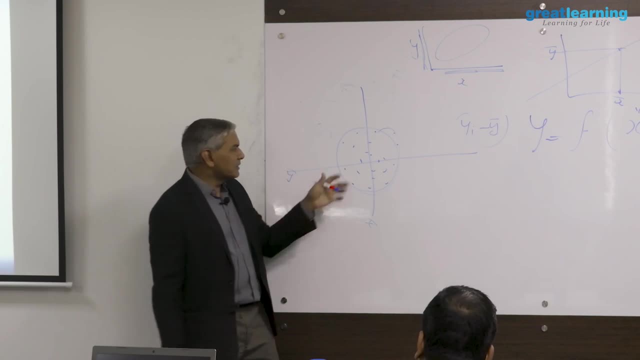 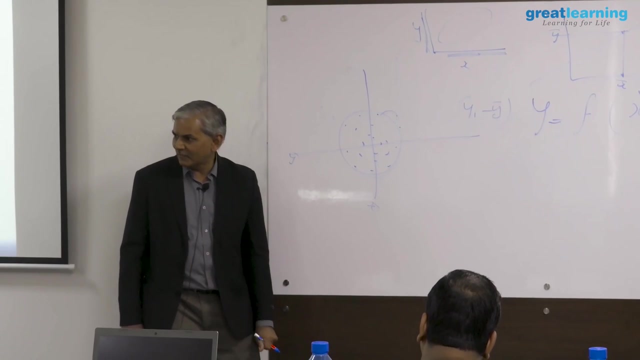 What is the probability? Probability is 0.. That particular configuration of data points that you want from the universe, which symmetrically distributes itself around these two x bars and y bars, to give you the r value of 0.. Ok, That probability is 0. It will never happen. So, even in the real world, if there is no, 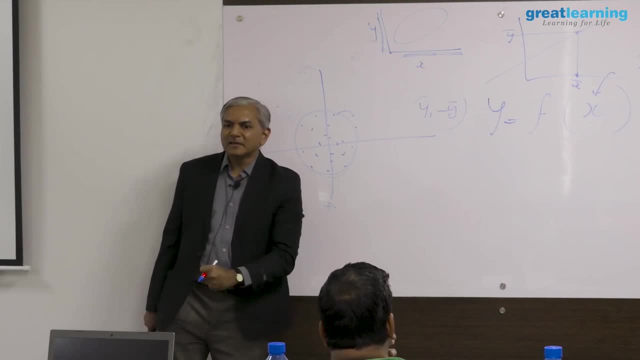 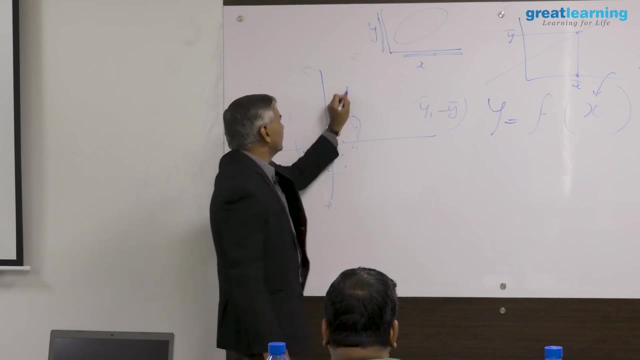 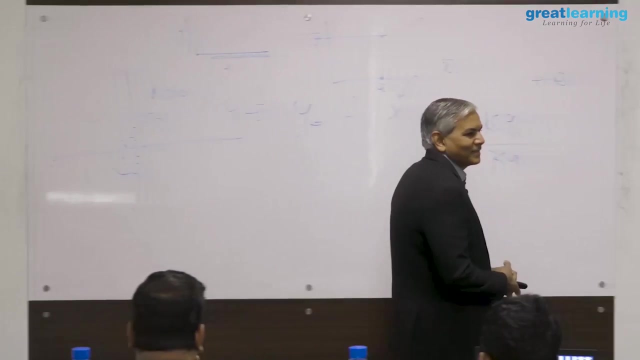 relationship between x bar and y bar because of your sampling. sampling brings in some asymmetry in the distribution. There will be some asymmetry in the distribution. You will end up with an r value greater than 0. This r value- we call it statistical fluke. 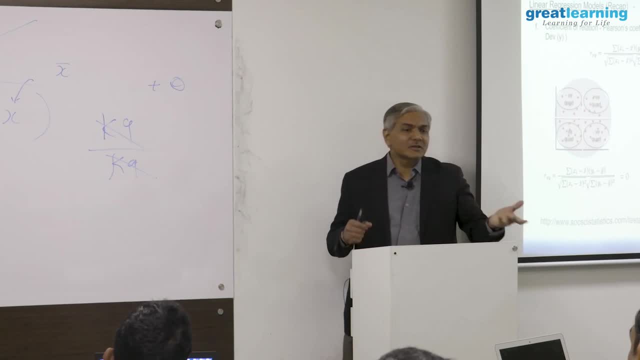 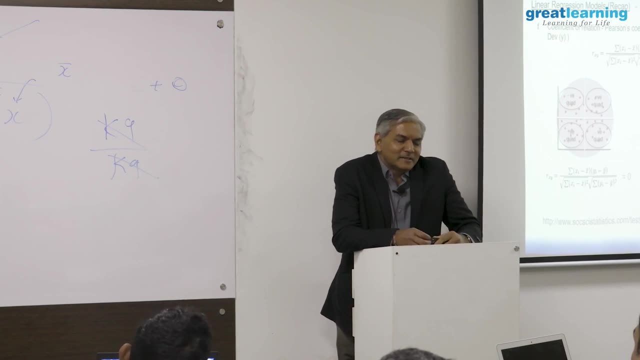 So when r value is very close to 0s, it could be by chance sampling problem. Ok, So if the relationship is real, it may not be a real relationship. So you have to go and further investigate whether the relationship is real. it might be real or is it fake. 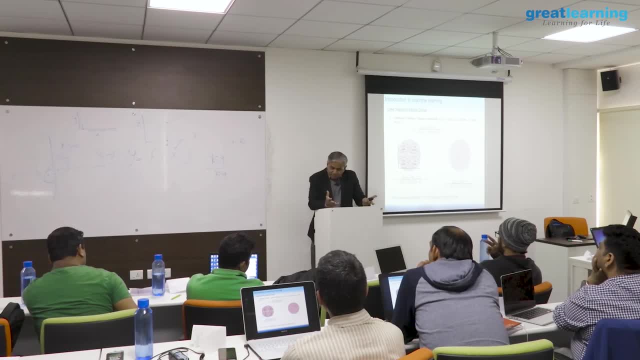 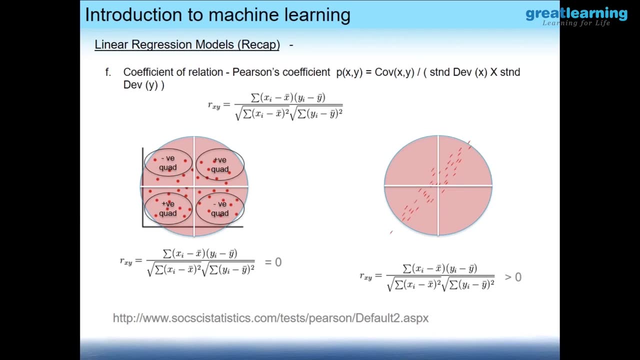 It might be possible also, r value is greater than 70, but it might be a fluke. No, that is very true. That will happen when your sampling is completely gone, case You have done some mistake in sampling When, when it can happen. All right, all right, shall move on. 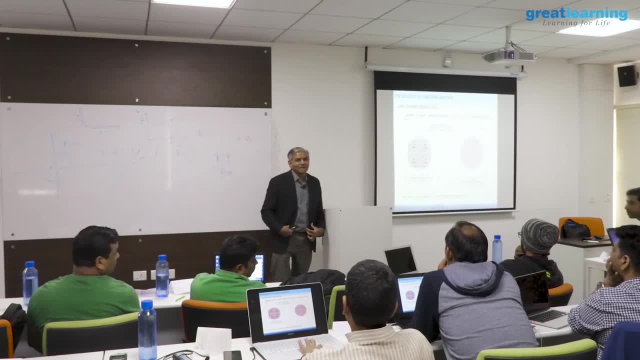 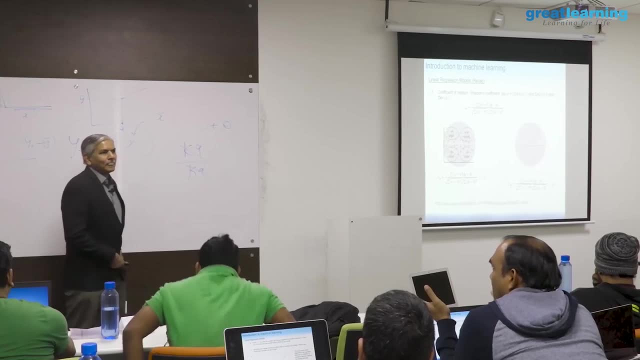 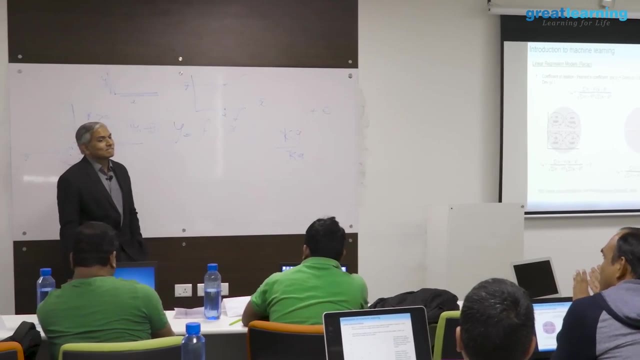 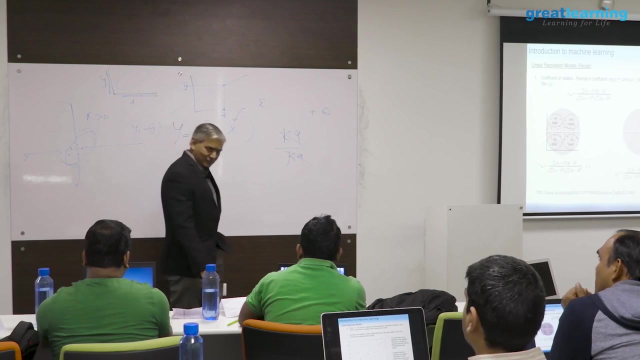 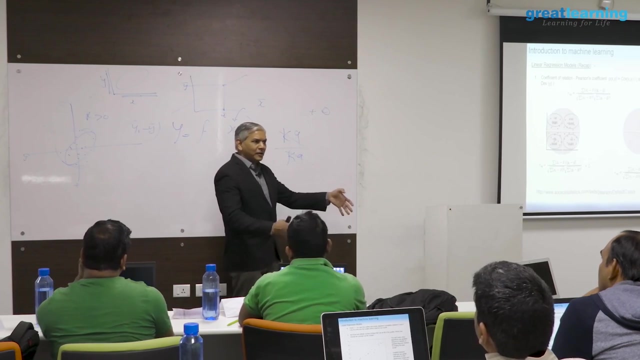 Thank you very much. Thank you, Yes, both case we have to use this. we have to use for both the situations, to select the independent dimensions and, within the independent dimensions, knock out those which are very strongly correlated. So is this, is the only PSN, only the way to find out. 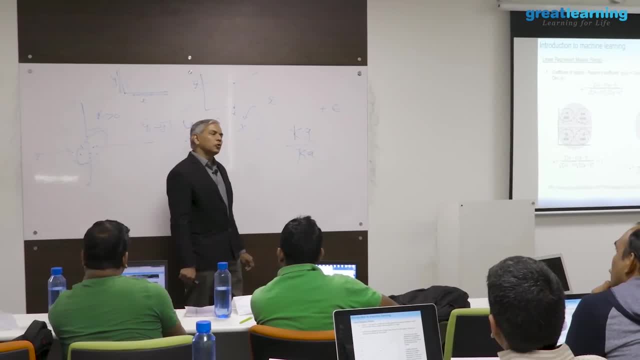 No, no, there are other methods of it. Cal PSN is the most commonly used for correctionalism. There is one more available. There are many such algorithms, But this one which we mostly use in this, our cases Shall we move on. 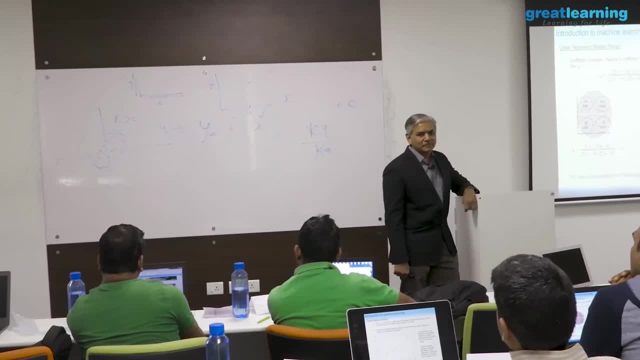 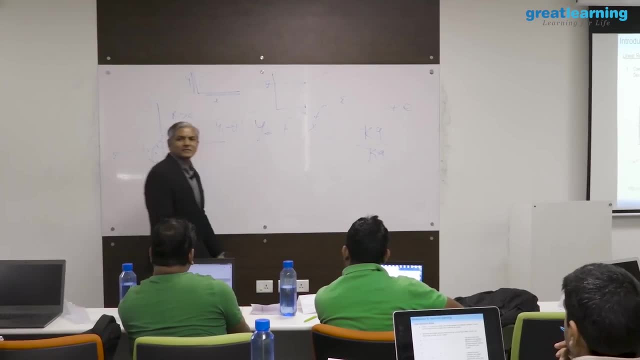 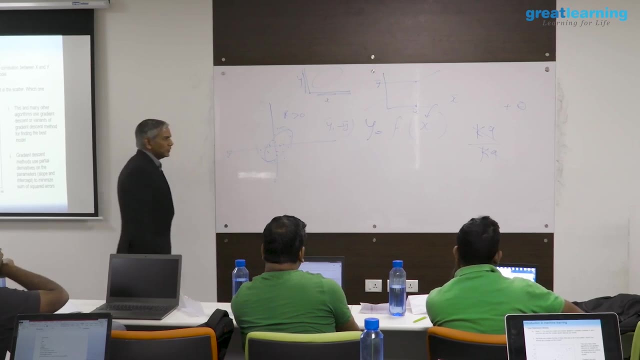 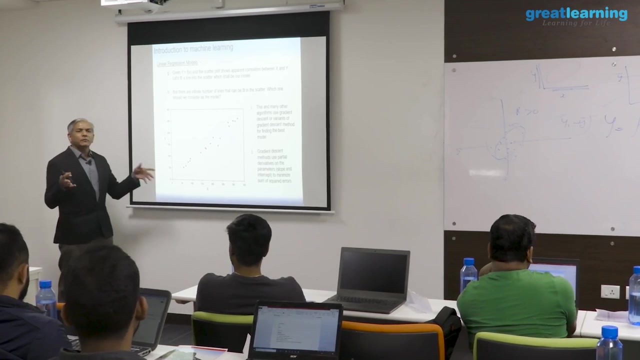 Okay, Now this algorithm that we are going to use. what this algorithm will do is we are going to, given the data set you have. okay, suppose this is the distribution in X and Y. In your data set, you have only one independent column and the one target column. 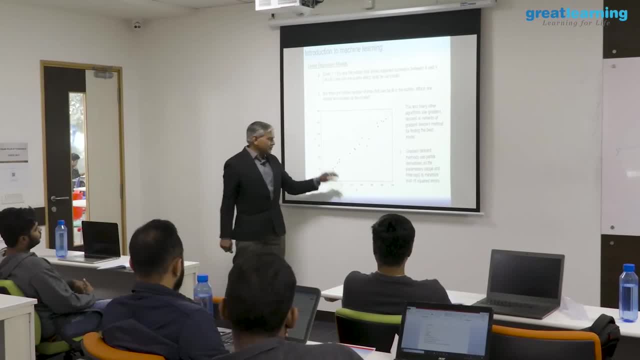 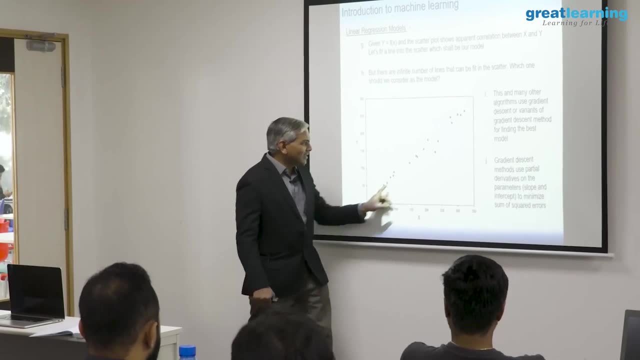 And you see, notice, the distribution is like this. So this is a good predictor of this Y. But let me understand in precise terms what is the relationship between Y and X? I see that there is a relationship, but what exactly is that relationship precisely? 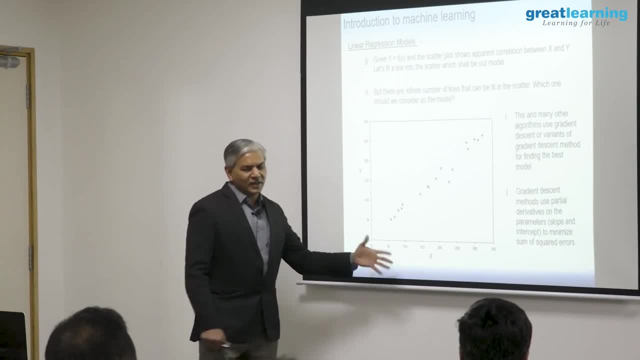 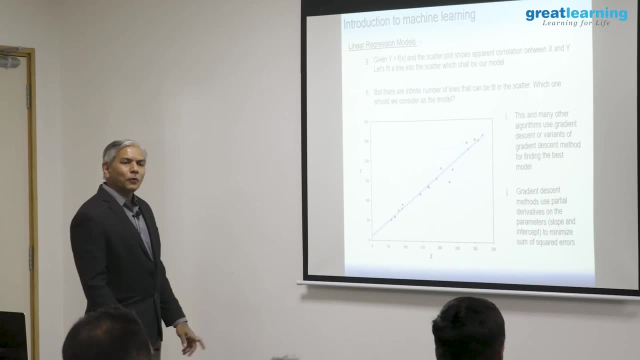 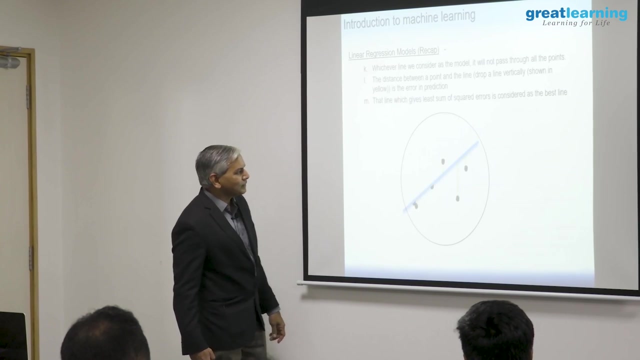 I want that. That precise relationship between Y and X will be your model, Represented by a line in this case. okay, The algorithm. what this algorithm will do is it can find out multiple lines here. Multiple lines can be shown here, right? 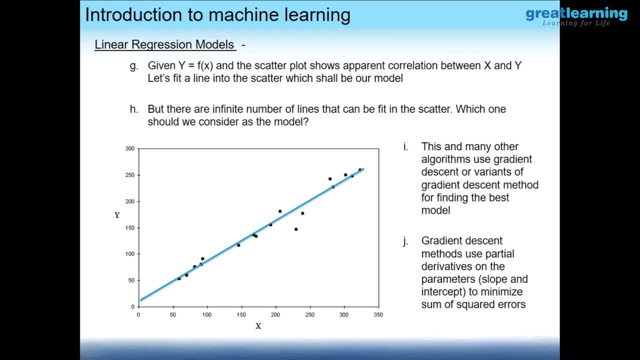 What the algorithm will do is. it will start with some random M and random C. Y equal to MX plus C, Y equal to MX plus C is the expression. Hey guys, I am talking to you, not to them. Y is equal to MX plus C. 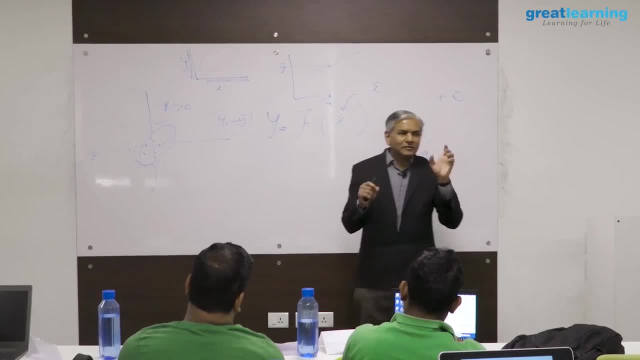 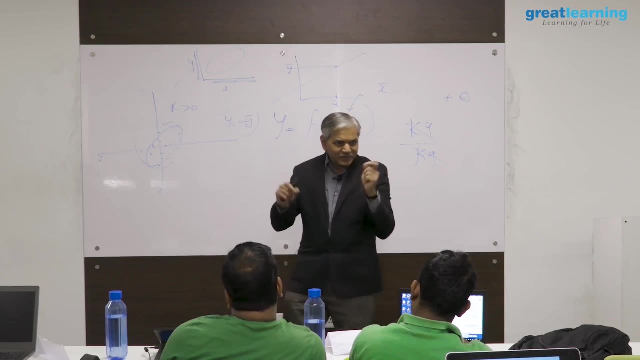 So by changing M and C, whenever I change M and C, the relationship between X and Y changes, which means the line changes. The line represents a relationship, So whenever I change M and C, the line will change okay. 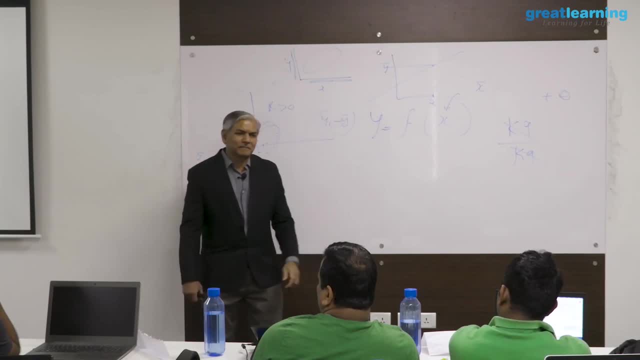 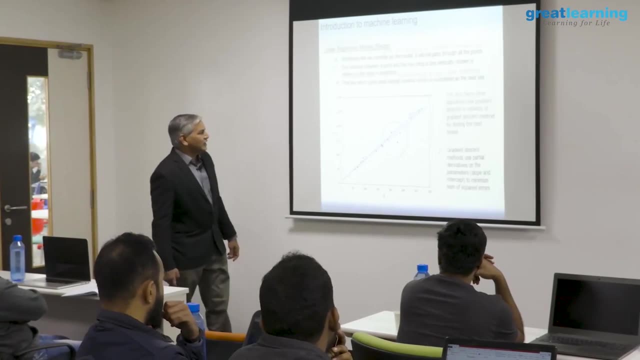 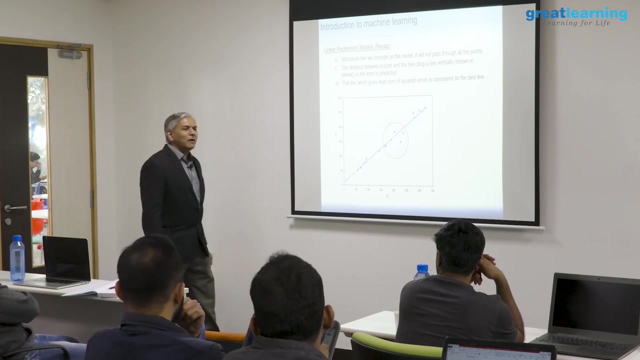 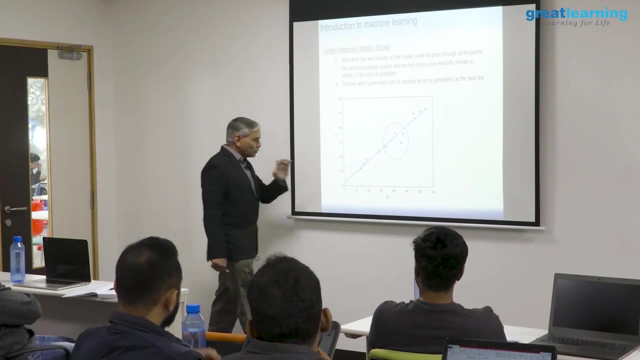 This algorithm will start from some random M and random C And it will evaluate the different possible lines before it finds what is called the best-fit line. okay, Now what is this best-fit line? Amongst all the lines possible that it has checked, best-fit line is that which goes. 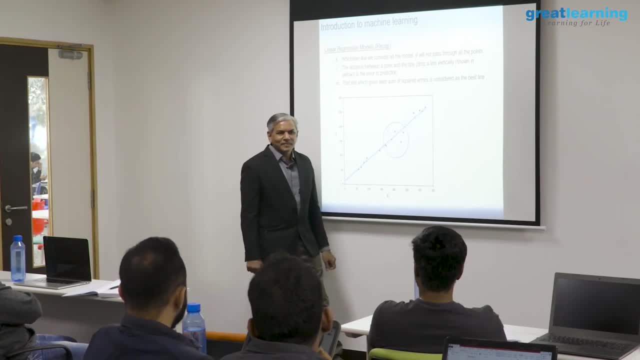 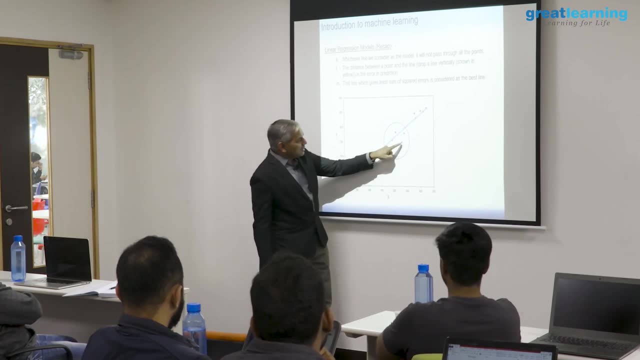 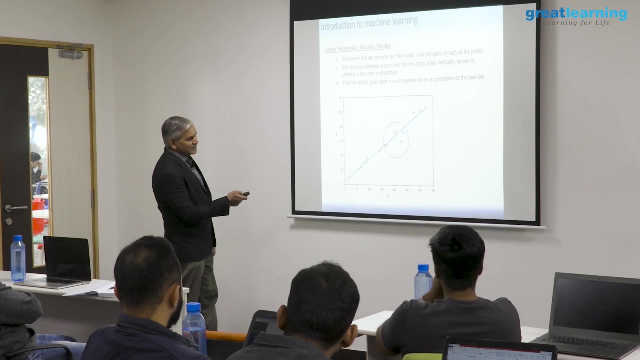 through the maximum number of data points. It can't go through all of them. It goes through maximum number of data points and, at the same time, it minimizes the distance between other points and the line. Okay, Okay, Okay. So between other points and this line, this distance, you see the distance over here. 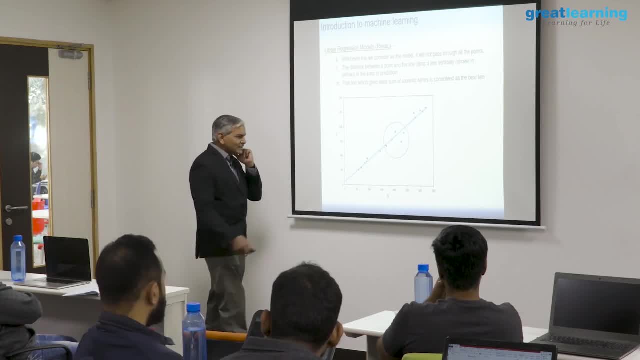 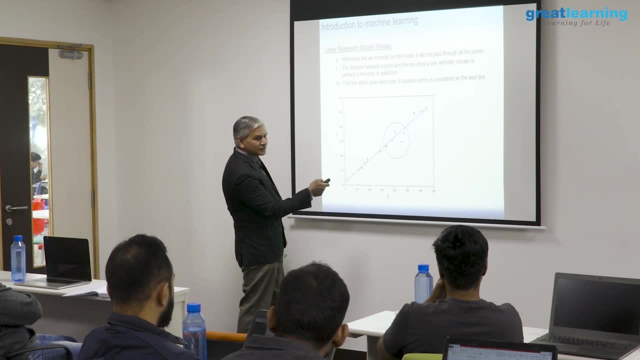 This distance is called error. What it means is, for a given value of X, your line says the value of Y should be this, but your data available in your data set is saying the value is this: The blue line here is the predicted values for the different X. 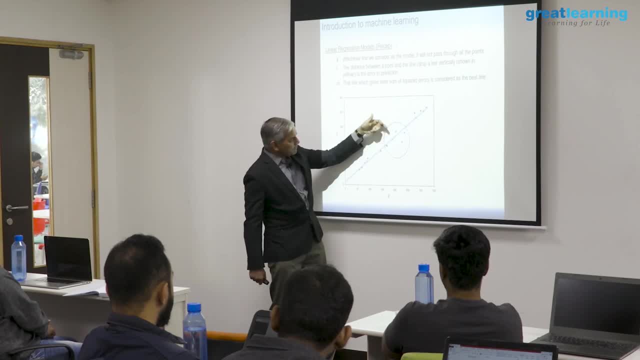 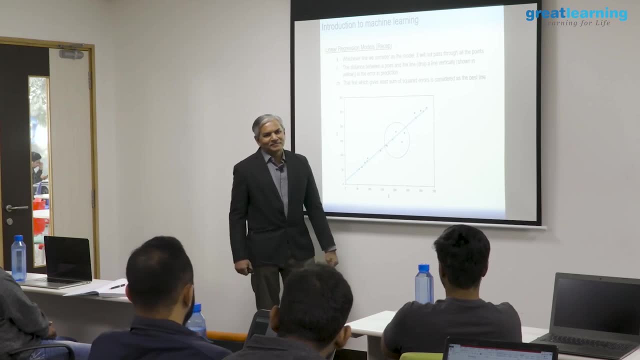 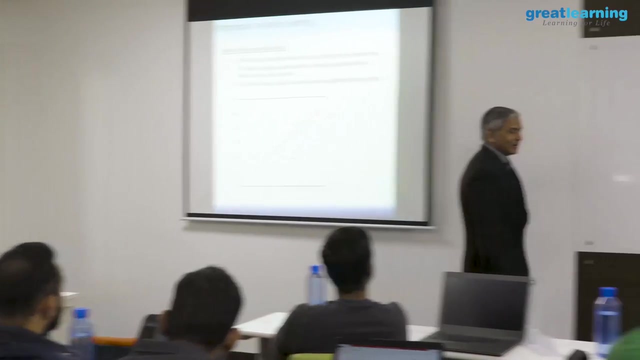 Actual values are the black dots. So whenever you have a black dot above the line or below the line, that means there is a difference in prediction and actual. The difference is called error. Okay, Don't mistake the word error. Error doesn't mean anything negative, but it is used for something that you already. 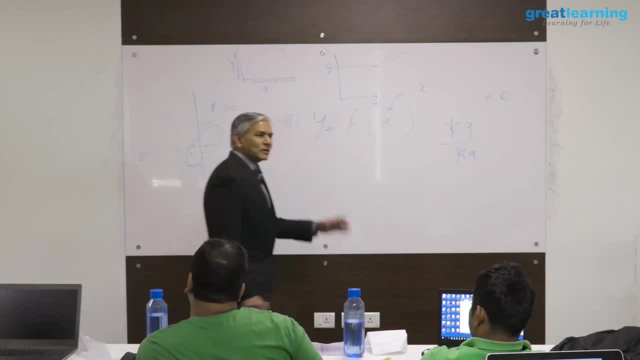 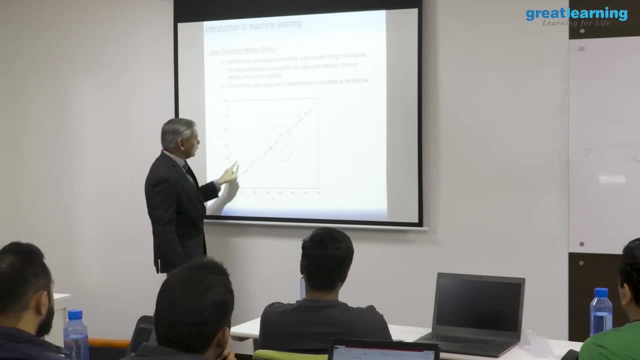 know. I will tell you what it is. So, amongst all the different possible lines, there will be only one line which minimizes the sum of all these errors. Okay, So if you sum up all these errors across all the data points, the minimum sum error. 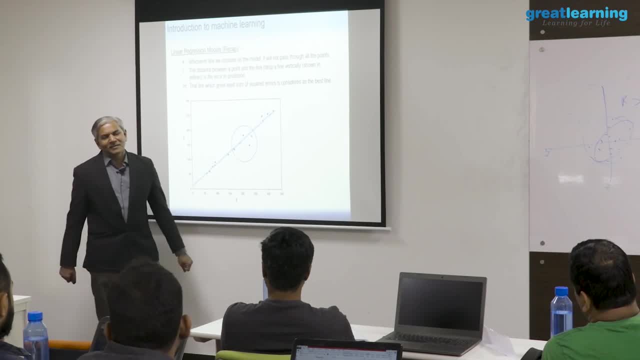 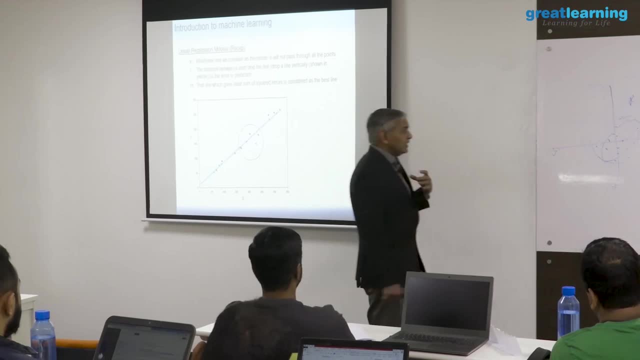 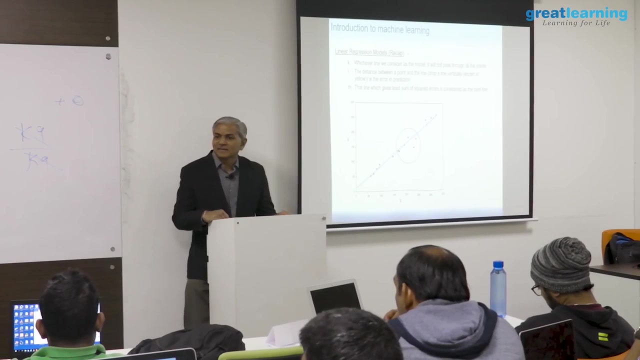 will be given to you by only one line. That line is called the best fit line. The algorithm will find out for you, from infinite number of possibilities, the best fit line for you. It is like looking for a needle in a haystack, And to do this it makes use of a process which is called the gradient descent. 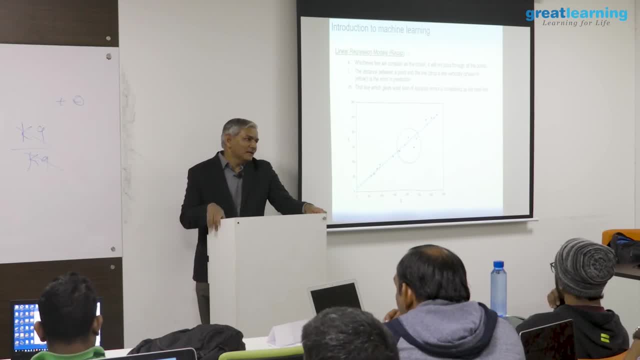 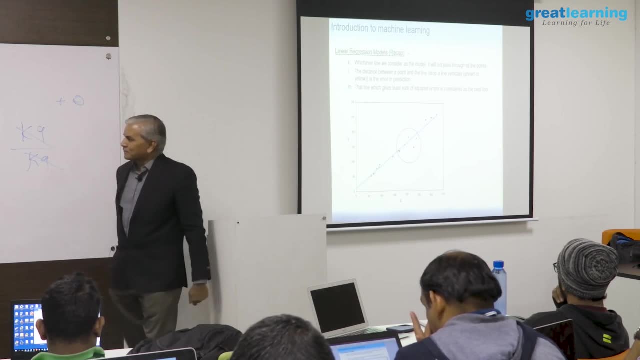 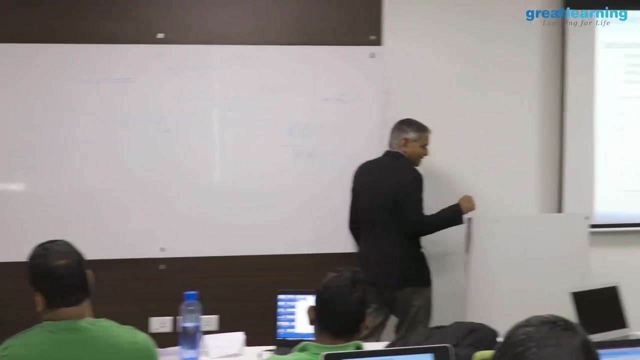 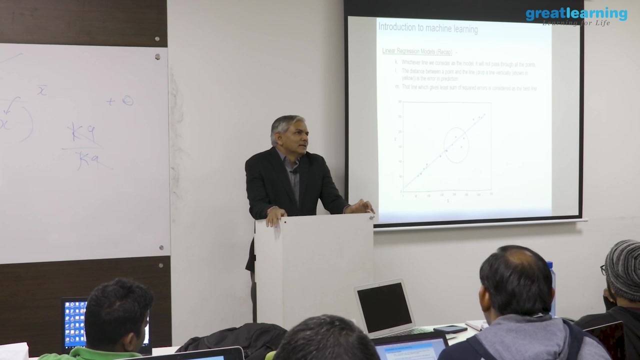 All algorithms use under the hood a learning process, a process which they make use of to find the best model for you in the given data set. That process, in this case, is called gradient descent. So the error that we are talking about, basically, that will be very significant to what our 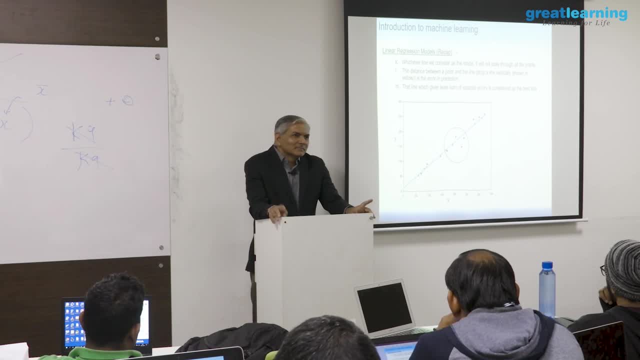 algorithm is Okay, Thank you. What is alpha 1?? What is alpha 1?? What is alpha 1?? You are talking about type 1, type 2 error That comes in classification. This is regression. However, the same concept will come into play here, also in a different way. 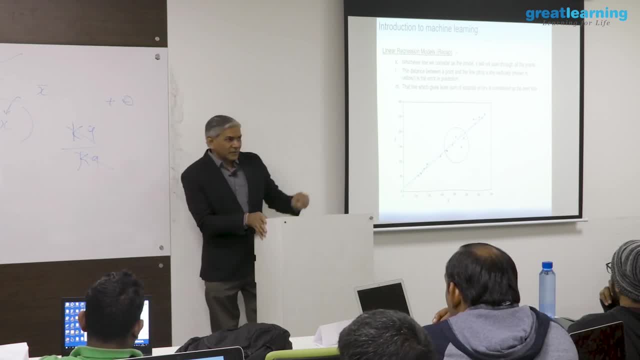 I will tell you what that way is. Yeah, So we will see that way. So again, once again, you had a particular question. We are too far away from those points, right? Shall I move on? Any questions? Yeah? 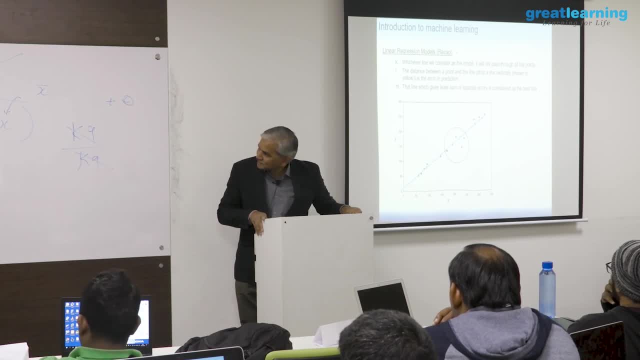 So the number of points is the priority to the distance is more than the number of points, right? Yes, There are two things. you told The maximum number of points it should go through and also the distance. But the distance is the most priority because the error should be less. 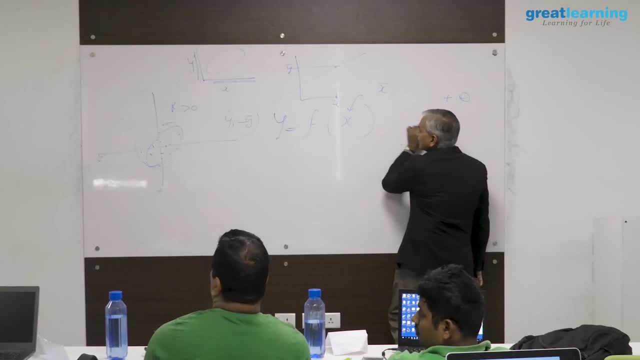 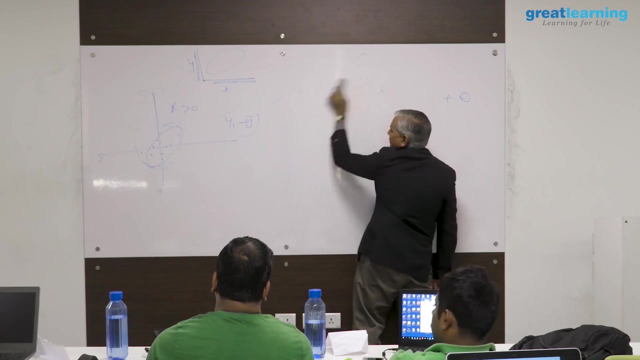 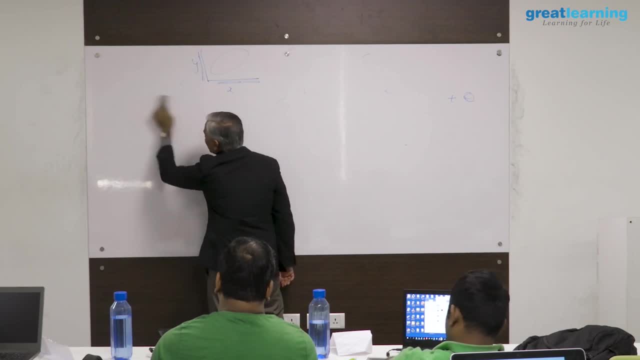 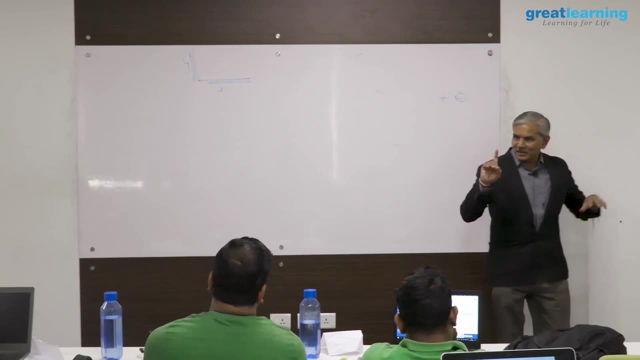 Yes, Yes, Yes, Yes, Yes, Yes, Yes. So it has to be taken together, Both of them equal priority. but there is only one line which is satisfied. that condition- driving condition- is the error should be minimized. That is only condition. ok. 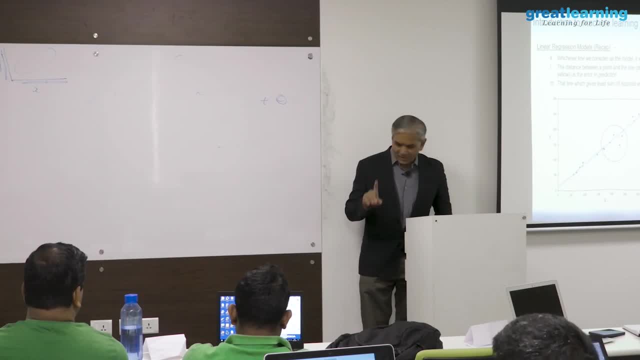 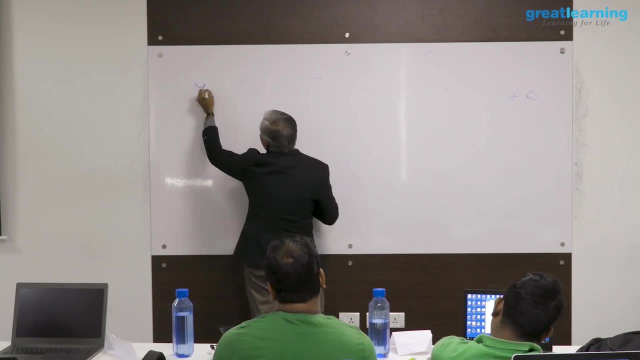 So there are no two step processes here, just only one step. So let me explain this to you. If I plot equation of line is: y is equal to mx plus c. I am going to take one simple case: mx plus c. 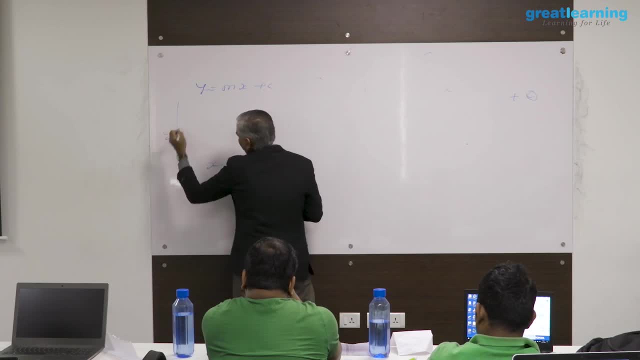 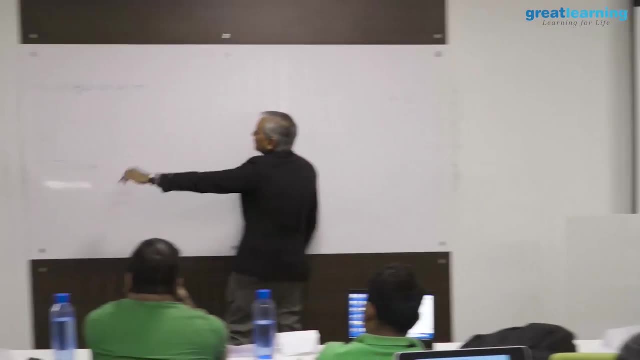 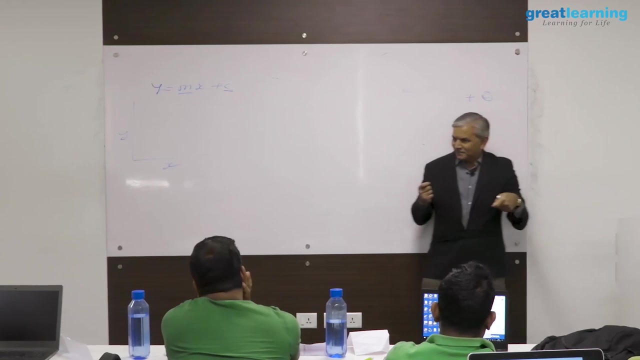 yeah, original mathematical space. you have x, you have y- one independent variable, one dependent variable. ok, So now we have two parameters that we can modify, and whenever I modify m and c, I will get different lines: this is m1 and c1,, this is m2 and c2,, this is m3 and. 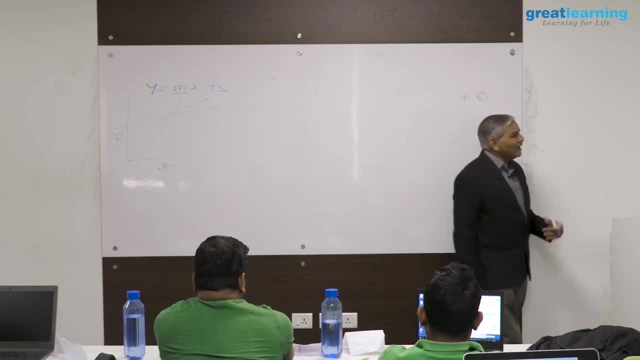 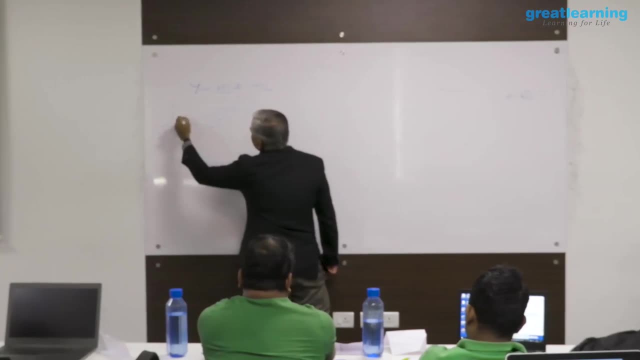 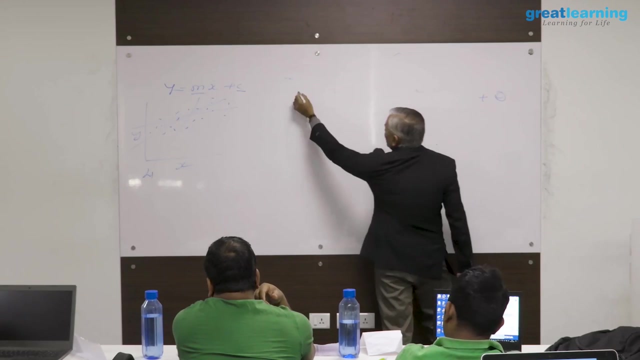 c3,. I will get different lines. Each line has its own m and c. right, but not all lines are good lines. So if I have this line, for example, this is l1,. if I take the l1,, l1. 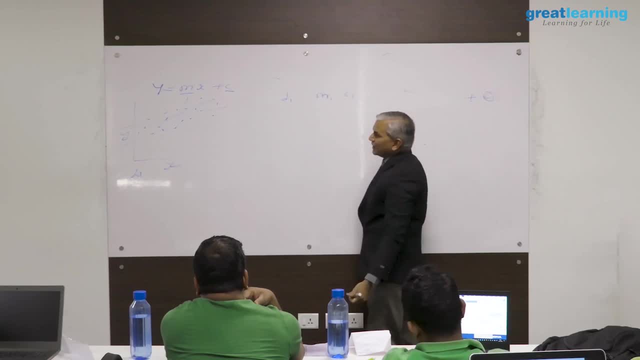 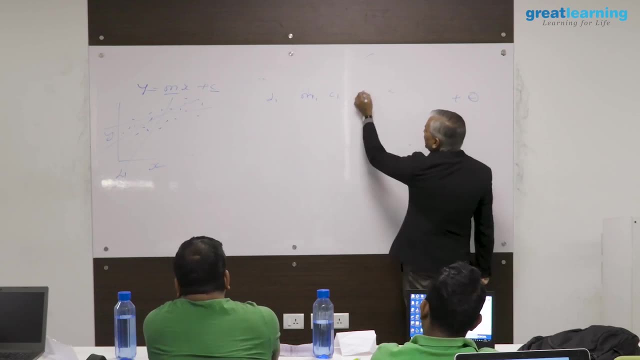 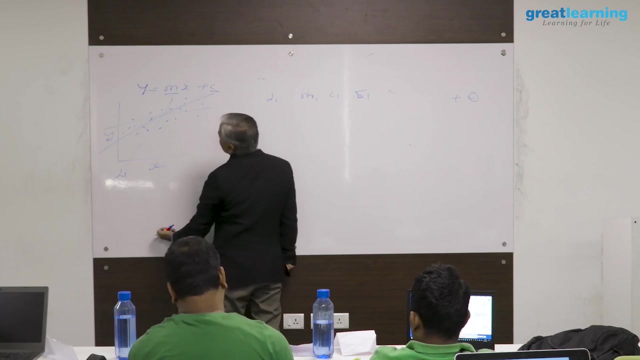 is made of m1, c1, I see that many of the data points are away from l1 on both the sides, so the error e1 is very high. Ok, If I take, say, the next one, l2,, I will call this l2, I call this l2, I see that l2 has 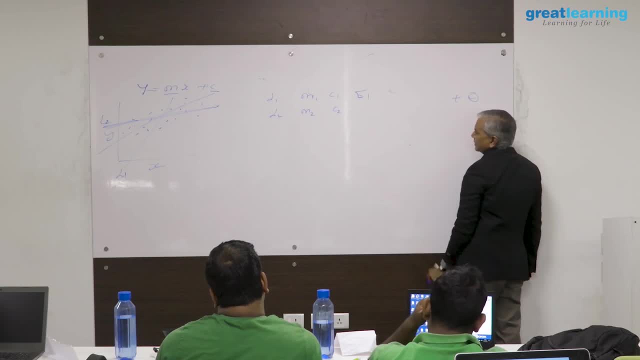 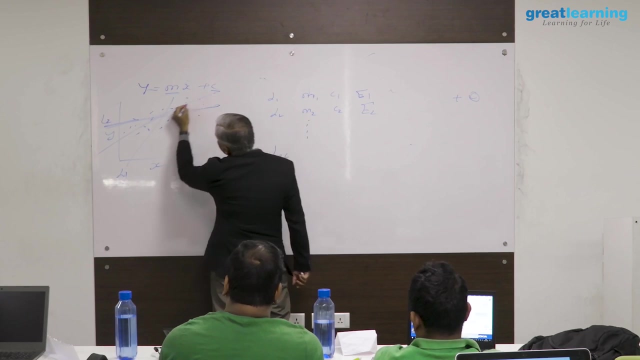 its own slope, its own co, the same intercept and it also does lot of errors, but not as much as e1, e2.. I try out various lines. then I come to lbf- best fit. best fit line is this: 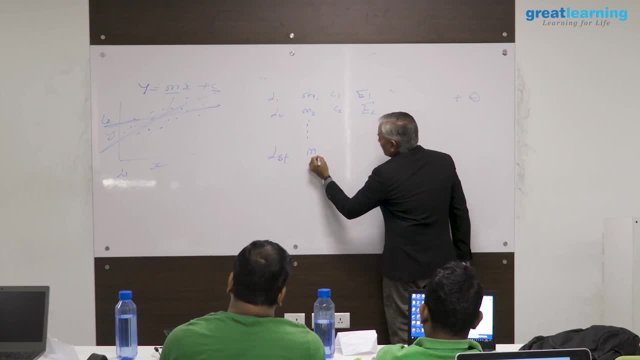 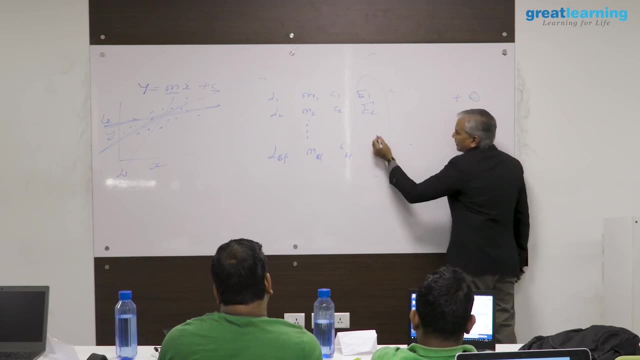 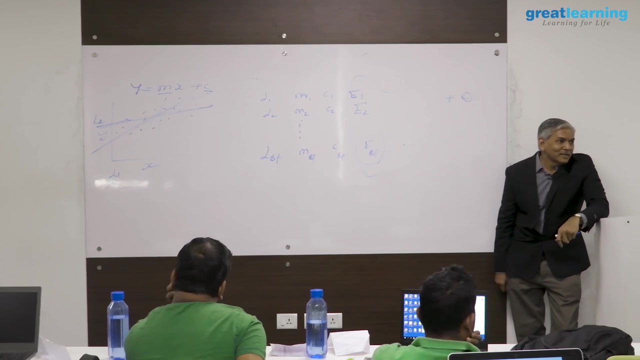 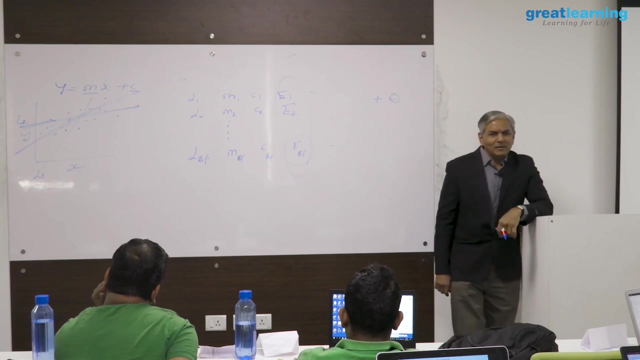 which has its own m best fit, c best fit and e best fit, and of all these errors this will be the least. e best fit will be the least. Now the question is: by changing my m and c, but just a small minute amount, I will get a different line. So there are infinite. 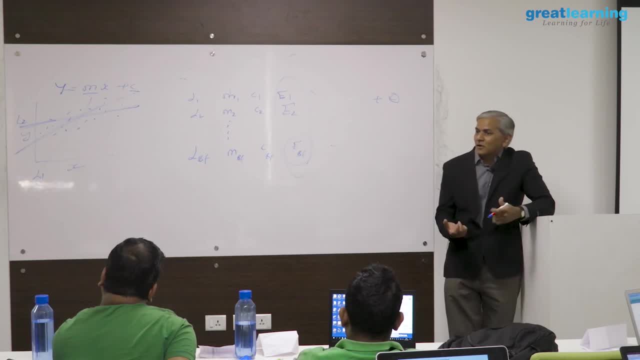 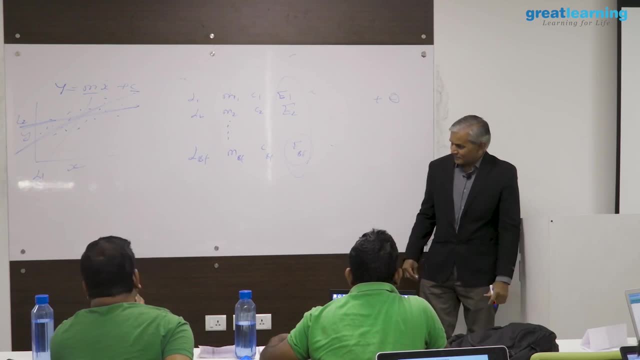 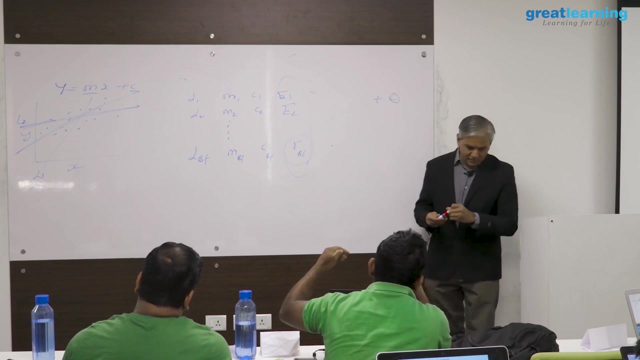 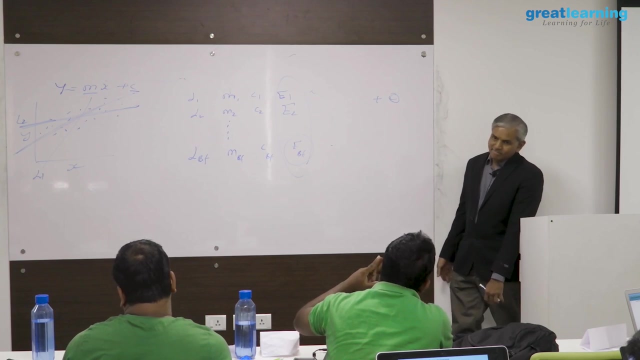 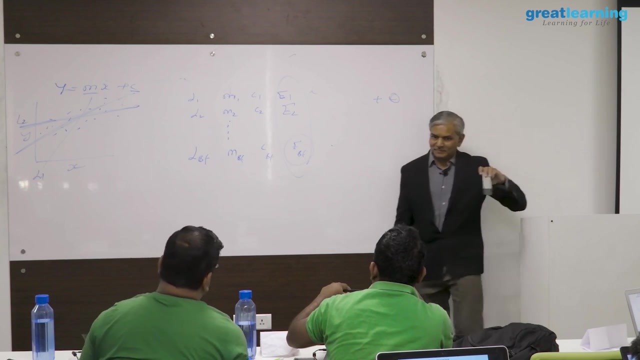 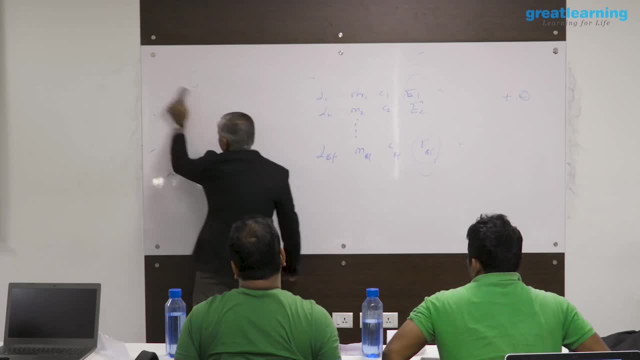 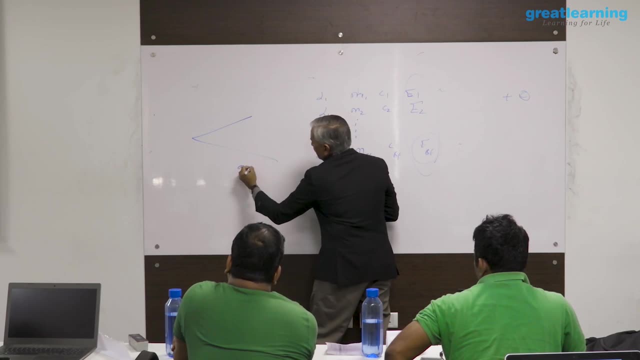 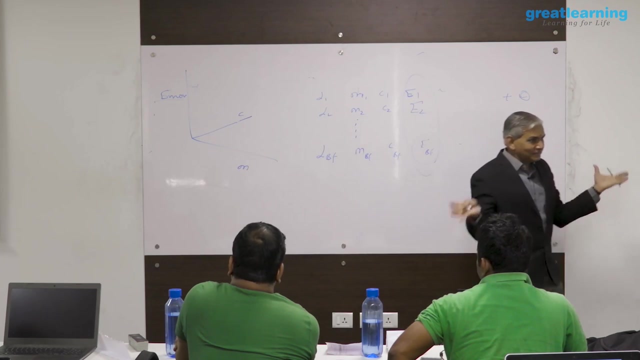 So instead of looking at this mathematical space, I can actually look at another mathematical space which is related to this. that mathematical space is between m and c, and this dimension is error, where error means sum of all the errors put together. okay. 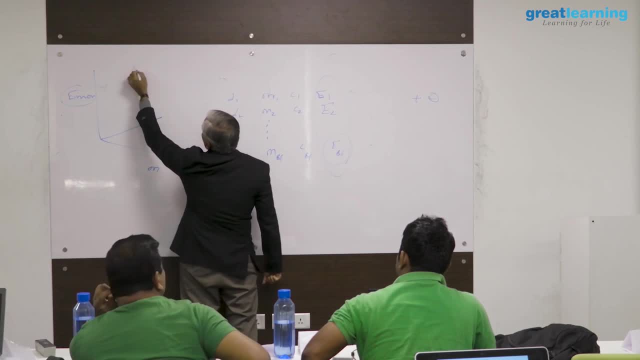 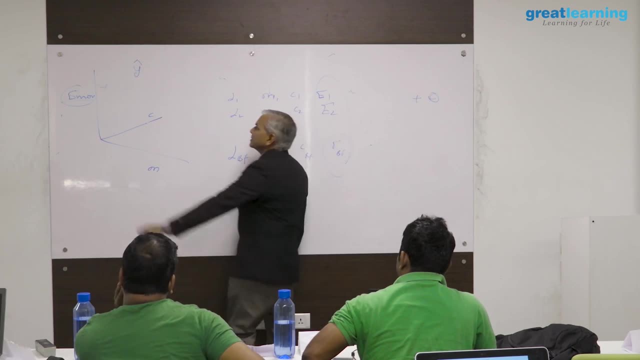 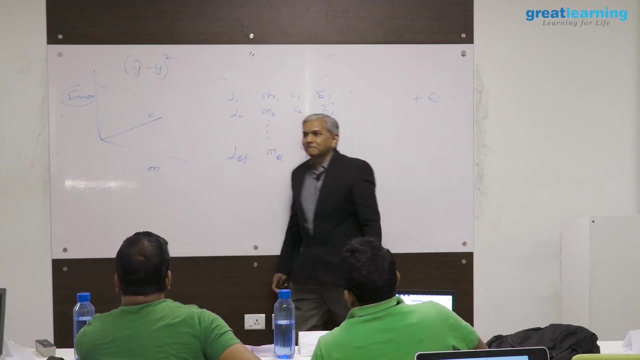 In the linear regression this error is calculated as y hat, that is, predicted value of y Minus y actuals. okay, raised to power, 2, divided by n. n is the number of data points. i is equal to 1 to n. 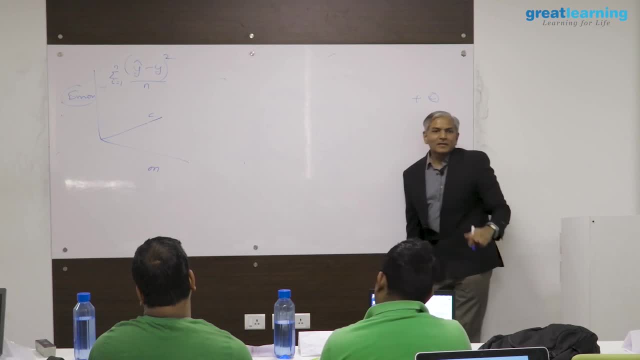 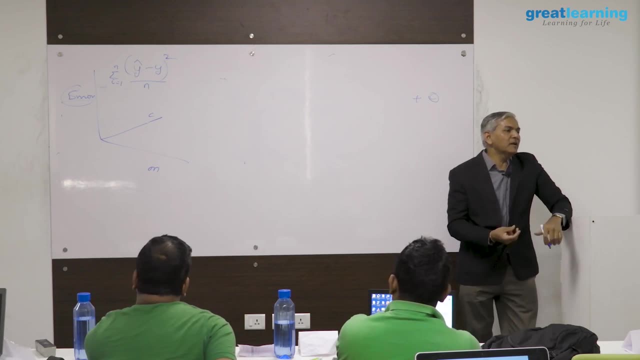 We call it squared error, sum of squared errors. Sum is sigma squaring the errors. So the error done by m, The model, is nothing but a sum of squared errors. N is the number of data points you have. Isn't this formula for variance? 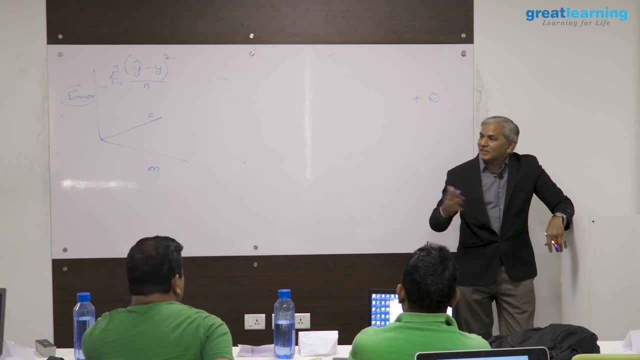 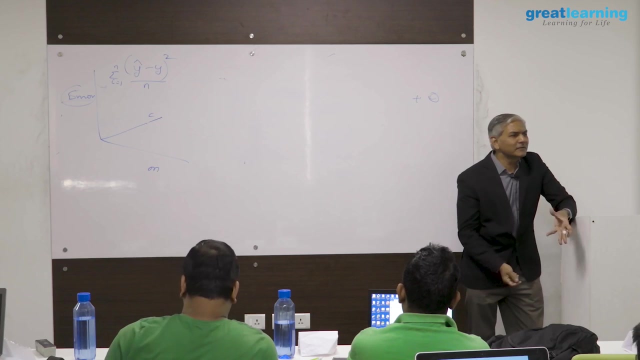 So error is nothing but variance. How data points vary. scatter across the best fit line, The lesser the variance, more reliable the central value is. The lesser the variance of the points across the model, the better the model is. Same concept comes to you in a different way. 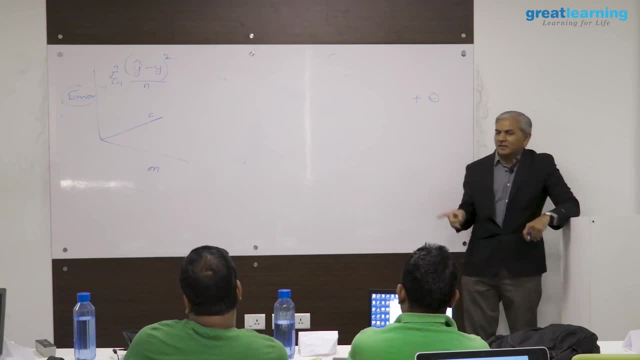 Okay, So sum of squared errors is nothing but variance, variance of the data points across the model. So I want to find that model where the variance of the data points across the model is the least. This is slightly confusing, See, when you say covariance and you said, like you have more value of covariance, then 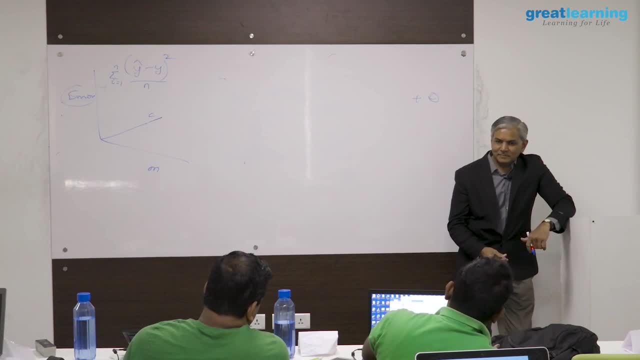 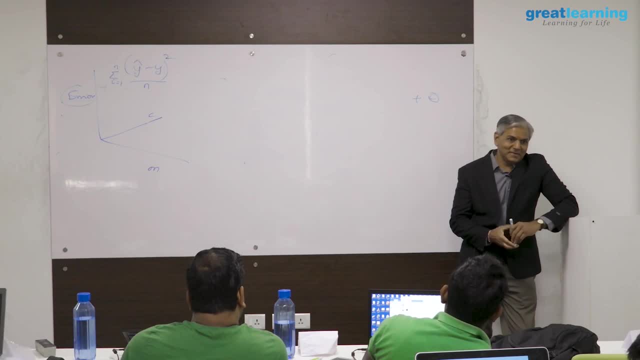 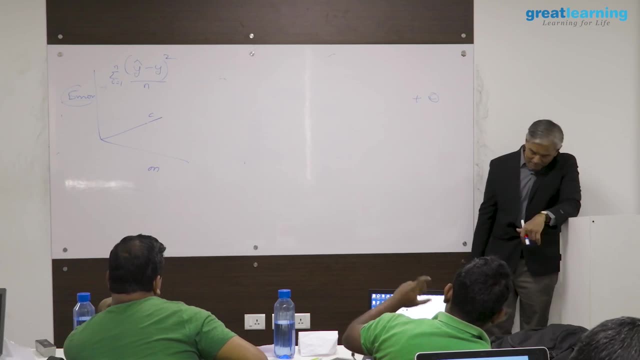 What is that? What is that? Okay, Okay, The stronger the r is, the better the predictability. So degree of covariance can be should be higher, whereas variance should be lower. Variance in integer dimension should be lower, Okay. 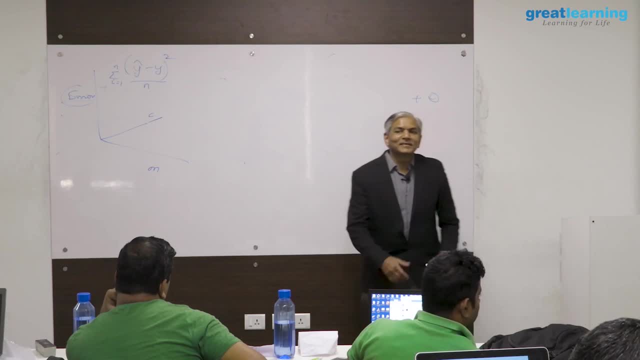 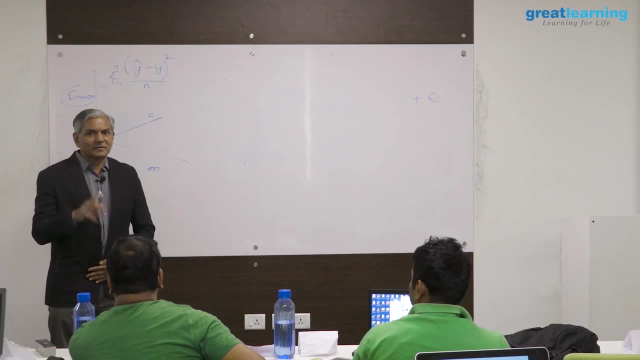 Just compare with some other box model. So always we are, We can change it once again. Once again We are omitting the outliers. so in the data which we are collecting, we are removing the outliers. This is common falsification. 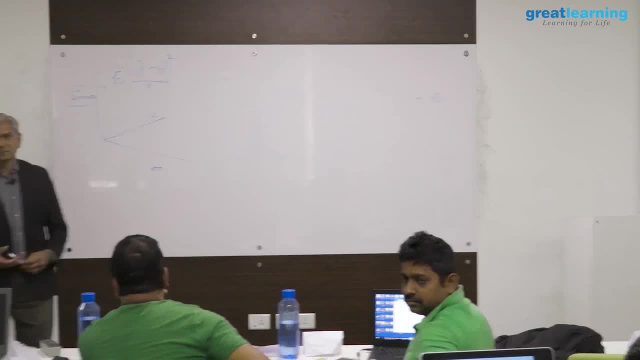 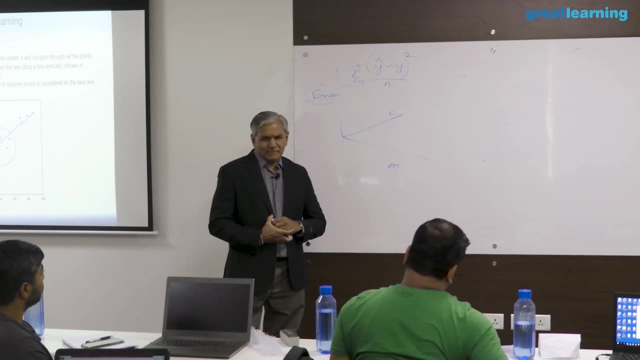 This is common falsification. This is common falsification in the like a group of data which is affecting the sum model. So always it will be in the linear model type. Yeah, I will get your question How we insert box plot. you are adding for round class. 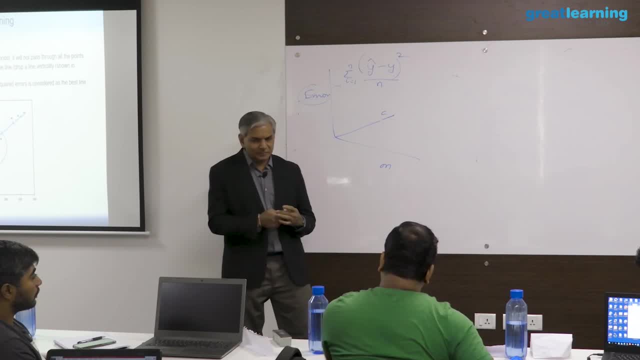 So we are removing it, So we are collecting the data which is affecting, which is going to affect the model. So if you are plotting in the any linear regression model, it will be in the linear model, Not necessary. I will take your question. I will just hold on a minute. I will take the question here. 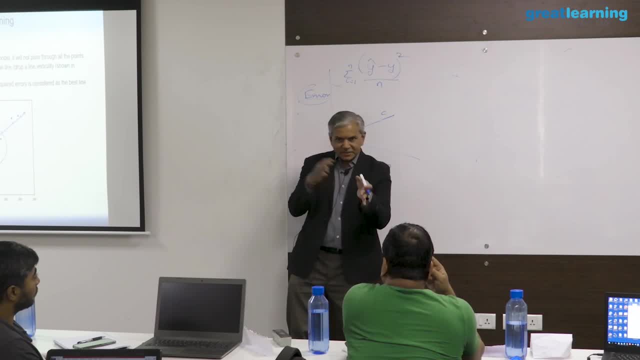 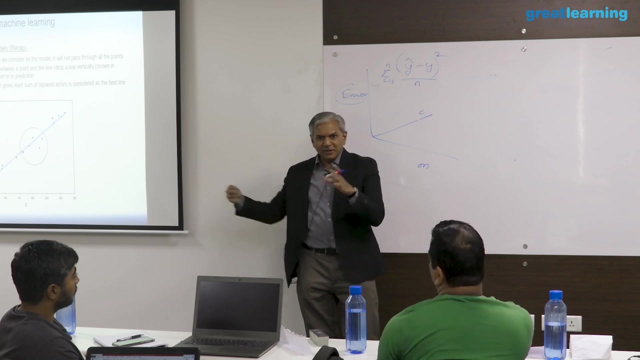 Within 1.96 standard deviation. this and in this side the data points might still have noise in them, which causes spread across the model You are talking about outliers, which is lines 1.96 standard deviation greater. So by removing that, yes, you are cleaning. 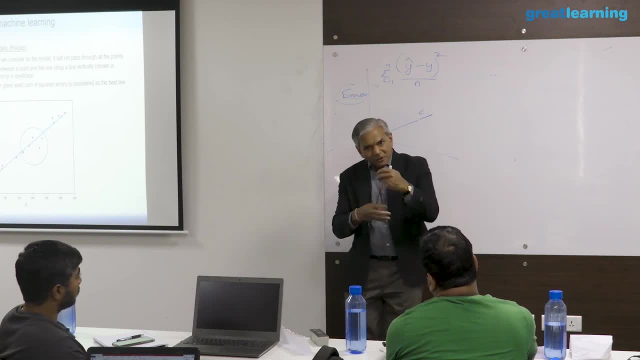 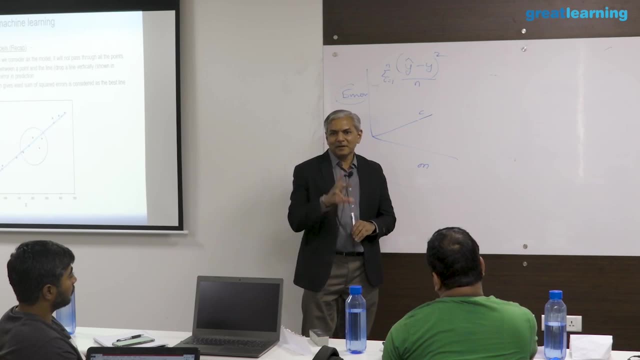 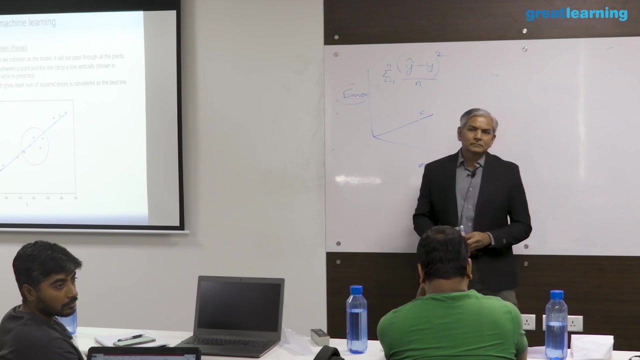 the data, but within the 1.96 standard deviation, still you have noise. That noise will appear as scatter around the models, It will appear as variance around the model, But once we are omitting the unmodded data, so it will be in the like a linear regression. 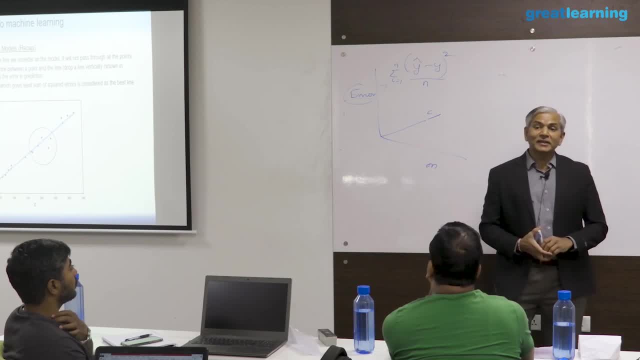 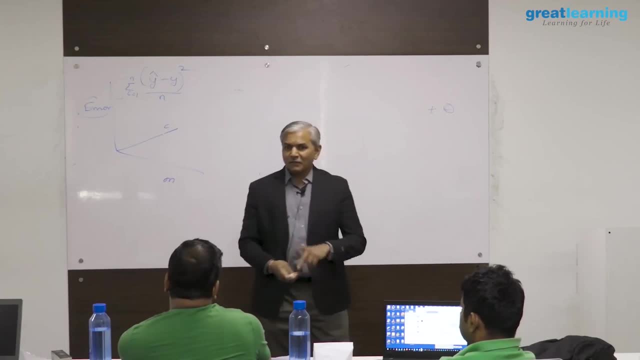 model, but with some noise Right, It will ever be one single line, kind of. Actually. no, you have asked a very, very important question. Yes, So you have asked a very, very important question, which I will just answer. this, because this is a very important question, which will be: 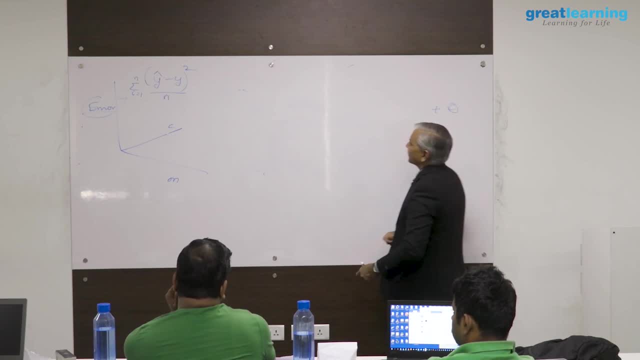 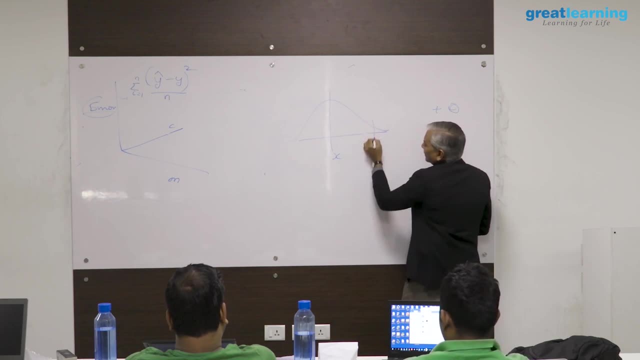 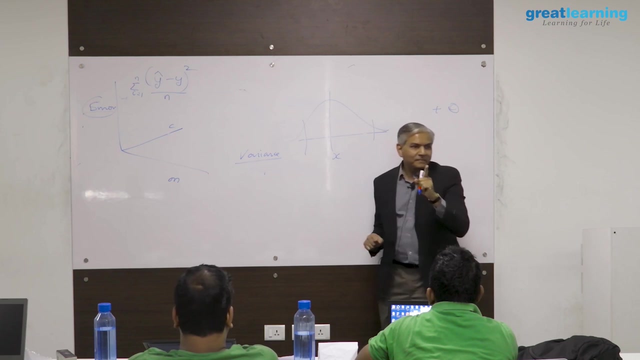 helpful down the line. Just hold on a minute. I will answer this question first. Now, if I take any axis, any variable x, it has a spread. This spread variance, what you call variance variance. there are two types of variances. One is called stochastic variance. 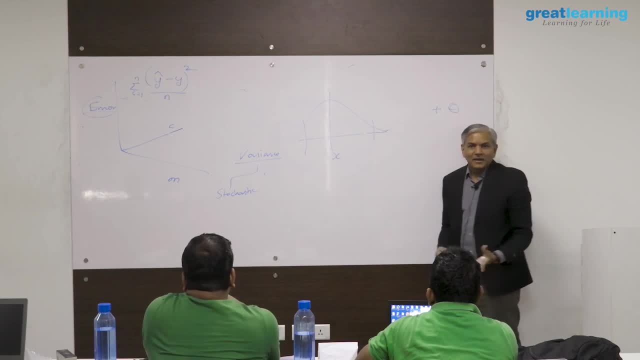 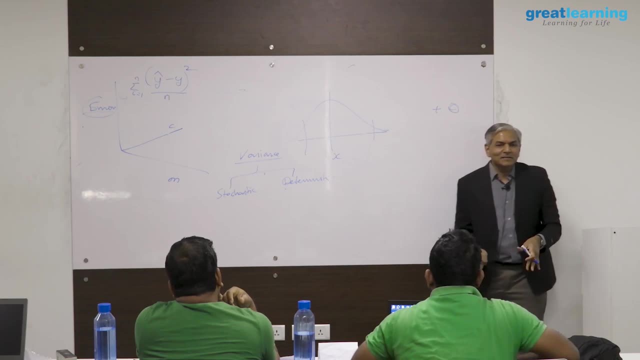 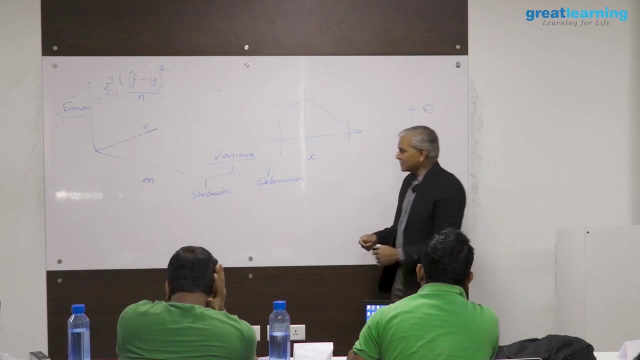 which means nothing but probabilistic variance. The other one is called deterministic variance, which means variance that happens for reasons that I know. I know why that variance happens. That is called deterministic. But variance also happens in your data set for reasons that I do not know. We call them noise That. 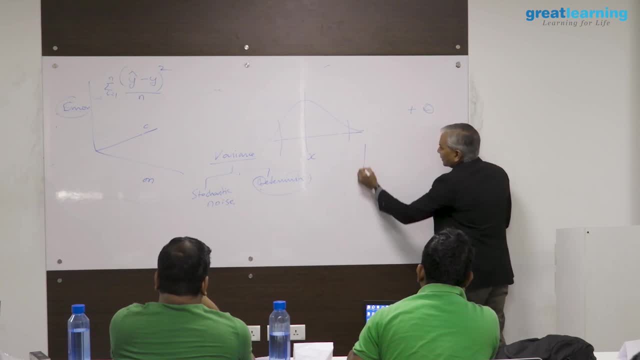 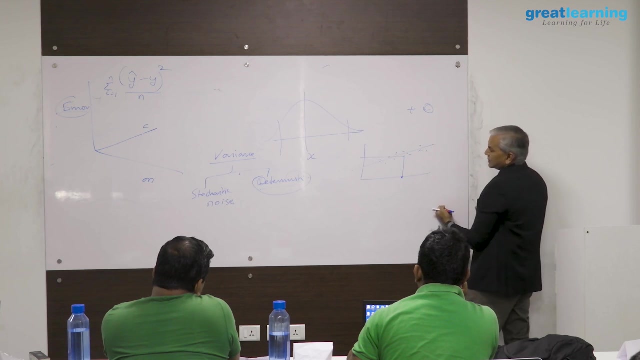 is called noise. Alright. Now if I have a plot like this, a linear model, and I have distribution of the data points around this for a given value of x, now look at this Actual value is this in your data set, but the model is saying it is this. Similarly, there is another actual. 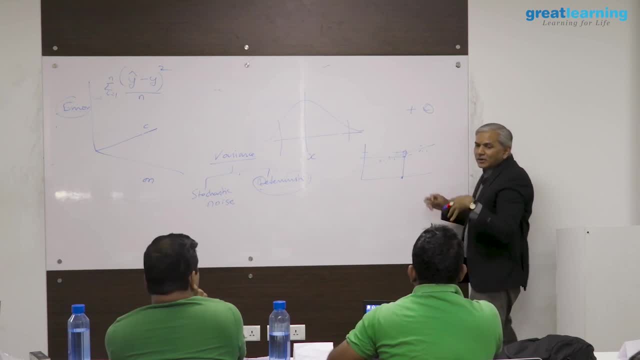 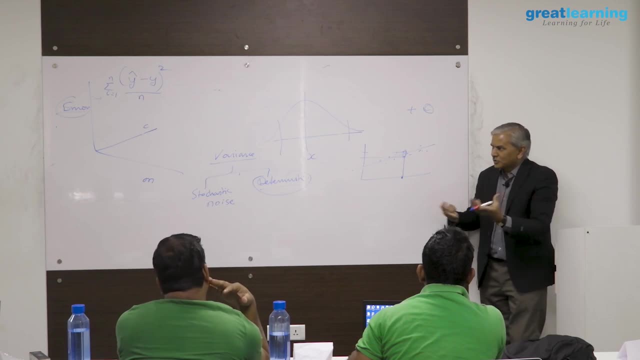 value, which is this. Why is this variance occurring? I do not know. I do not know why that variance is occurring. This is called- And I do not want to use the words right now, I will use it down the line- This variance. 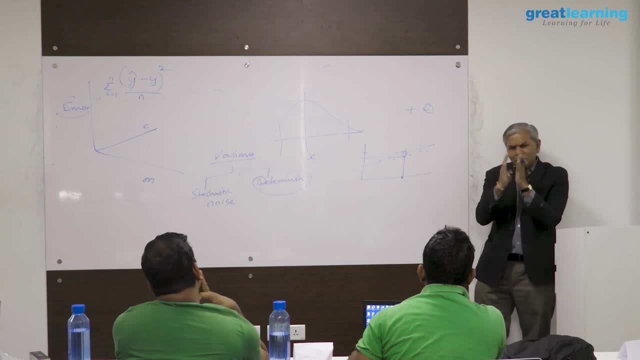 that you see, for a given value of x you have multiple values of y, but they are very close but still there is a variance in them. That variance is called stochastic noise For a given value of x, the fact that the value of y is spread around its central bar. 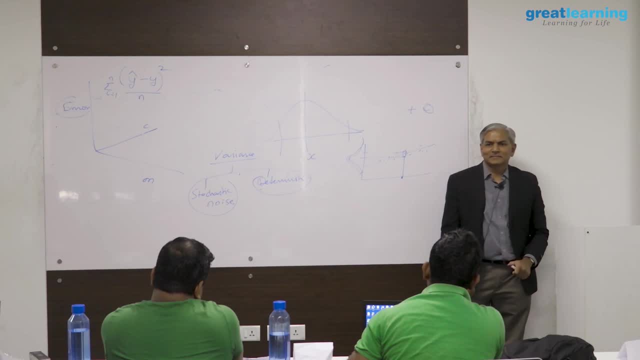 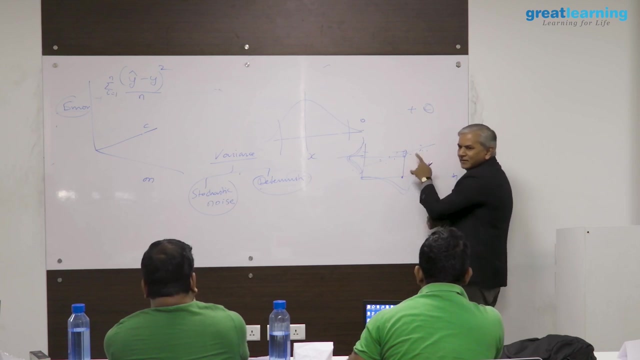 this is deterministic. We know that this is going to be this way. Alright, So when you address the outliers- outliers is something which is lying two standard deviations away, or 1.96 standard deviation away- You are addressing the outlier, But you are not addressing the. 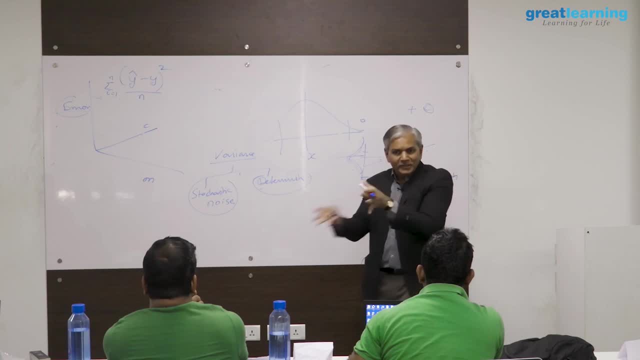 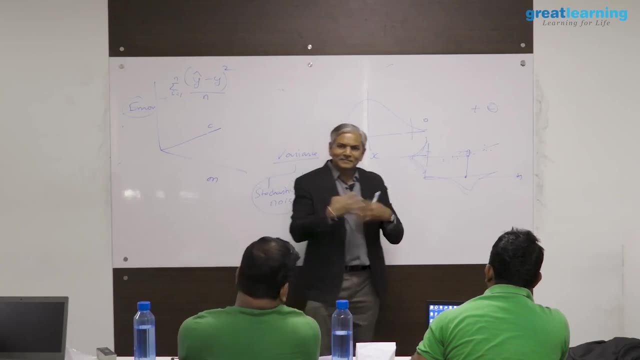 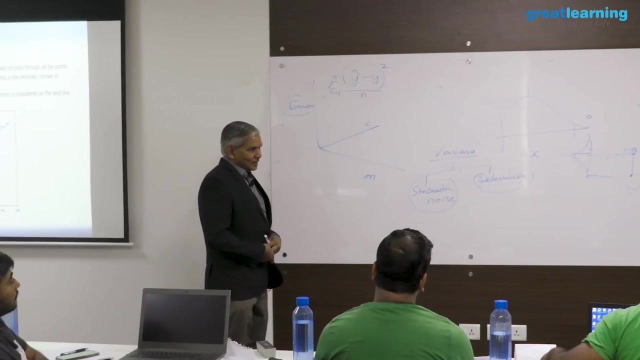 random variance which exists in the data points within the 1.96 standard deviations. Those will cause a scatter of the data points across the model. You were talking about the real, actual data point or the prediction point. Prediction is your line right. 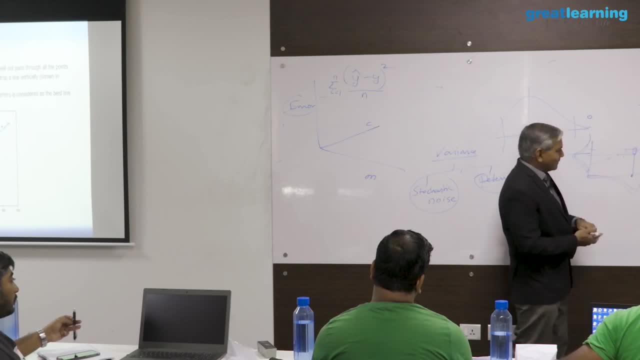 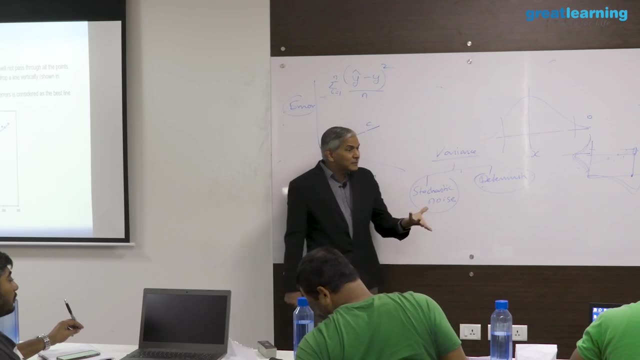 Prediction is your line Okay, So there are some patterns right. The prediction point Actual is the black data points. Between the actuals and line there is a gap. that gap is my stochastic, unexplained variance. I do not know why it happens. 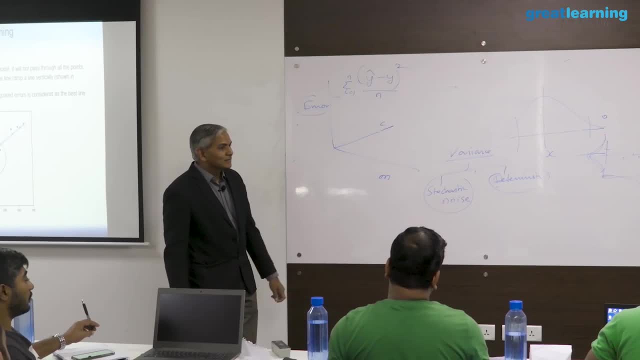 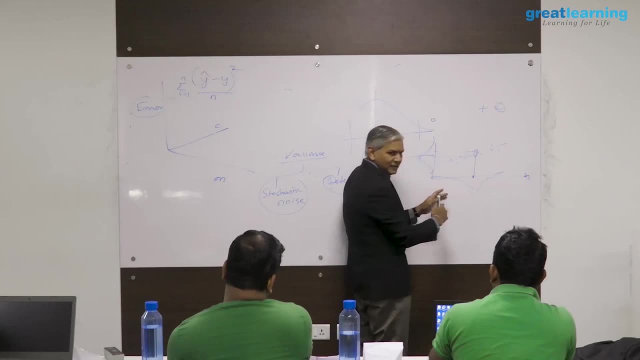 That is in the actual data, Yeah, in the actual data. Deterministic is: I already know my y bar has this spread and my x has this spread. This spread is also variance. I already know it has this spread. I know it will be like this only. 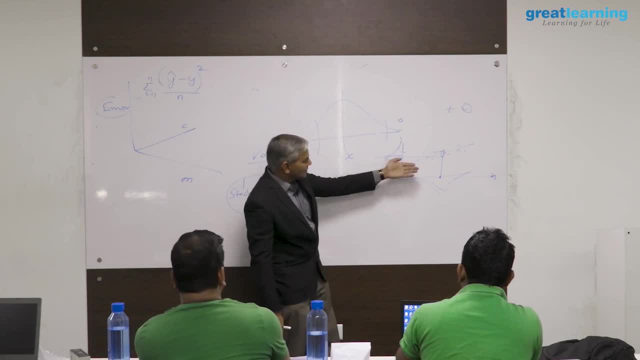 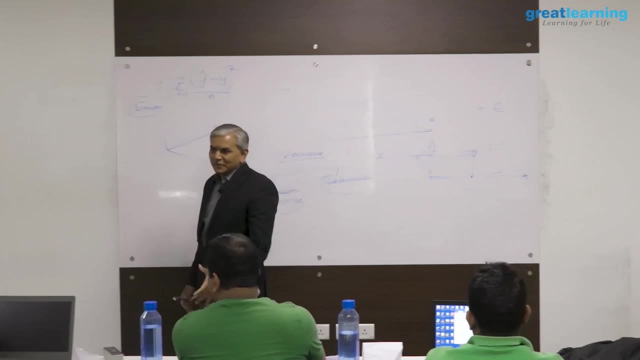 I have no reason for worrying about that. What I am worrying about is for a given value of x. why are there multiple values of y? That is stochastic. we do not know why it happens. That is what we call noise. Is it because of lack of domain expertise? 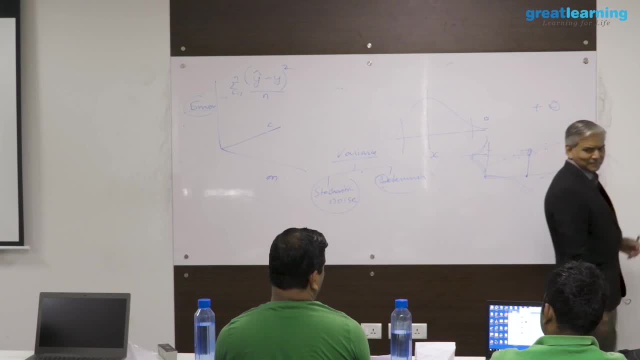 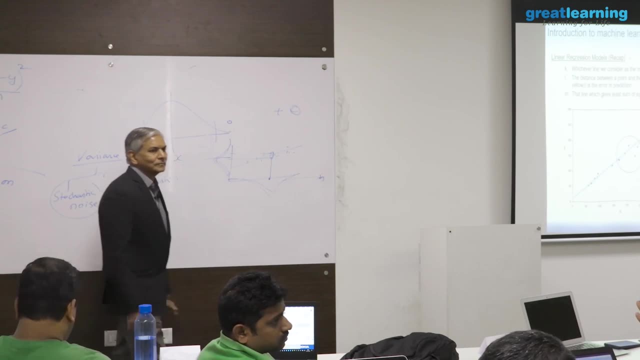 Nothing to do with domain expertise. Even the domain expertise will have this problem. So when we have a multi dependent variables, right. so here we are talking about trying to find out the only one variable. Yes, One and then y, Okay. 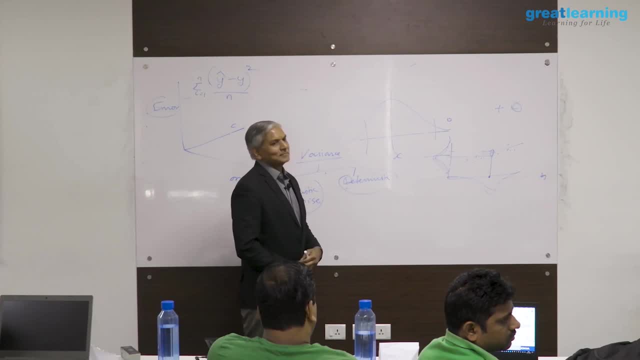 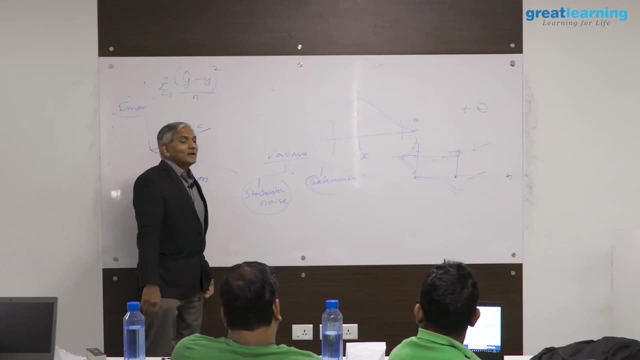 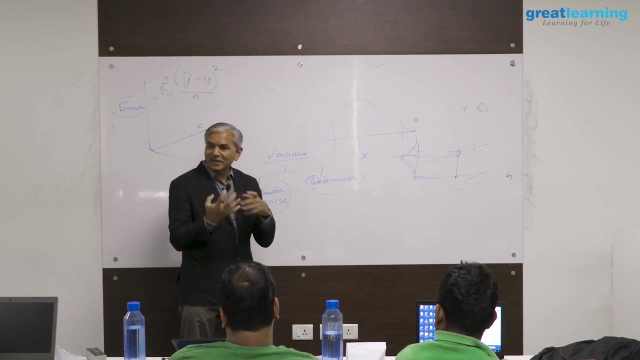 But maybe when we are we have to analyze it in the togetherness cultivation analysis, Right? Maybe that is creating this kind of noise because we are trying to target only single one variable. That can happen. That can also happen When the different variables actually interact with each other. there is collinearity in. 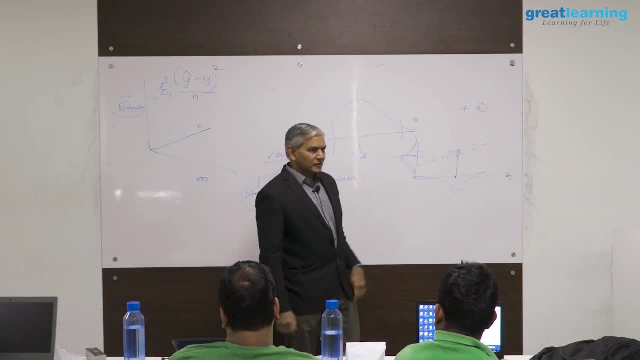 your data set, you can have trouble with this noise. That can happen. The noise may get cancelled out or the noise may get magnified. Okay, One more question. So we are looking for best fit line, which give us a least error, which is the definition. 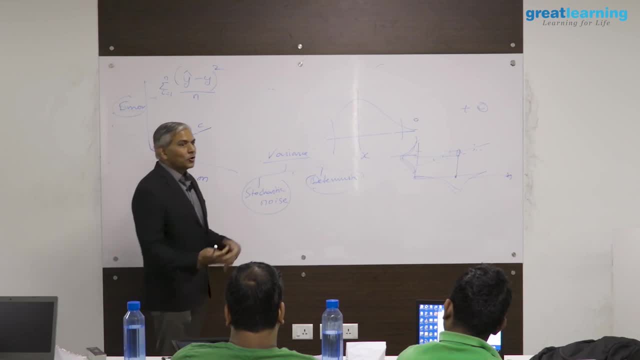 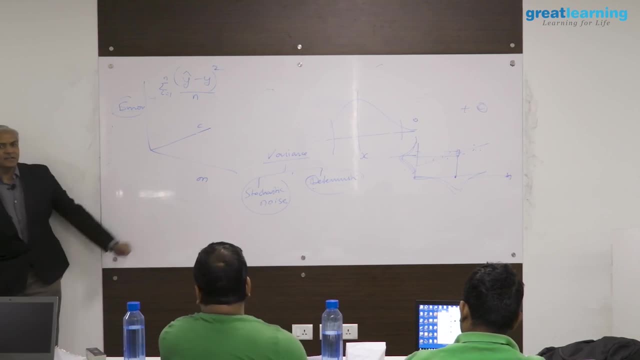 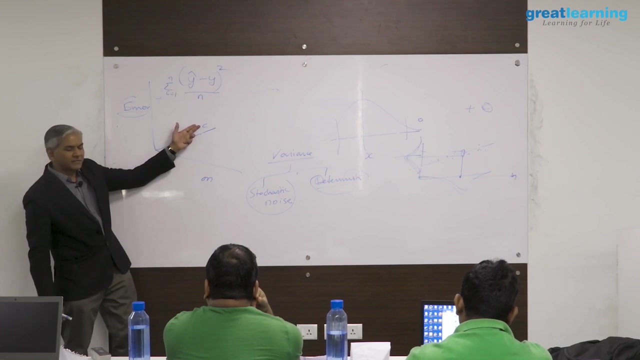 of least mean like… I will tell you. I will tell you what is least. that is what I am going towards now. Okay, So I have different combination of M and C. So I moved away from my original mathematical space into another mathematical space where the dimensions of the different slopes and 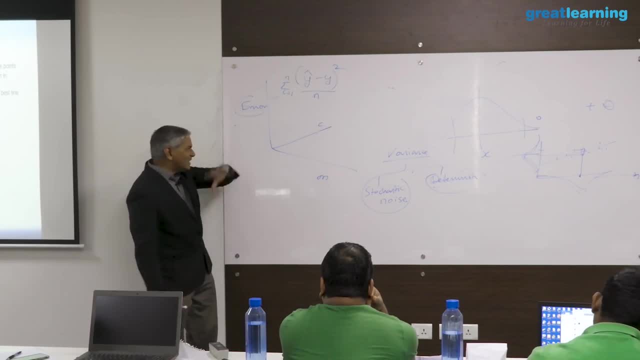 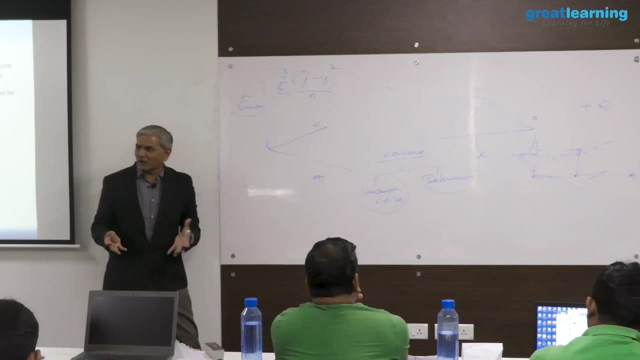 different intercepts, different lines. okay, Each line gives you some error gives you some error. The formula for this error is the sum of squared errors, which is nothing but variance across the line. Whenever you have a squared term. this is called quadratic. 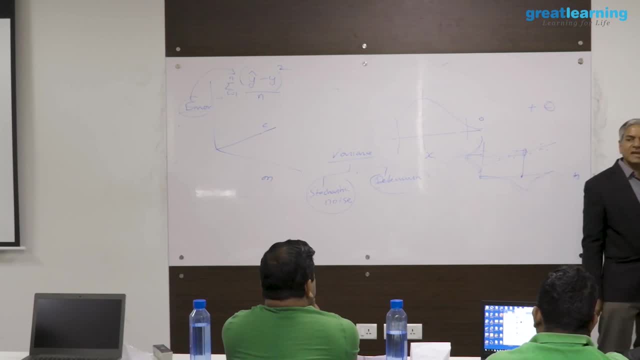 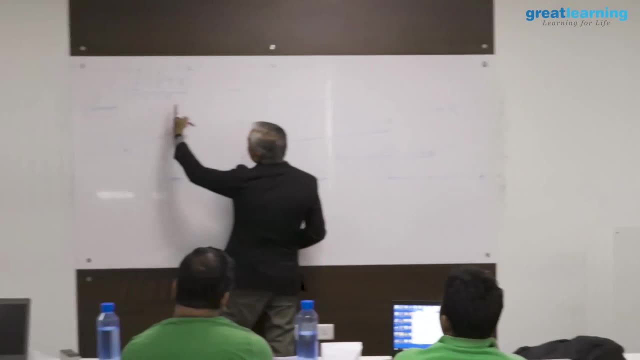 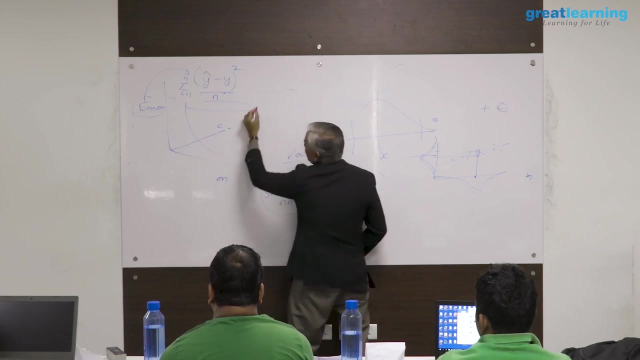 equation in mathematics, All quadratic equations. they have a property. the property is called their convex functions. Convex functions means when you plot them, when you plot them against their independent variables M and C, they will always acquire a bowl shape, three-dimensional. 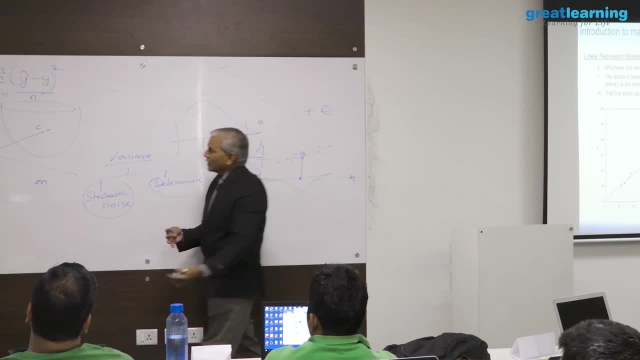 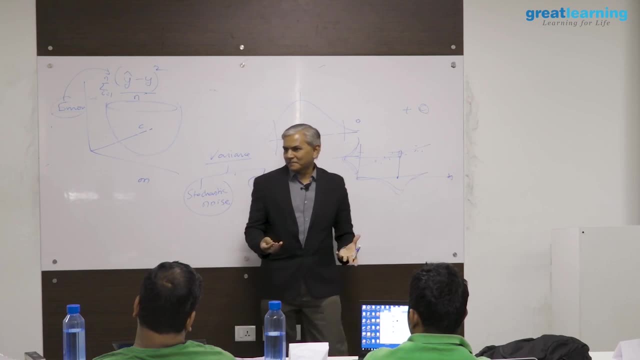 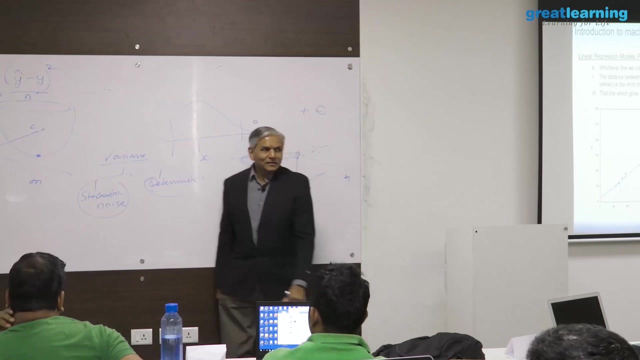 bowl. Such functions which acquire this kind of a shape, a bowl shape, in the three dimensions, such functions are called convex functions. They are guaranteed to have one absolute minima, parabolic structure, one absolute minima, So for some combination of M. 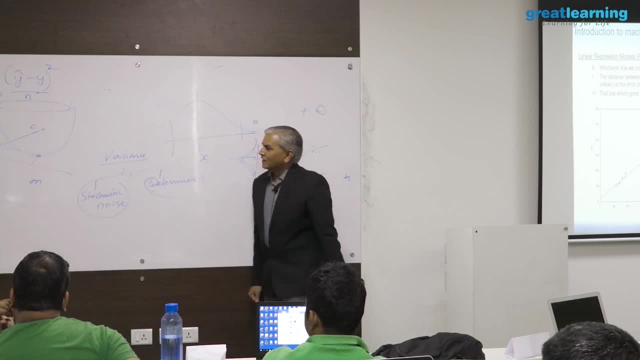 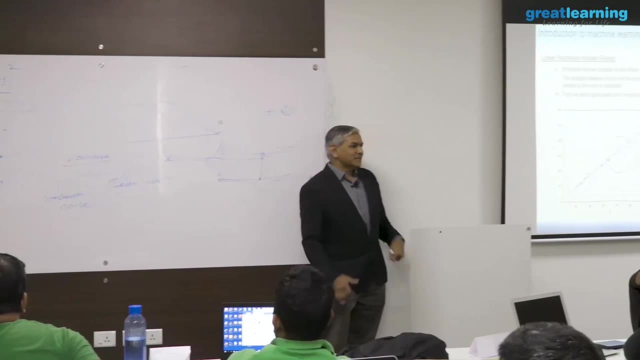 and C. they will always acquire a bowl shape. They are guaranteed to have one absolute minima c. I will get the least error. That combination of m and c which gives me the least error is my best fit line. So the algorithm will start from some random m and c. So maybe this: 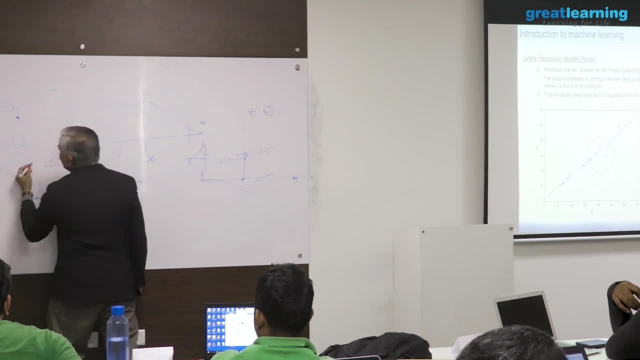 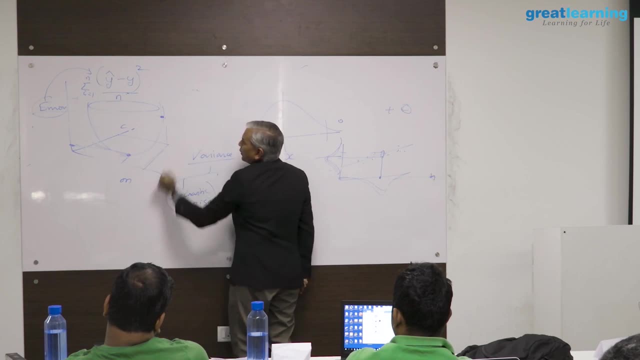 is the random m and c. This is my random m and this is my random c. When I use this I get a line, but the sum of squared errors across the line is very high. So each point here is one line in the original mathematical space. So in the original mathematical space. 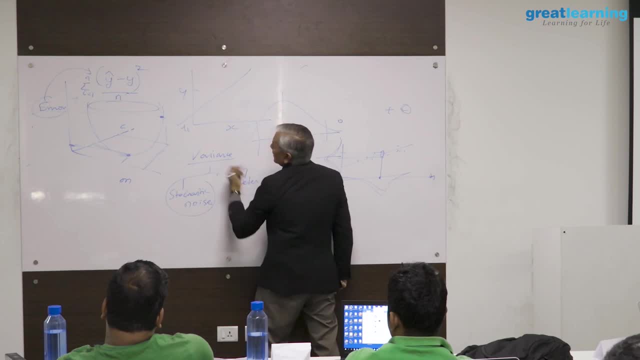 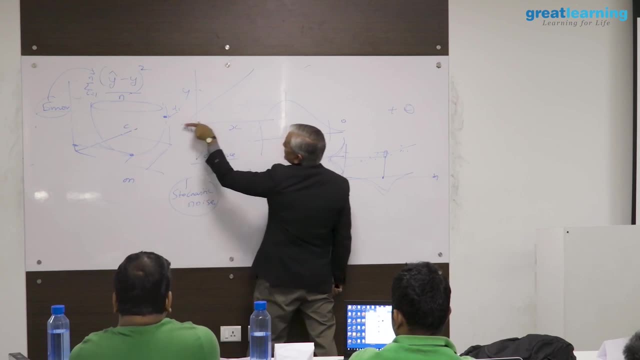 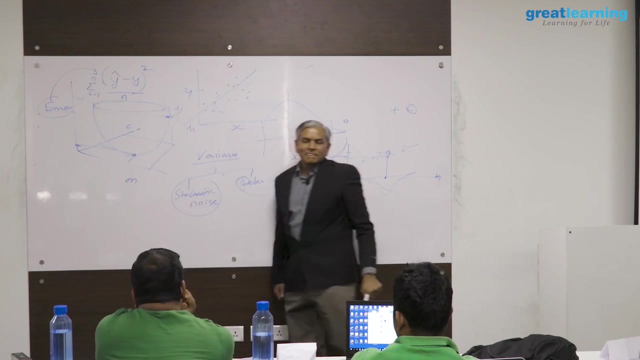 between x and y. if this was my l1, maybe this is the l1,- it had some m and some c. That m and c is this point. This point represents this line. This line had some sum of squared errors. The sum of squared errors is this: 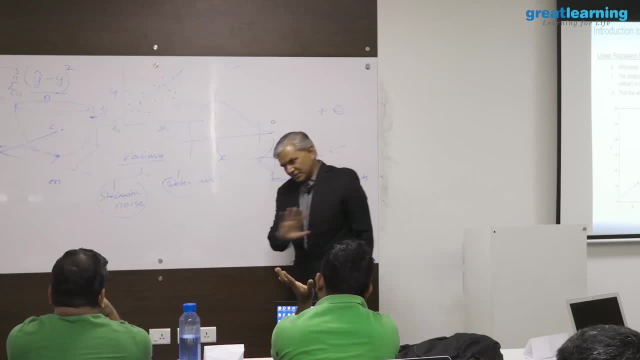 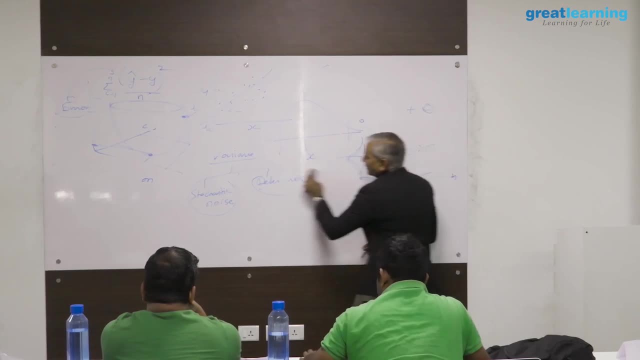 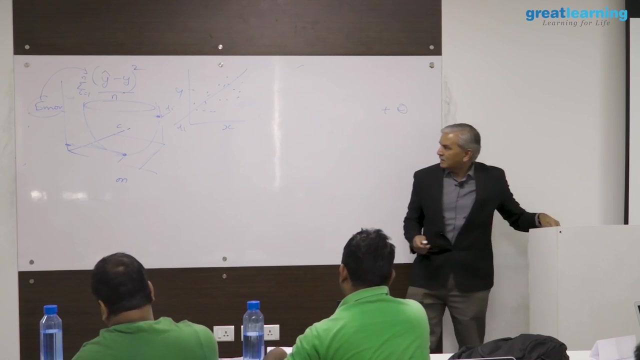 So you talked about one m, but if it is multiple, still it will be like similar, Still 100% guaranteed. But we can't visualize it. Alright, no kidding, Let's move on Now what this algorithm does is. it starts from some 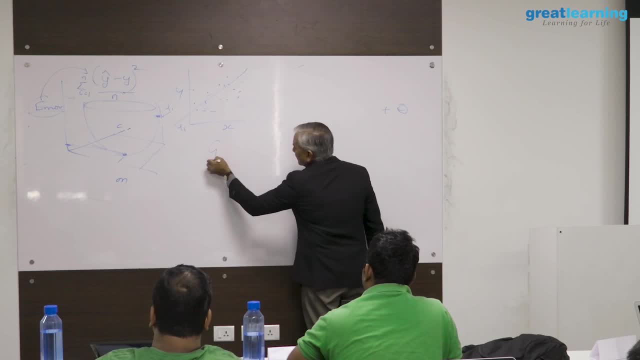 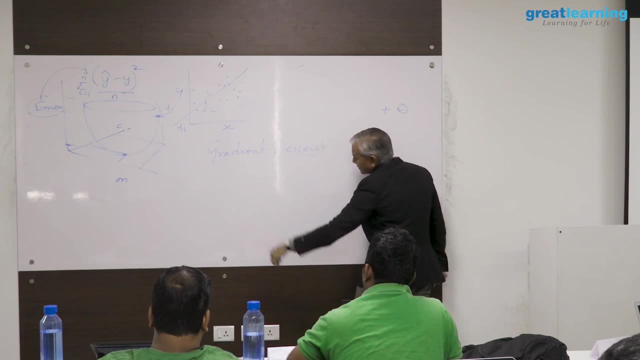 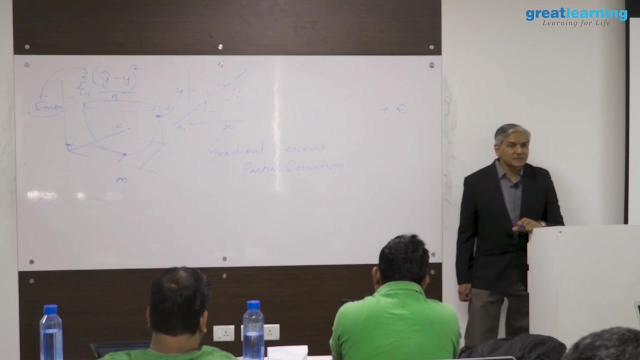 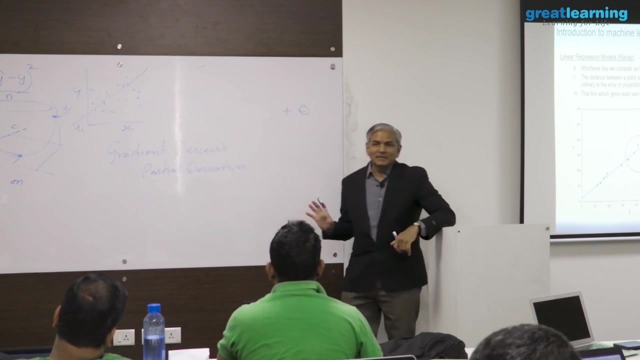 random m and c, and it uses a concept called gradient descent Descent. As the name suggests, we have to descend Gradient descent algorithm, Which internally makes use of what is called partial derivatives. Partial derivatives And this term partial derivatives. I will tell you what it is. It is not a rocket science. 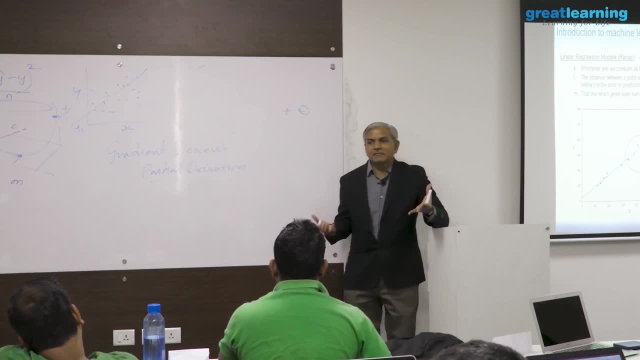 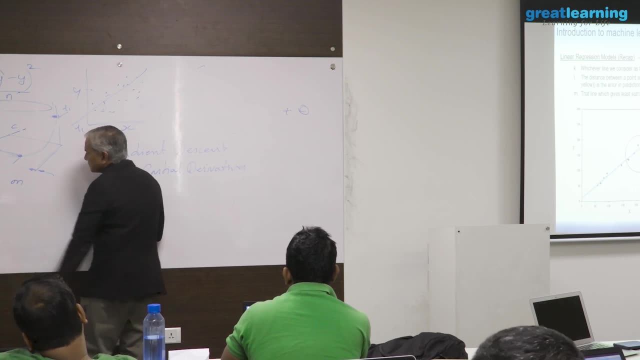 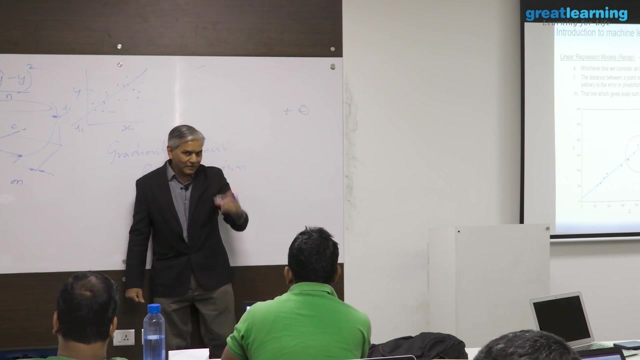 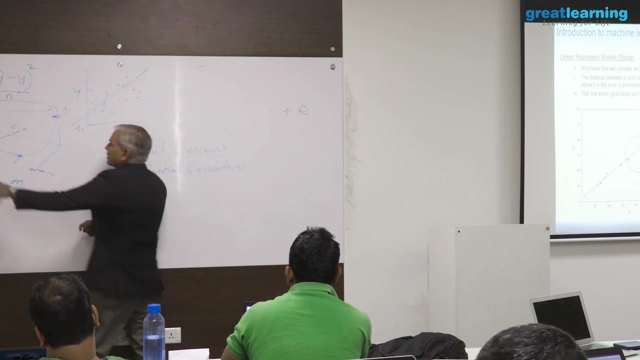 It is dy by dx. It is exactly dy by dx. What it does is for a small change in m in this direction or this direction, For a small change in m in this direction or this direction from the first m, the random m, For a small change in m in this direction or this direction, dx. How much the error drops. 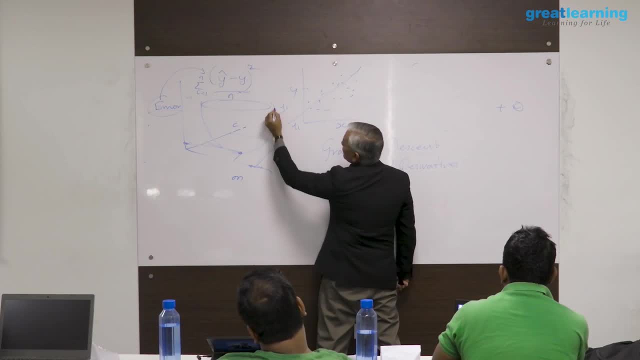 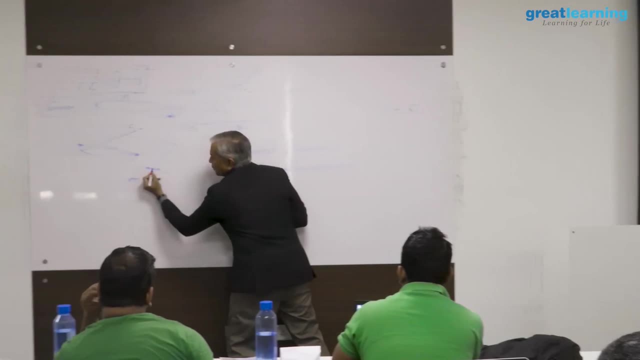 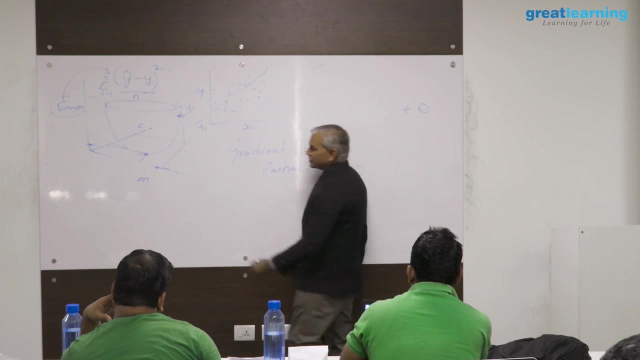 or increases. So when I change it in this direction I am going further up. The error increases, Dy increases, Whereas if I go in this direction I reduce my m, My dy decreases, That is, my decreases. So it notes down that I have to move in this direction. But you have taken 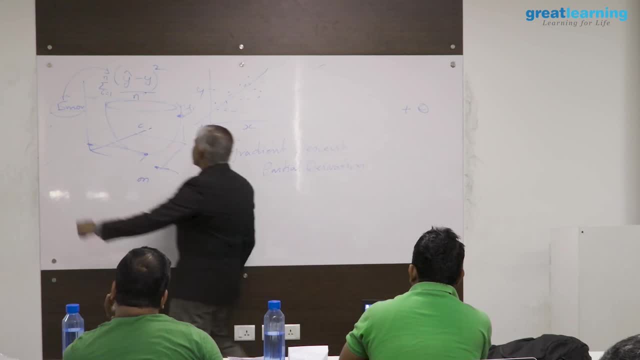 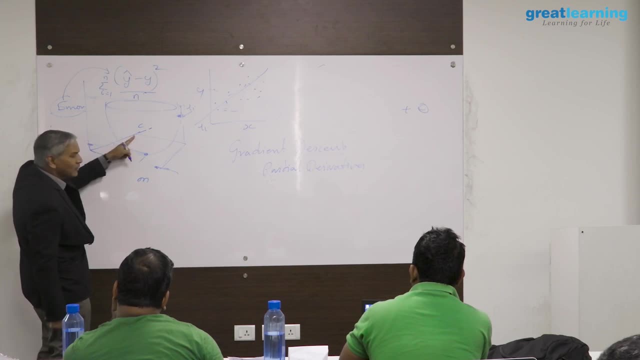 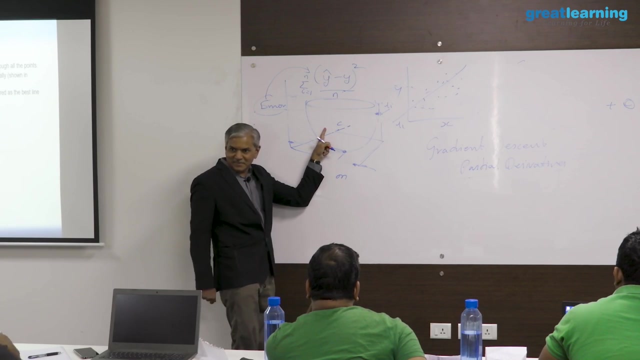 only m right now. How about c? So do the same thing with c. If I increase the c slightly here, what happens to my error? If I c slightly here, what happens to my error? I will go in that direction where my error decreases descent. So using this concept of partial 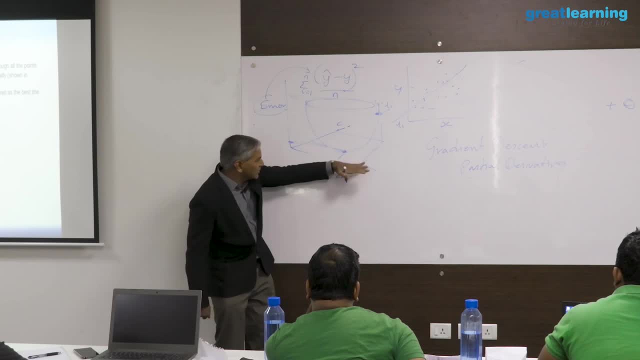 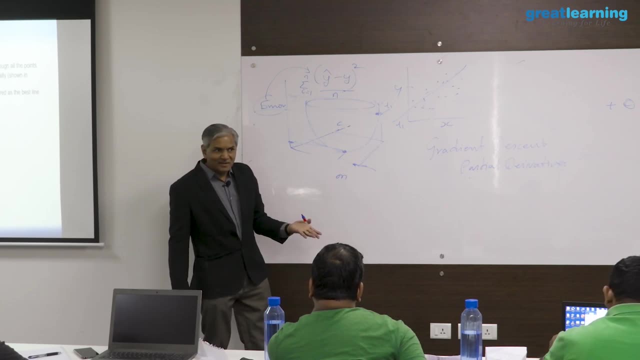 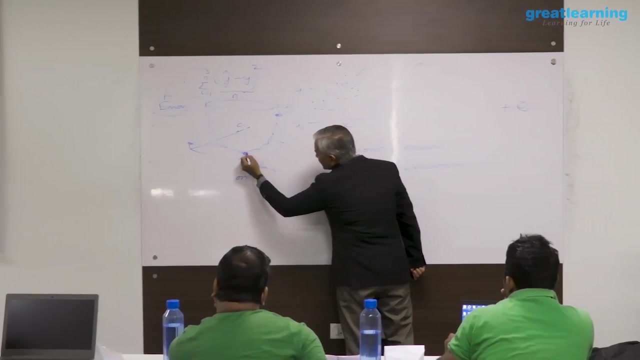 derivatives, which is nothing but dy by dx, applied on individual dimensions, one at a time, one at a time. that is why it is called partial. It finds out, it moves from this line to the next line, to the next line, to the next line, until it reaches this point. 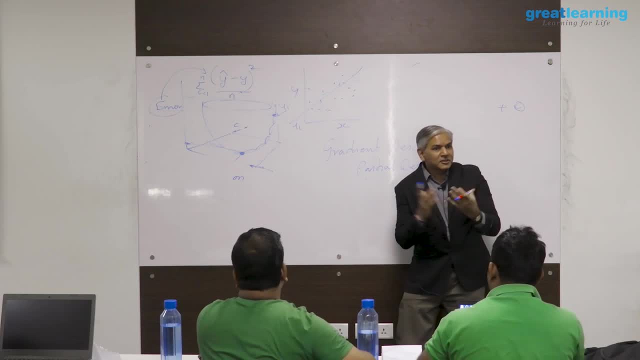 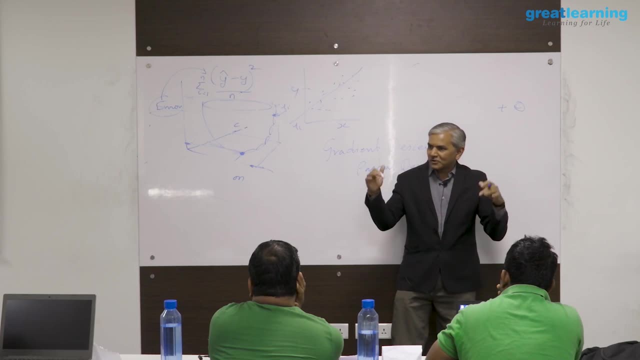 At this point, what will happen is, whichever direction you move in beyond this, the error is only going to go up, Whether you go this side or that side, error is not going to come down further. So it realizes that it has reached the global minima. 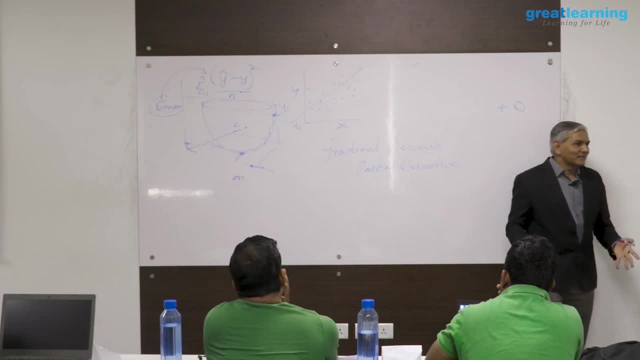 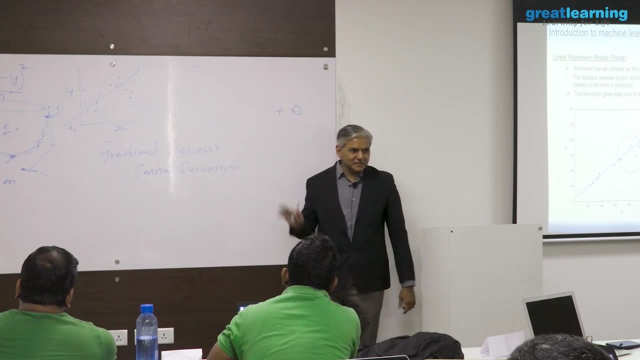 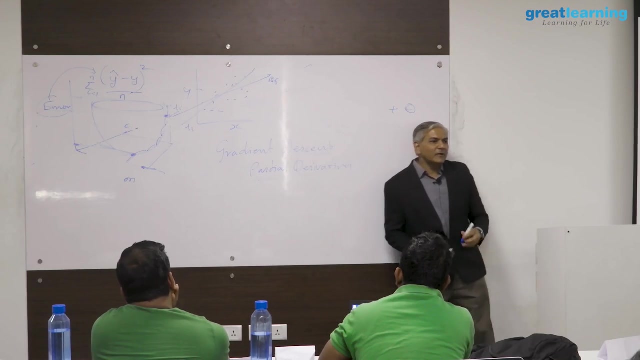 This is your best fit line, Which is the relation between m and e plus c, m, Correct m, c, m, e put together, This is your best fit line. That best fit line happens to be this line B, So it does not evaluate infinite lines. It uses this gradient descent concept and 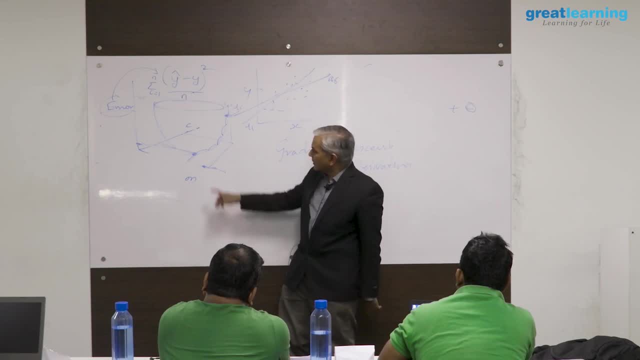 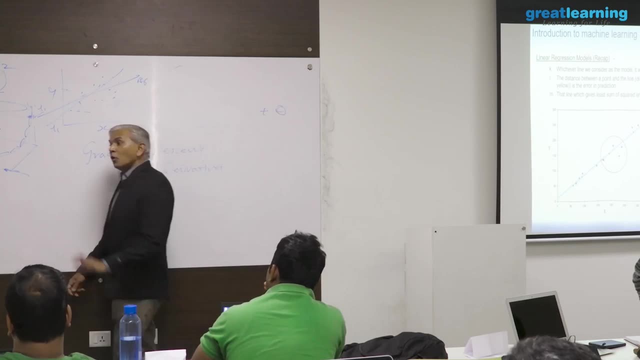 finds out for the next best fit line, Next, next, next, and reaches the global minima. So is there a chance of jumping that? Yeah, There is, And there can be local minima as well in case of Not in quadratic functions. 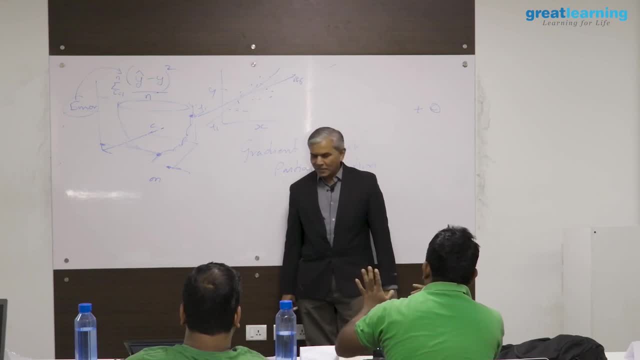 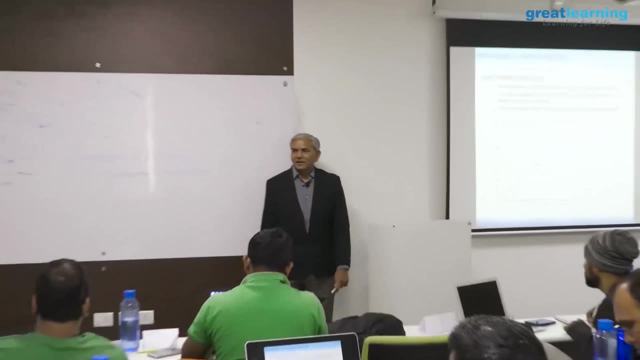 So in linear regression we will never have group functions. You will never have. If we use neural networks, you can get stuck in local minima. Okay, sir, Linear regression- the error function being quadratic, it guarantees you will reach absolute minima. okay, But in the process of the linear regression it is a function that is like: 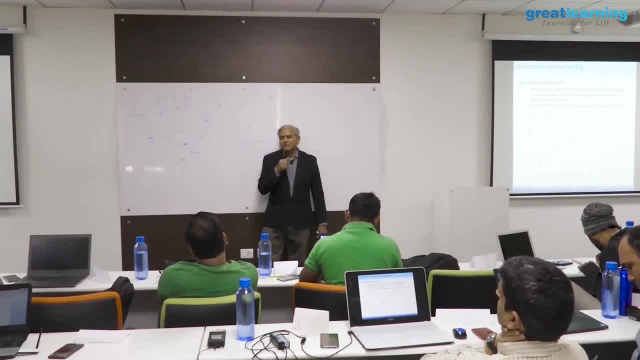 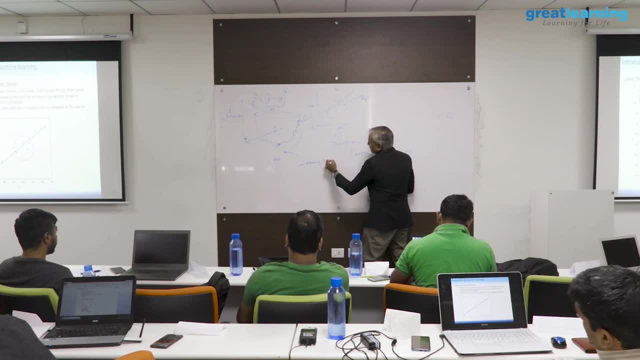 a network. So which number should I get? Four, Five in the process of jumping, there is something called learning step. okay, We are too far away from this, so I will not. I will just tell you the concept which is used, along with: 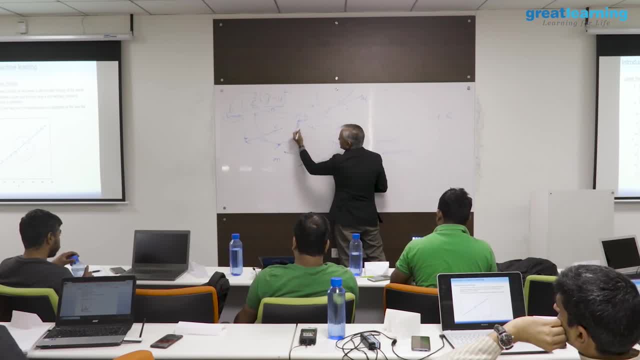 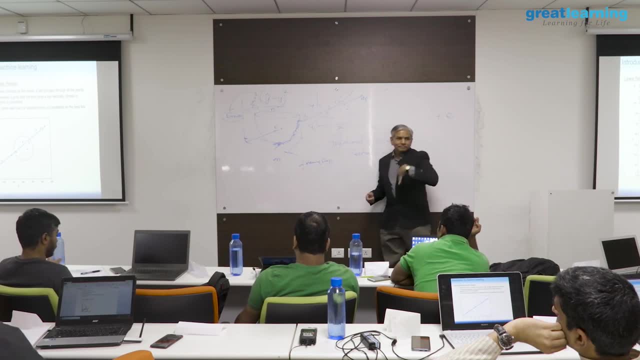 this partial derivatives. If the learning step, the amount of change that you do in dy and dx, if the learning step is too high, you might jump and oscillate. You might jump the global minimum, go on the wrong side and keep oscillating backward and forward, infinite. 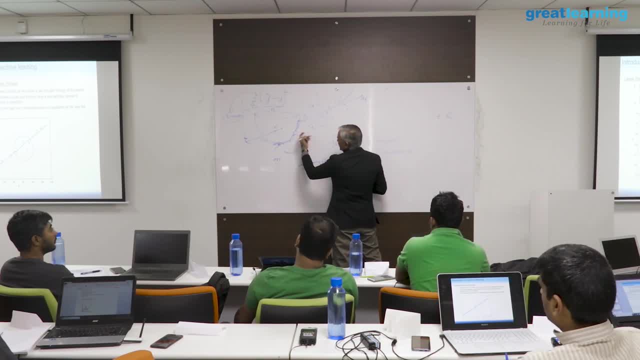 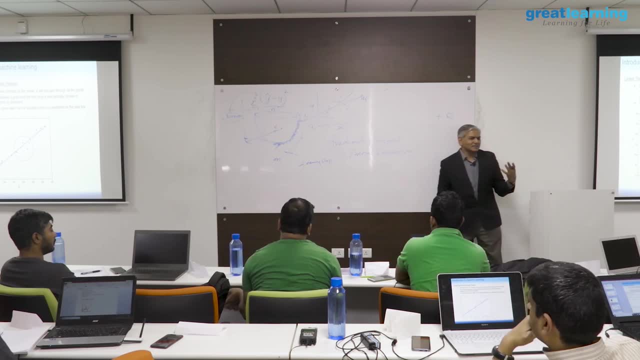 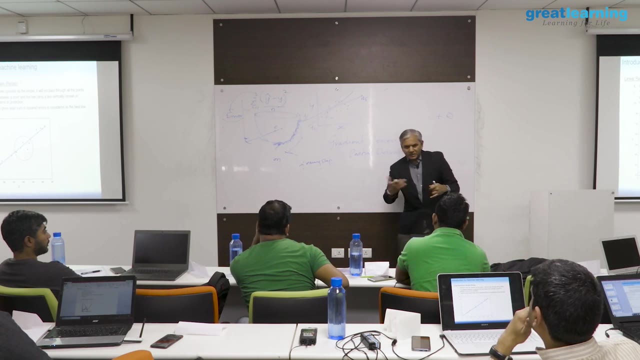 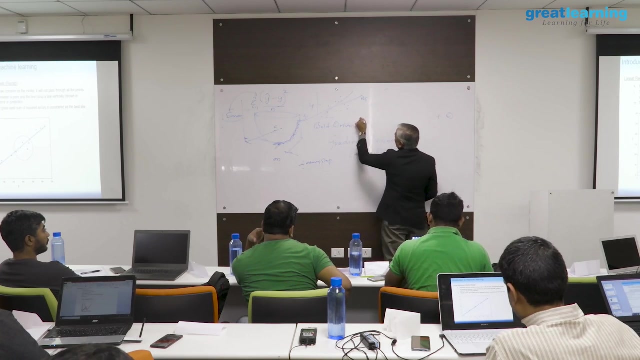 loops, So the learning step is adjusted. As it keeps jumping down, the learning steps become smaller and smaller. There are various ways of handling this to prevent the oscillation. One of the ways is, as you jump towards your objective- the goal- the steps become smaller and smaller. This algorithm is called bold driver algorithm. 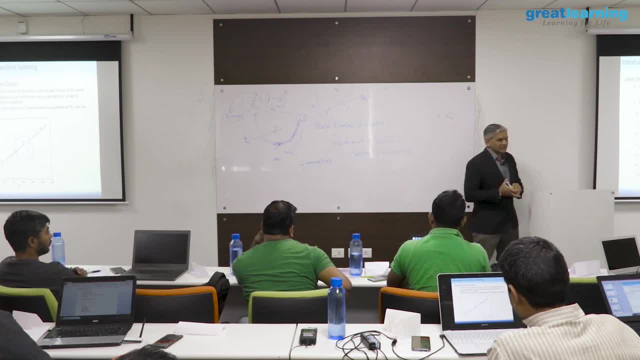 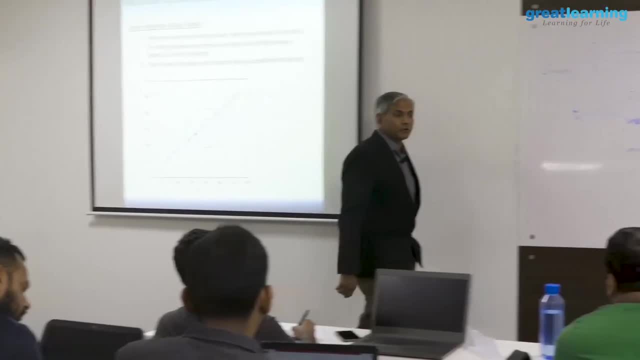 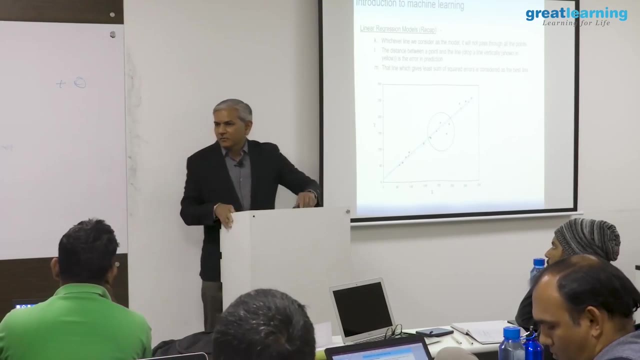 which is part of your gradient descent, one variant of gradient descent. When you do deep learning, this partial derivatives- will become very important for you to understand how the neural networks work, how the back propagation of errors happen. those things will come into play. okay, But we still have lot of time before we reach there, So hopefully, 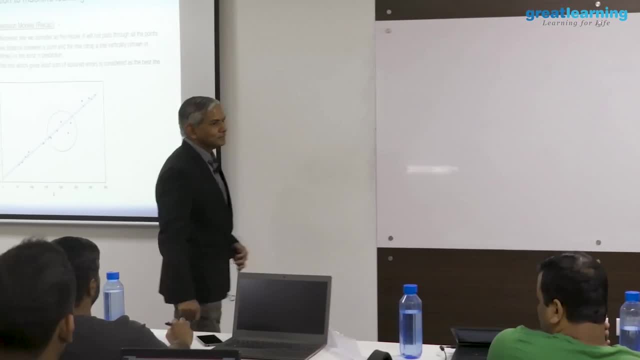 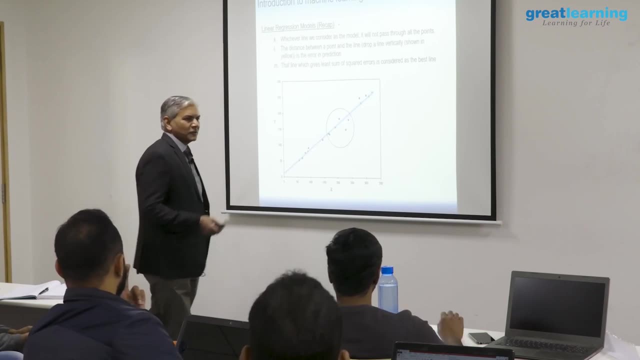 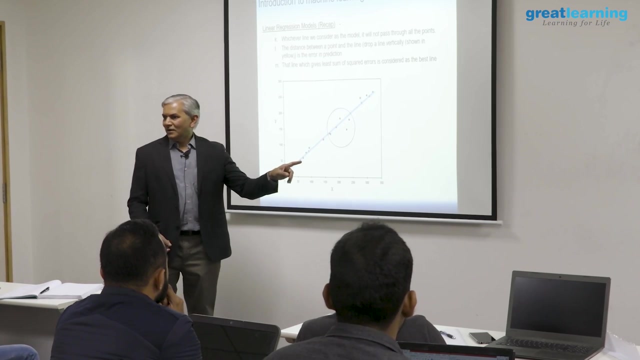 I will spend some time on this one day and tell you what this is, But you have various other algorithms now which have come up which is apparently better than this. Okay, we will talk about those things down the line. Shall, I move on? All of you, Okay? 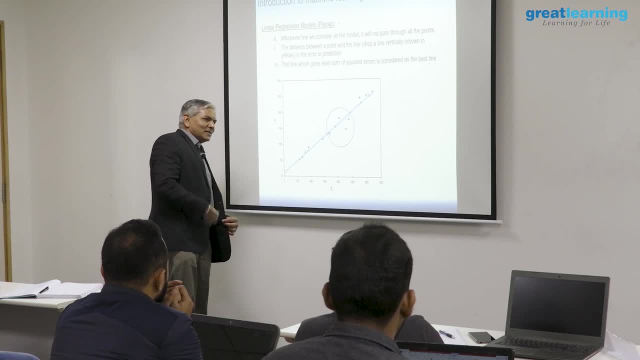 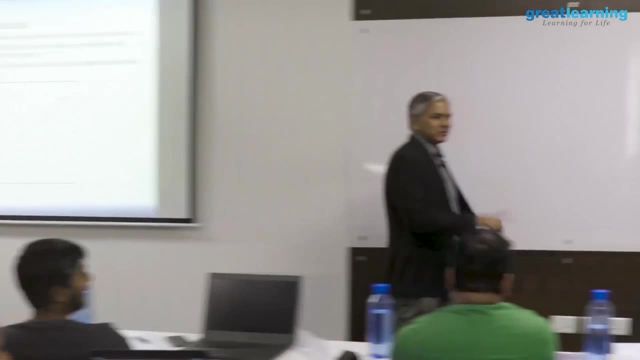 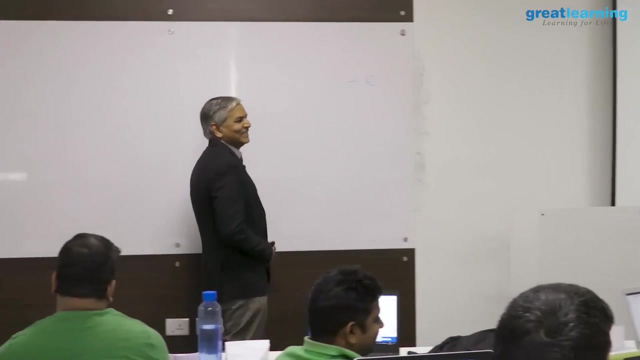 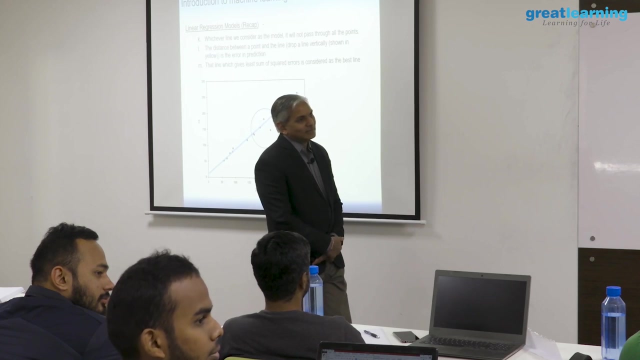 Your questions are still parked right. The two questions. what are those two questions? Why there should be no collinearity? 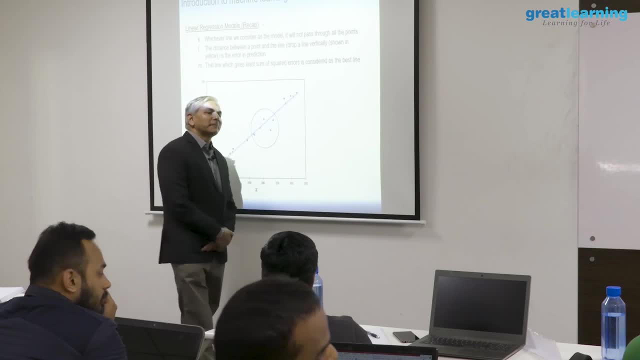 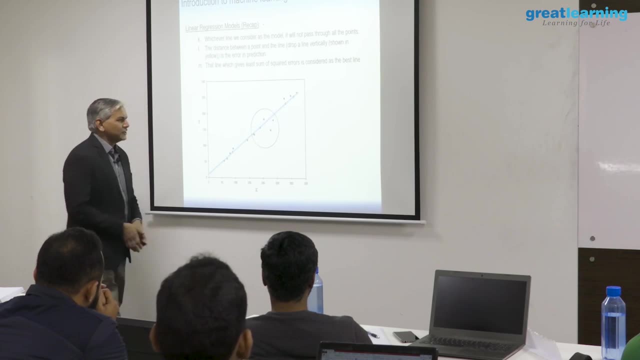 Why should there be no collinearity? What happens if there is collinearity? That is one of the questions which came up. I remember that Good, So my strategy worked. Okay, let us move on. Okay, We will discuss those things in detail, right, Okay? 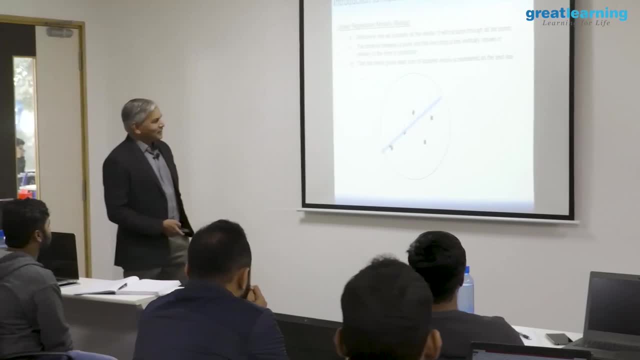 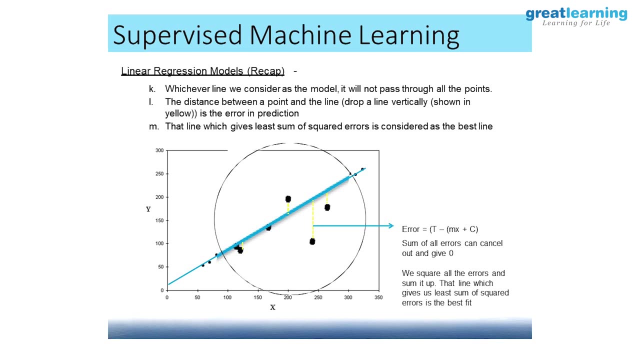 So keep in mind- we are looking at these data points closely- The distance between The distance between the actuals and the line. the line is the predicted values for a given value of x. the predicted value of y is the blue line. 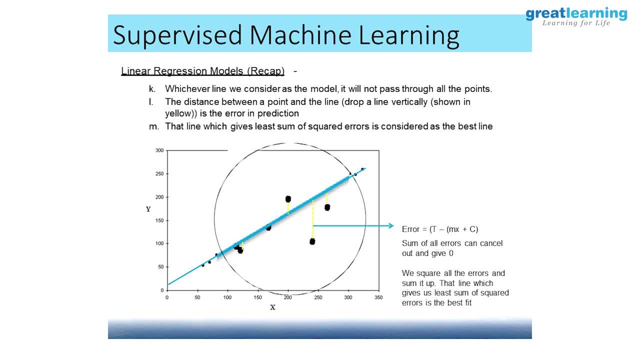 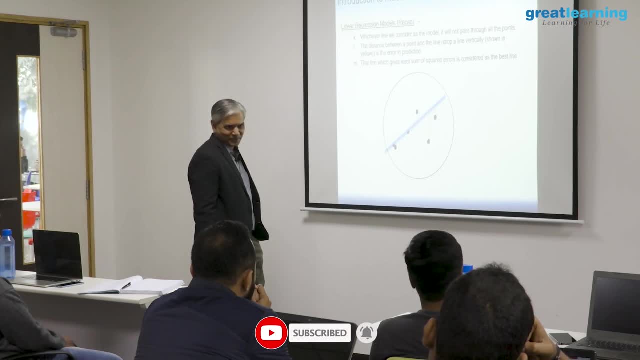 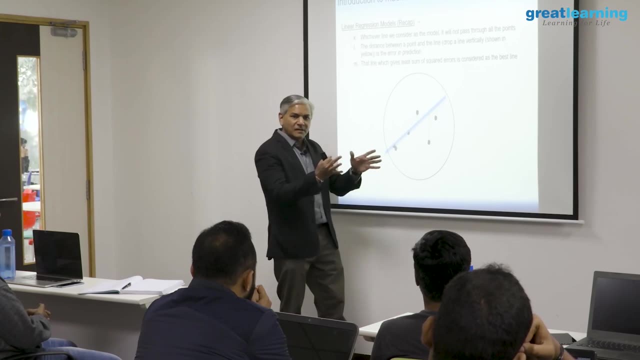 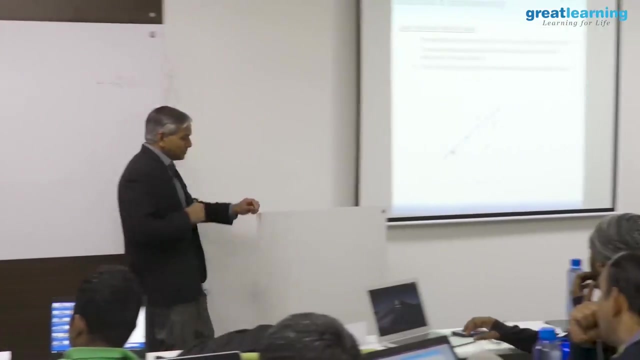 The distance between the actual, which is shown by the black dot, and the line that distance is shown by yellow dashed lines. this distance is a measurement of error. The objective is: square of these errors, all these errors squared, that sum should be minimized, ok, which is not very difficult to conceptualize. once again, 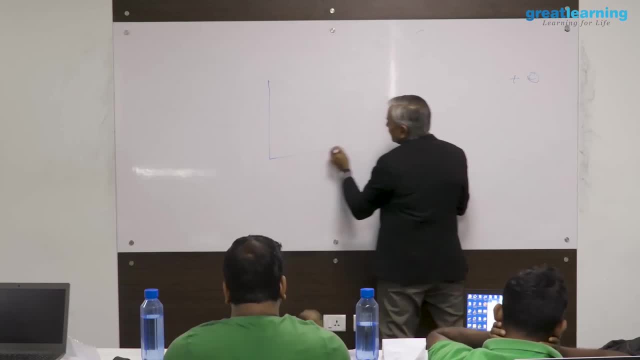 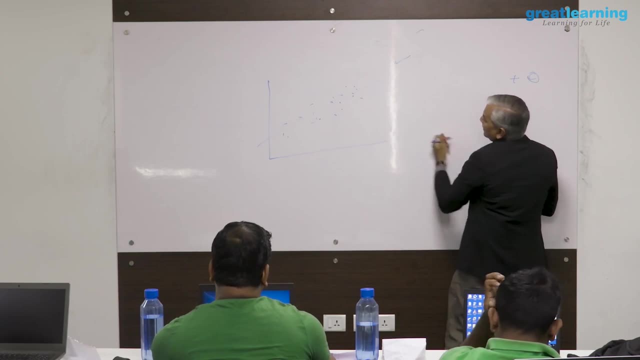 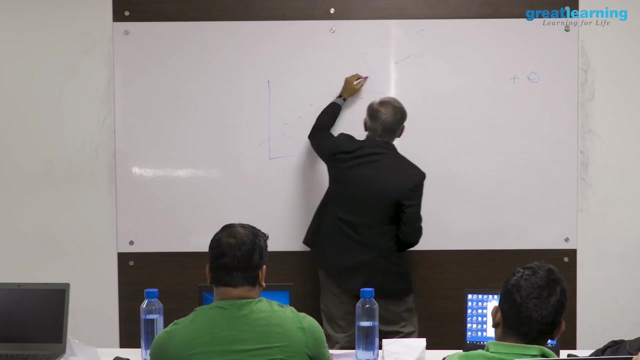 So if I have my linear model drawn like this best fit line, the data points are scattered around this. you look at the data point from this angle. when you do that, you will see a spread, This variance. this is called sum of squared errors, which is nothing but xi minus x bar. 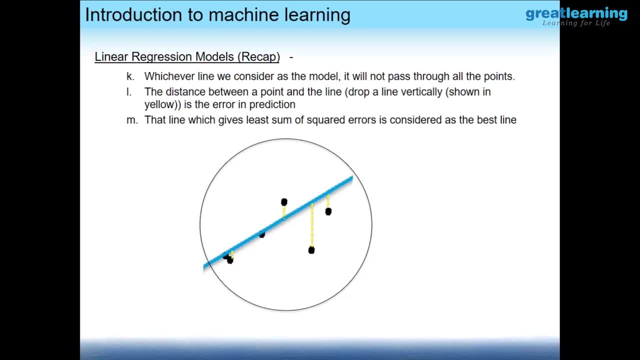 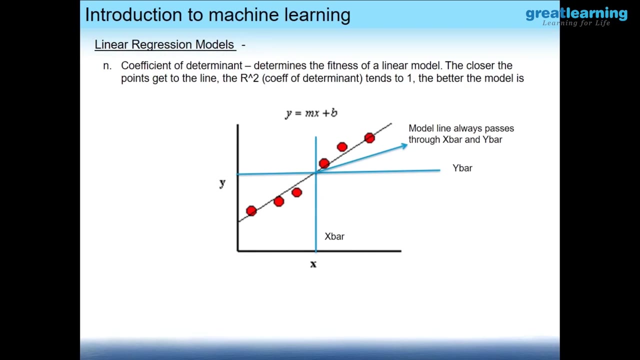 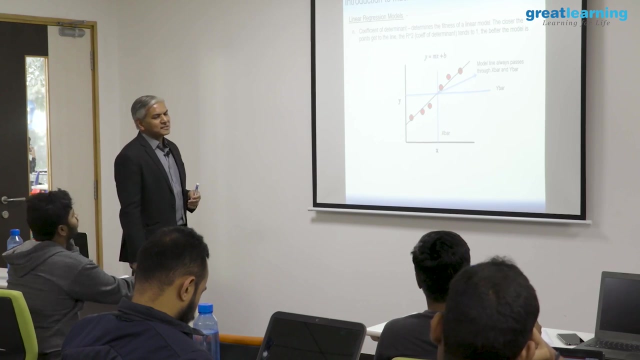 x bar. here is here. These are the predicted lines. so formula remains same. That variance is called sum of squared errors. that variance we have to minimize. The minimal the variance is, the better your model is alright. So let me explain this to you, because you are going to come across these terms down. 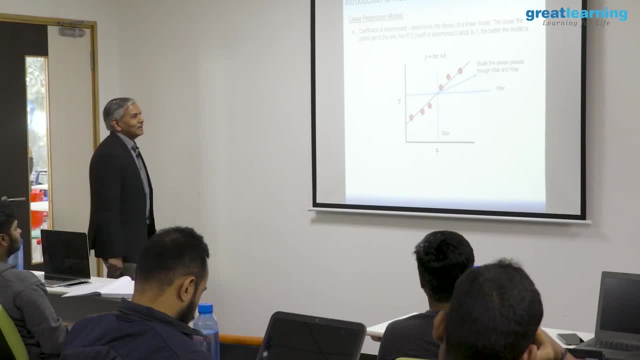 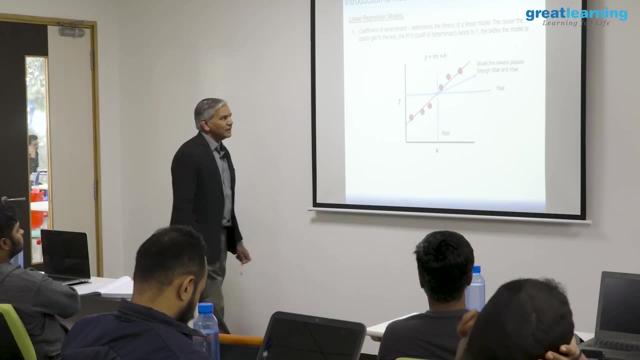 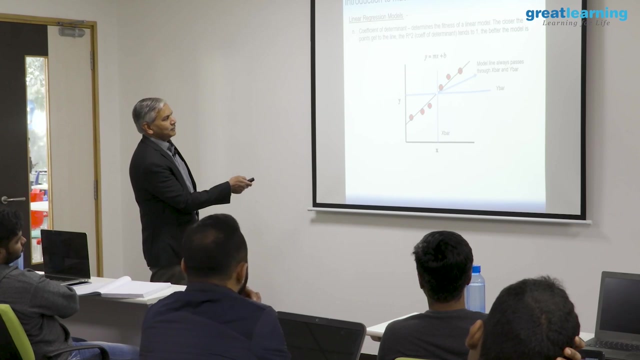 the line. so let me explain this to you in slightly more detail. We are looking at this model And the distribution of the points. the rate points is given to you, The blue lines are x bar and y bar. And keep in mind your model. the best fit line will always go through the point where 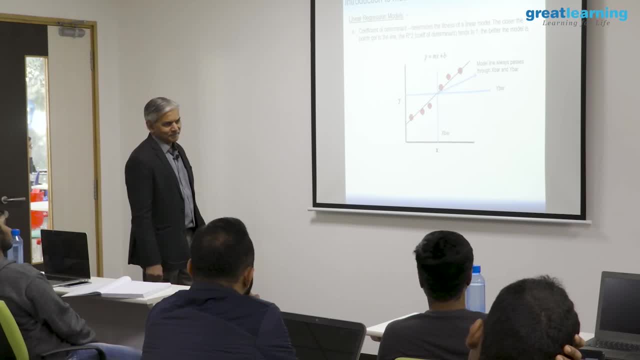 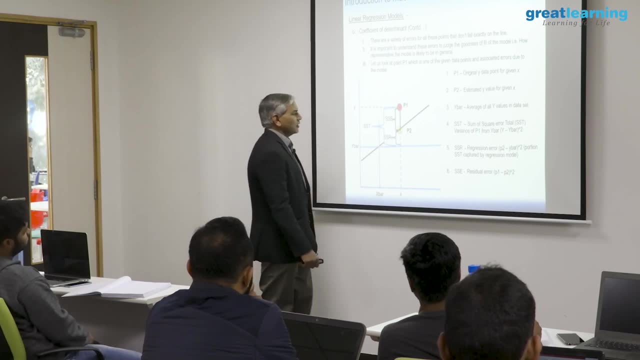 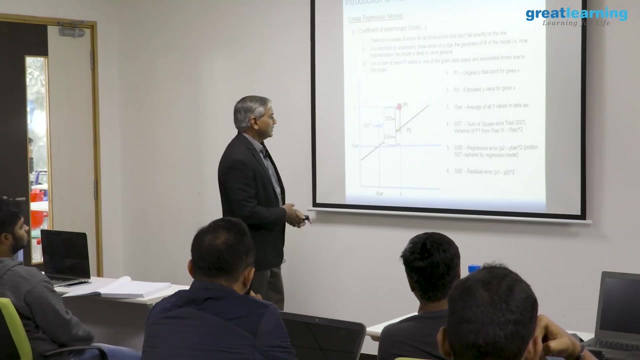 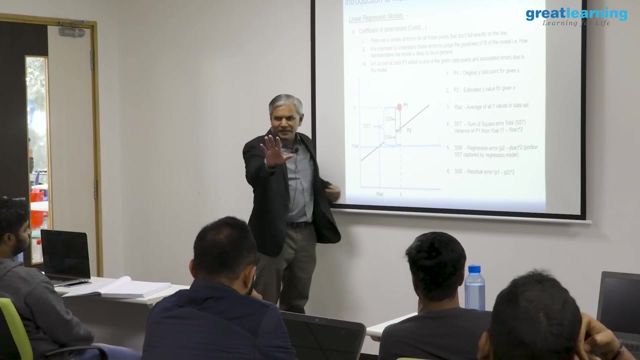 x bar and y bar meet always. ok, Now look at this. do not worry about these terms, it is all I mean. not very difficult to conceptualize, Visualize what happened. yeah, there you go. Now if I take the red point. red point is the actual point in my data set. 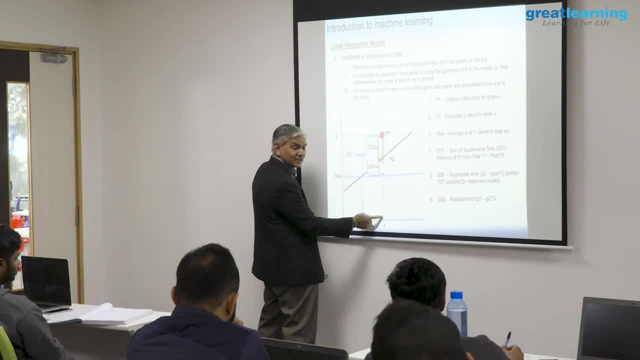 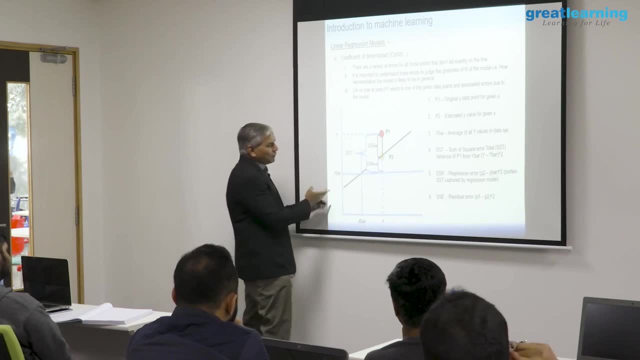 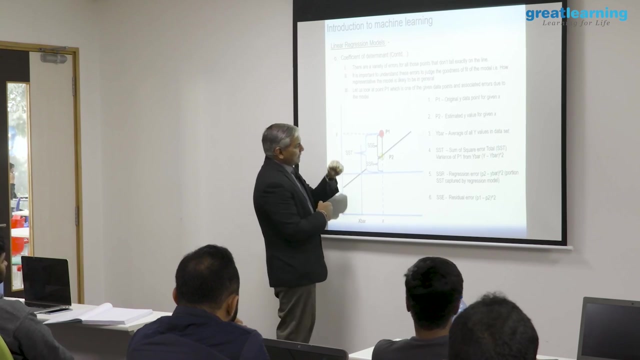 In your data set, in your data frame, there is a record with value of x and its corresponding value. y is red, the p1.. But the model, the best fit line, says the value should be yellow, p2.. The distance between p2 and p2 is 0.. 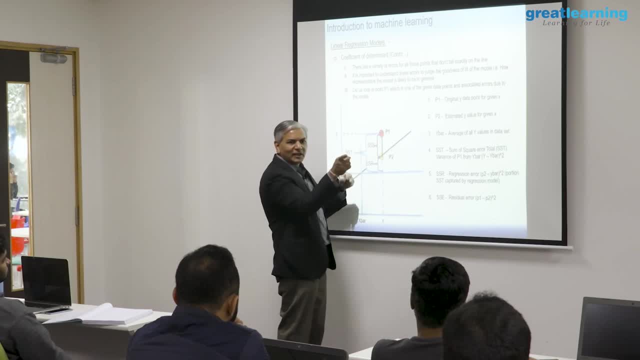 Ok, So this is the p1.. This is what we call error, the variance, This is what we call sum of squared errors. ok, I am showing you only one data point here, but you have to imagine there are multiple data points here. 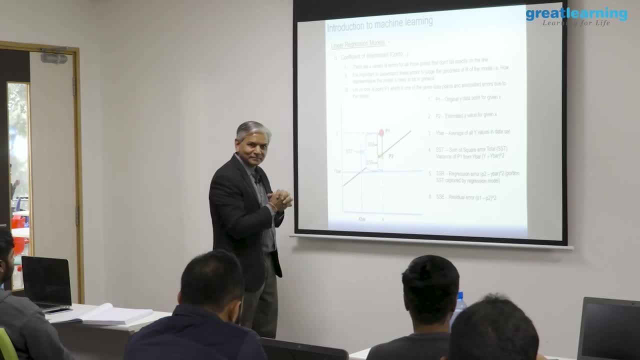 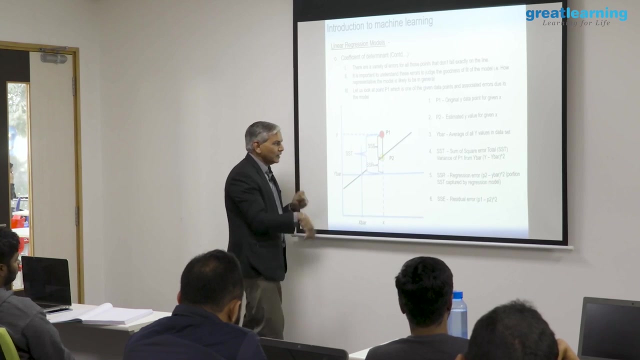 Sum of squared error applies all together. ok, So this contributes to the sum of squared error. There is another term that we use, which is called total error: Total error. across all the data points put together, The total error is nothing but the difference between y bar the expected value of y and. 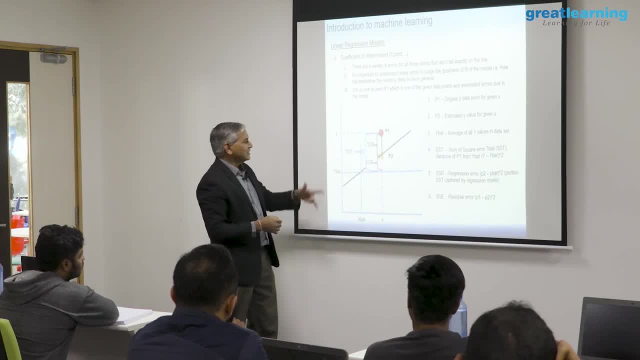 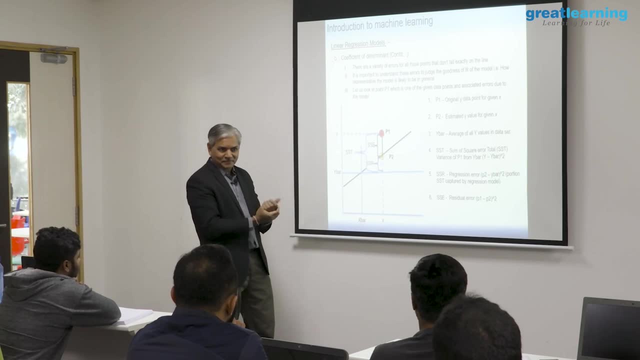 the actual value of y. In your data there is a distance between the actual value of y and the predicted value of the. the expected value of y, Expected value, is y bar. That distance is called total error. Of the total error, your model is 0.. 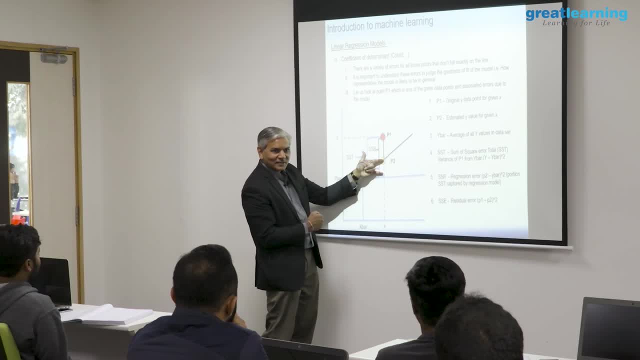 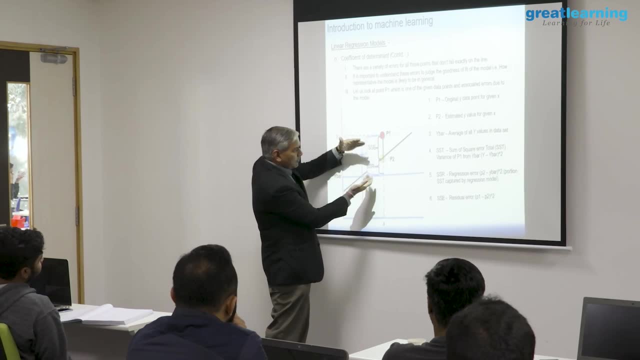 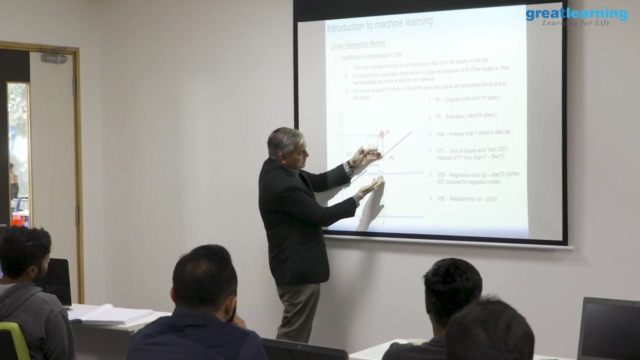 Ok, Your model has captured this much. Your model is a regression model, hence the name given to this is regression. error Of the total error: your model is predicted this much. error Of the total error in your data set: your model is predicted this much. 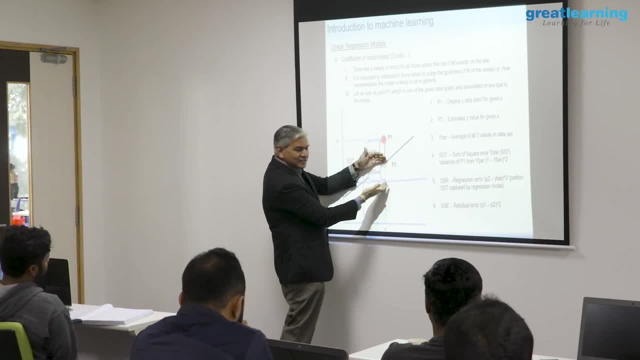 The difference between predicted and the y bar. This distance is called regression error. What it has not been able to explain is this: This is the distance between y bar and the predicted value of y. What it has not been able to explain is this: 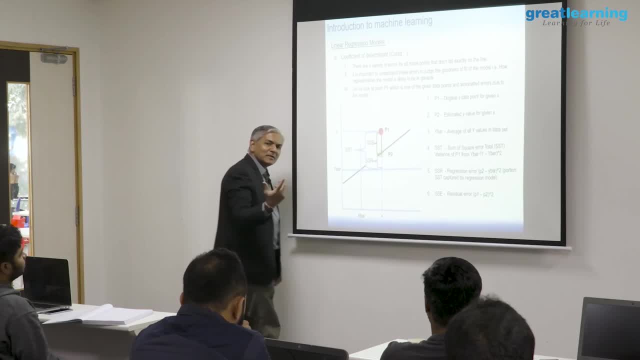 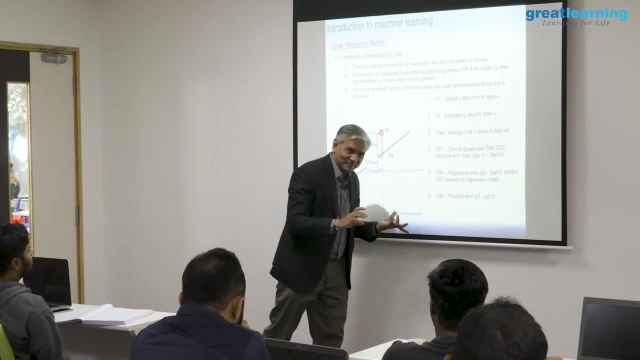 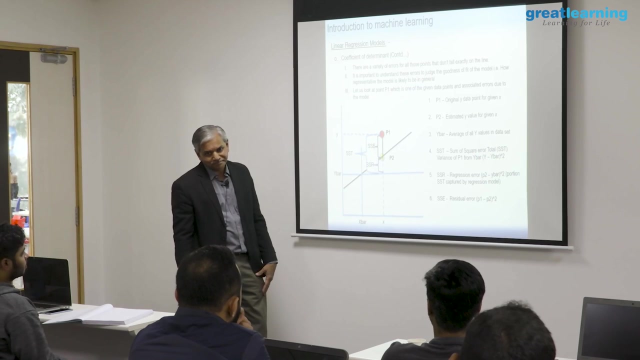 This is called sum of squared errors. Sum of squared error has another term, which is called residual errors. Residuals are those things which we dont have a reason for. We dont know why they occur. They are called residuals. Sum of squared errors is also known as residual errors. 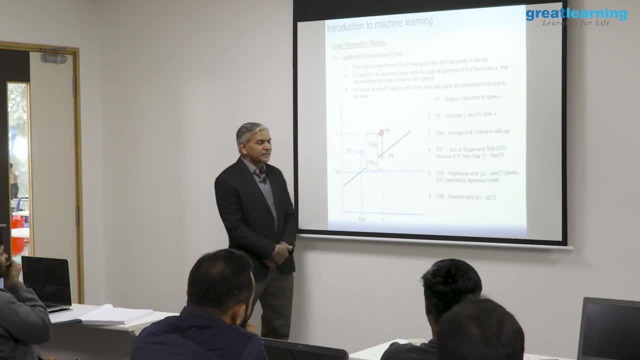 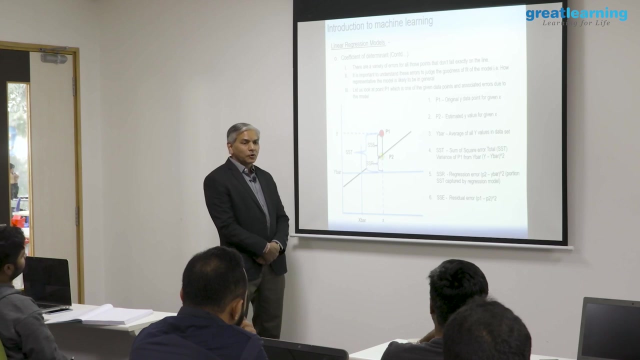 So when you build this model, especially when you go to your deep learning part and all those things, you will come across these terms: Total error is the distance between your actual data point and expected value. So, first of all, what this is: expected value. ok, So if the average height of this class is 5.5, the difference between 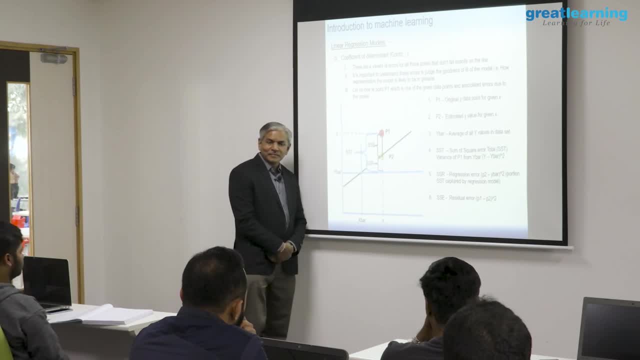 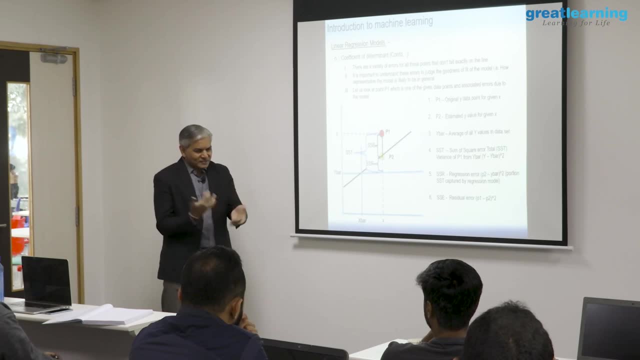 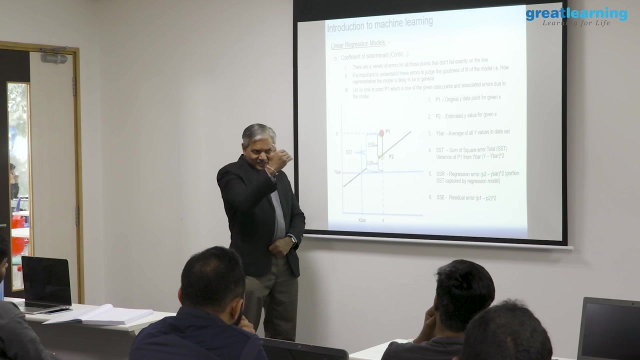 your height, and 5.5 is a total error. Now you have built a model to predict the height of a person in the class based on the characteristics of the person, So your model predicts some value for you. So the model predicts the height to be 5.3, your actual height is 6, 6 minus. 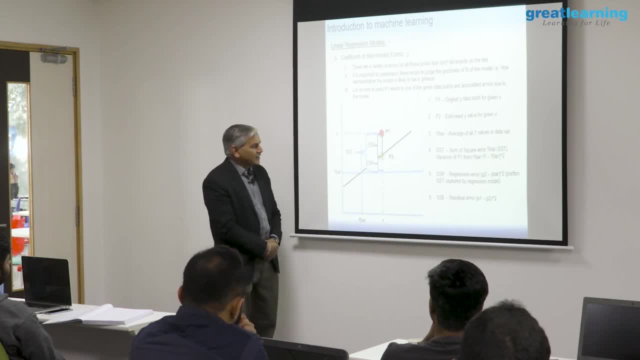 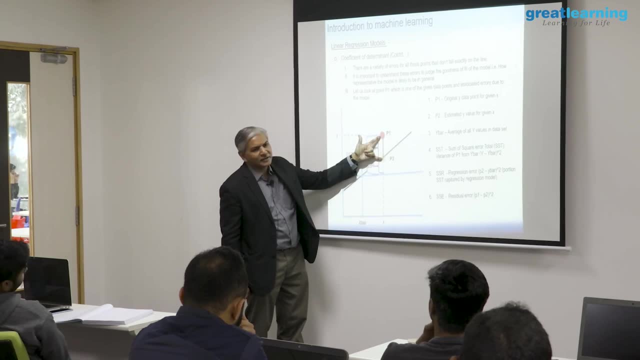 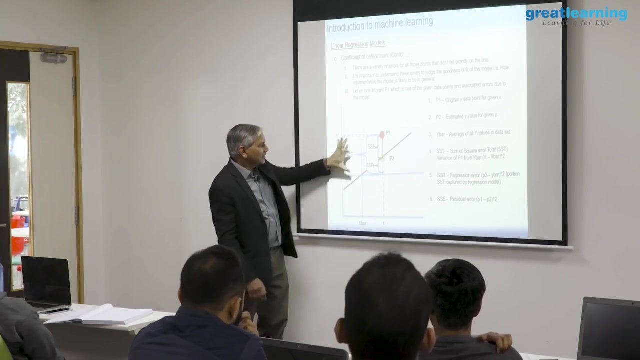 5.3. that is, 0.7,. 0.7 is the distance between: 0.7. is this distance your actual height minus predicted height? right The distance between your height and the class average? that is a total error. 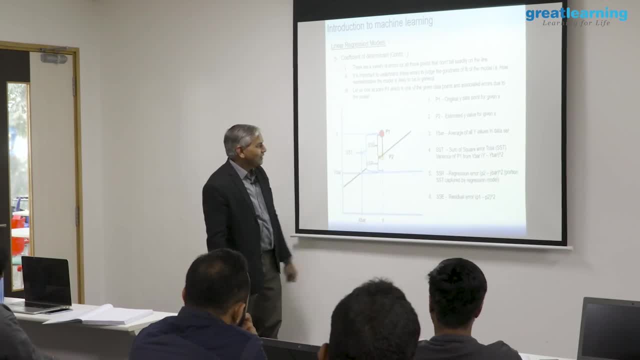 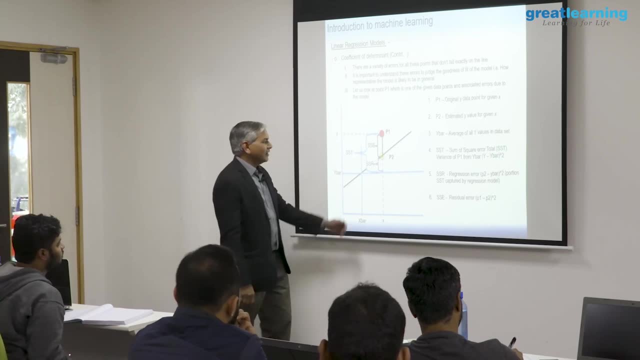 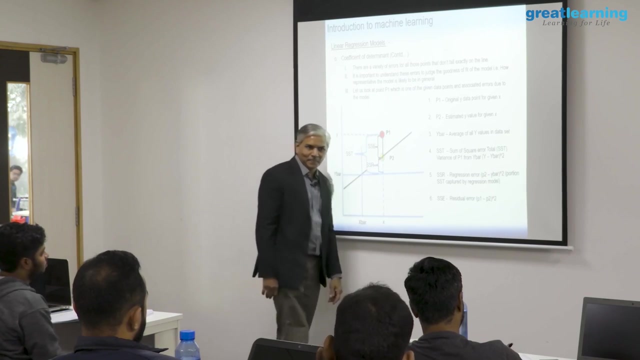 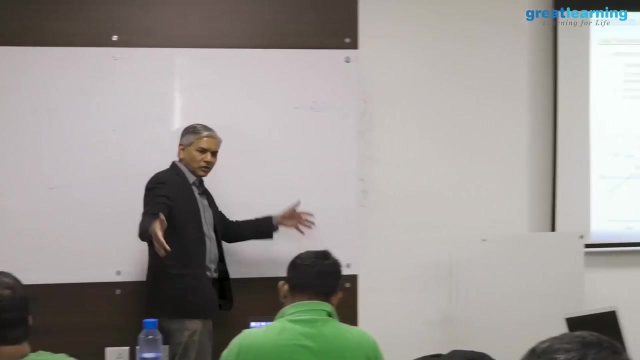 So you will come across three terms: total error, sum of squared errors and regression error. Keep in mind regression error and residual errors. these two together is a total error. And do not mistake the word error. error means variance, error means variance Of the total. 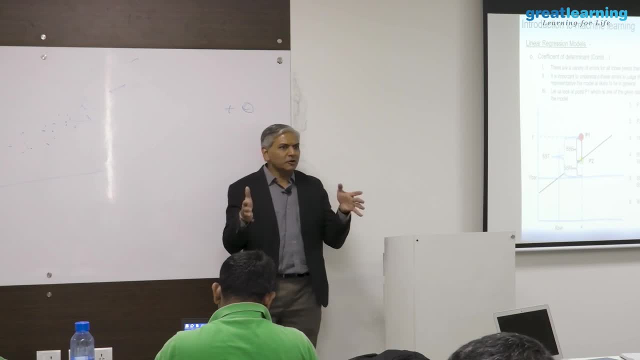 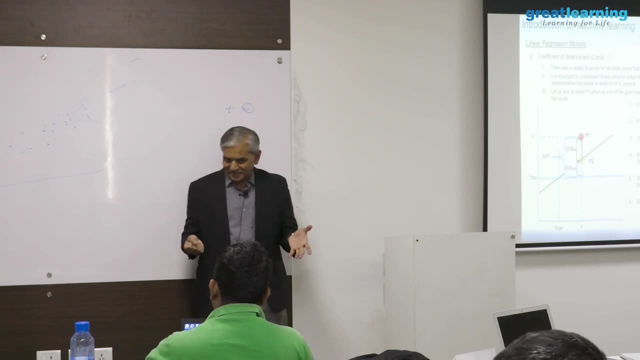 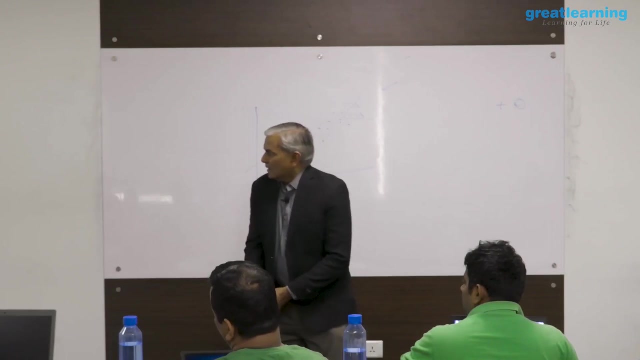 variance in your data set. I told you one part of the variance is caused by the deterministic variance. The other part of the variance is caused by the stochastic, non-deterministic. same thing. Non-deterministic is your residual errors: sum of squared errors. 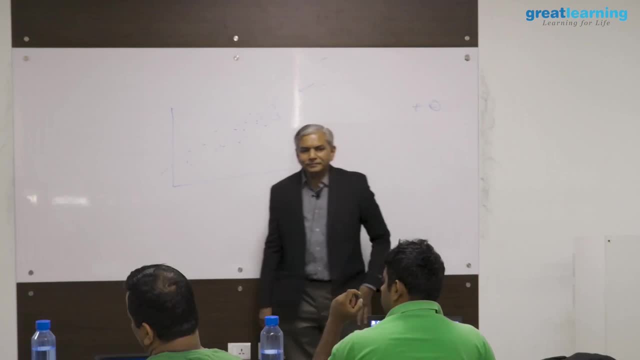 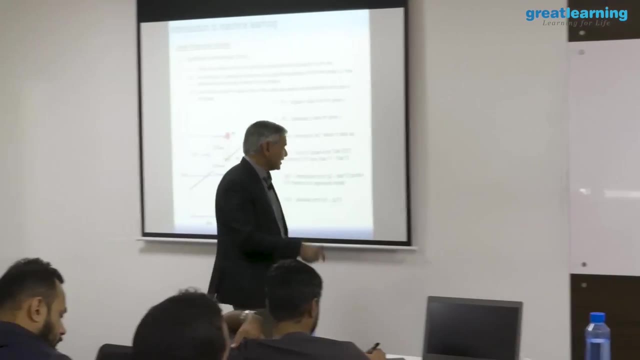 Sir, so you told this: see total error or the regression error, not a residual error, is particular to particular point, right? No, in this case I am showing you only one point, but you have to imagine all the points together, because this SSE, SSR, they are across. 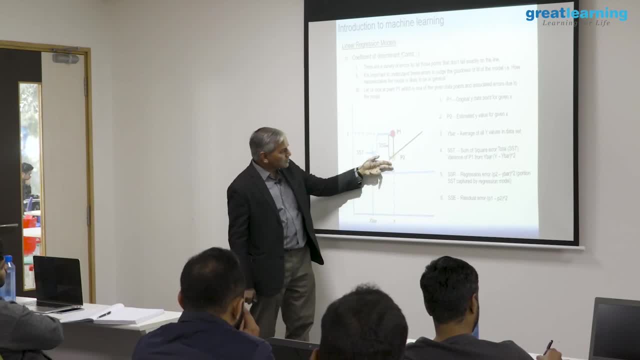 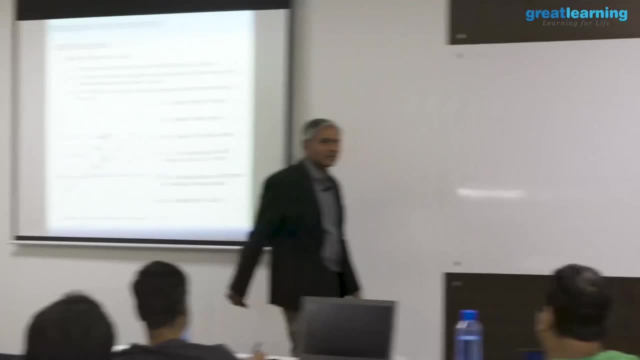 all points put together. What I am saying is what contributes to SSR and SSE. that is what I am showing you. So you have to imagine all the points here. that becomes too cluttered. that is what I am showing you: What contributes to SSR? what contributes? 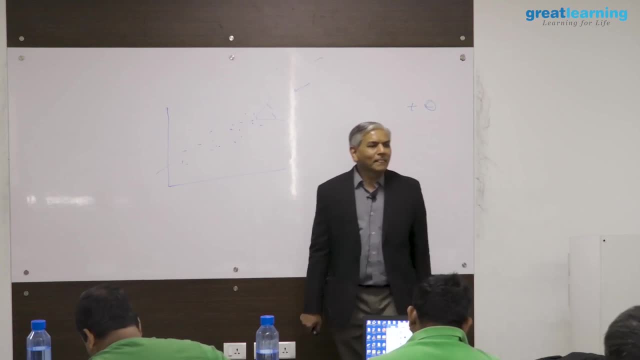 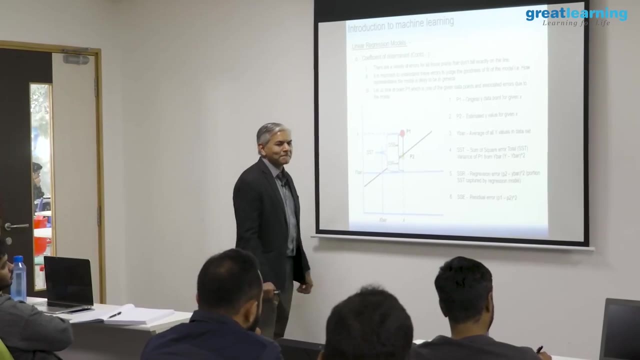 to SSE. that is what I am showing you over here. So least error is belonging to SST, right Yeah, least error is belonging to SST means We are talking about total error. Total error is this. I want to minimize this. 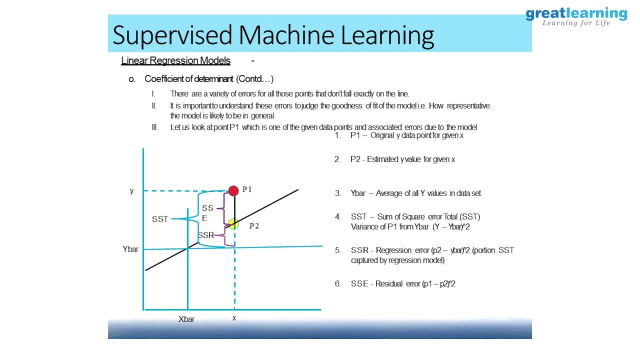 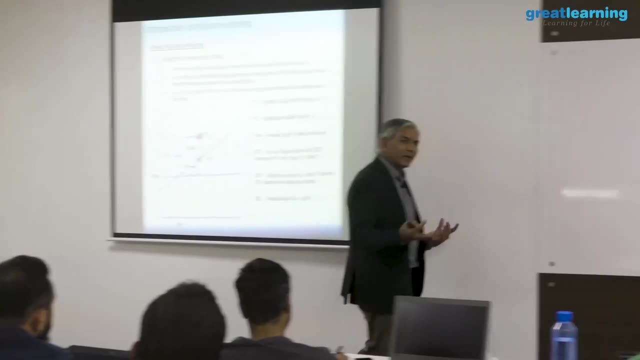 unexplained error. that is what my objective is. The gradient descent works in finding the best fit line for you. where best fit line is that line where this error is minimized, Because I do not want a model which is not able to tell me why. I want a model which 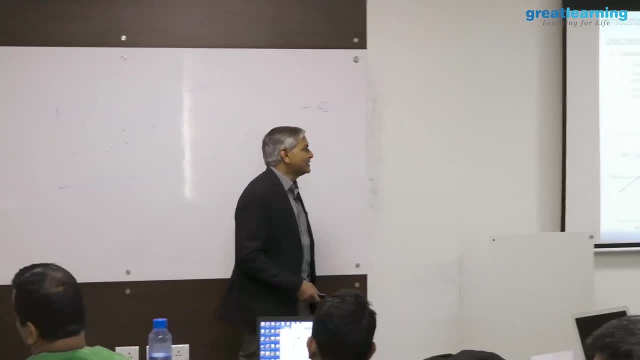 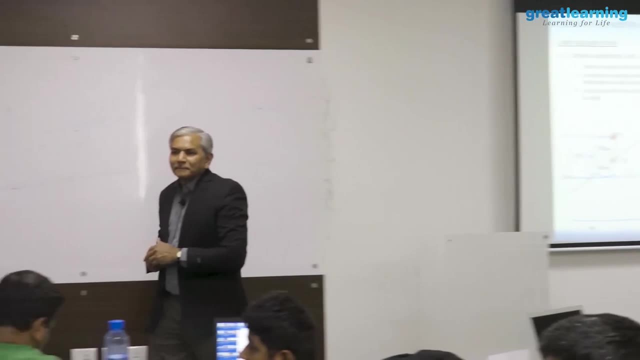 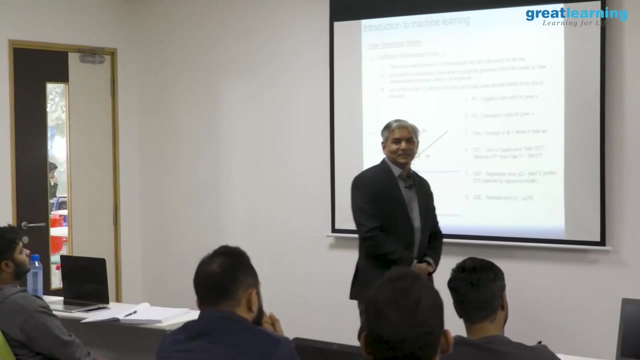 tells me why this error. So you will not try to reduce the regression error? No, we will not try. we will not do that because I am a deterministic. I know why it happens: It is because of the variance of the 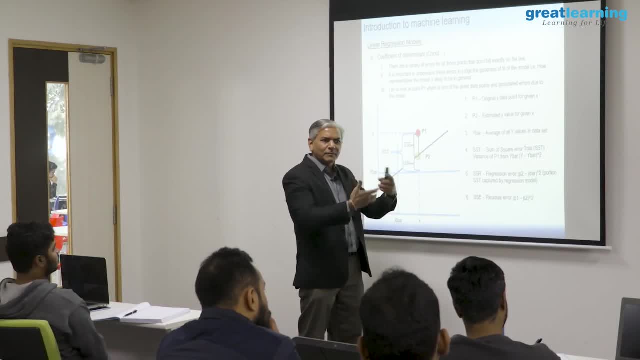 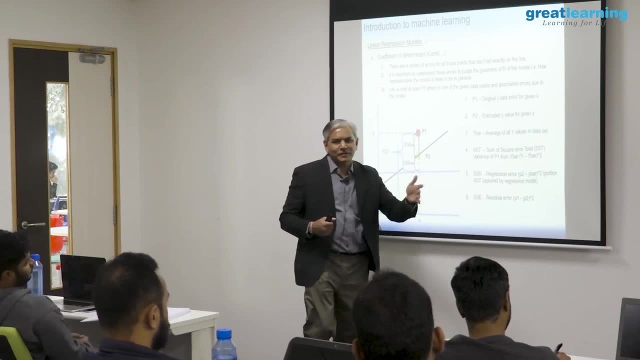 It is because of the natural variance in the process. When you are running a process, many things come into play. factors come into play, because of which the values change here and there around the expected value. that is ok with me, But for a given value of input there. 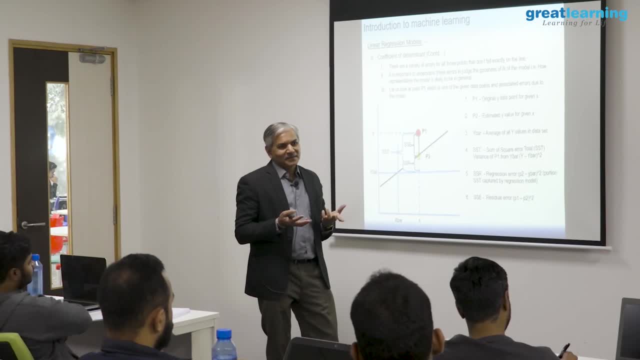 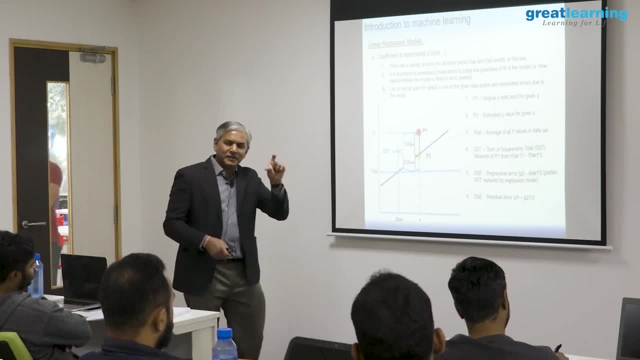 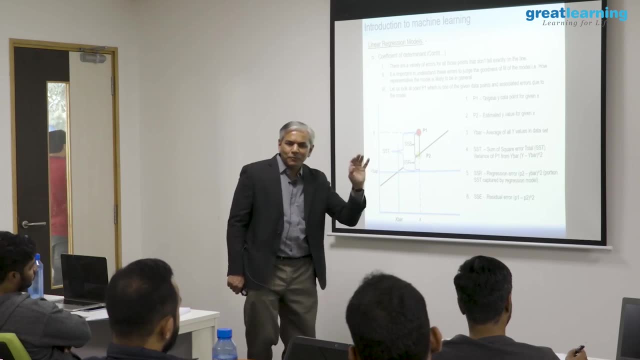 multiple values of y. That I do not understand. That part is my unexplained error. I want a model which unexplained error is minimized. I do not want a model where unexplained error is very high. What is the use of that model? It will not predict anything. 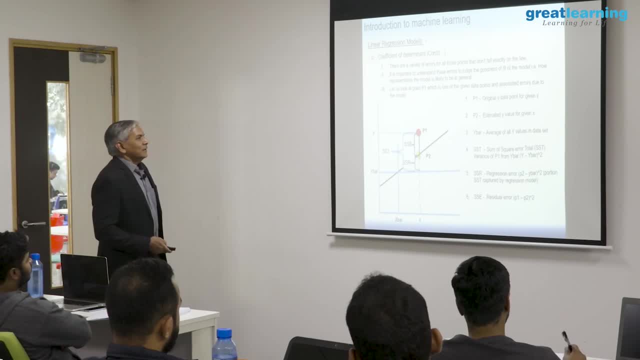 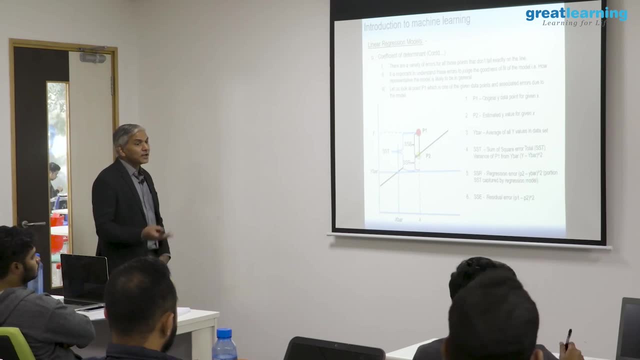 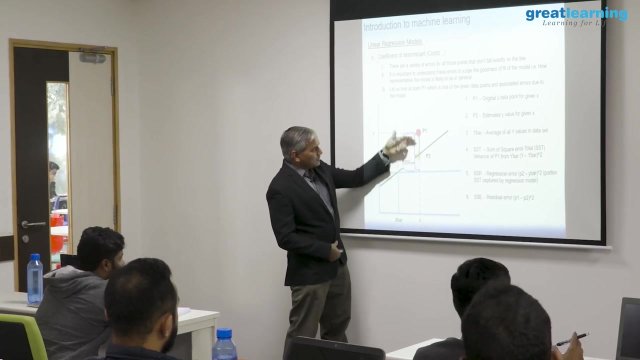 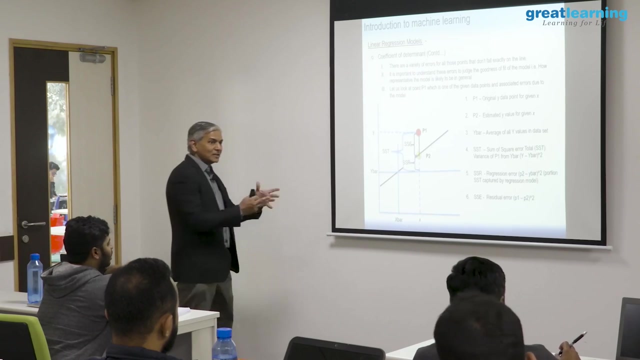 When you say, given value of x, you have one value of y. So in this case, in this case, p2 is that one value, p2 is predicted value, but you have multiple values of p1s spread around the line. That gap is unexplained. That variance is what we call stochastic random. 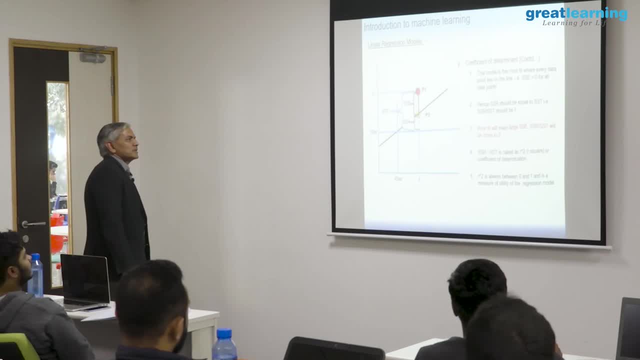 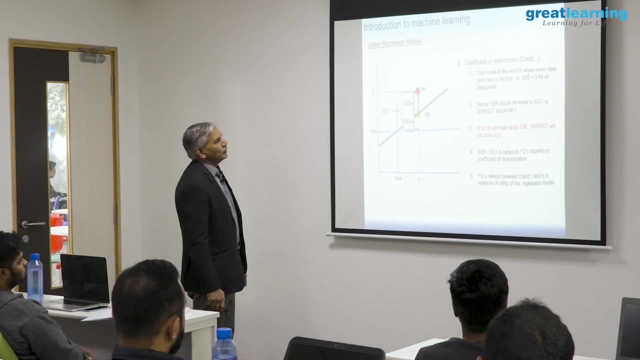 variance. We do not know why it happens. So, basically, the idea is to minimize SSE. that is all. The bottom line is: minimize SSE, So increase the SSR to SST ratio. that is what our objective is. Ok, All right, Let us move on. So before you build the model, you have to evaluate each 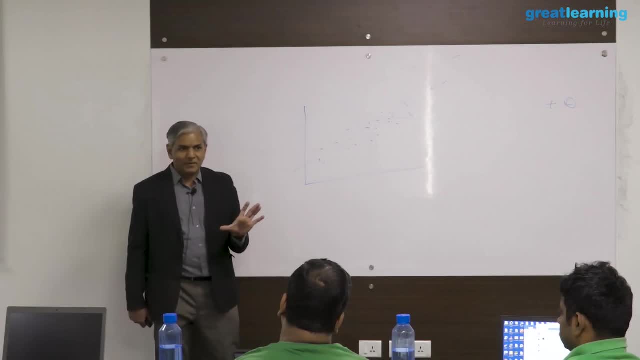 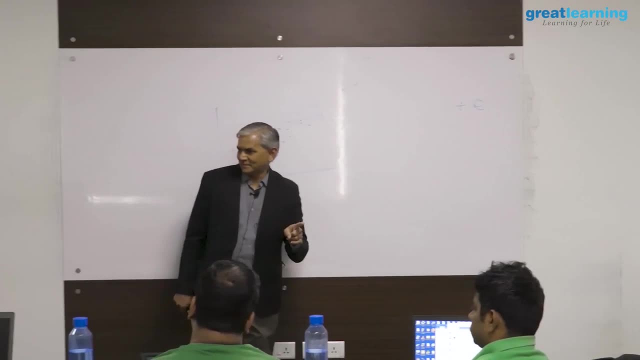 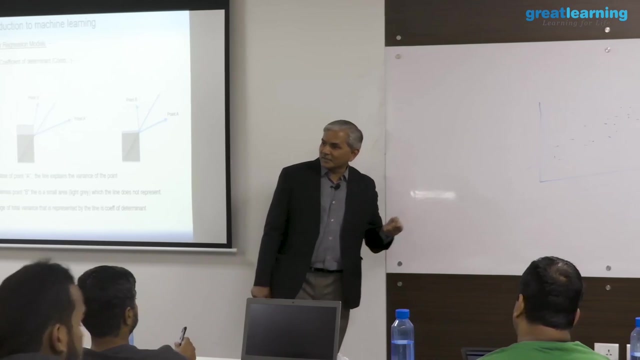 independent dimension and see what is the R value. R value coefficient of correlation comes into play to help you identify good predictors, given the target. Ok, Once you build the model, I want to see how good the model is, how reliable the model is For that. 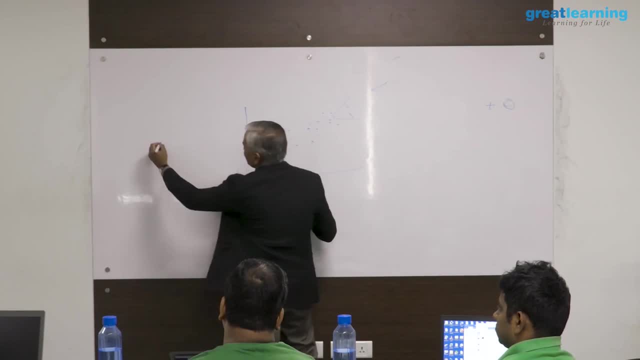 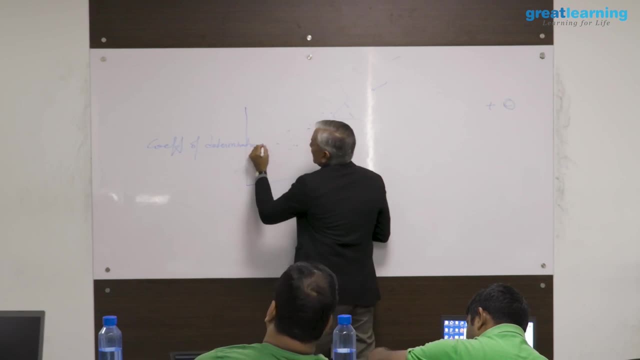 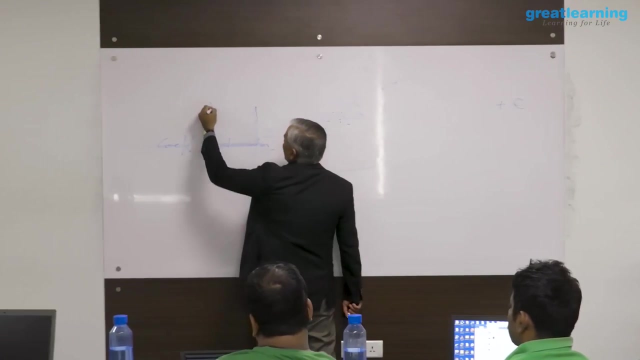 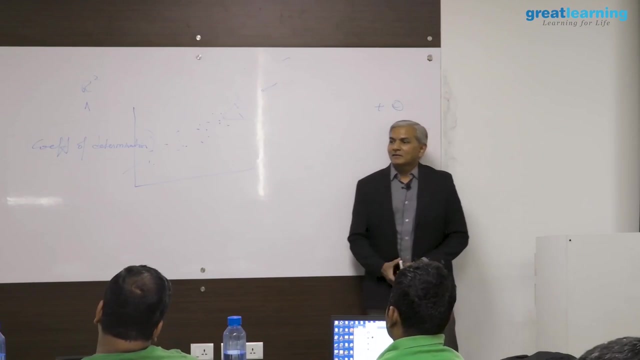 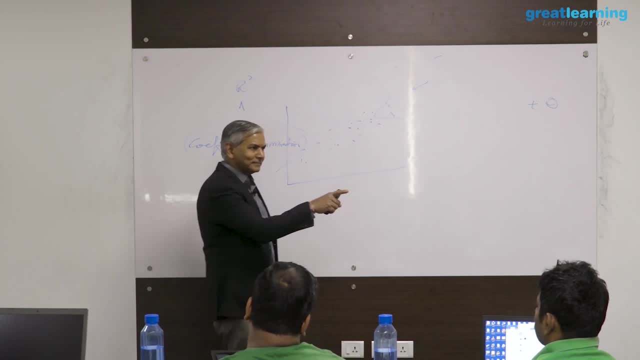 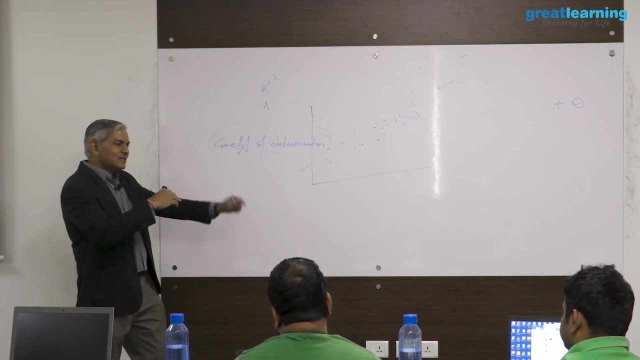 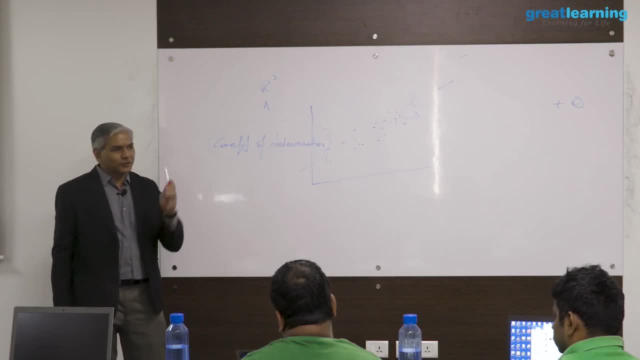 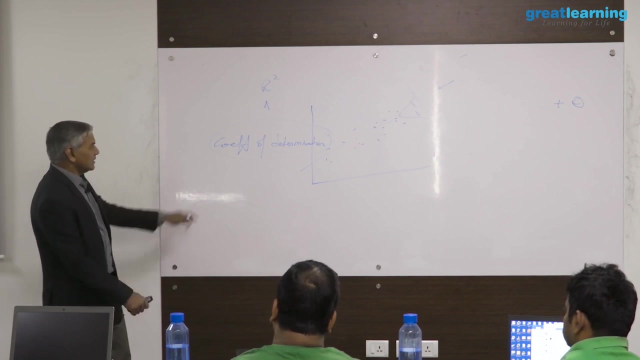 model between one dimension and one target. It is only true at that point In multidimensional, multivariate analysis where you have more than 2, 3 dimensions, you cannot say: R square is R into r. Ok, So R square is just a symbol which represents another metric called Newton's. 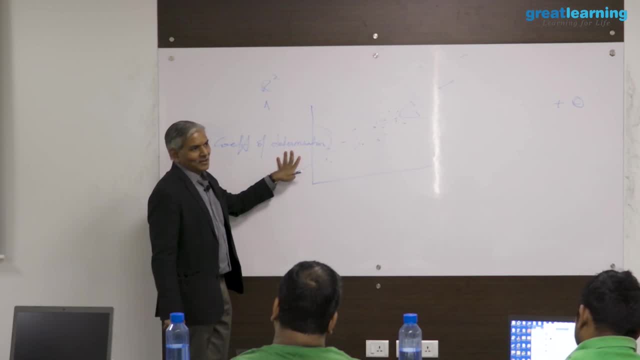 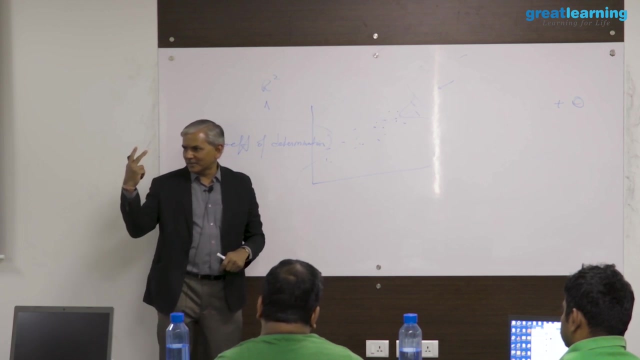 another metric called coefficient of determination: How much of the total variance in your y has been explained by your model? Keep in mind the total variance in y is consisting of two components: deterministic, non-deterministic, stochastic, random. How much of this total? 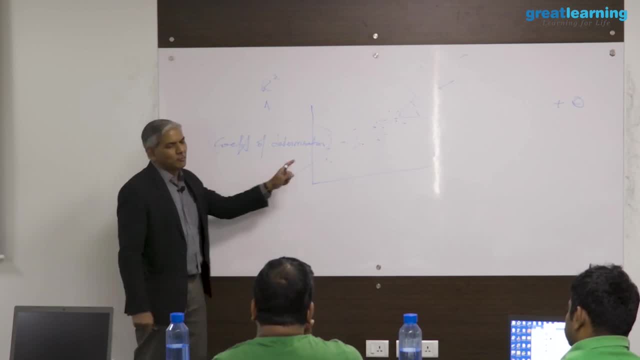 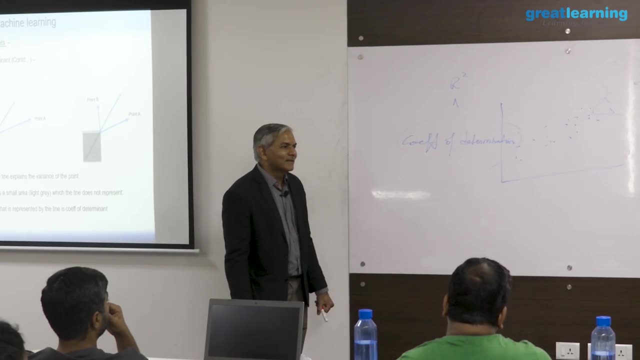 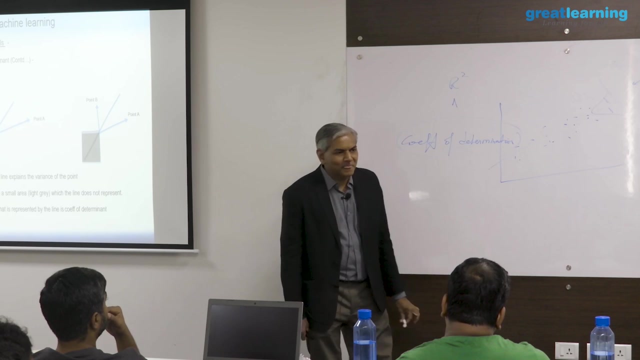 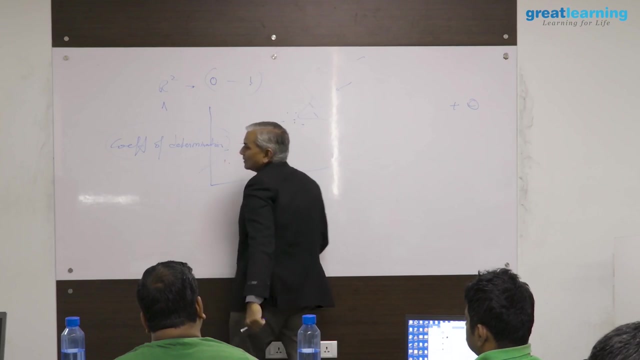 variance in your y has been explained by your model. That measure is called coefficient of determination. Obviously, a model which captures explains maximal of the variance in y. it leaves behind very small residuals. that model is the best one. So r square, it ranges between 0 and 1.. 0 means your model is not able to explain. anything Absolutely zero. 0 means it is useless. 1 means your model is able to completely explain all the variance in your target. there is no residual. Such models don't exist. You can never build such models. Usually, r value will be between 0 and 1.. The closer they are to 1, the better. 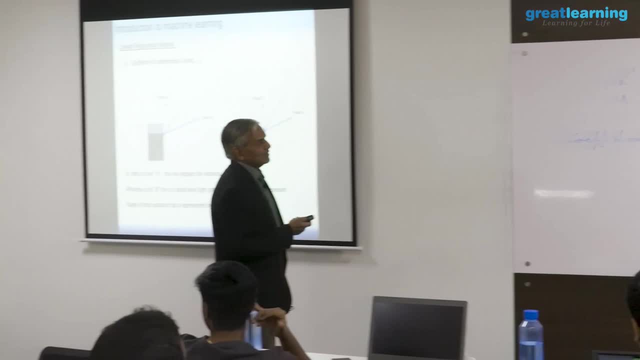 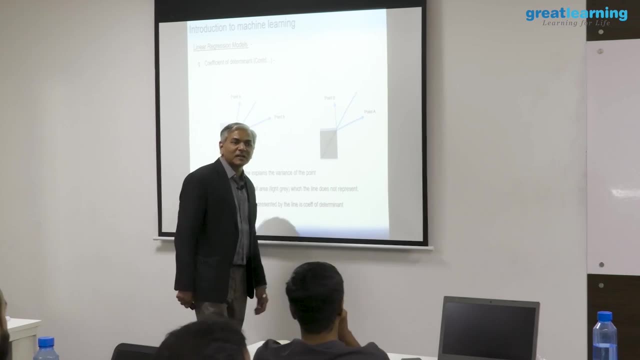 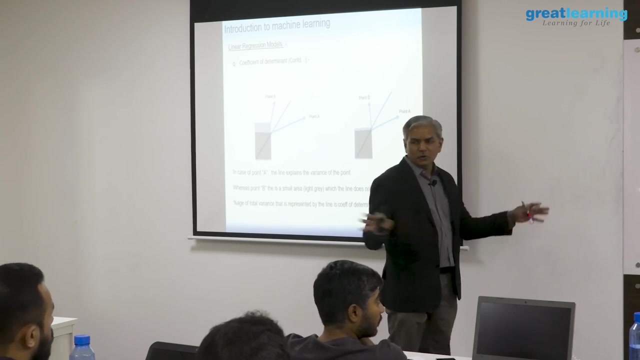 the model is Because in simple linear models, its square term, it can never be negative. But keep in mind, in multivariate analysis, analysis it is not just a square cup, it is something more than that. So it will always range between 0 and 1.. Are you all ok? 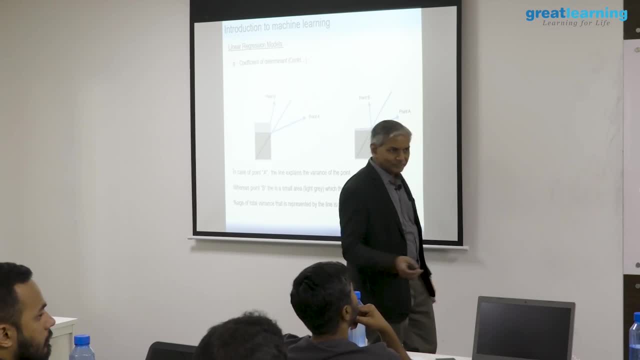 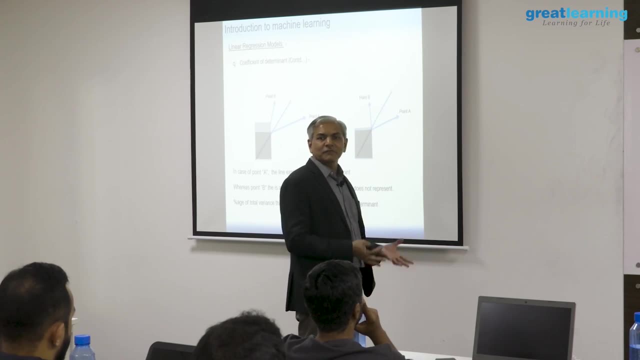 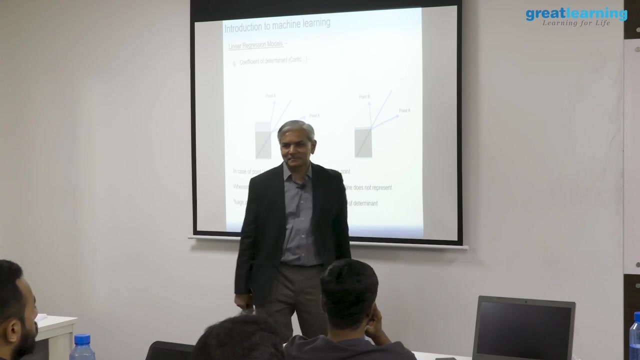 How much? how much variance in y may play If, say, this is R 8. That means your model is able to explain 80 percent of the total variance in your y, total variance which includes stochastic and deterministic right. So your R square should be as close. 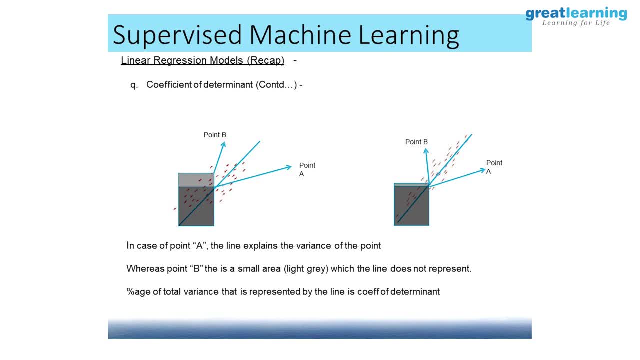 as possible to 1,, your model will be good. So this metric is used to evaluate the performance of the model, while R is a metric which is used to evaluate the independent dimensions when you are building the model Geometrically. if you take one simple linear model of one x and one y, that is what I am. 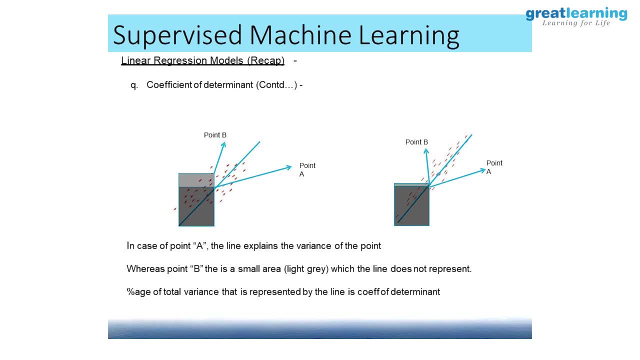 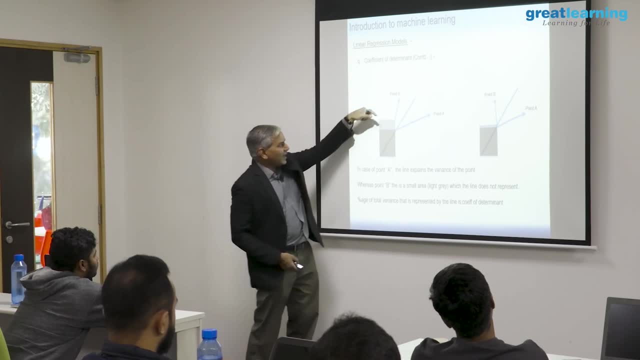 showing here. So this is where your x bar and y bar meet. Please look at this carefully. This is my y bar. this is my x bar. ok, So there is an actual data point: x i minus x bar is this: y i minus y bar is this: 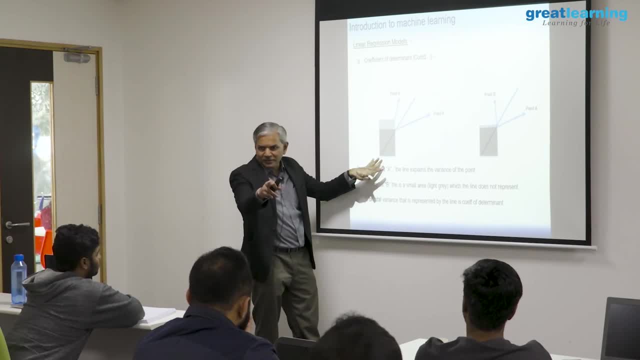 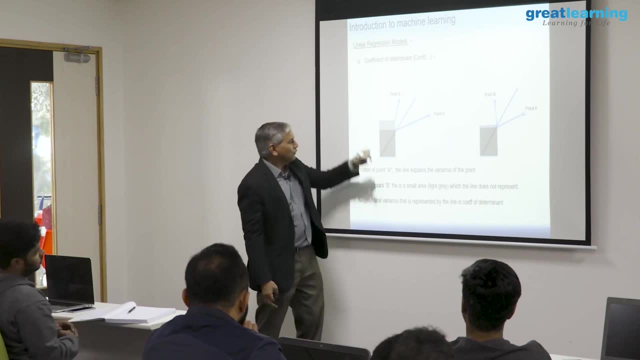 That gives us an area rectangle. we saw that earlier right. That area represents the total variance in your data point, The total variance in this data point, the covariance in this data point because of x and y. this is that area, the light grey area. 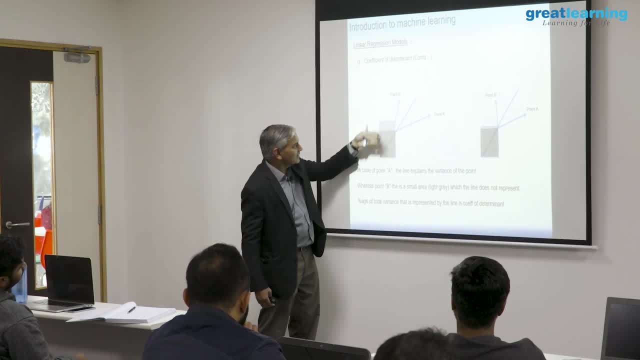 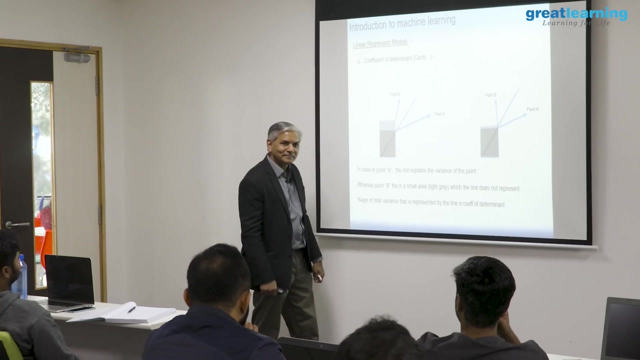 The light grey area is this: it is behind this dark grey. the light grey area is this: That light grey area is a geometric representation of the total variance because of x and because of y in this data point. Of this total variance for a given value of x, your model is predicting a value of 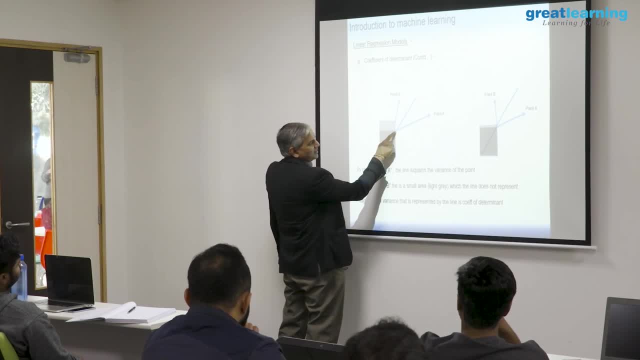 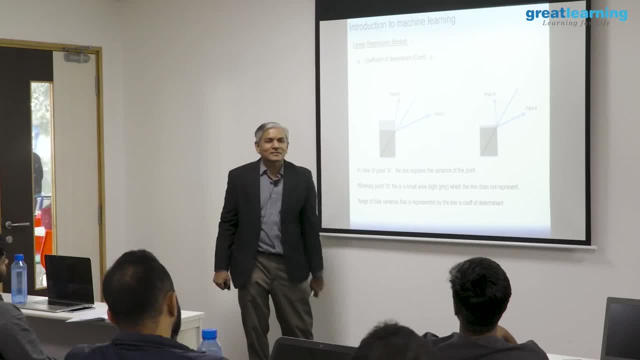 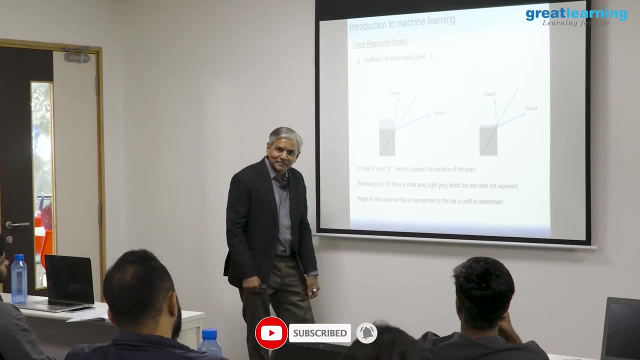 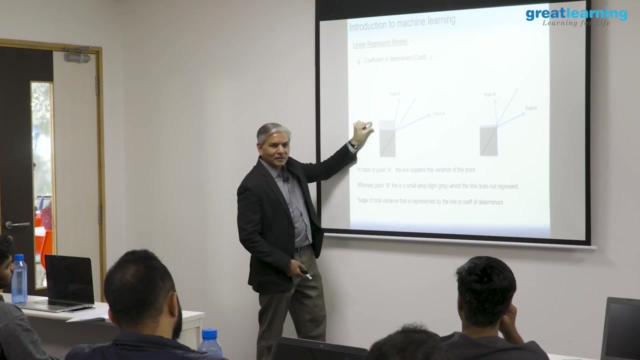 This dark area is the explained variance. How much of this total variance has been explained? captured by your model R square is the ratio of the dark area to light area. What you are seeing on the top, this is the residuals, unexplained variance. 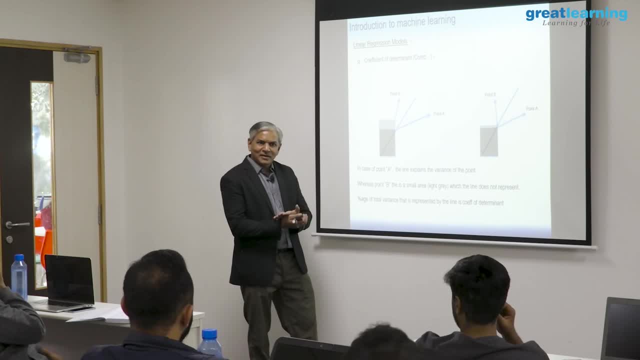 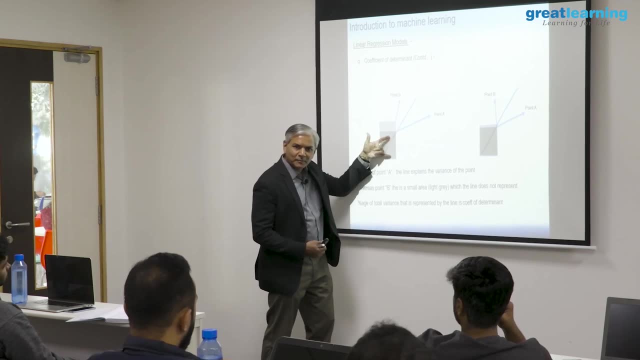 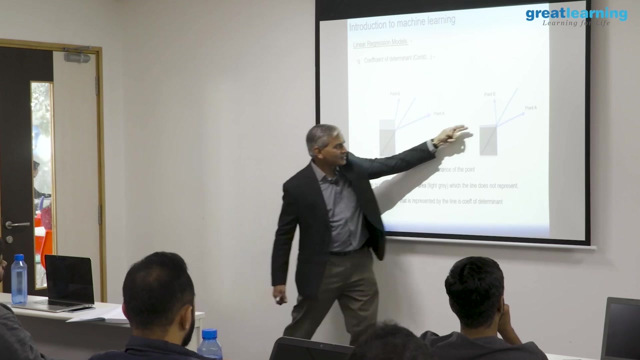 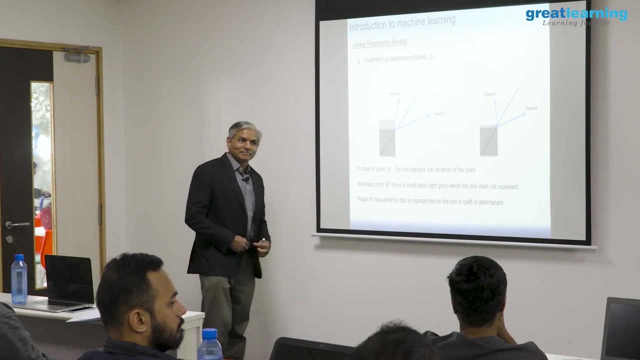 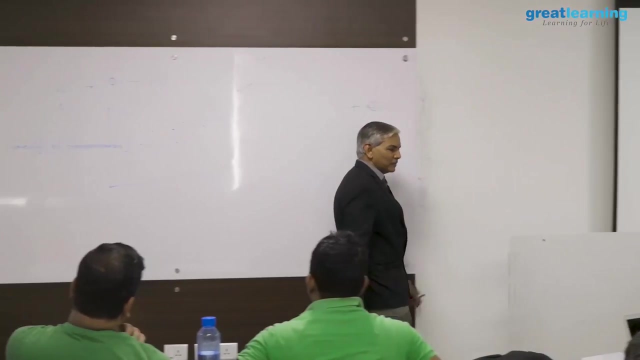 So r square is again a ratio where the ratio is between the two. So the ratio is between the total variance in the data points and the variance explained by your model. That ratio is called r square. Obviously, the lesser the residuals unexplained variance, the better the model is. 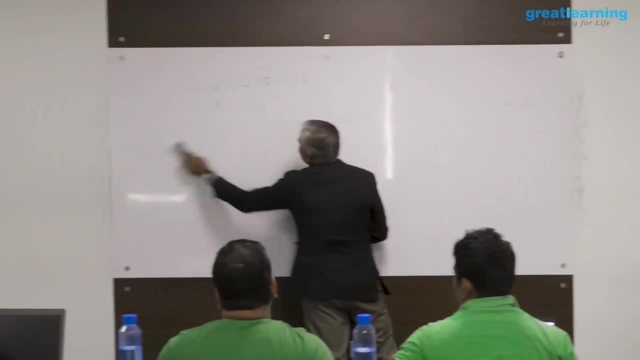 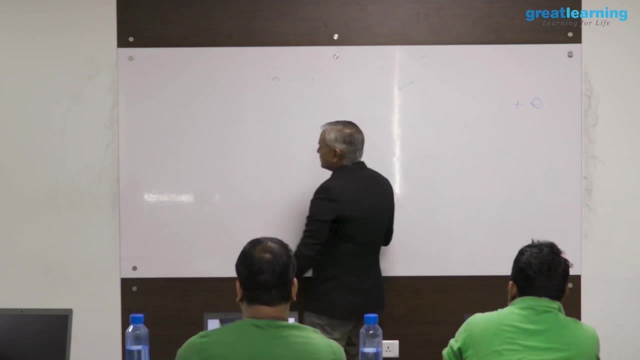 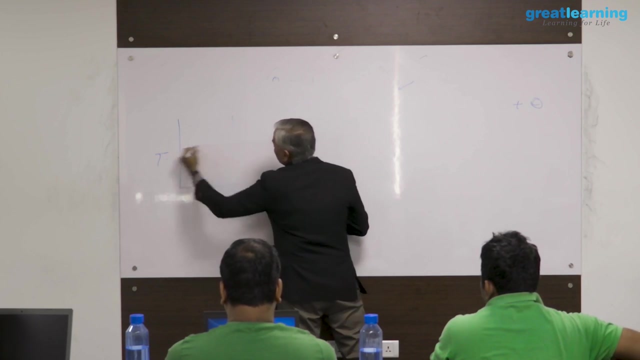 We want more r square actually. Yes, exactly. The problem is go back to our discussion on r, where I told you: if there is no relationship between these two- the target and the independent variable- you have to give, get a perfect. 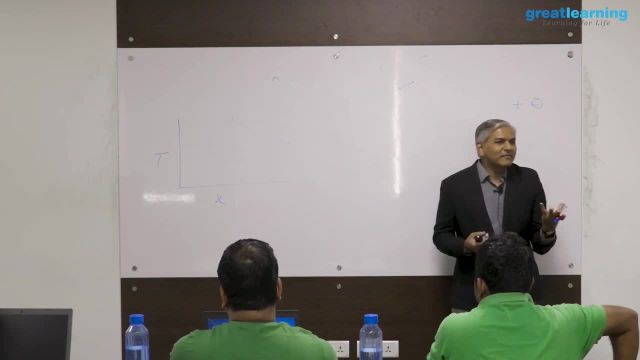 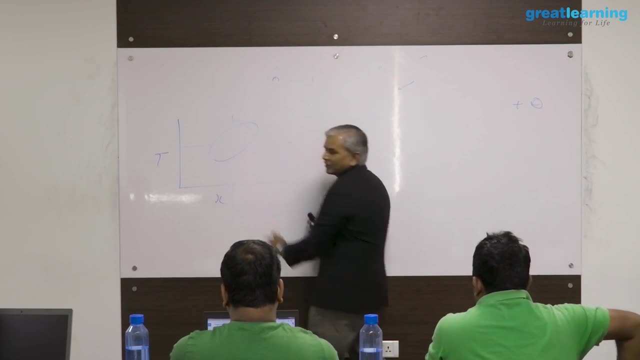 symmetrical distribution. But the probability of getting a perfect symmetrical distribution is 0, which means you are going to get some asymmetrical distribution. The moment you have asymmetrical distribution, your r value will be greater than 0, magnitude this way. 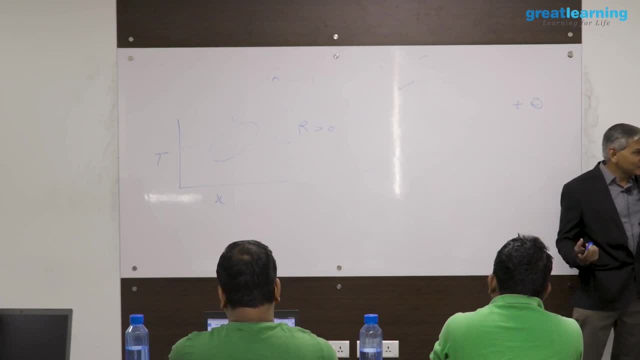 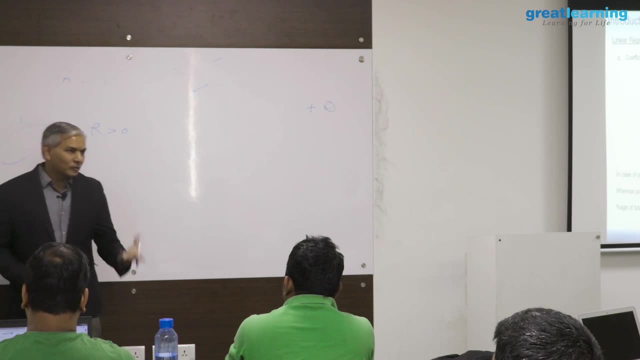 or that way, which means r square will be greater than 0.. r square is not considered as a very good metric for evaluating the models because it is easily impacted by fluke relationship, So we make use of another metric that is called adjusted r square, which is nothing. 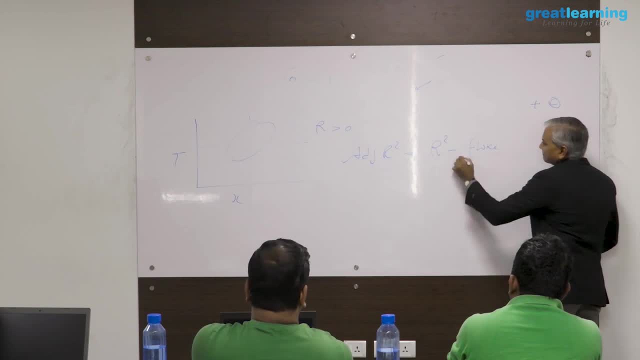 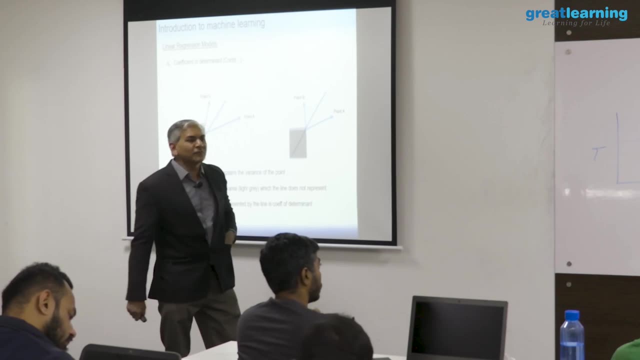 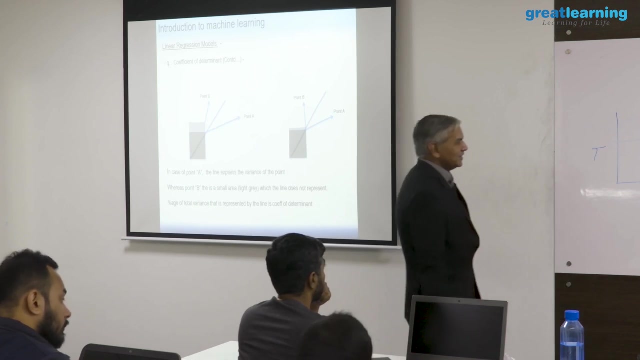 but r square minus fluke. There is a formula for this. how do you find out the fluke content, which I am going to avoid right now because it is too detailed to discuss. In case you are interested, let me know I can share it with you. Conceptually, it is easy to understand. 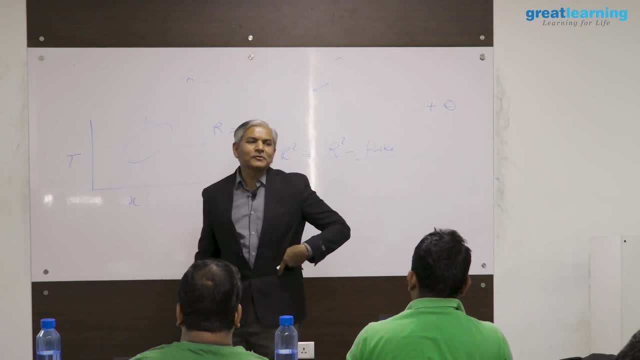 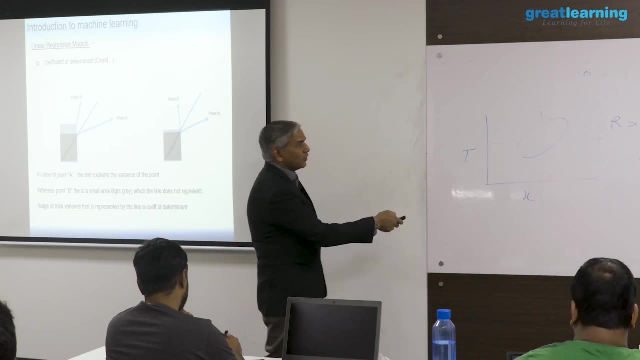 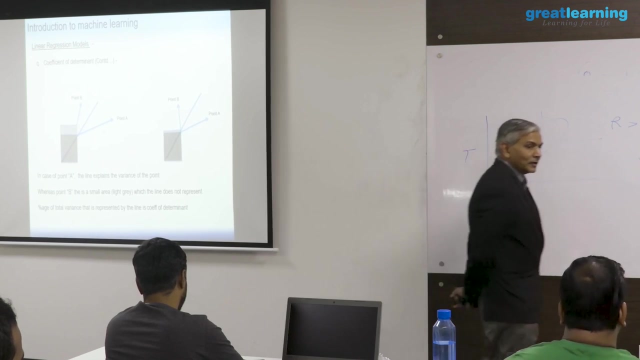 but the argument is very lengthy. We will not have time for that. that is why I am going to ignore it right now. So the metric that we will make use of To evaluate our models is adjusted r square, not r square. 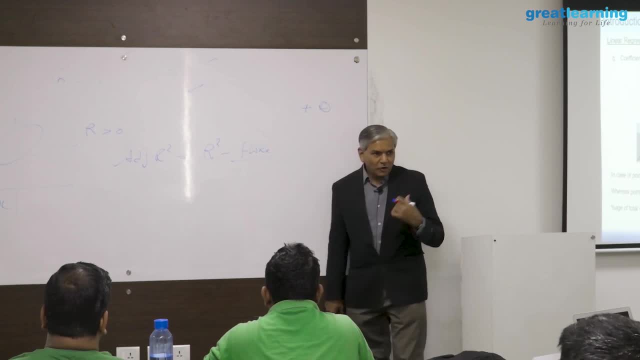 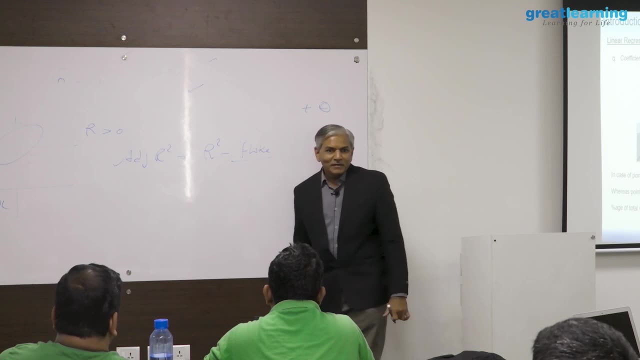 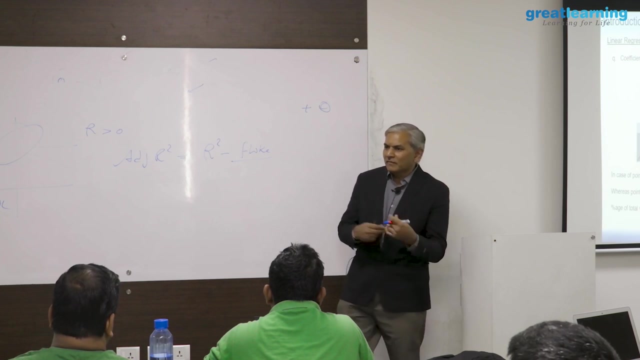 The beauty of adjusted r square is whenever, in your model building exercise to predict your target, when you include useless variables, variables which do not really have any significant impact on the target But their relationship is statistical fluke. When you use such useless variables, r square 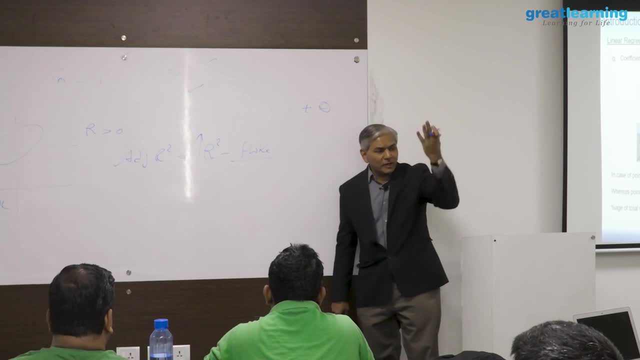 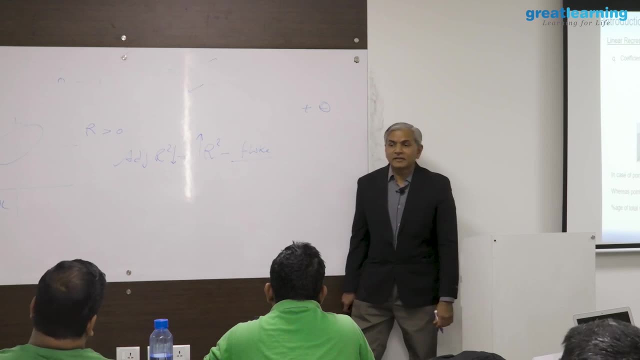 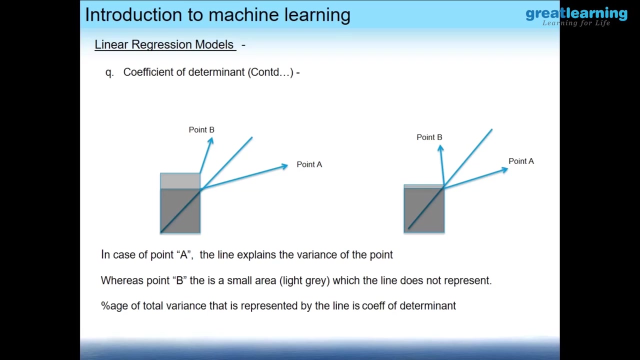 will keep on going up and up and up it will become. it will come closer and closer to one. But adjusted r square will go down, it will decrease. So when you include useless variables in your model, adjusted r square will go down, it will reduce, whereas r square is likely. 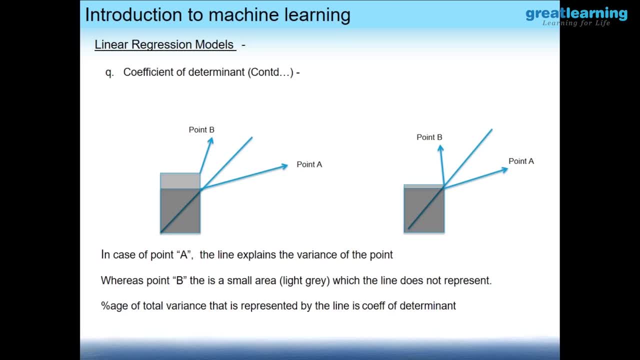 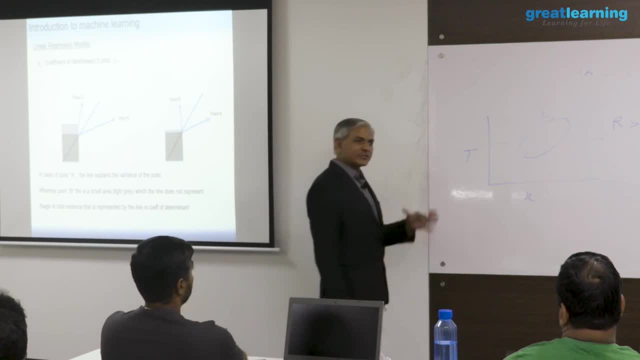 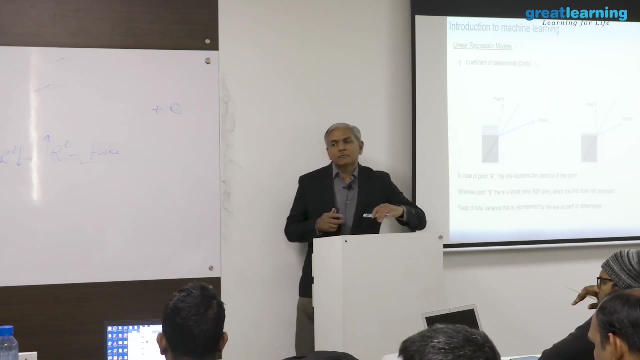 to go up. Adjusted r square will go up only when you include good variables in your models. Good variables are variables whose relationship is significant, strong. So we use adjusted r square for evaluating our models. One thing that you need to keep in mind conceptually: 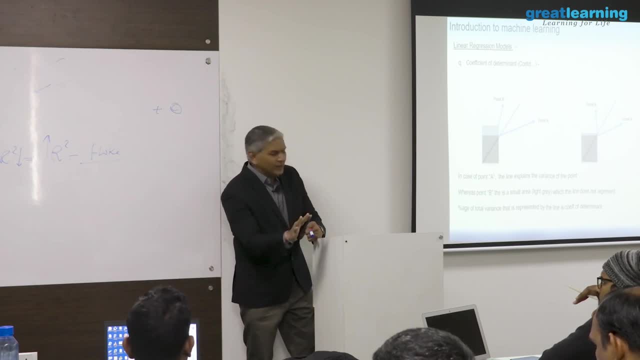 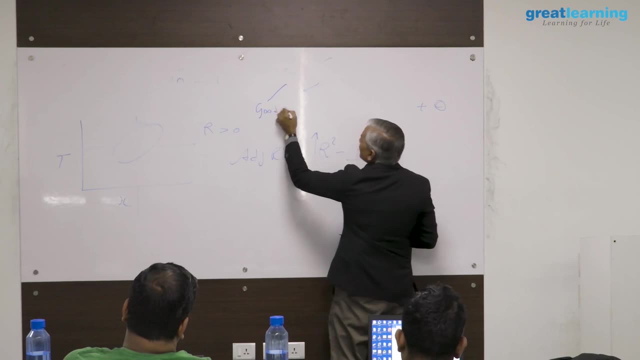 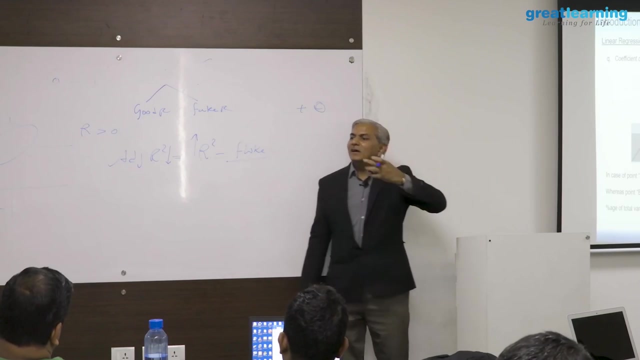 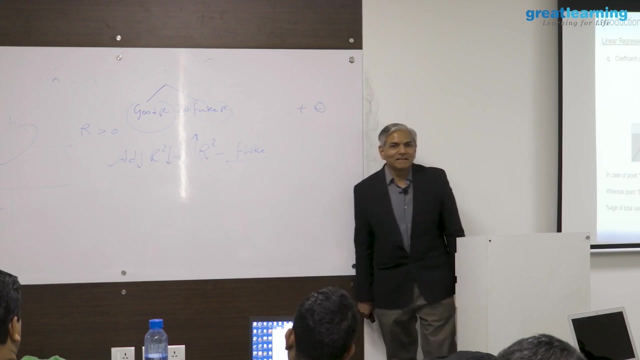 get it clear: any attribute that you use in your model building, any attribute, that attribute will always have both the components, good and bad. It will always have both the components. good r and fake r. It will have both the components. But in good attribute the percentage of this will be very, very high compared to this In. 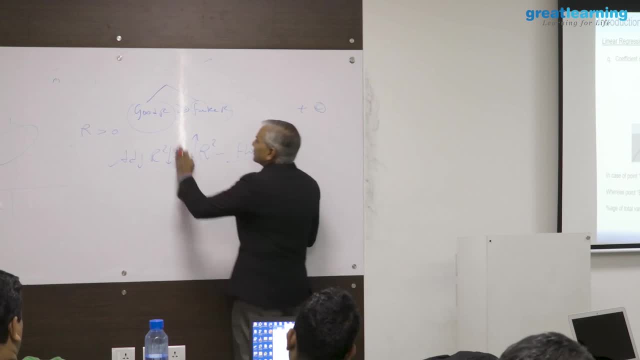 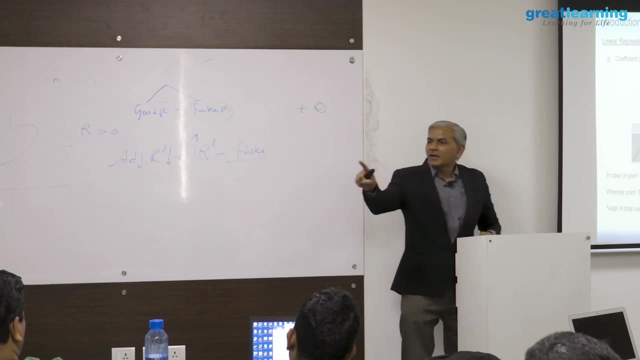 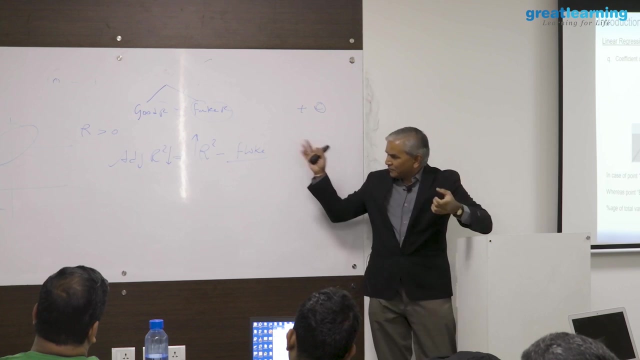 a poor attribute, useless attribute, percentage of this and this will be almost similar. That is why, when always it is the same 자, then always, in every basis we think about good, or R value is close to say 0.5, 0.6, part of it will be caused by fake R, part of will be. 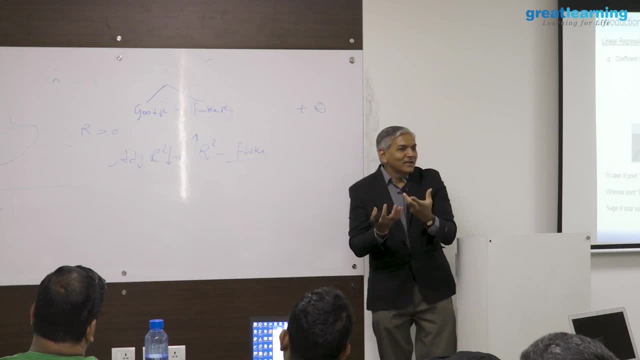 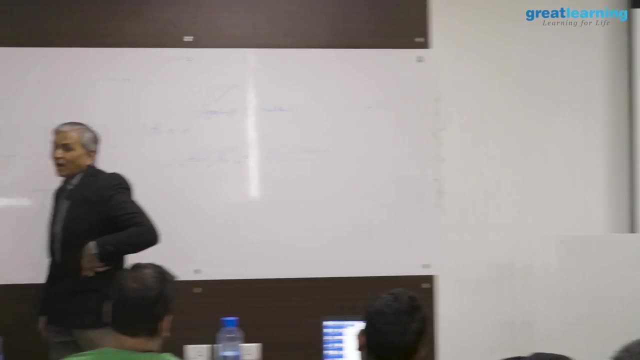 real R? how much is real? how much is fake? I don't know. that's why it calls for further investigation before you decide to use that in your model. When R is close to 0.5, 0.4, 0.3- we don't know what- how much of that is fake? how much? 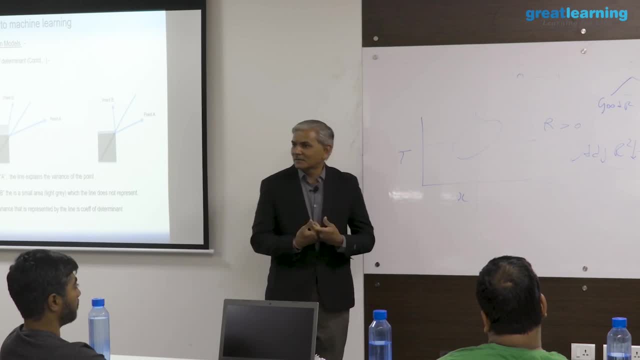 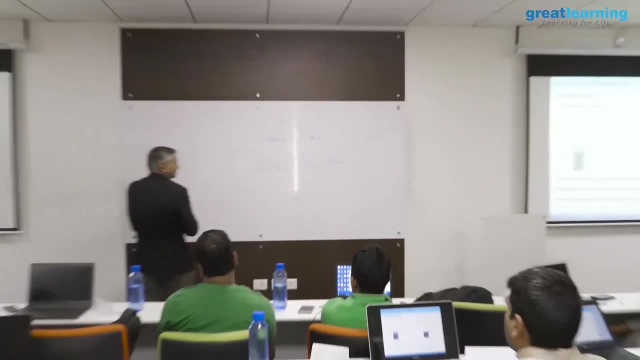 of that is real? we don't know. that's why you need to further investigate Before we include or exclude, how we get the explainability of the fake. what is actually causing fake Randomness in the? your sampling techniques itself will bring in fake. 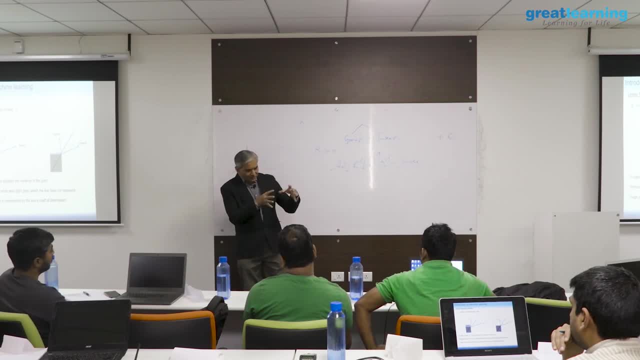 When you use random function to sample from population. since he asked this question, whenever you do sampling, any technique- you use clustering, layered sampling, mixed sampling. whatever you do, your sample will never be a true representation of the real population. 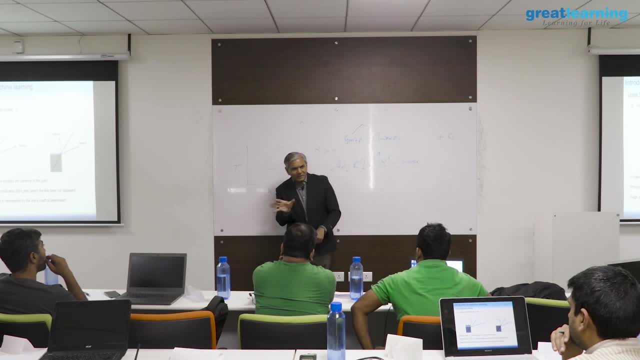 it will never be. So it's distributions will be slightly different from the distributions in the population. That change in distribution is what will introduce fake R. So only if sampling which introduces fake Sampling, sampling is the source of this. Ok. 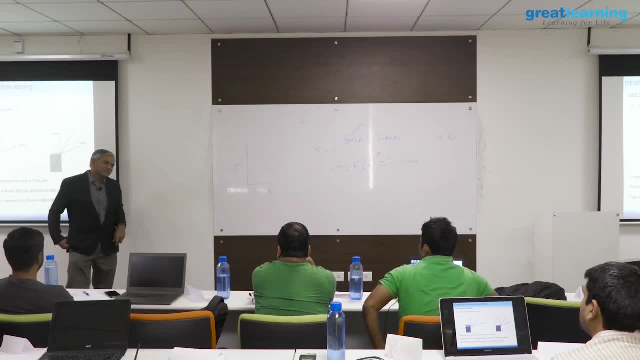 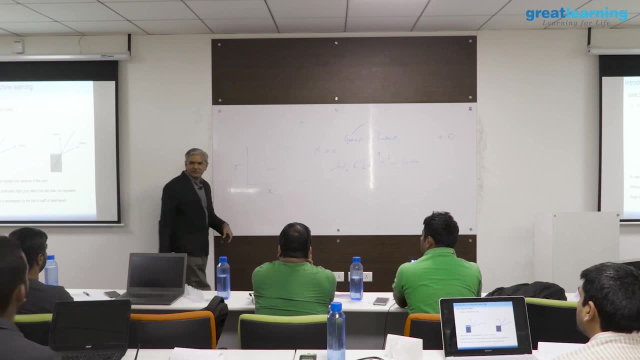 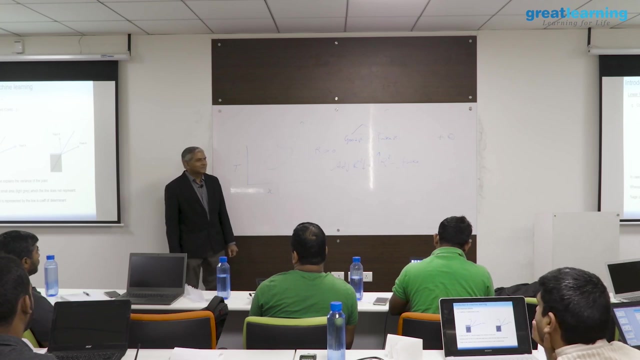 Right? Did I show you that video where I showed you universe to be under flux, continuously changing. it's never static, whereas your sample is a snapshot Offering in the video? I am just taking you through the concepts. I am not telling you why. what is the formula? 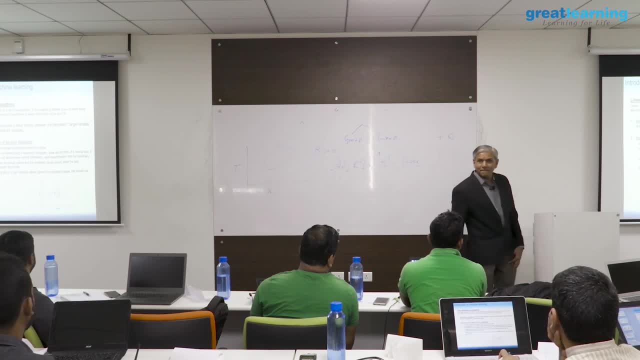 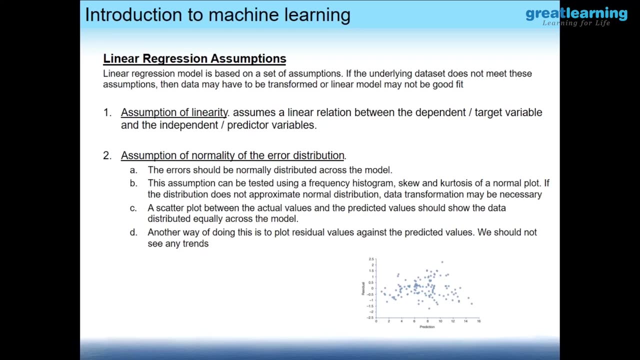 for all these things. they will become too heavy for you right now, But I will eventually take you through, in case you are interested, Some assumptions that this linear regression models make. we already discussed this assumption of linearity. The relationship between the target and the independent variables are expected to be linear. 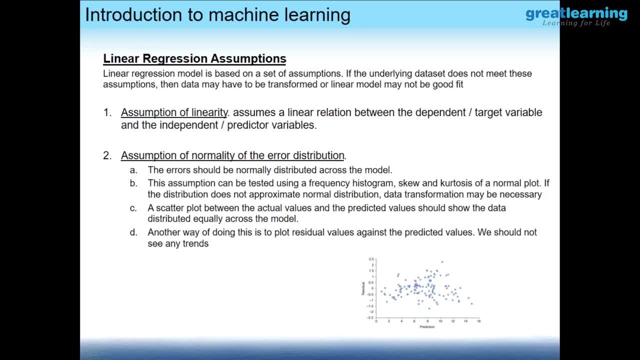 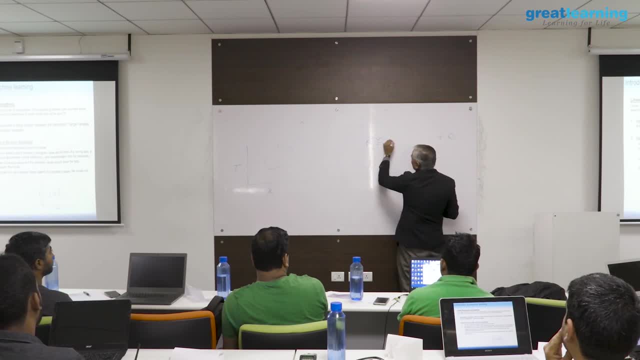 Oh, that brings me to another point. Please be careful when your R value is close to 0,. what does it mean? Ok, I think that is what I ended up saying: There is no linear relationship between x and y. 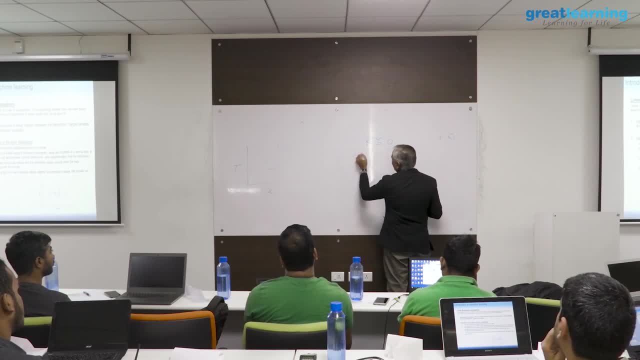 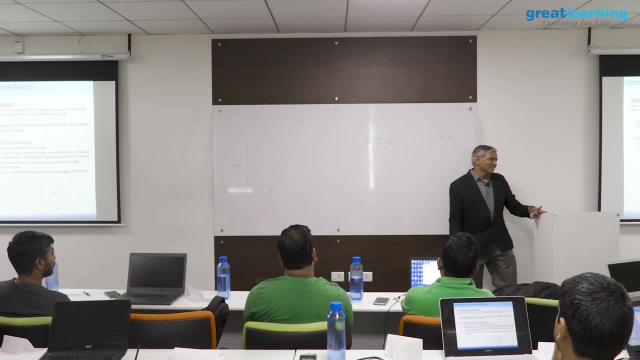 Ok. When R value is close to 0 between y and x, that means there is no linear relationship. That does not mean there is no relationship. For example, if I give you a distribution like this: this is x and this is y and this. 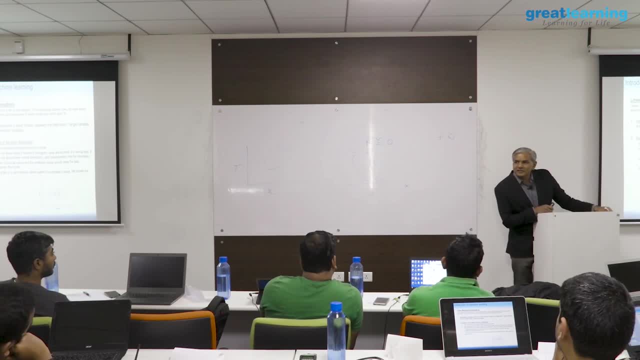 is parabolic. There is no linear relationship. When you find R value for this distribution, it will come close to 0. But they are related. There is non-linear relationships. So whenever you do this analysis, R value is close to 0.. 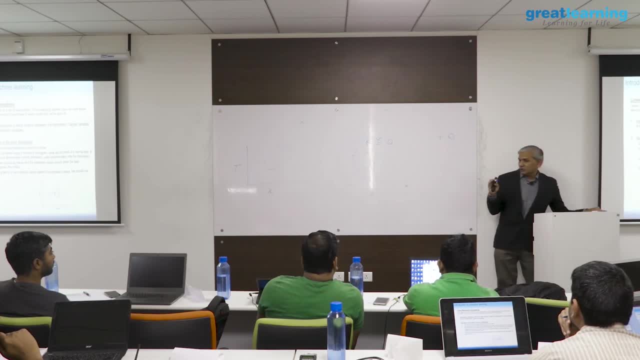 Ok, So this is a non-linear relationship. Whenever you do this analysis, R value is close to 0, go back and check your pair panels, pair plots: Is the relationship non-linear? If the relationship is non-linear and you are building a linear model on that, you are. 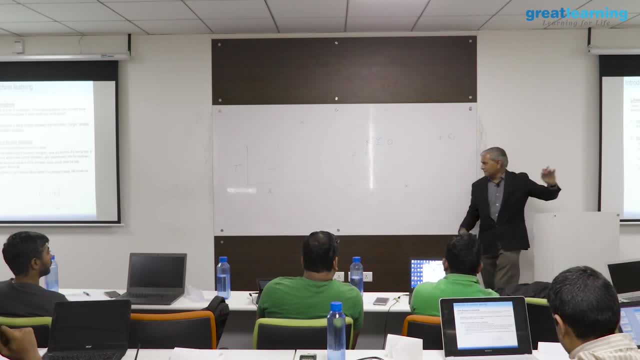 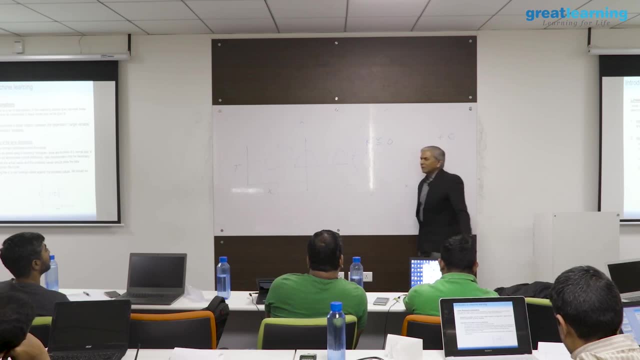 doing a mistake, a fundamental mistake. Ok, Same way, if you have a distribution like this, R value will come to 0.. But there is a relationship between y and x. A sine omega t. A is the amplitude Sine theta. you know what theta is. 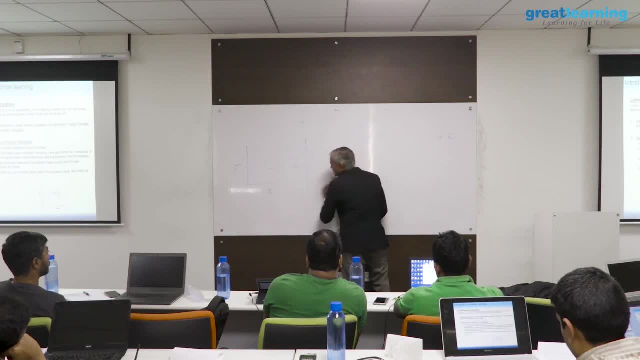 So when R value is close to 0, that does not mean there is no relationship. It means there is no linear relationship. If you have such attributes in your data set, then you may have to think twice before you use linear models. 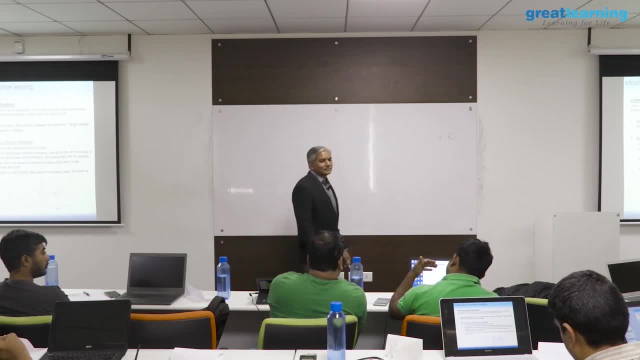 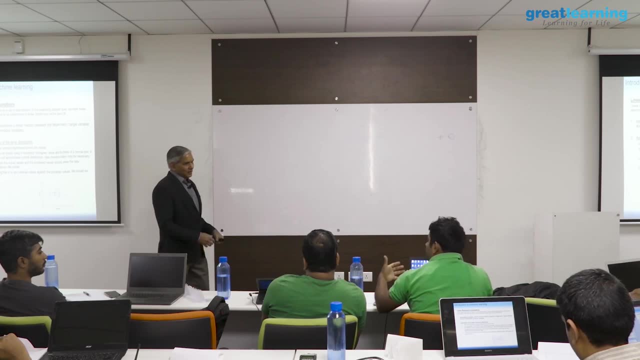 So unless we draw this pair plot, we will not come to know that we have this kind of non-linear relationship. Ok, So is it always suggestible to draw pair plot for each 100 percent? If you ask me, I will always say: pair plot is the most important tool you have in your 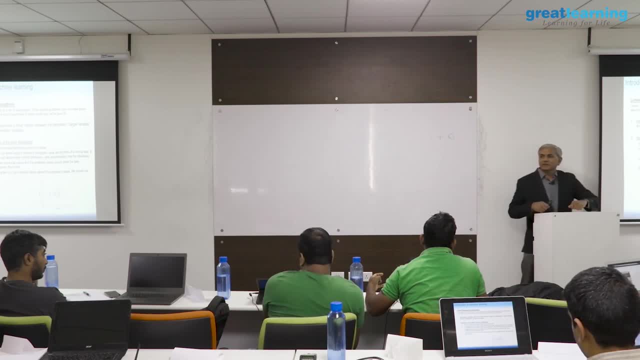 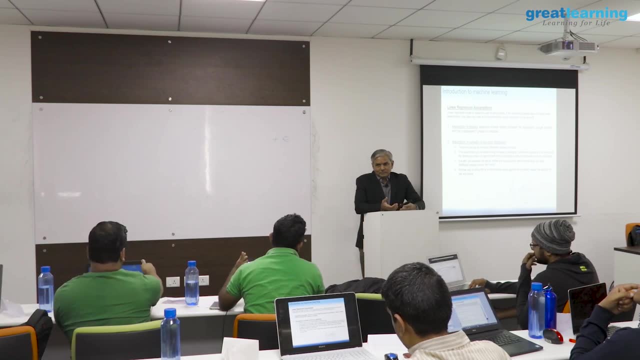 toolbox which you should use to understand your data And suppose we got some pair plots. we should not try those attributes for the model. Try different models may be a non-linear model. Ok, So now that brings me to a question: what is linear and what is non-linear? 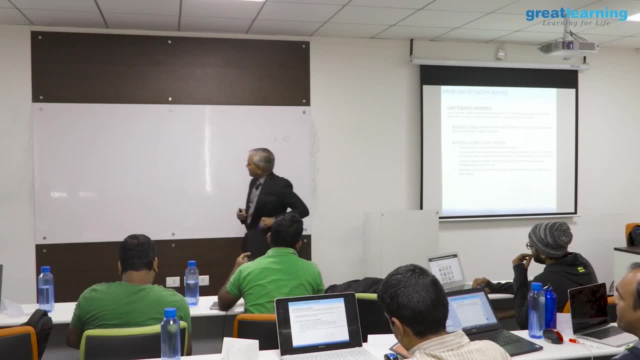 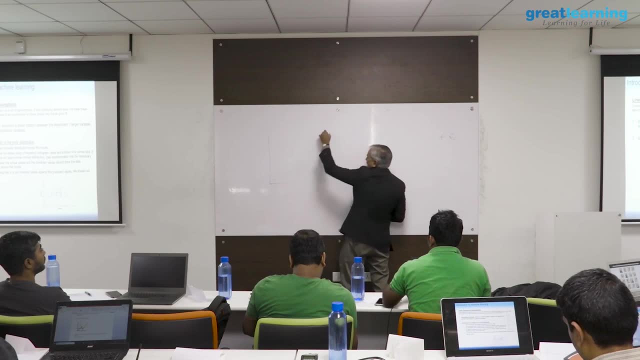 Ok, Now look at this. This is slightly funny and, at the same time, something which is actually serious. This y and x. mathematicians will say: suppose this is x, this is y and the expression is: y is equal to x square. 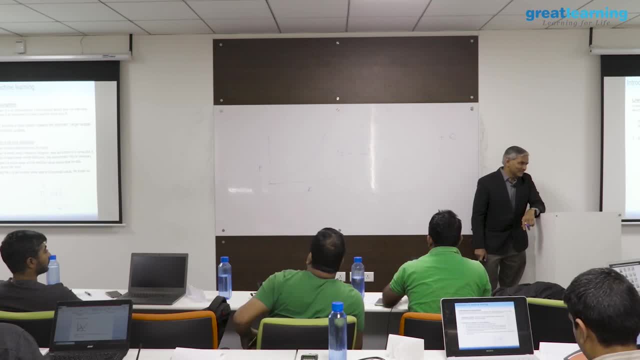 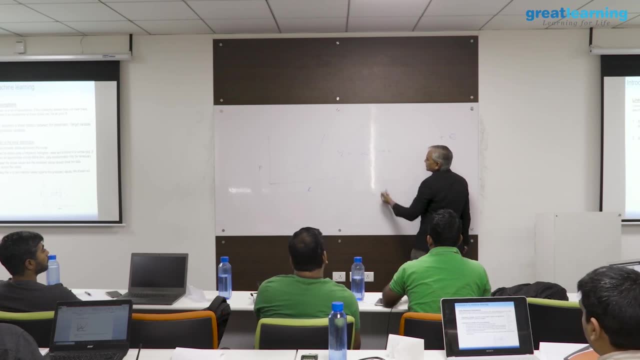 Mathematicians will say this is a non-linear function. Data scientists call this linear function. Ok, What? We can replace this with some value, k. so y is equal to k. So I can convert this into a linear and then build linear models on this. 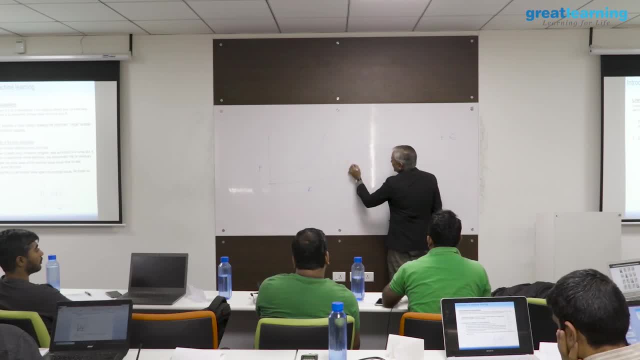 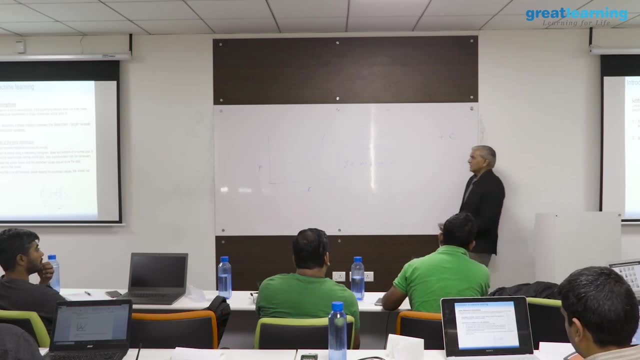 So when you build linear models, y equal to m, x plus c- the reason why they are called linear models is these coefficients: they are not raised to the power, they are raised to the power 1. That is why they are called linear. 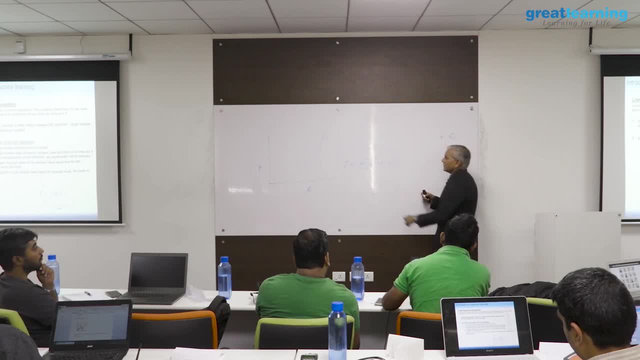 They are linear in terms of coefficients. If I have a model like this- y equal to m, x square plus c, for us it is a linear model, Ok, So do not get confused with this. A lot of mathematicians will say: this is not linear, but we, for us, for us in data science. 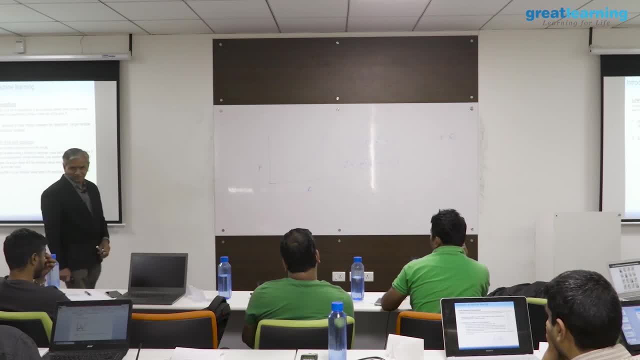 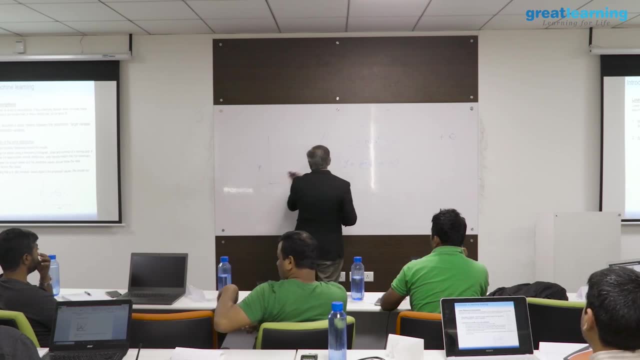 scikit-learn or R. this is a linear model. It will show us a trend. It will show us a trend, You will see. you will see that if you do an auto m p g case in auto m p g case, m p. 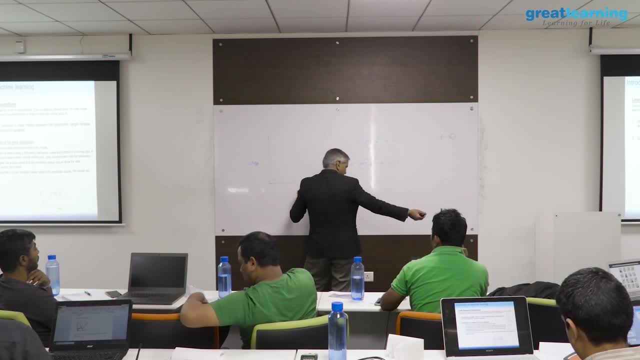 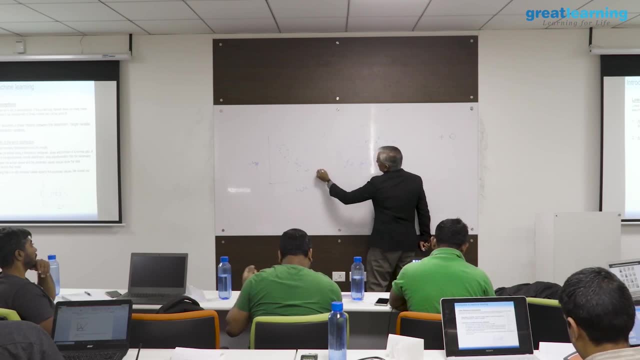 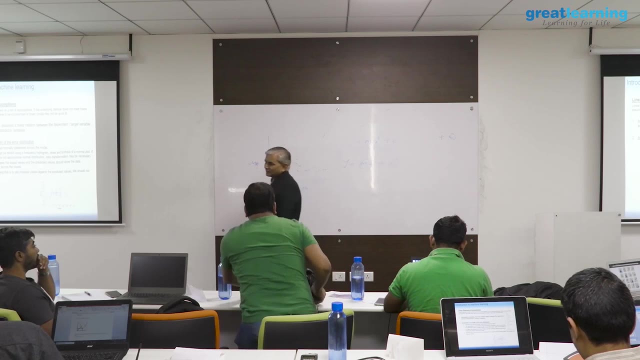 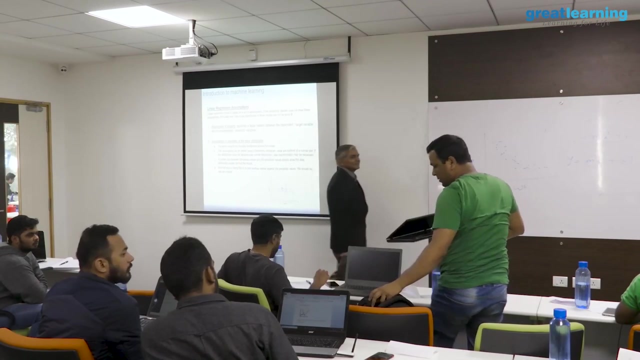 g is the target and your x is, say, weight of the car. you will see that the data points are scattered like this. You can still use linear model on this. You can still use linear model on this. Ok, So if R is close to 0 and if my scatter plot is showing quite dispersion, so in that case, 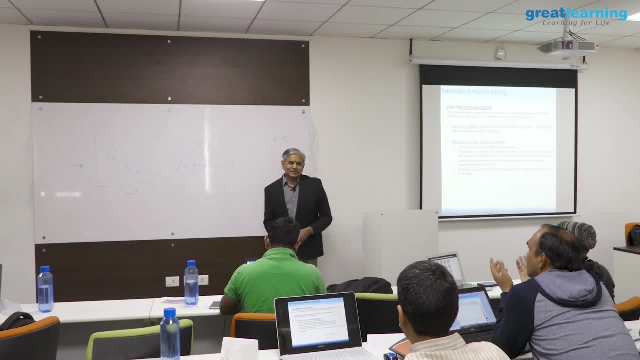 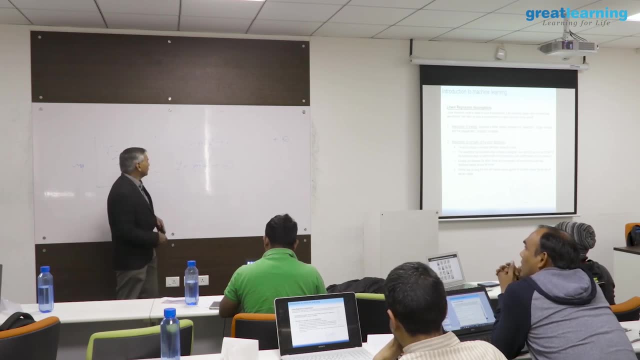 I can say it is a linear model, So I can remove it. Yes, But if R is close to 0 and if there is some parabola kind of thing, in that case Non-linear models you might have to go to. 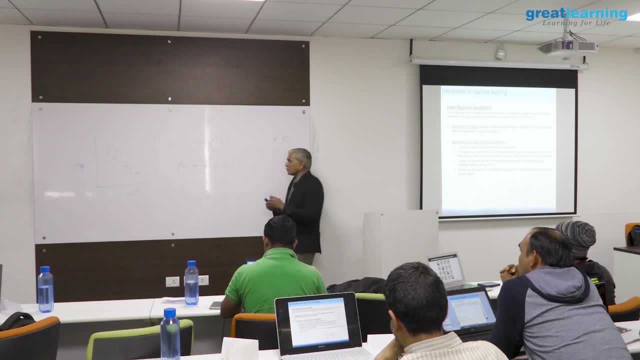 Non-linear models are models where these coefficients themselves are complex coefficients. They are not simple coefficients, They are not simple ratios. They are something like e raised to power, i, theta and all those kind of things. Ok, Ok. So if we have a in multi variable case, if one is showing linear relationship, other 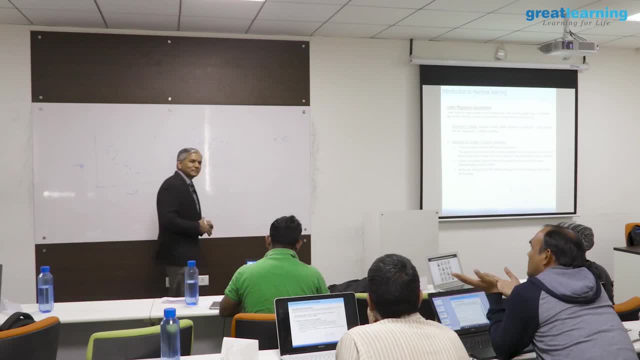 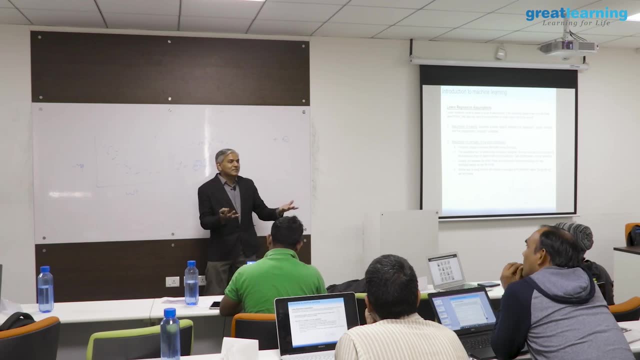 is in that case. So you will have to try both build a linear and non-linear see which generalizes Finally what is the objective Objectives? it should have minimal bias variance errors. Which one gives you that minimal bias variance error? 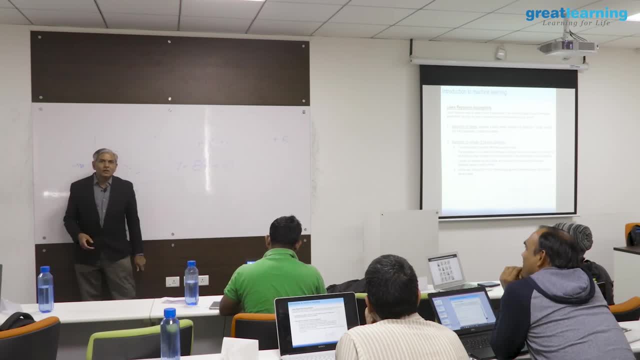 Put that in the page. Combo is what we call ensemble techniques. ensemble techniques In production. we never put one single model into play. we always put a multiple models grouped together in a play. We always install multiple models put together, Varun, good morning. No problem, sir, that's okay. Camera is facing me, not. 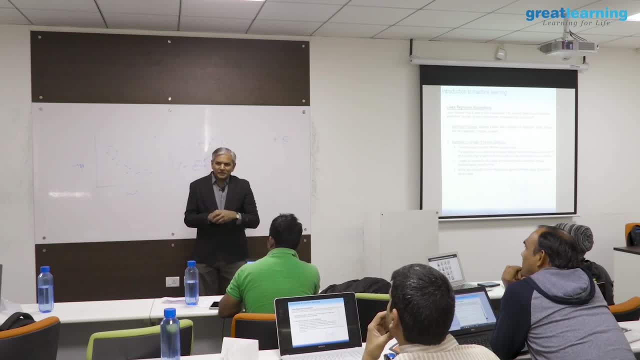 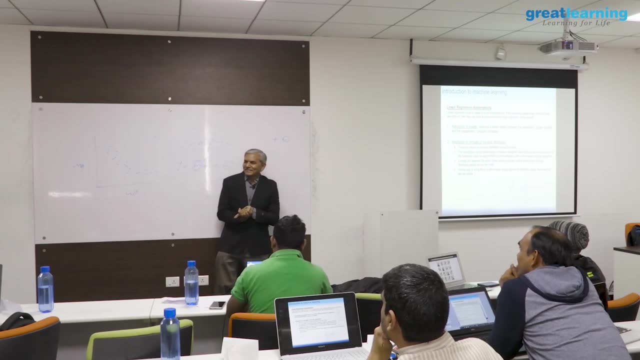 you it's okay. Okay, but don't knock the camera off here. He is also sleeping, Right. So what we do is: have you seen this Kohn-Benneger-Karotapathy? Have you noticed that the audience never go? 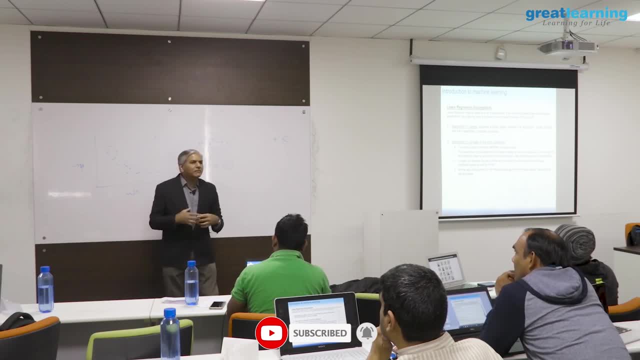 wrong. Now, the audience individually may not have very high IQ, but put together they rarely go wrong. This concept is called wisdom of the crowd. The same concept is used in data science also. when we productionize our models, we don't put one single model into play. we 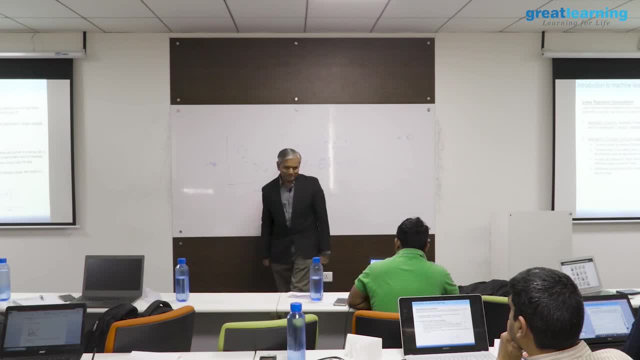 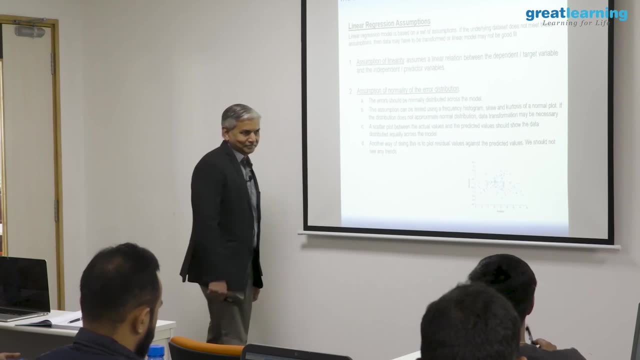 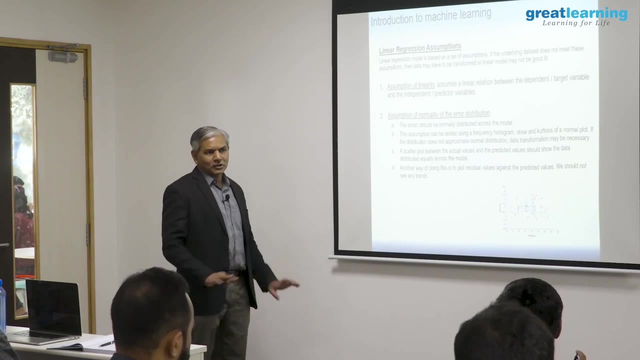 always put a collection of models into play That is called ensemble. The algorithm assumes that there is a linear relationship between independent variables and the target variable. It also assumes that there is no relationship between the independent variables. That all algorithms do. there is. 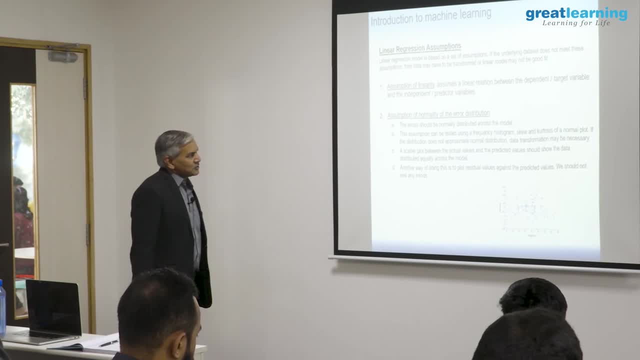 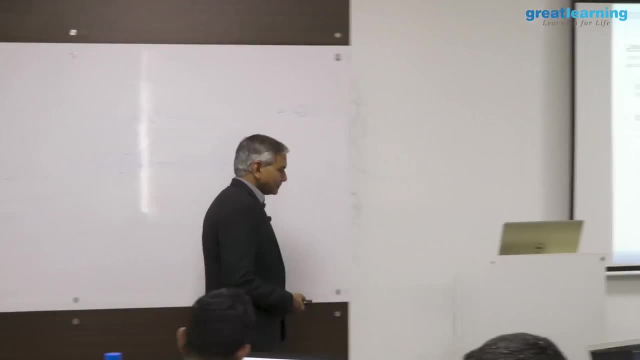 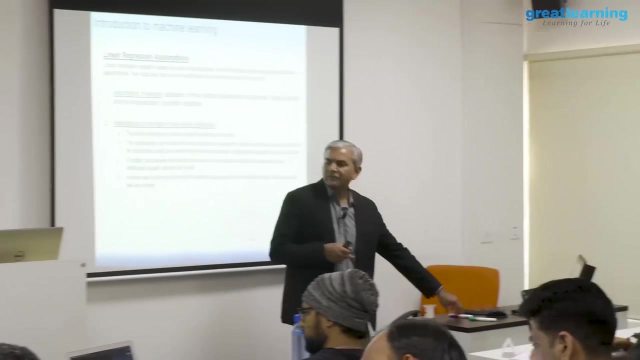 nothing particular about this algorithm. Assumption of normality of error distribution. This algorithm assumes that the model that you build, the best fit line, the best fit line, would be such that the variance around the best fit line would be equal to the variance around the best fit line. The variance around 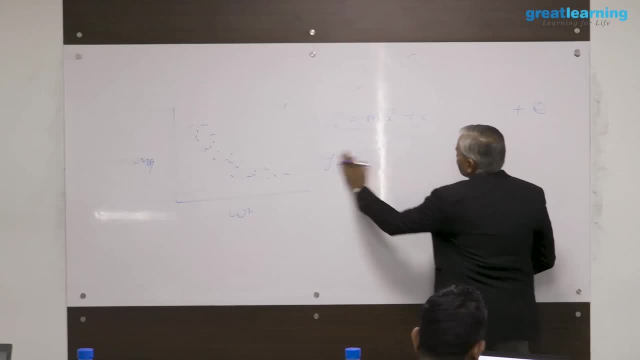 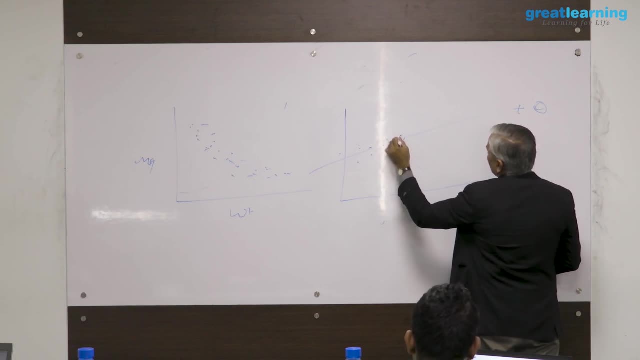 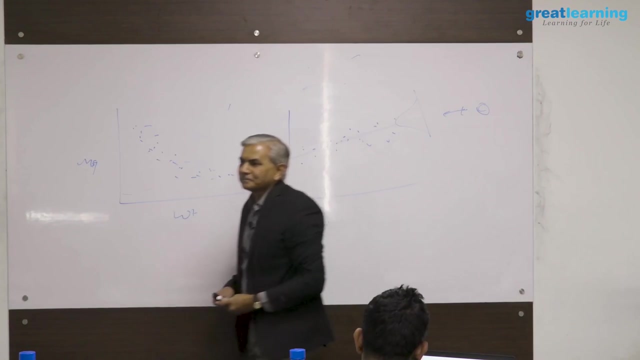 the best fit line will have last HC. that means it will have normal distribution. What do you mean by this? If this is my best fit line and the data points are scattered around this, and when you look at it from this angle, it'll have a normal distribution. This is. 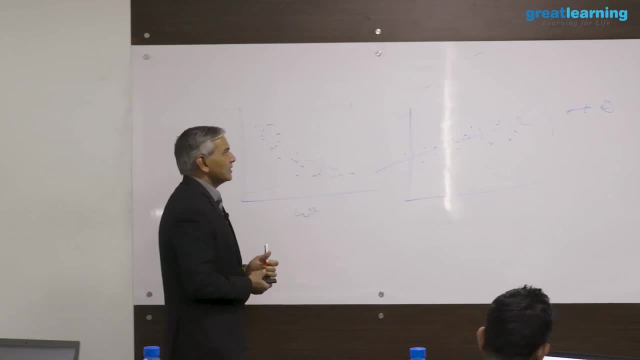 not guaranteed. Sometimes you interfere with the best fit line and the best fit line. you might see a distribution like this: More errors on the positive than on the negative. so you have the können und die universe. You simply something different. like this, otherwise you. will not understand this. as a result of this, You won't have a difference between some of the finding problems and also you will not understand this as the difference between information and some counter NH and some co skyrim, so that you will have a difference betweenInter presenting and. 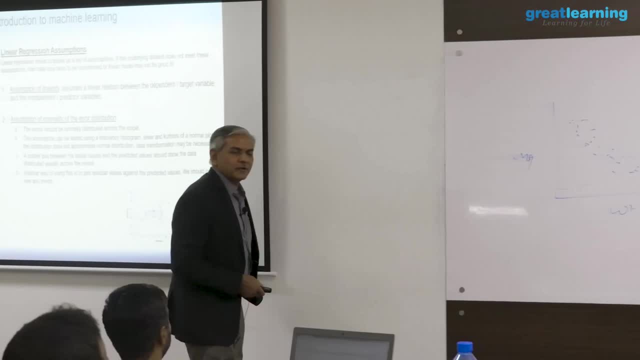 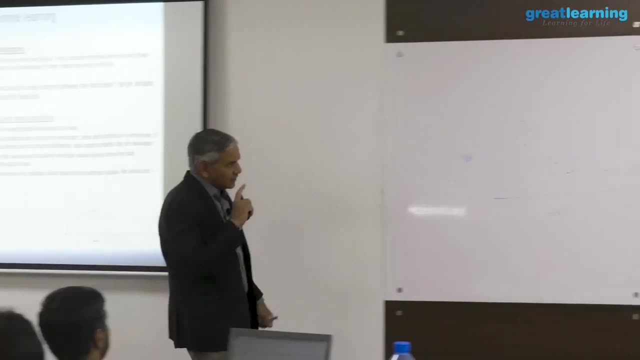 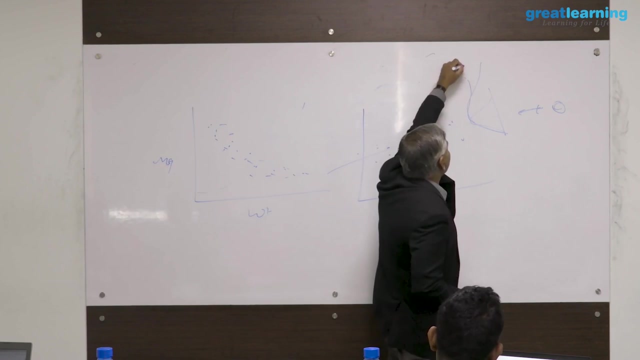 on the negative. This happens when you have outliers in your data sets. This algorithm- all algorithms- will go down on their knees when it comes to outliers, but this particular algorithm is prone to outliers If you have an outlier somewhere in your data set. the 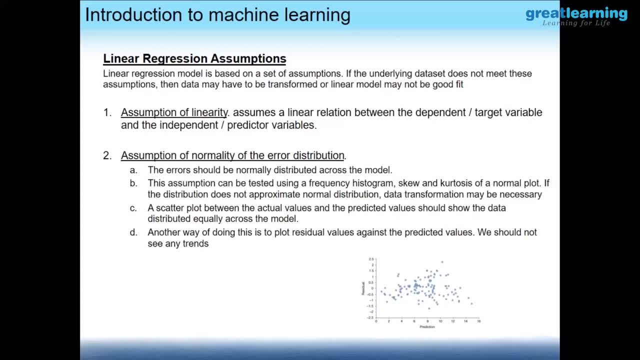 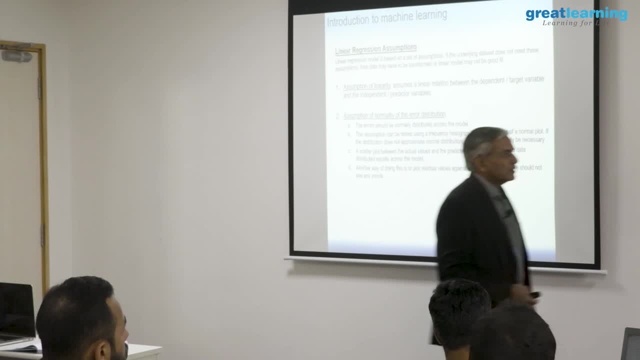 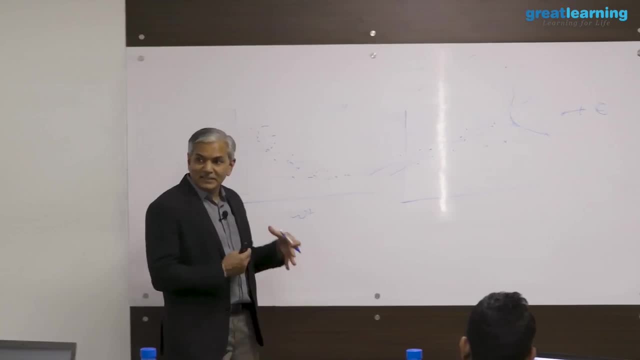 best fit line will get pulled towards that. It will get pulled towards, it will gravitate towards the outliers. So when that happens, the best fit line that you get the M and C that you get that M and C may not be the right M and C for your production, So model: 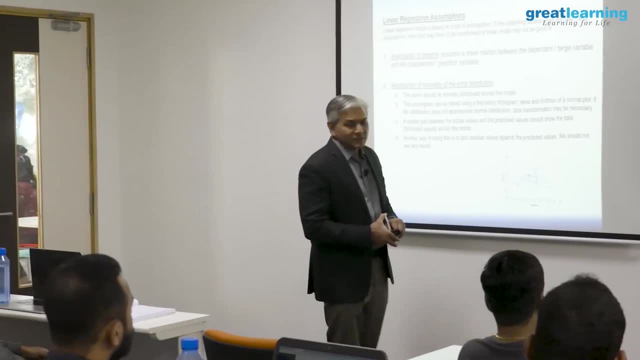 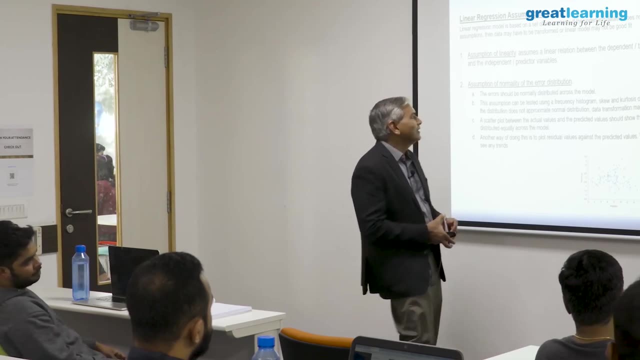 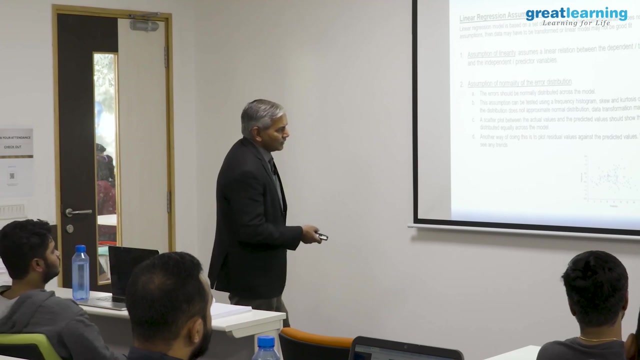 may perform poorly there. So when you build up models- linear models, any model- the first thing you have to do is handle the outliers first. There are various types of outliers. There are various ways of testing this out whether this is happening or not. One of the 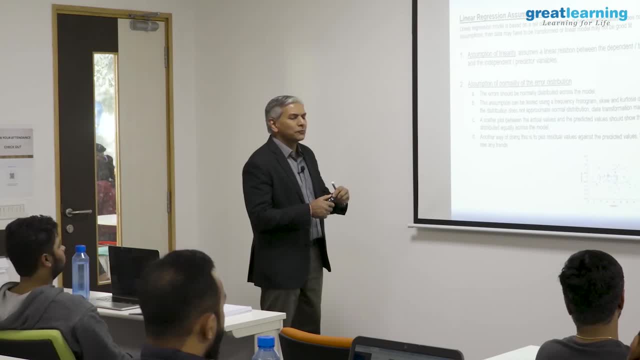 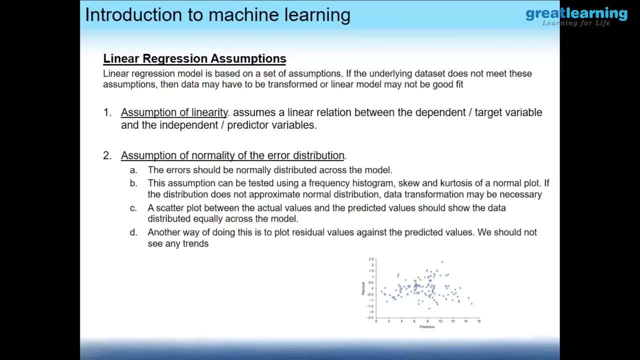 ways of testing this is you do a scatter plot between the actual values of y and predicted values of y. Between actual values of y and predicted values of y, since the data spread around the best fit line, there should be no correlation, the distribution to be scattered. 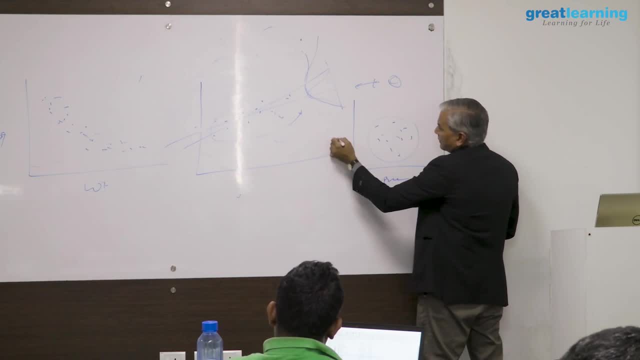 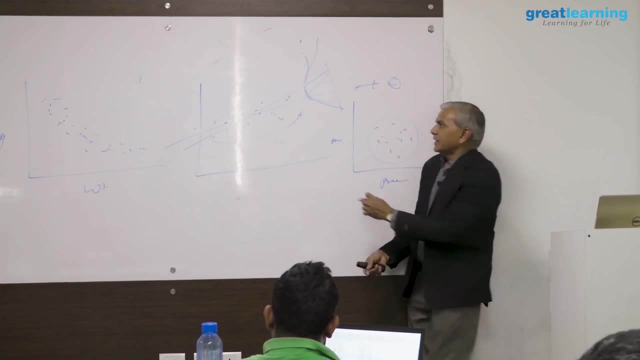 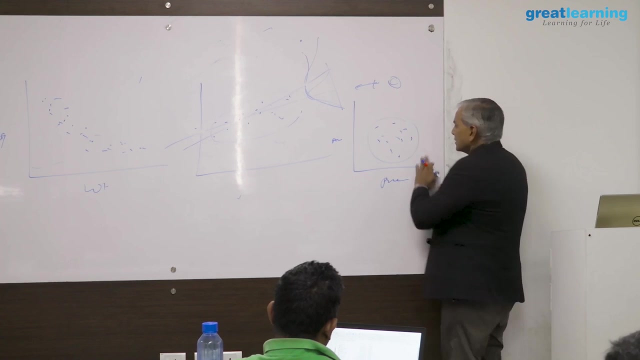 like this: Predicted value of y, actual value of y. there should be no correlation between them. When there is no correlation between actual and predicted, that means the data is evenly distributed across this best fit line. Sometimes you might notice there is a trend in these errors. There is a trend, there is some kind. 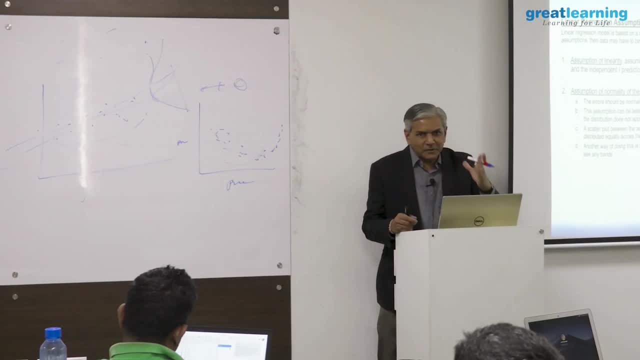 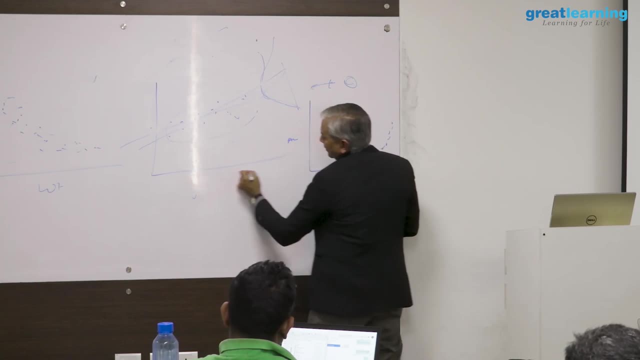 of a trend In the difference between actuals and predicted. there are trends, Which means there is a trend in the residuals. As the value of x increases, the residuals increase in magnitude. As the value of x increases, the residuals increase in magnitude. When you see such trends, 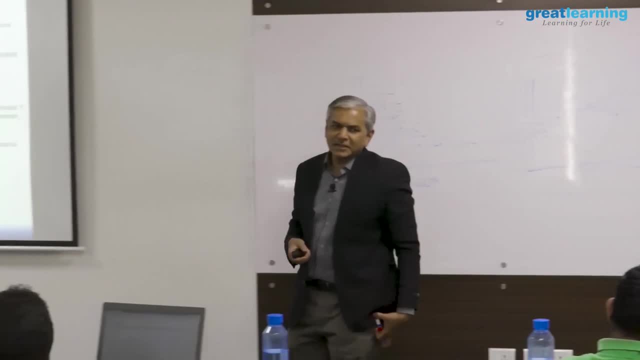 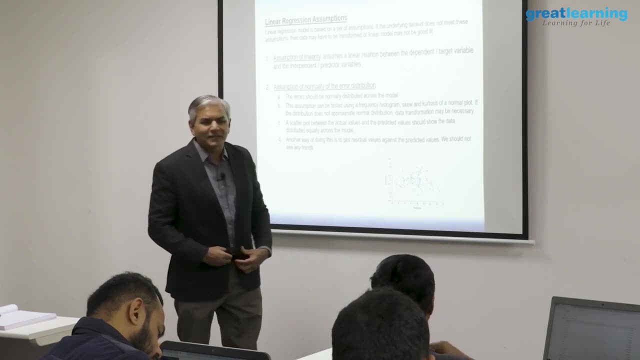 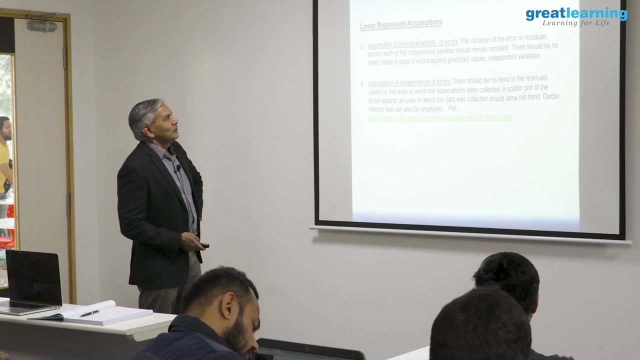 trends in the residuals. that means there is something not correct with your data sets. Maybe you are having outliers, maybe you are building models on non-linear data sets. those are kind of things which will come out. I don't know whether you heard this word: homoscedasticity of errors, homoscedasticity, heteroscedasticity. 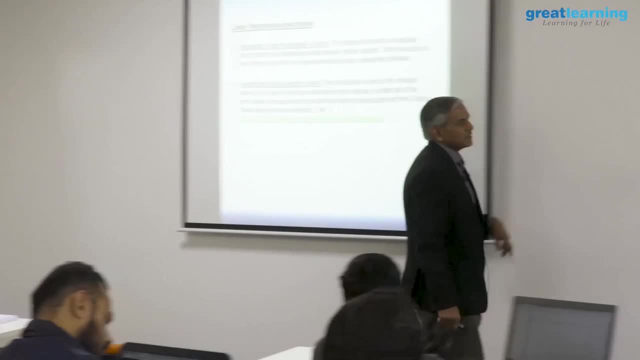 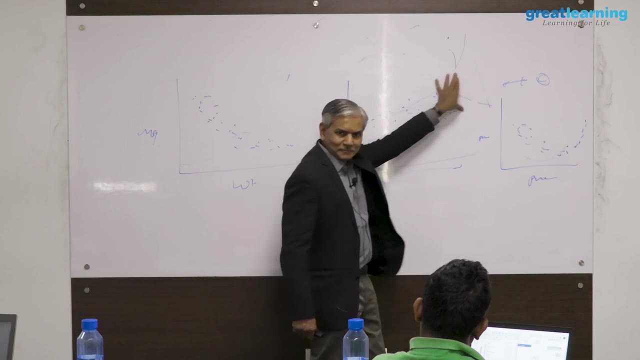 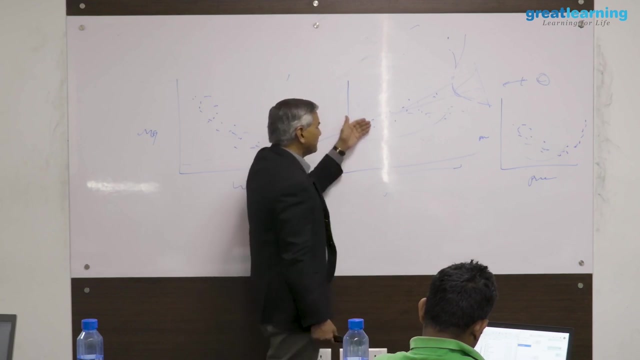 there are two things that will come across in statistics. What it means is, as you build the model, the errors should not spread out like a cone. The spread of errors across this model. for all the range that you have, the spread should be more or less uniform. 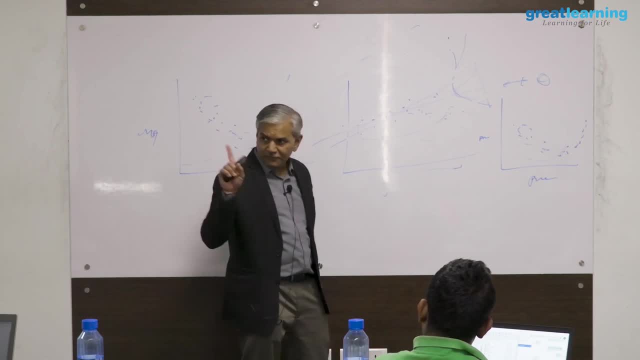 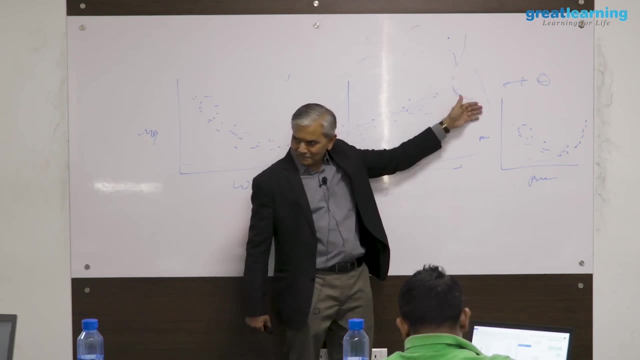 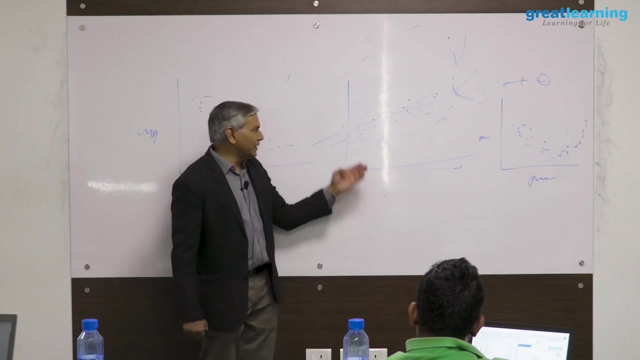 Sometimes you will see that as the value of x increases for the best fit line, the magnitude of the error increases. The spread is still normal. But the magnitude of errors- the residuals- for higher value of x- is different from the magnitude of errors for lower value of x- the independent variables x. 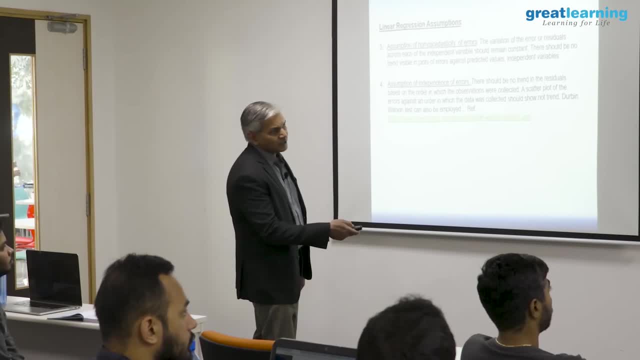 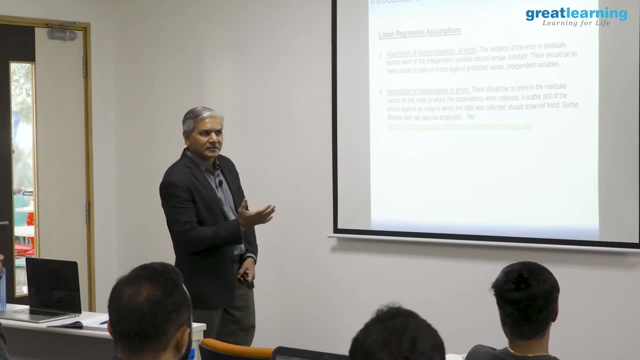 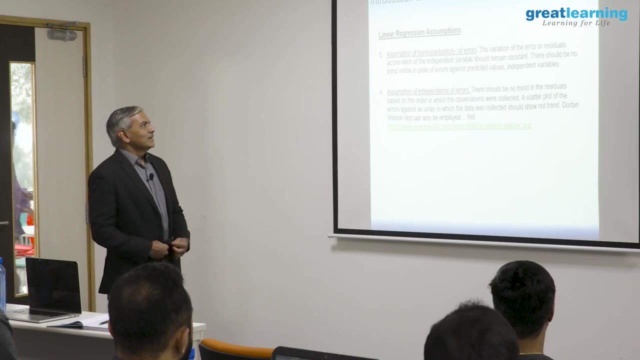 Such things indicate heteroscedasticity, homoscedasticity. The expectation is it will be homoscedasticity. homo means homogeneous, So the residuals, irrespective what the range of x is, will be similar across all the range. Ok, 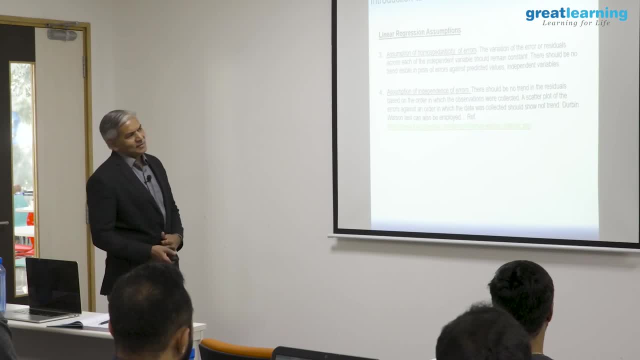 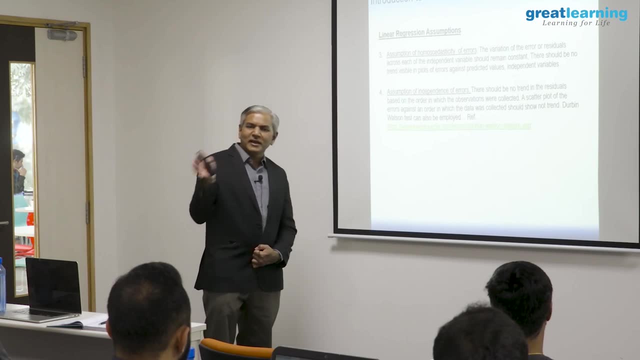 Assumption of independence of errors. I mean error done in one record is no way influenced by the error done in another record. Error done on one dimension is no way influenced by the error done on other dimension. The dimensions are independent of each other. 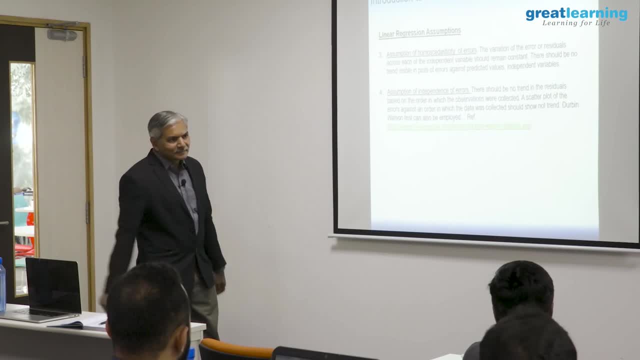 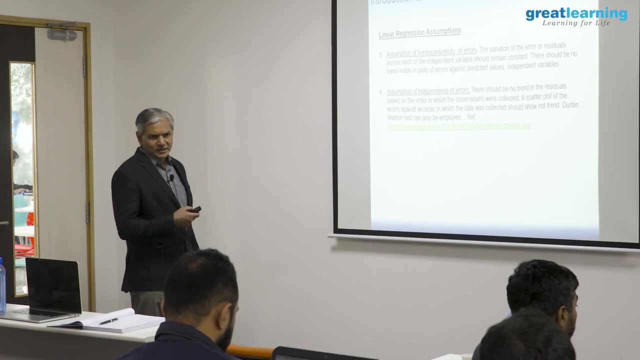 That assumption is what is usually violated, But still, we go ahead and build our models. I found a very good what you call site which discusses these errors. I have given you the URL here. By any chance, you have done this. Durbin-Watson test statistics. you have done statistics. 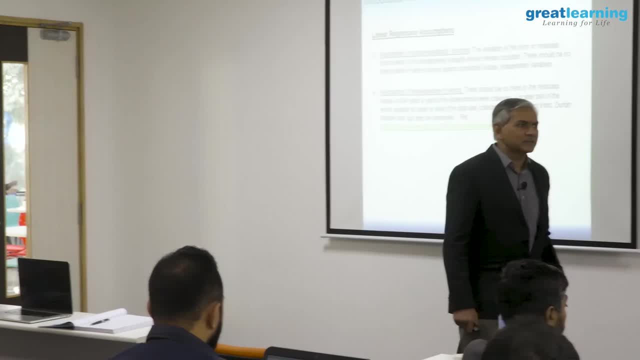 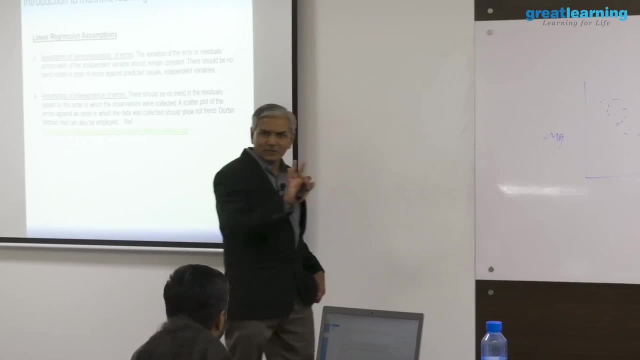 right, the inferential and this thing, descriptive statistics, inferential statistics. you would have done z-score, z-test. you have done all the t-test and all these things you have done, right? Ok, If you have done those things and if you remember those things, maybe you would like to visit. 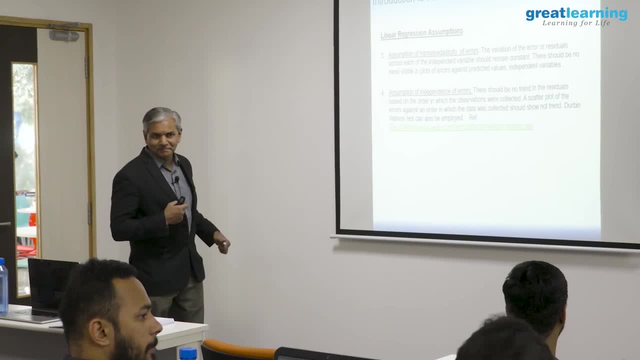 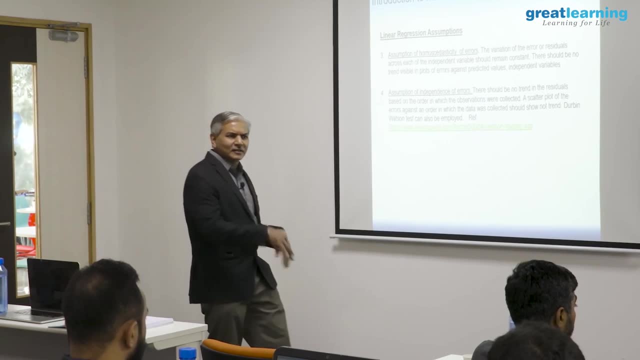 this site lot of information. Please expand your horizons. Go beyond this. Ok, Go beyond what we teach you in the class. It is just not possible to teach everything in the class for the time limit. So go beyond the whatever we teach. expand your horizons, yeah. 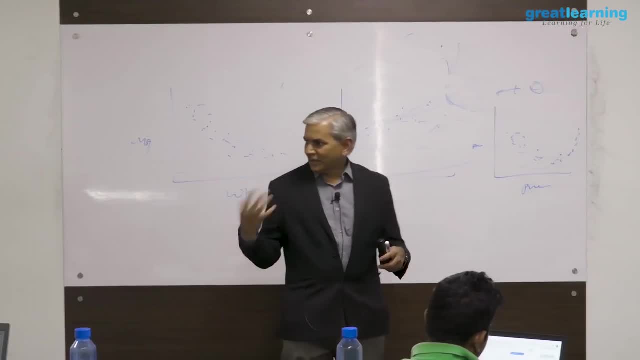 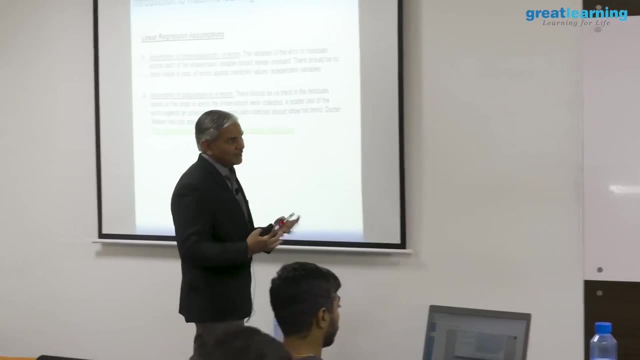 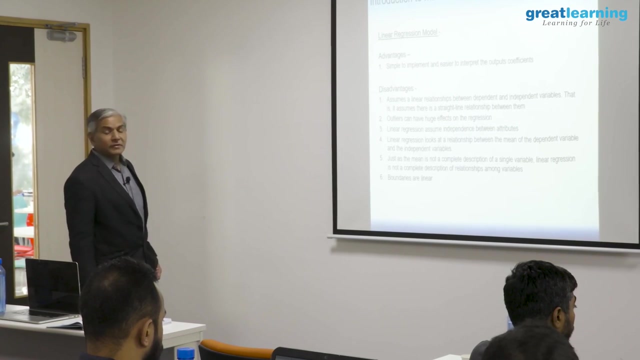 That is what will give you a very firm, sound footing into data science and you will be able to face situations confidently. So wherever I come across any URLs, any articles, I will share those things with you on the site Advantages. we are still not out of the woods. 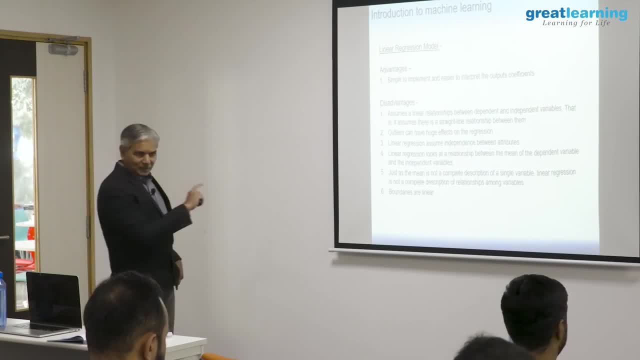 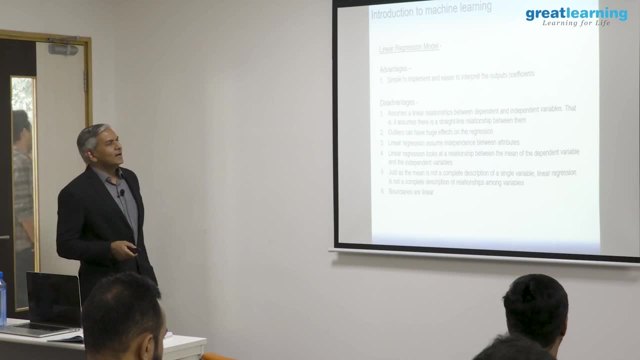 There is still much more to come. We have not yet learnt the full stuff, But we will do hands on and then we will see the other stuff. Advantages is very simple to implement and it is easier to interpret, provided the number of dimensions is less. 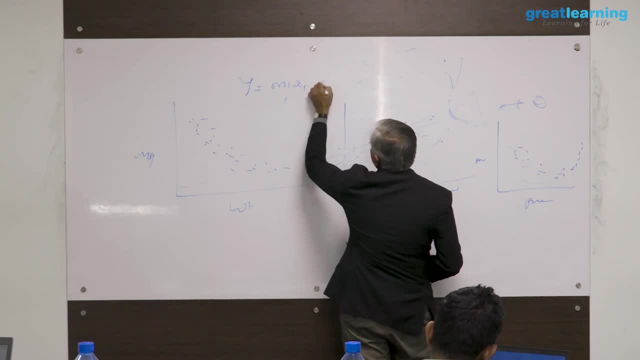 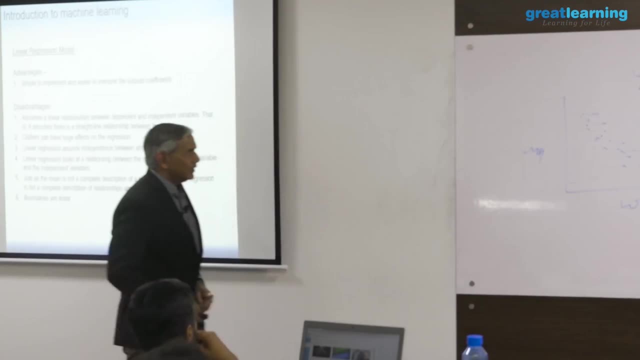 So when I have equation like y equal to m1, x1 plus m2, x2 plus c, I can give a physical meaning to this. I can say: for every 1 unit increase in x1, how much y changes? That is given by m1. 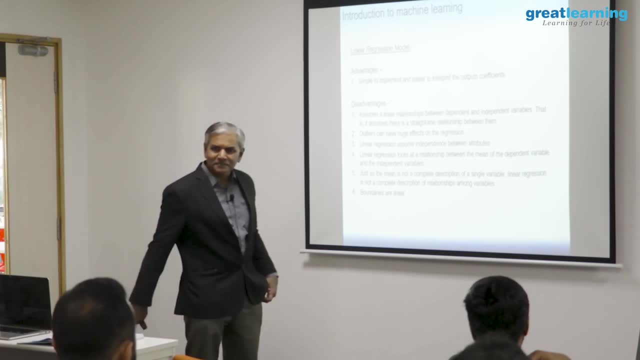 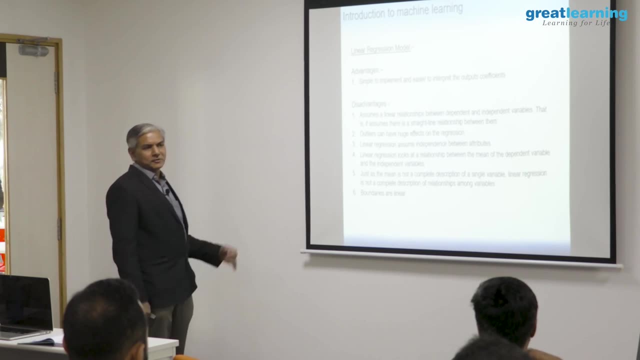 So I can physically interpret this, I can give physical meaning to this equation. You cannot do this in all the cases. You may not be able to do this. suppose you are using neural networks. you cannot interpret those models. You do not know what they are. 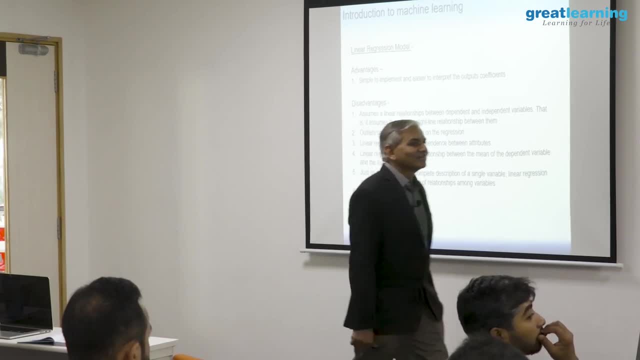 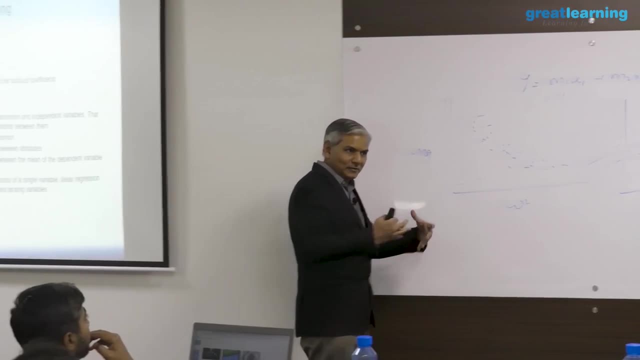 They are all black box. Sir, what do we mean by physical definition? Sir, I can convert this. whatever this formula is telling me, I can map it to English, right? I can tell you in day to day language what it is telling you. 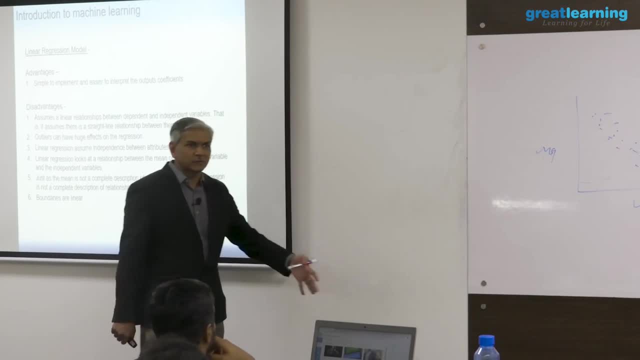 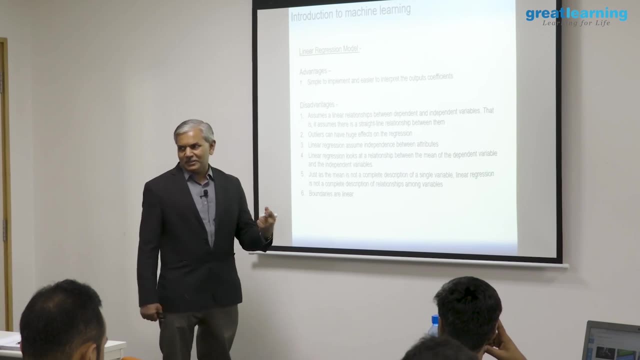 I won't be able to do that if I use, say, random forest. You are going to do ensemble where you will do random forest. Random forest is a black box model. We don't know what it is actually doing inside. Support vector machine is a black forest. 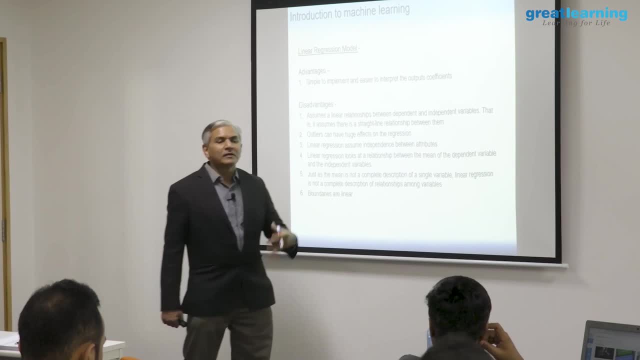 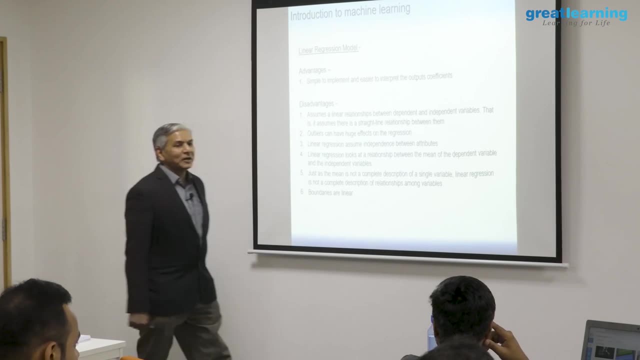 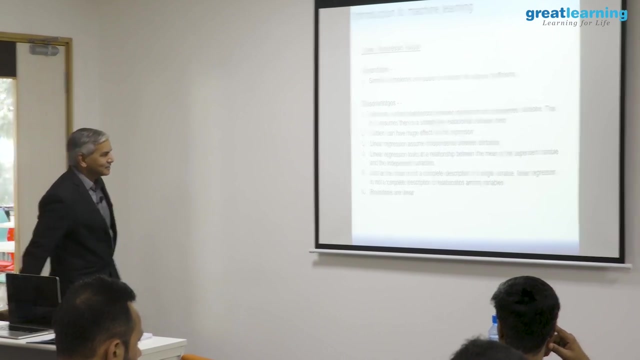 We don't know what black forest. black forest is a pastry black box. We don't know what it is doing inside. right, This model is a white box. Outliers can bring it on to its knees. This particular model is prone to outliers. 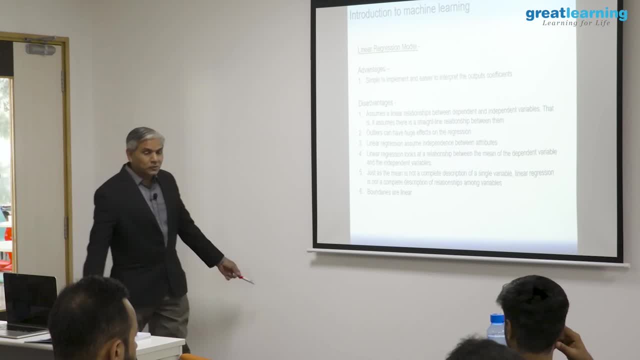 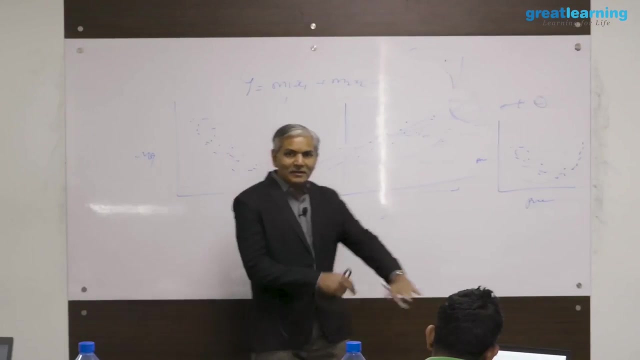 All linear models are prone to outliers. Decision tree is not prone to outliers And one. this is a very important point, Since the linear model goes through the point where x, bar and y bar meet the best fit lines. the lines evaluated for you go through where the x bar and y bar meet. 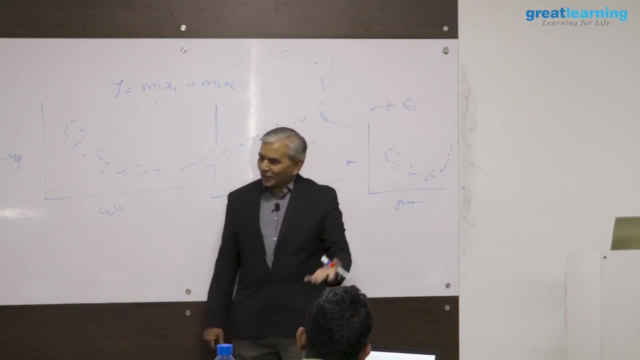 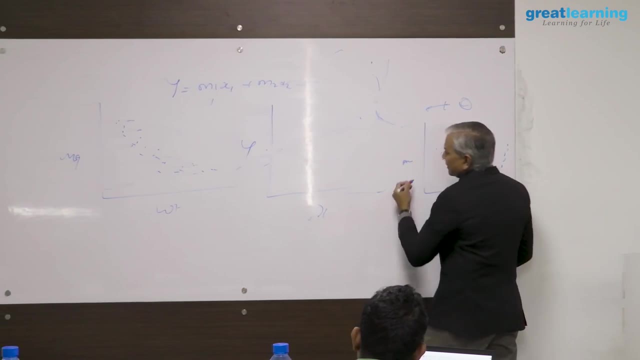 If your x bar and y bar are not reliable, then your model itself will not be reliable. So if I built a model on a dimension y and x where this is a very large spread, very large spread where x bar is not reliable, 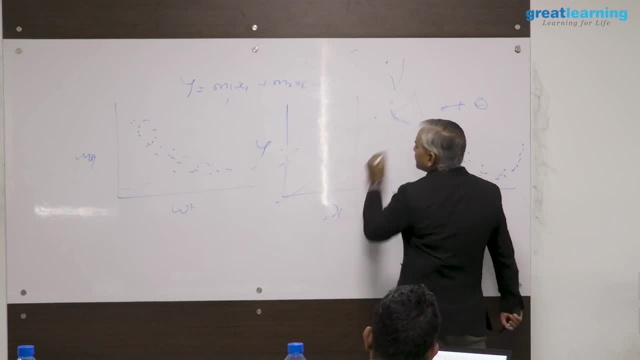 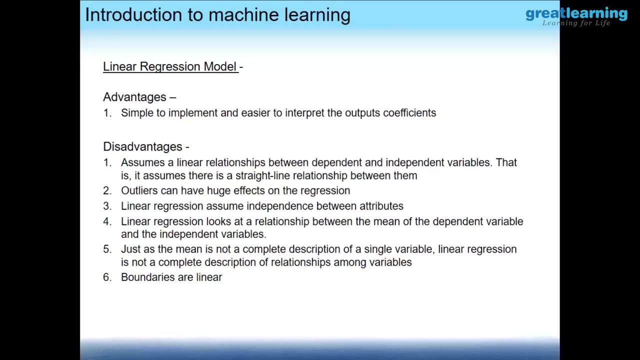 When x bar is not reliable, how will the model which is going through the x bar making use of this x bar, how will the model be reliable, right? So the more time you spend in selecting your attributes to build the models, the higher. 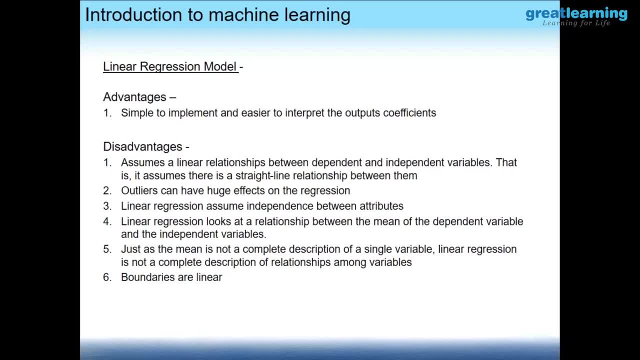 the quality of the attributes that you use to build the model. So the more time you spend in selecting your attributes to build the models, the higher the models, the better your models will be, And the last boundaries are linear. This is a problem not in regression, this is a problem in classification. 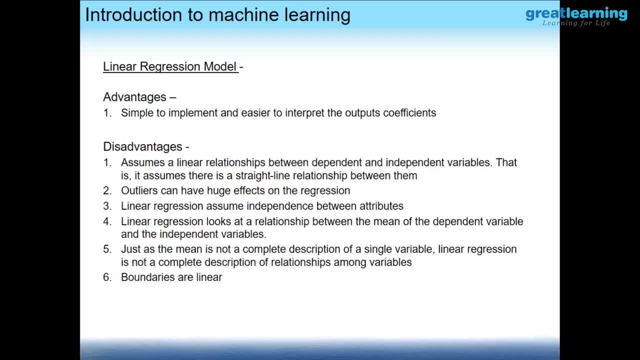 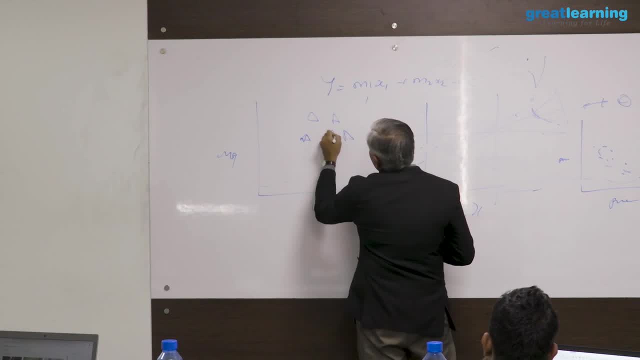 So if we can use linear model for classification also. So if you are having distribution of classes like this and then this and you are trying to build linear classifiers, you will get probably a line like this as a best fit line: 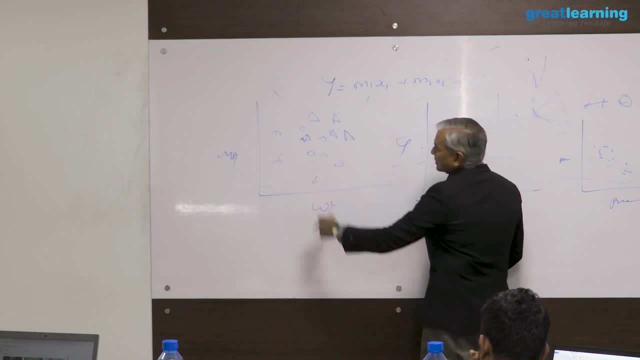 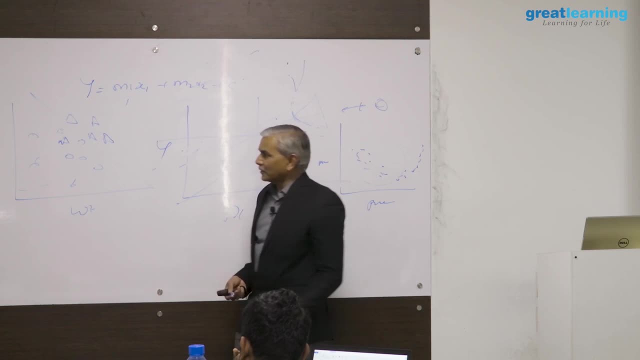 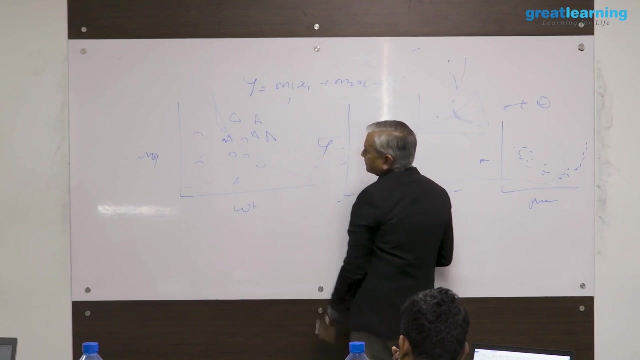 So above is this triangle, below this is circles and one triangle is, whereas, on the other hand, if you have made use of non-linear stuff, non-linear models, then probably you would have got a better result. Maybe you would have gotten something like this: ok, 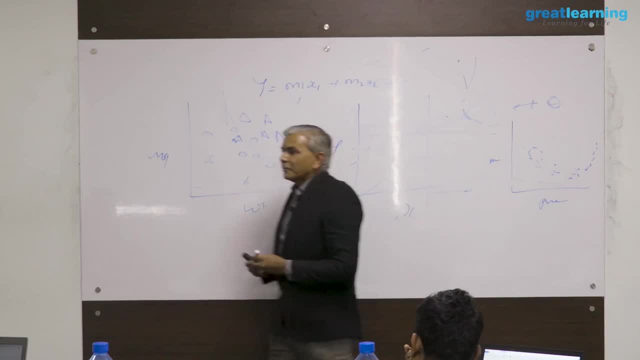 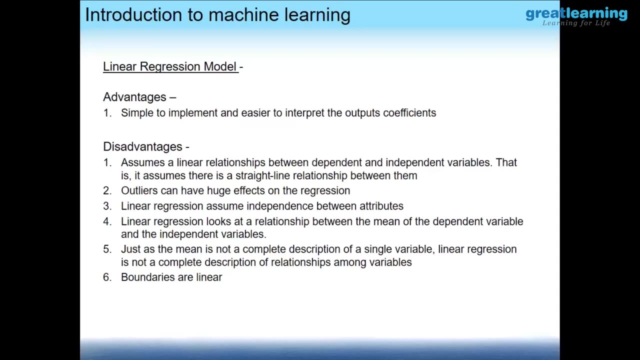 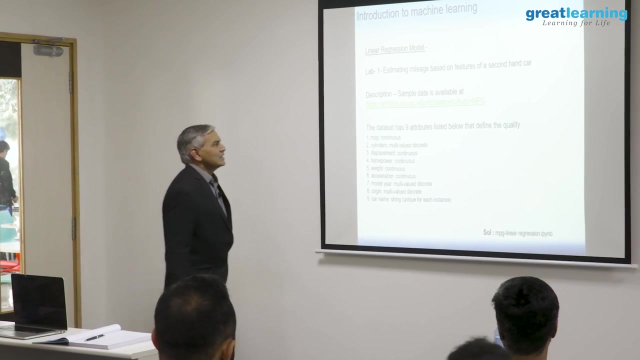 So if you use non-linear models, it might do a better classification than linear models. So this limitation is not in regression, it is in classification. Ok, Let us do one hands-on. ok, The hands-on is not auto-MPG dataset as it is given here, it is the other one which 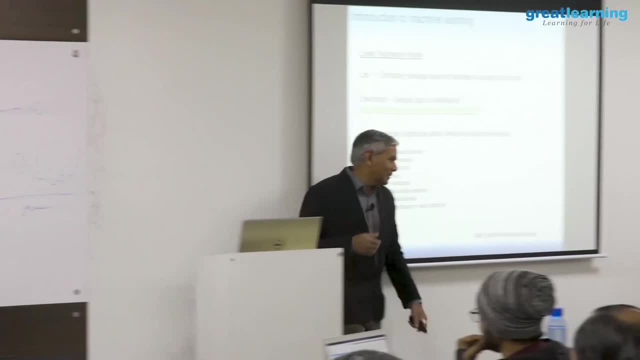 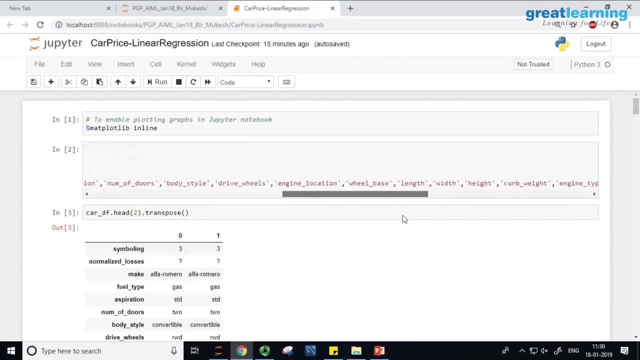 is simplistic, So we will start with simpler ones. The other one which I have given to you is CARP. ok, CARP is linear regression. I have taken the dataset directly from the UCI site. It is called imports underscore. 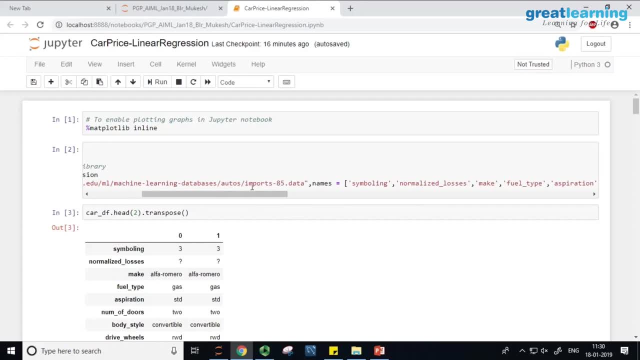 Imports hyphen 85 dot data. This is the name of the data file. ok, So instead of downloading it, I am directly reading from there. So let me begin. Matplotlib is an instruction to the Jupyter notebook to plot make. all the plots in the 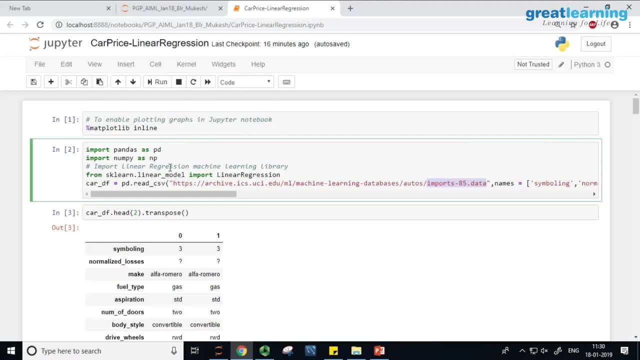 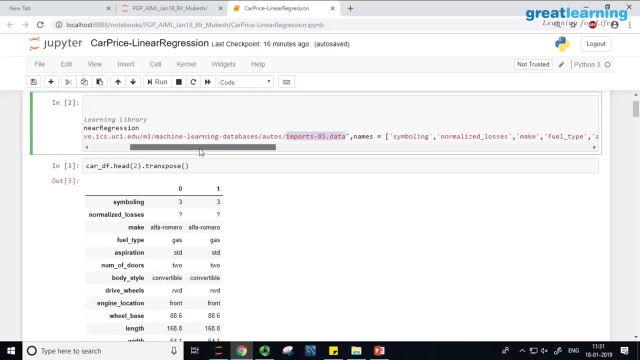 notebook itself. sorry, Jupyter server. I am importing pandas, numpy and from scikit-learn linear model libraries. I am importing the linear regression. You can have linear classifiers also. Then I am reading the csv file which is available in this URL. it is a comma separated file. 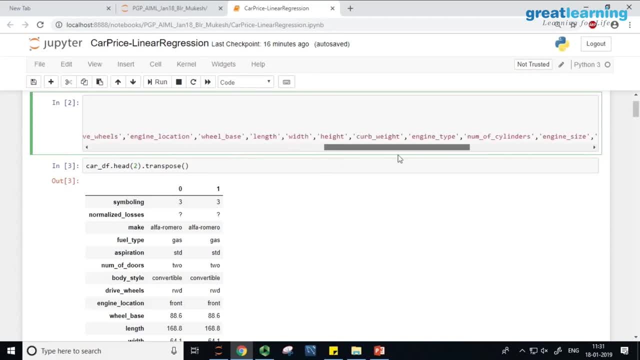 and I have taken all these column names from the UCI dataset. So that gives me the data frame which I call CARP, underscore df. This is my data frame, All of you? ok? Ok, So this is like loading a data into a table. 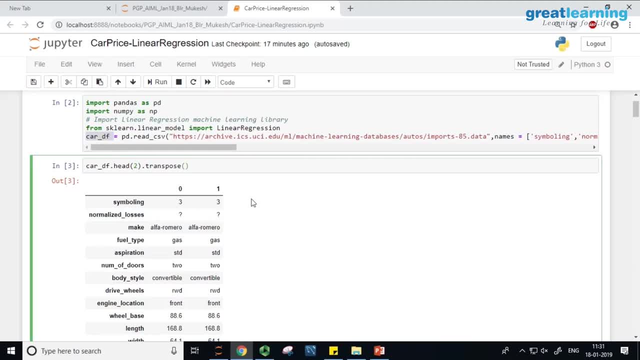 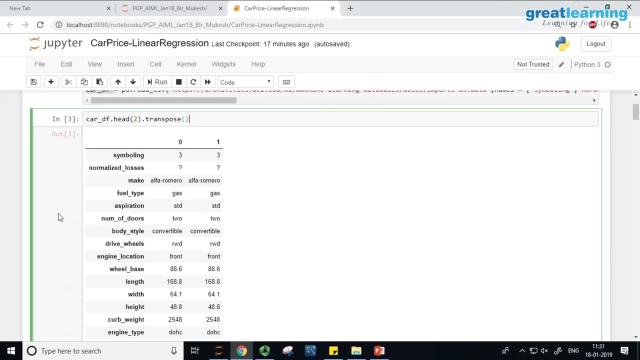 So let us look at two records. Transpose is not a must, but since the number of columns is huge, I put a transpose. I am seeing first two records: record 0 and record 1.. There is obviously missing data in some of the columns and there is string data types. 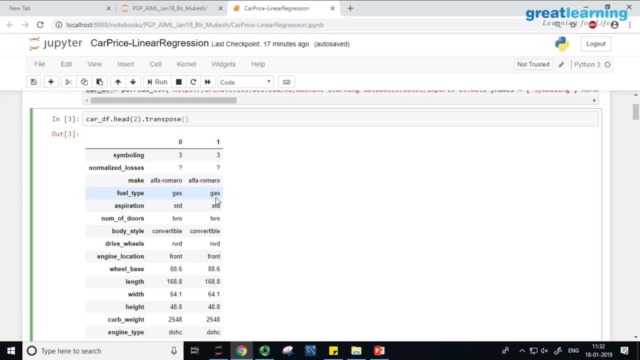 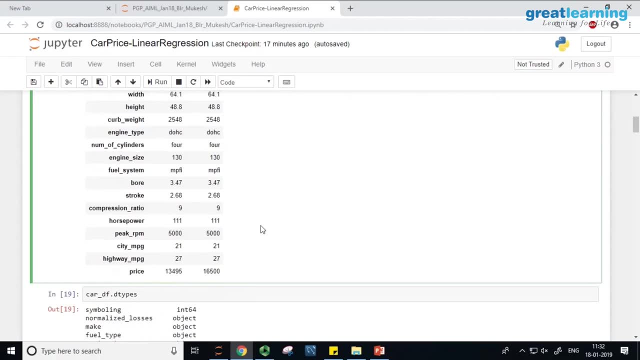 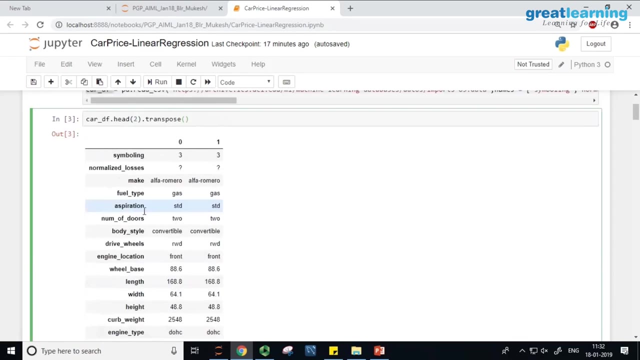 in other columns. fuel type: gas: it is string data type. Number of doors: 2,. it is a string data type. All right, no problem, go down. Our objective is to predict the last column. Given all these independent variables, can we predict the price of the car? 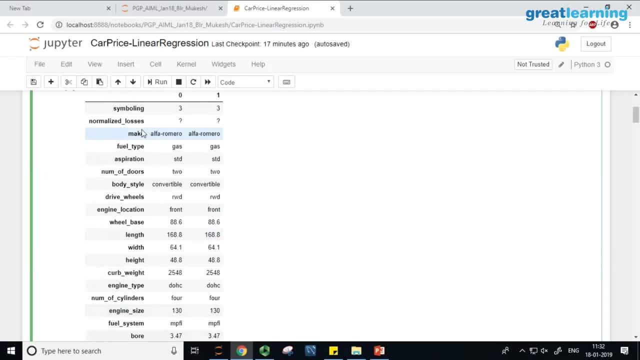 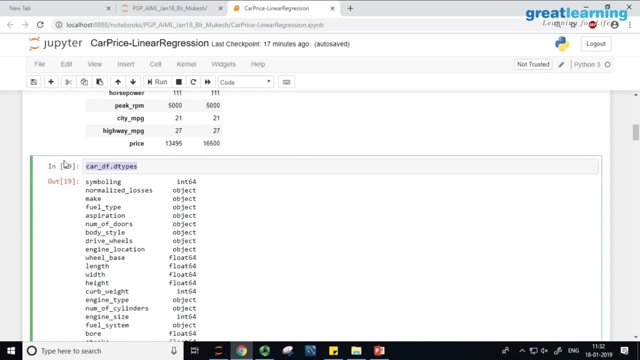 Is there a relationship in price and all these variables? That is what we want to find out. What is that relationship? But before we do that, look at the data types. Many of the data types are object. Object means string: Machine learning algorithms. 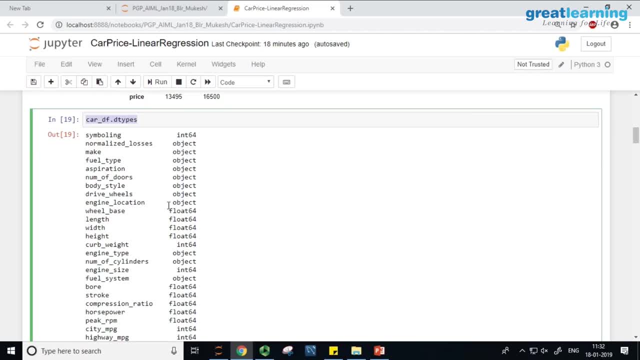 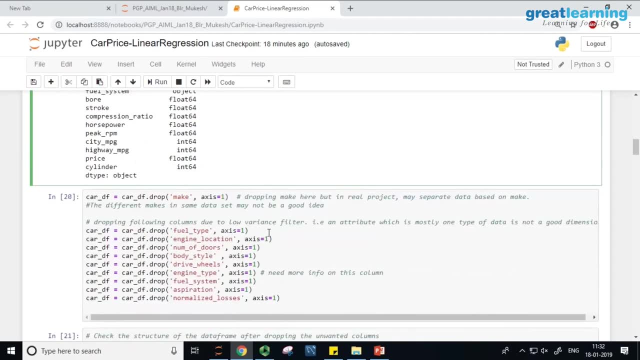 Machine learning algorithms cannot handle string data types. they have to be converted in numbers. So what I am doing here is I am going to convert into numbers, but before I convert numbers I am doing I am dropping some of these columns. 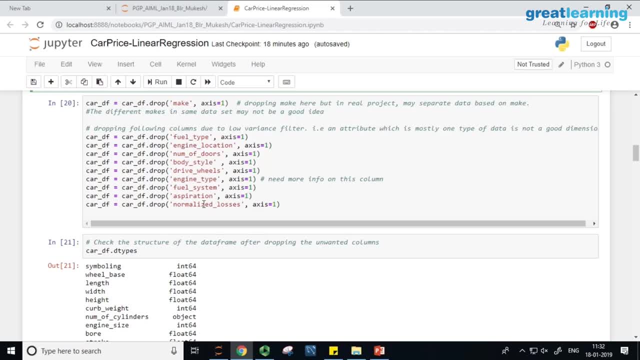 The reason I am dropping these columns is if you go and take a frequency, count on these columns- fuel type, for example, or engine location, for example- most of the records have only one value for this. This is called low variance filter. Look at all the data provided to you. in the data you have columns. where in the columns? 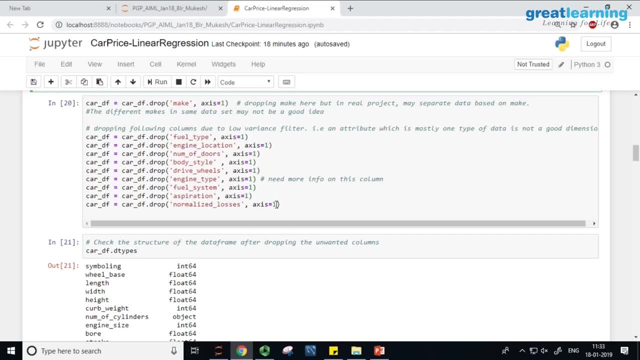 there is not variance at all. there is a gender column, Gender column. all the data is about males, then that column is useless. it is not going to give you any information. Such such columns are called low variance columns. now they are supposed to have multiple. 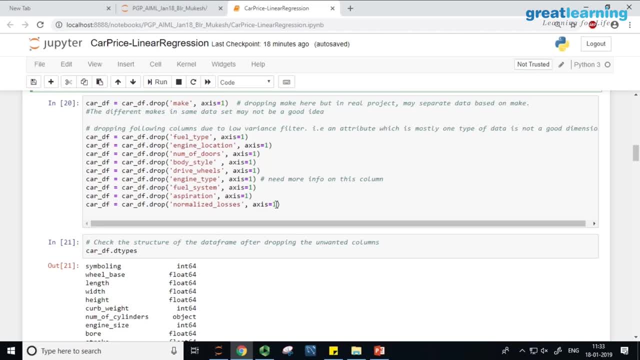 values. they have only single values, a few values. We remove them from the analysis. Now, what we are going to do is we are going to convert these values into numbers. We remove them from the analysis. So, when I just did this, 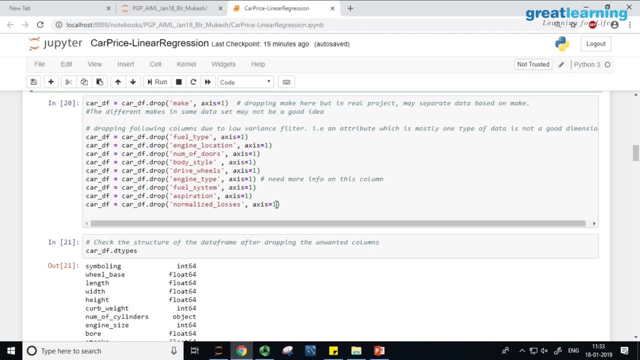 So we would visually do this check and get to this conclusion. Yes, yes, You do a frequency count. verify the conclusion. I have already did this. I have manually browsed the data file. this is an excel sheet, CSV file. 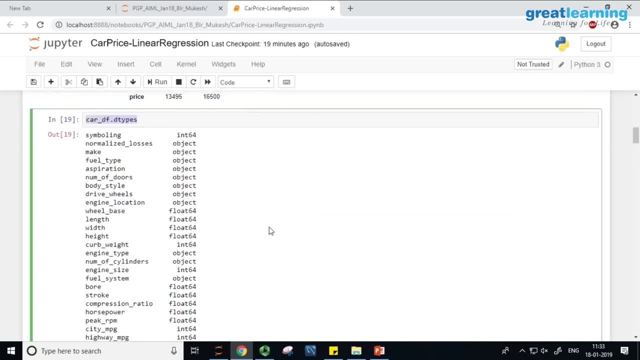 You can actually see. let us do it now. why are we talking? Let us do this. What you do is go to this site and let us download this data So you can actually see. let us do it now. why are we talking? 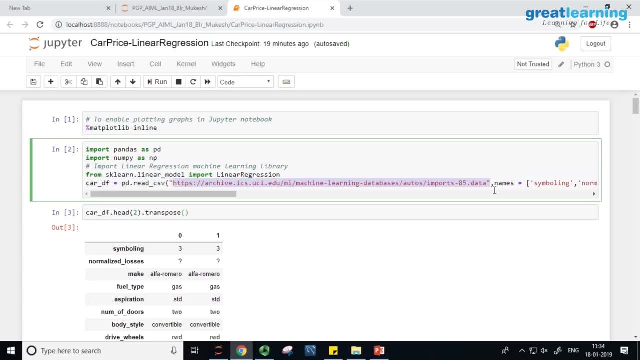 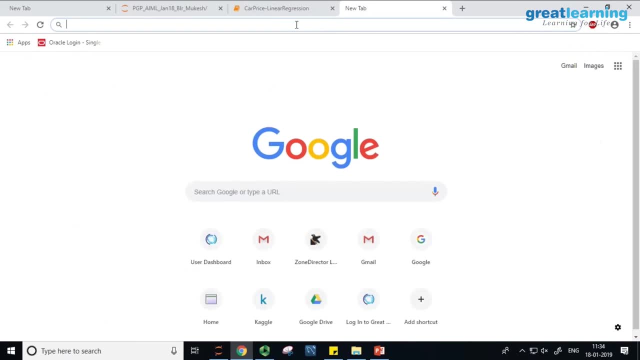 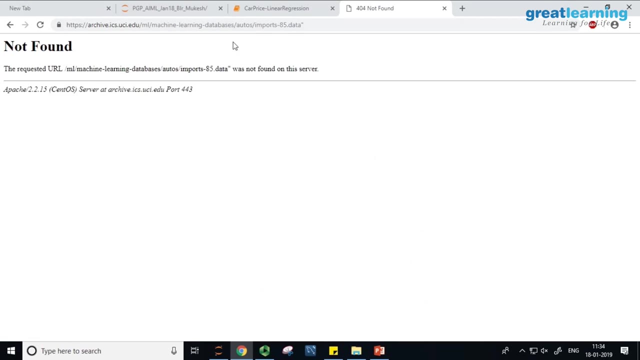 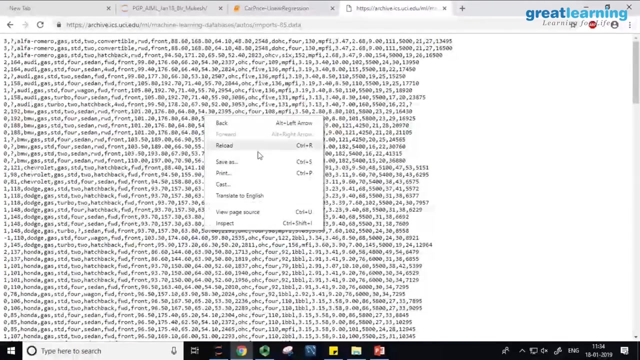 Let us do this. You can actually see. let us do it now. why are we talking? Let us do this and let us download this data set Control C. ok, Now HTPC is manifested. Thank you, Now we will save this down. we will save it as. 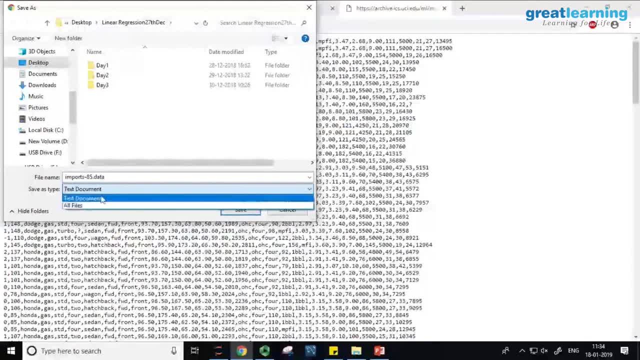 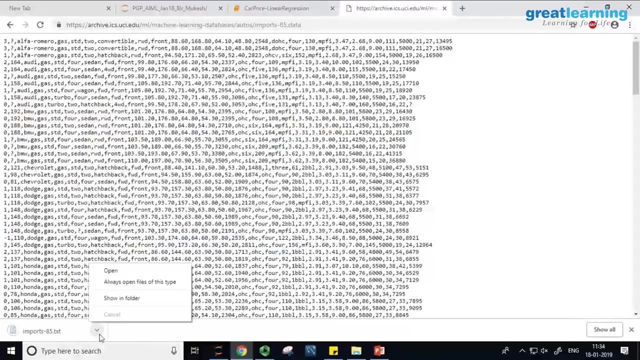 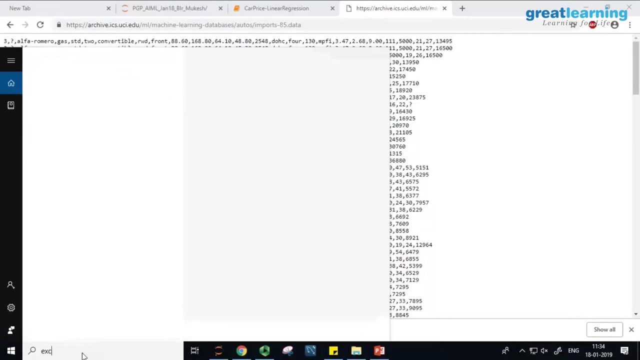 we will save it as. let us save it as declaration tables- Yes, text document, and then we will load it up. I will just call it. ok, where am I saving it? I will save it on desktop. ok, done, Let's open it. ok, Let's start excel. Excel is. 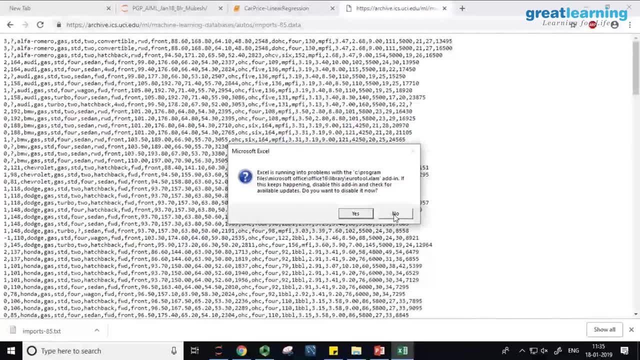 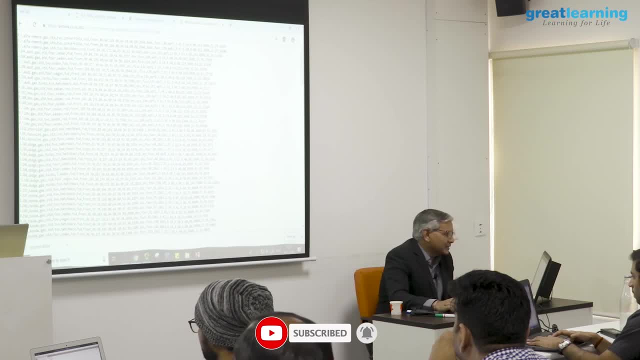 running into problems. let's see. oh god, oh ok. ok, it is going to clash with their recorder, So I am not going to open this. Let's get on to this code. but do this analysis. you will find that these columns are having low variance filters. They are fit to be kicked. 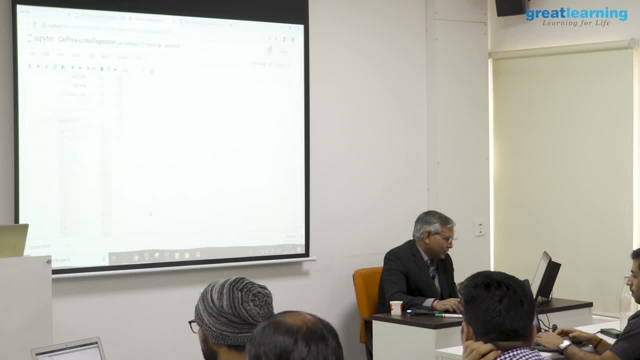 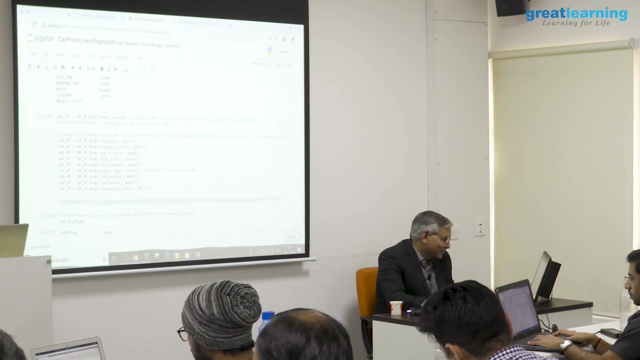 out right. So then what I do is: I saw the car data types, the column data types. Most of the data types are object string types. I drop my useless columns. Number of doors: most of them have four doors. Then fuel type: 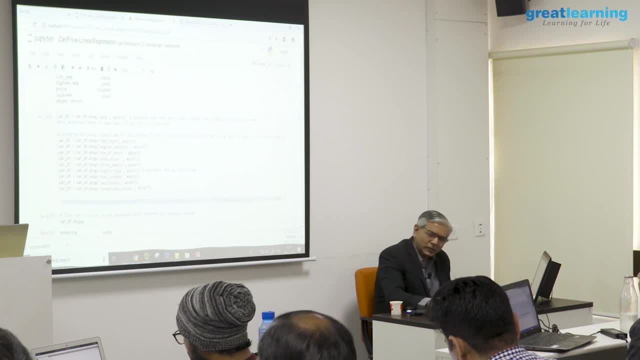 most of them are giving the fuel type as gas. Engine location, most of them is front, one or two is in the reverse rear, so on and so forth. So once I drop them, I am still left with some object, data type, Number of cylinders. 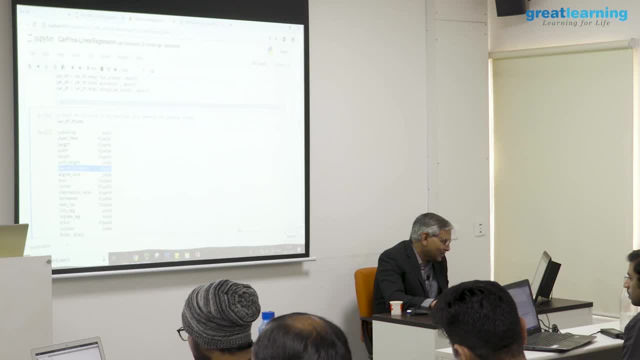 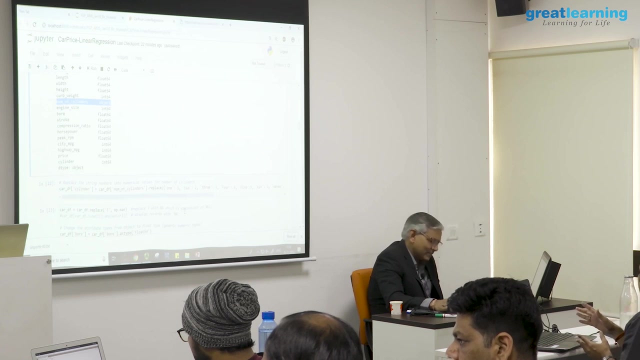 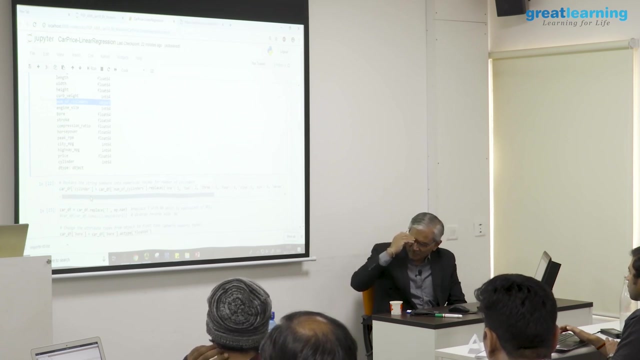 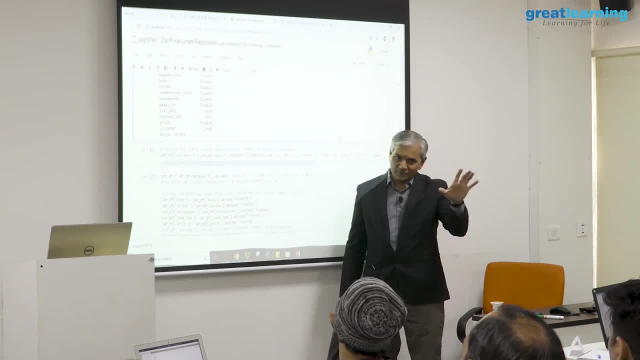 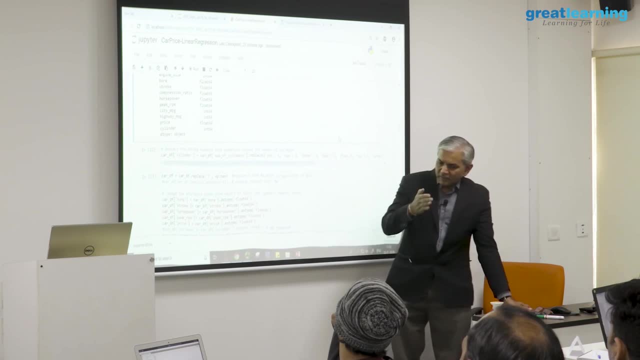 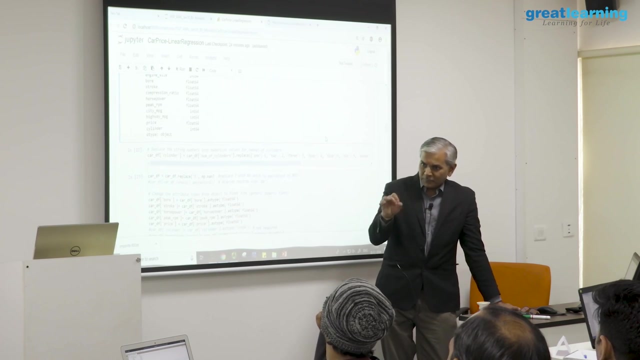 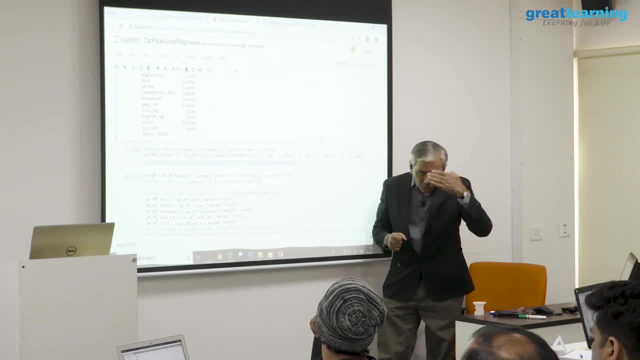 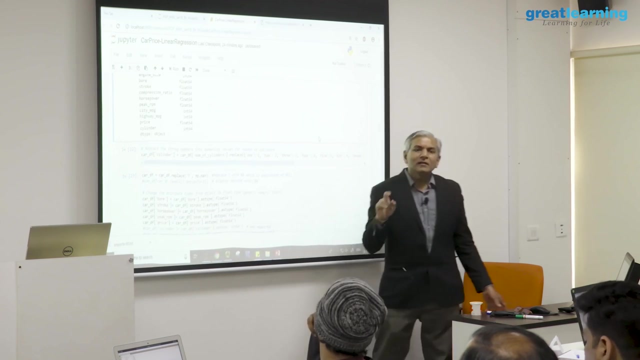 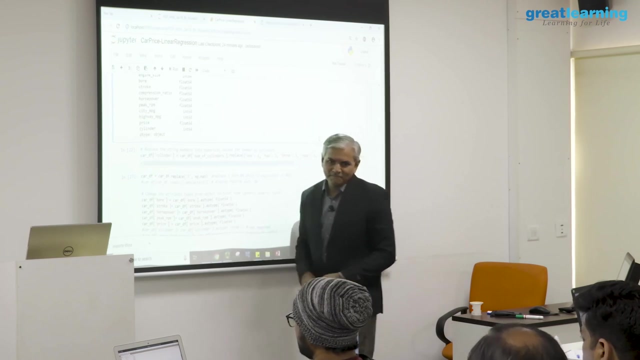 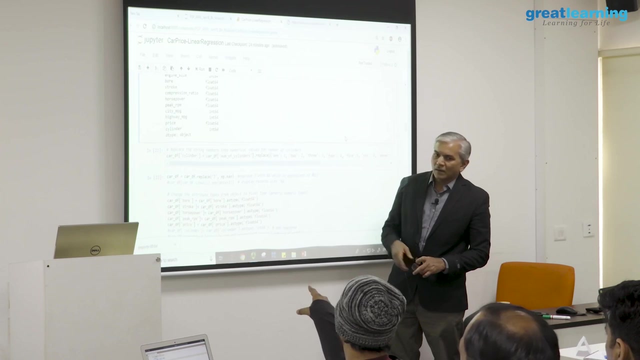 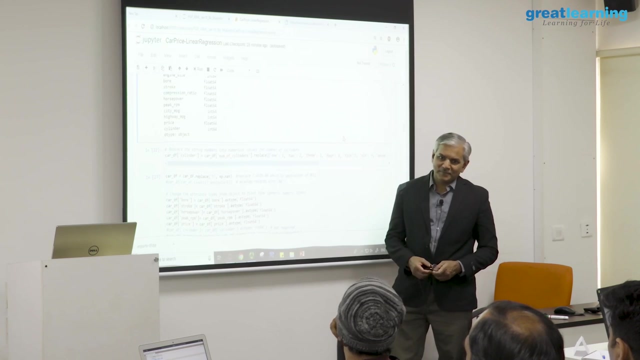 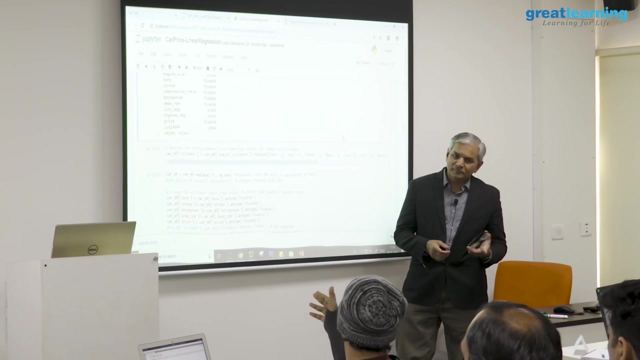 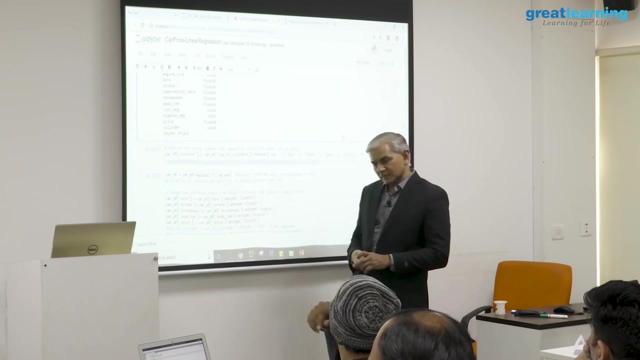 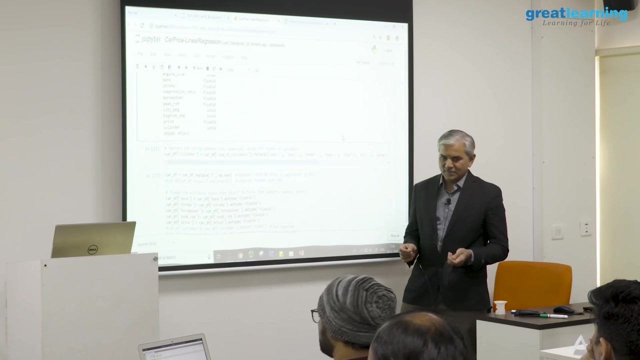 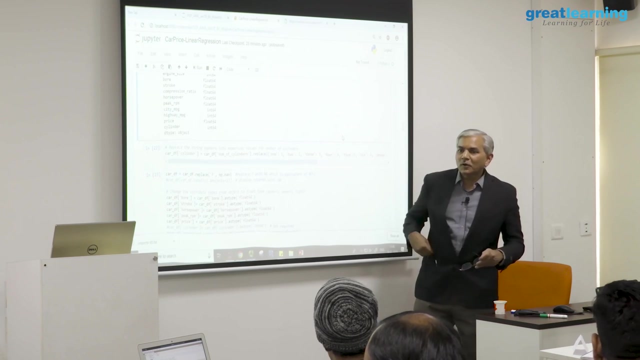 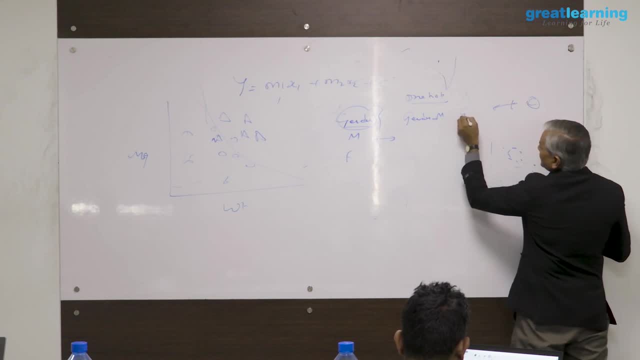 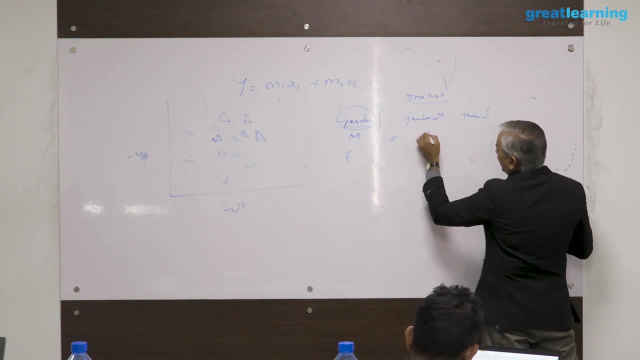 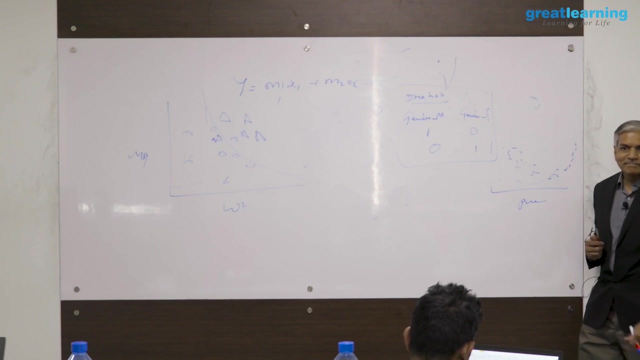 M. gender underscore M. gender underscore F: Wherever the record is M, you will have 1 here, 0 here. Wherever the record is female, you will have 1 here, 0 here. So this column will be dropped In your data set. you will be left with this column: 1 and 0 will be. 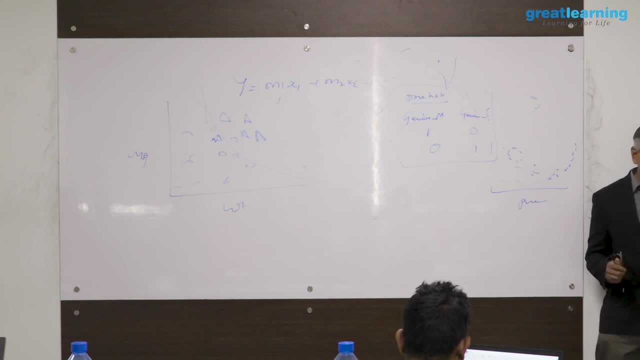 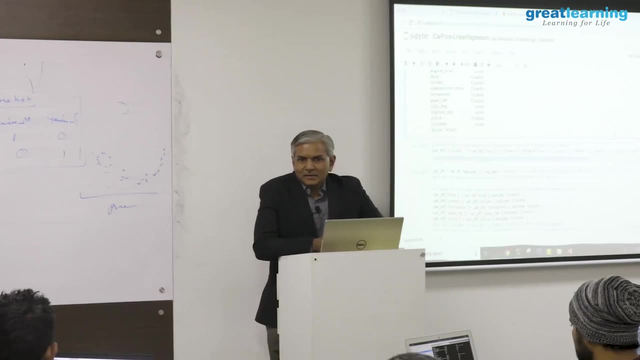 stored on the hard disk or in the in wherever you are storing it. as numbers Limiting numbers Last class, we had used this category, not category Category, as in K, nearest neighbors. Yeah, We used what Category, or something? 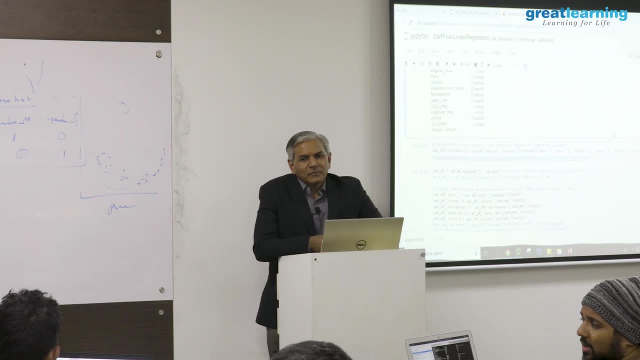 Yeah, we just manually converted. we did not Category Category Last time we just converted to category and then we changed it to 0 and 1.. See how we converted: Category: Category, Category, Category, Category, Category. 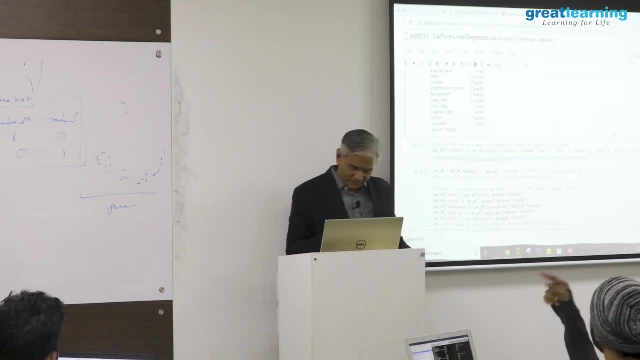 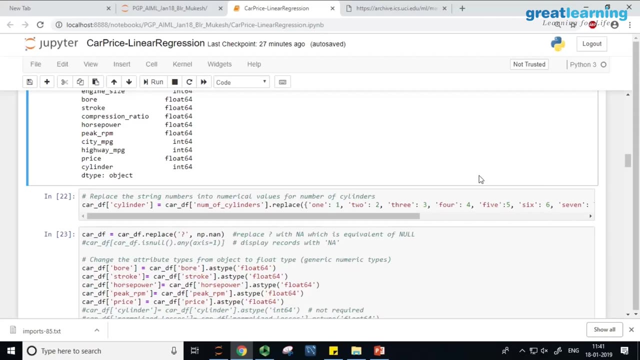 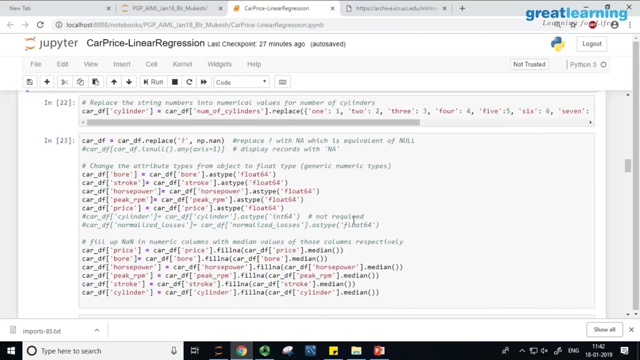 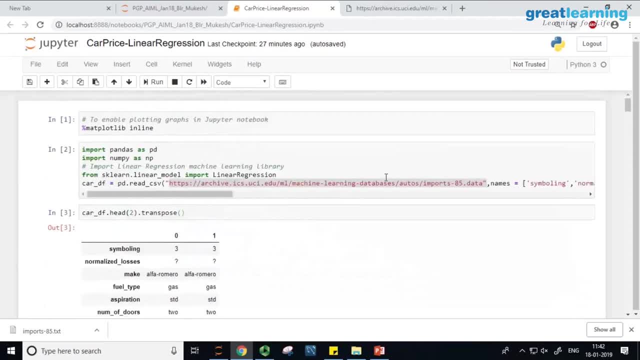 1, 2, 3, both 1, 2, 3, ask for the number, But what happens? if you see cities? let us see. if you count 2, 3 cities, it does not have 1,, 2, 3.. If you have, let us say: 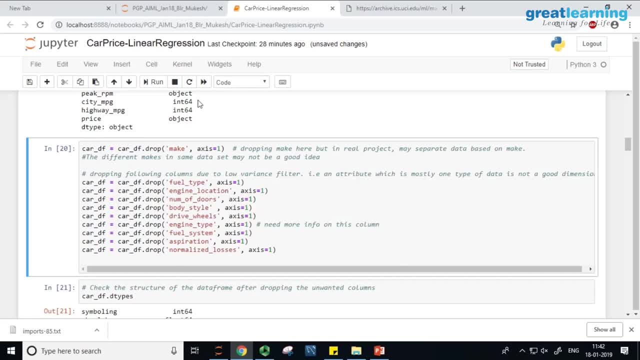 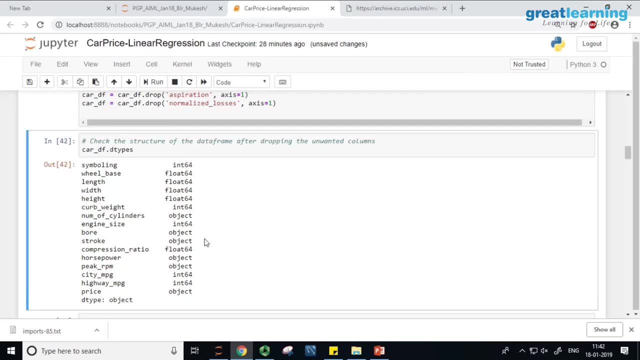 Bohran's took is right now. also, there is no feedback, no object, So I am dropping my these data types. ok, and here car data types. let us say again: bore and stroke is still object data types. ok, Here I am converting my cylinders. 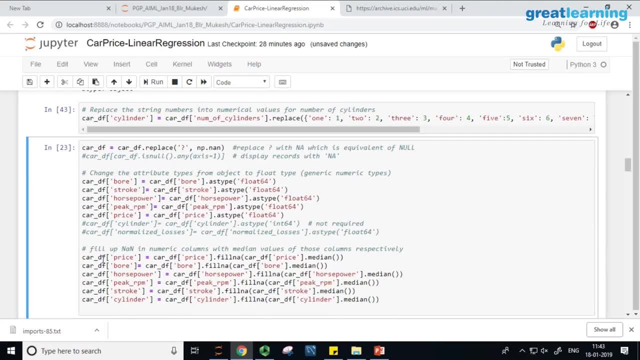 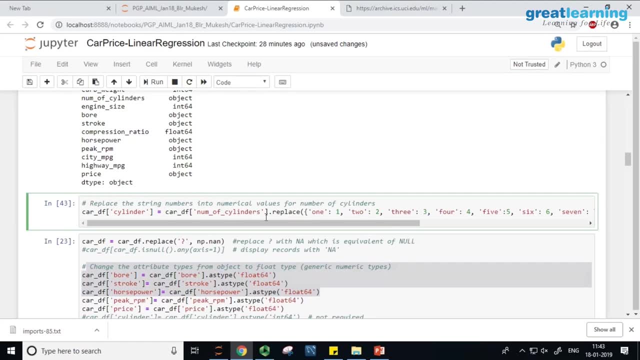 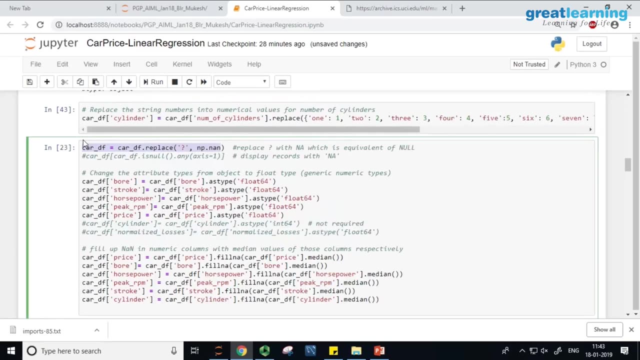 into numerical data types. and here I am converting my data types into this thing float. ok, Guys, all of you with me on the cylinders till cylinder point. ok, After cylinder point. what I have done here is based on the experience I had in the other data set where they were missing values in in auto mpg data set you will see missing. 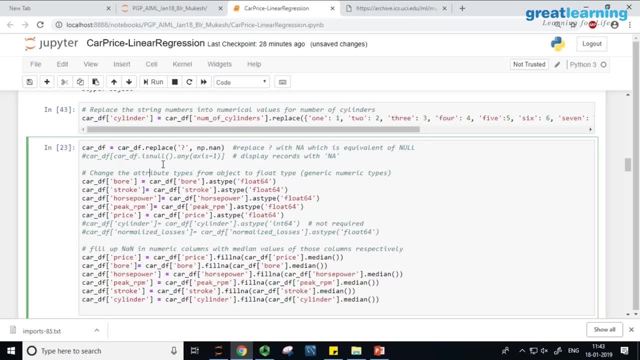 values. ok. So what we do is, if we come across any missing values, replace it with nan. nan means not a number, null values, ok. So what I am doing here is car underscore d, f, dot, replace where. if you come across with some question mark, replace with nan. but I did. 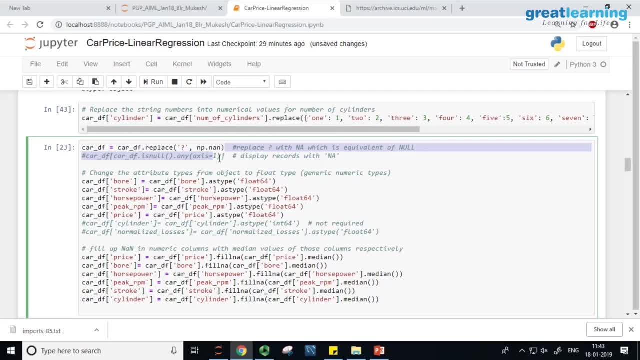 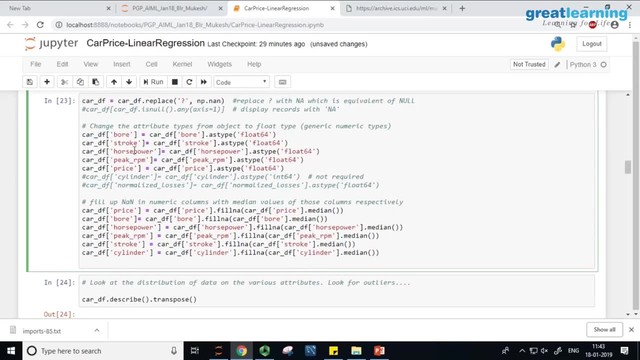 not find any question marks in this data set. the question marks were there in auto mpg data set. ok, So we do not. we can actually delete this line. we do not need it. Then at this point, what I am doing is there are question marks there. 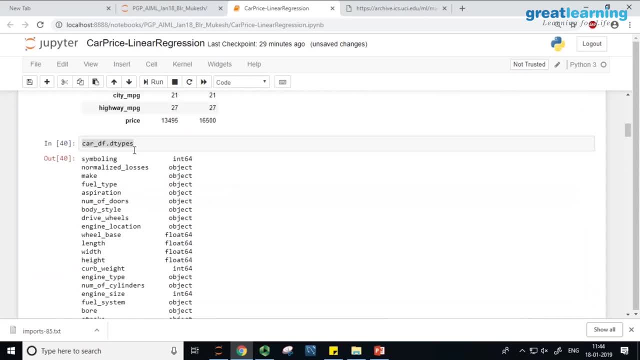 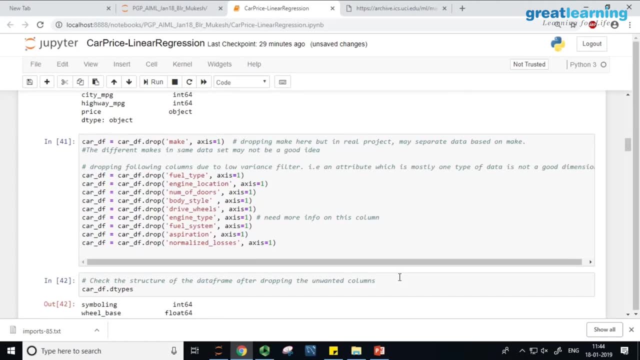 Oh yeah, sorry, there are question marks there, correct, we saw it here. right, we saw it here. question marks here. sorry mistake, There are question marks here. these question marks now would be replaced. Replace with not a number, null values. ok, When you replace question marks with null. 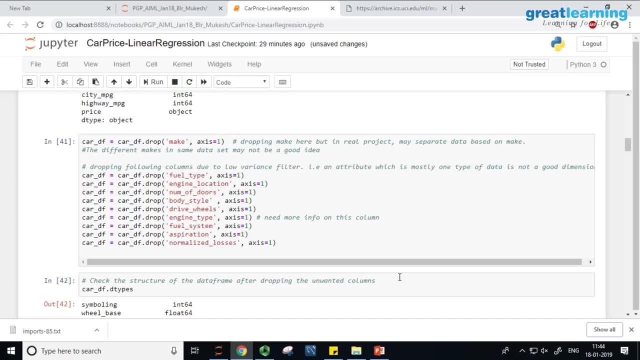 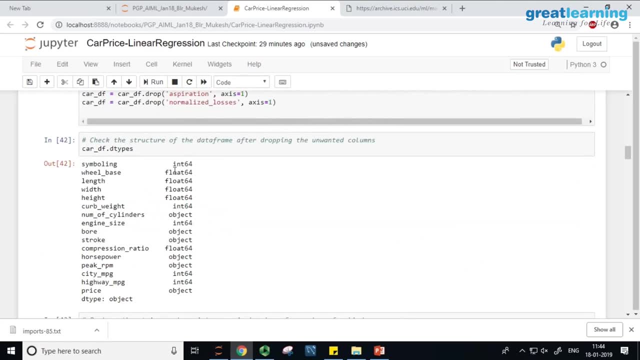 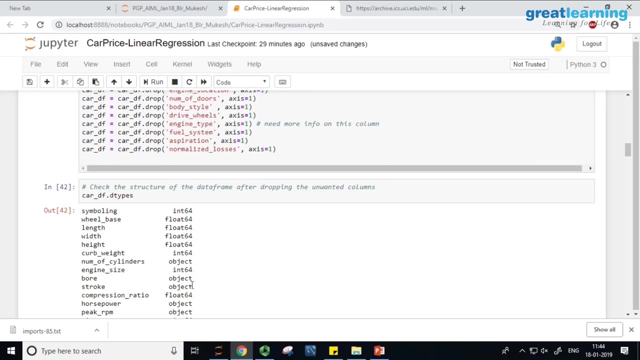 values. you can do numerical python operations on it and convert into appropriate values. ok, That is why we did this Move on. my data types right now are: after changing the data types here, after dropping the columns here, some of the data types are still object object. 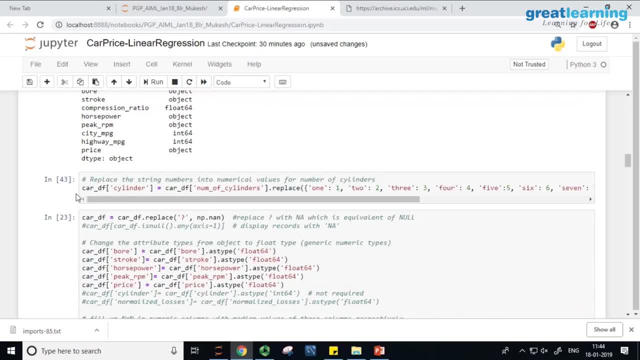 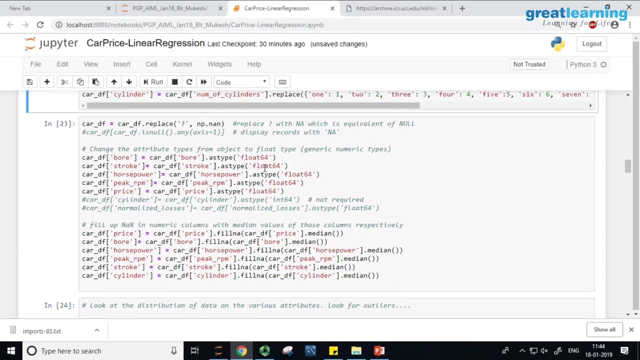 means string data types. So what I do here is I first convert my cylinder into into numericals, then I change my data types here. look at this car underscore d, f bore. I replace that with as type float. I replace stroke column as type float. So I am changing all the data types to float because many 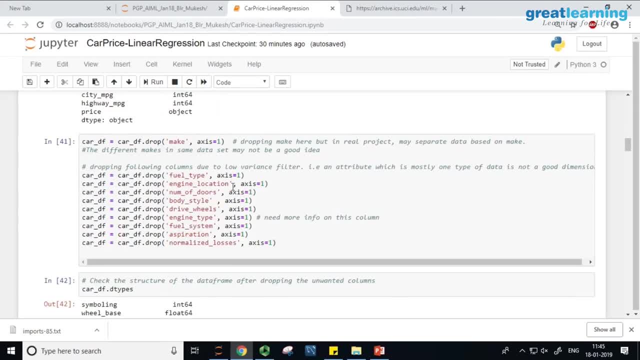 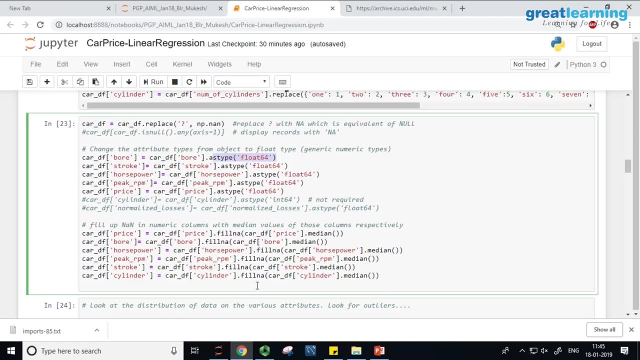 of these columns. let us see which column had that question mark: normalized log. So I am changing the losses- normalized losses. it is already a numerical column. I think, yes, it is already a numerical column, So I do not need to change it. there you go, it is already. 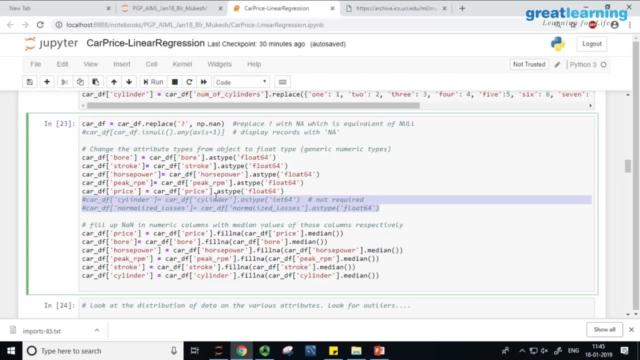 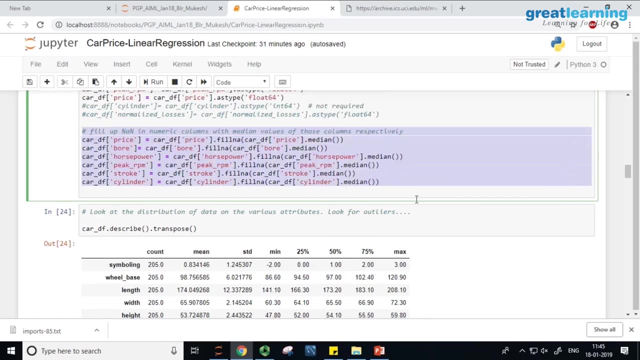 a numerical column So I do not need to change it. rest of the columns, which are object data types, I am changing into float types. till this point, is it ok? Once I have changed the data types to numbers- numerical- I know there are many missing values. 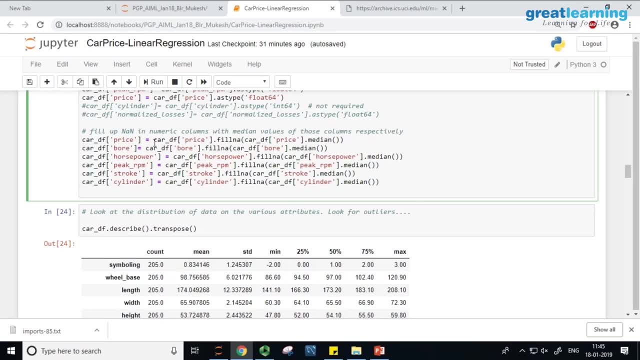 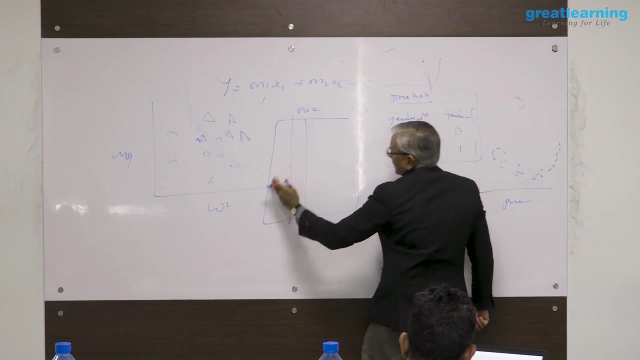 So the strategy I am using here for missing values is replace the missing values of price column with the median of the price column. I want to explain this step to you. So I have, I have a data frame and in this data frame I have one column. this column is call. 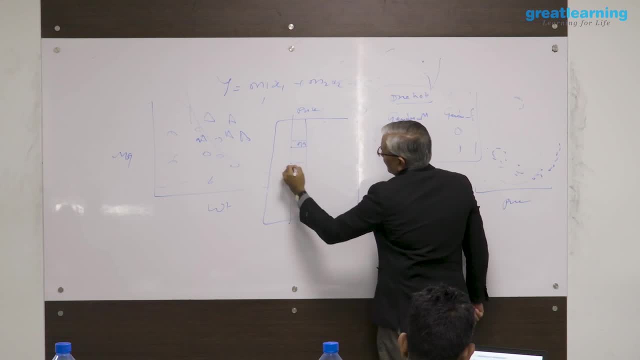 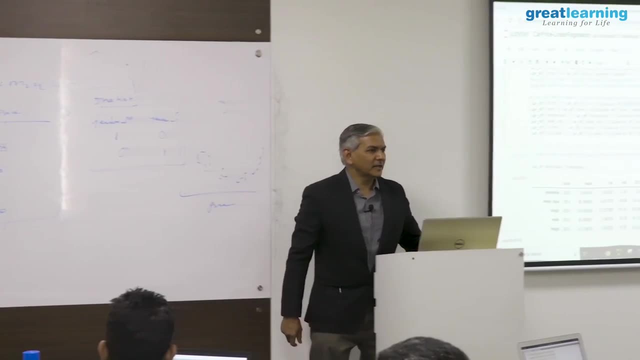 price. In this column there are many NAs: NA, NA, NA, NA NA. Wherever there are question marks, we replaced all of them with NAs. The question mark has been left behind by the data entry operator because when he was. 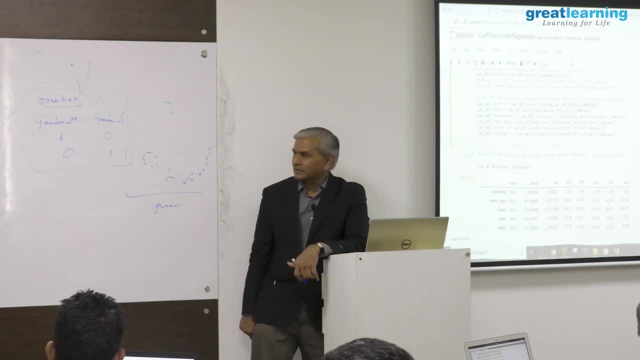 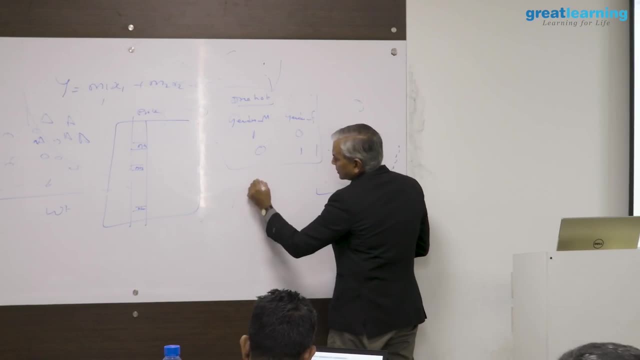 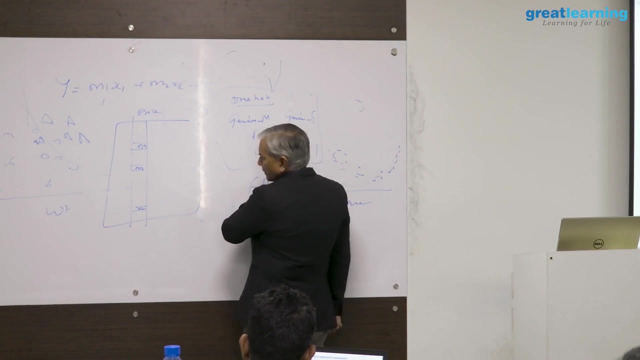 entering the data. he did not have values for those columns, those records, So we replaced question marks with NAs. all this became Ana. Because now these have become Ana, I can use the function fill Ana. What this function does is, if you see that syntax, what it done is find out the median. 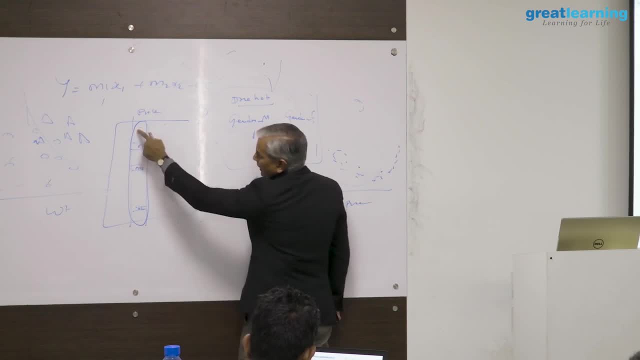 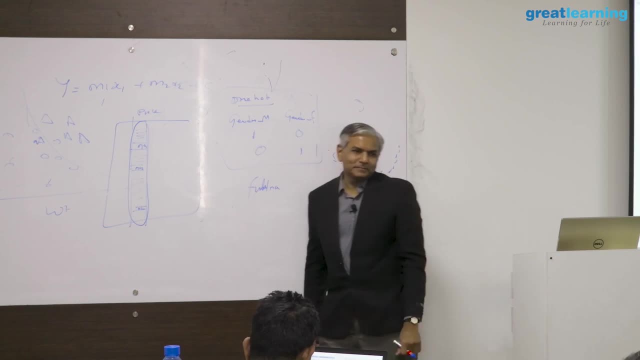 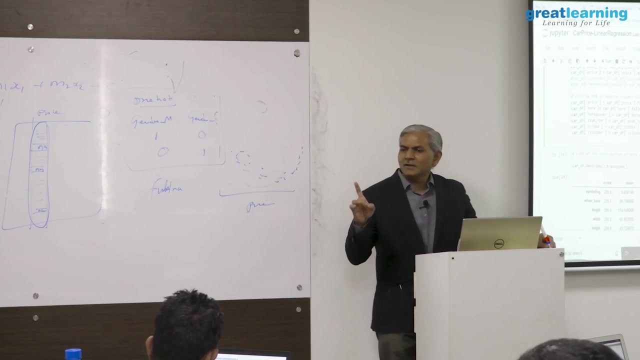 of this column. whatever values are available, using those values, find out the median. replace the NAs with the median of this column. It is always safer to replace missing values with Na- sorry, missing values with median- because means they are easily impacted by outliers. 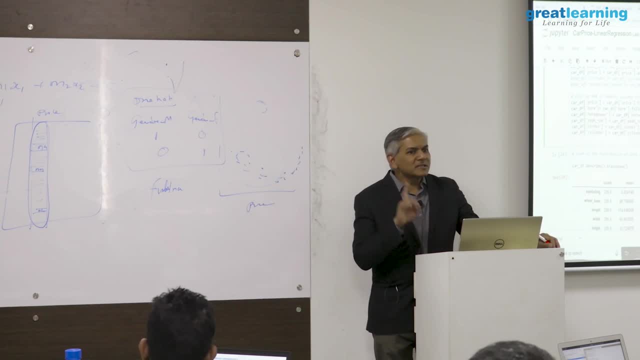 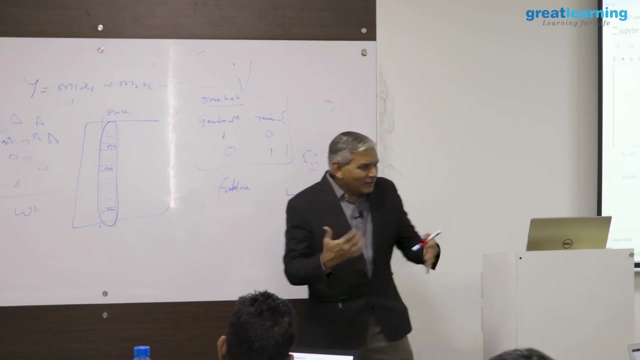 Ok Mode is using categorical variables. we are running with float variables So we always replace mean or median, but we are not yet check the outliers. all columns will have outliers. mean get easily impacted by outliers. So if you replace these values with mean and go and replace, remove the outliers then 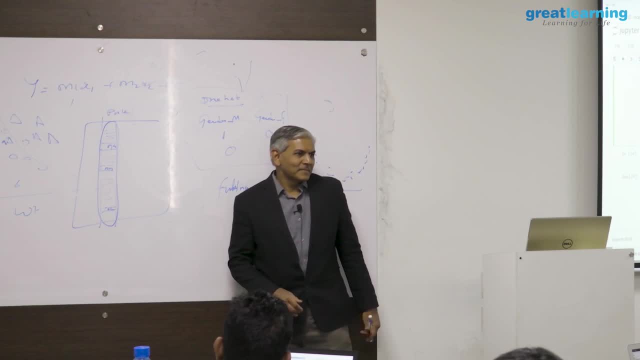 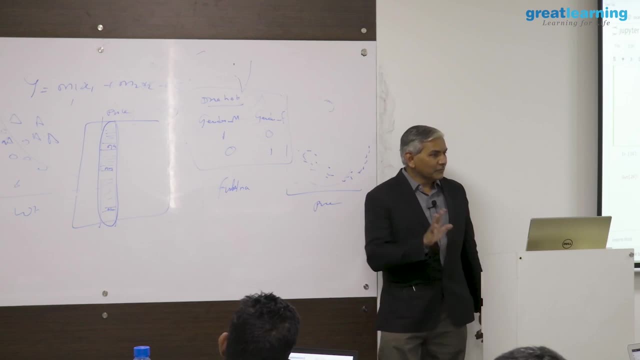 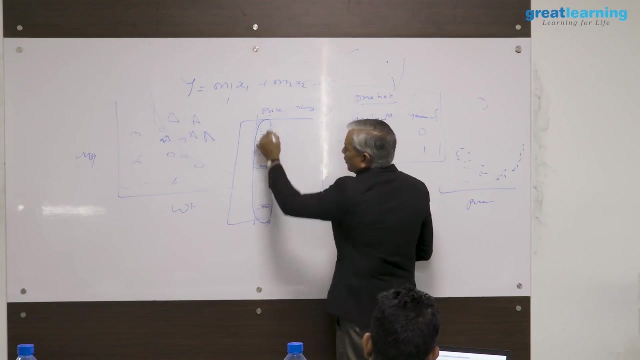 these values will be completely incorrect. So replace with median median is not impacted by outliers right. And the beauty of this is: in scikit-learn I can find median of even an object column. The column is supposed to be numeric but because it has question marks, the data frame. 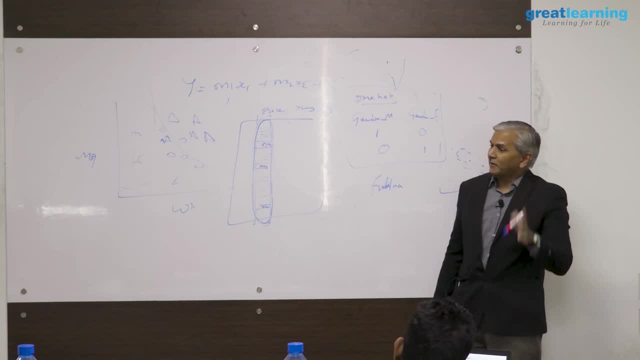 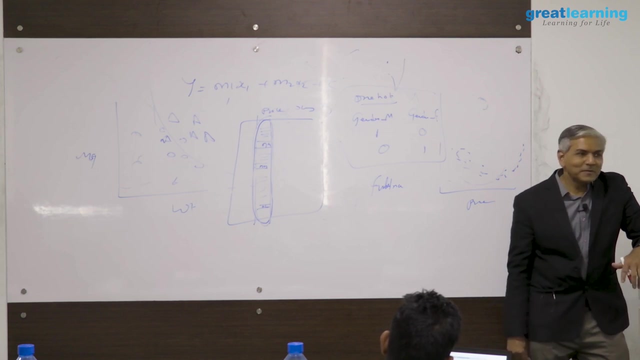 is converted into the object data type. But you can still go ahead and find the median of that column. why? Because median is physical central value. Mean is mathematical average. It is a calculated central value. You cannot find mean of an object data type. 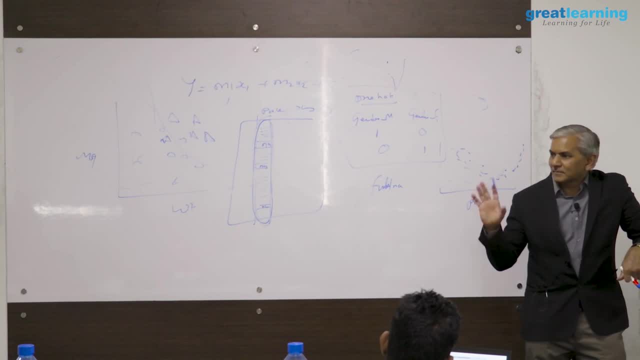 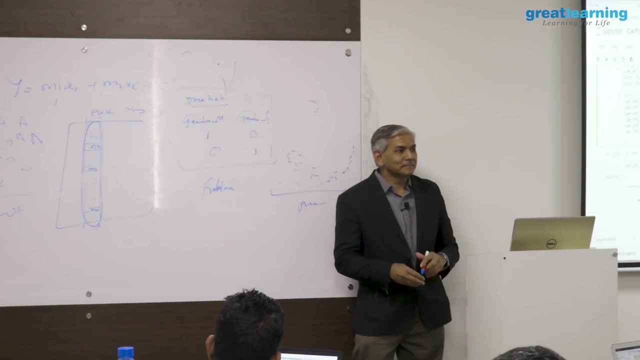 You can find median of an object data type, right? All of you getting the difference. That is where the difference between Python and R comes. In R, I will have to first convert in numerical value, even to find median. Now how do you, how do you address missing values? 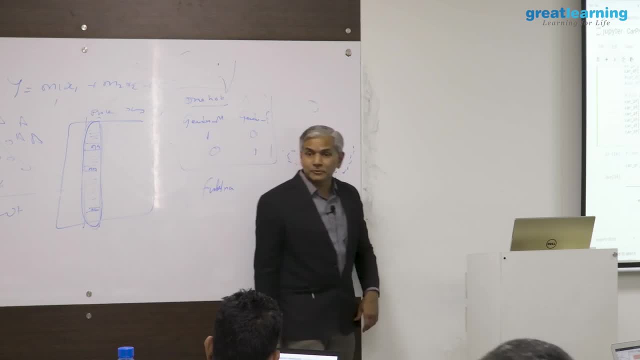 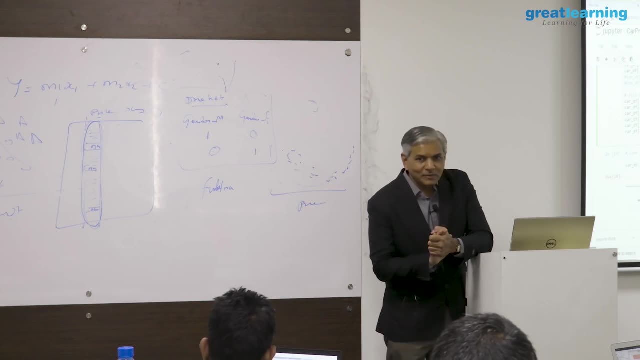 Ok, Ok. How do you address missing values depends on your analysis of the data and why the values are missing. The values can be missing because of some random reasons. We call it randomly missing values- Values which are randomly. you don't see any patterns in them. 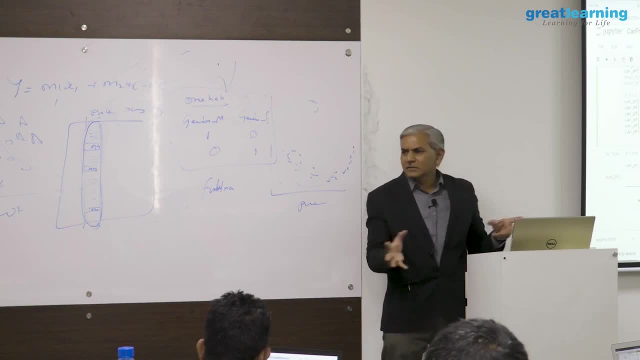 They are missing values in all records, in all columns, randomly distributed. Then we say that data is missing at random, There is no particular reason for it, Ok, Whereas there can be situations where the values are missing because of some reasons. They are not because of randomness. 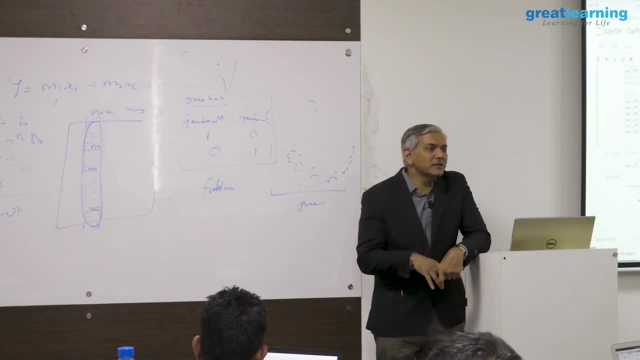 For example, if you take income, usually you will find nobody wants to disclose their income, So you will find missing values in that income column, many of them. So depending on what is the reason for that missing is, you will apply different strategies. 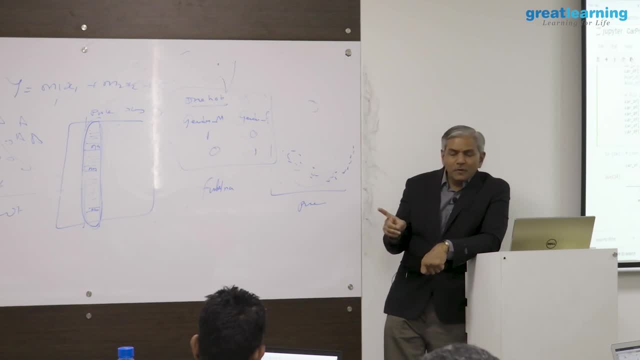 If the it is income column where the values are missing, column where the values are missing because of the nature of the column, then I might have to build a sub model, a model inside a model, where I predict the values of the income based. 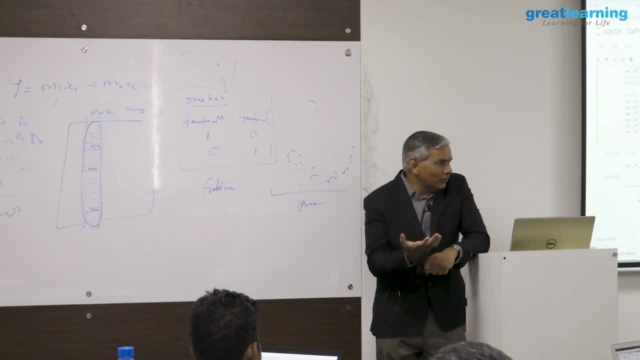 on the other attributes available. So my domain knowledge will come into play, which will help me understand what is the other attributes that this income column is going to rely on depend on. how can I guess it So whenever I create such imputed values? 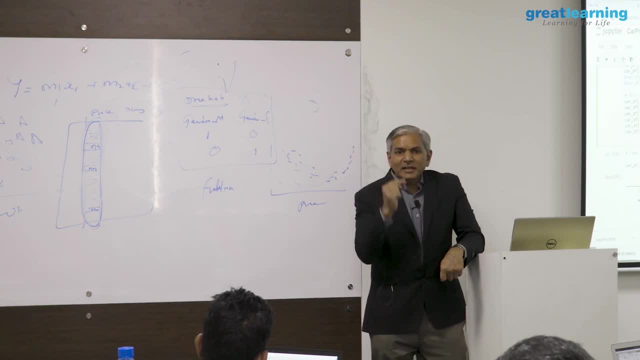 as we call them. I will create a new column, income imputed, So I will not touch the original column. I will create a new column called income imputed, where all the data available is copied as it is, including the missing values, and the missing values are imputed from the other. 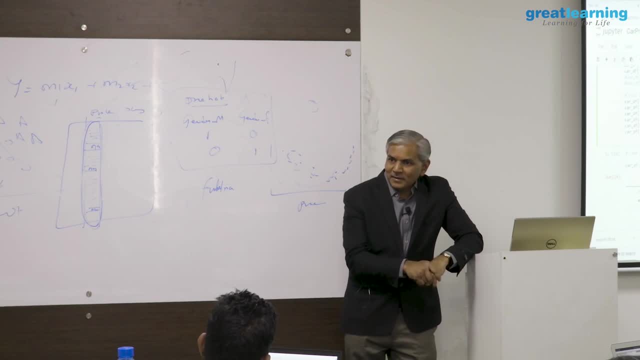 columns. that is one strategy. If your data is missing at random, then replacing the column with a medium is the default strategy we use. Look at the spread of the data on that column. if you see long thin tails mean is not reliable. so we replace with medium right. 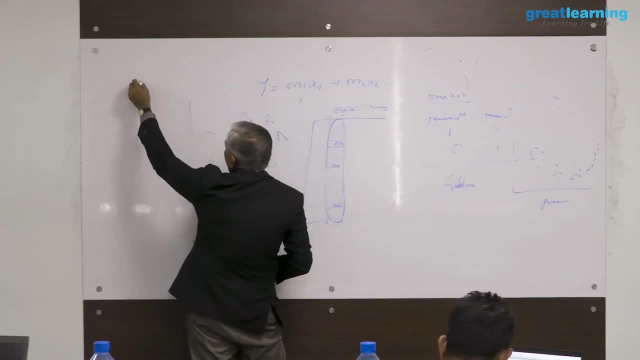 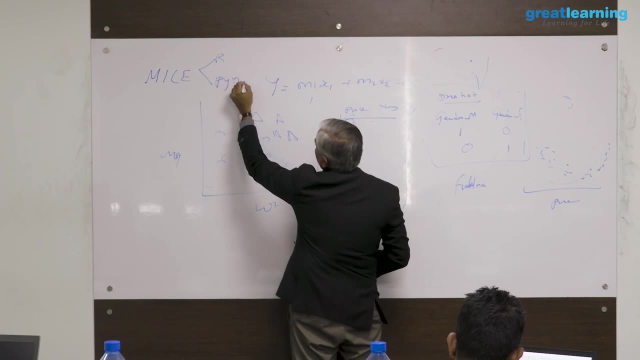 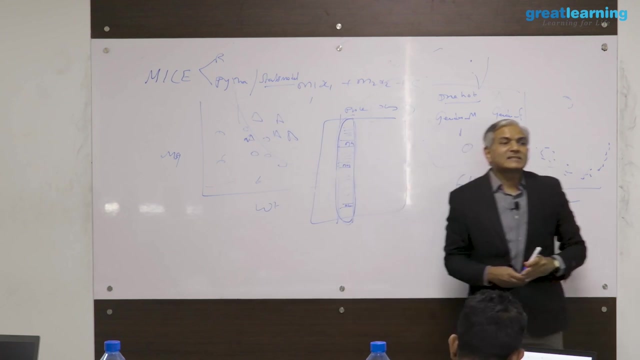 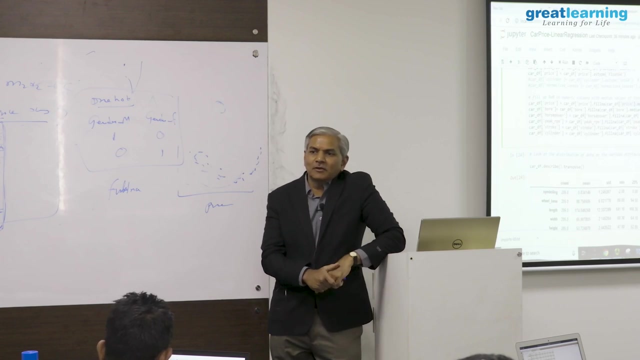 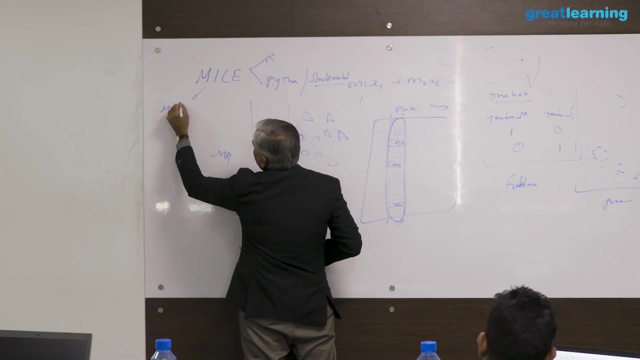 There is a package available called mice. it is available both in R and Python. In Python, it is available in another package called StatsModel. StatsModel Mice stands for multiple imputations through chain equations. multiple imputations through chain equations- right. So the piece of lemme. 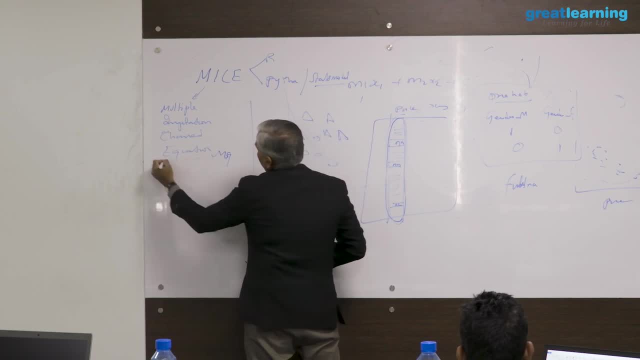 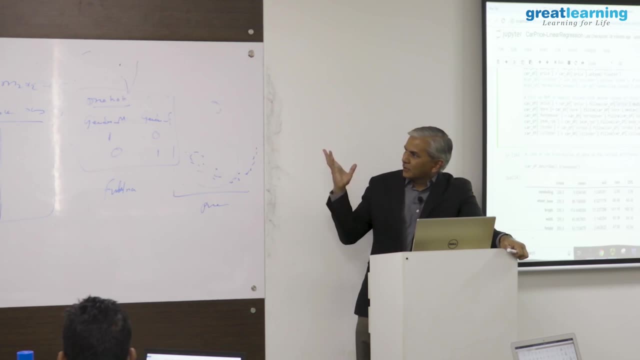 Yes, when you run this what you call package on your data set, it will automatically try to replace the missing values in all the columns with predicted values. where predictions will be based on the other columns, it will establish the relationship. it will see which one is. 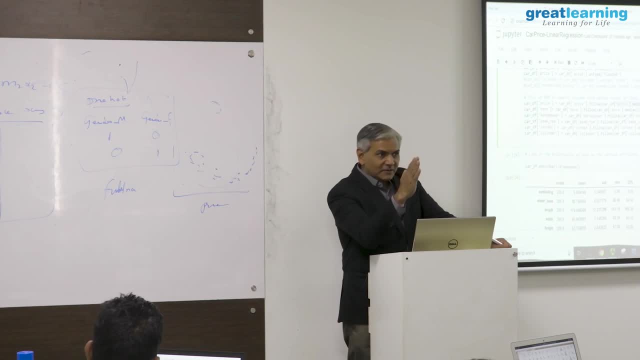 the strong relationship it will go and impute. So one column's missing value might be imputed multiple times from multiple columns. Please go and read about this. it is a very powerful package. When something comes with power, you have to be very careful in using it. 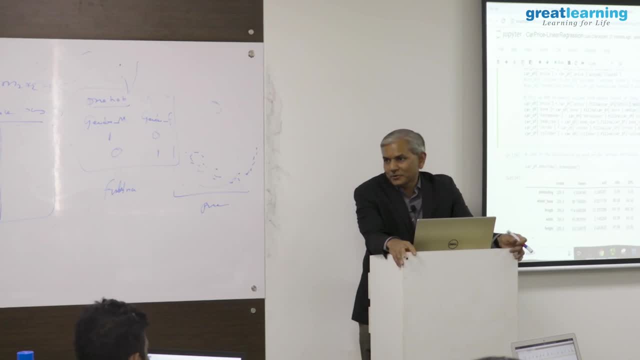 So read about this MICE. I am not going to cover it here, but it is a very beautiful package. you should read about this. And just to add to the confusion, apparently the MICE implementation in Python is very slightly different from MICE implementation in R. Now they both call it MICE. 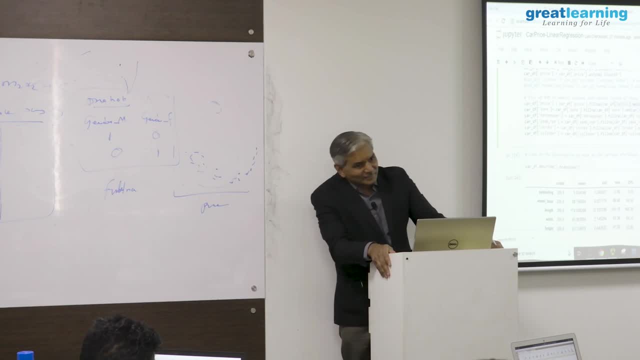 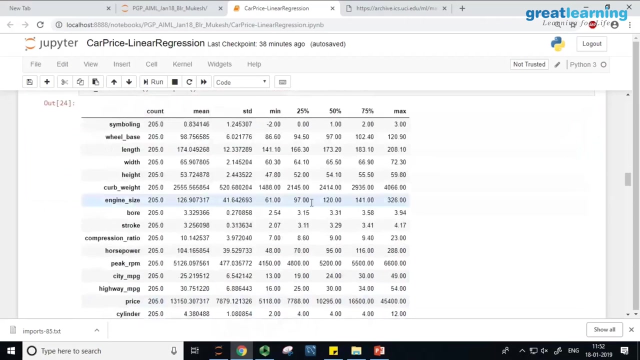 Suggest a lot of things also: low values and automatic drop. So these are the tools that you should be aware of. you should have in your portfolio when you start doing data science projects. All right, all of you think on this. shall we move on? 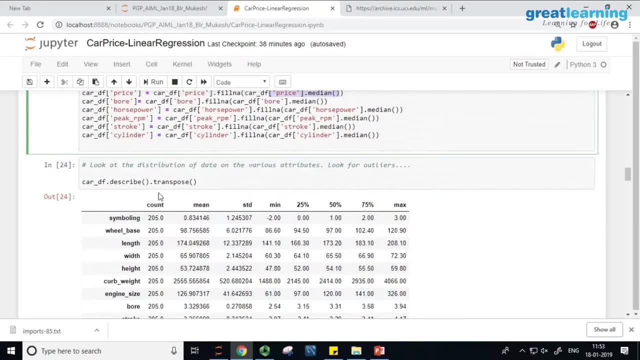 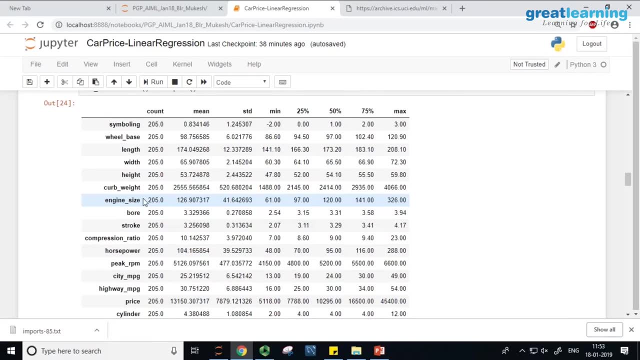 Once I have done this, then I go and do my basic statistics. div describe- Describe the descriptive statistics, and you know how to interpret this. All of you are aware of this. Take any column, say height of the car. first thing you should look at is difference between 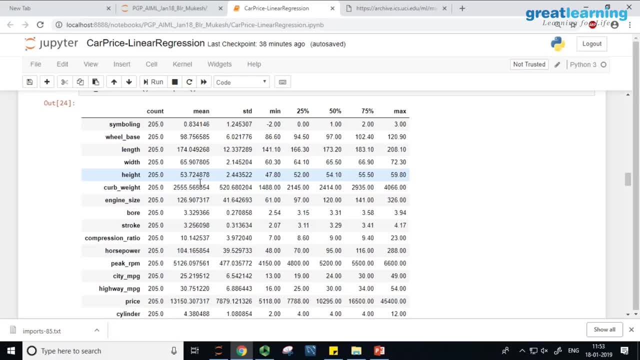 mean and median. The mean is 53.72,, median is 54,. not a very big difference: 53.72 and 54.10, not a very huge difference to worry about. Look at the distance between. 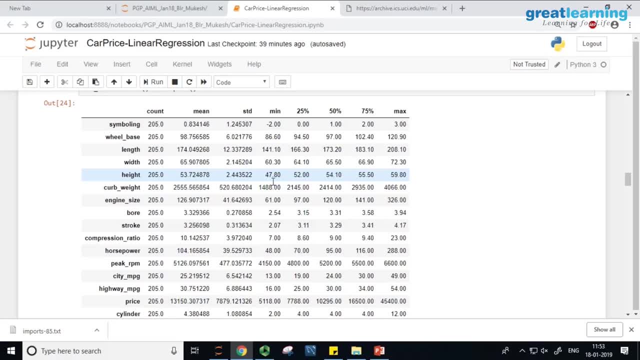 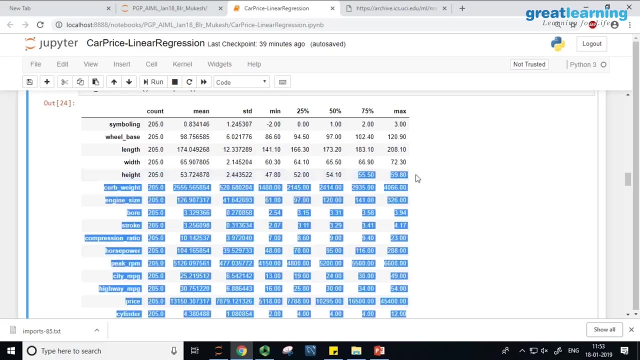 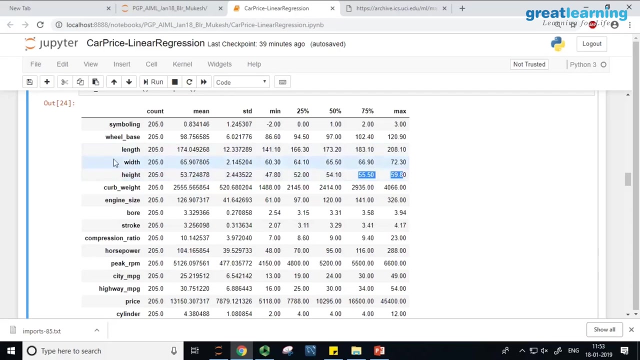 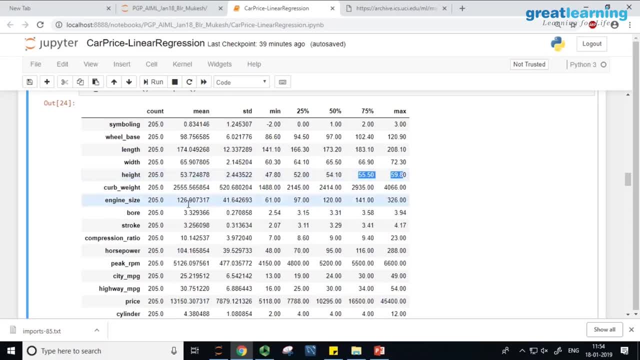 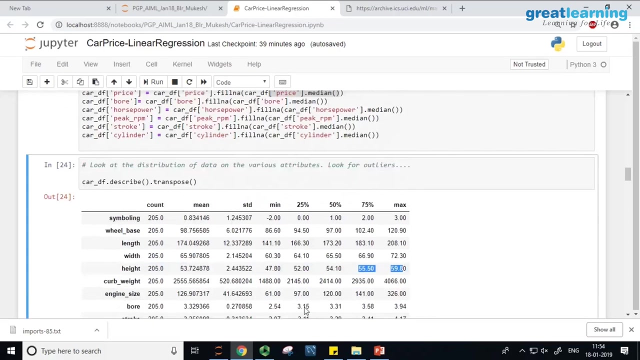 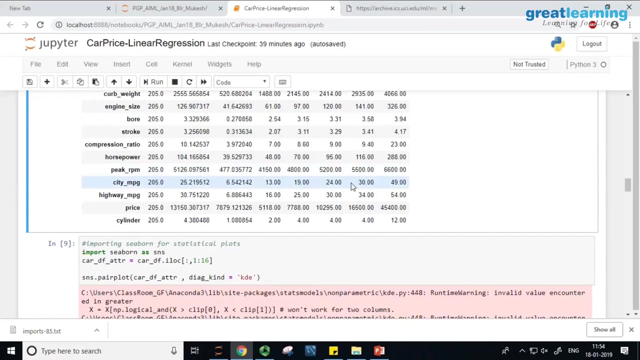 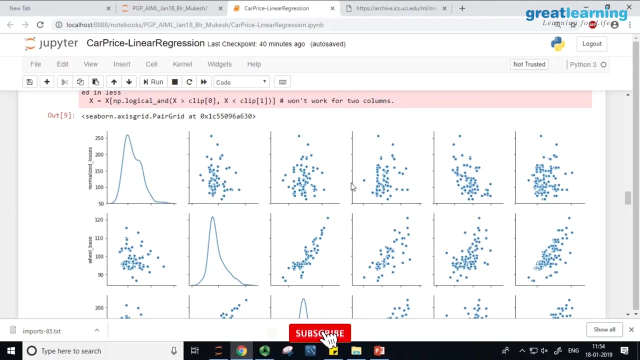 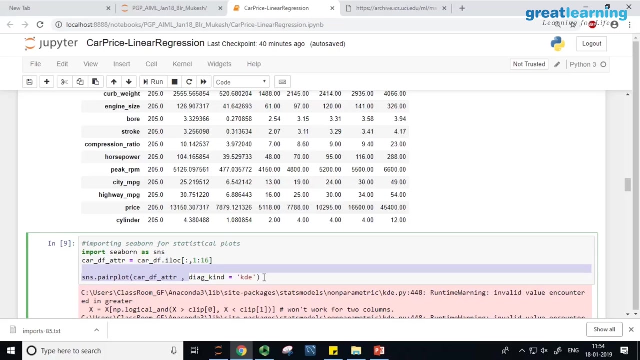 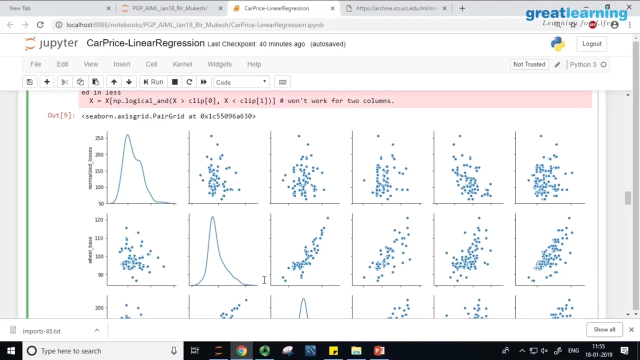 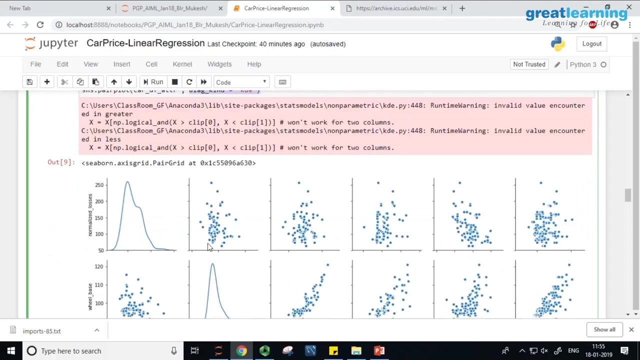 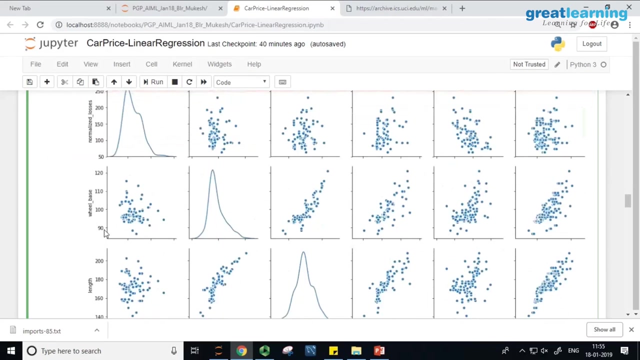 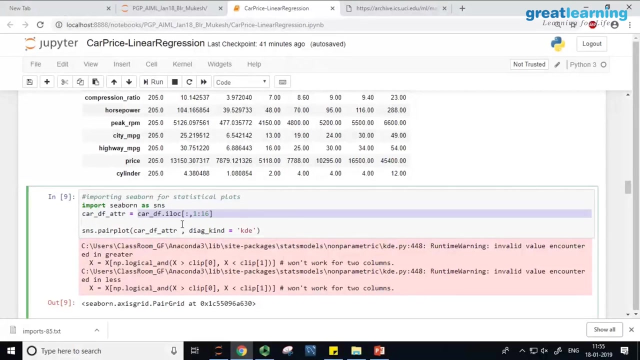 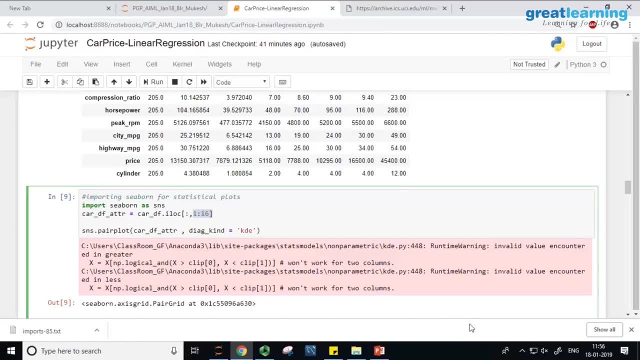 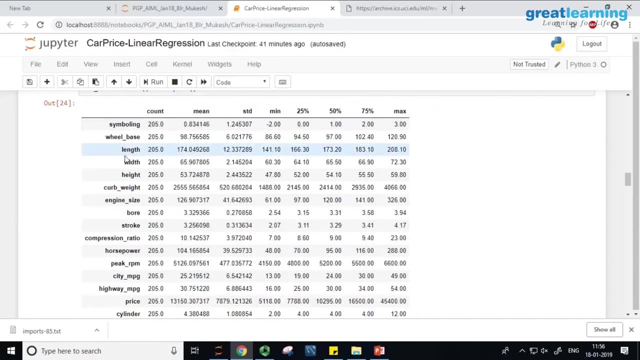 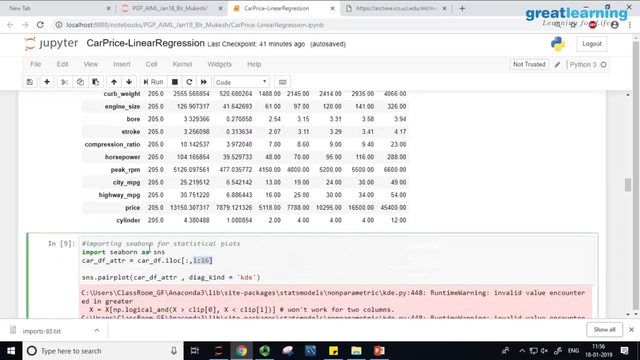 all rows, column 1 to 16,. yeah, column 0 is my. column 1 to 16,. how many are there here? 4, 5,, 6,, 7,, 8,, 9,, 10,, 11,, 12,, 13,, 14,, 15,, 16,? I have not taken the price column here. 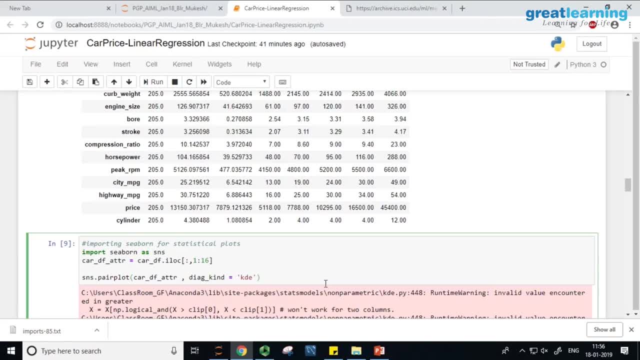 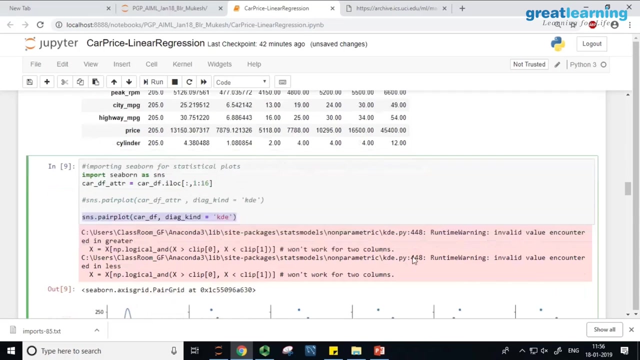 so what we do here is: instead of doing this, you do this, you do this. just knock comment this out. ok, snspairplot- car underscore df- kde. you do this. we will do this. pairplot. now we are done. 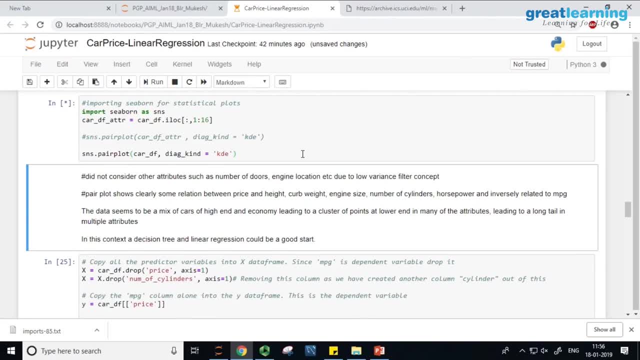 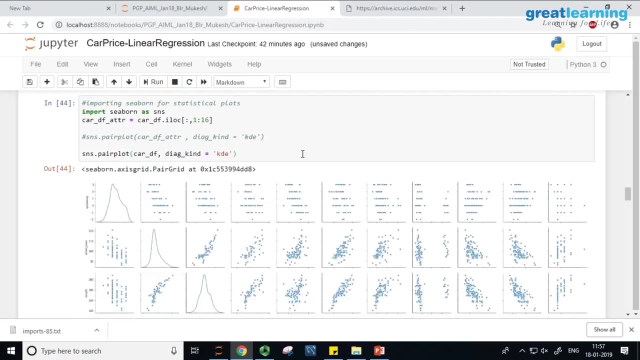 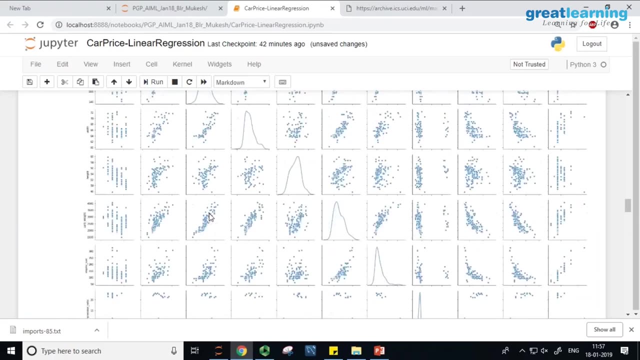 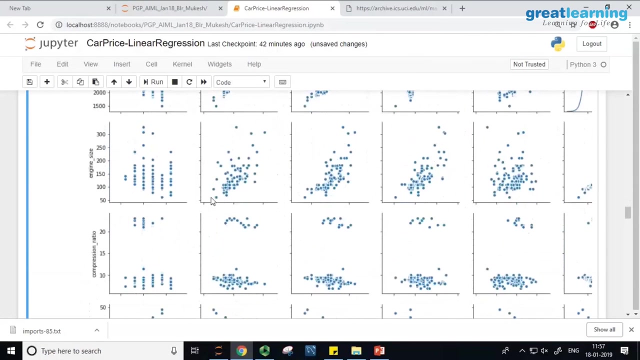 We run this, so let us let it plot. fortunately it is coming out fast. yes, sir, got it. now I want to make sure my price column is reflected here. we are going to predict the price, right. so price column is, I think, second last or something: cylinder, mpg, price column, price. 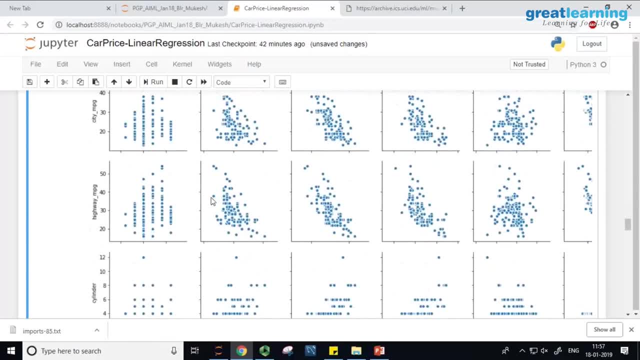 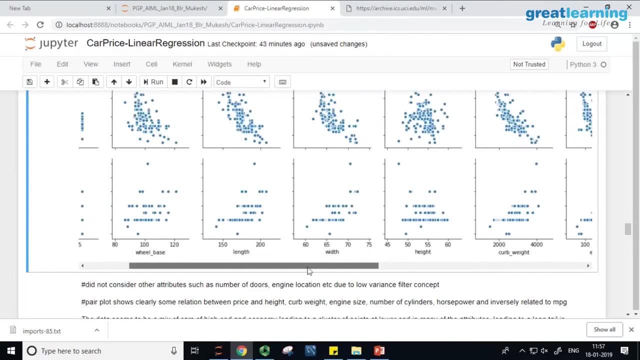 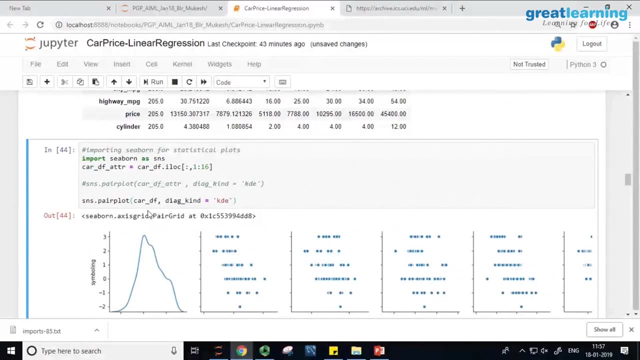 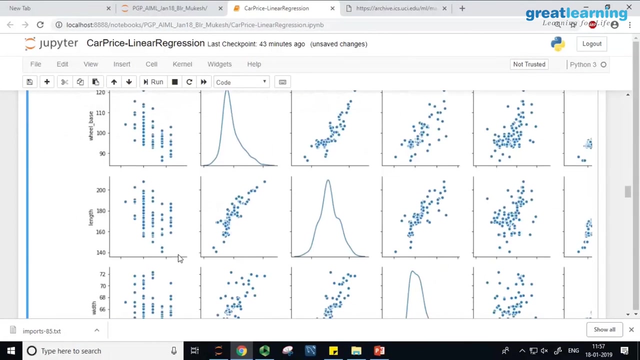 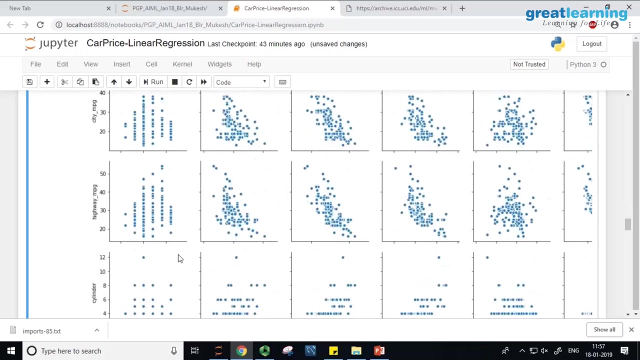 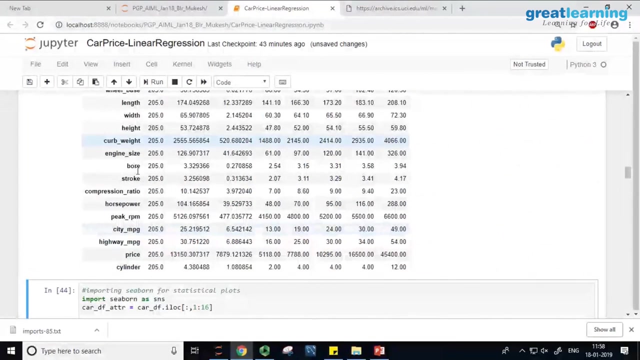 mpg. it is last but one. why is it not showing to me I am not getting it? one second, I probably did not. car underscore df. are you able to get the price column? yes, sir, yes, it is there in the data set. it is there in this price variable. car underscore df- describe. 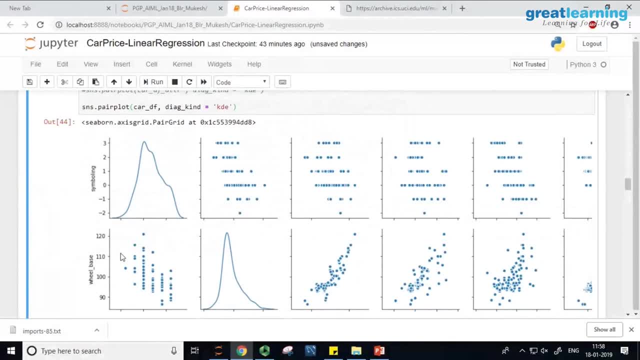 it is there in this data set, but you guys are getting it alright, all. ok, let us look at that. ok, The first thing that you need to do is when you do pairplot is first thing that you need. 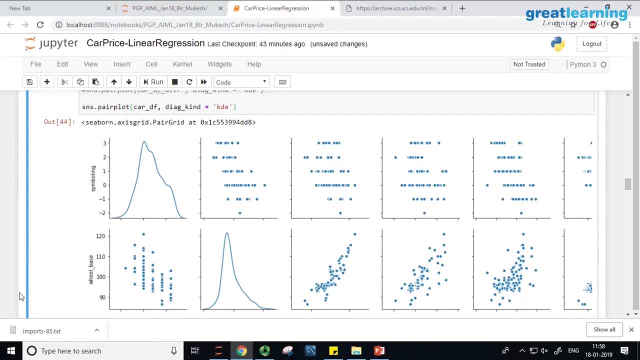 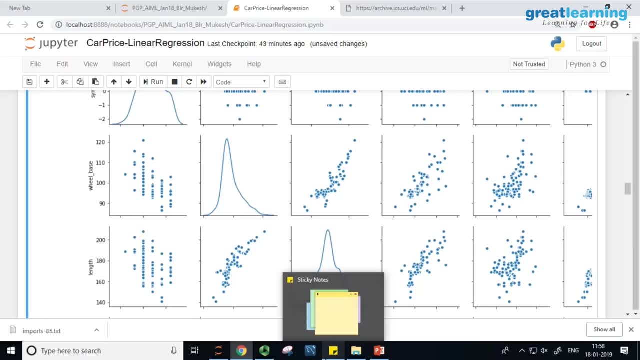 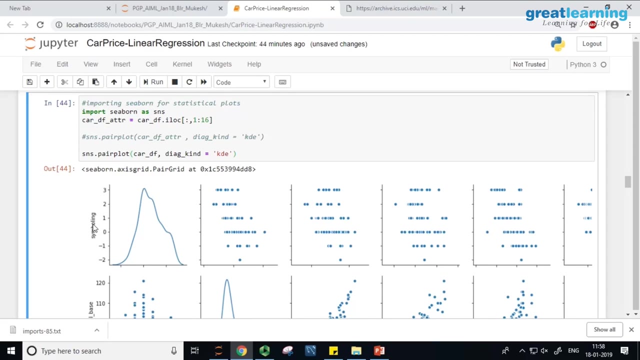 to understand is: first row and first column is same, Second row and second column is same, third row and third column is same, so on and so forth. ok, and when I do a comparison of a column with itself, if I do a comparison of 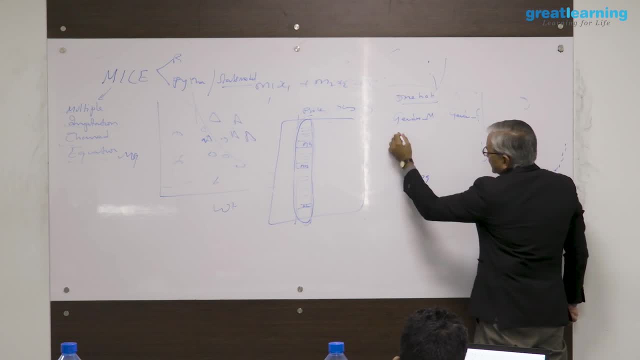 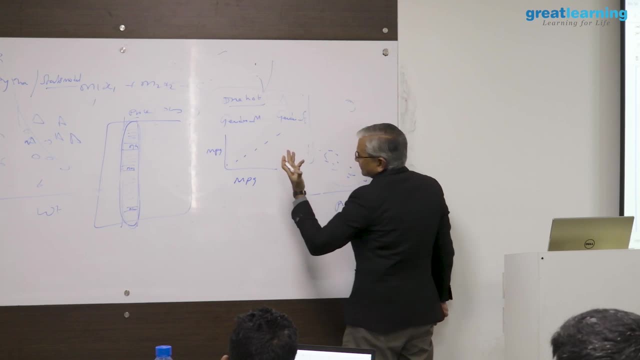 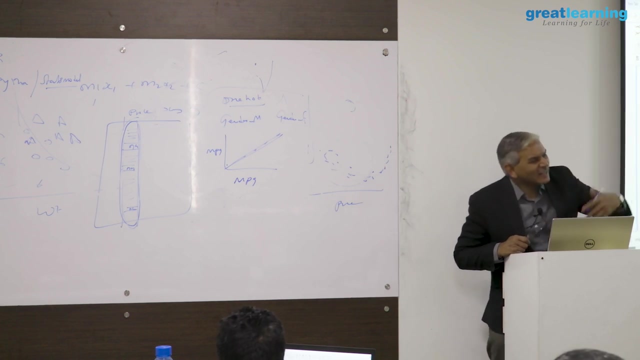 say mpg versus mpg versus mpg, what kind of a plot will I get? scatter plot, it will be a straight line. there will be no information here, there is no spread, nothing. So trying to do a scatter plot for a column with itself is useless. it is not going to. 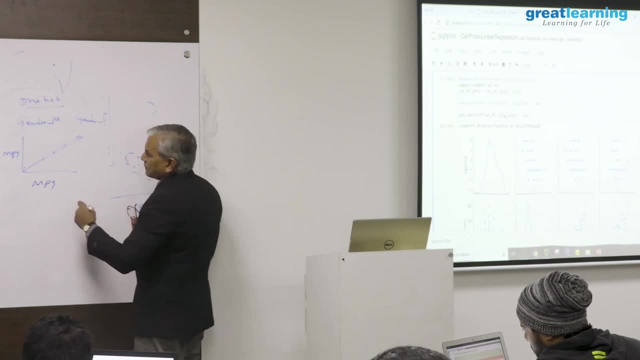 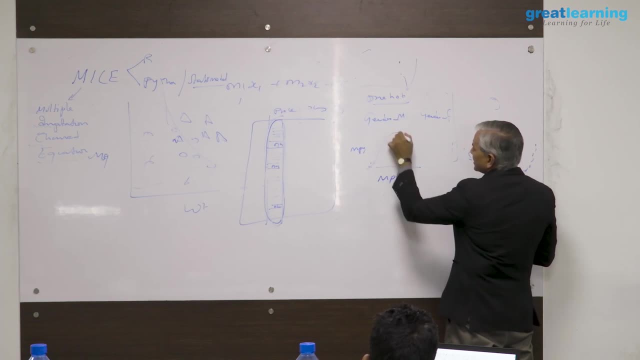 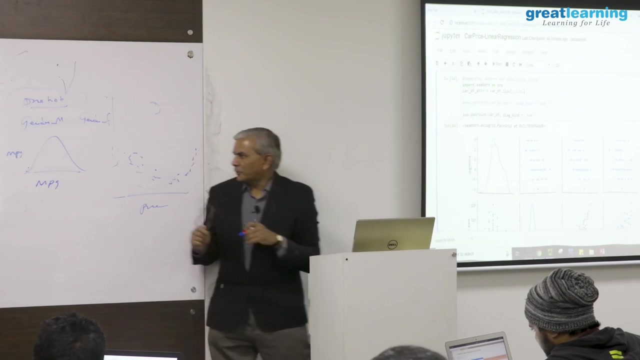 give you any information. So whenever it comes to that point where you are going to look at a column versus itself, what they have done is, instead of giving you scatter plot, they have given you a density curve. by default, they give you histograms. we have changed it to density curve. the advantage: 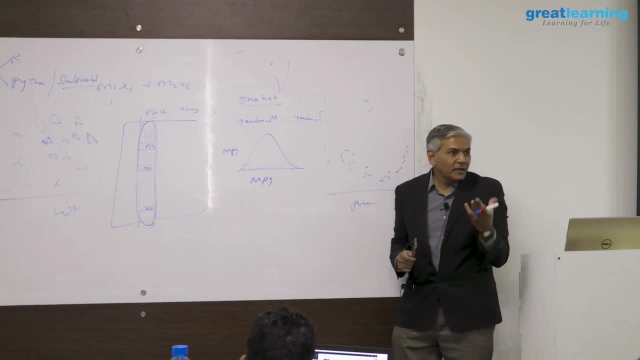 of doing. that is in R. if you do this pair plot, it will leave out the diagonals as blank. it will not show you anything there, whereas what happens in scikit-learn is they give you a distribution. why leave it blank? use it to show the distribution on that particular. 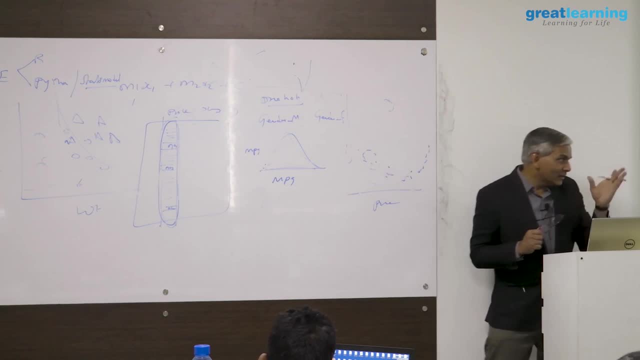 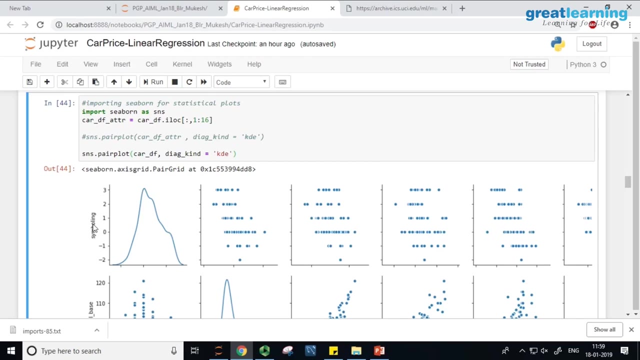 column. ok, so that is why diagonals, you will see the distributions, how data is distributed on that particular column. ok, So let us look at the first: the diagonals in the diagonals, in my case, first column. 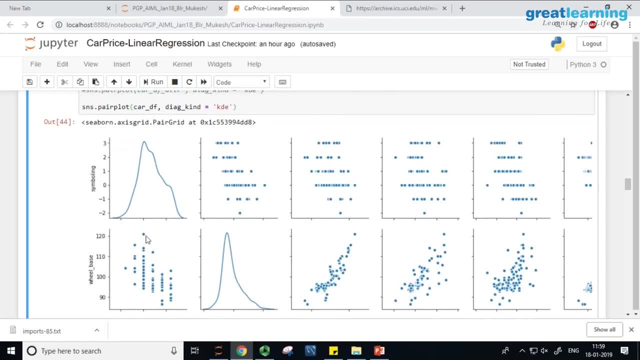 is symboling on its diagonal. Ok, Honestly, I do not know what symboling is. maybe I should have done that homework. Next column is wheel base. wheel base is basically how spread the front wheel and the back wheel the distance between them? ok, 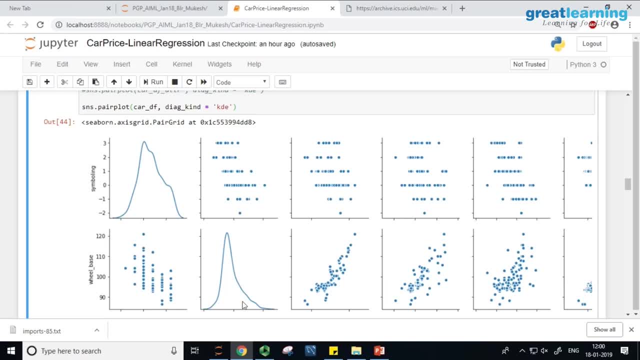 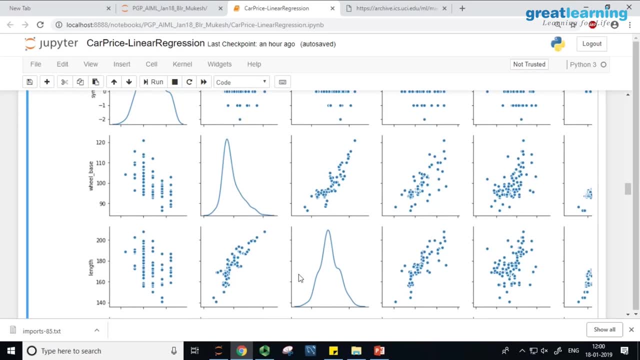 We see a normal distribution, except for higher values, higher values. there seems to be some kind of tail. does not look worrisome? Look at the length of the car. again, almost a normal distribution, but we see some kind of overlap here. 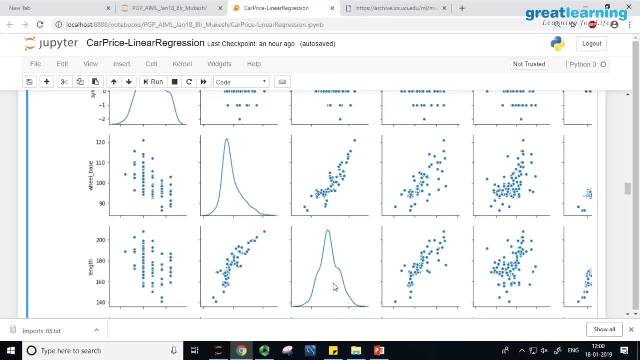 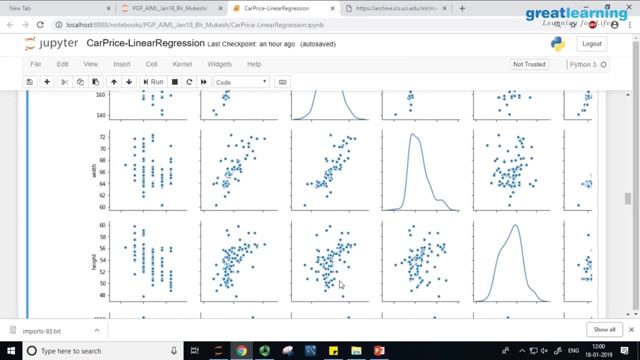 Between the, you see multiple gaussians here, one behind the other. may not be of concern right now, because they are all kind of overlapping. Remember which was the column where we saw perfect match, the central values. what is the column? 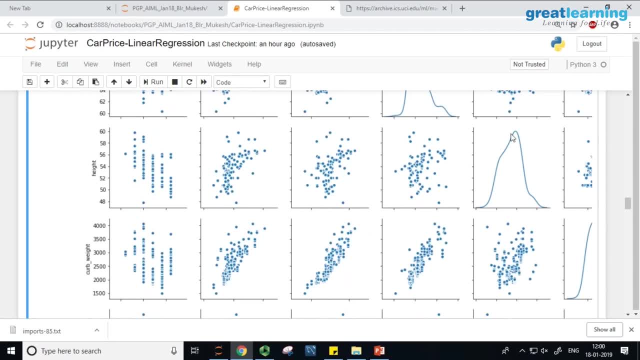 Bore: Height, Height, Height was the column. This is the distribution of height. So in distribution of height now look at this- the distance between mean and median was almost very nil And the tails were also equally spread. We were expecting a normal distribution, but unfortunately it is not normal. 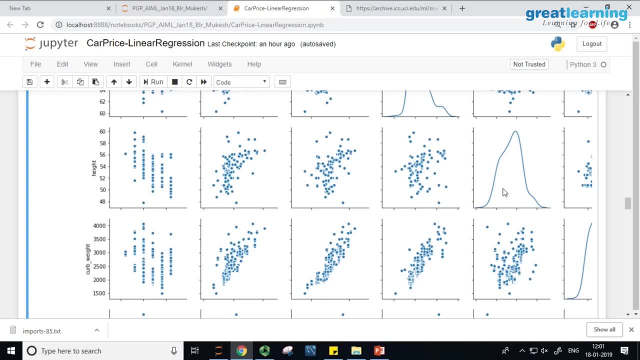 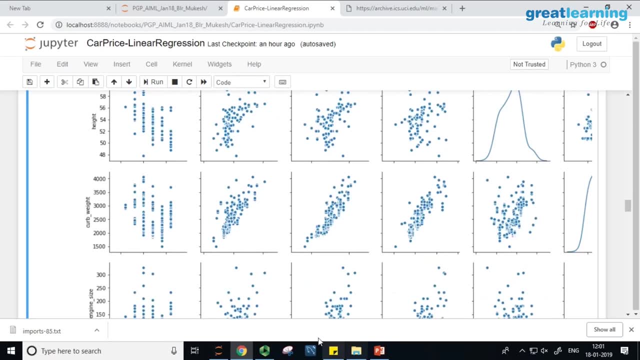 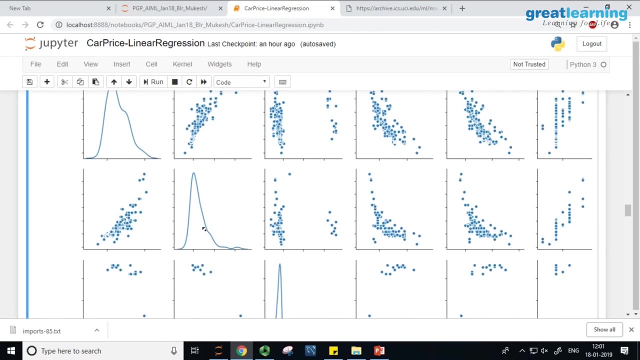 What it is showing here is two gaussians. two normal curves are overlapping each other. ok, This is what we call the mix of gaussians. Go to the other columns. look at this one. this one has a long tail on the right side. 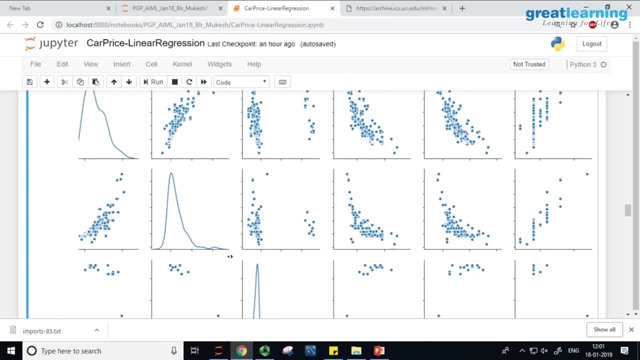 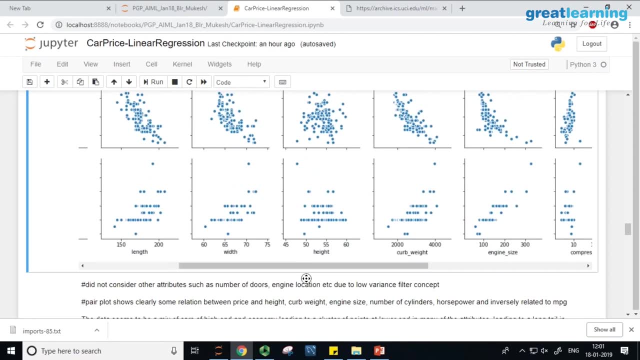 a long tail It also seems to have, but these gaussians are ignorable. they are very small compared to the other one. ok, So look at the distributions and, on the distribution part, on each and all columns, some concern. 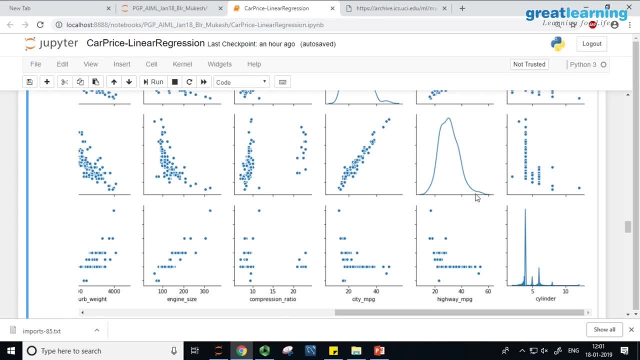 but not too much to worry about. You should never expect a theoretical symmetrical normal curve in the distributions. All algorithms assume that the data on the independent dimensions are distributed normally. Ok, That is all they assume. apparently not so, but still it is close to normal, so I am happy. 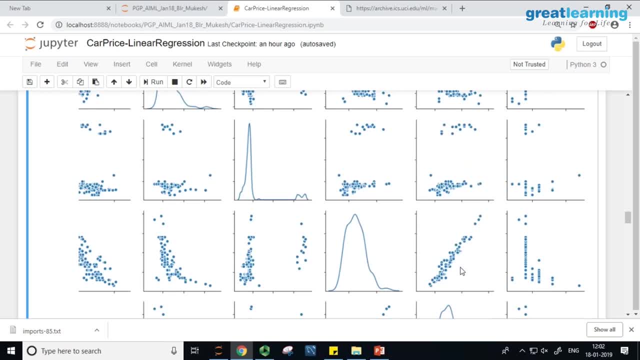 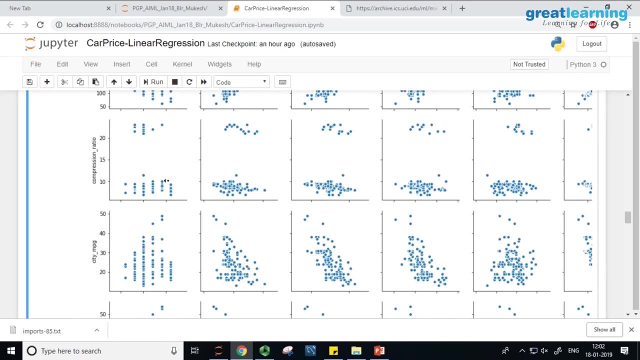 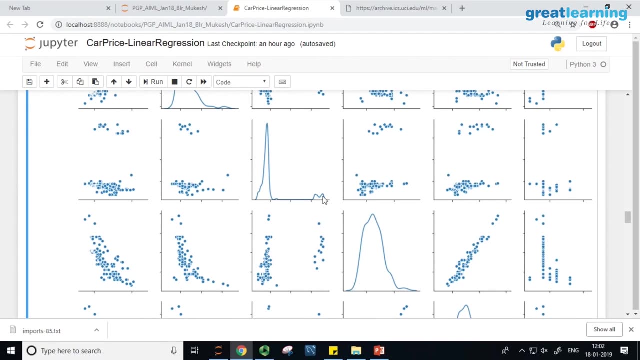 with it. Can you explain the compression ratio of that one, This one, This one? Ok, Compression ratio. you see here, this is compression ratio and compression ratio. what I am seeing here is there are two different clusters in it, two buckets in the data on that particular. 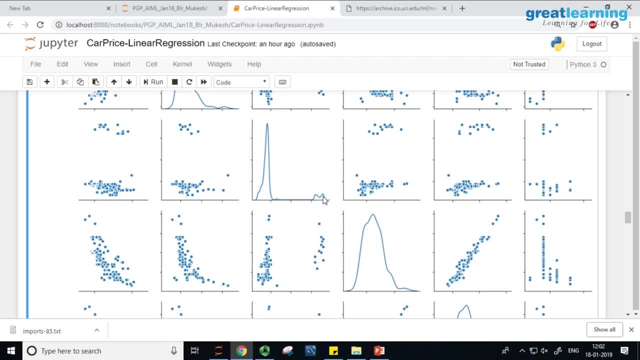 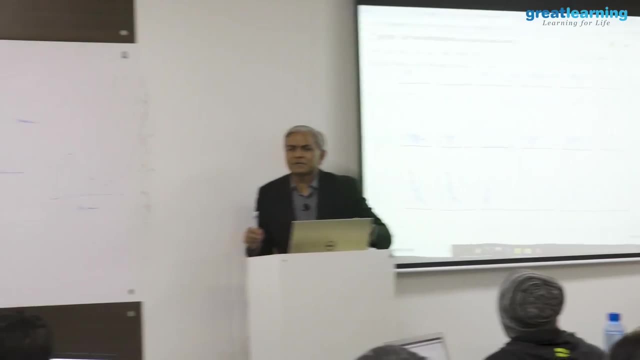 dimension. Ok, This is a clear indication of mix up of gaussians. When you build models, especially linear models, you should not mix gaussians. Every gaussian has a particular characteristic. What do you mean by gaussians? Gaussian means distributions. 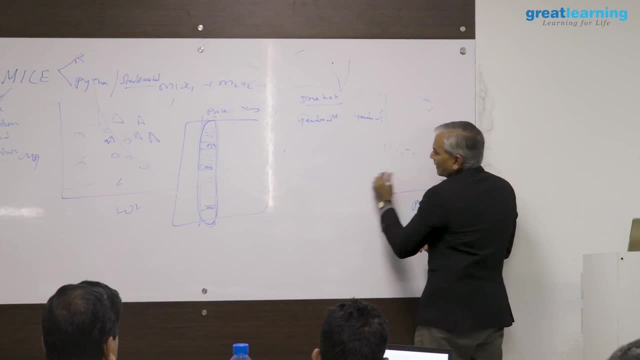 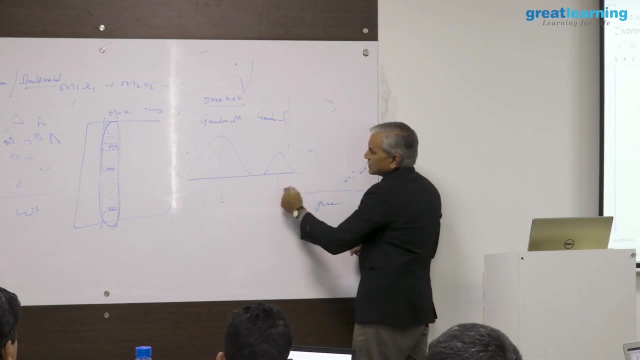 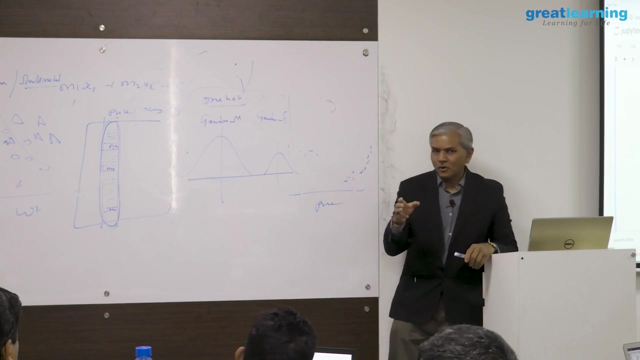 Ok, So if on a particular dimension you have two different distributions, you are talking about two different processes which have generated this data. Ok, Remember, in statistics you would have done a t-test or a z-normal test. when do we say: 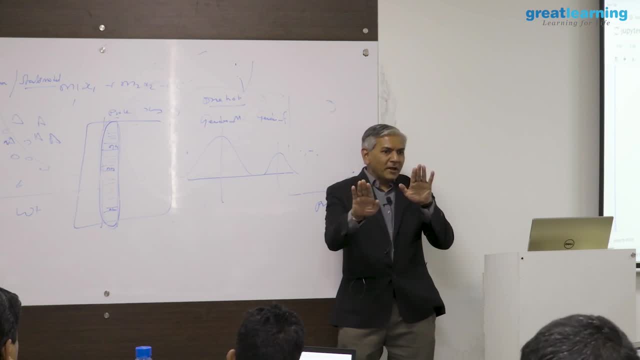 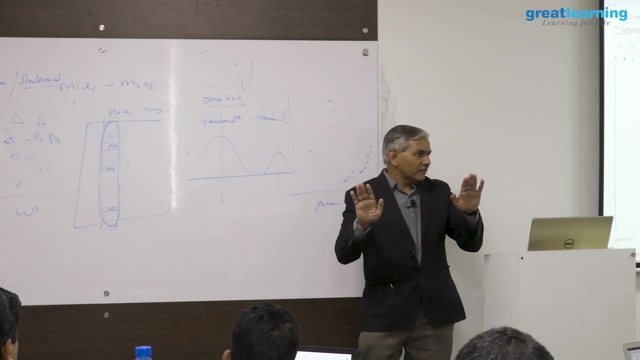 the two datasets belong to the same process. When they are significantly overlapping each other, the central values are not very far away from each other. If the central values are very far away from each other, likely that the two datasets have not come from the same source. 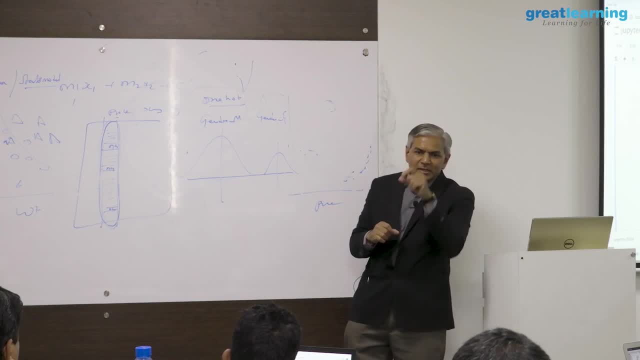 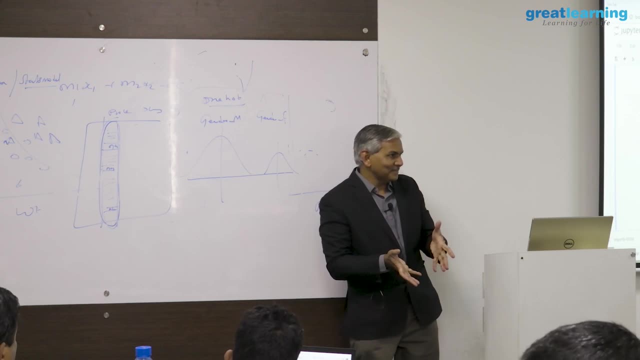 If the two datasets have not come from the same source, how can we include them in one single model? What is a model Model is predicting the behavior of the source, the process which generated the data. Right, What happens when you use mix up of gaussians like this is you are going to find x bar. 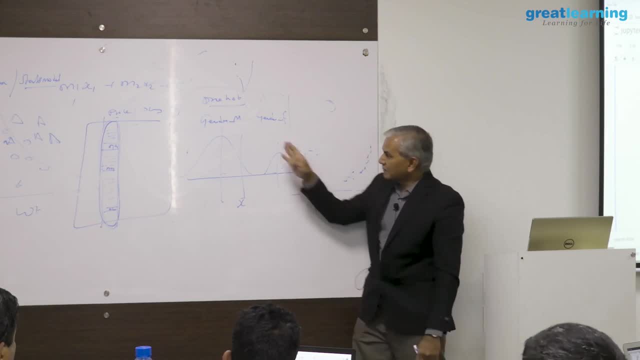 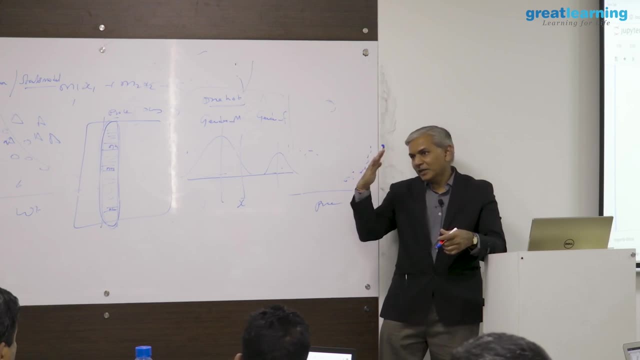 x bar is going to lie somewhere in between these two, which neither represents this nor represents this, But your linear model is going to go through the s bar x bar, so your linear model will neither be good for this prediction nor will be good for this prediction. 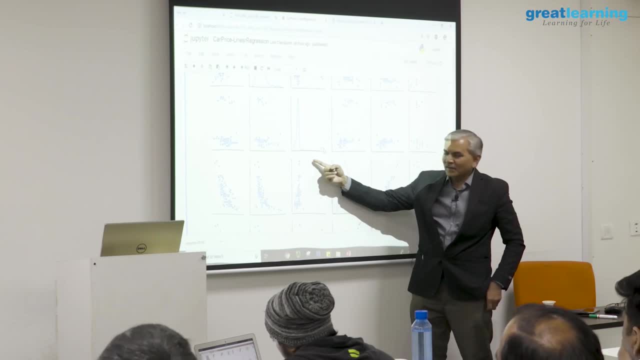 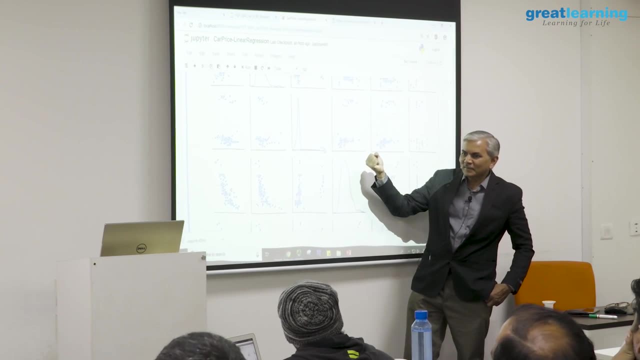 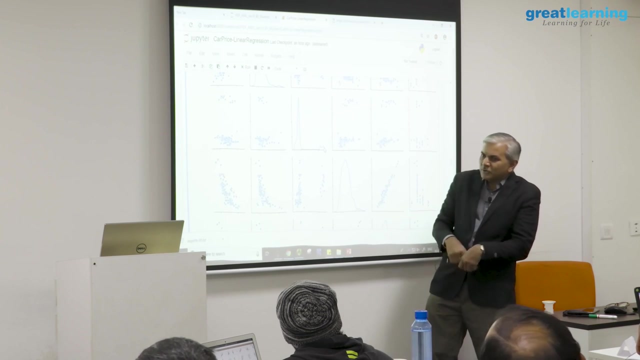 Ok, He has done some typo, hence lot of typos sitting on the extreme end. This happens when you measure these terms in some fractions, and he has either added one extra 0 or something of that sort he has done, because of which you are seeing outliers. 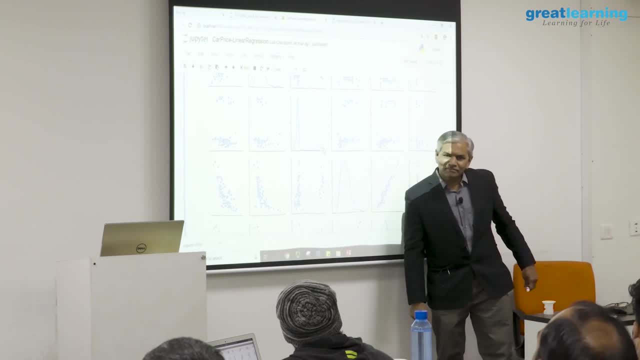 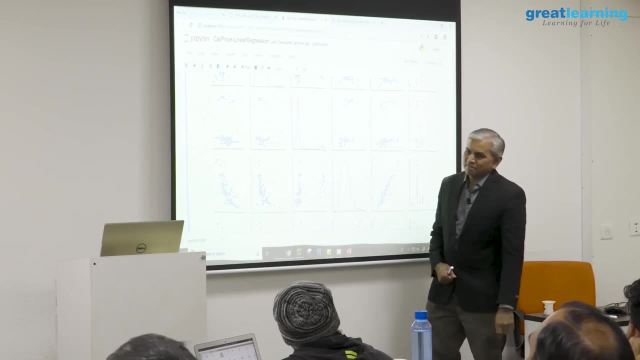 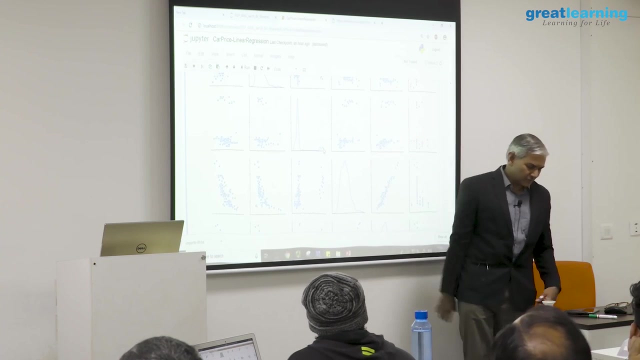 cluttered together in one group. So I have to go and find out what are these records? which is causing this long tail in this cluster? My hunch and experience tells me this is most likely a typo rather than data coming from two different sources. 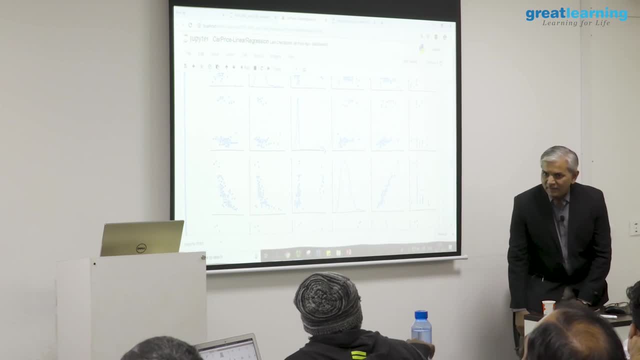 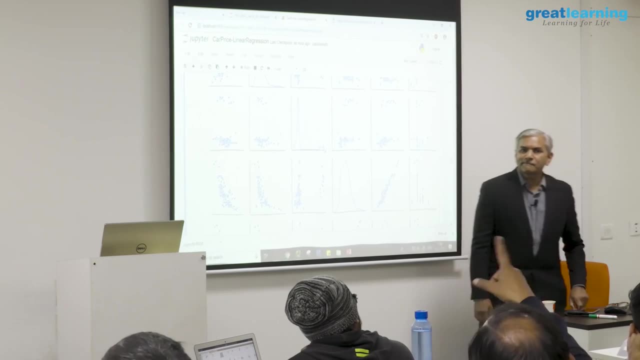 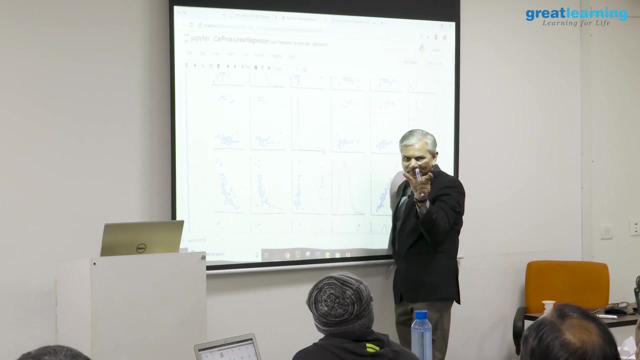 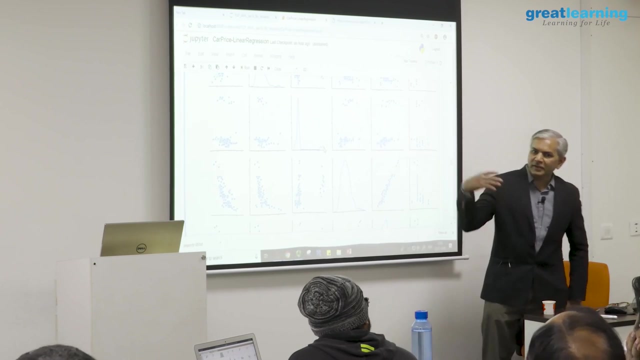 How do you identify the proportion? Go and put 1.96 standard deviation limit. Yeah, this is outliers. Ok, Outliers, Outliers. So I can detect anything which is lying beyond 1.96 standard deviation on this dimension. 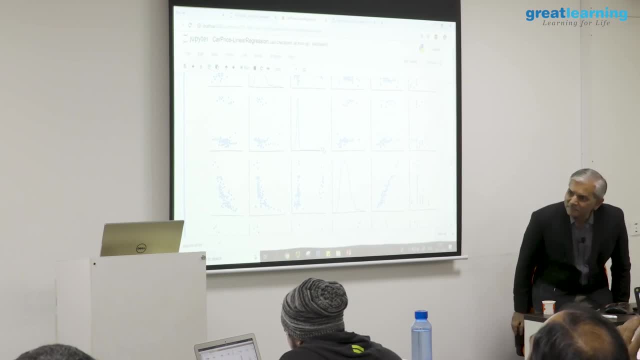 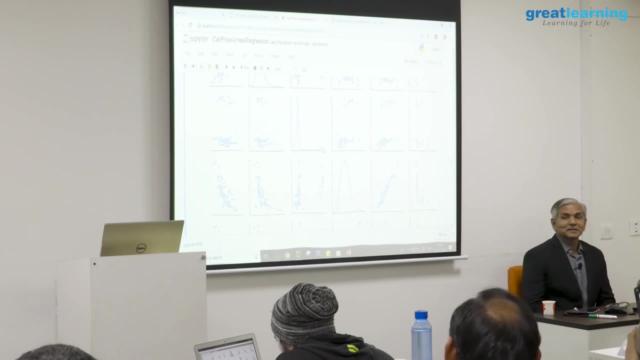 Sir, I can identify these two, But standard deviation will be given for the complete observation right. But that includes data of the Doesn't matter. Doesn't matter As long as they are beyond 1.96,. they are suspect. 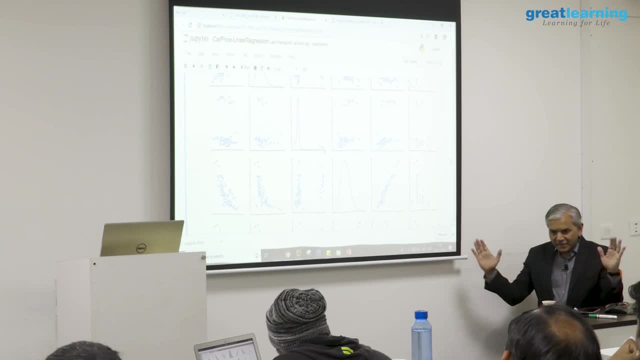 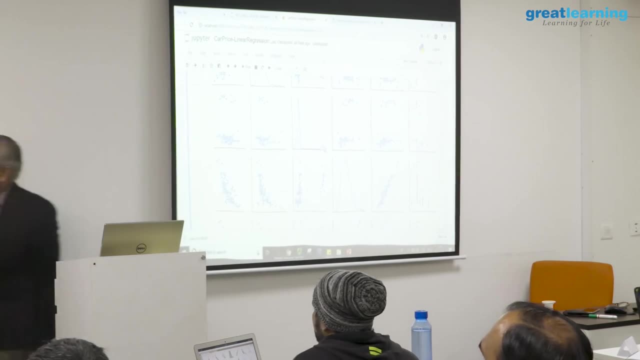 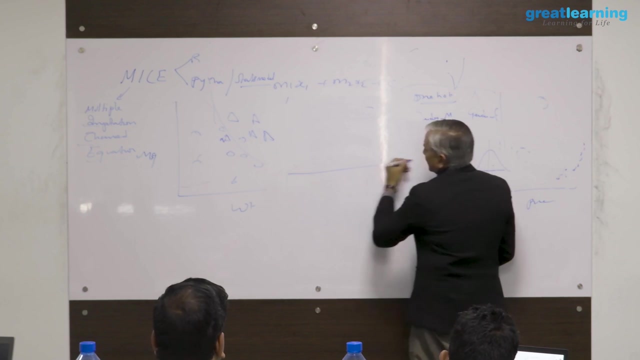 So when you replace those outliers with values, proper values, then your standard deviation will collapse. Ok, I think the cylinder is the best example for what you are describing. I will look at this, Guys. since this point has come up, I will discuss this. 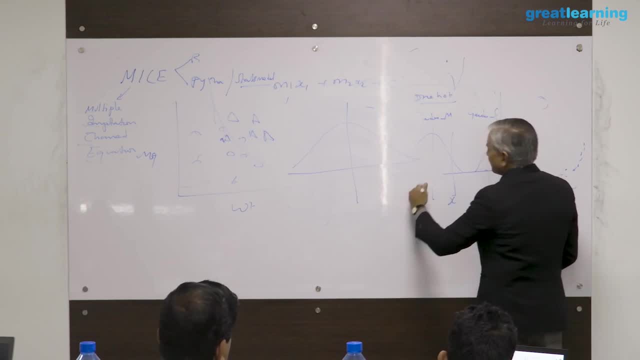 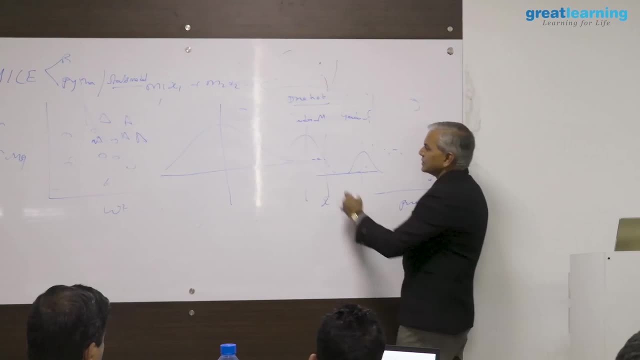 In your original raw data set. suppose it is, beautifully, you have outliers here. You do something about the outliers, You identify the records and replace all these values with the median. suppose you do that. Ok, When you do that, you remove the outliers. You replace all the values with median, Your curve will become sharper. When the curve becomes sharper, standard deviation decreases. When standard deviation decreases, the data points which are earlier not outliers, now they become outliers because your standard deviation is decreased. So 1.96 standard deviation- both sizes decreased. 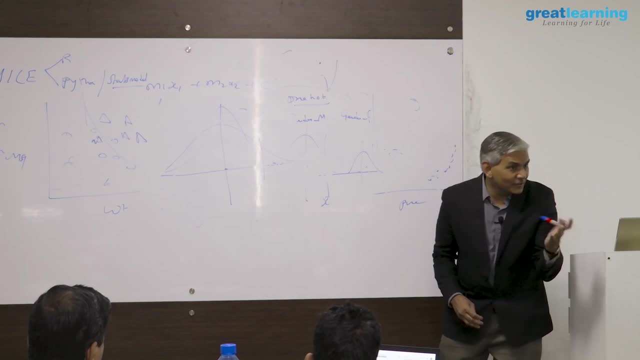 So new data points will come out as outliers which earlier were not identified as outliers, And this will come out as outliers. So 1.96 standard deviation, both sizes decreased. And this will continue to go on infinitely. So just handle the first level of outliers. 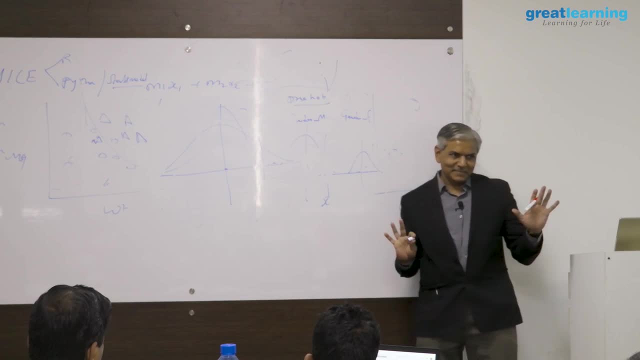 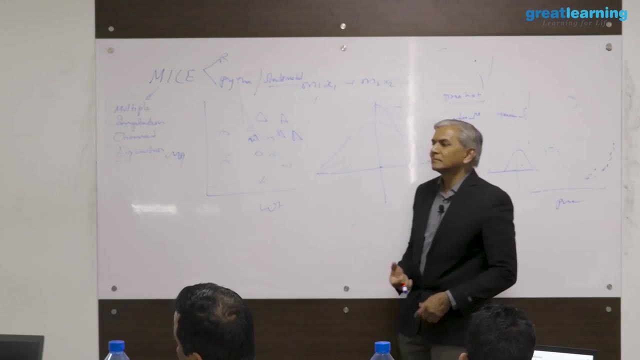 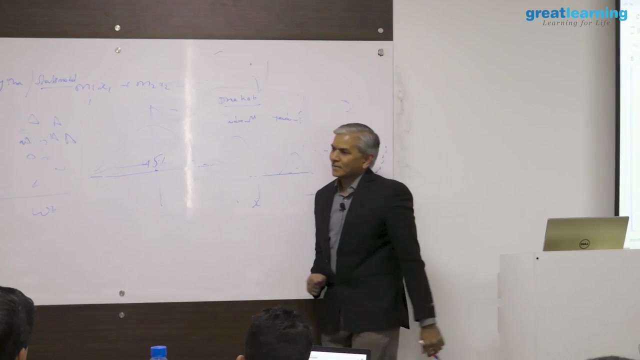 Forget the second level of outliers. They are not really outliers. One question: Yes, Generally, if f minus 2 and standard deviation plus 2, why do you mention 1.96? 1.96 because 1.96 covers 95 percent of the confidence level. 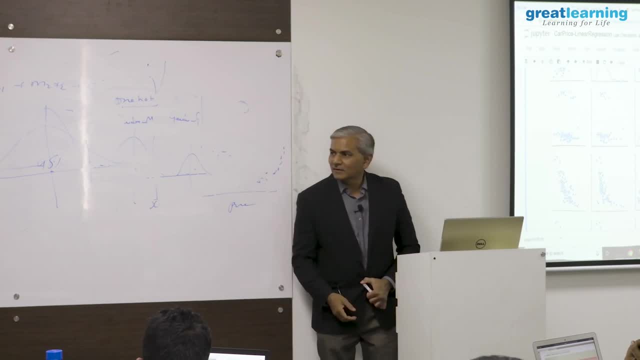 Some people use 2 standard deviation. Some people even use 3 standard deviation. Ok, That depends on your where. it is a matter of life and death And I want my model to be perfect, as close as possible. That means I want my deviations to be very tight. 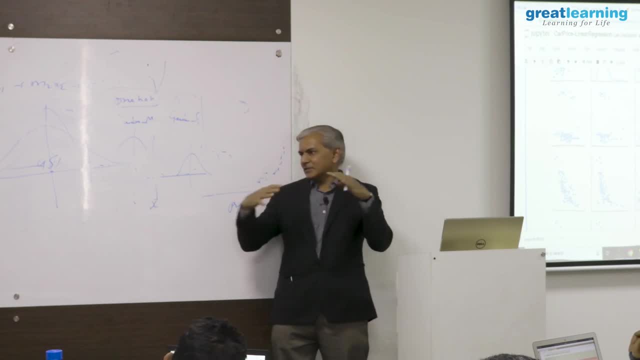 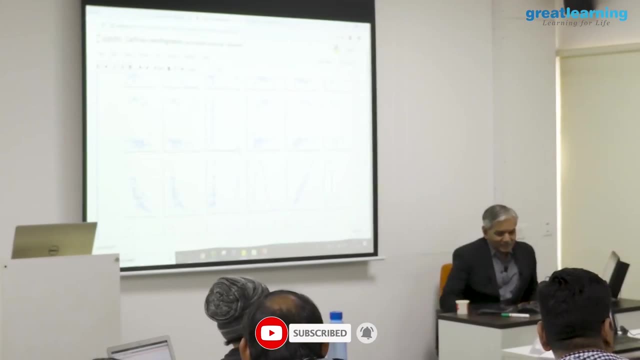 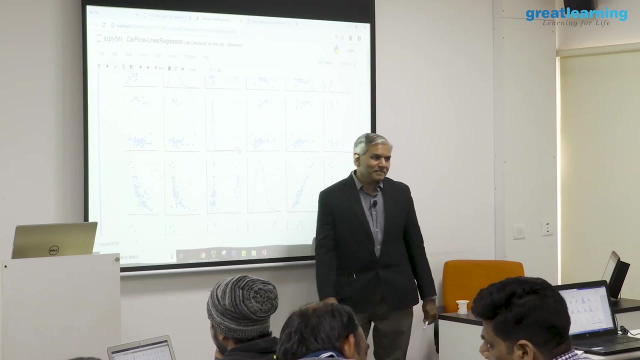 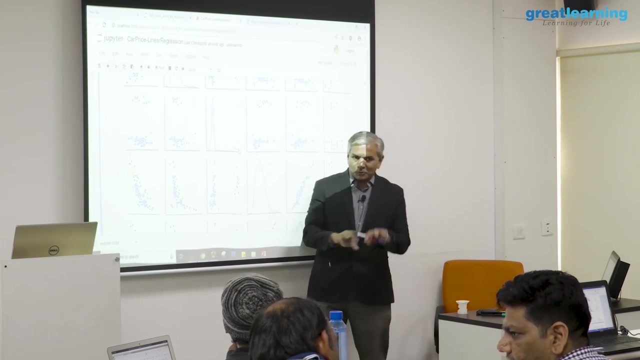 Where I can tolerate some errors. my deviations can be low, So it depends on your requirement Because of two different clusters, which I am seeing here. Ok, But since the size is very small, Mahanchaya says it is outliers And the outliers have been introduced through some manual problems. 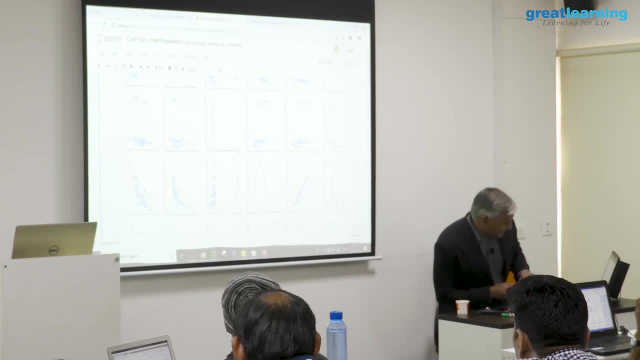 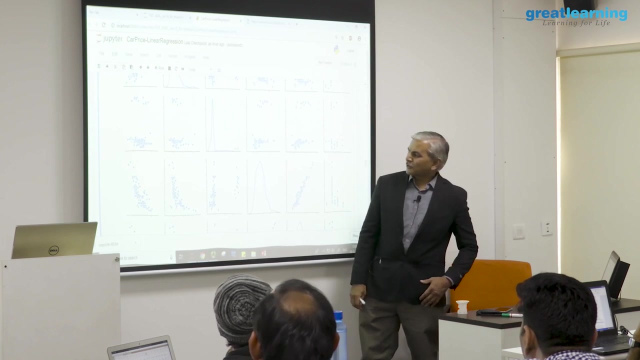 Alright. So in this case it is good to remove the outliers, or we can just remove the record. We can remove the record. There is also one strategy: Removing record is always the last option Because you are going to lose so many other column information when you remove those records. 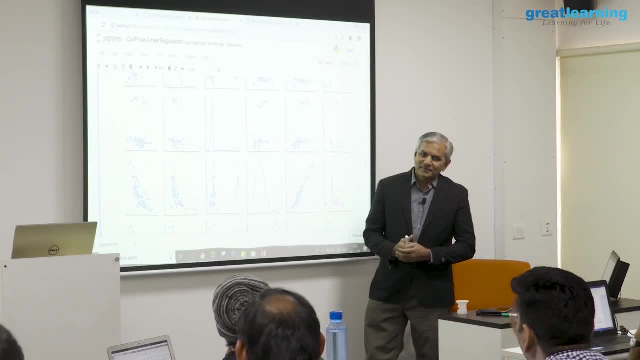 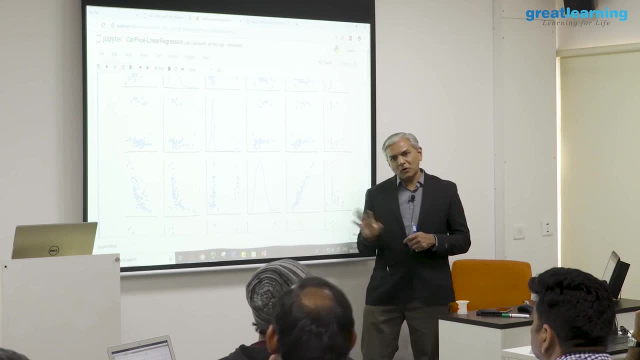 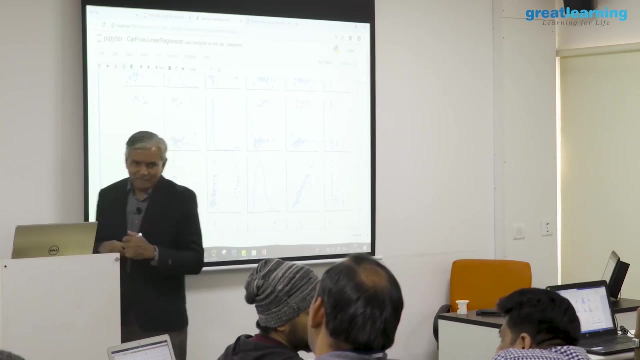 Ok Row. only He is talking row, He is dropping the rows. So if you start dropping the rows for all columns where there are outliers, your data set might shrink. So that is not going in the large exercise. So what happens here is 30, yeah, 30- attributes: the breast cancer ones. 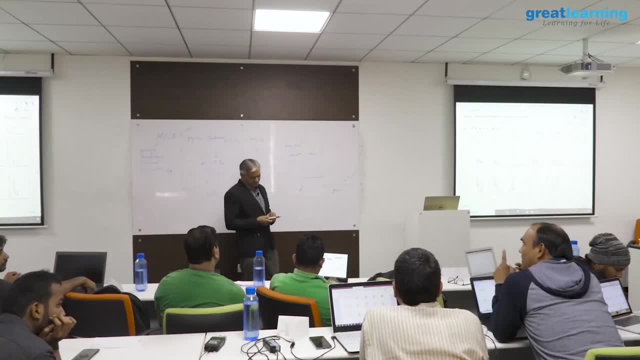 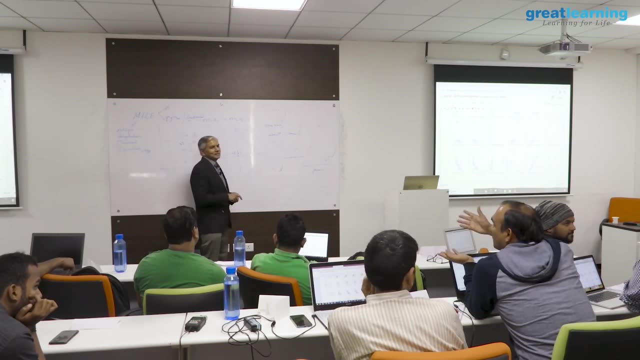 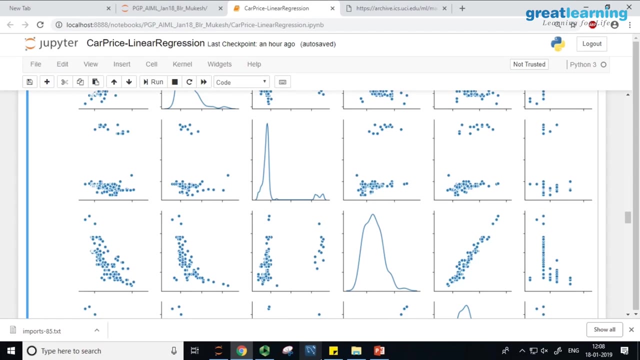 Right. So every column except one, every column has outlier. So when we are removing the outlier for every column, So dropping records is always the last option. when you have plenty of data, When data size itself is restricted, dropping records is not a good option. 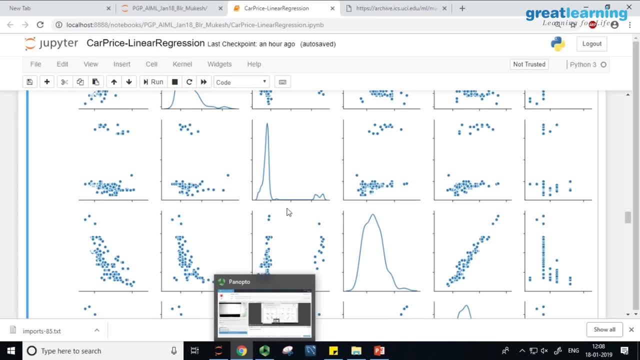 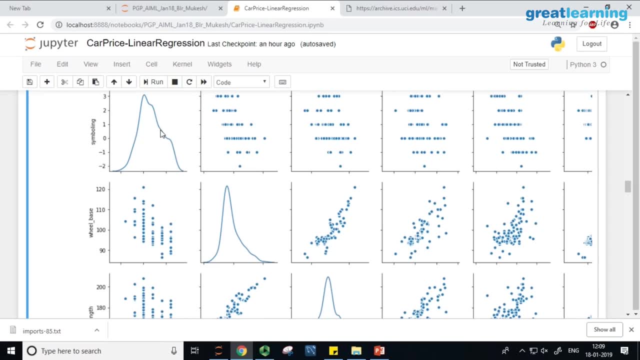 Shall we move on, All of you? Ok, Let us move. so now always start by analyzing the diagonals first, how the data is distributed on each column. This is my univariate analysis. this is what the output of DF describes. how your data 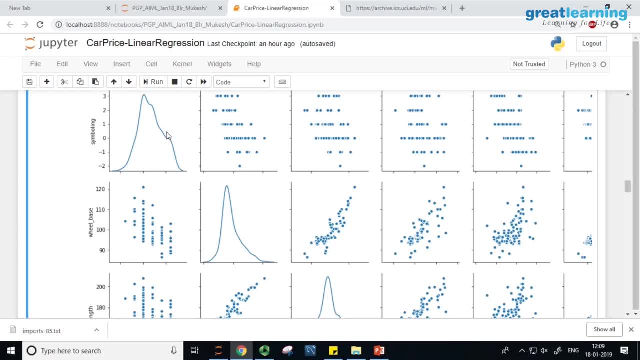 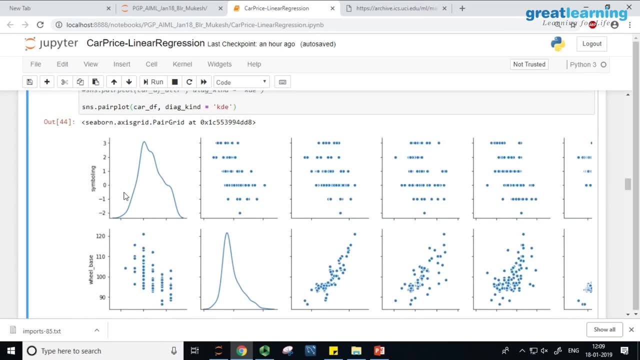 is distributed on that particular column. it is a basic statistics. it is a descriptive statistics. Next we do is bivariate analysis. In bivariate analysis, how these columns interact with each other. for example, if you look at this one, this is telling you interaction between the symbolizing, symboling and this. 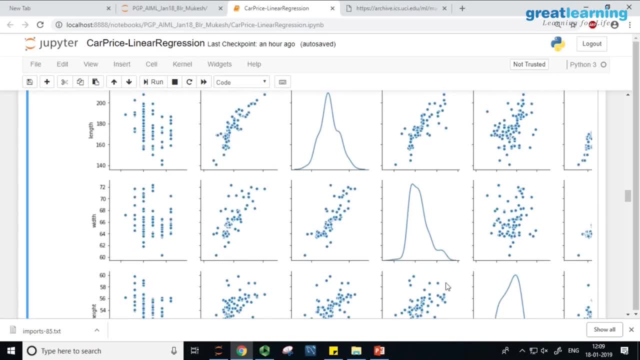 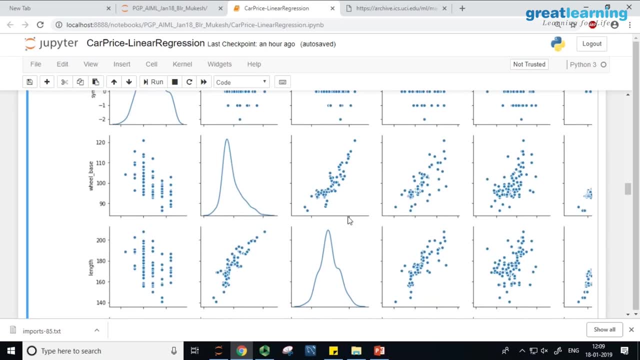 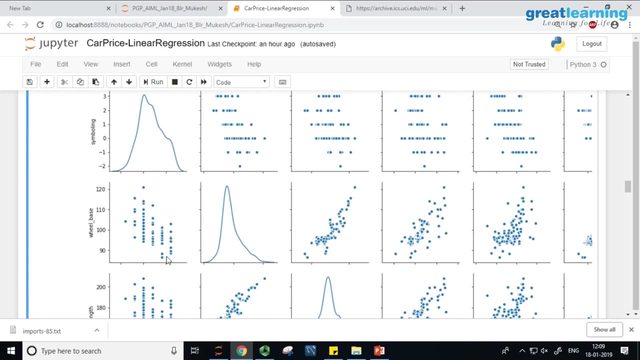 one wheel base. By the way, in this square matrix, above the diagonal and below the diagonal, it is mirror image. Either you focus below the diagonal or above the diagonal. ok, So let us take below the diagonal. So I know this first column is symboling. symboling versus wheel base. 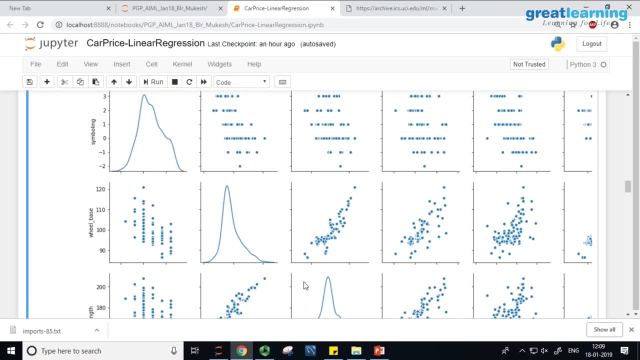 What it means is, as the value for symboling increases, you see that the wheel base trend is going down. Wheel base is shrinking as symboling increases. But I am also seeing lot of noise For a given value of symboling. there are multiple values of wheel base. 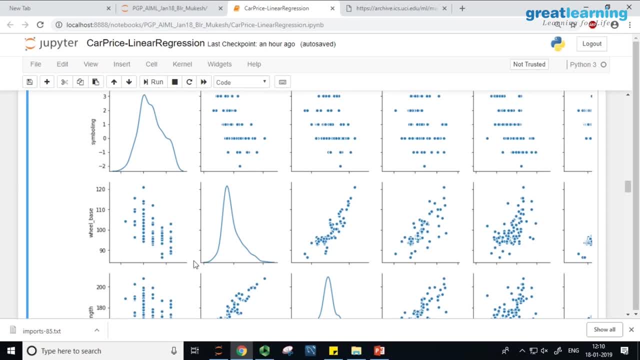 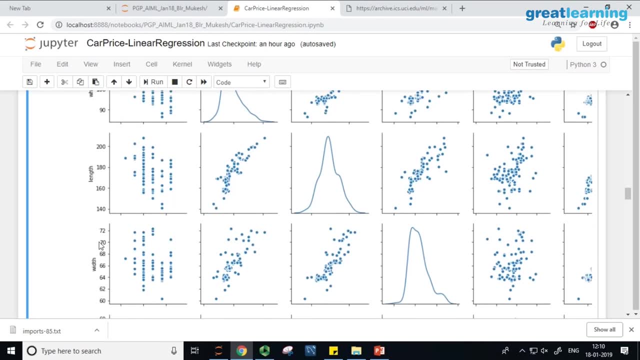 So between symboling and wheel base there is a negative relationship. there is a negative relationship. Look at this. this is between symboling and length of the car. Since length of the car and wheel base are almost kind of related, you will see a negative. 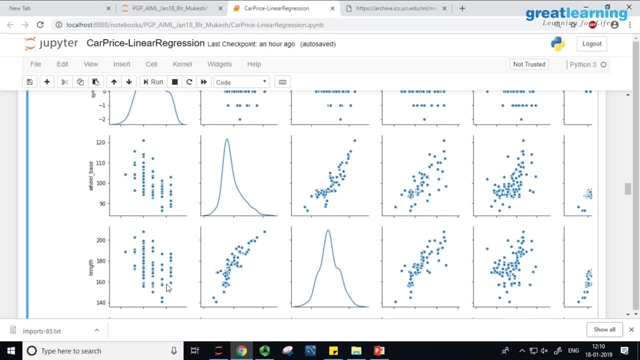 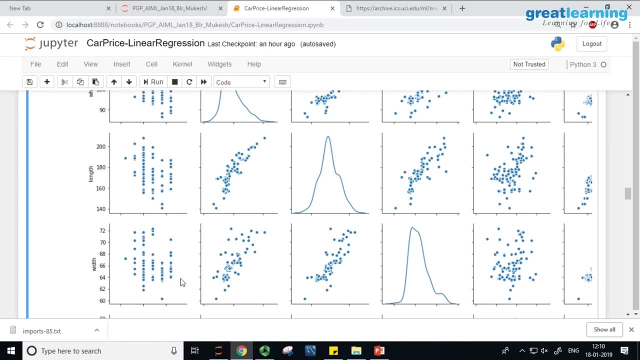 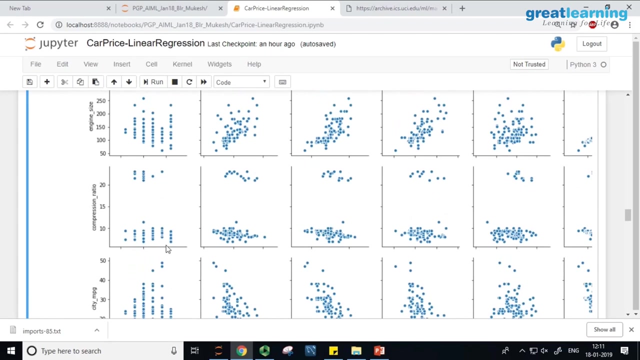 relationship here. also, but not as well as in this case, Look at the relationship between symboling and width. it is almost circular distribution, no significant correlation between the two. right, We can continue to do this analysis. let me just look at. look at this one. 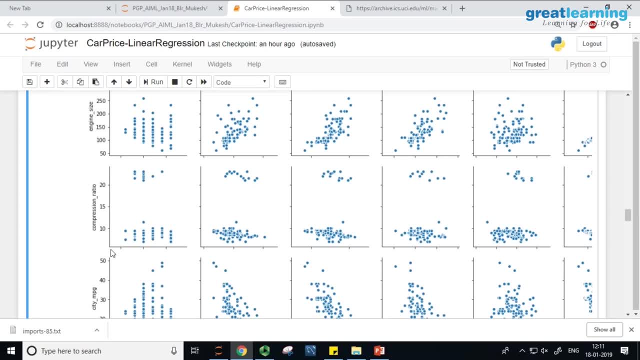 This is compression ratio. yeah, and symboling For increasing value of symboling compression ratio that you find is, I mean in this range for one group of cars, whereas for other group of cars, the symboling range of symboling. 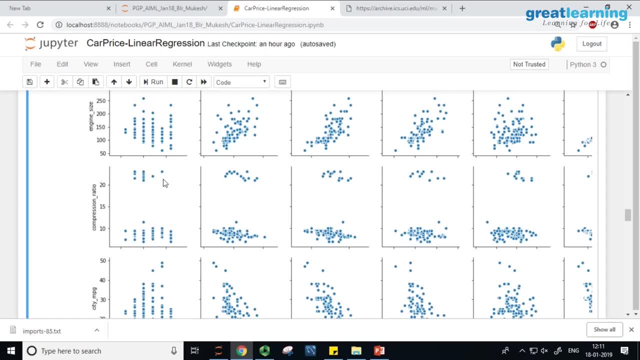 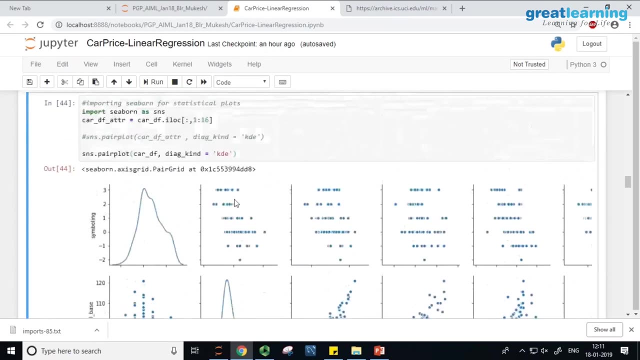 is very small For this cluster. if the cluster is a real cluster, the range of possible symboling values is much less than this cluster. That is what is coming out of this analysis. Okay, Now let us look at the other columns. 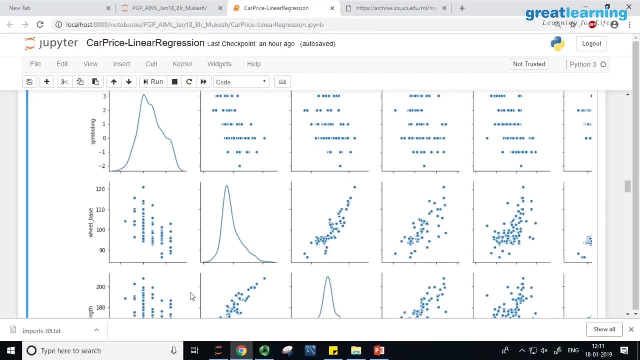 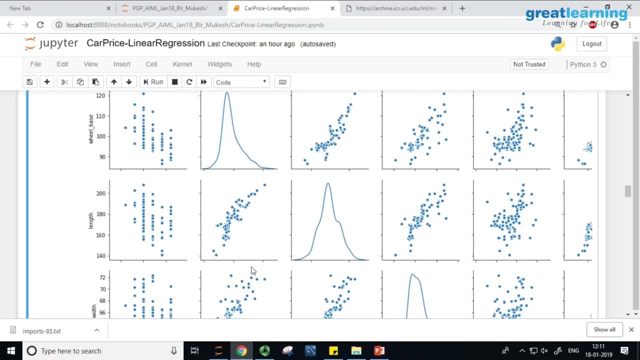 Let us look at this one, look at this. This is relationship between wheel base and length. Obviously, as your wheel base, this is wheel base. as the wheel base increases, the length of the car increases and you are seeing a positive relationship here. 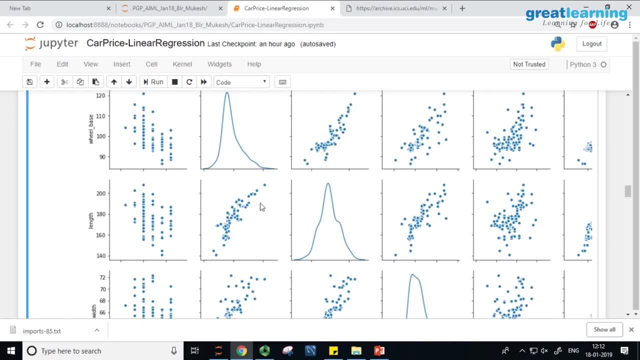 The R value will be very close to 7 or 8.. So this is the case where you have two dimensions and both the dimensions are interacting with each other. They are not linearly independent, But the algorithm assumes that all dimensions are linearly independent of one another. 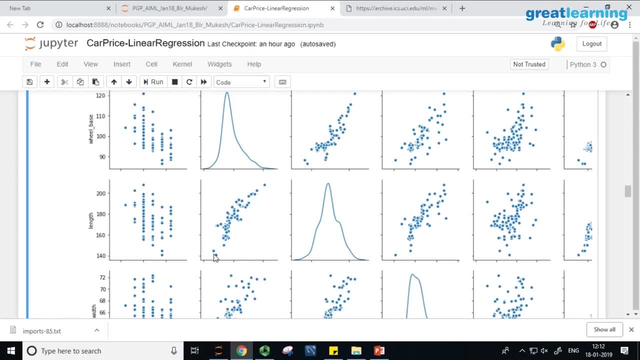 Okay, So we have ways of handling this. One way of handling this is find out, using your domain expertise, whether calculating the length of the car is more prone to errors, or whether calculating the length of the car is more prone to errors. 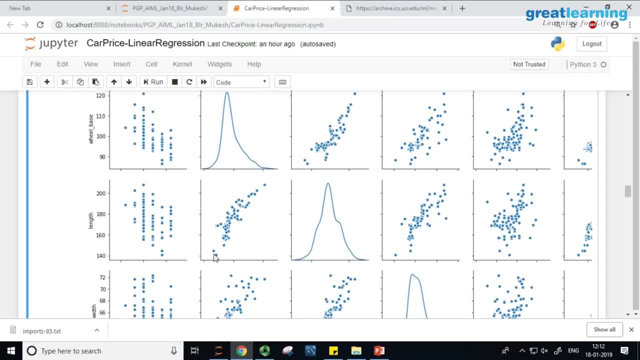 If calculating the wheel base is more prone to errors, measurement errors. If calculating the length of the car is more prone to measurement errors, drop the length of the curve, Keep the other one. However, if you are not able to take that call, you might want to run a principal component. 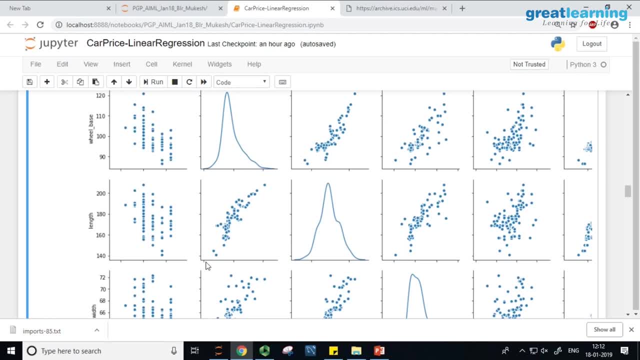 analysis, a mathematical technique, or singular value decomposition, another technique. Okay, Using those techniques, we can create synthetics. Okay, We can create a synthetic dimension out of this. That synthetic dimension will be a composite of these two, so I will drop both of them. 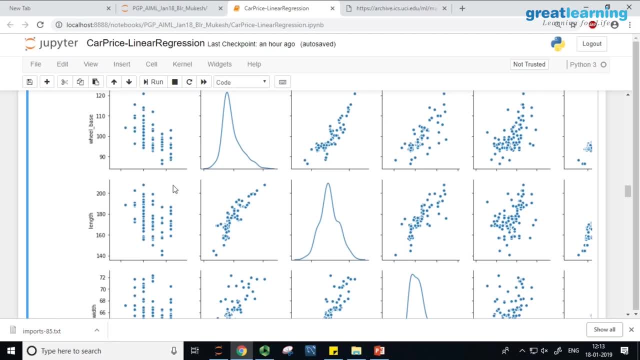 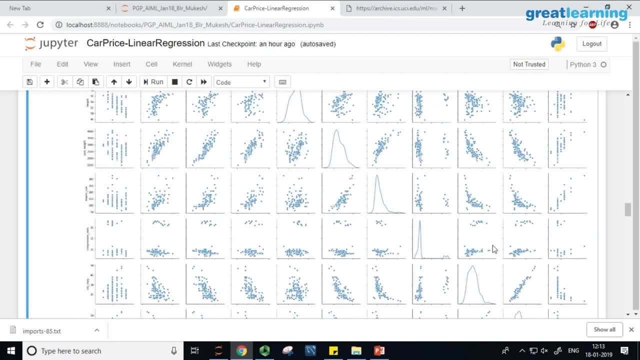 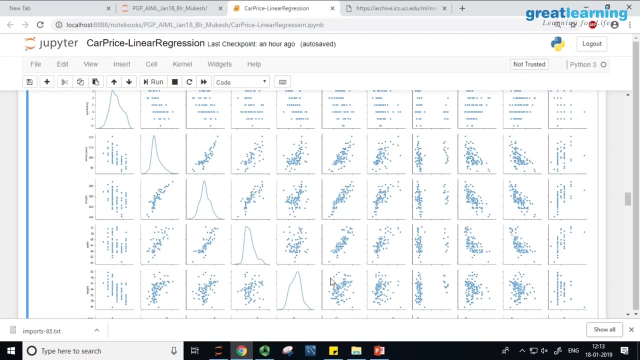 and keep the synthetic dimension. I will talk about this when we come to PCA, principal component analysis. Right now, I will ignore this. Okay, So in the dataset, what I am saying is there are distributions amongst columns which have linear relationship. 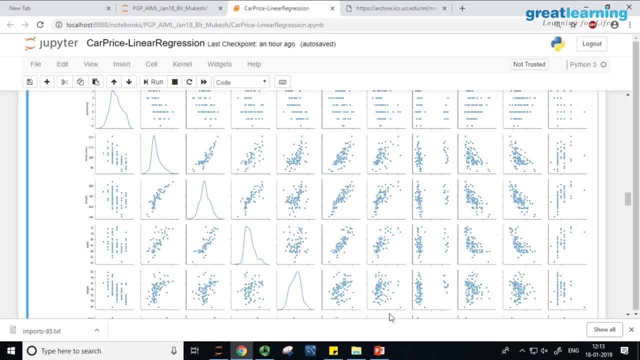 There are distributions amongst columns which are indicating no relationship. Okay, This one, this one, these are all no relationship, But this is negative relationship, negative relationship, so on and so forth. It is a mix. Some columns are related, some columns are not related. 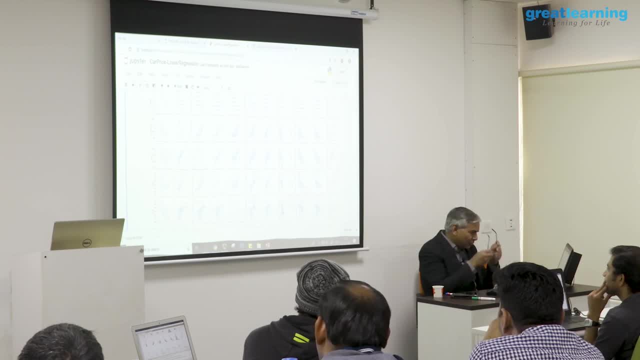 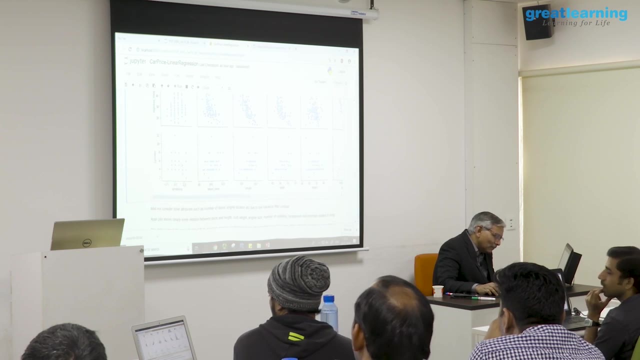 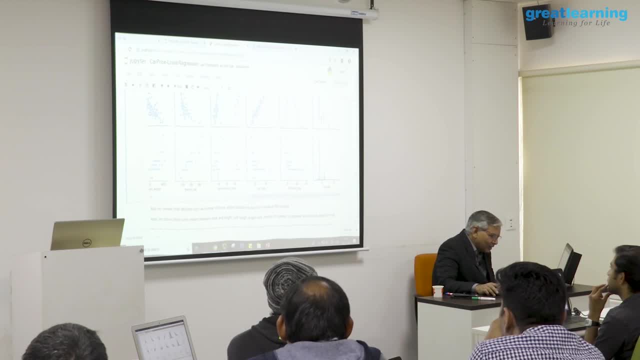 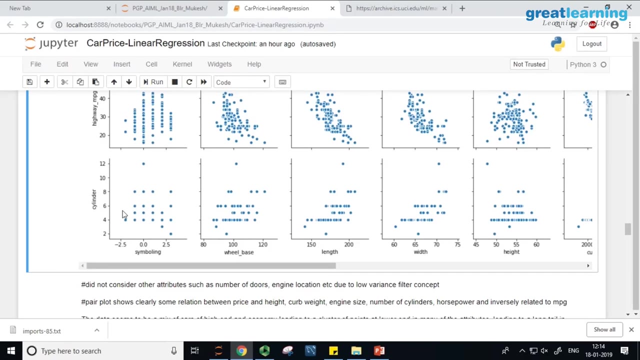 This one, This one, This one, Okay, Okay, What is it? What is it Okay? If you look at the cars with number of cylinders, Okay, In your dataset, most of the cars have 4 cylinders, 5 cylinders, 6 cylinder and 8 cylinder. 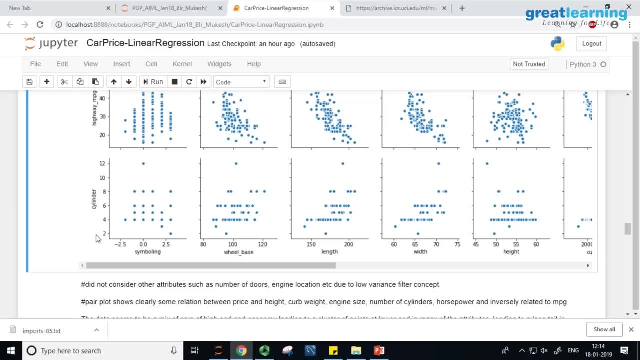 Okay, Most of the cars- look at this- have 4 cylinders. By the way, these data points might be sitting on top of one another, so that does not mean your data set has only 1,, 2,, 3,, 4,, 5, 6 records for 4 cylinders. do not do that mistake. 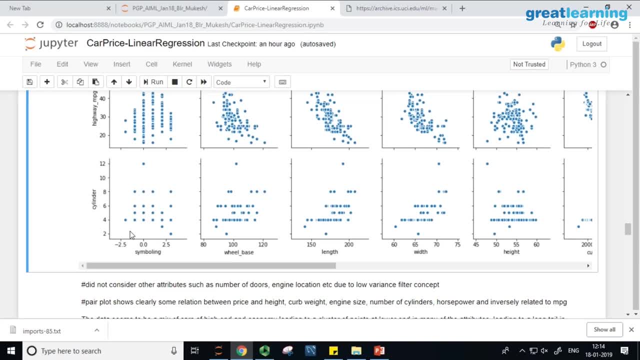 Your data set might have hundreds of records for 4 cylinders, but they are all sitting on top of each other. that is why you are seeing only 6 dots. Most of the data have 4 cylinders. some of them have 5 cylinders, some of them are 6,. 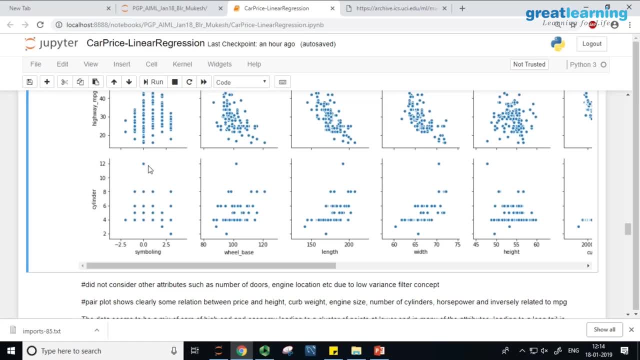 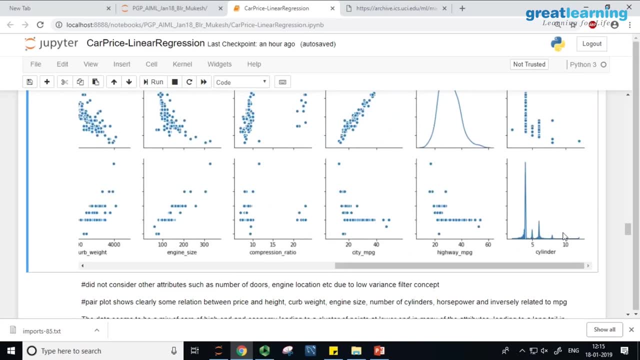 some of them have 8, only few records have 12 cylinders. very few records have 2 cylinders. Now, when you go to the extreme end where cylinder versus cylinder, that is why you see a peak in 4, some peak in 5, then you will 6 and the small peak here. none of the 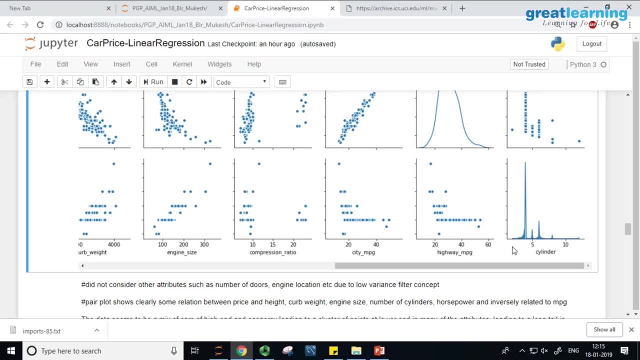 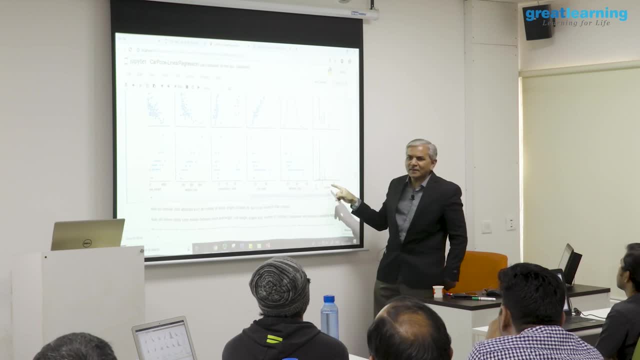 other have any peaks. Now, cylinder is a numerical column, integer column. you can have 1 cylinder, 2 cylinder. then what do you mean? You mean by the spread? What is the spread? How can you have a spread on integer columns? 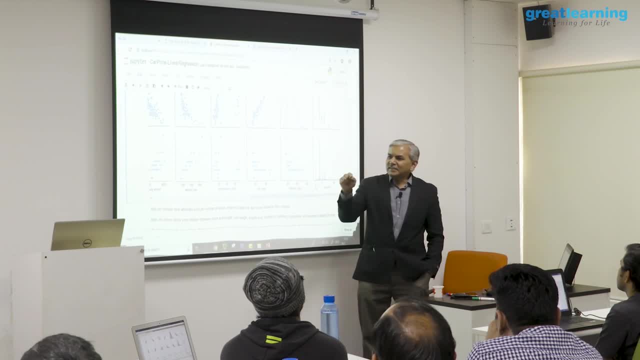 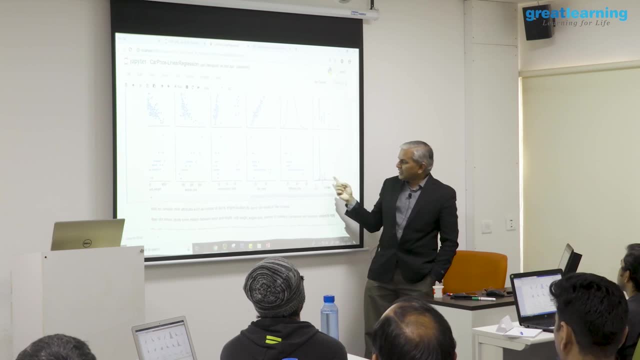 This diagram which I plotted here is called KDE Kernel Density Estimates. So there are 3 words in this. first word is it is an estimate. it is an estimation of the possible distribution density. distribution density estimate in the population. In the population, how the cars are distributed. 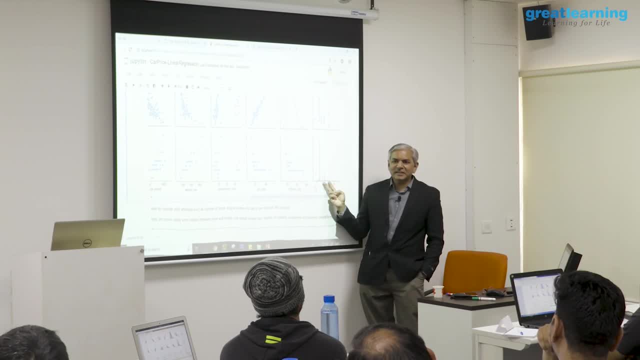 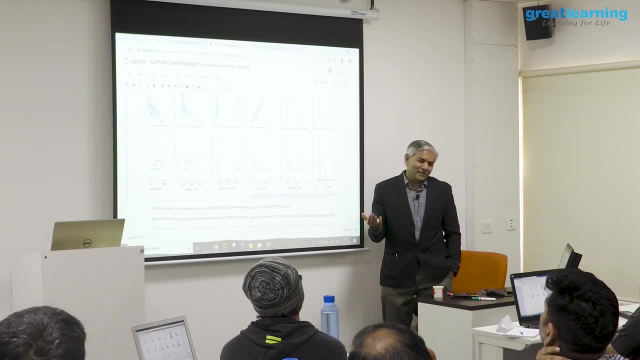 Distributed around this value in cylinder. It is a density estimate based on a mathematical function. That mathematical function is called Kernel. So using a mathematical function, on the available data, I am estimating how the density distribution of this column is likely to be in population. 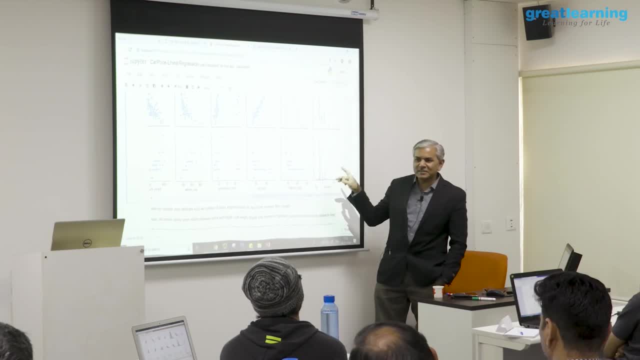 That is why you are getting the spread. The spread is not in your data. the spread is the estimate of the distribution density in the population, Based on the observations in your data set. So for integral columns also you can have spread like this: because what that Kernel? 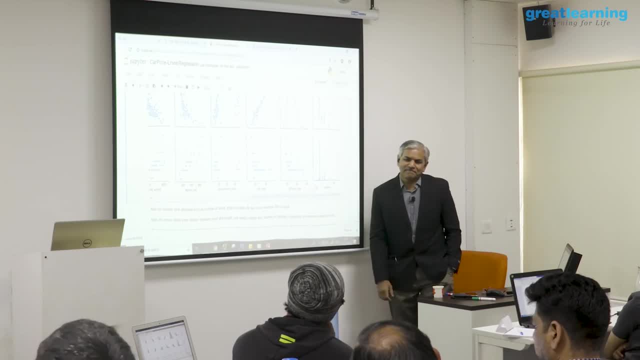 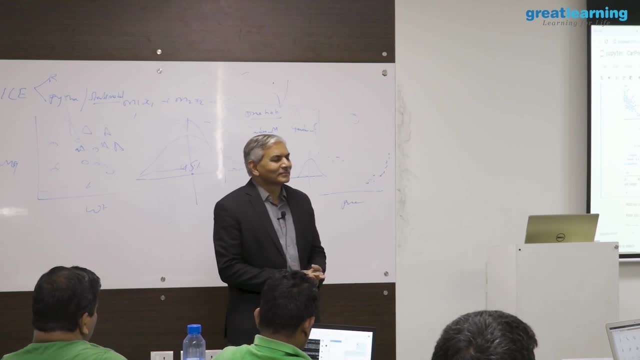 is telling you is in the population. it is likely to be like this: If you are building a model on this data set, you are saying that the modeling is something that has to be understood. what does it mean? I actually went and studied what symboling is, but unfortunately I forgot. 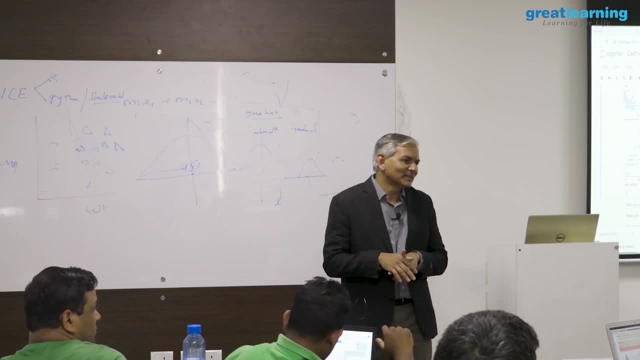 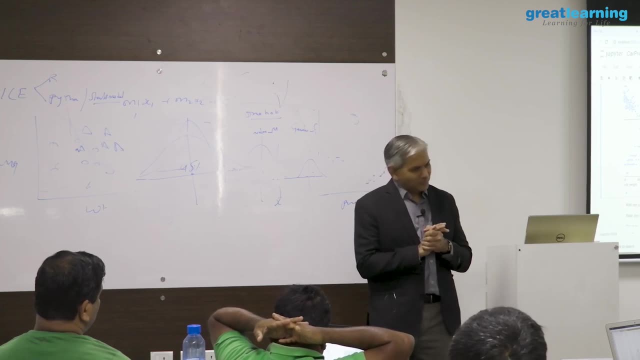 I should have known. I mean the model. If I come to know that this is not a very significant model, what is the model? I mean the model, I mean the model. You can drop it. See, you cannot do model building without domain knowledge. 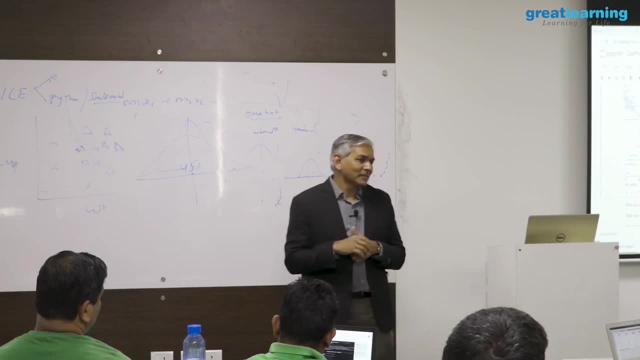 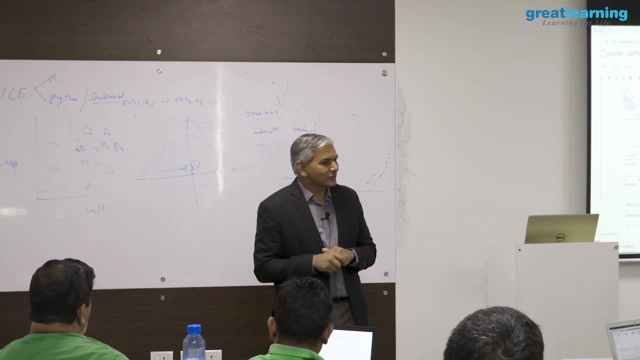 You have to have domain knowledge, We have to go and find out what the symboling stands for. But in your drop statement, like they are not dropping symboling, so we should, I think. Why do you think we should? Because I mean, it is also categorical. 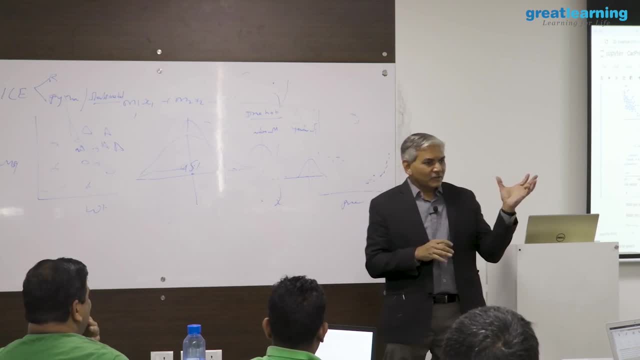 So what? So what Does not matter If a car coming from Japan versus car coming from US, the mileage miles per gallon is going to be different. So it is a categorical variable. origin of the car is categorical variable. It has an impact on mileage. 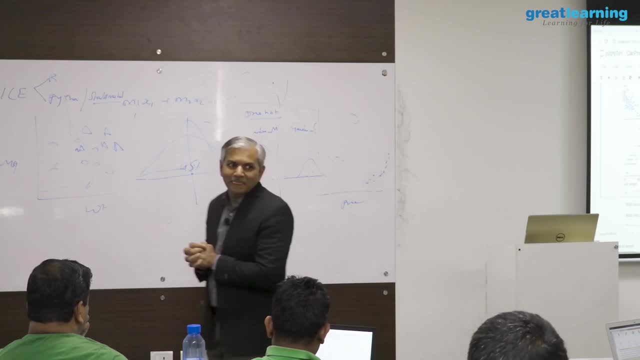 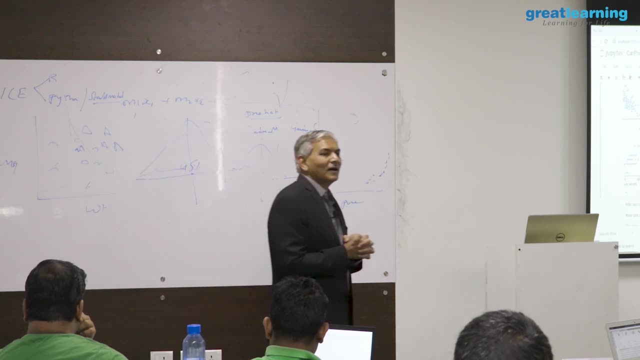 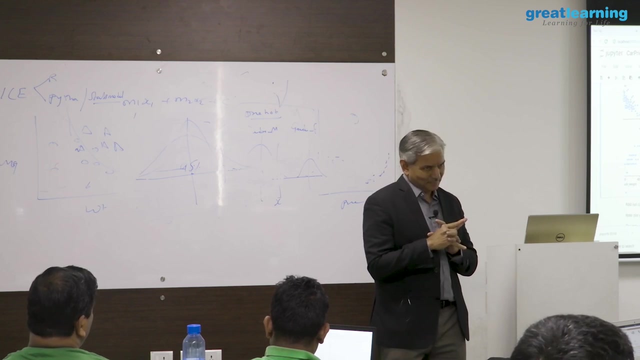 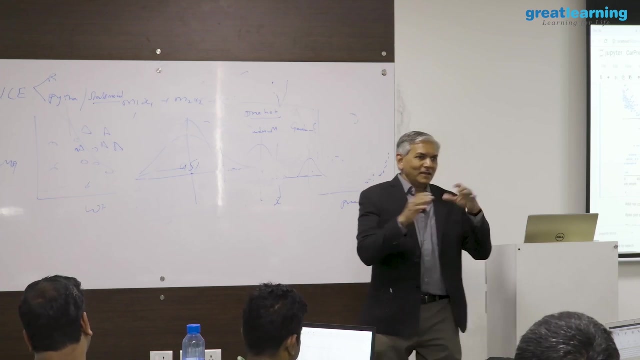 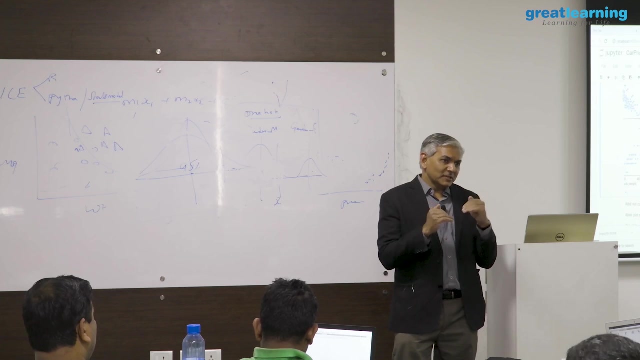 If you just use the. So if you use the, 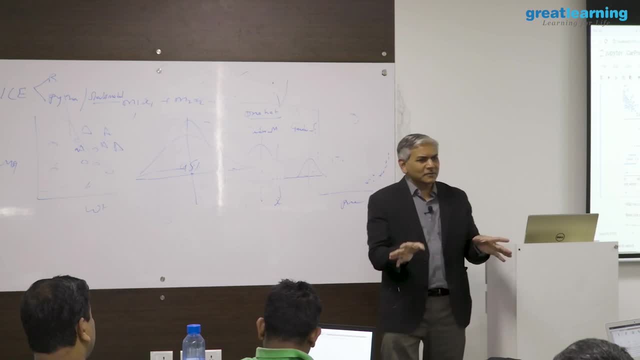 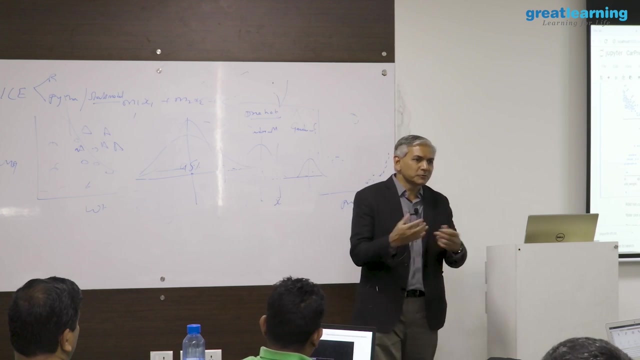 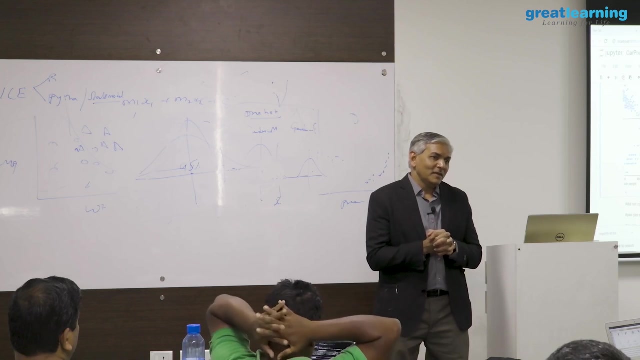 it might be some distribution, but is that distribution good enough for you to use it? you have to take a call, And that call you will be able to take, both based on domain knowledge. 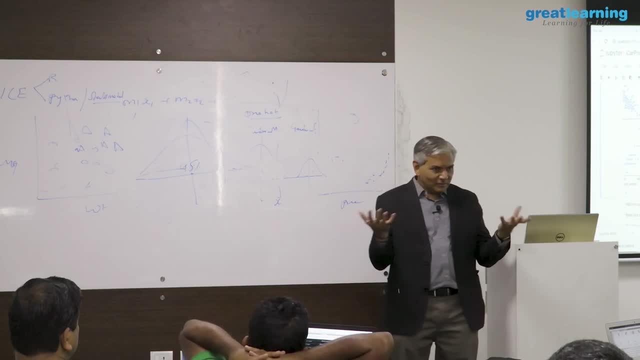 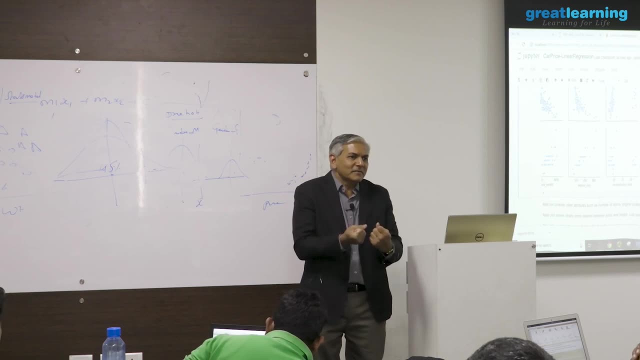 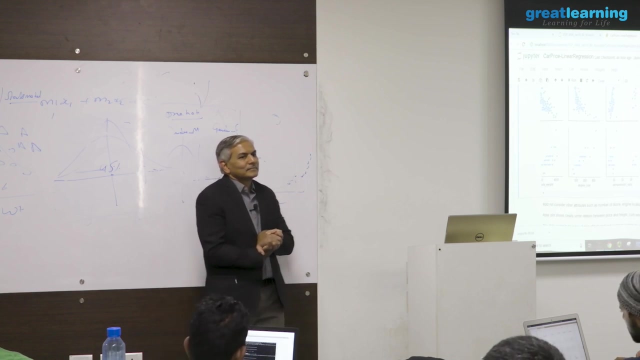 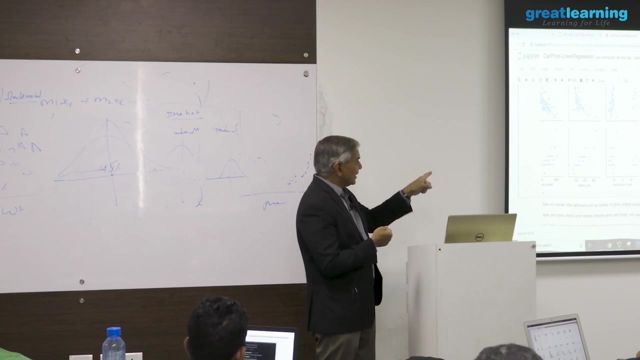 If I know the drivers in the in the, the people who use the car is 50-50 amongst these gender in the market. I know that, but for some reason the data which I have does not reflect that. This analysis is done on the original data set. it is not on the dropped data set. 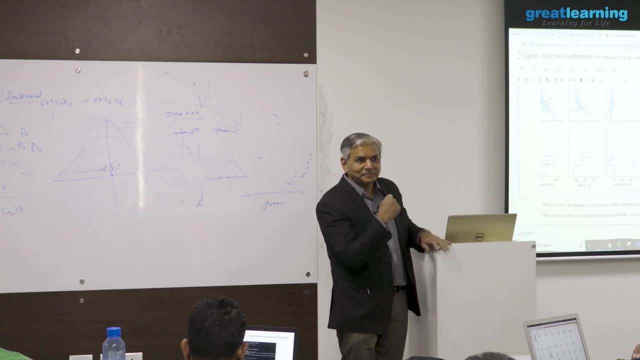 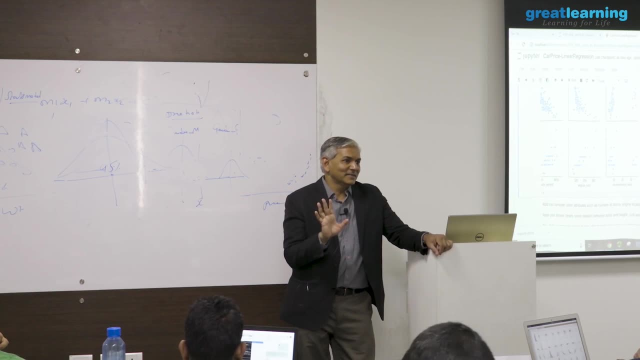 You should always this analysis on car DF, you should always do this pair plot analysis on the original data set, always Ok Once. because this, this analysis, this analysis is what is going to tell you which dimensions are likely to be important. 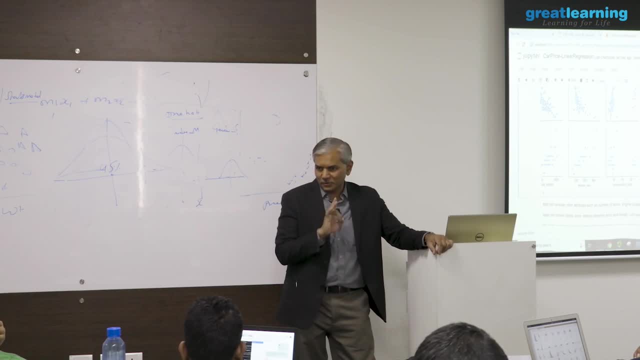 which are not likely to be important. You should always do this on the original data set. Hey, you got your coffee, Yes, Yes, right, But I think here we have already dropped it and we are doing this analysis. This is not on the original data set. 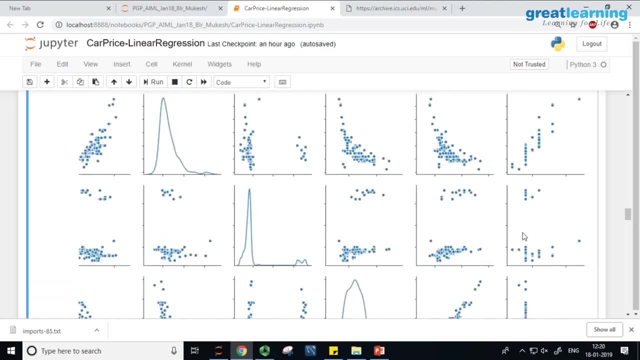 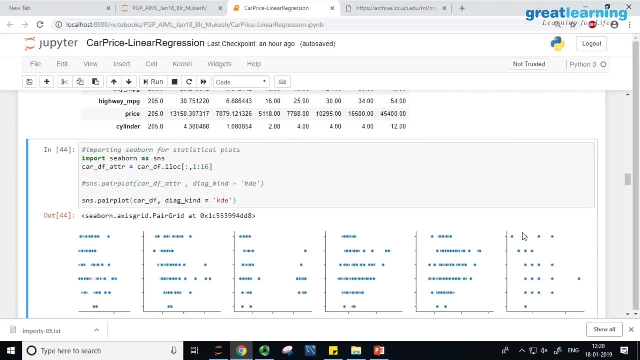 Hey, no, no, no, I change it here. no, I change it here. I asked you to. If remote fuel type and generation, all of that will probably remote and then we are doing this analysis, Then what time is it? 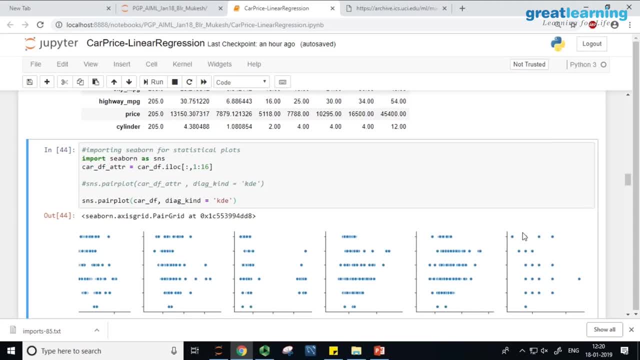 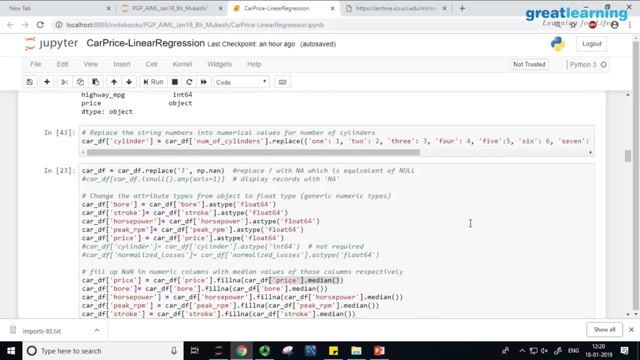 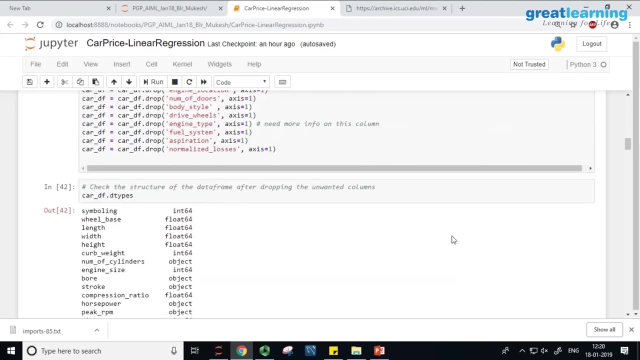 No, I commented out this line. I just now did that, But you have already dropped the call. No, you drove first and then you ran the sample. oh, you are talking about this. yeah, you are talking about this, yup. 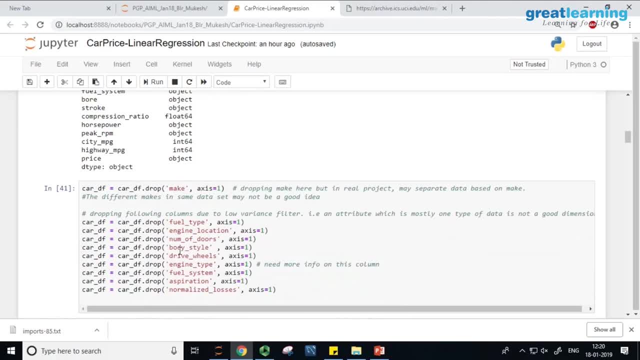 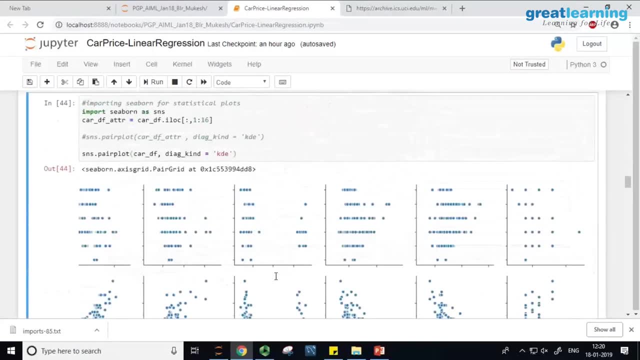 ok, yeah, yeah, You should be doing this. before you do this, before you do this, Always do your analysis of the raw data set. Ok, all right, Let us shall we move on. Just one question, Yes, please. 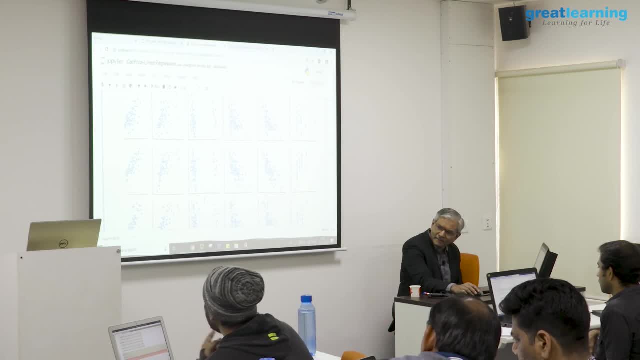 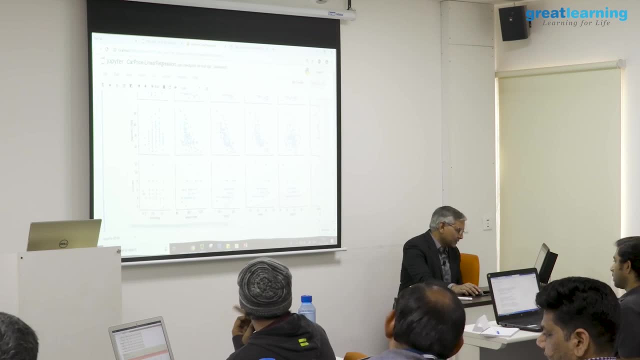 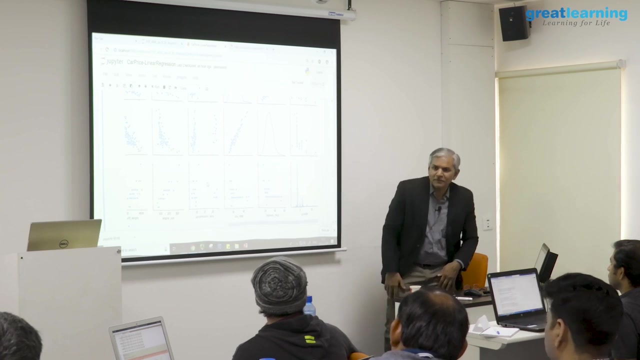 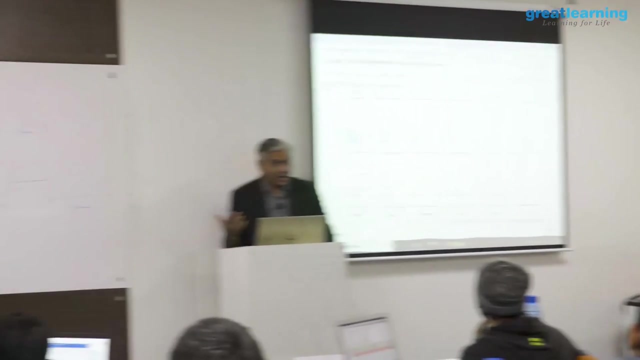 We did analysis on: oh Yes, sir, Ok Go, No. what you can do is go back to your data, find out what is a car model, go and refer to the manufacturing, because you have all this information- Whether this car model can have 12 cylinders. 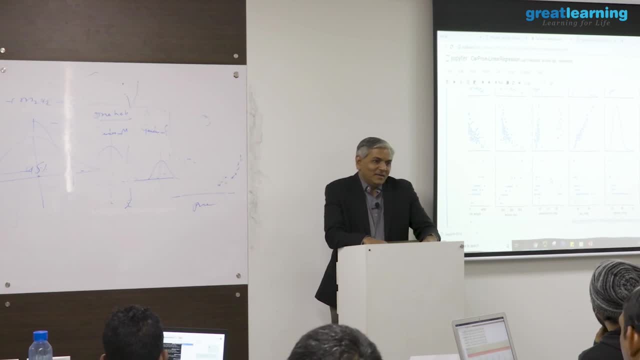 That analysis will do. that is what you have to do. See: missing value replacement, outlier replacement- all these things you cannot do without your any domain knowledge. you have to have domain knowledge. When I went and studied this data set, I found out that for a given car, say Toyota, some particular 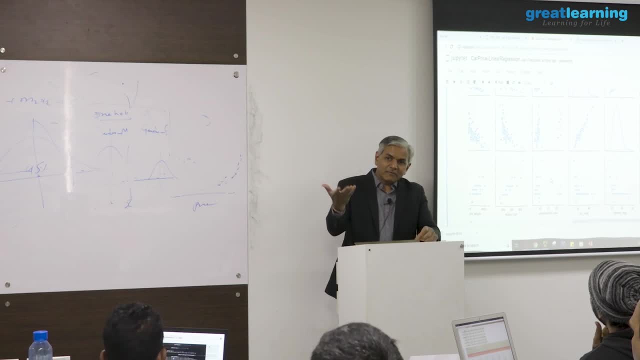 within Toyota, one particular sub variant, the data given for mileage was unreliable because the factory manufacturing label itself says the mileage, miles per gallon, is going to be in this range, whereas this guy is claiming to be so high. So the data itself became a question mark. 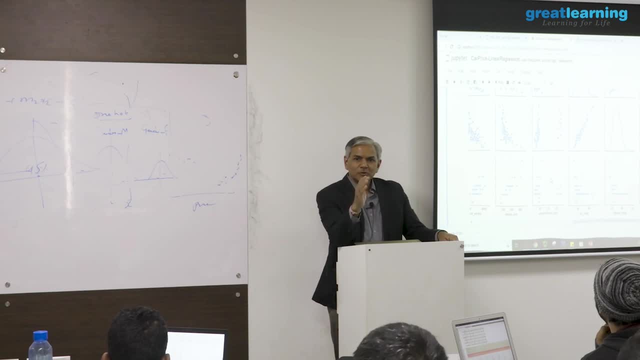 So you have to do that analysis. ok, So when you do a real life project, when you get into capstone project, you have to reflect all these things. how did you analyze your columns? how did you handle your outliers, how did you handle your missing values? and you have to justify your strategy, why you 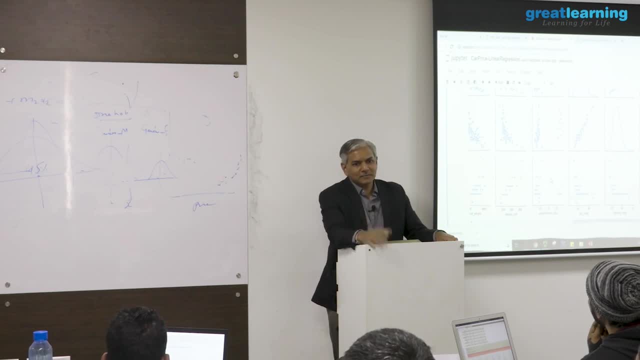 did that. You cannot blindly replace something with a median. That may not be the optimal strategy. Ok, shall we move on? Ok, so for symbolic purposes. symbolic means cars are initially assigned a risk factor symbol associated. Ah, risk, correct, correct. 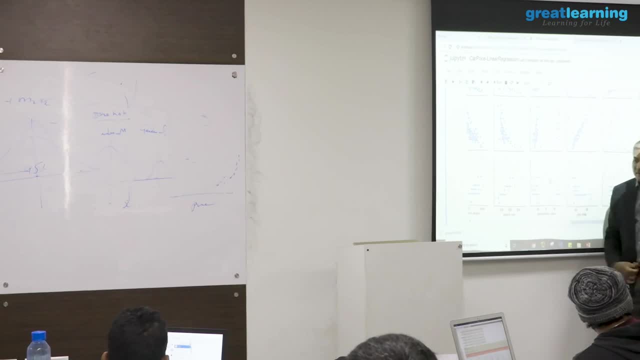 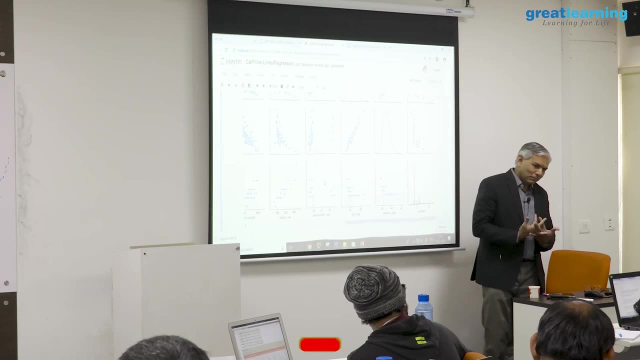 They are assigned risk factor. that risk factor is what they connect with symbolic. Can I just read out more louder: Yes, Cars are initially assigned a risk factor symbol associated with this price. that gives more risk to the symbolic. Yes, This is a symbolic symbol. 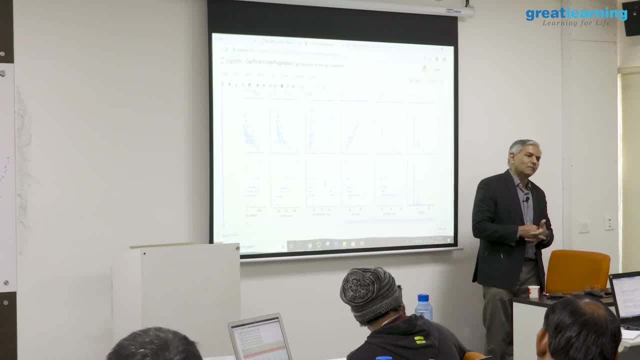 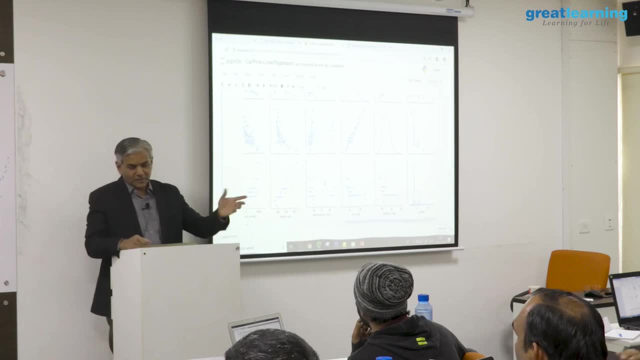 It is a symbolic symbol. It is a symbol symbol, So this is a risk factor associated with the car and I, again this reminds me, the risk factor associated with the car depends on the color of the car. I do not think we have. 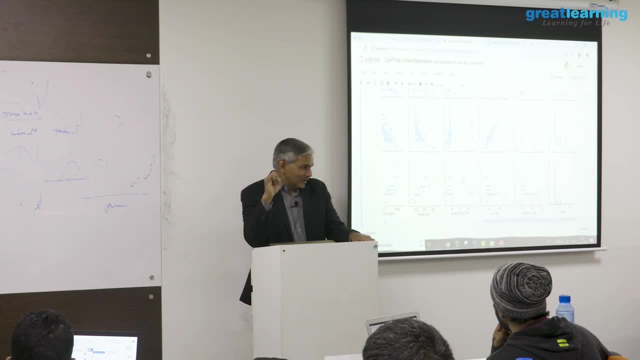 color here it depends on how the car has been driven. how the car is driven These days, lot of people you know they take pride in telling that my car has so many chips by this high end foreign brands. they all come with embedded chips. those embedded chips. 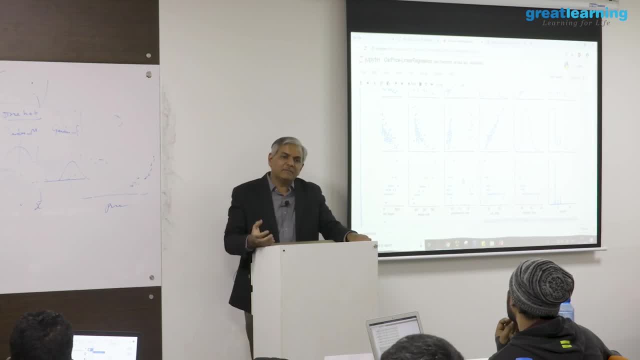 in real time. they capture the data about your driving style and pass it on to a central server where they sit down and analyze and the risk factor is adjusted, recalculated, recalibrated based on how the drive, how the car is being driven. the symboling reflects. 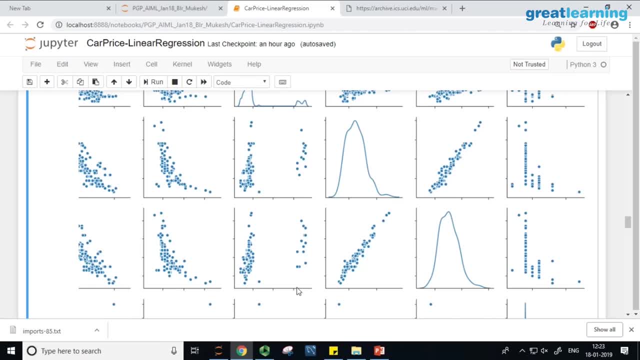 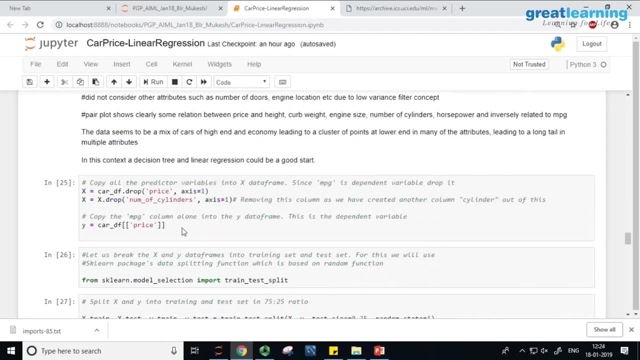 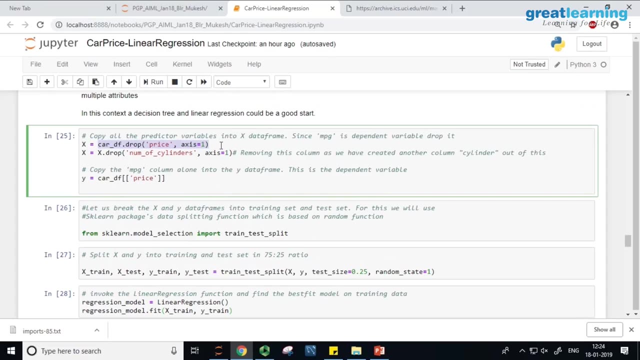 that right. Okay, let us move now. are you able to understand how to interpret this pair plot? It will come through experience, but this is where you have to do it. okay, move on. so what I am doing here is from the car underscore df. I am dropping the price because that is. 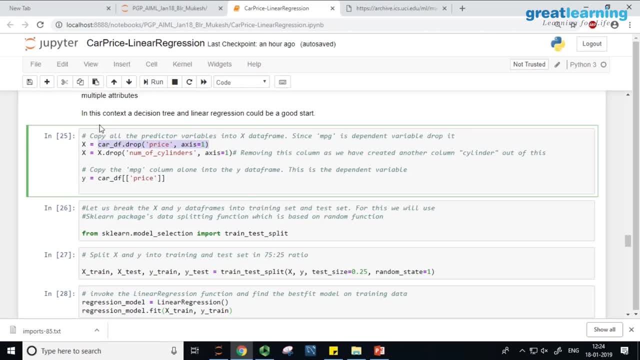 my target and whatever columns I am left with. I am capturing that into x. so I am creating a new data frame called x, which will now have only those columns which are independent variables. target column price will not be part of x. Then, once again, I am going to. I am dropping number of cylinders here, because this is the. 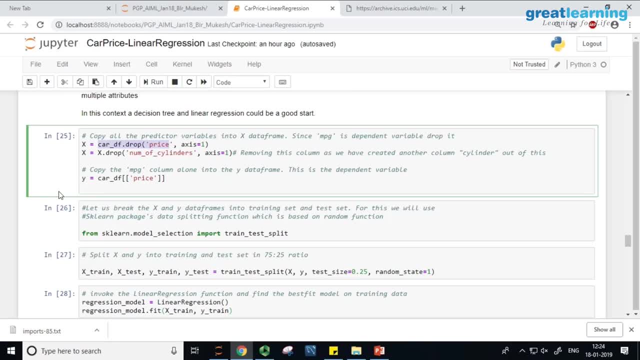 same problem. it is a low variance filter again, but if you wish you can keep it. Then what I am doing here is from car underscore df, I am dropping the price and, sorry, I am not dropping the price. I am selecting the price column and storing it in y y variable. 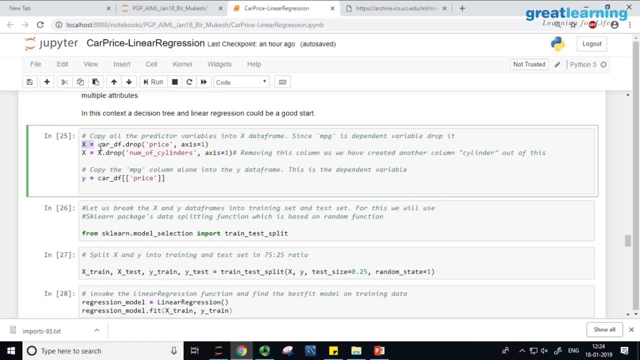 Okay, So x variable is all columns except price. y variable is only the price column. So if you have 1000 record 10 columns, this will become 1000 record 9 columns. this will become 1000 records 1 column. are you all okay with this? 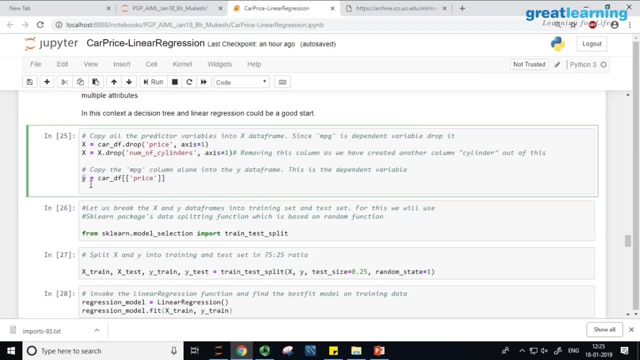 So I have segregated the independent and the dependent variable. If this was r, I do not need to do this, Because r takes in as input only one single data frame and along with that a formula, whereas in scikit-learn I have to separate this data into independent and dependent variables. 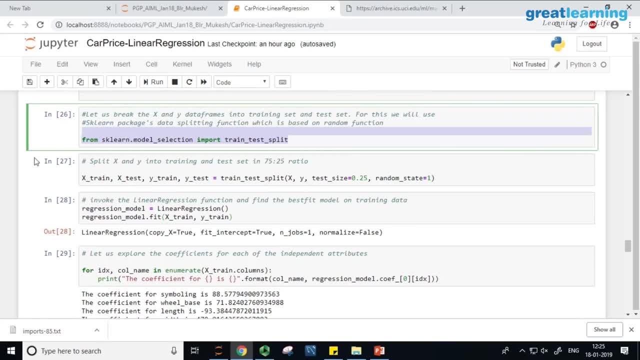 Then I am making use of the random function which generates the training set and test set. we call it train test split. when I make use of this train test split on x and y, I am asking it to split the data. So I have a set of data and a ratio of 75, 25,: 25 for test, 75 for training. 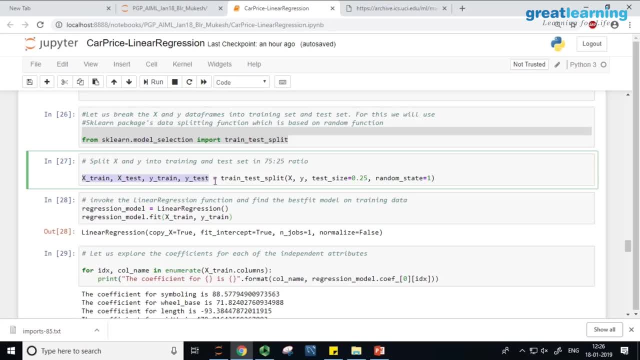 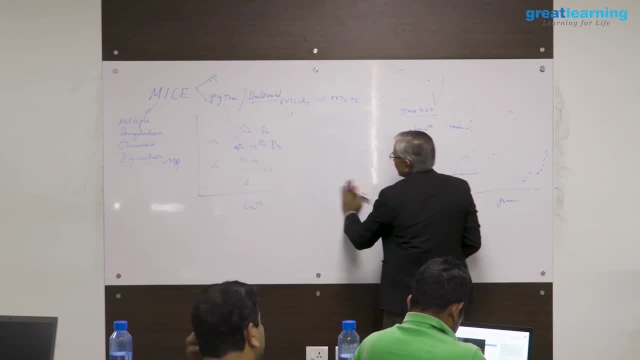 The output of this will be 4, 4 data sets. So let me explain this to you because some people will get confused here. So if my this was my data frame df, this was my target. variable iv- independent variables- target. 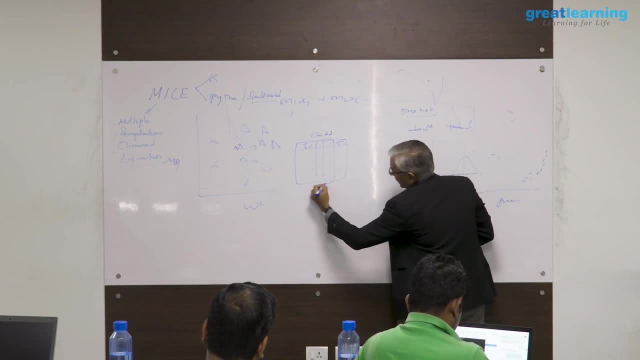 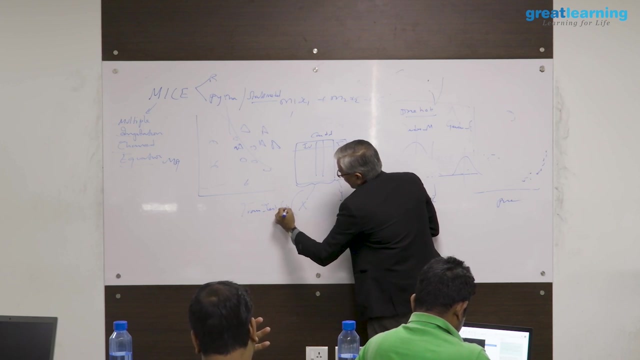 First thing which I did is I captured the independent variables. Okay, Okay, Okay, Okay. So I took the target variables and stored them in x, I took the target variable and stored it in y. Then, on this x and y, I did a train test split. 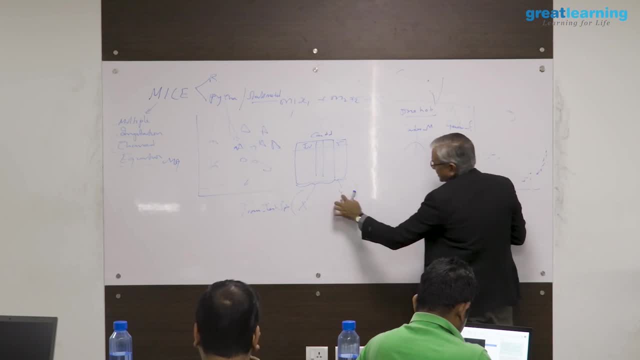 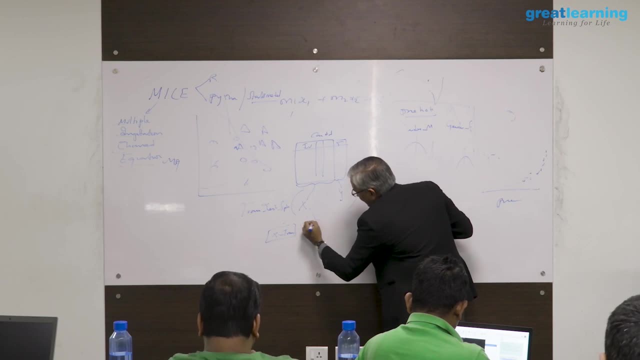 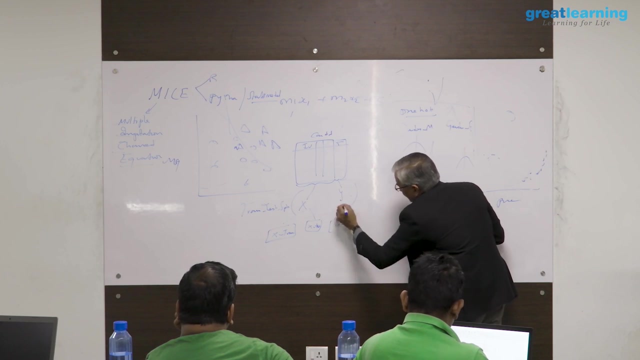 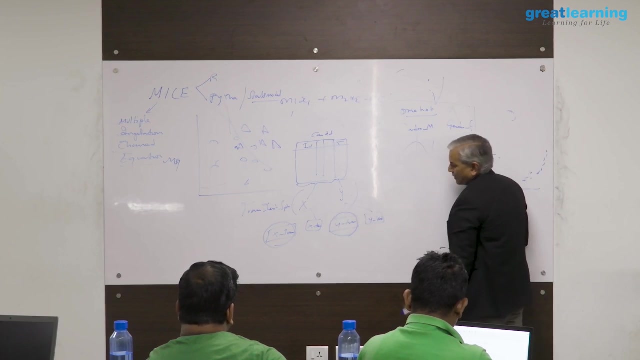 When I do this, what happens is it breaks this x and y both into x underscore train, x underscore test. Okay, Okay, Okay, Okay, Okay, Okay, Okay. So I have y underscore train, y underscore test. This training label y underscore train is for this x underscore train. 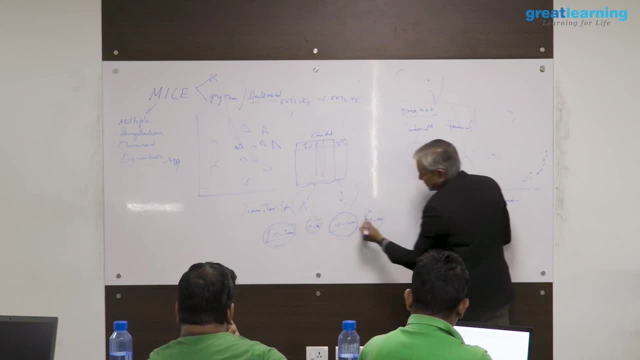 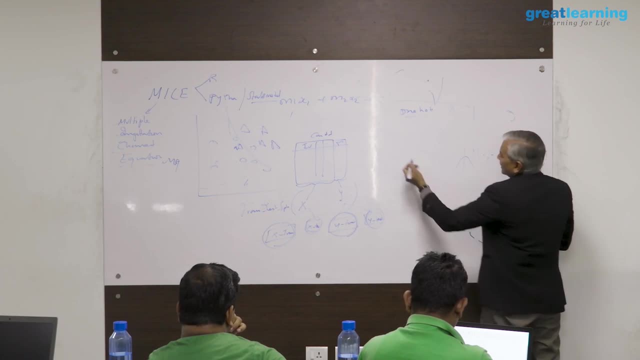 This is my test data: x underscore test. corresponding y underscore test. Now, when I build the model, what I will do is I will call the fit function Fit And with the fit function I will supply these two, This one x underscore train and y underscore train. 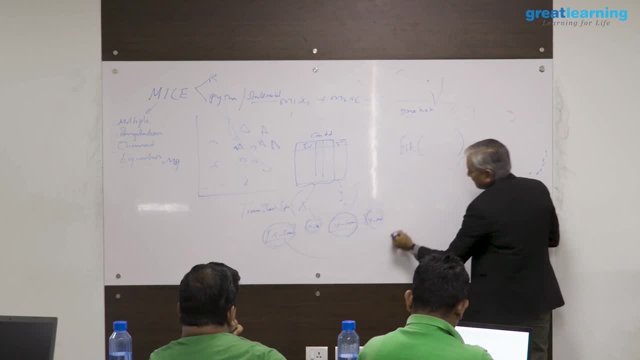 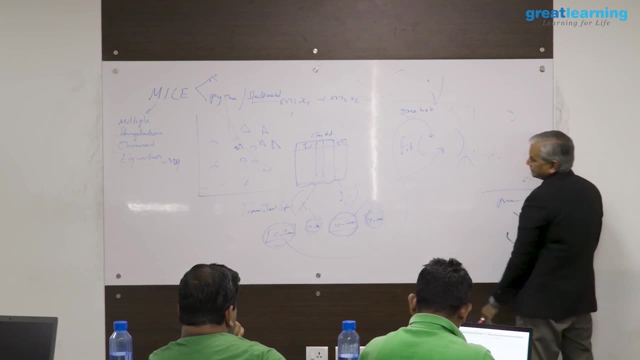 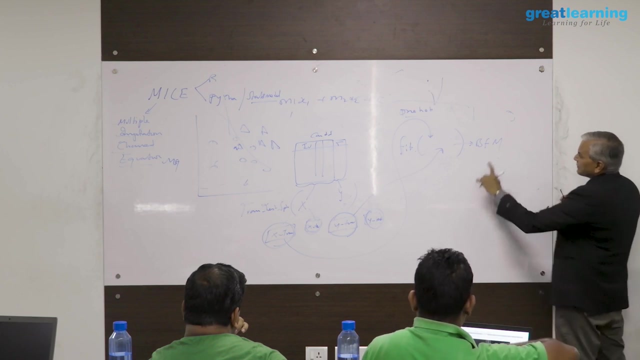 I will supply these two. This is at this point the gradient descent will come into play. It will identify for you the best fit model. The best fit model will reflect the relationship between y and y- Okay, The relationship between y, this one- and x. 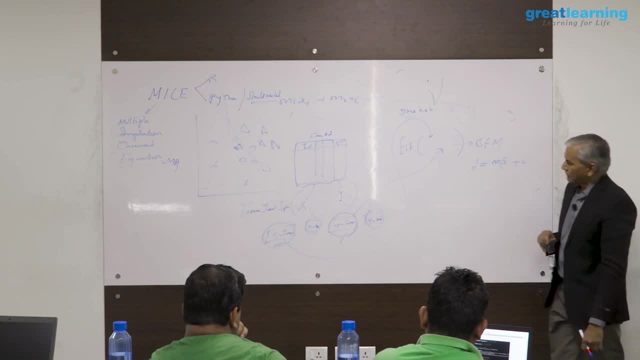 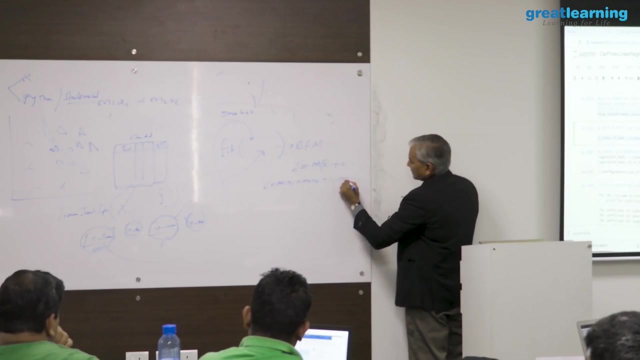 This x comes from this training set, So it will be of the form: y is equal to m1, x1 plus m2 x2, so on, so forth. How many columns are there? 1, 6.. So m is 1, 6.. 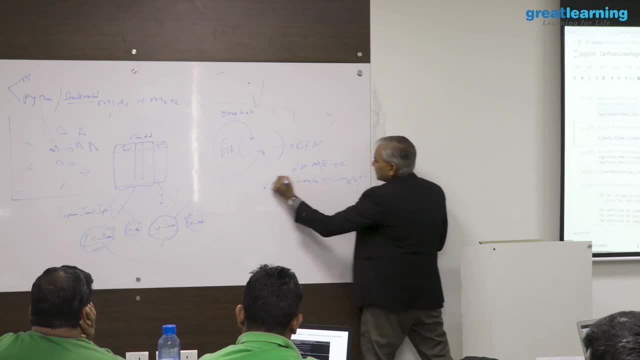 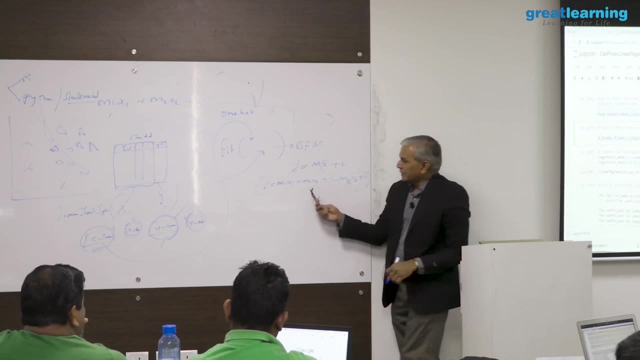 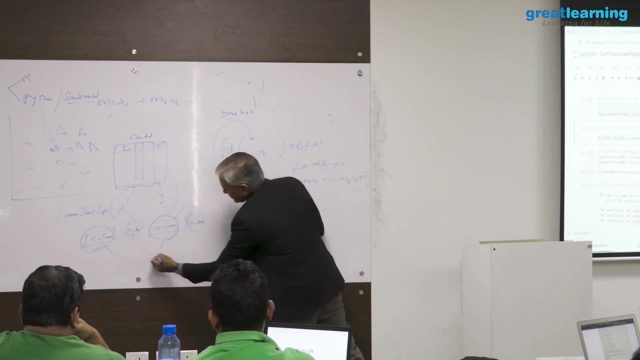 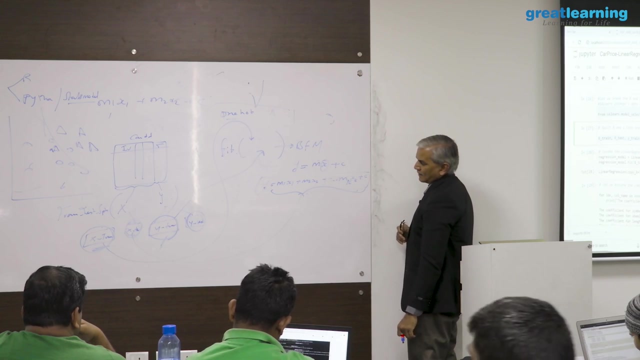 Let us the M1 0,1. 1.. This will be the model. Once the model, we want to evaluate it, we want to see how it performs. To this model I will supply the x underscore test values, which means these values: 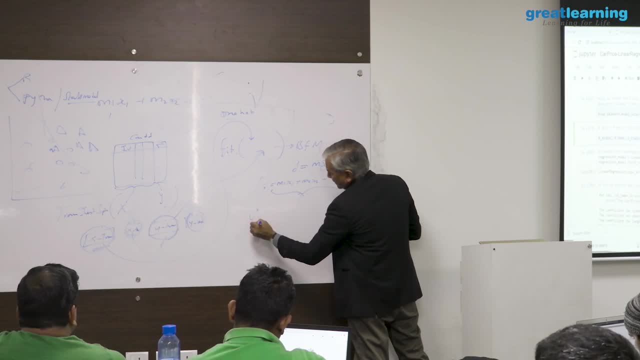 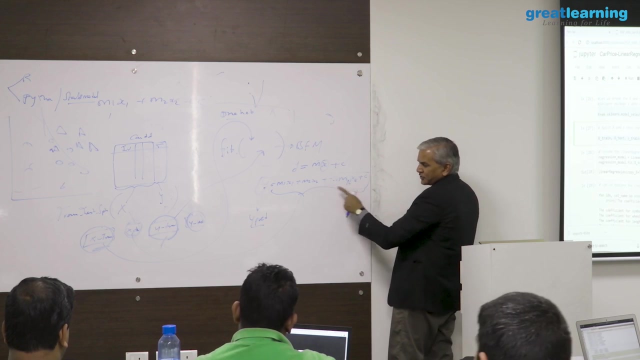 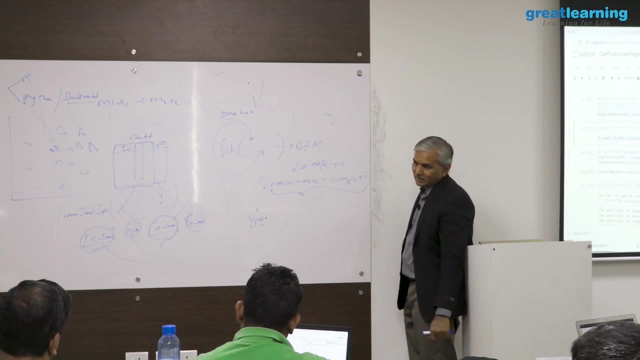 And it will give me the predicted values y pred. Are you getting it? So I supply the test data, the x underscore test, only the test data- to this model. The respective columns get multiplied by their coefficients for every record. For every record I get y underscore. what is the predicted price for this car? 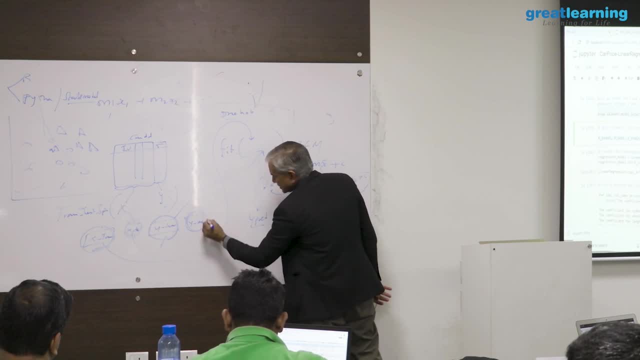 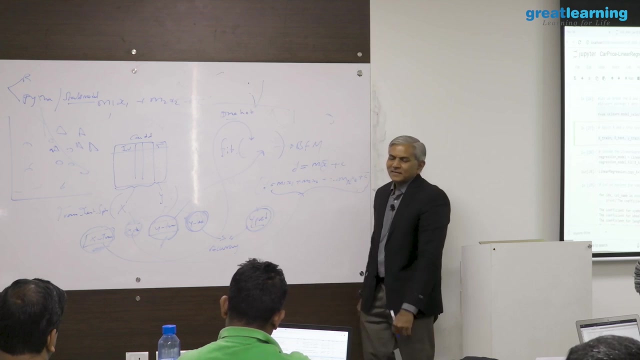 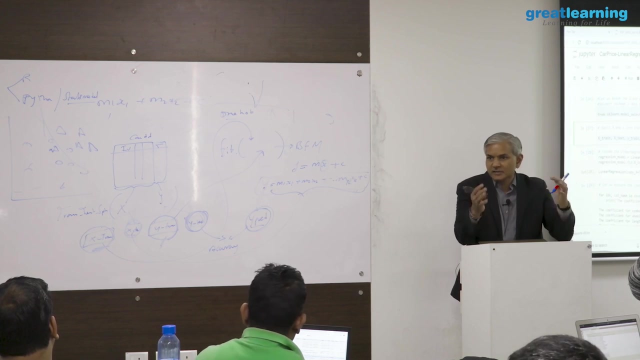 In the data set. I know my actual y underscore test is this: predicted y is this: What is the difference between these two? That will be my accuracy. Accuracy will be the difference between the y underscore test, which is actual test labels, versus y underscore pred, which is your actual test labels. 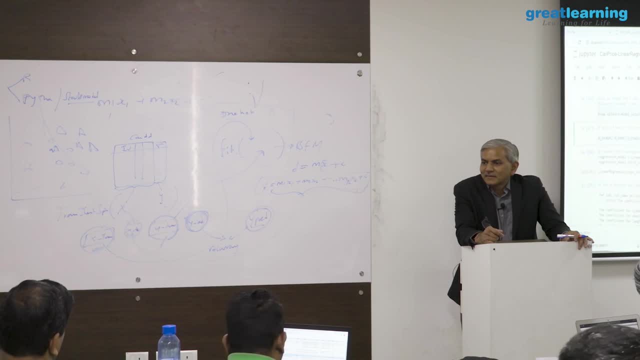 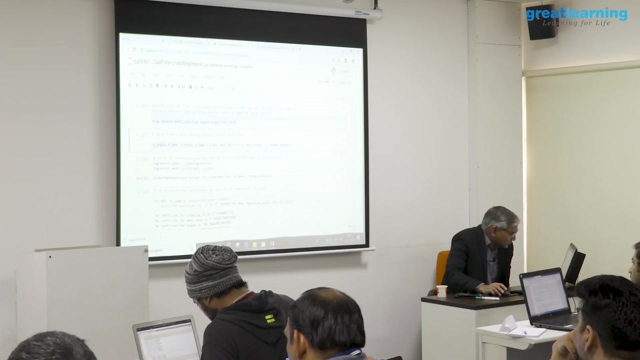 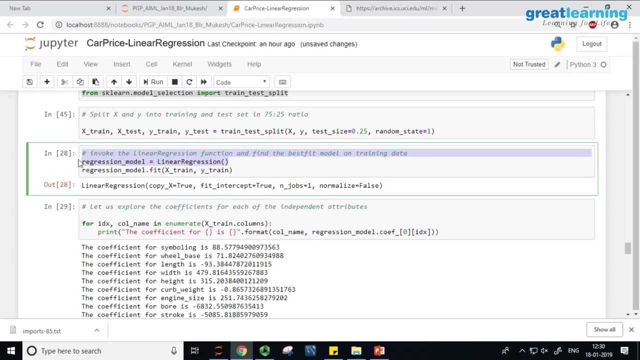 Your predicted test labels right. So let us see this, but before we go there. yeah, we will. I think we can do it comfortably. So let us look at this train test plate. I am calling the linear regression here. This is where I am instantiating the linear regression model. 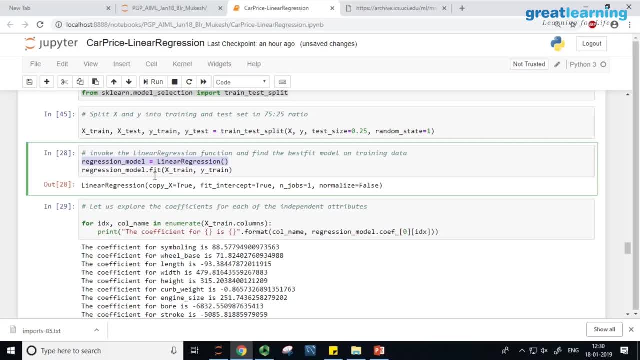 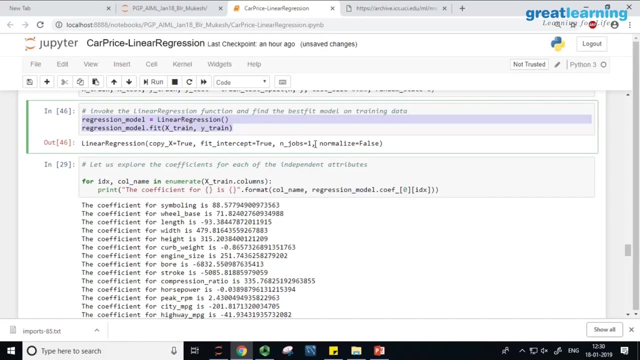 This is where This class becomes an object, and in that object there is a function called fit. I am calling that fit function and supplying the training set. When you run this, this is the point where the best fit line, using gradient descent, is found for you. 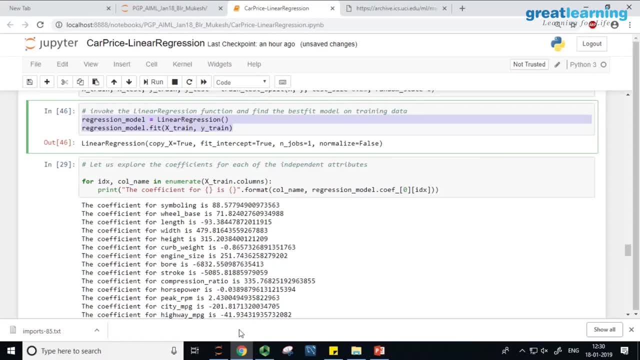 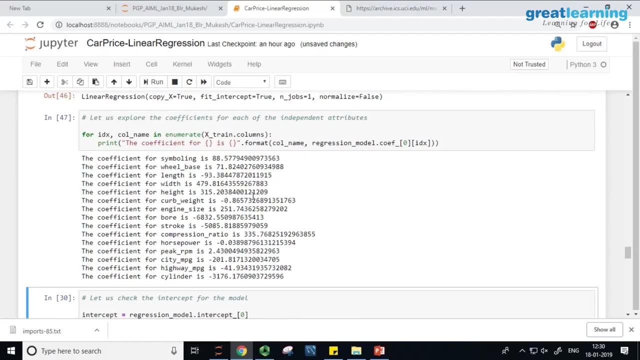 Now look at this. I am printing out the coefficients of all those: the best fit line, the best fit plane, hyper plane, rather. So when I print the coefficients, These are the coefficients. Now we need to understand what this is. You said there are 16 columns. 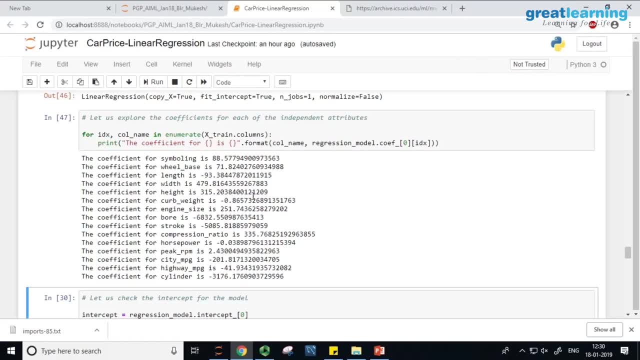 So the 16 columns have 16 different coefficients: m1, m2, m16.. This is that m1, m2, m16, m1 is 88.57, m2 is 71.82,, m3 is minus 93.38. 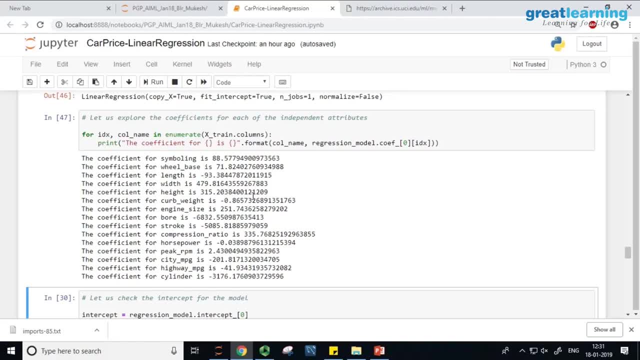 All these are those m1s. So let us understand what it is. Ok, What it means. What it means is for every one increase in symboling one unit increase in symboling the price of the car goes up by 88.57 units. dy by dx. 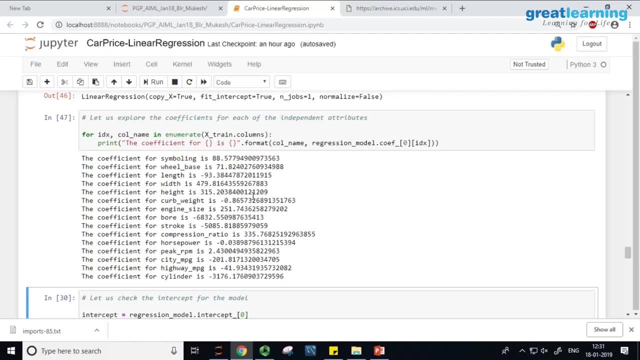 For every one unit increase in the wheel base, the price of the car goes up by 71.82 units. whatever the units may be, For every one unit increase in the length of the car, the price drops by minus 93.3 units. 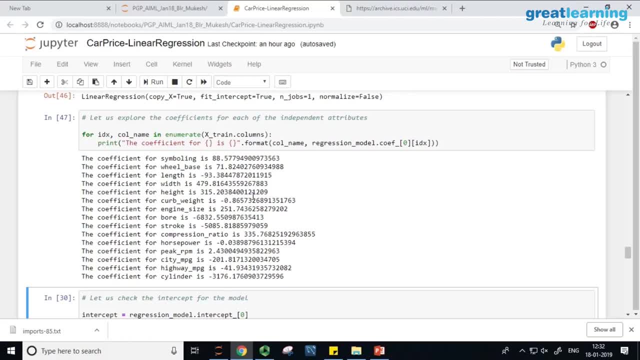 Now look at this. This is where you need to be careful. We know that wheel base and length are positively related. We saw that Then. how come one has a positive relation, other has a negative relation, But both of them should be positive. no, 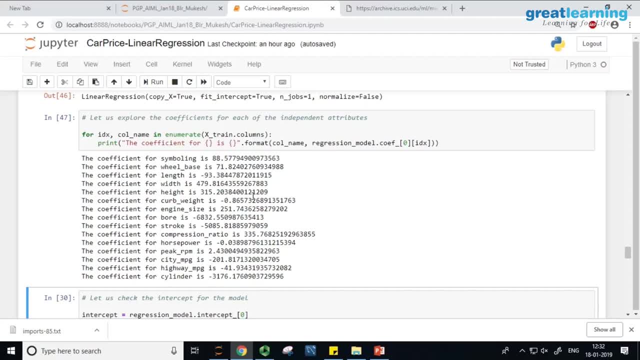 Wheel base and length are positively related, But one of them is having a positive impact on the target. the other one is having a negative impact on the target. How can that be? Such things indicate to you something is not right in your data set. 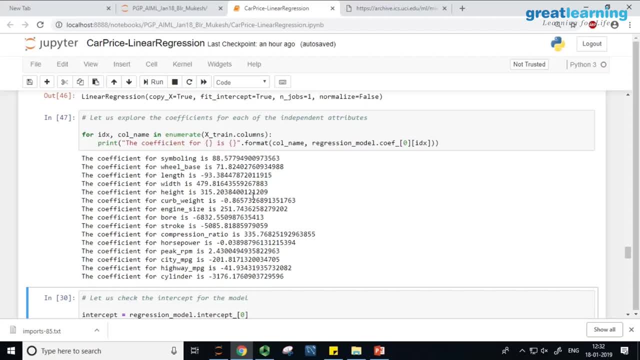 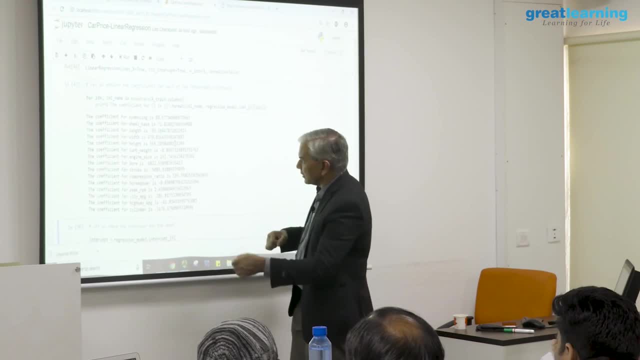 And one thing which is not right in your data set here we all know that is multicollinearity, Multicollinearity, Multicollinearity, Multicollinearity, Multicollinearity. Indian size, when engine size increases by one unit: the miles per gallon. sorry, not. 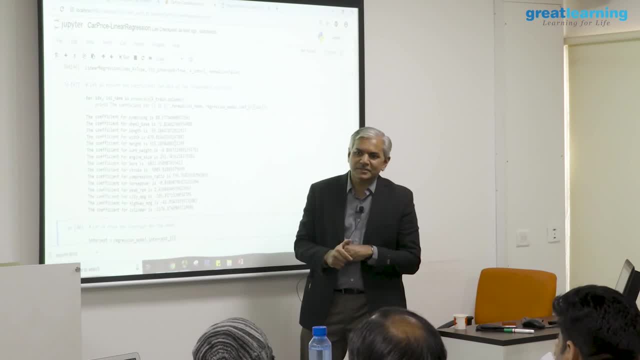 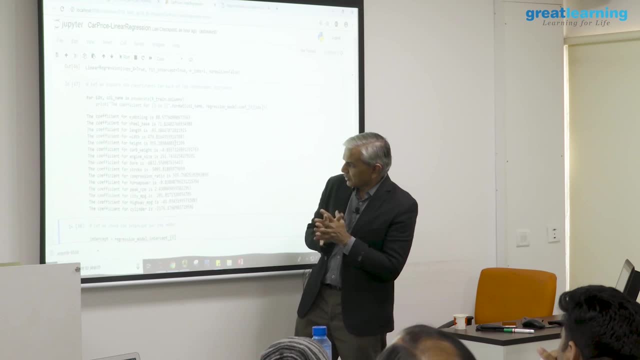 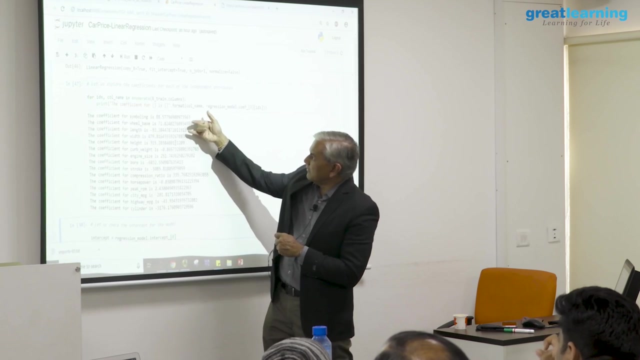 miles per gallon price goes up by 251.74 units. That is the way you have to interpret this. But what is happening is some of these ratios are kind of not gelling in. they are not fitting in properly. For example, we already found the length and the wheel base. they are going in opposite. 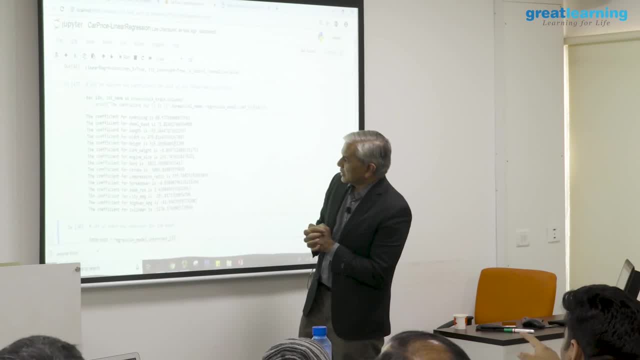 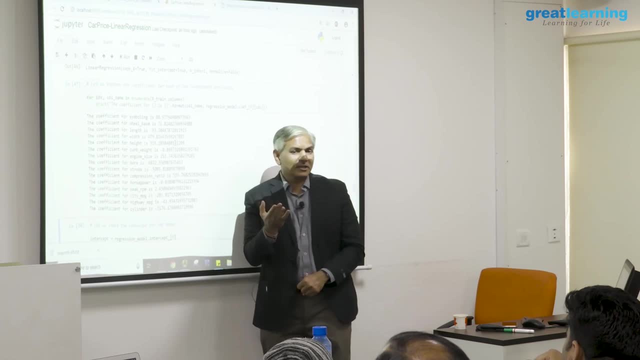 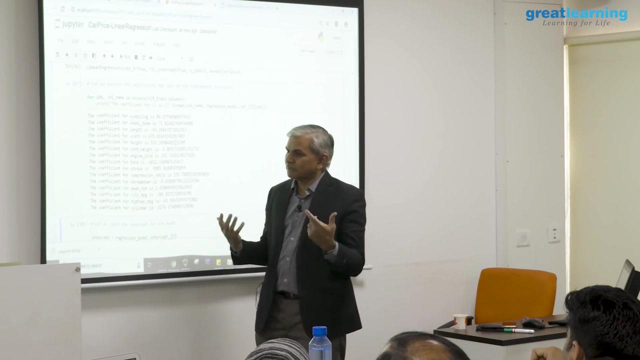 directions. Okay, Okay. Okay, That is one problem. Then we have horsepower. When horsepower increases by one unit, your cars car price goes down, whereas actually, when horsepower increases by units, cars price should go up. Horsepower increase means large cars, large cars, you pay more price. 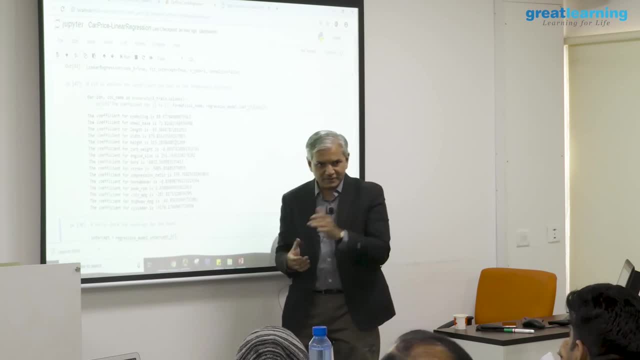 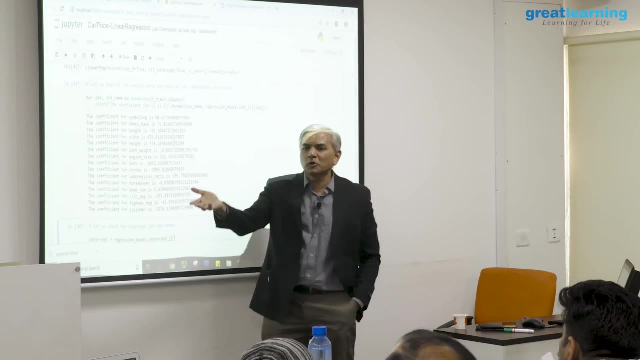 Bit more considered. but this is not only negligible, it is on the wrong direction, Right? Good point, Right So. So let us see: how do we try to understand these coefficients which are not falling in line with our domain knowledge? 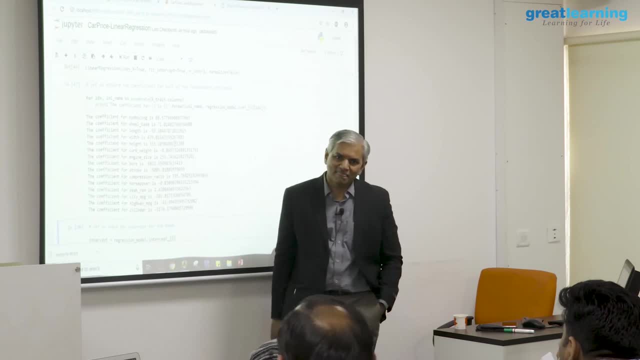 So this coefficient is what we are talking about, right? So is it saying the weightage kind of thing? Yeah, One thing I am trying to understand is when we say 88, okay, it increased by 88 when unit change, keeping other constant. 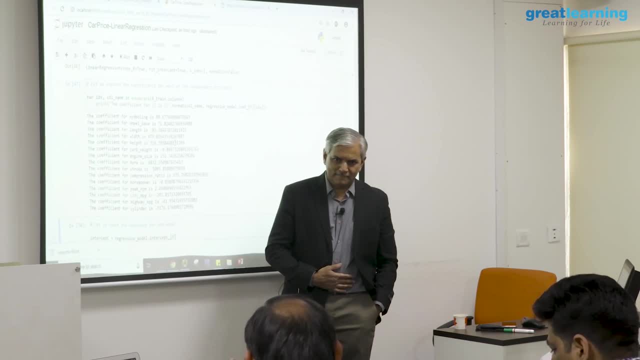 But some values is talking about 6000 line, 6000 scale. one is talking about 88. If we compare among each other, the value is the same. Is it the same? Yes, That is the problem. Is it the same? 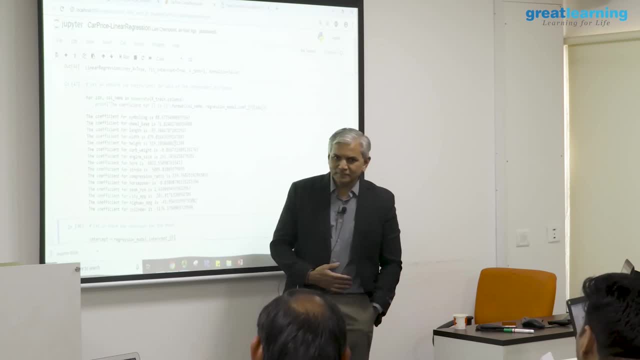 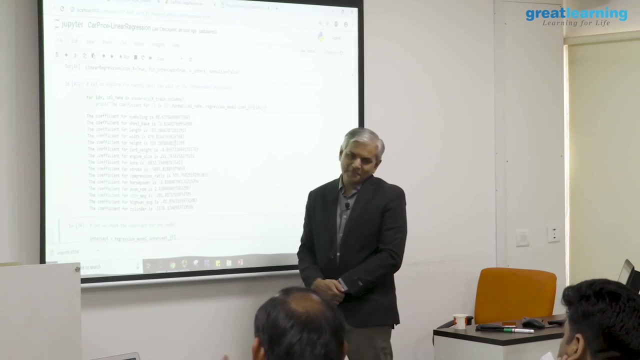 Yes. Okay, So you are saying, you are saying that the value is the same, right? Yes, The value is the same. Yes, How do you say the value is the same? Yes, That is the same. The reason why the 6000 is happening is probably you have an outlier on that dimension, which? 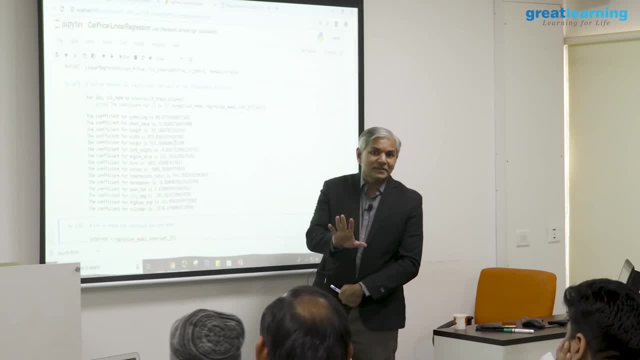 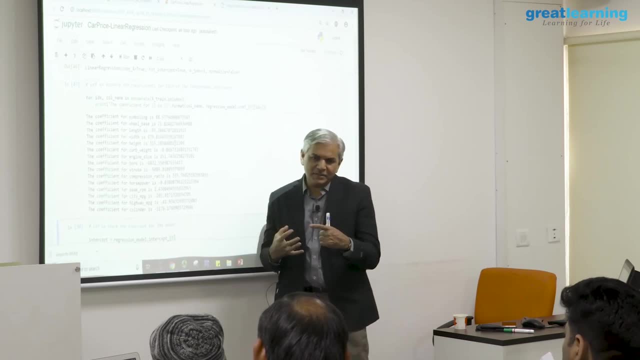 is pulling it right, So we have not addressed outliers here. one reason could be that. The other reason is: if you are, if you are not able to, I mean if these numbers are not falling in place, then we can convert them into z-scores. The entire data set can be converted into. 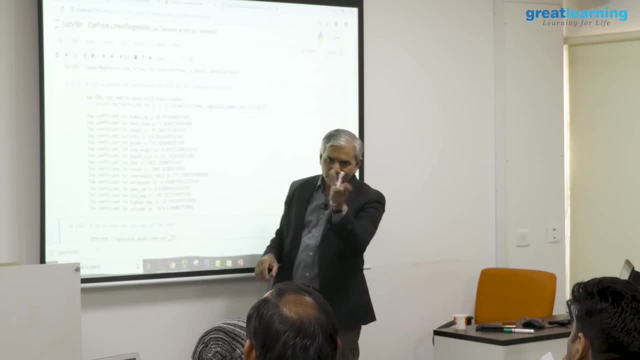 z-scores and then we can look at this. but the magnitude of the difference, you will still see that the magnitude is still there. ok, the difference is still huge. And the root cause of this problem that we are seeing, the root cause for this, is one: 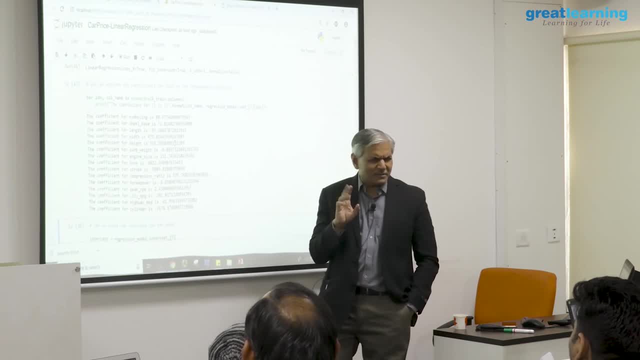 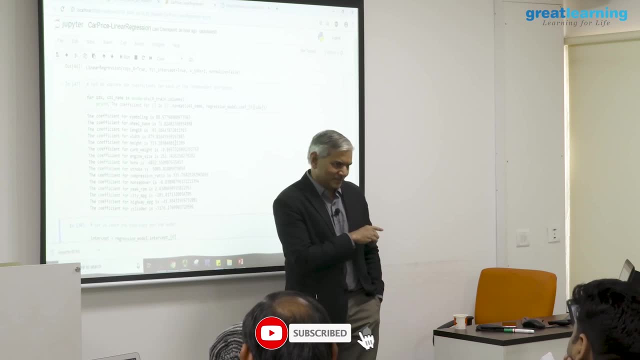 we have not handled the outliers. two, we have some kind of a what you call correlation between the independent variables, which you noticed we have not done anything about that multi collinearity right. So those are the core reasons which will come across in all data. 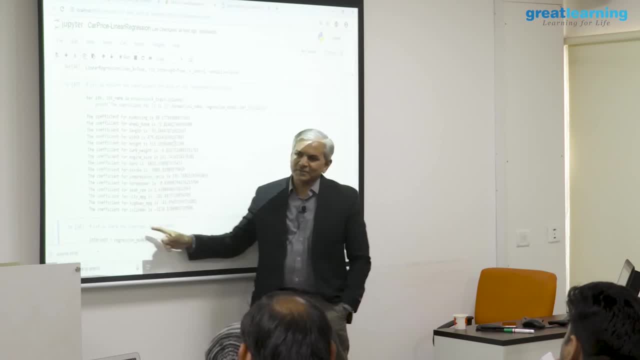 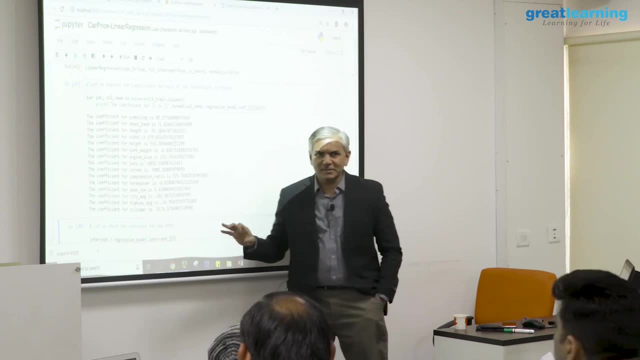 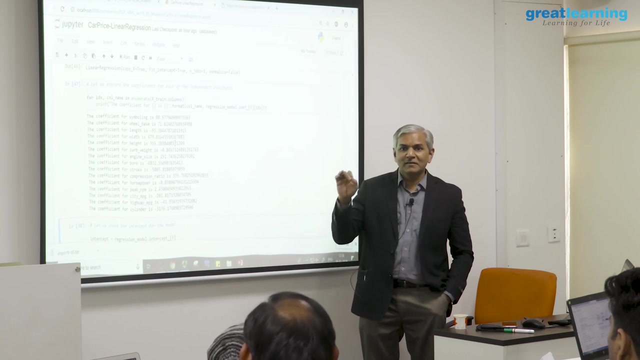 set which lead to overall model level problems. ok, Now I am going to take you through further down, into slightly more deeper stuff. Let me see if I can cover it today. if not, we will start with fresh minds tomorrow, because I need that particular thing needs lot of. 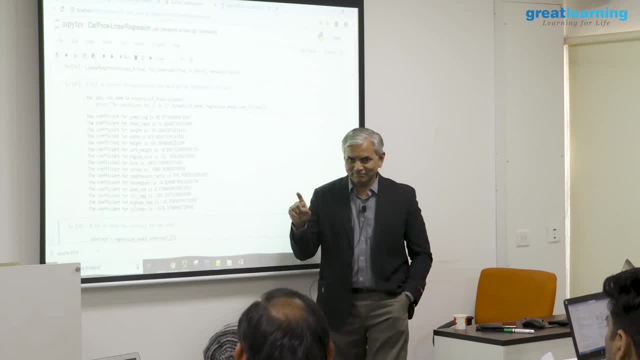 brain energy, Brain power, Brain power. So right now all columns has specific units. they are not normalized, So this coefficient is on the not normalized data Right. So it is always better to have to normalize the things and then calculate the coefficient. is it like that? because otherwise we are not able to create the coefficient. The coefficients will not change when you normalize. it does not matter. By normalizing you are just centering the data to 0.. The the relationship between y and x will remain. 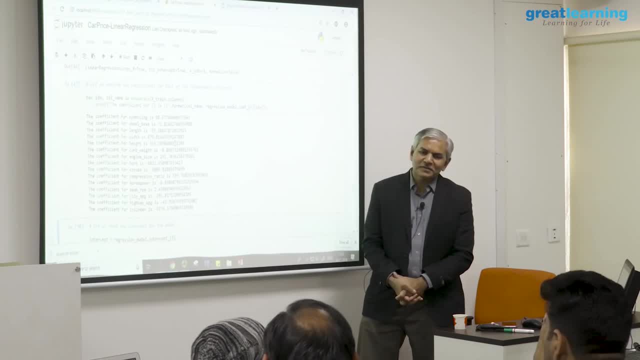 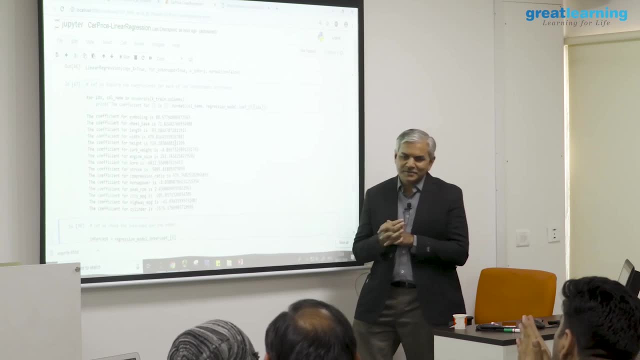 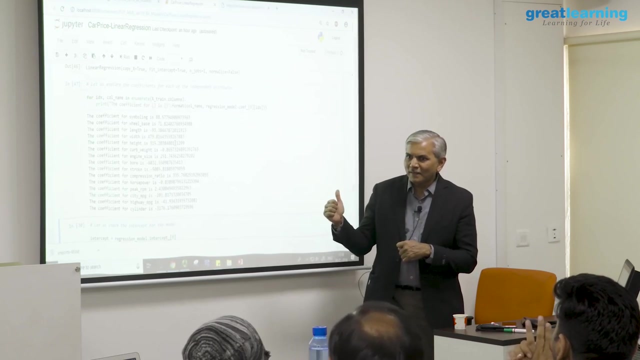 same whether it is a normalized data or a non normalized data. coefficients will not change. Linear regressions are not impacted by normalizations. The accuracy score, the coefficient, everything remains same. ok, Shall we move on? Yes, So linear regression only gives a coefficient m, but not the power of that x square. those. 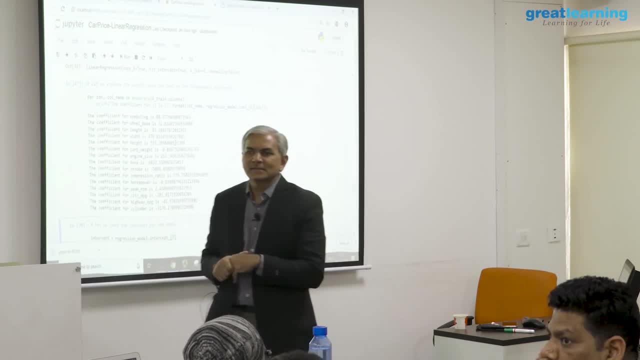 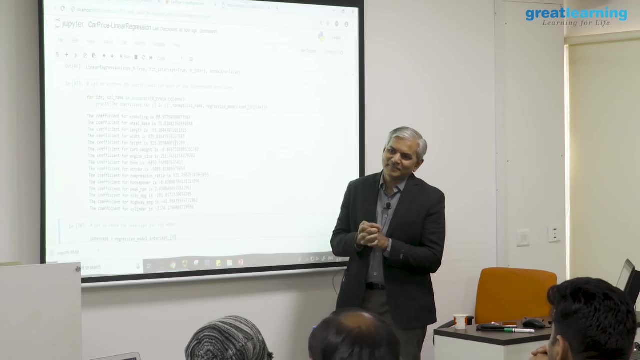 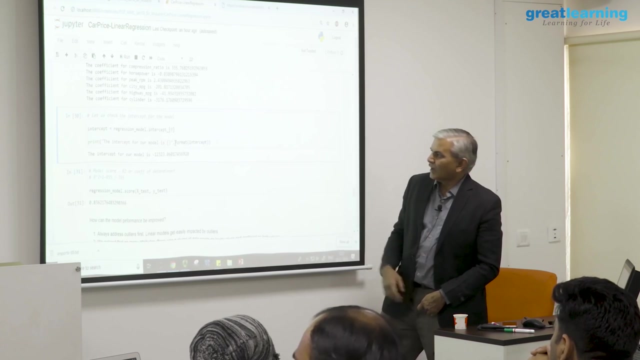 things. Yes, So linear regression only gives a coefficient m, but not the power of that x. square those things. No, no, this is simple linear model. If you build quadratic model, then it will right. So let us move on and let us see the intercept. This is the intercept. I am printing the intercept. 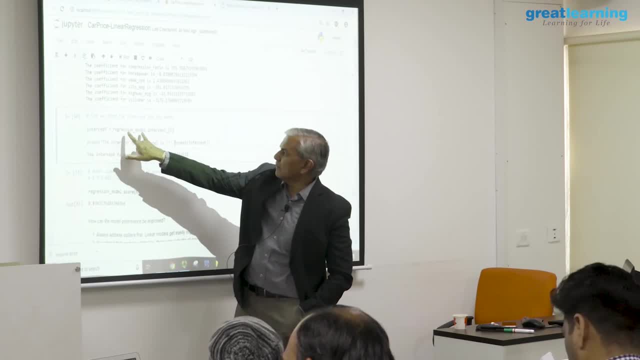 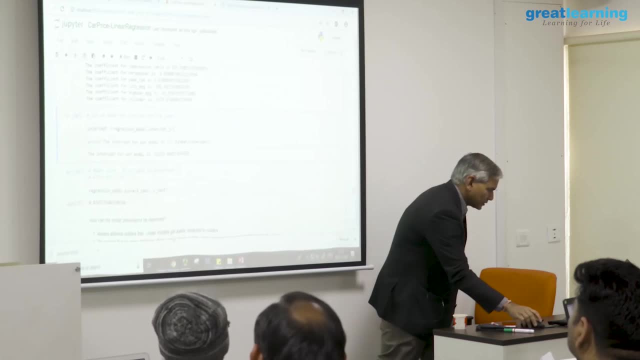 What you need to do is model dot intercept. This is the model name. model name dot intercept This function. this function will give you the intercept, Whereas if you want the coefficients, you have to use model dot coefficients. Look at this. 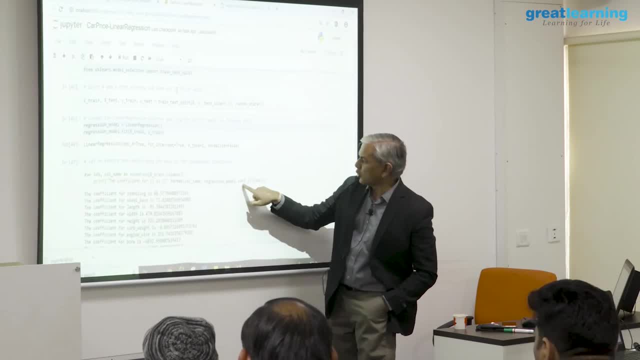 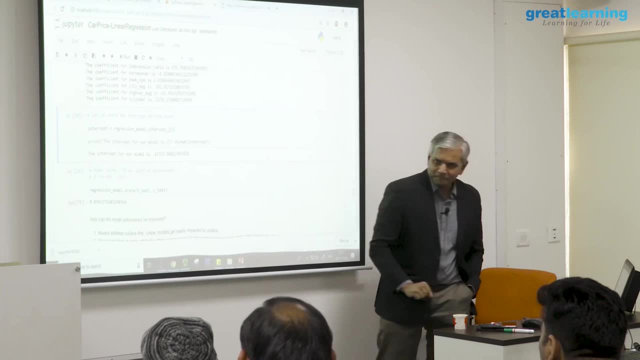 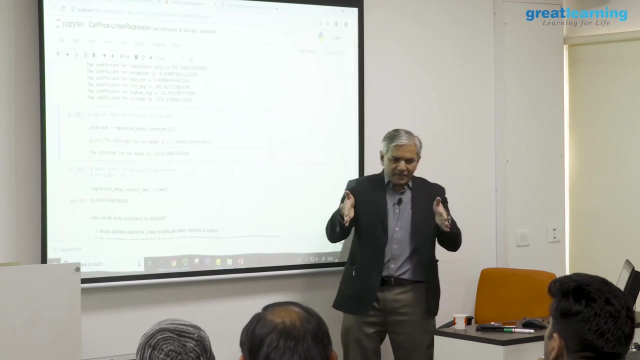 For coefficients. it is model dot: coef underscore. Coef underscore will print the coefficients. Model dot intercept will print the intercept. Now the intercept that we are getting is minus 1, 2, 3, 2, 3.. There is an array. In that array we are passing the index. This: 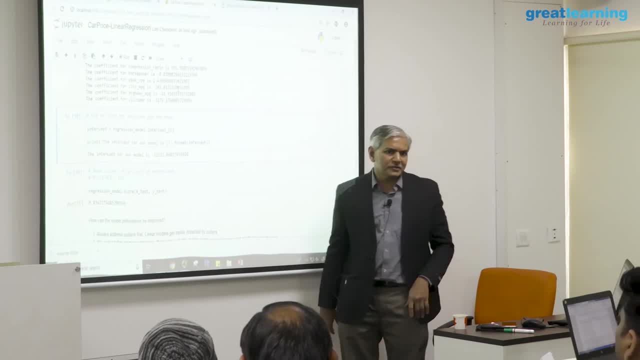 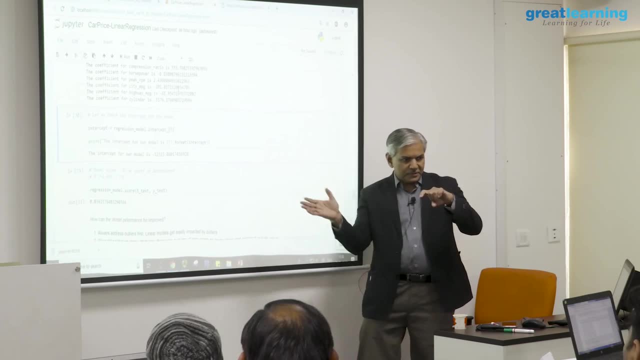 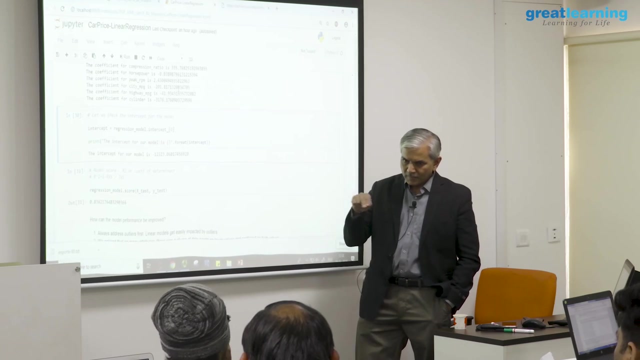 is the first one is intercept. In the other array we have the coefficients. I am just trying to Coefficient of the passing field. Yeah, that is a different array, Right? So I am saying Passing, Passing No, no, the zero and value coefficients. 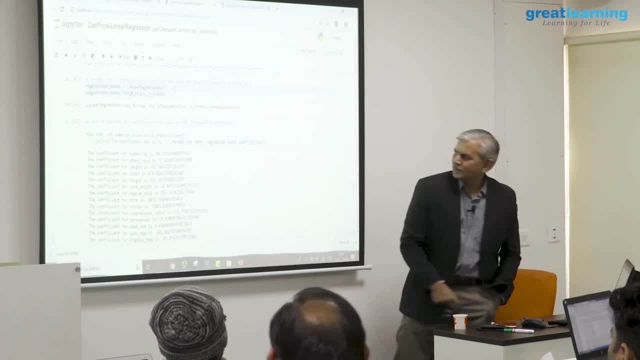 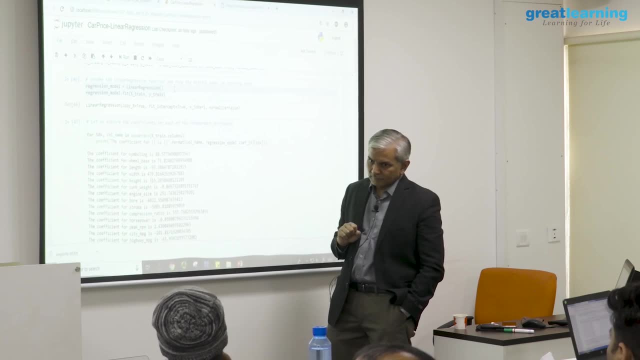 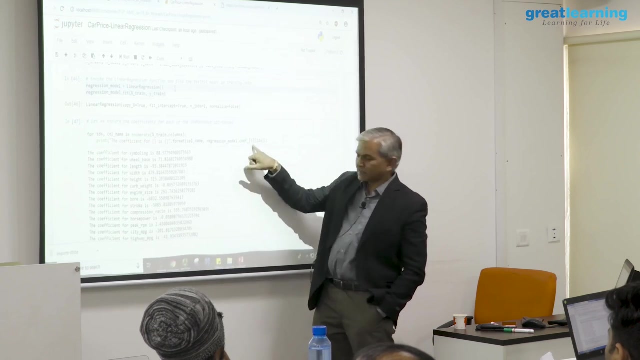 I mean the data set, dot coefficient Data set. I just typed that code. data is not showing. Now are you sure you are getting 0 and a IDX? No, no, you have to do this. See, this is. this is a different array. In that array. 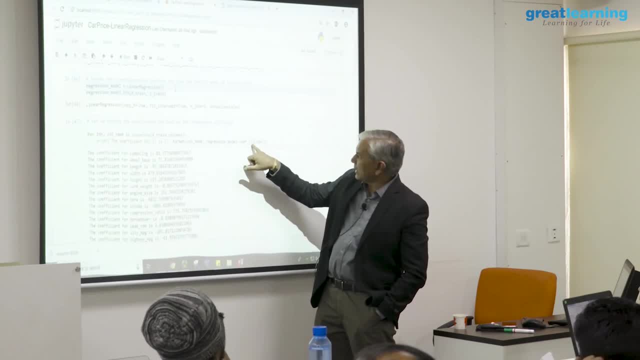 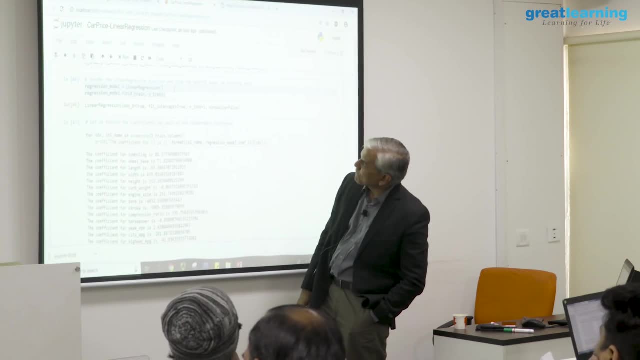 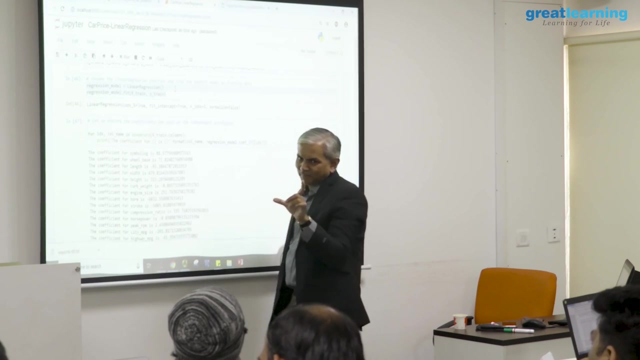 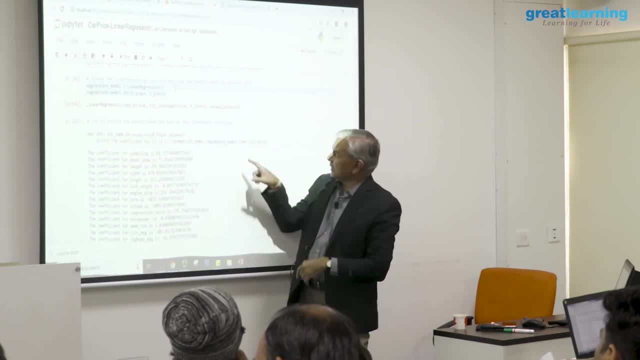 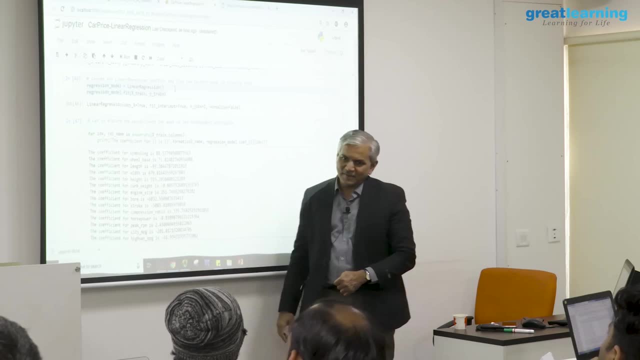 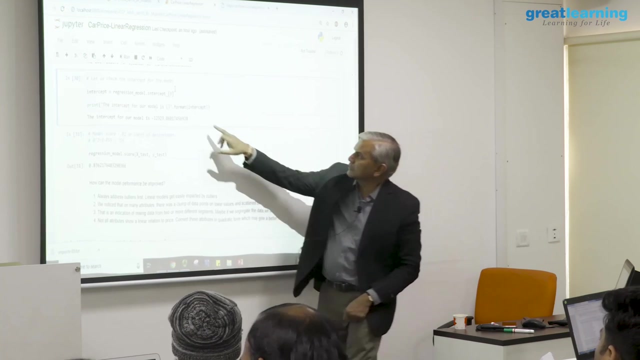 fit line has coefficients. all the coefficients are internally stored in an array which is accessible through this function. This function is accessing that array and printing out the results. Similarly, there is another array for your intercept. it is accessing that array using intercept. We do not know what that name of the array is. we can only access that. 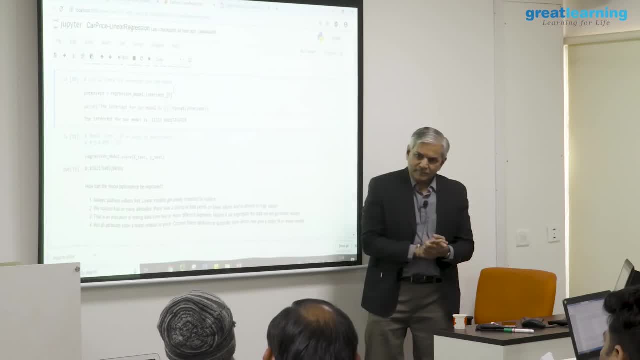 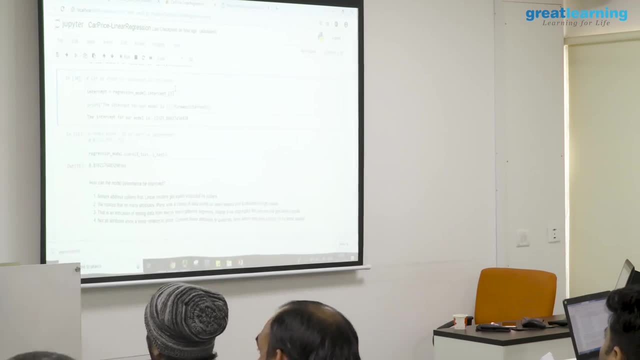 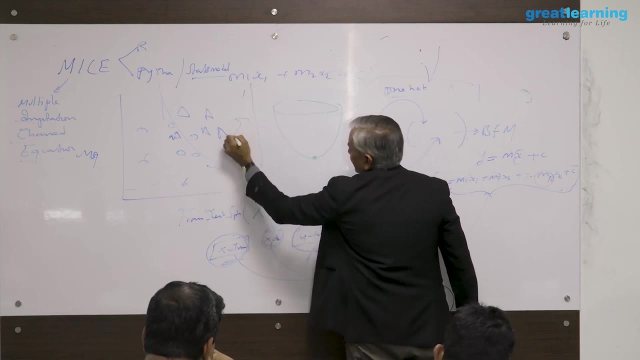 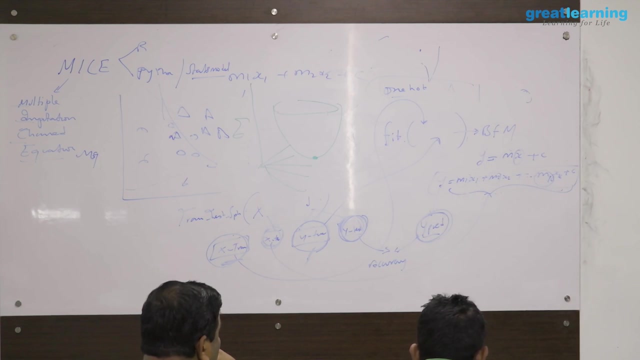 array through this function. This point in the graph, all these coefficients in the graph are the lowest points. This is the lowest point in your error. This is error. There are multiple 16 dimensions over here. This is the lowest point. This combination of coefficients gives the lowest. 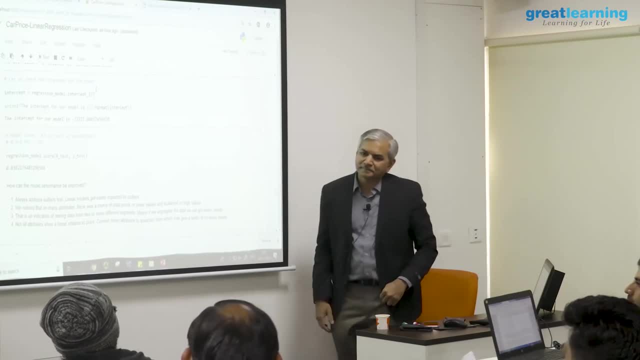 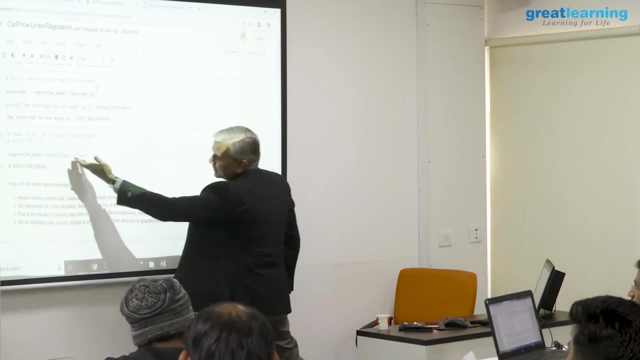 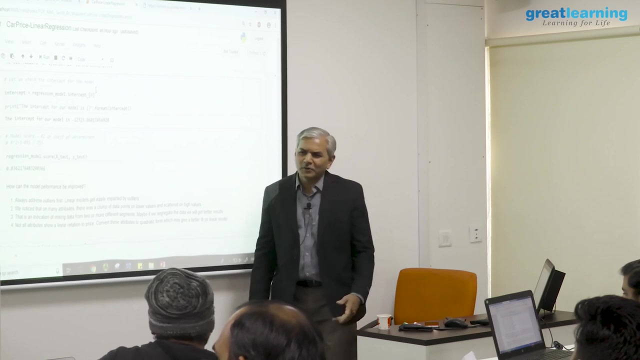 point in the error graph the best fit right. So let us look at the performance of the model on test data And, as you can see, performance on the model on test data is 83.6 percent. Not bad, not good either. 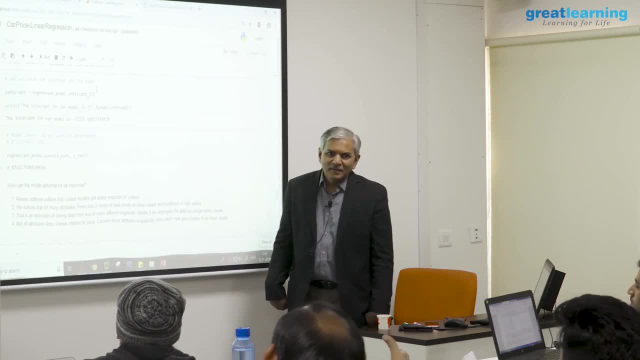 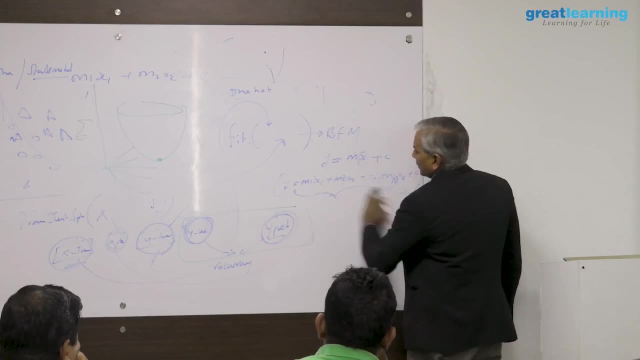 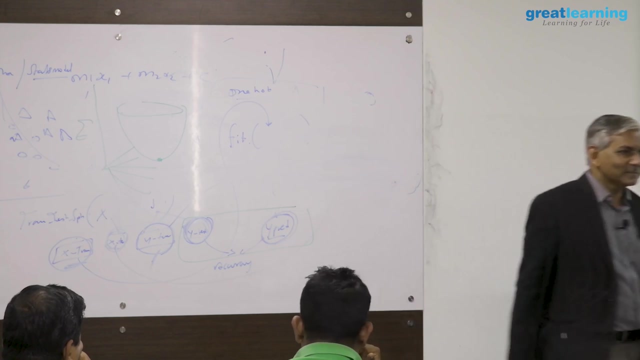 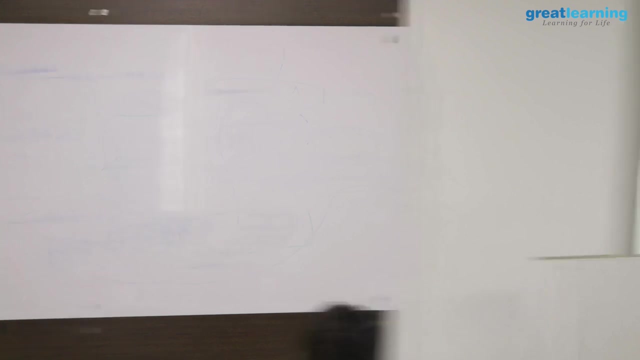 So what does it mean? 83.6?? The comparison between this and this. ok, So the 83.6 percent. what do you think it is? No, no, no, no. This is your coefficient of determination: 83.6 percent of the total variance. 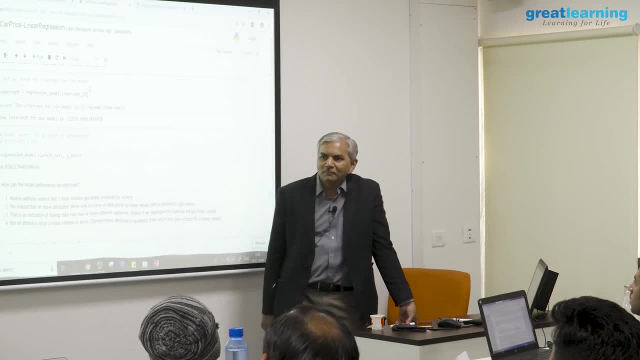 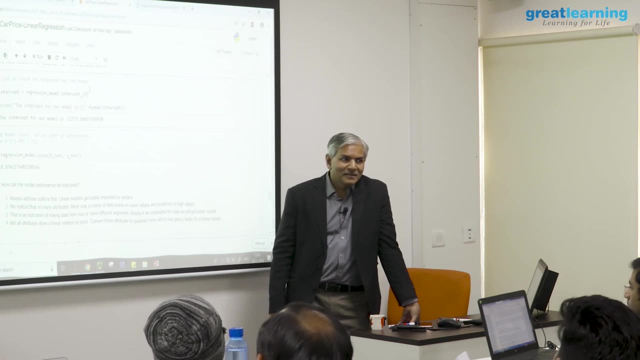 in your data test data has been capitalized Correct by a model R square. this is not adjusted R square. this is R square. That means I have written, I do not know why. Yes, it is That we do. 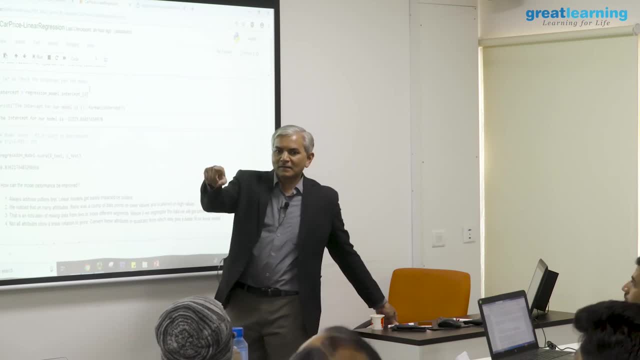 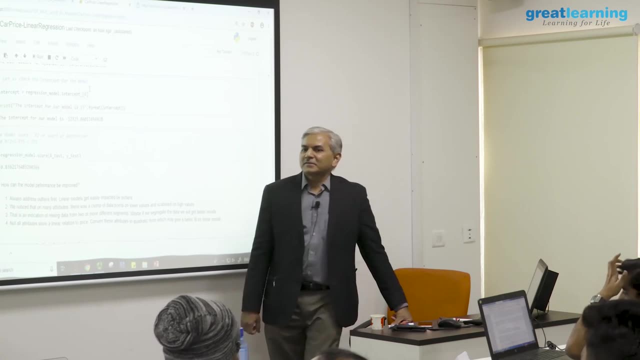 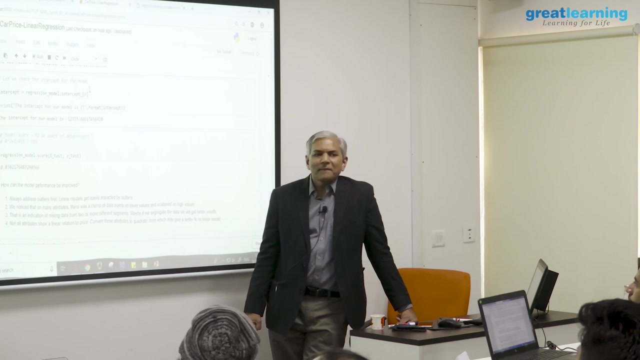 Yes, suppose for that X minus mean, X minus X bar raised to power 2 by n, that residual error is 17 percent R square. 17 percent of the variance in the test data has not been expected. Intercept is one of these dimensions. 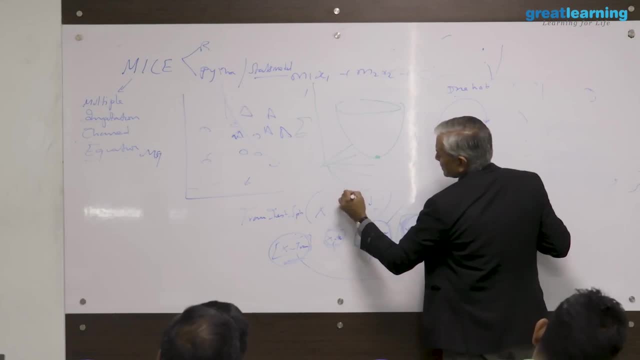 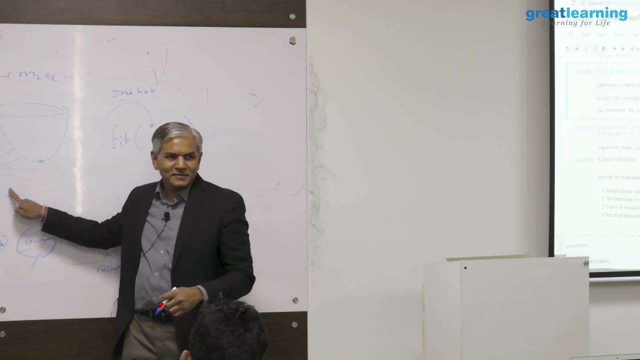 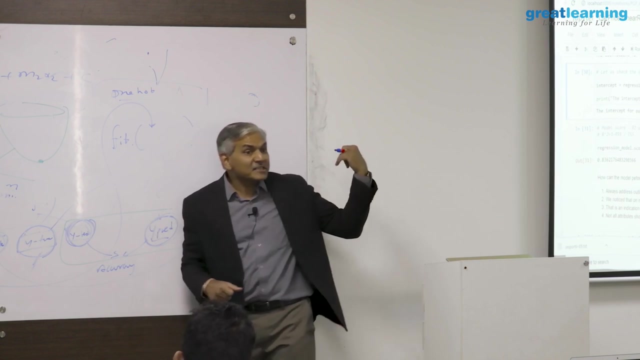 Error is a function of slopes and C Error is a function of m and C. So C is one of the dimensions. What I showed you earlier was only one m and C. Here you have 16.. 16 m's and one C. We cannot visualize it so I am not able to show it. 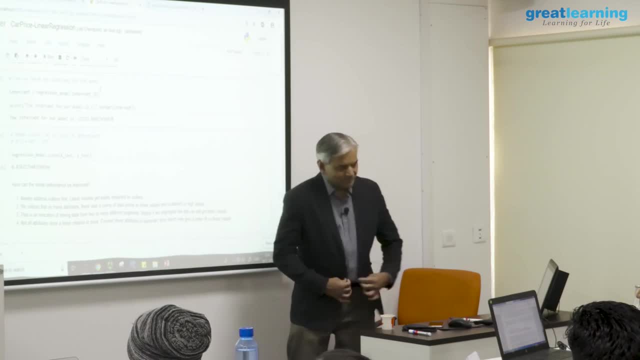 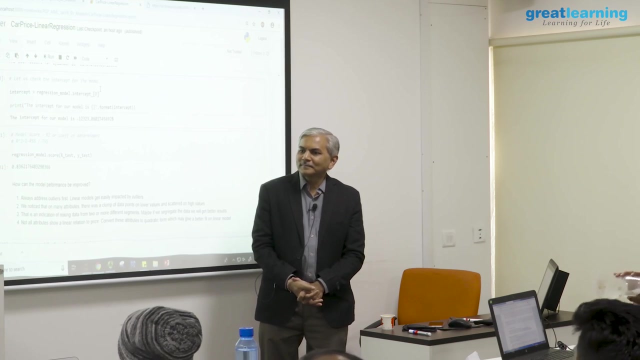 It is 83.6 percent prediction in that model. It is the coefficient of determinant How much of the variance in test data has been captured by your model, explained by your model. Shall we move on? Ok, Now we need to improve the performance of the model. 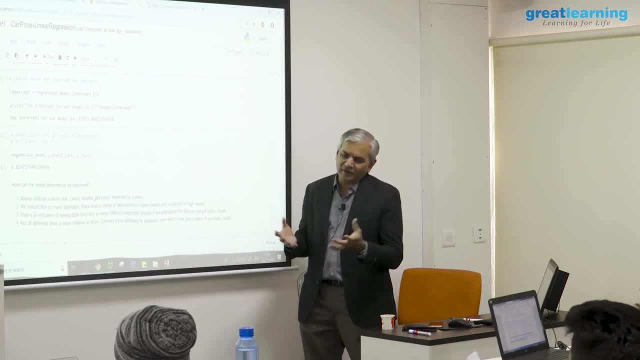 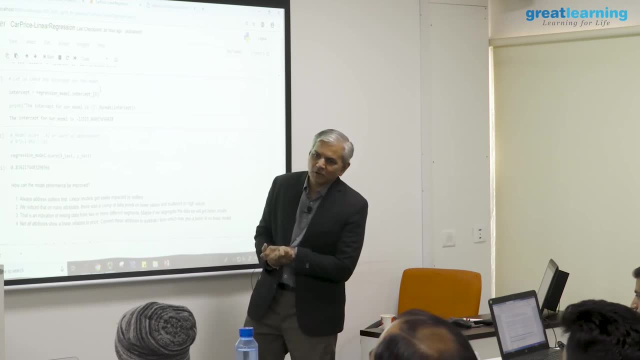 Your first cut model will never give you a result- Very rare. So you will always end up in another cycle where your objective will be: how do you improve the performance of this model? How do you notch it up? So there are various things you can do. 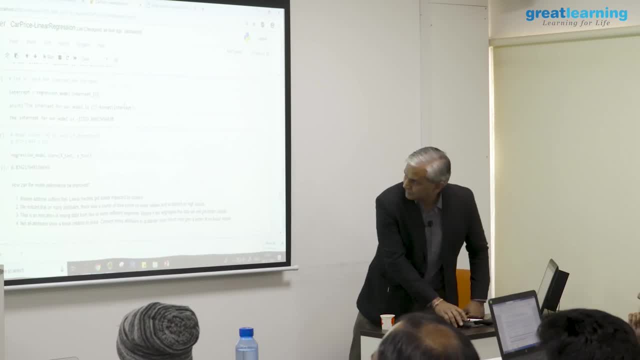 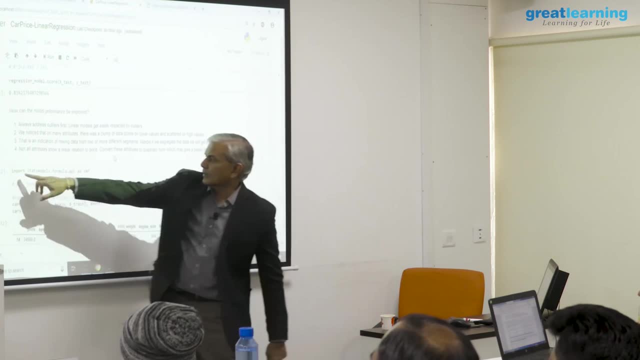 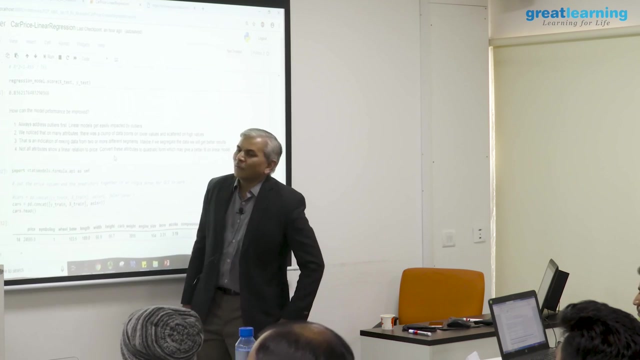 But before you do that, I would like to introduce you to a library called stats model. Stats model, the formula, API, SMF, Stats model functions. Ok, What happens is when you build this linear models in R. R gives you a lot of statistical. 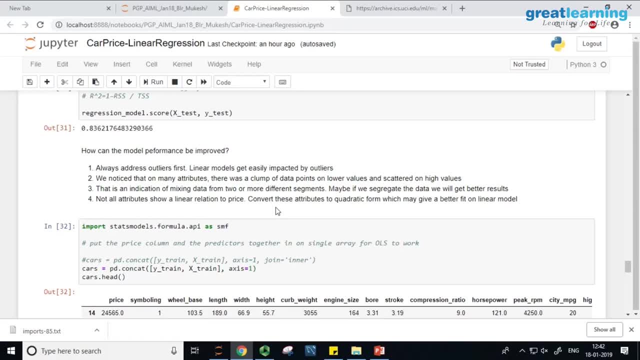 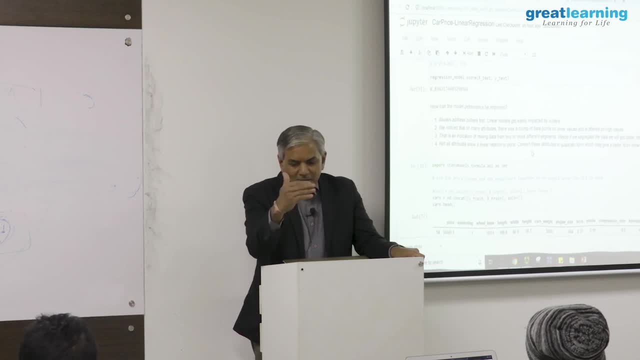 information about your attributes and your models. Scikit-learn, linear regression, does not give you those information, But there was a lot of demand for that kind of R kind of analysis in Python. So those people who support Python, Scikit-learn. they came out with this library called stats. 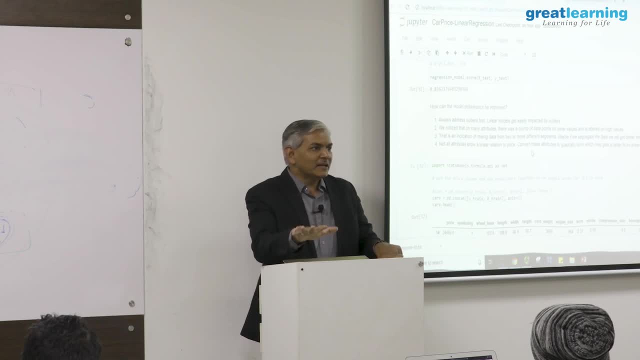 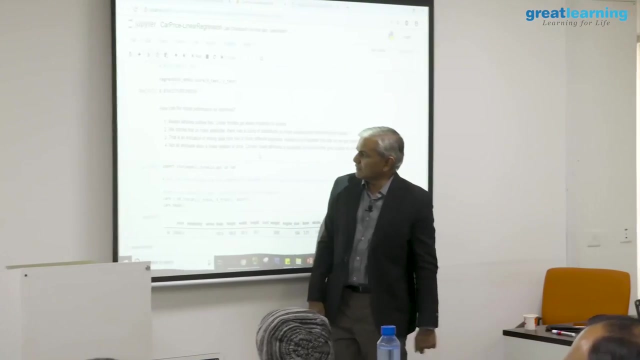 model. Stats model tries to replicate the behavior of R Ok And gives you similar kind of statistical analysis as you would have received or gotten obtained in R. So let us see what it does and why is it required. So I am importing from importing stats model, dot formula, dot, API. 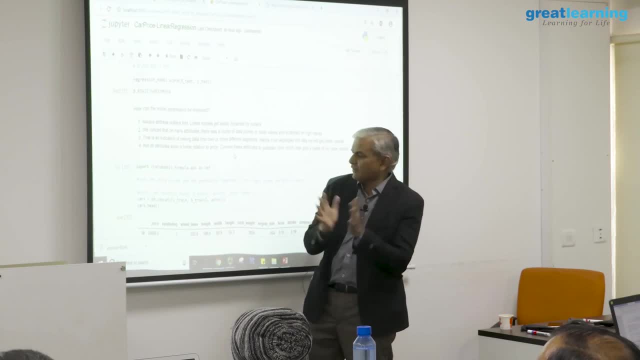 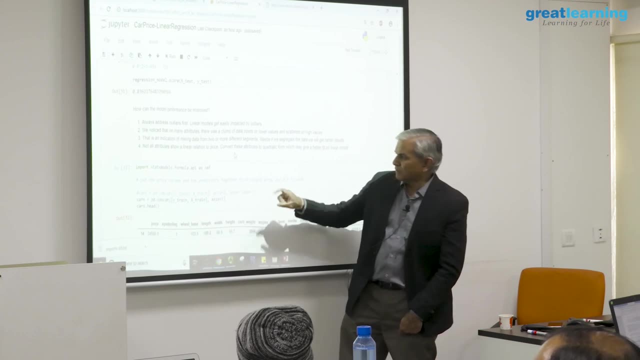 I am importing something called SMF. SMF is a bunch of statistical functions And this. I am going to build a linear model using this. But before I do that, But before I build a linear model using this, I have to combine my X train, Y trains into. 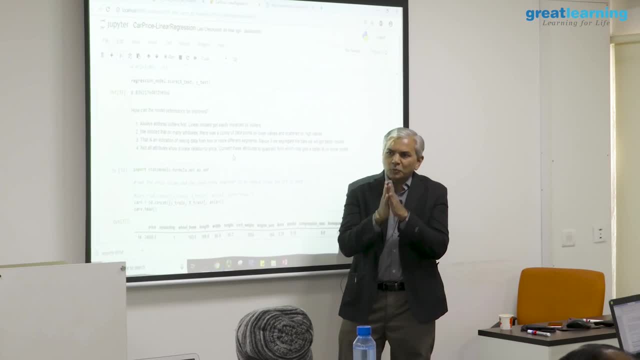 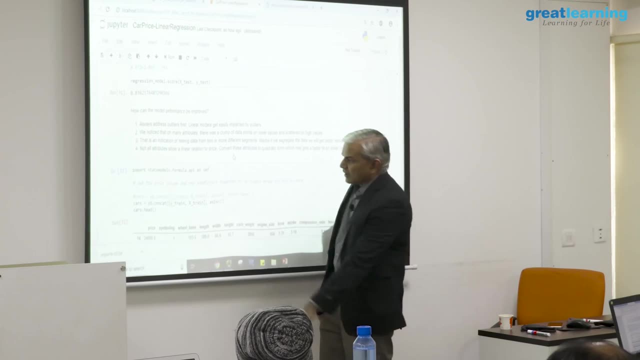 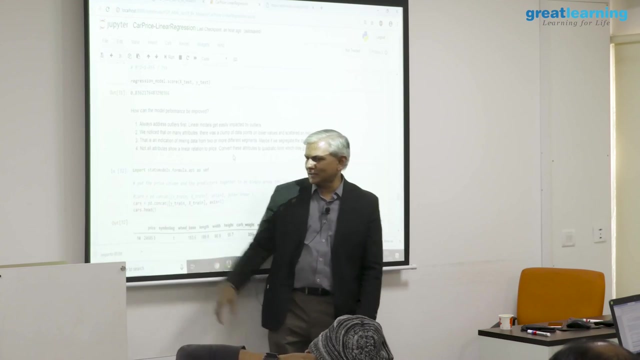 one data frame. because R takes as input one single data frame, It does not take independent variables- dependent variables- separately, So I am recombining the two into one. using concat function. I am creating a new data frame called cars, which now has both the Y and the independent. 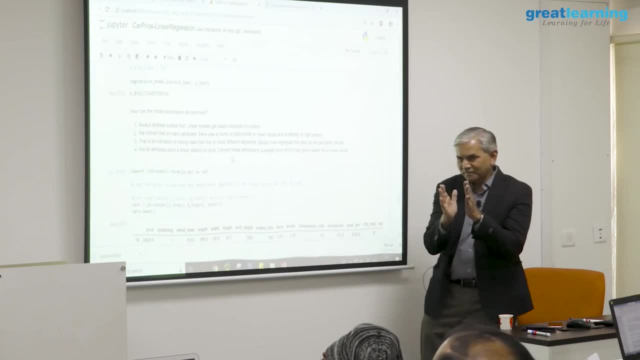 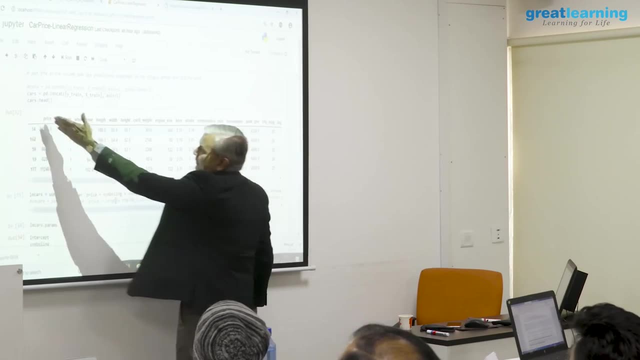 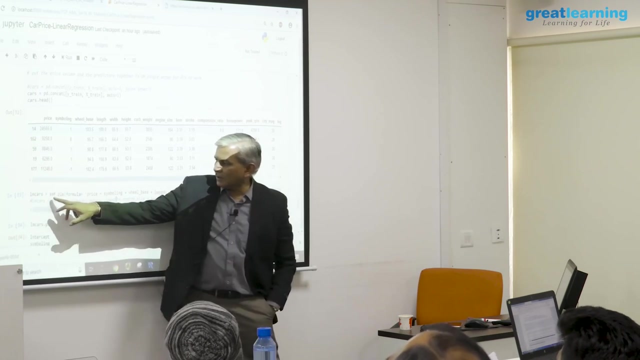 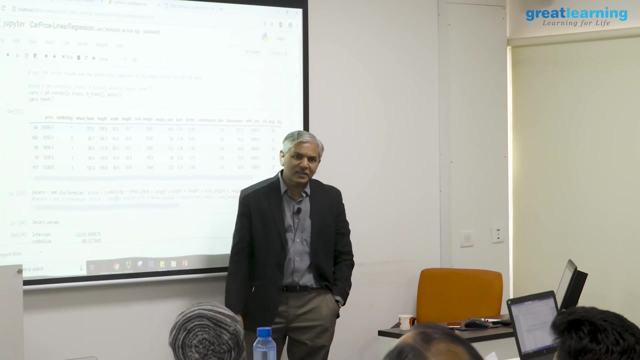 variables put together For training, For training. Ok, Now look at this. When you do cars head, you get the price column on the first point, first column, and the rest of the columns. Now I make use of the SMF dot OLS. OLS stands for ordinary least squares, linear regression. 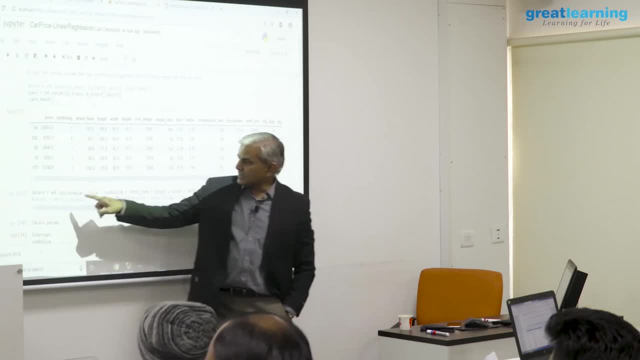 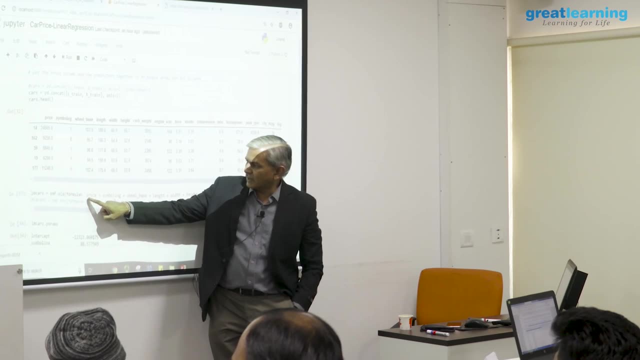 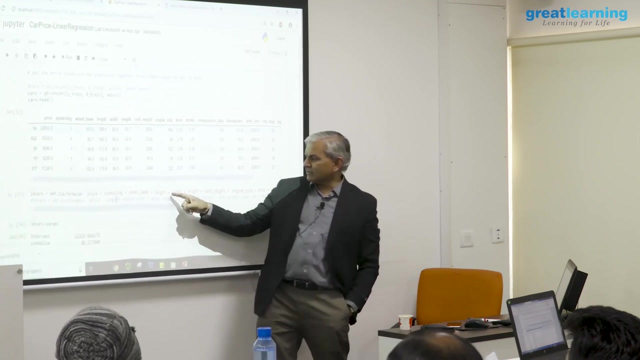 linear regression, ordinary least square. And as input to this function, And as input to this function, And as input to this function, I give price a formula where I say price is a function of the various columns, The plus which you see here. this plus is a field separator. 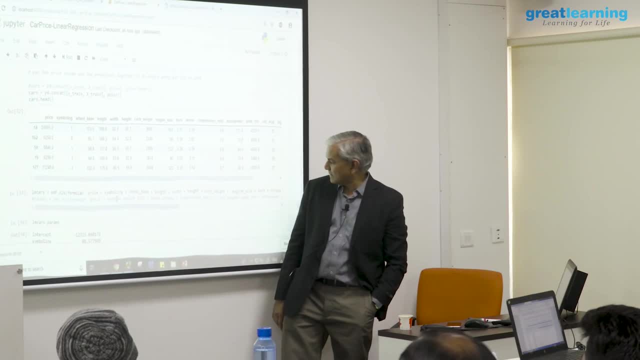 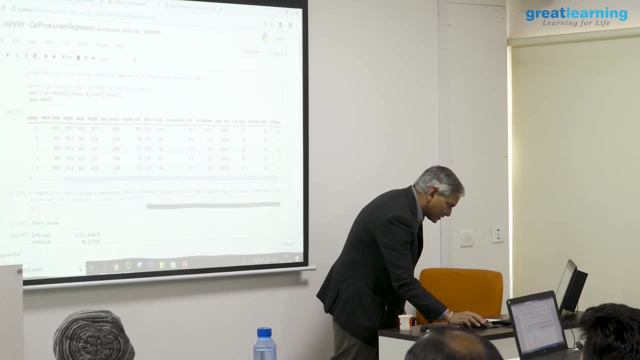 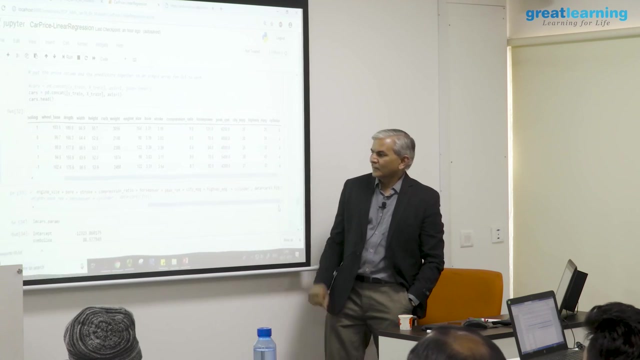 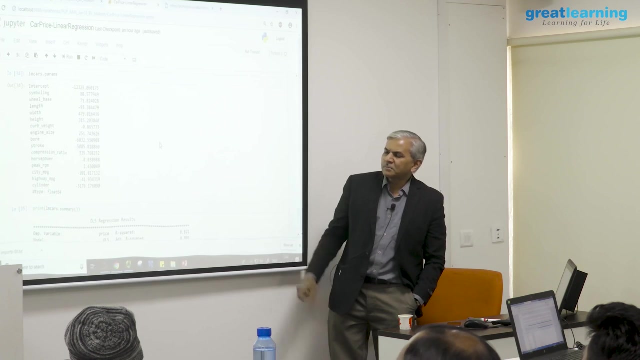 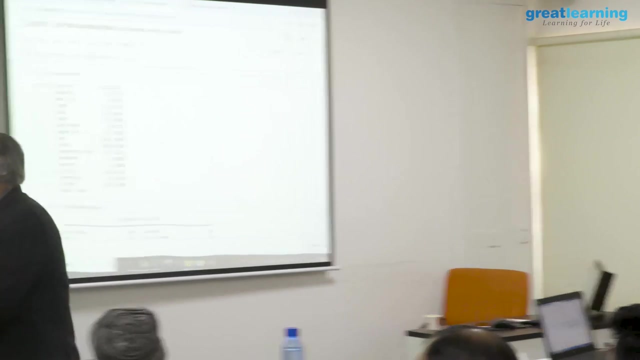 It is not a mathematical plus, And at the end of it you will see the data file name. sorry, the data file name is cars. There you go. data is cars. So the output of this is once again the same model, But this model has been built in R, R based R, similar to R libraries. 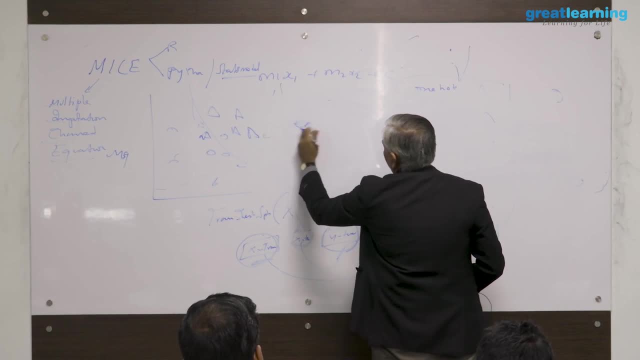 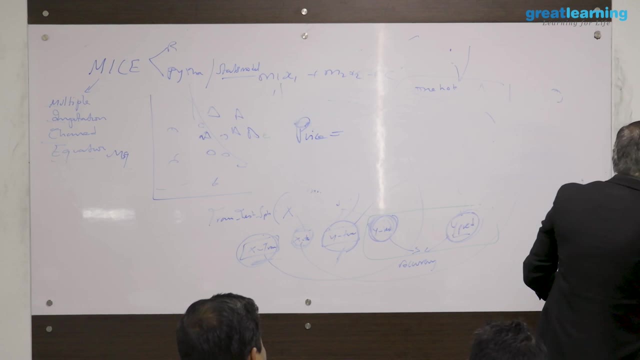 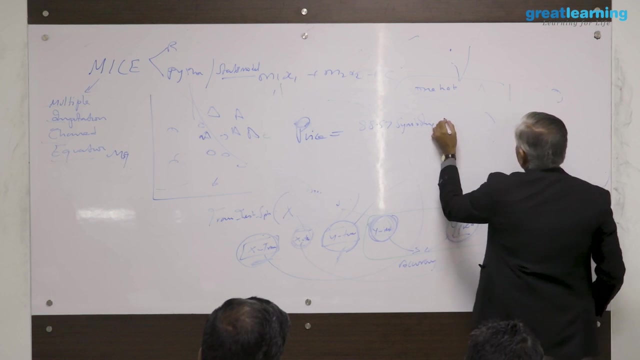 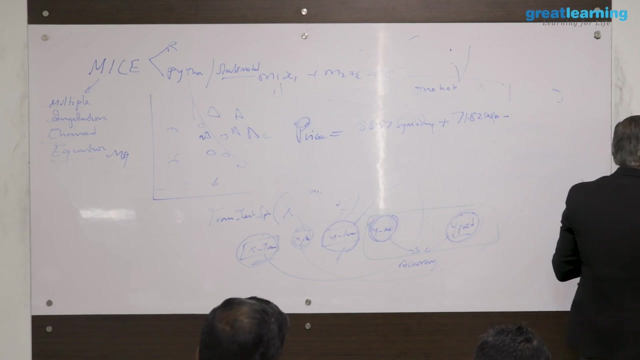 So the model is: price is equal to Price, Price, Price, Price, Price, Price. So I will take the intercept and later. So the symbolic is 88.57 symboling plus 71.82 wheel base minus. I will just take one more. 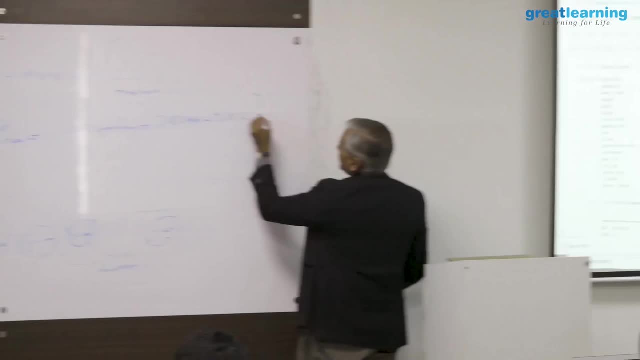 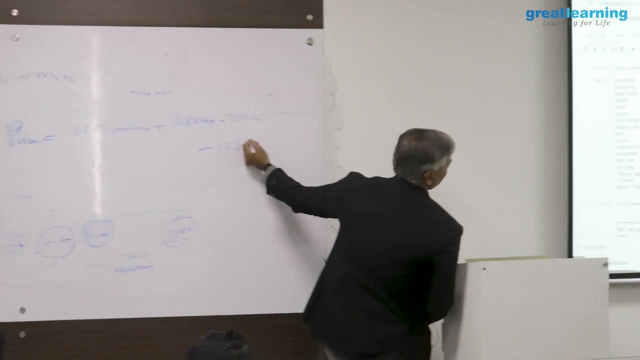 93.38 car length, CL, and so on, so forth. The last thing being minus 123.. existem Snow cube. The last thing being minus 123.慢 뭐, 3 Minus 123.. um, And so on, and so forth. 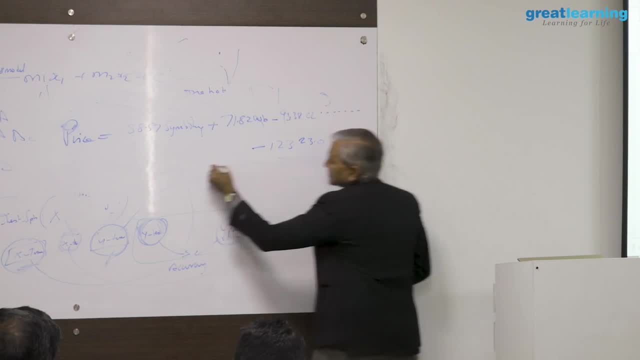 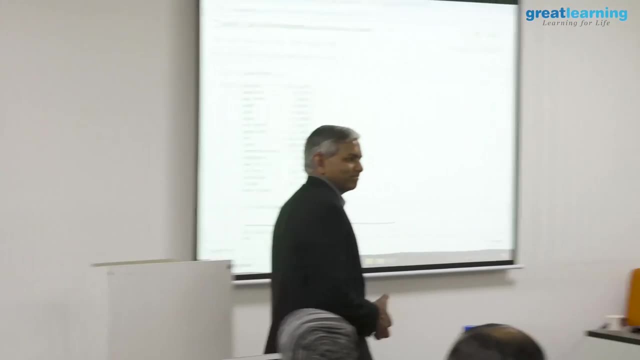 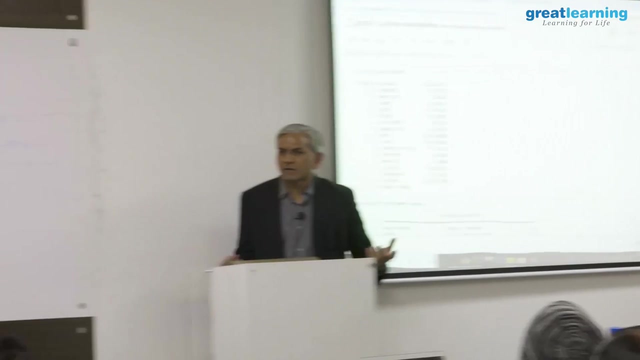 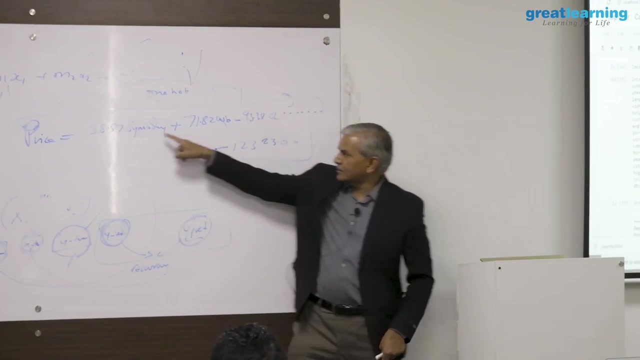 And so on and so forth. 06 or something, intercept. This is your model. This is the representation of your best fit line. Now you can write a code in Java. in Java, where you have a function where function takes as input 16 variables, multiply those variables with the respective coefficients. 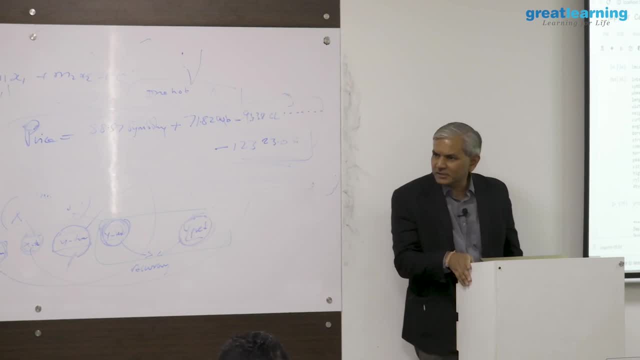 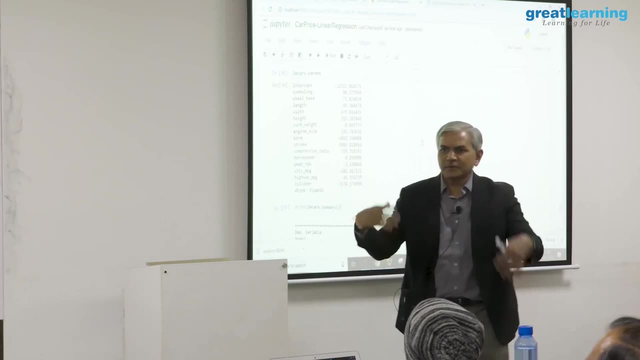 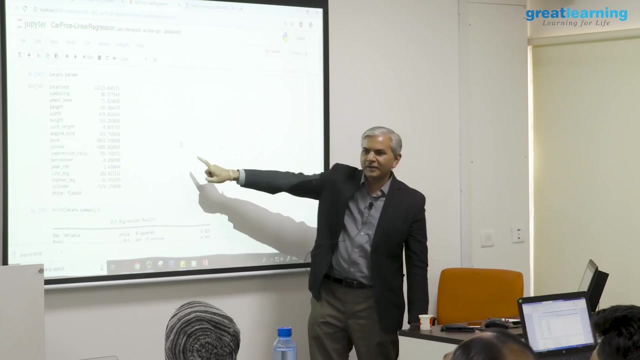 subtract this intercept from that and give the output as a predicted price. Convert that Java code into runnable jar file. productionize it. your model is in production, alright. So that is the model, Same model we got in scikit-learn, same model we are getting here. 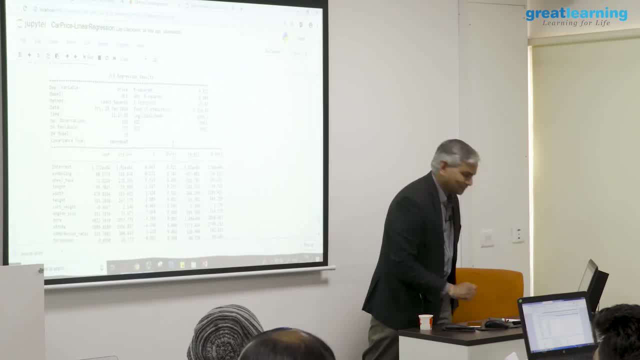 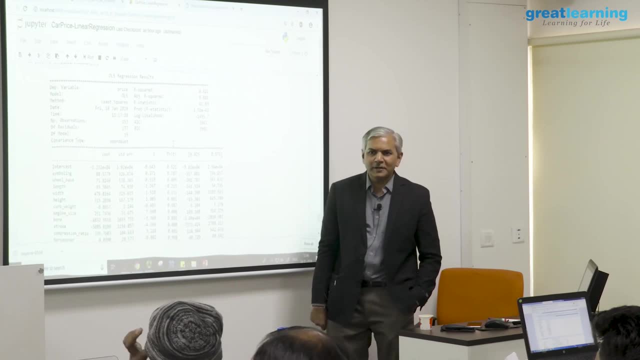 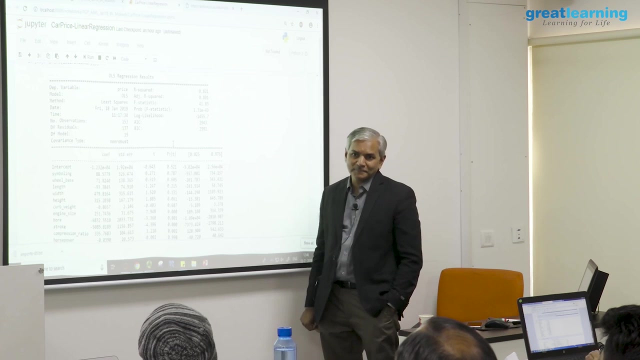 but here we are getting some extra results which we did not get in scikit-learn. Do some of these things look familiar to you? R square, adjusted R square. look at the difference between R square and adjusted R square. Adjusted R square will always go down when you add useless columns. R square will. 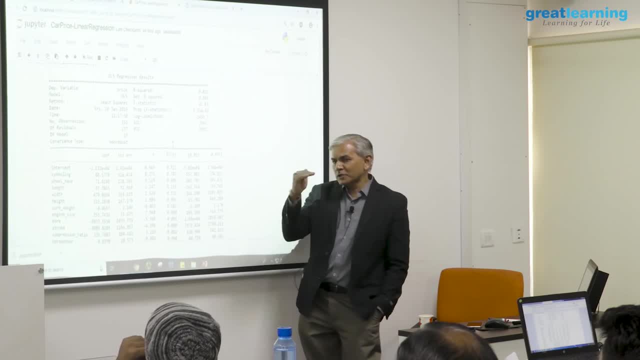 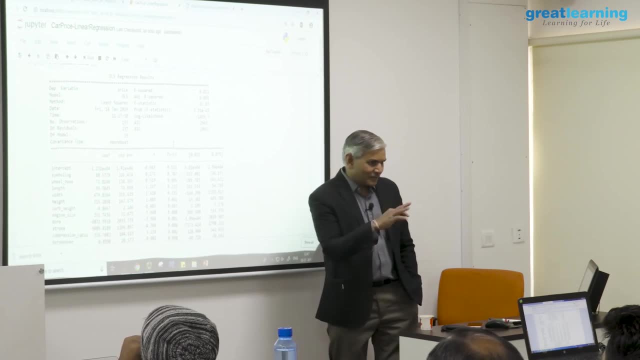 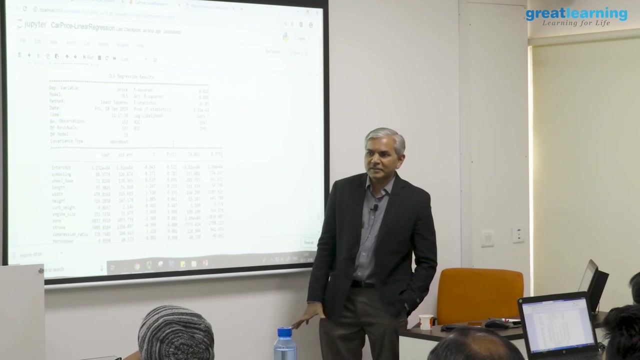 always go up, So adjusted R square will usually be less than R square. F statistics, analysis of variance. remember these words: Fisher statistics, analysis of variance. Then we will also have AIC, BIC. What is AIC, AIC? 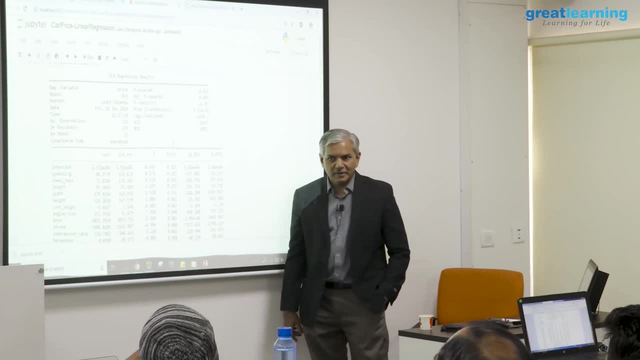 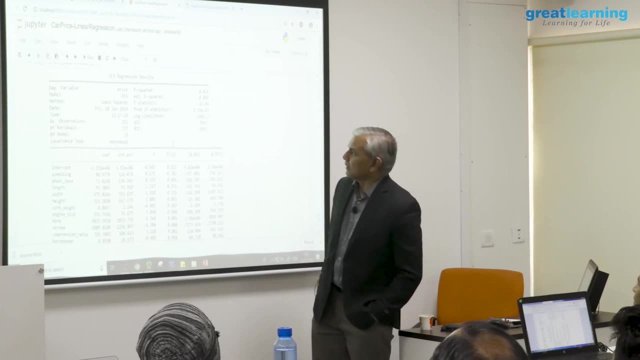 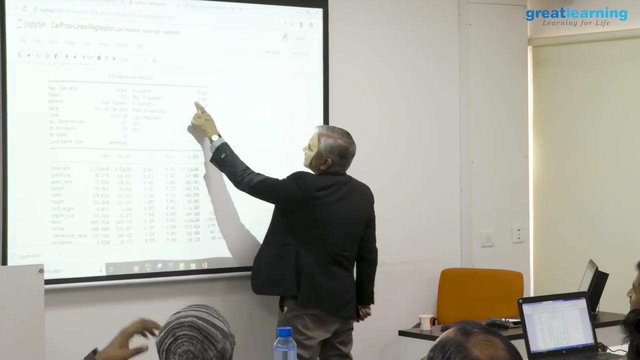 Hey Guru, we have. we would have covered in stats. AIC is Akaike Information Content, BIC is Bayesian Information Content. alright, forget it. no problem, not required. Let us go straight down. Most important of these is your adjusted R square. Adjusted R square. 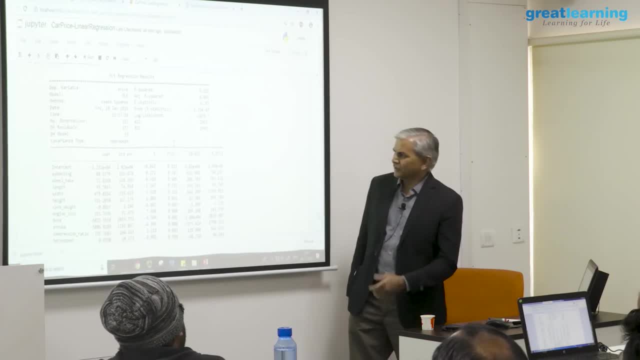 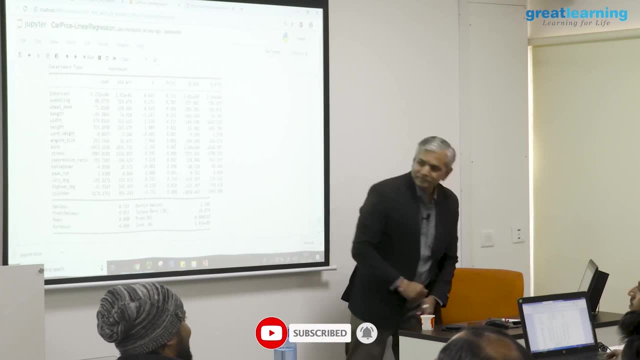 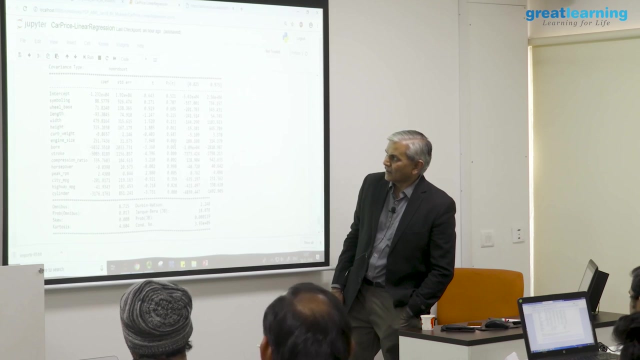 is lower than R square 80 percent. Is it okay with you? You have to. you have to decide. But before I go there, I will come down to this. Okay, I am going to stop at this point. What is this table telling you? I will just take one example, and you have to use that. 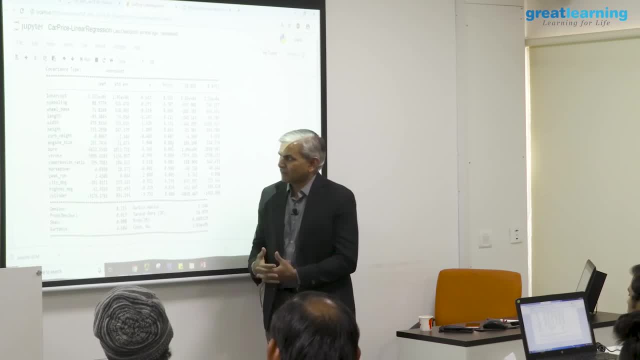 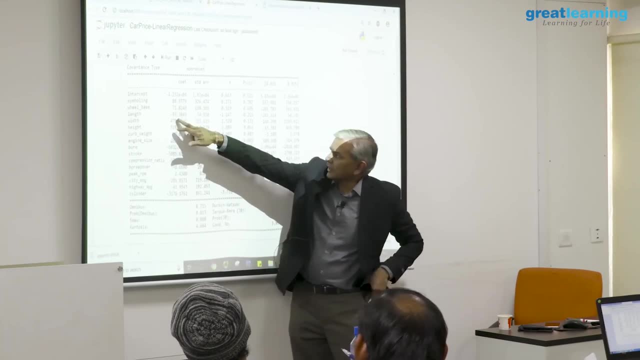 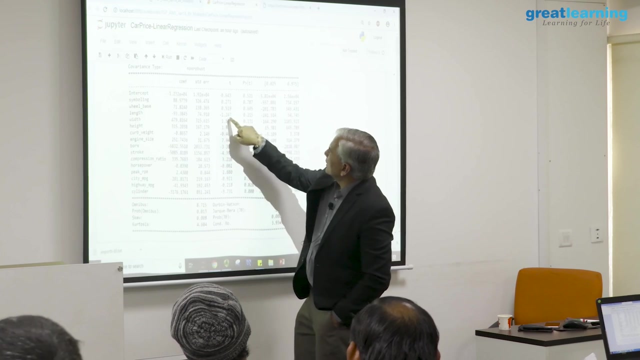 example on others. okay, Then I will tell you why this is not there in Python. Now you take any any one of these dimensions, say length. The coefficient for length is minus 93.3.. We have already seen that. And then it gives you standard error t values, probability. 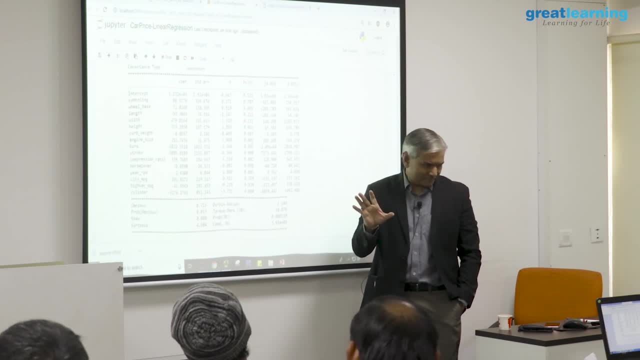 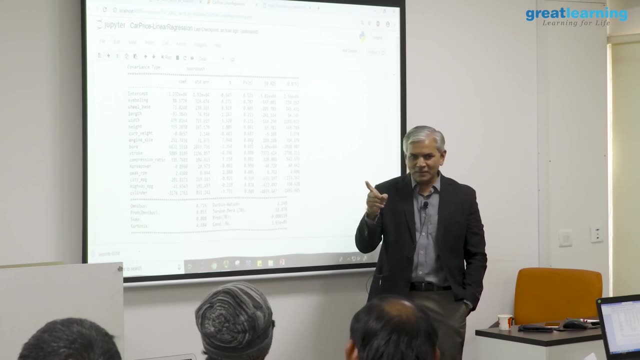 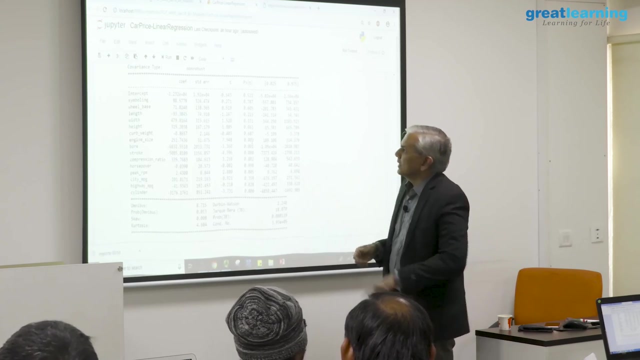 values. Remember your hypothesis testing. When do you reject null hypothesis? When do you accept null hypothesis? You remember those concepts. Remember we use a p value there, right, p values. That is what is this? okay, Now the thing is, let us take one of these. 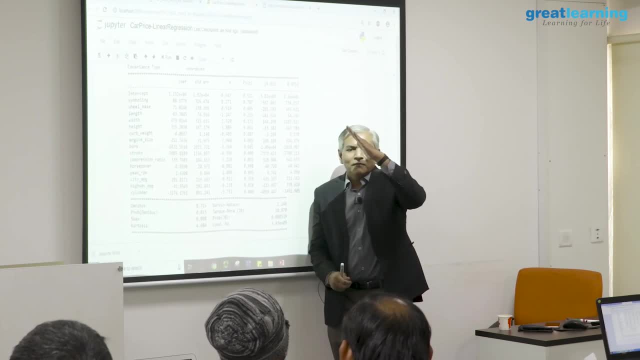 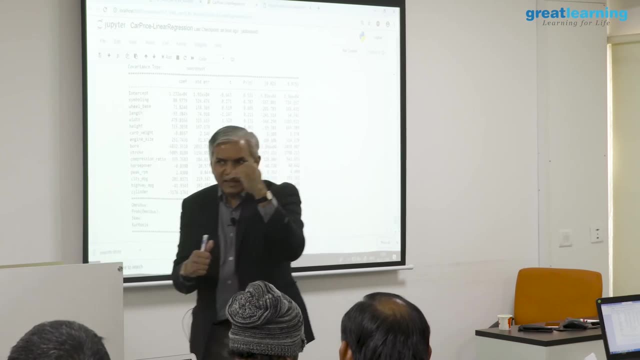 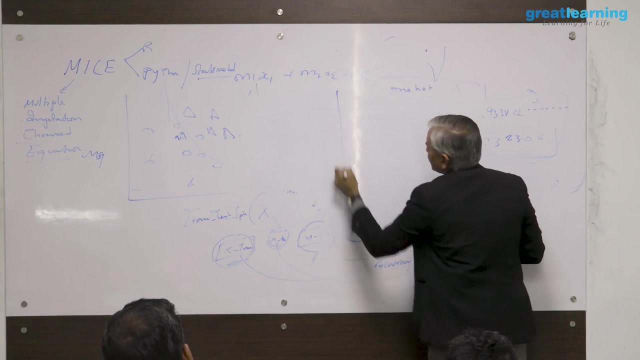 example, length. I told you to find the best fit line. the algorithm will try out various lines, okay, And you will find out the errors for each line for you using gradient descent. And I also told you that the best fit line that it finds out will always go through the x. 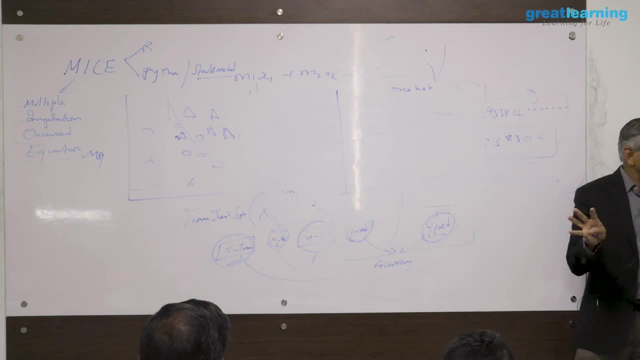 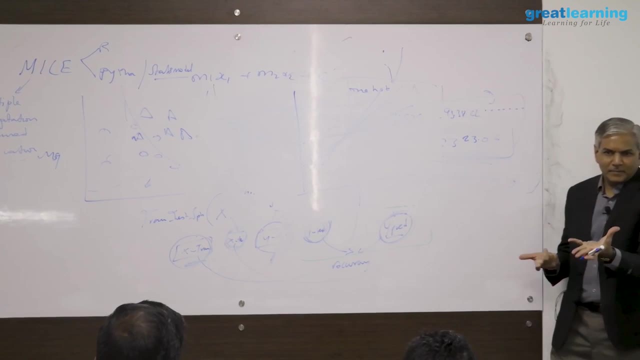 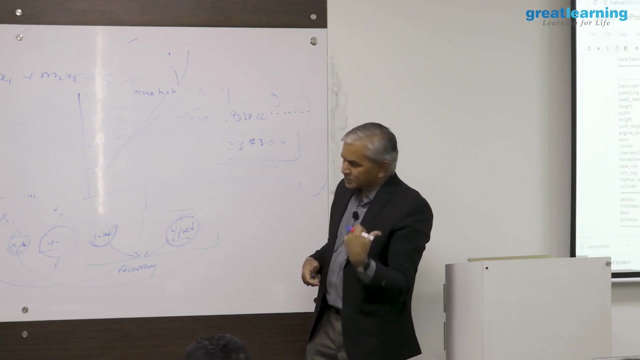 bar y bar Agree. So it would have tried out various lines for you before finding the best fit line. So for each line on this particular dimension length, you can take any dimension. or for each line on this particular dimension called length, you would have had different slopes. 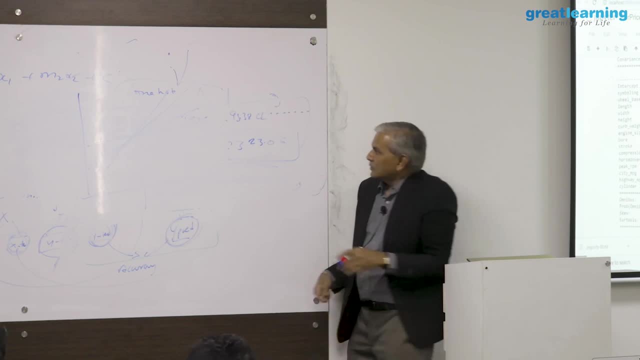 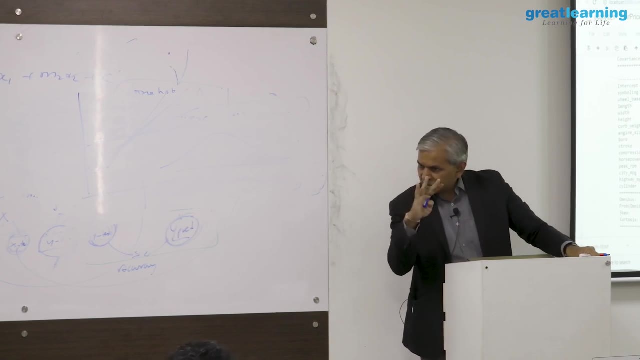 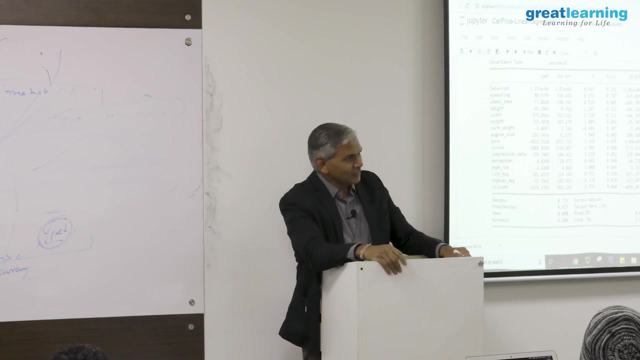 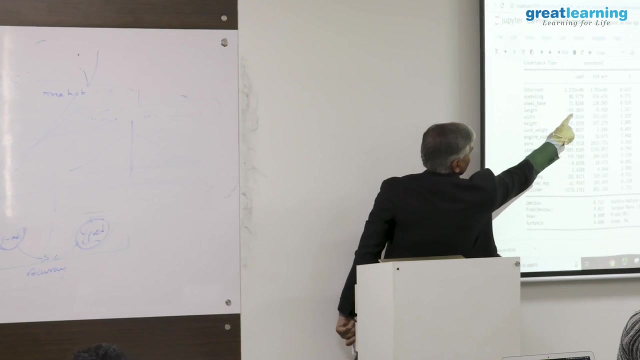 each line would have had different slopes, different coefficients, So those coefficients would have distribution of their own. those different coefficients which it tried out on the length dimension before it found the best fit line, those coefficients would have had different distributions Of that distribution, the one given to you for best fit line, minus. 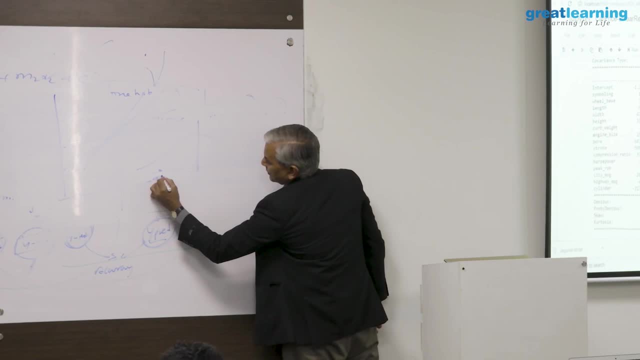 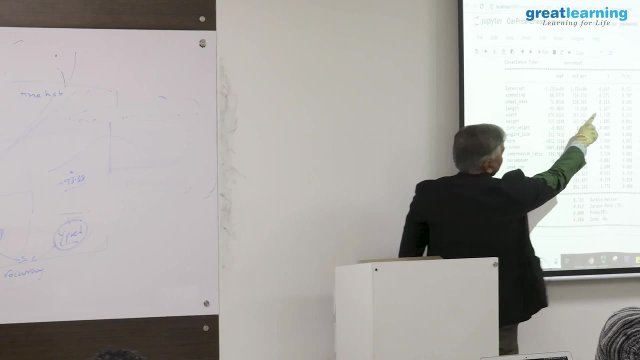 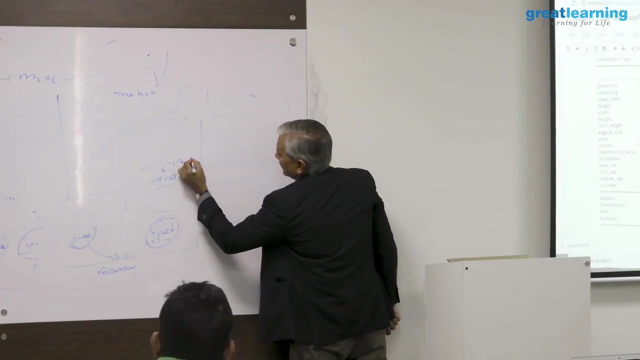 93.38,. may be this one minus 93.38,. how far away it is from the central value is given by your t score. This is minus 1.2,. whatever it is t scores, What is t score? T score? 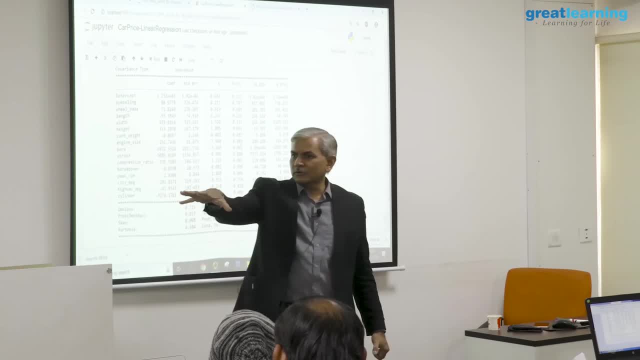 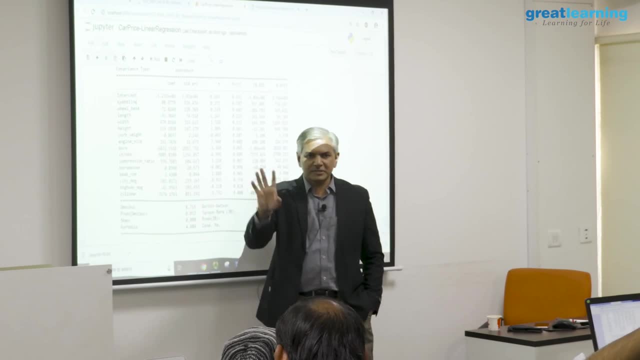 is a z score. All of you remember z scores: x, i minus x bar by standard deviation: How many standard deviations away a data point is from the central value? We use z score for that. When you use student's t distribution, we call it t scores. Formula is same, Remember. 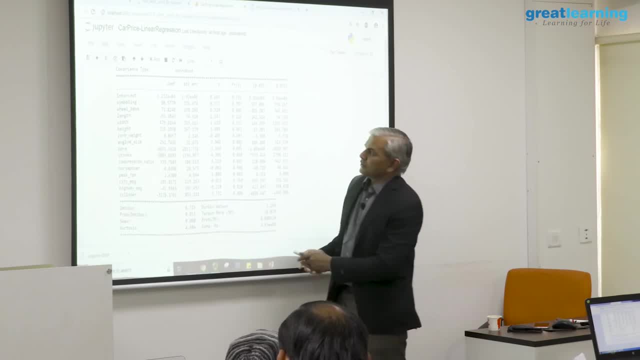 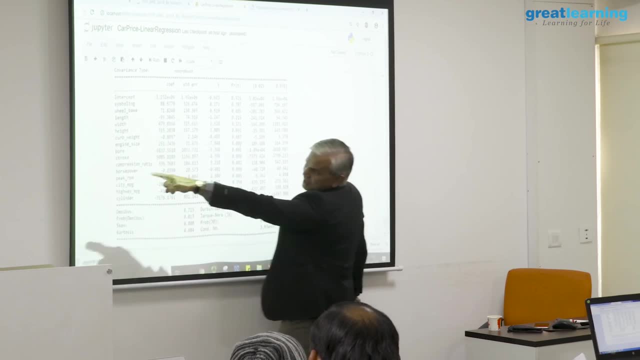 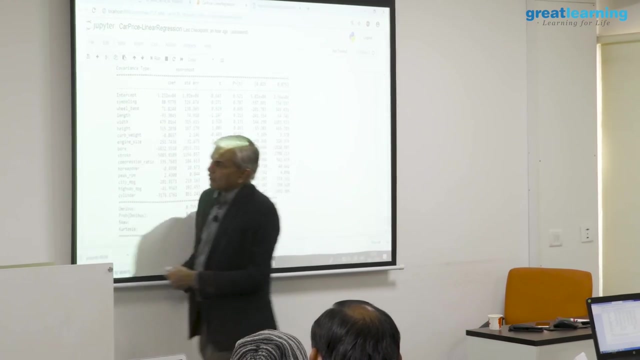 student's t distribution. Ok, The formula is same. So the selected value for coefficient for length, how many standard deviations away it is from the central value for the distribution of coefficients on length That is given by this, The standard deviation of this distribution? 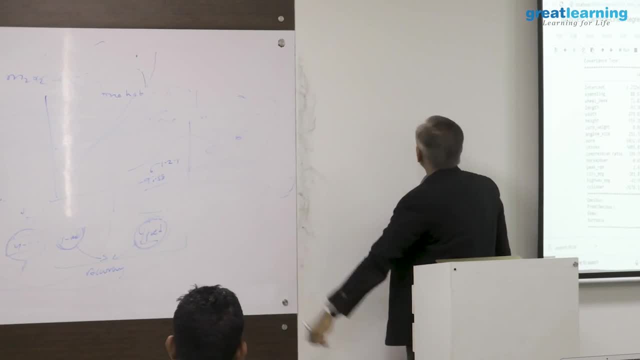 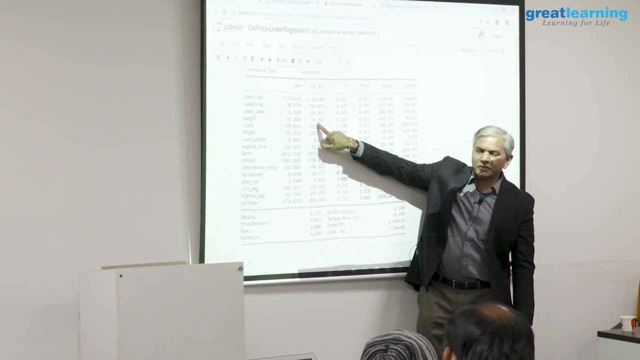 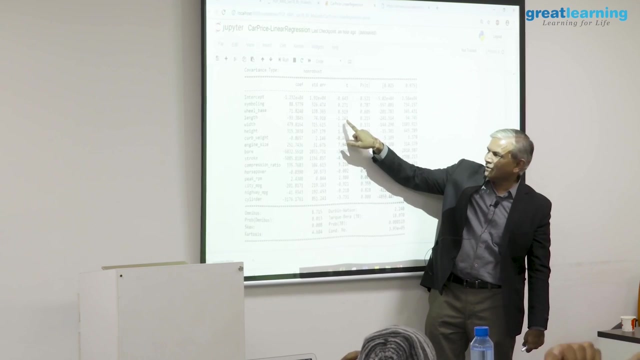 the standard deviation of this, which we call standard error in t distribution that is given by this. This is the standard deviation. This is how many z scores away it is. your selected value is from the central value is this: You multiply these two, Multiply these. 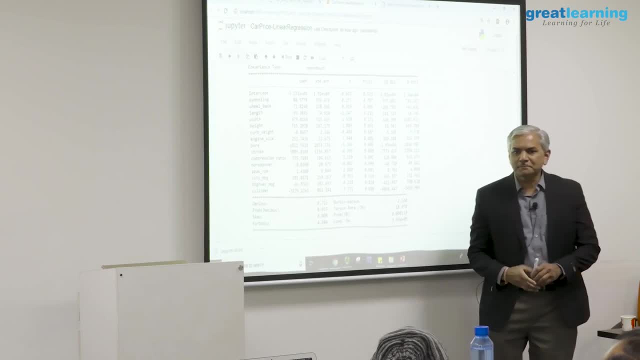 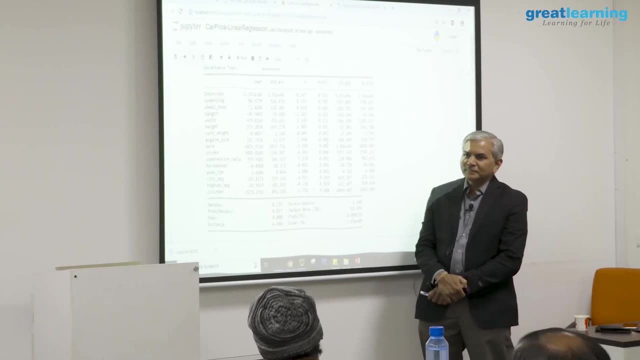 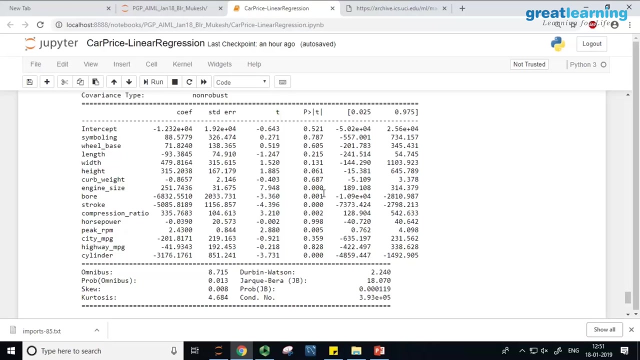 two. please Multiply these two and tell me what is the value you get Into minus 1.24.. 73. You will get back the same value. You will get back this value. Ok, Look at this. If I am doing, 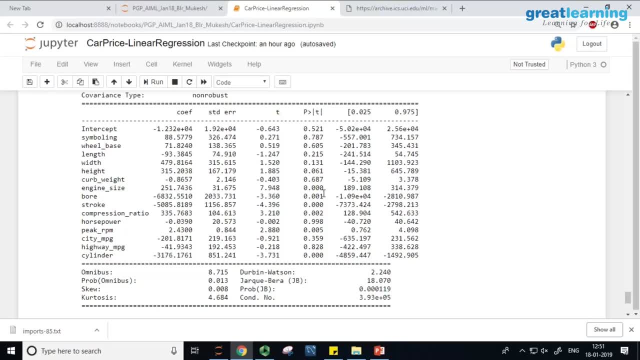 z score. z score centralizes your data, converts the x bar in y bar into zeros. I take any value: xi. xi minus x bar by standard deviation is my z score Agreed. x bar is 0 because it centers the data. So that means z score is nothing but xi by standard deviation. So 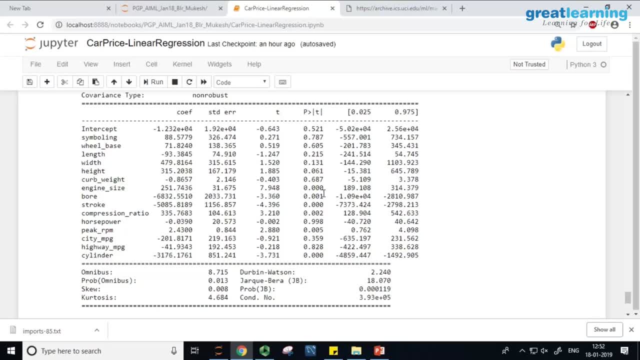 xi is nothing but this. And then we are given underенноеu t that Gran mamy we called zone. Then we get the. that means actually we are getting z operation Which is from t. That z score into standard deviation, Here we call it t and we call this standard error. So when 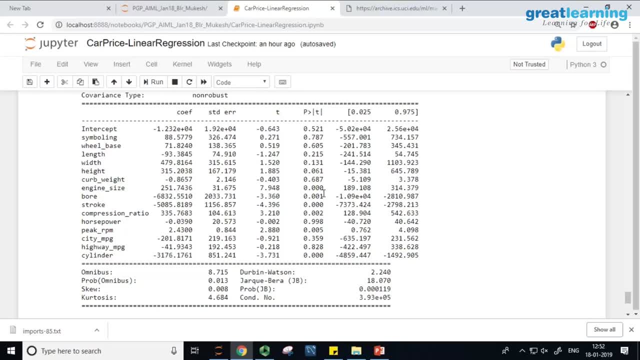 I multiply t with standard error, it gives me back the value that you had over here: xi. It gives me back the xi. So that is the way to interpret this. Of all the various coefficients tried out on this length dimension, we select you this one. How far away it is from the 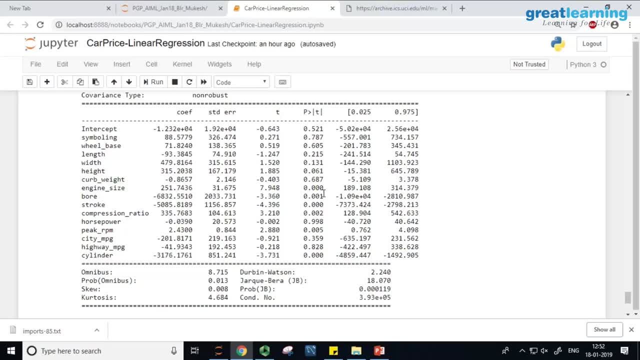 central value. If it is too far, maybe it is not reliable. I will do that analysis using this. The most important analysis which I want to take you to is the p-value. What does this p-value tell you? What the p-value is telling you is- I am going to talk only for 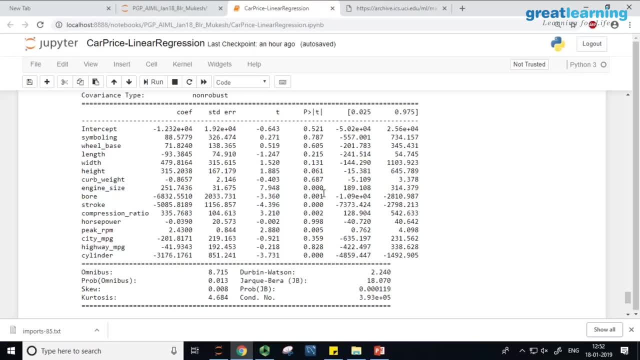 length, but the same thing applies for all. What this p-value is telling you is: probability is 0.2.. What is the cut-off probability for your confidence level? 94 percent, 0.05,. 5 percent: 0.2 is much higher than 0.05.. What this is telling you is: even if 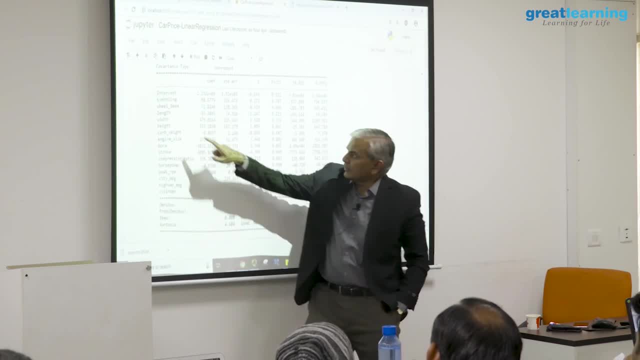 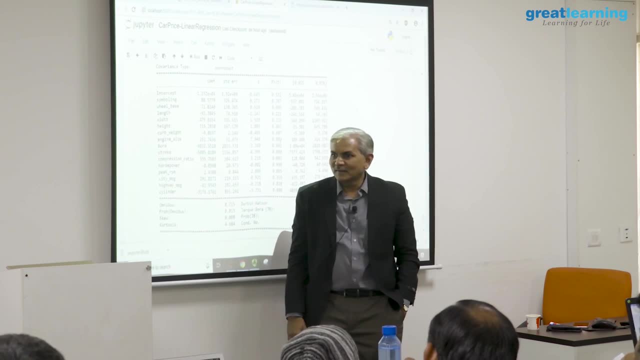 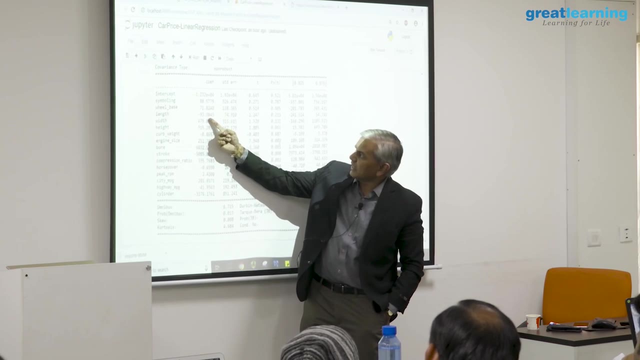 in the population there is no relationship between the length and the price of the car. no relationship between length and price of the car- null hypothesis- and you have taken data from that population. you are likely to find this kind of a relationship between length and price in your data. 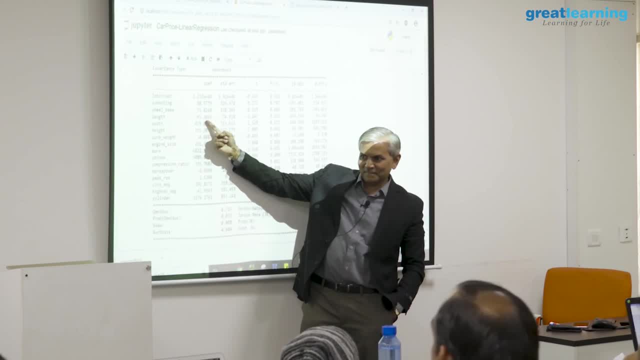 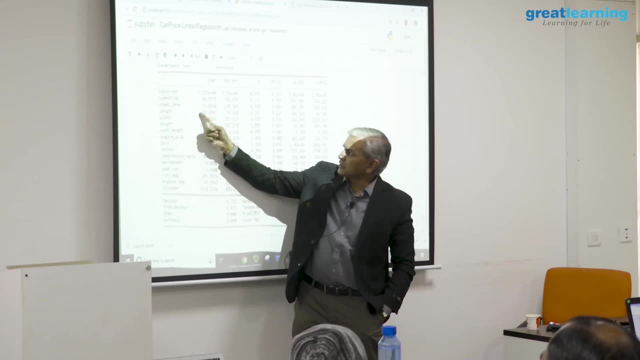 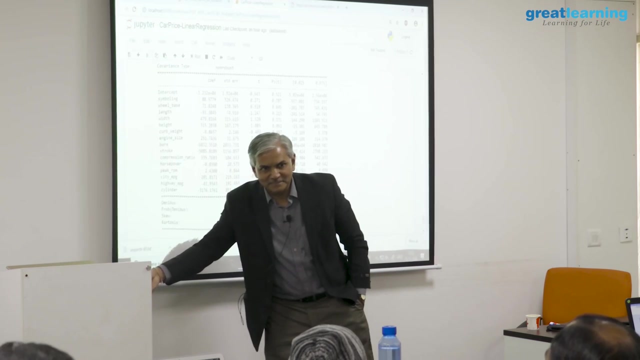 Which means this is a fluke relation. I repeat: what this p-value is telling me is probability of finding this kind of a relationship between length and price in your data, even if there is no relationship in the population. In population, the slope is 0 between these two And from. 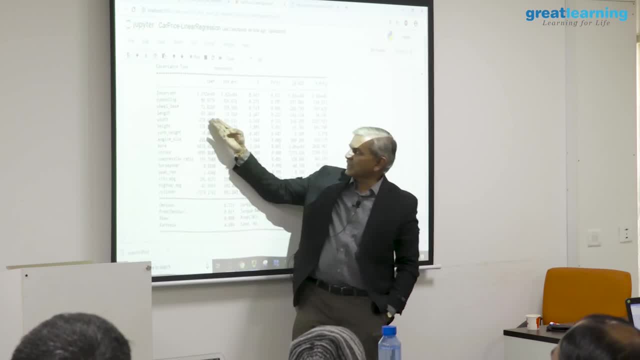 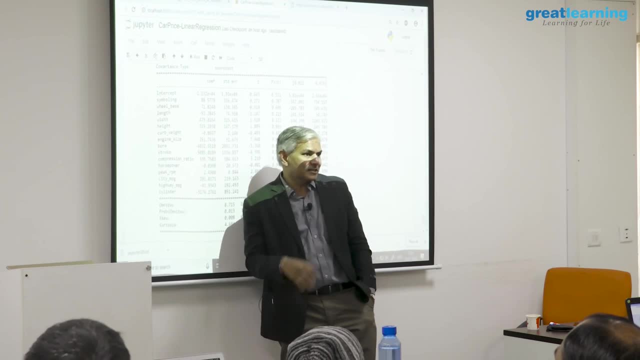 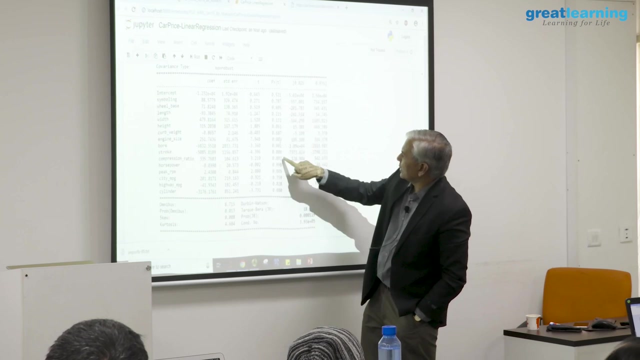 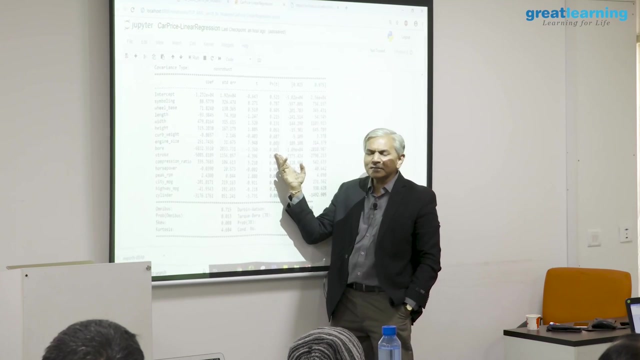 there you have taken a sample, random sample. The probability of finding this kind of relationship is very high, Which means This relationship is fluke. It is a statistical fluke. It is not reliable. Look at this one p-value. Look at this one stroke p-value is almost 0.. What it means is if, in the real 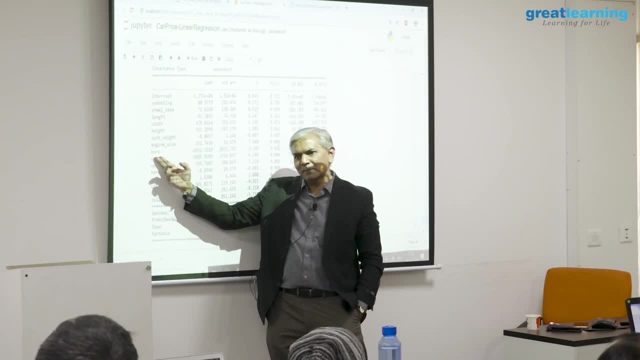 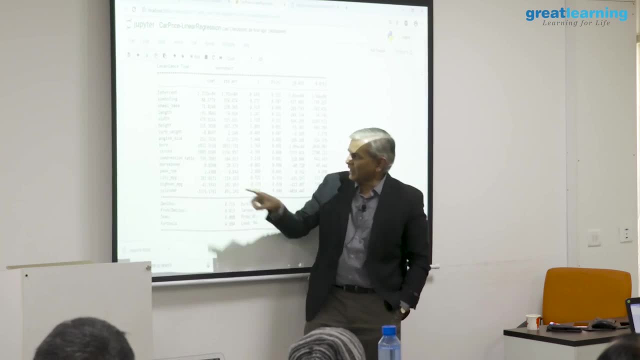 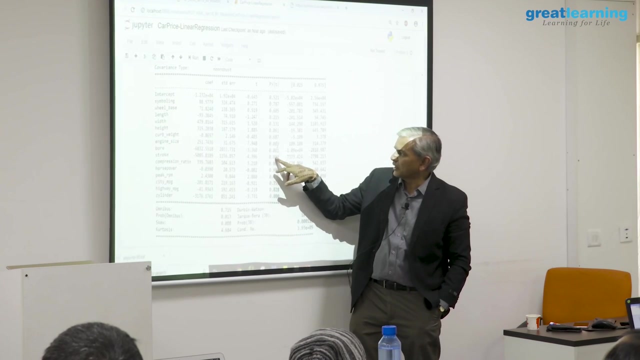 world there is no relationship in bore and the price and then from that population you have taken this sample, Finding this kind of a relationship between bore and price. the probability is very low. Probability is very low. I am talking stroke, sorry. Probability is very low, Which means 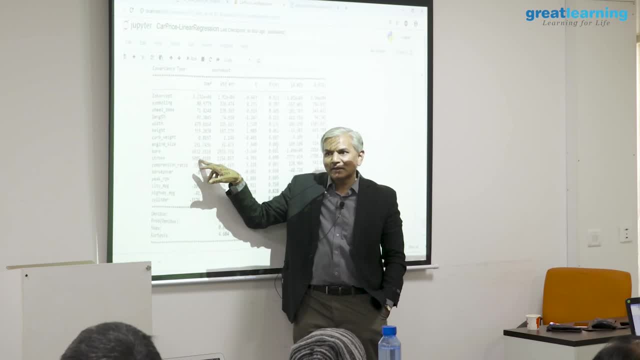 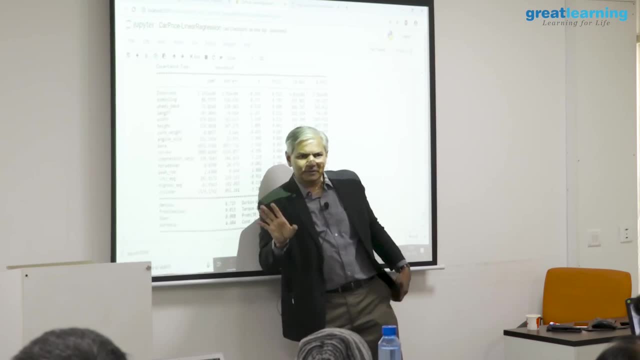 this relationship is not fluke. It is likely to be there in the real world. So let me put this pictorially and explain this to you. Then we will wind up. Let us take one of these columns- stroke and price- Same thing applies to all- And then let us see where it is going to be, And then let us see where it is going to be, And then let us see where it is going to be. So let us see where it is going to be And then let us see where it is going to be. So 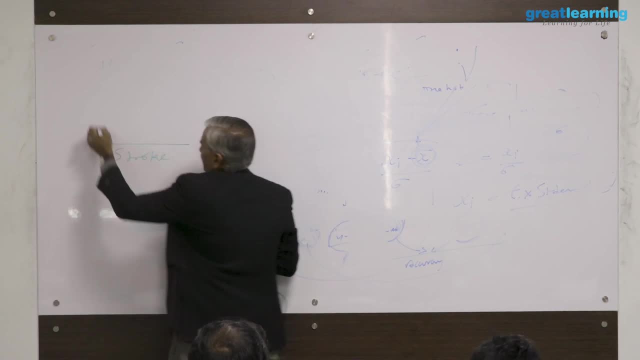 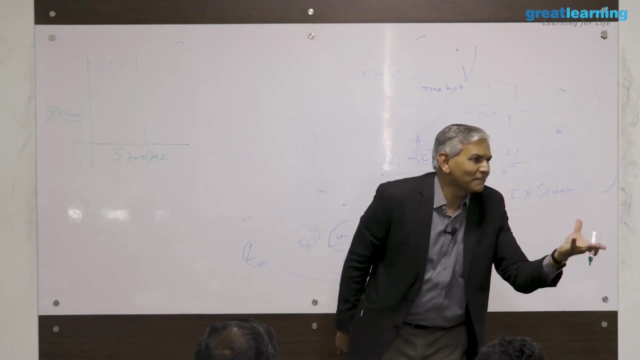 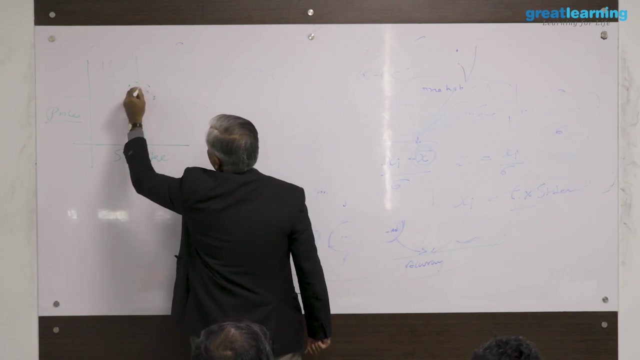 If suppose, between stroke and price price, if suppose there is no relationship between these two, then how will the scatter of the data points look? Agreed, All of you. R value will be very close to 0.. The scatter of the data points will be circular. 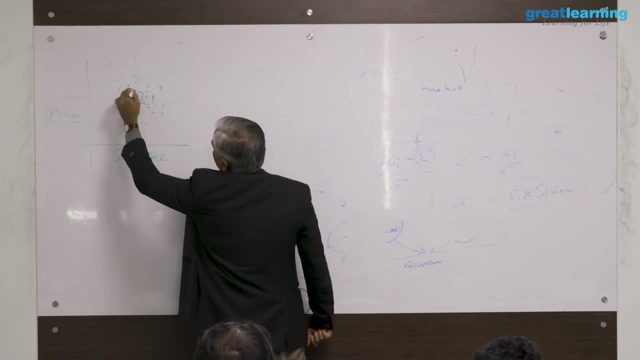 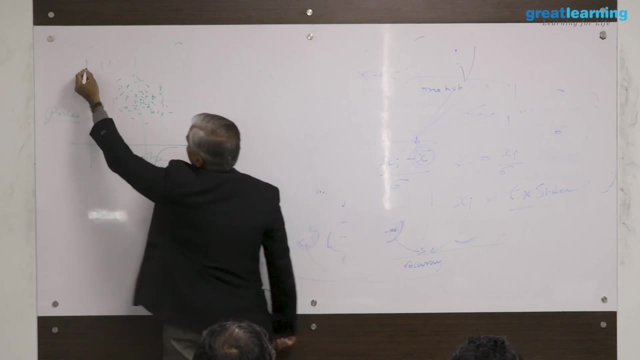 Okay. Now what you will observe is most of the data points are near x bar, y bar. As you move away, the density falls. That is why you get a plot like this on this and a plot like this on this. Are you all okay? 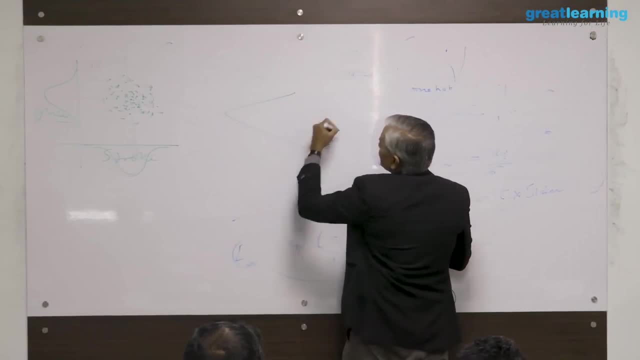 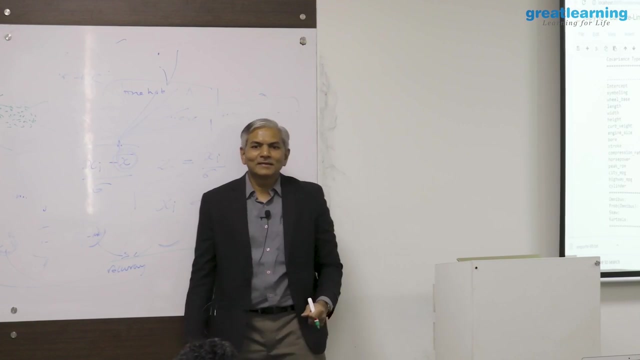 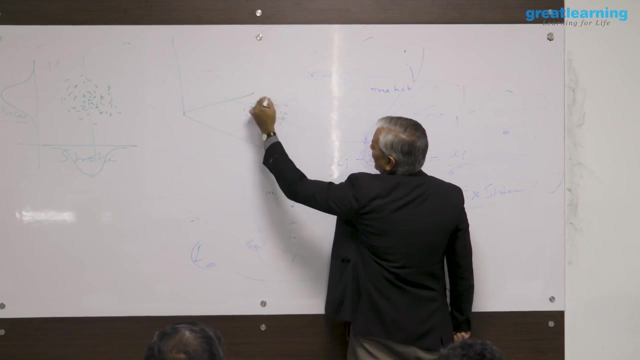 When I convert this into 3 dimension, where in the 3rd dimension this is my x bar, y bar. If I plot the density on the y axis, question to you is: how will the distribution look? Parallel Cylinder, Keep in mind: very close. it's very high. As you move away, the density falls. 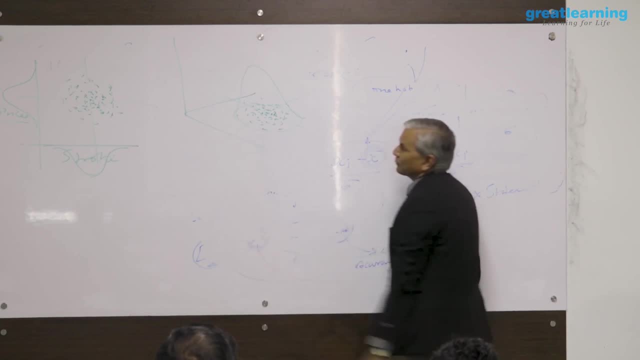 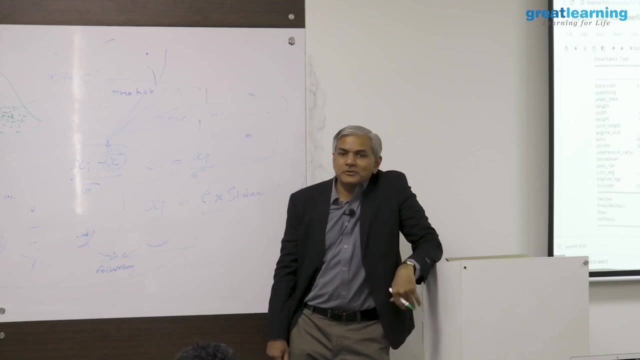 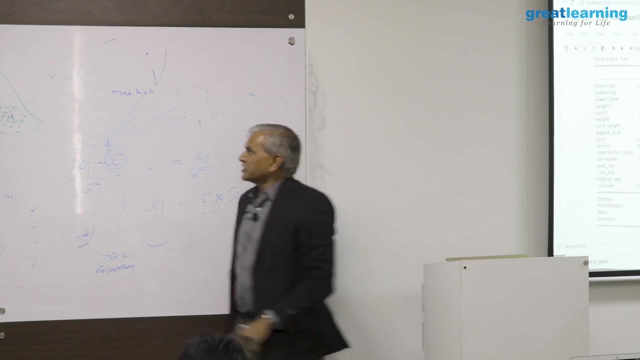 So this will be your normal curve: A 3 dimensional normal curve. A 3 dimensional normal curve is a shape of the density of distribution between two dimensions which don't correlate. This is the shape of null hypothesis. Null hypothesis is in your universe. the data is distributed like this: 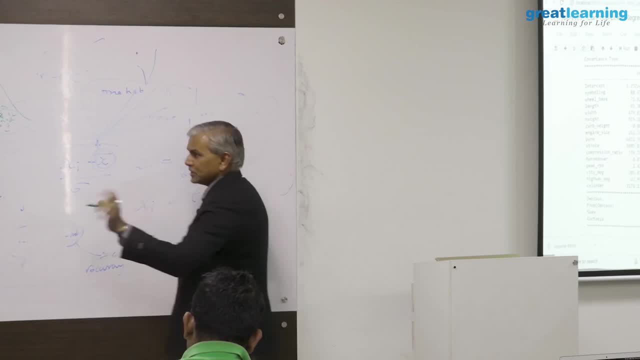 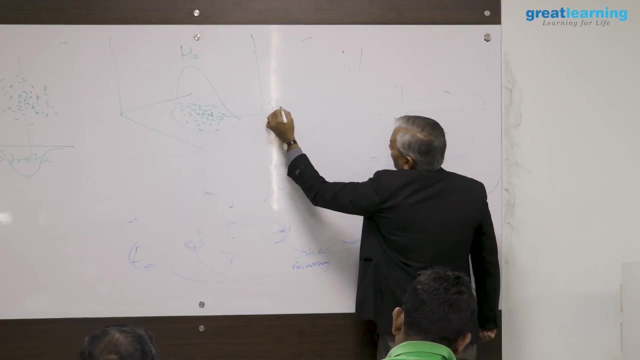 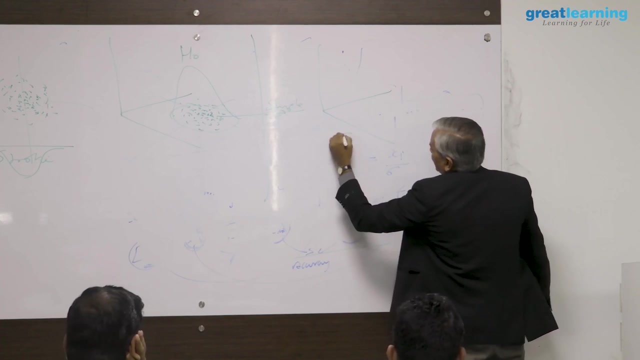 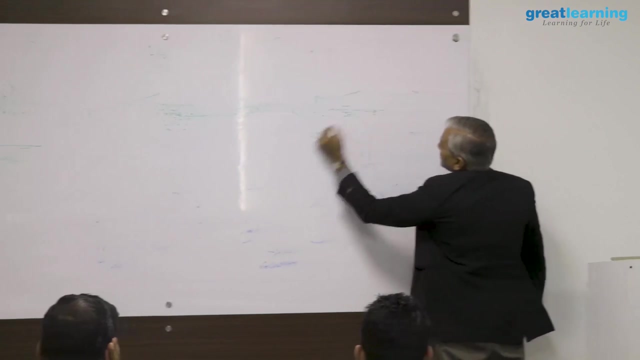 Agree, We don't know what the universe looks like, but null hypothesis is it looks like this. If so, and from there I have taken a sample, and in the sample I am finding the distribution between this core, whatever it is, say core and price. I am finding the distribution like this, where this is: x bar, y bar. 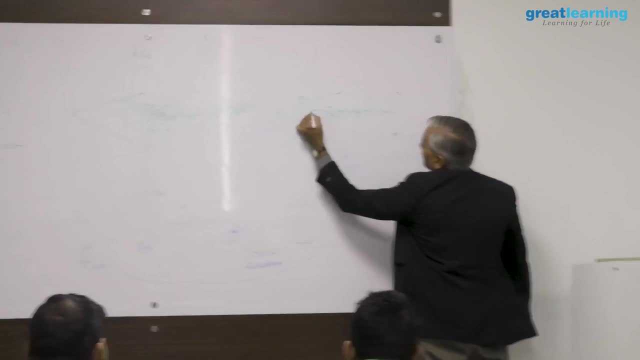 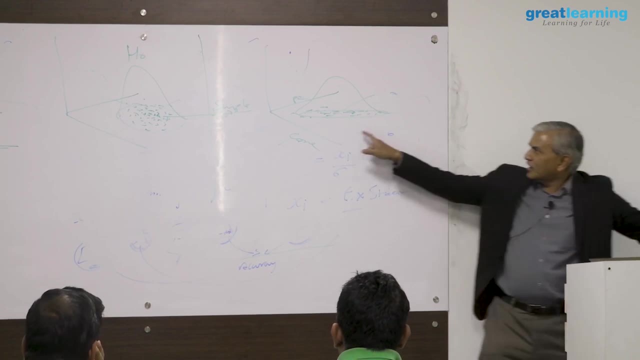 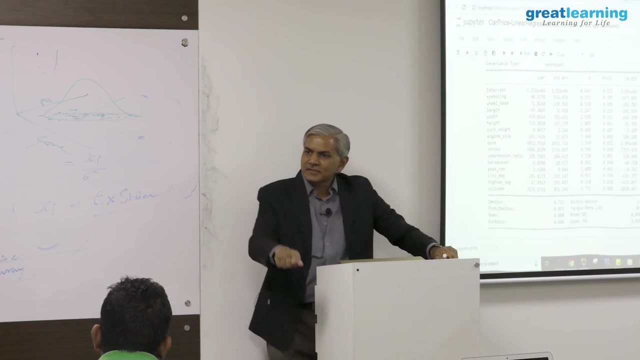 I am finding a squashed bell curve. I am not finding a symmetry bell curve, I am finding a squashed bell curve. This relationship is what is expressed as this coefficient. Now the question is: what is the probability of finding this kind of a distribution in your data if the real data is like this? 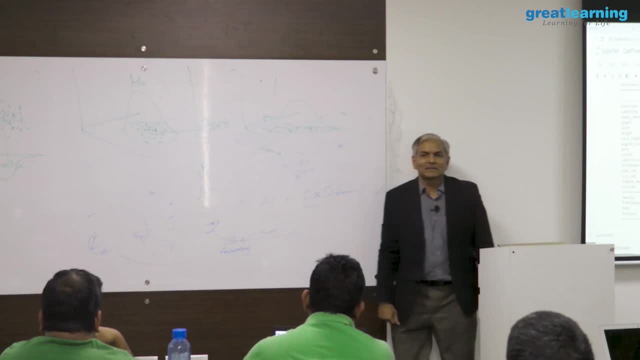 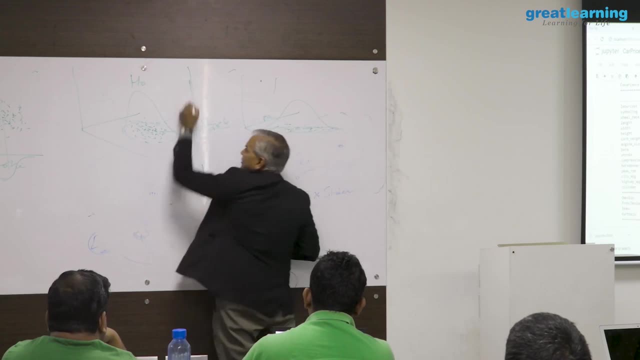 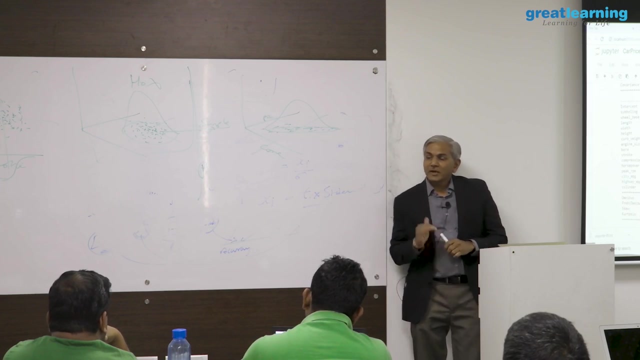 That probability is expressed as p-value. If the p-value is very low, less than 0.05, that means the distribution is very low less than 0.05.. That means your universe is not like this. we reject the null hypothesis. 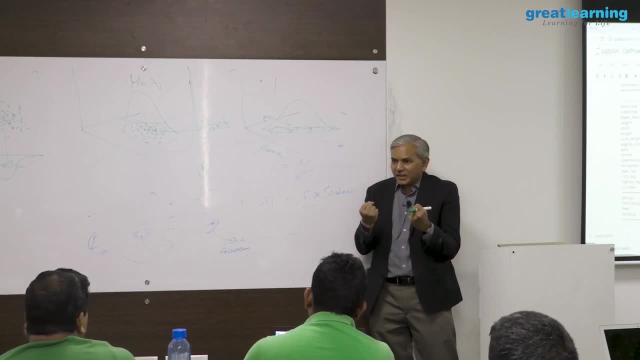 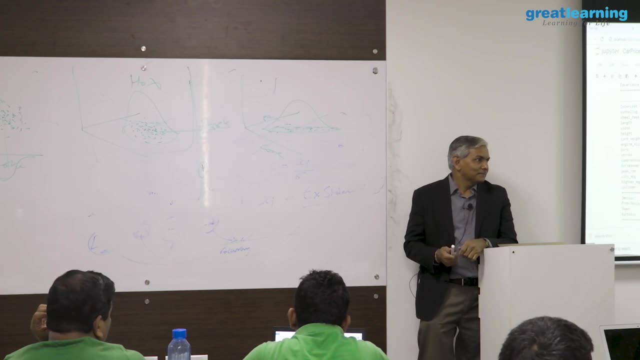 Whereas if p-value is greater than 0.05, we say that there is not sufficient evidence to reject the null hypothesis. So I am unable to reject the null hypothesis. May not be, I don't know, but I don't have sufficient evidence to claim that there is a correlation. 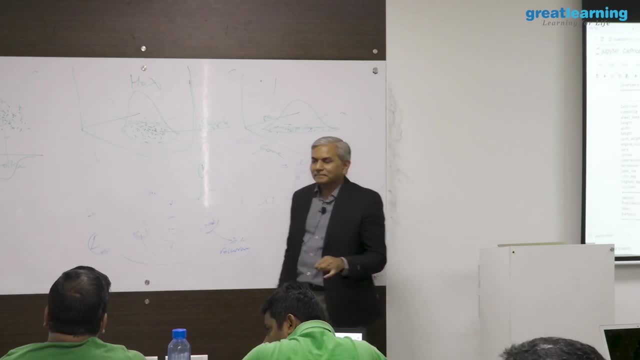 Shouldn't the null hypothesis be? I mean by default? I mean we are trying to prove the other way around. No, we are trying to establish whether null hypothesis is likely to be true or not. We can't do the other way. 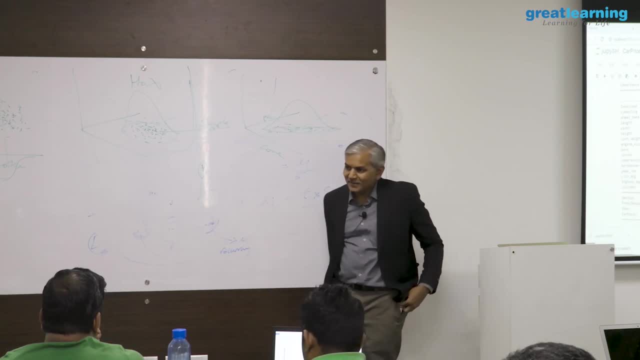 We can't prove alternate hypothesis to be true or not. We can't do that, So shouldn't the null hypothesis be? there is a relationship already and No null hypothesis is no relationship. They are independent. It always negates your alternate. 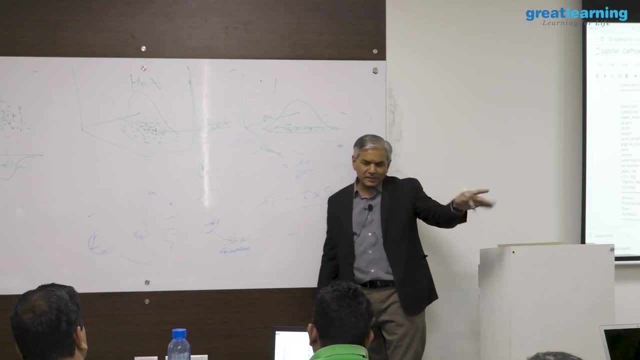 Alternate says: there is a relationship, Null hypothesis, nothing doing. there is no relationship. No relationship means this is the way. Now the question is from this: you have drawn this. The question is from this: you have drawn the sample. In the sample, you are saying this: 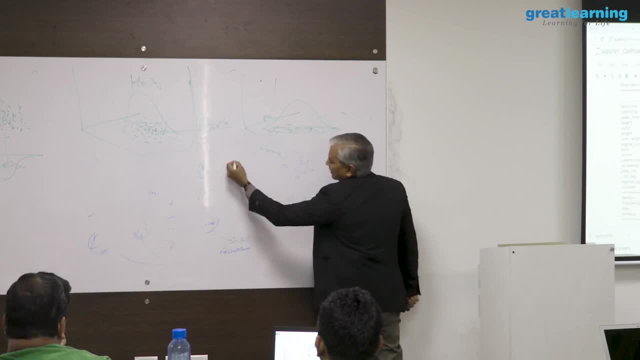 What is the probability of seeing this kind of distribution? if it is coming from this: If the p-value is less than 0.05, we reject the null hypothesis. If p-value is 0.05 or greater than equal to, we say we don't have sufficient evidence to reject the null hypothesis. 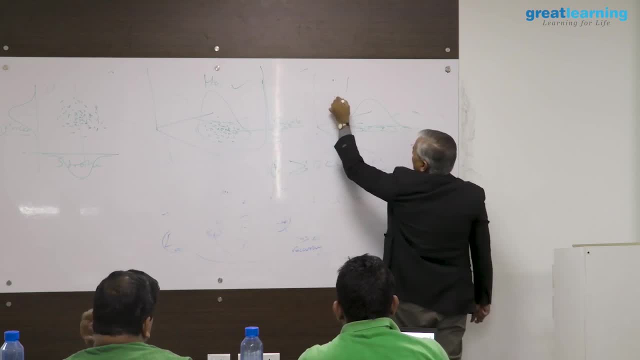 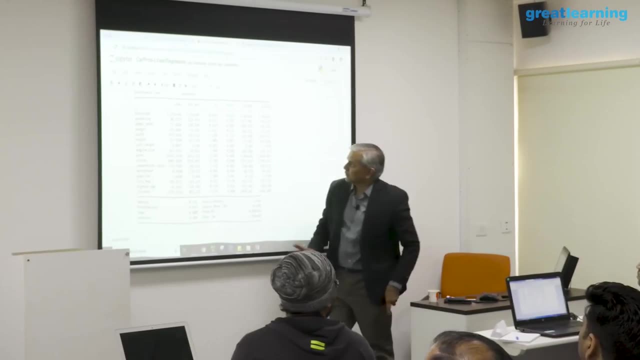 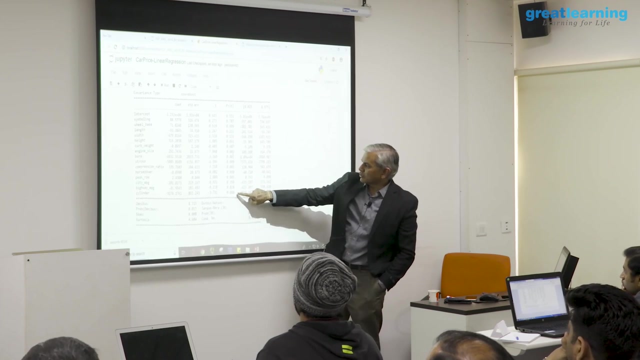 So we accept the null hypothesis likely to be true. we reject this. This analysis R provides, Python doesn't. And if you look at this, this is the p-values. So this tells you the importance of the attributes. Those attributes whose p-values is greater than 0.05, useless. 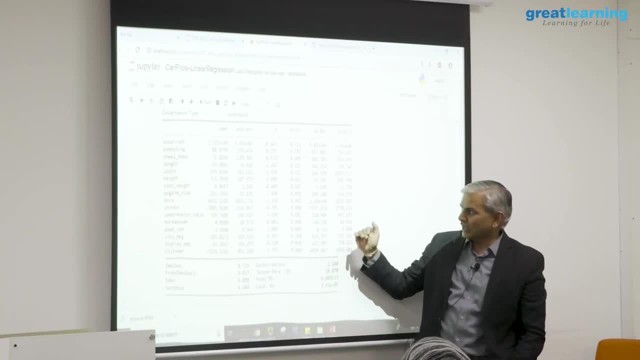 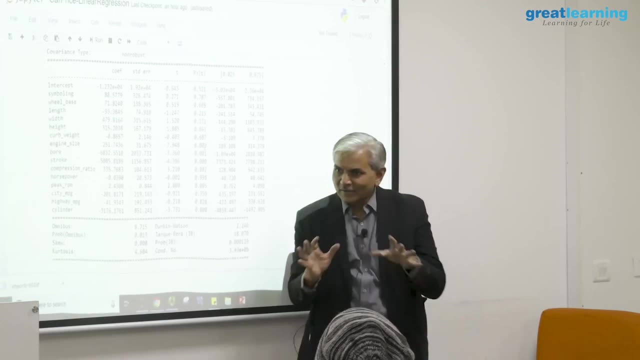 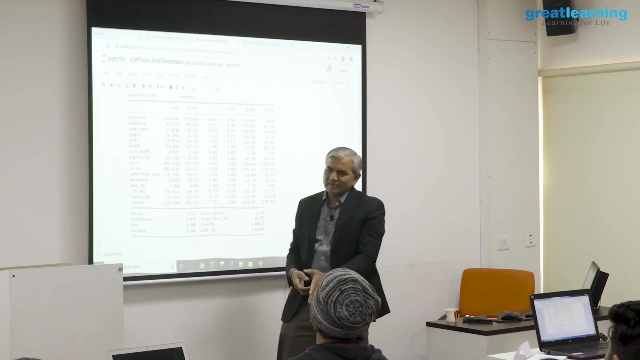 Statistical fluke. Those attributes where p-values is less than 0.05, good attributes. Let me be a killjoy In the statistics community. in the real world there is a vertical split between the statisticians. One school of thought says p-values is not reliable. 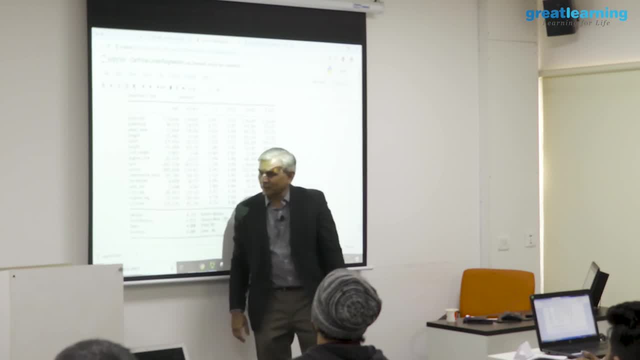 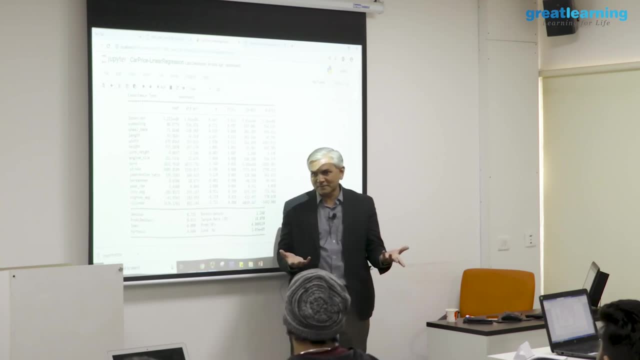 The other school of thought, which comes from the conventional statistics point of view. they say p-values is reliable. The reason why they say p-values is not reliable is you can go and check it yourselves. Suppose I drop one of these dimensions with high p-value symboling. 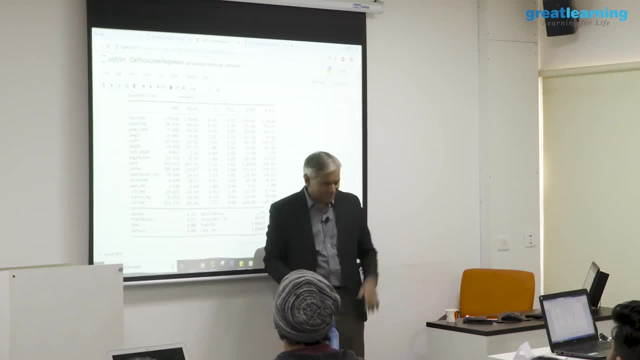 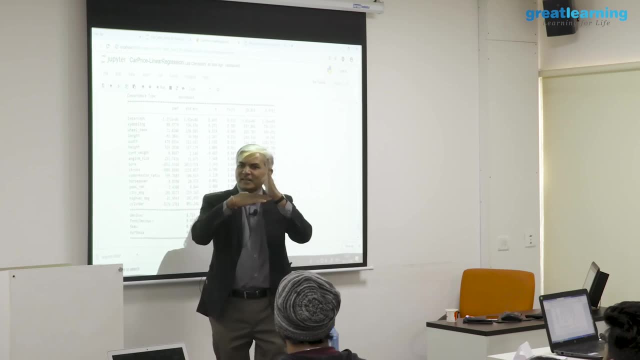 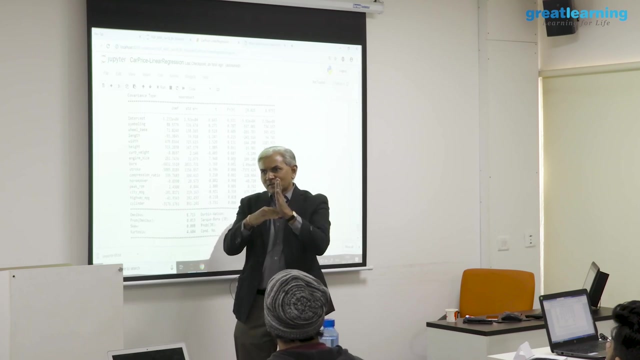 And redo this analysis, All the other p-values will change. Now the question is: between your price and your length. if there is a relationship given by the coefficient, why should that coefficient change when I include another dimension, the width, Why should it change? 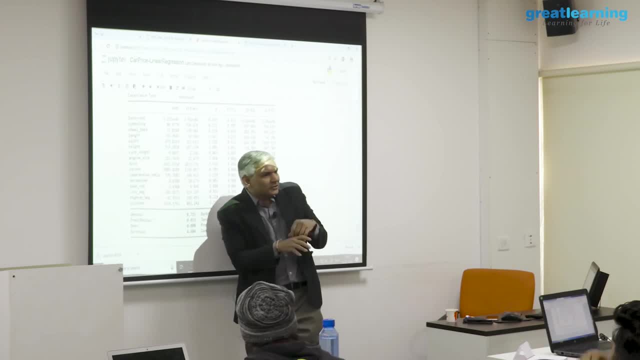 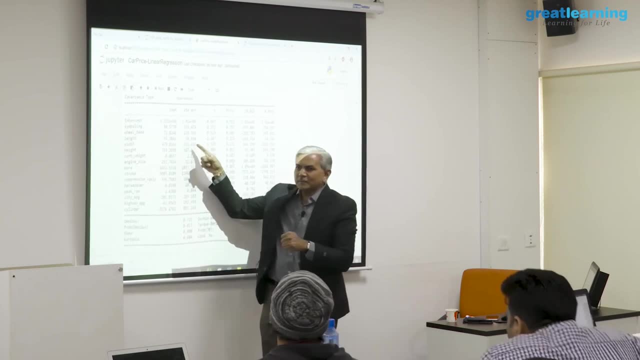 It should not change right. The relationship should remain relationship. Why should the intensity of the relationship change when I add another dimension to it? But when you actually go and analyze this, drop the dimensions. you see that all coefficients change. Correspondingly, all the p-values change. The values will also change. The reason why they change is collinearity. They are not truly independent. Since there is collinearity and they impact each other, the coefficients are not reliable. Hence the p-values are not reliable. It is because of this reason this split between the statistics community on whether they should rely on this or not. 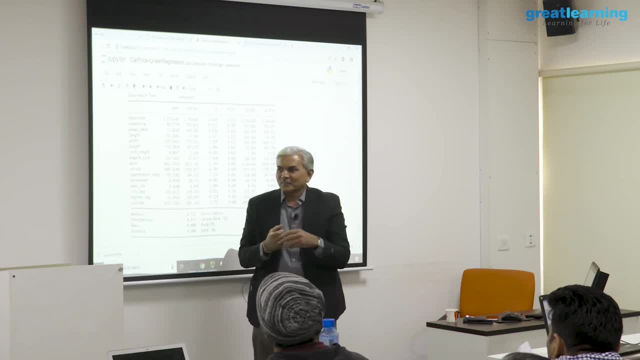 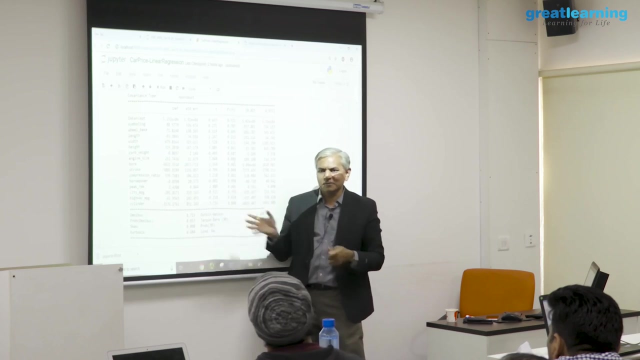 scikit-learn guys said: forget it, we don't need this, We have other ways of establishing the reliability of the dimensions and the models. Let's use that. That is why scikit-learn does not give you this facility, But then subsequently, under pressure, they came out with stats model libraries, which gives you this. 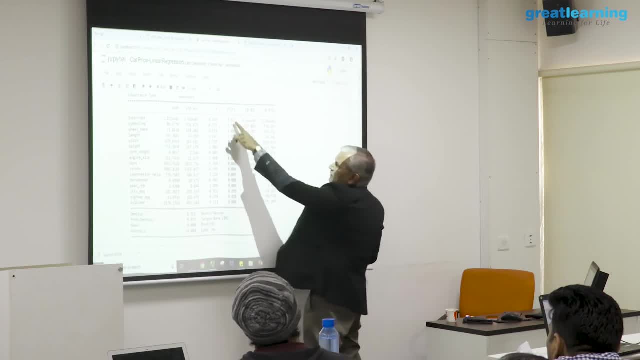 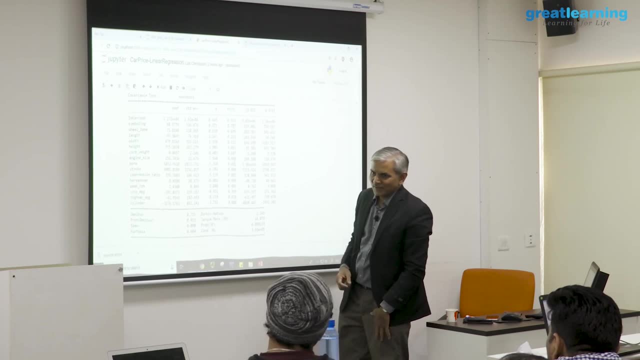 Now, just to end up the show, what it is telling you is p-value and what it is telling you is the 95% confidence within which these values lie. So if you guys remember, 95% confidence level. area of rejection. area of. 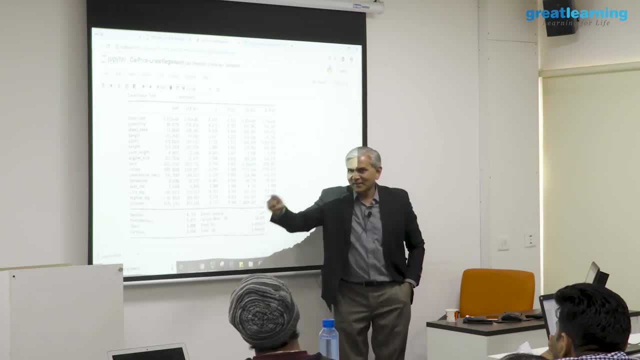 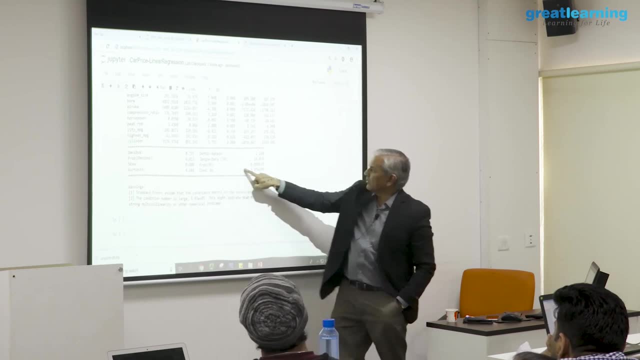 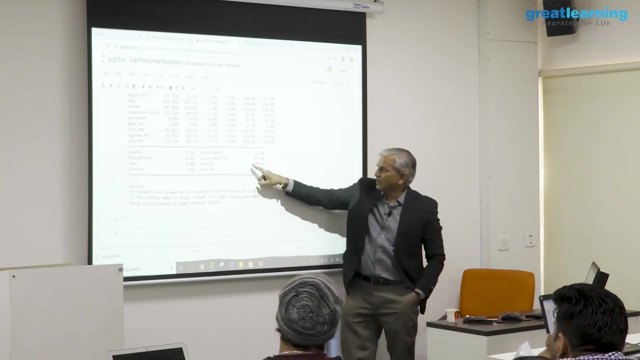 You will see all. You will be able to connect to those using this. I am going to jump this, I am going to move forward. Last one: Overall probability value of the model itself. Can such a relationship between the price and the other good attributes? 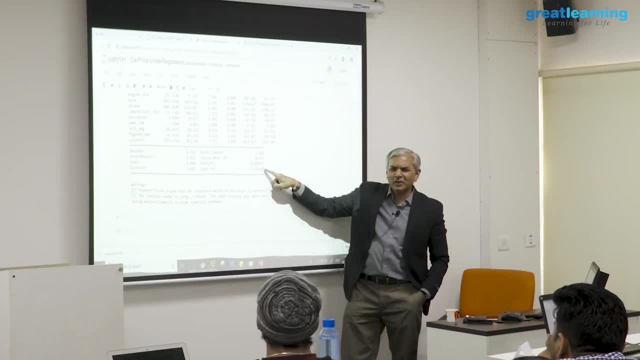 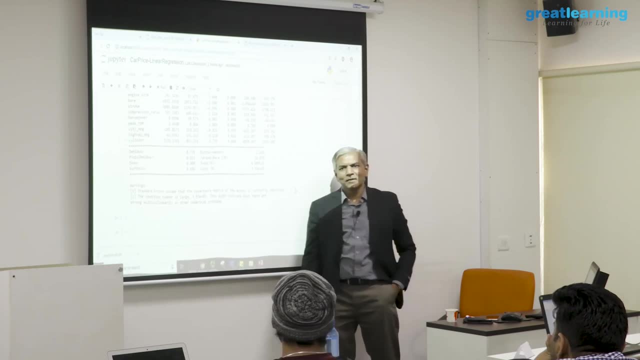 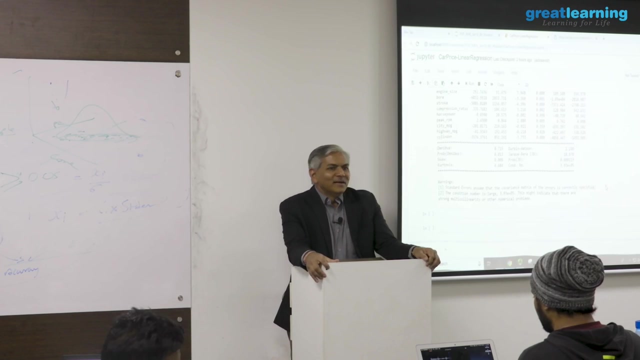 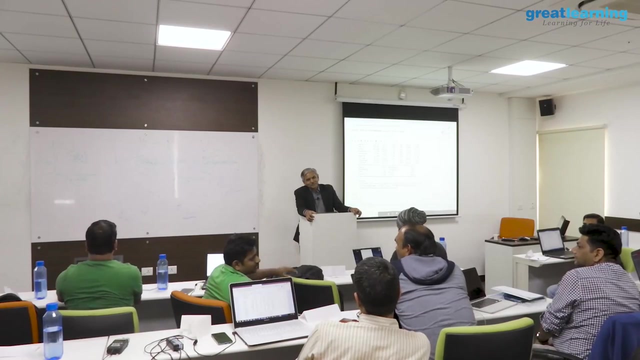 Does such a relationship exist? P-value is very low, which means null hypothesis overall is rejected. Model level p-value is very low. So, after removing all the unnecessary things, all the unwanted dimensions, hopefully you will have a reliable model If you are working for people who believe in statistics and 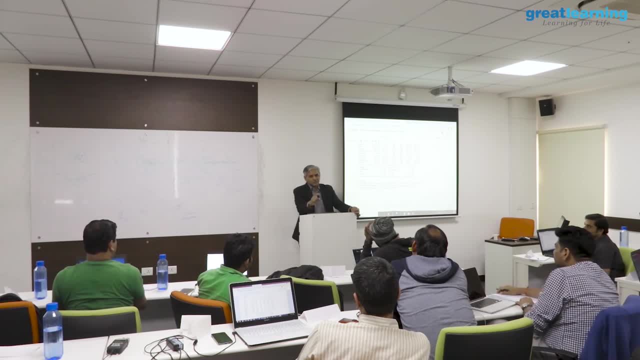 I mean not that I do not believe in statistics. Those people expect p-values from you, Then you have to use stats model. If they do not care about p-values, do not come here. There are other ways of deciding whether a dimension is reliable or not. 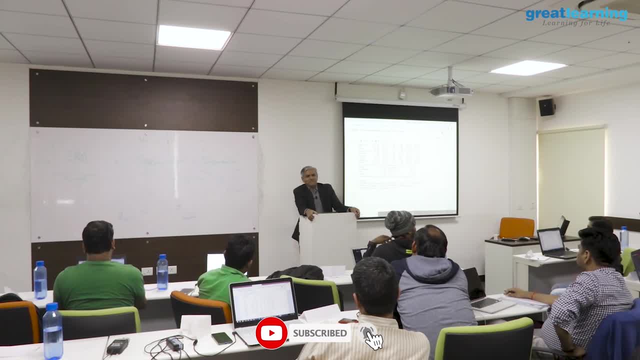 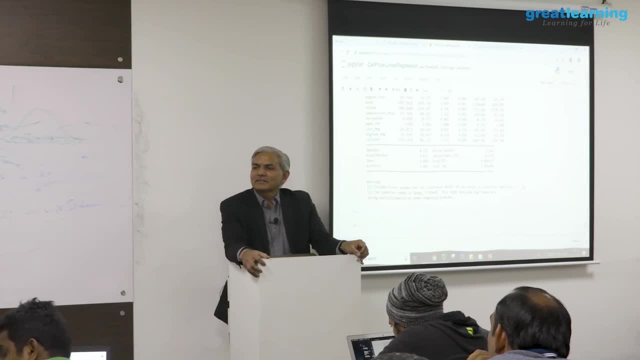 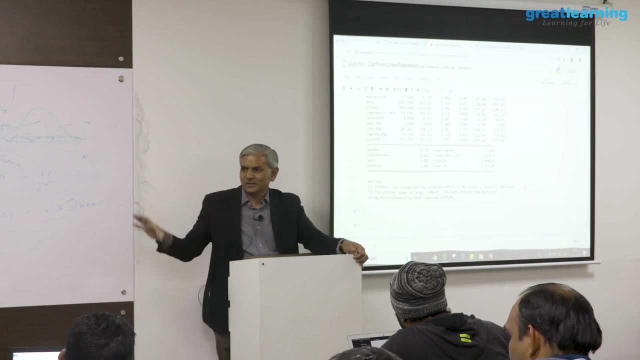 Ensemble techniques and all these techniques are available with us, So we use that technique. Use decision tree regression. That will list out for you the dimension. as you will see now after lunch, It will list out for you dimensions in terms of importance. 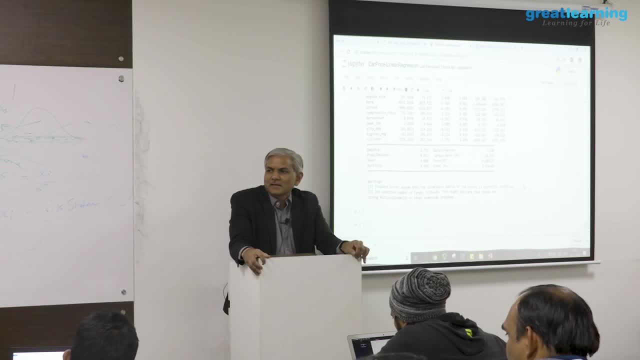 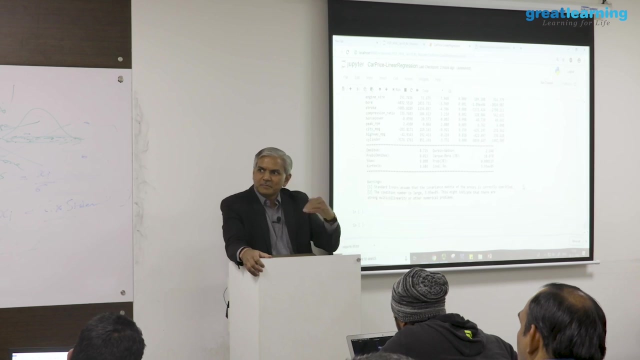 Which dimensions are more important. They use Bayesian statistics. They do not use p-values. You remember Naive Bay? You would not have done Naive Bay. You do not remember Bayesian this thing- Distributions. They use that for this. Some statisticians say that Bayesian distributions are more reliable than this. 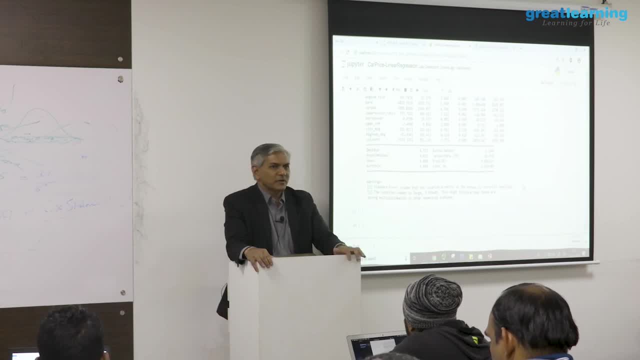 All right, sir, I am going to call it an end of the day for today, for me, For you guys. it is going to continue. We will meet tomorrow at 9 o'clock again. Yeah. 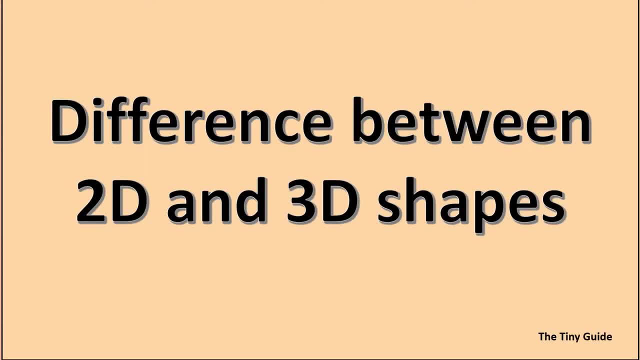 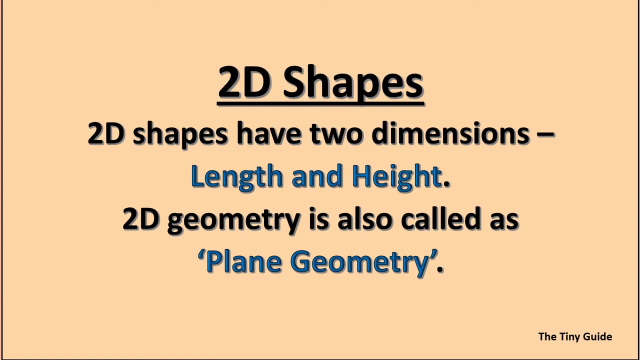 Welcome to our channel, The Tiny Guide. Today we will see about the difference between 2D and 3D. It is really interesting because we see these shapes in our daily lives. First, we will see about 2D shapes. 2D shapes have two dimensions: length and height. 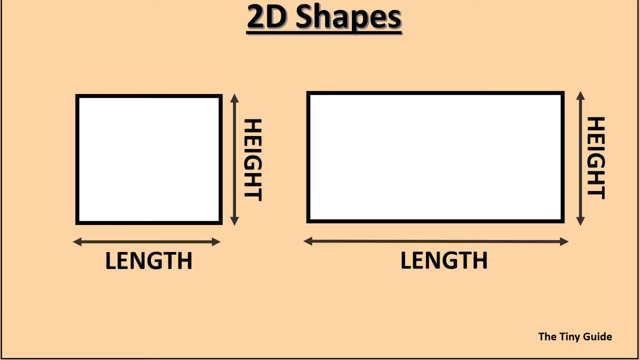 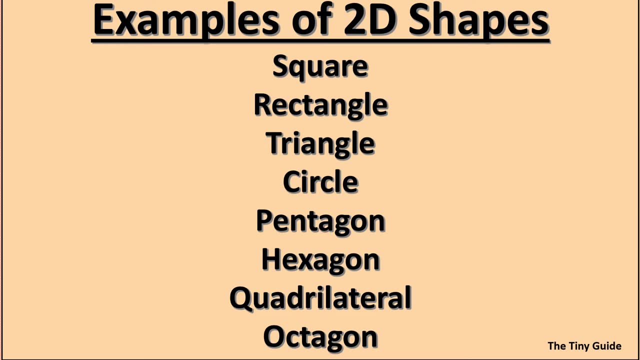 2D geometry is also called as plain geometry. Now we will see how to identify 2D shapes. These shapes have only length and height, as shown in the video. Examples of 2D shapes are square, rectangle, circle, pentagon, hexagon, quadrilateral, octagon. 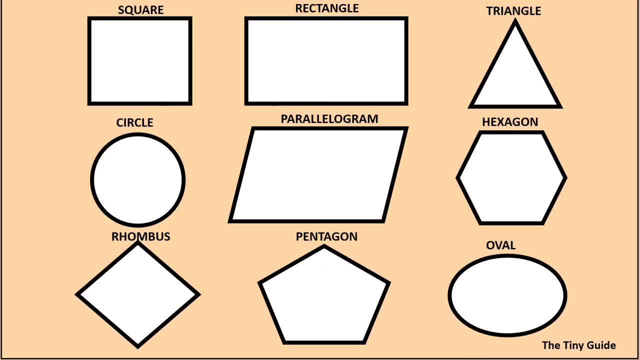 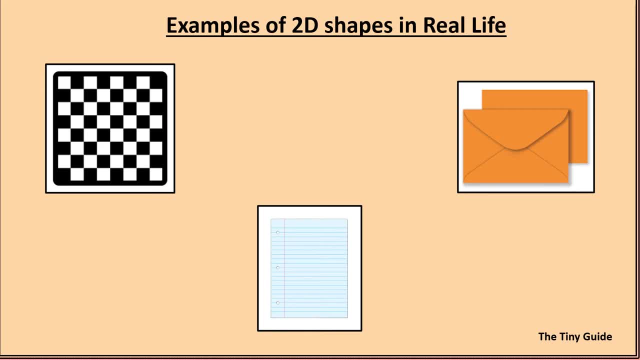 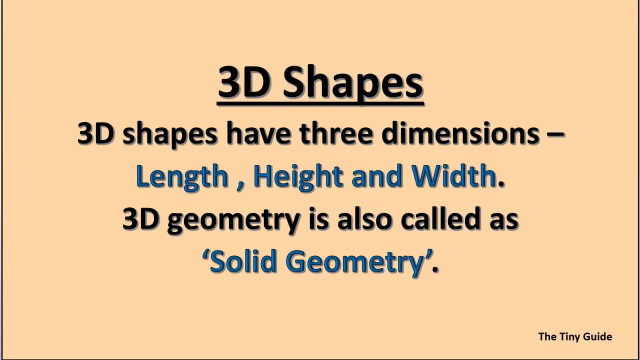 All these shapes have only length and height. These shapes are shown in the video. Some examples of 2D shapes in real life are chessboard, envelopes, paper, etc. Next we will move to 3D shapes. 3D shapes have three dimensions: length, height and width.